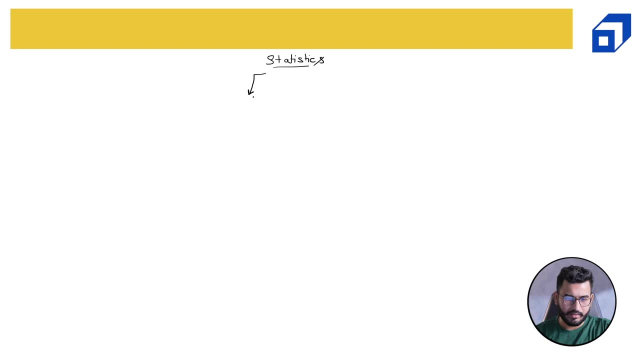 you can just adjust your speed about this video as you like. So statistics: the very first category is descriptive statistics. Then we have inferential and finally hypothesis. we'll be looking at all these three segments in a very detailed way, But let's start by understanding a little bit about each of these categories. So we 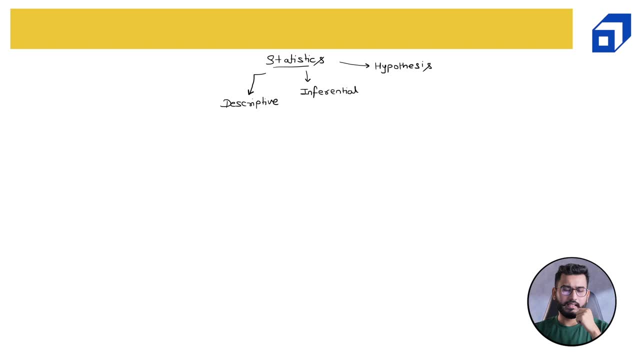 will briefly talk about what is descriptive statistics, what is inferential statistics, what is inferential and what is hypothesis? let's first take some random data. let's say we have this kind of data. so we have the data of, let's say, few students with their student id. 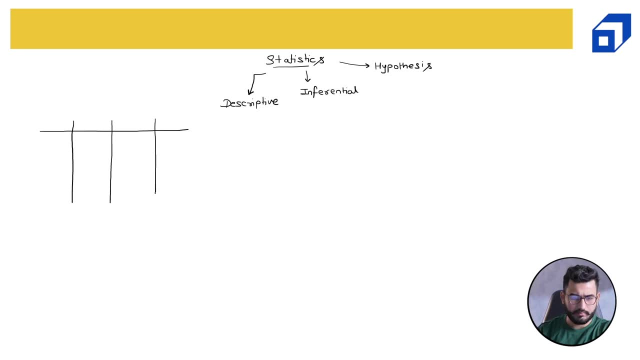 the name of the student, their marks and let's say their age and from which city they belong to. so for a student id i'll just write s id, then name, marks, age and city. and let's say we have few data points. let's fill this tables with some random data, so 0, 1, 0, 2, 0, 3 and so on till zero. let's say we have 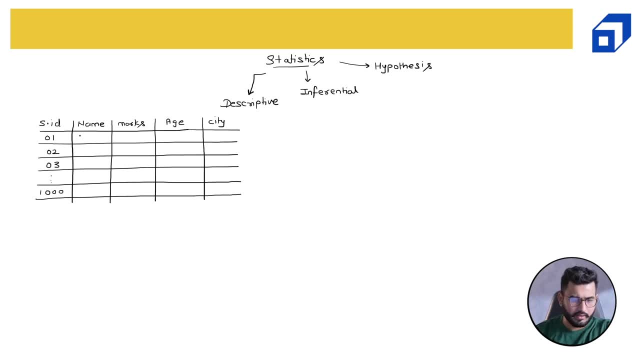 some thousand students. so one thousand name is, let's say sumit, um, maybe ravi, sanju and ankita. then we have marks. let's say one one hundred ninety five, 82, maybe this is 60.. then age: let's say 29, 28, 25 and 30. city, so i am from kanpur. 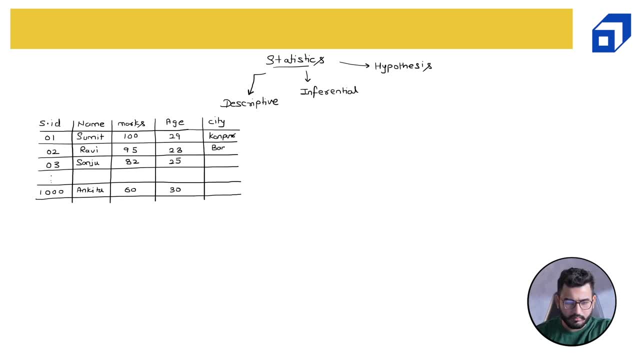 then ravi, maybe from bangalore, then maybe this is chennai and finally ankita from, let's say, jamshedpur. so we can just try it: jamshedpur. okay, now, given this particular data, we have to understand this data. so if your manager, or maybe, let's say, the principal of a particular school, is asking you to summarize, 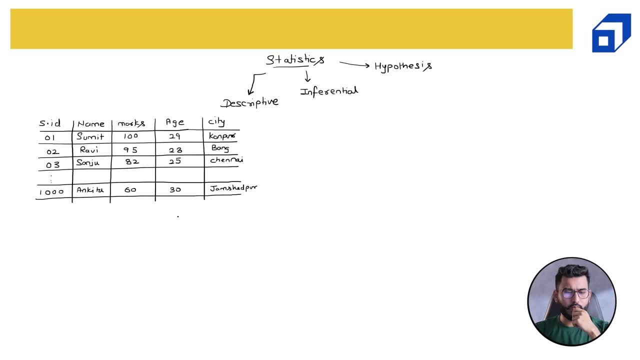 this data. now you will not be able to provide the information regarding each student right, so you will not be going to your principal or maybe the head of the school tool to explain the person that, okay, we have Sumit, we have Ravi, we have Sanju, we have. 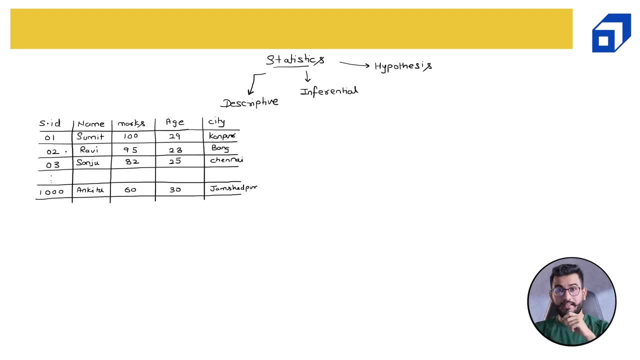 Ankita, the marks of Sumit is 100,, the marks of Ravi is 95,, the marks of Sanju is 82. It will take a lot of time and it is also not feasible, and the head of the school will not. 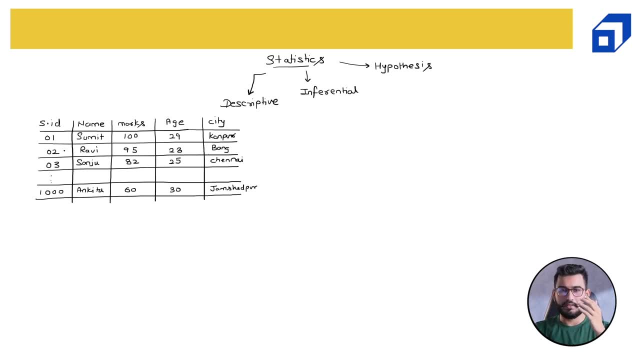 be having this much time to listen to all your information. So what he or she is looking for, He or she is looking for some information that can fully describe the complete class. So what is the metric that we can use to consolidate or to better describe the complete class is? 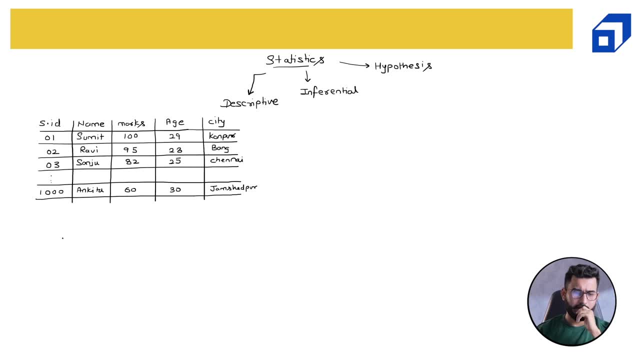 what descriptive statistics is. For example, I can say that this particular class is having number of students and, as let's say, thousand. Now, this is a statistic which is describing the class and hence descriptive statistic. Let's say, the average marks of this class is 85. Again, this number just 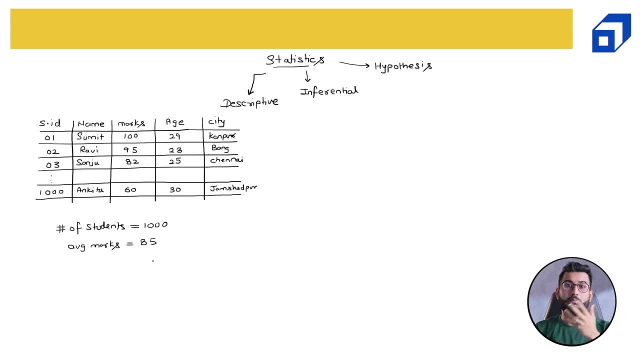 this one number is describing the complete class, and we will be talking more about what average is, But this number is talking about the complete class and hence this is a descriptive statistic. For example, let's say the average age is. let's say, let's say 25.. Similarly, maximum marks. then we have 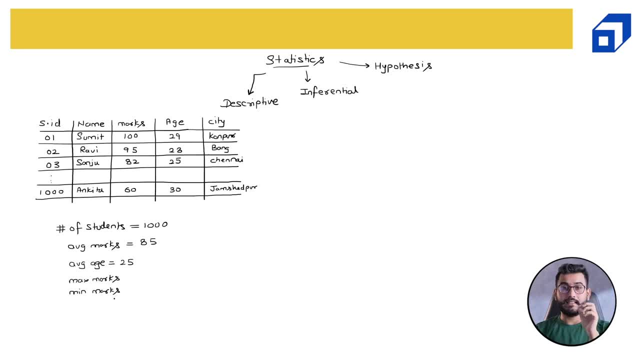 minimum marks. So all these numbers which describe the data in such a way that we could away that we just need this number to explain the complete data points, is basically known as your descriptive statistics. It's very simple to understand. right Now we have descriptive 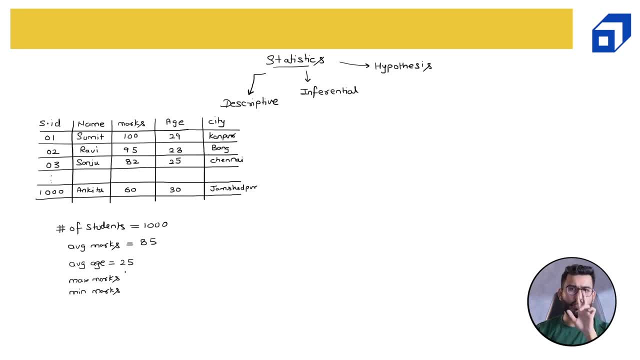 statistics can broadly be classified into two kinds of measure. So I'll just change my color and we'll write over here. So one is known as measures of central tendency, And then we have measures of variance, or you can say it is measures of variation. So I'll 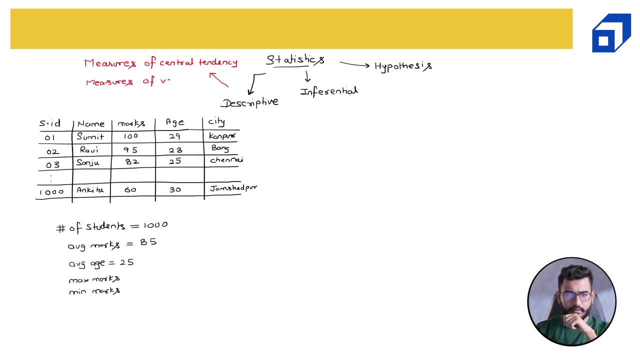 just simply write it as measures of variation. Okay, So we will be talking in detail about what are the various measures of central tendency is and what are the measures of variation. is So what we have learned regarding the descriptive statistics? it's basically those metric, So those metrics that can define the complete data. 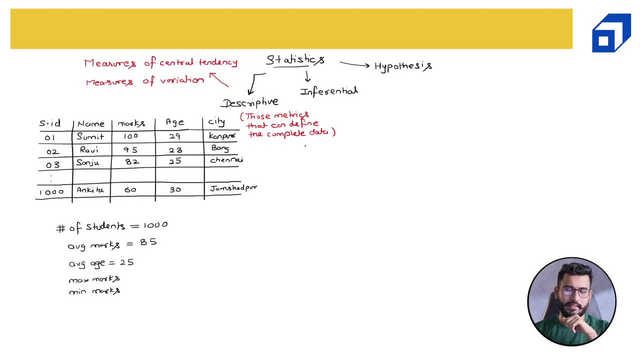 Or that can help us define the complete data. We do not need to look into each and every row. We do not need to look into each and every information. Remember, in a particular data, which is cross sectional, having rows and columns, each row is known as The information. So, using the power of descriptive, 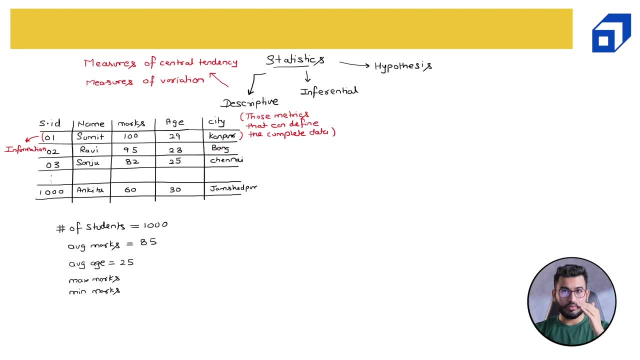 statistics. We do not have to go through each and every information. we can just use these metric to describe the complete data. right then, we have inferential. now how we can understand inferential. so i'll just quickly change the color and we'll take one example. let's say that is company. let's take any name. 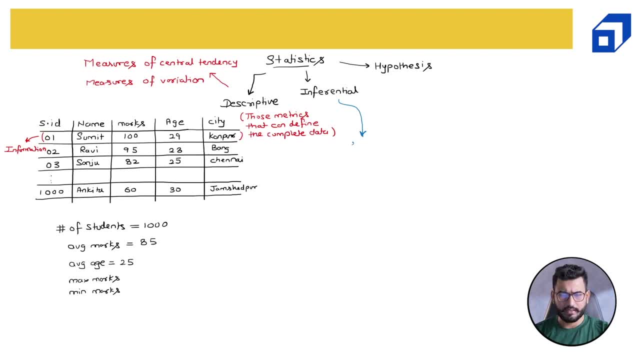 of the company. let's say there is a company known as scalar. now scalar wants to know, on an average, how many hours a student is studying in 12th class. so what's the question? how many hours a student, a student studies when the student is in 12th class. so i'll just write in bracket 12th class. 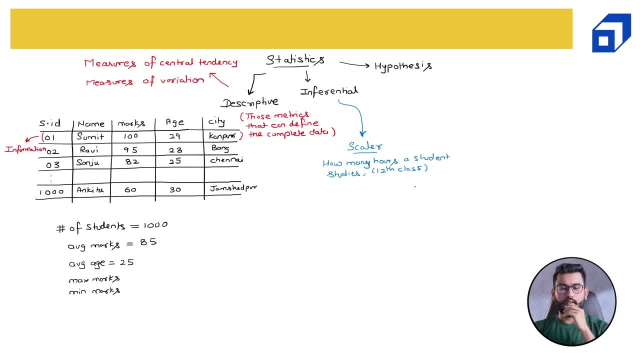 okay now, if i look into this problem overall, there will be millions of students in india, right, and if i just limit my scope of study to india itself, so there will be a lot of students that will be present in india right now, those who will be in 12th class right now, right, and it is impossible for any company to perform. 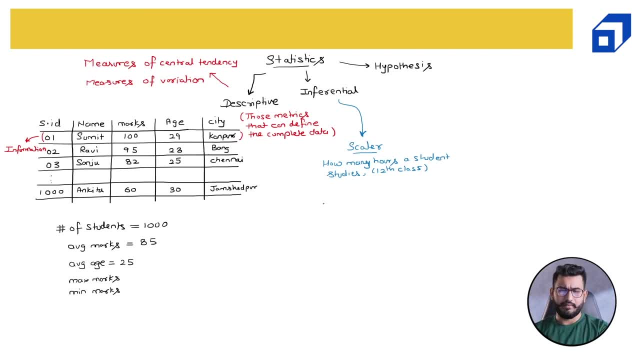 survey in scale. so let's say, if, if scalar has to get this number, a scalar has to basically get a average number. so I'll just write: average, how many averages so how many? or maybe just simply write it as: what's the average number of hours, so what's the average number of. 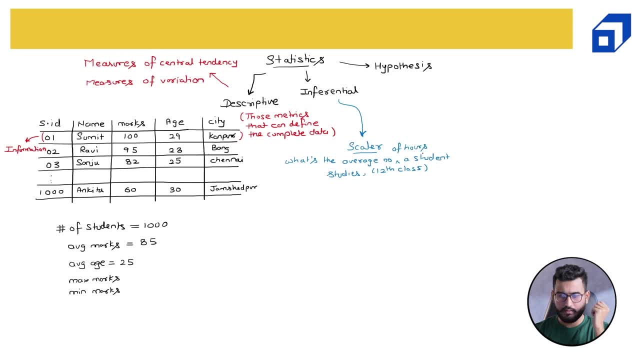 of hours a student studies in 12th class in order to find this answer, how we will take the procedure of how we will take the approach. so let's say this is my complete population population, all the students who are in 12th class this year. so 12th class students. 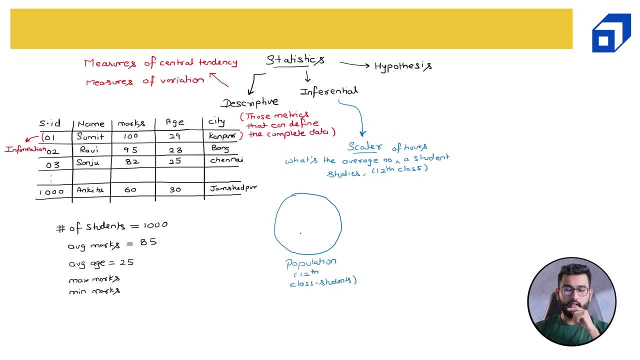 now there will be so many students, right? or if I just have to take a number, let's take: there are 100 million students. I'm just throwing a number, so 100 million students. in order to get this statistic, which is what's the average number of hours, I have to reach out to each and every. 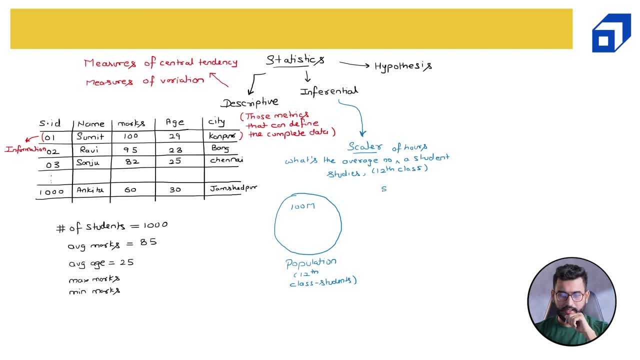 student. so let's say the entity scalar is performing this survey. they will reach out to each and every student. they will ask the student whether the particular student studies for one hour, two hour, three hour, four hour or maybe n hours. then we will collect the data, the scalar team will collect the data and the scalar team will collect the data. 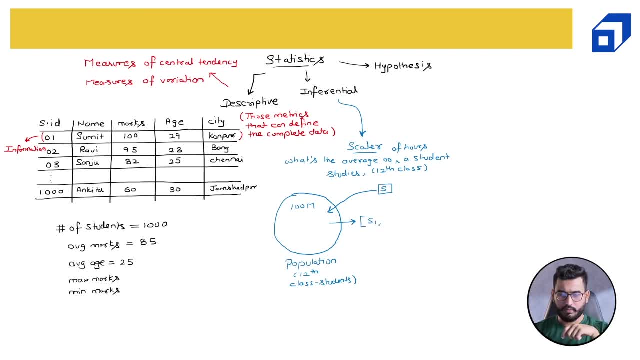 will collect the data. so let's say we have the data of a student number one, student number two, student number three and so on till student number 100 million. now, once we have this data, we will take the average and that is basically my output that i'm looking for. 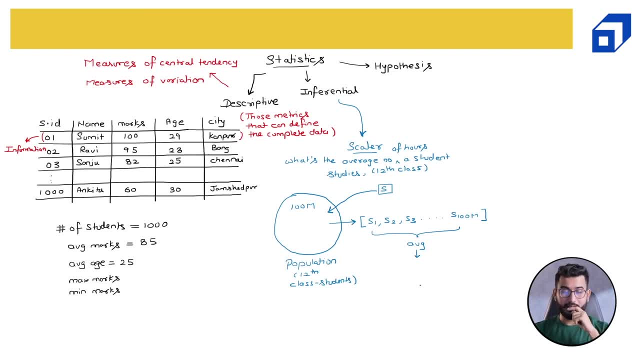 now, if we practically look into this procedure or into this problem, seems like this is practically impossible, because it is practically impossible for any company or individual to reach out to these many people or to reach out to these many observations, or entities or individuals- you can call it any anything right. if even it is possible, it requires a lot of time and lot of money, lot of. 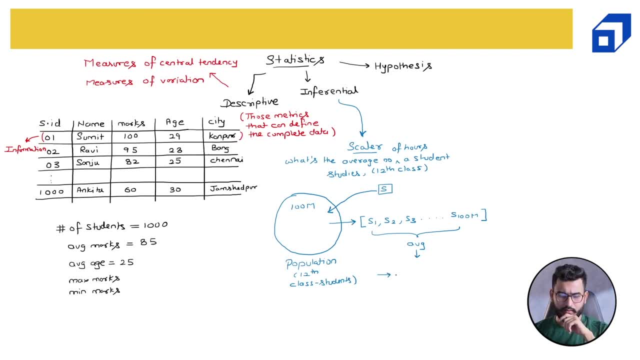 investment. so what are the practical problems? number one: a lot of investment, a lot of time investment. similarly, a lot of cost investment, a lot of lot of cost investment. so we have to invest a lot of things and none of the companies having this much time. so what is the practical solution for this? well, the practical solution is very simple. 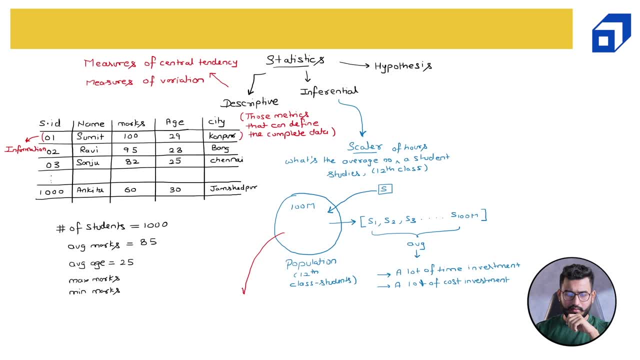 what we are going to do. we are going to take some, some few students, which we call as the sample, and we will also talk about how the sampling is performed. when we will be discussing about inferential statistics, we'll be talking about how sampling is performed. so let's say we are having a simple, random sample and the term simple. 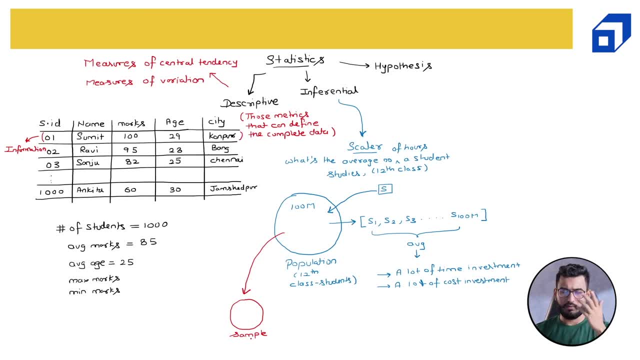 random sample will be. i'll be explaining you in a better way, so don't worry. so let's say we are having a sample. i have taken some random students. let's say we have taken 100 students from Uttar Pradesh. we have taken 100 from, let's say, Andhra Pradesh, 100 from Tamil Nadu, 100. 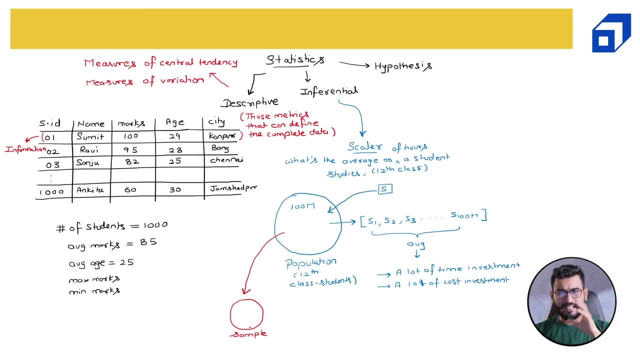 100 from Delhi NCR region. so, like this, we have created a sample and let's say this sample is having around one lakh student, one lakh now, in order to perform survey on one lakh people. it seems quite, quite practical, right, we can perform the survey on one lakh people. so let's say: 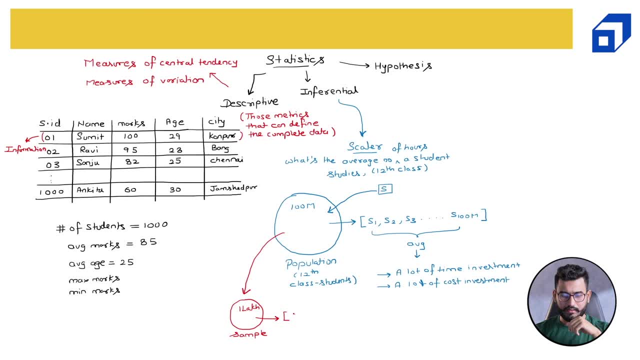 after performing the survey on one lakh people, we have the data with us: s1, s2 and so on, this till s1 lakh and now we can take the average. once we have the average. this is known as the sample average. so i'll just write: mu mu is a greek letter. 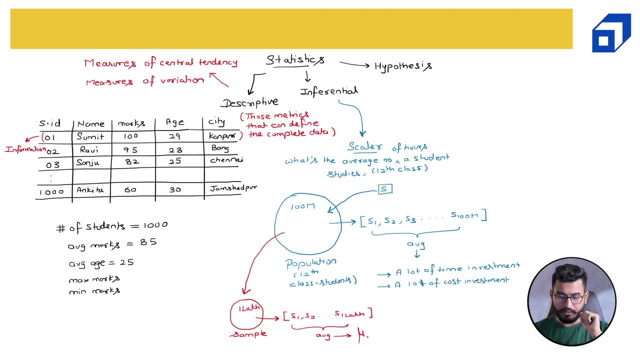 used to represent average, So average. then I'll write S sample average. I'll just write it in brackets also sample average. Now, inferential statistics is a branch of statistics which deals with approximating the population average or population parameter. Remember one thing: if I am talking about the average of population, it is population parameter. If I am talking 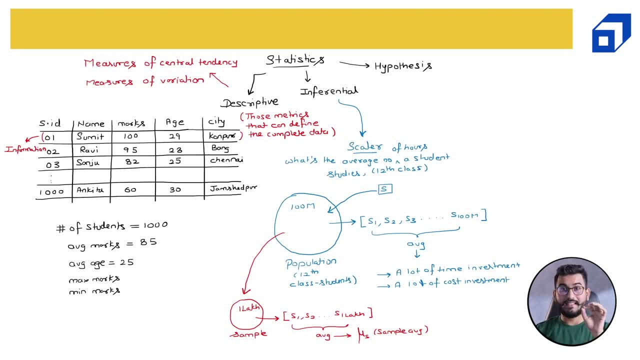 about the average of sample. it is sample is statistic, So there is a difference. So please remember when I'm when I'm saying a statistic, I'm basically talking about sample, because practically it is impossible to do anything on population. There are two problems either. 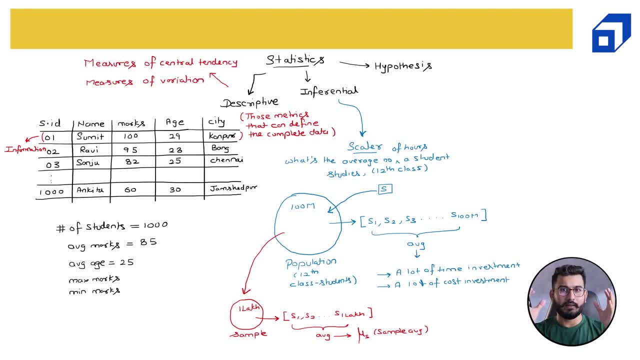 we are not able to reach out to all the observations in the population. So if I ask you, find out the average of average height of Indian men, Now it is impossible for any individual to reach out to each and every Indian male Right. So that's basically. 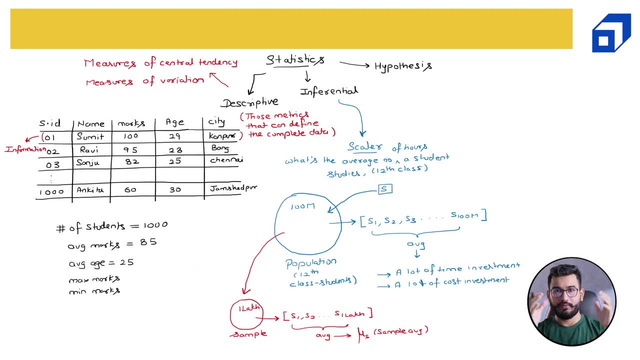 my population And if I can get that number, if I can get the average age of all the Indians in this, all all Indian males from India, then that is known as the population parameter. OK, So in financial statistics, coming to our point, inferentially, statistics is a branch. 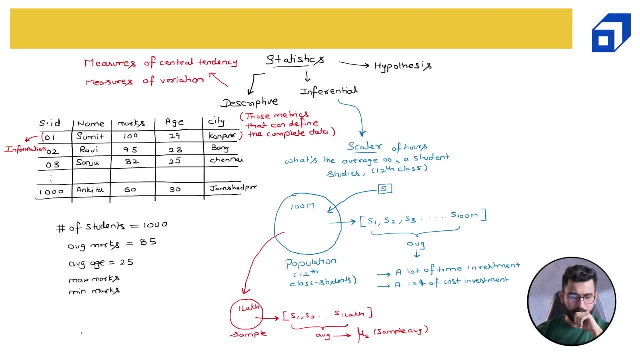 of a statistic which helps us to perform approximations. So using this sample statistic, I will try to approximate the population parameter. So let me just quickly write it over here: using statistic, we will try to approximate the population parameter, and that is basically known as the inferential statistic. Now there are some procedures. we have some few formulas. 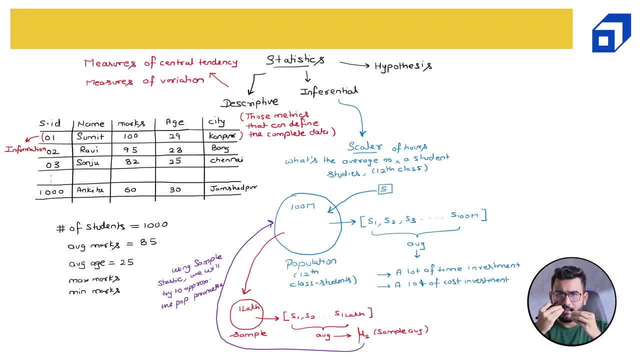 we will be talking about that, but this is basically the belief idea behind why we need inferential statistic, The last portion, or maybe the last segment, which is known as the hypothesis testing. When we talk about hypothesis testing, as the name suggests, we are trying to test something. Now, what we are trying to test? We are trying to test something which. 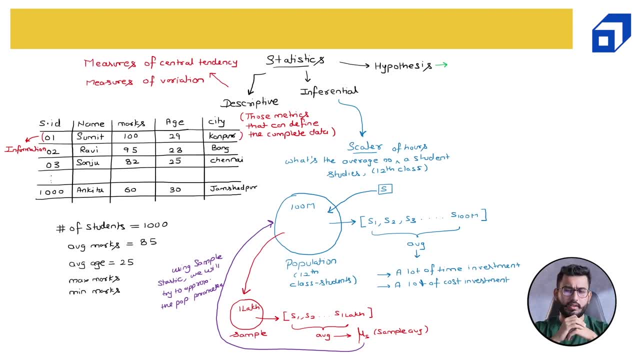 has been tested. We are trying to test something which has been tested. We are trying to test something which has been proven, or maybe a claim, or maybe an statement. There can be anything that we are trying to test. Let's take one very general example. So you guys, 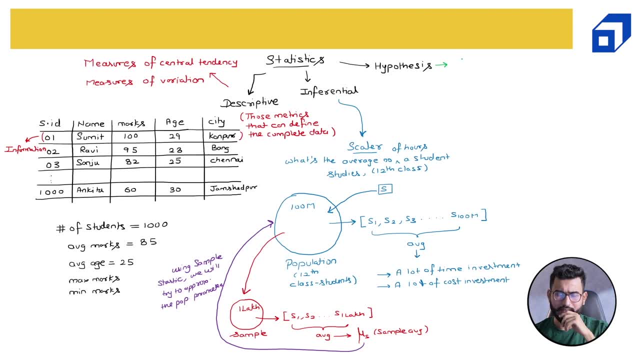 would have watched this Dettol advertisement which says that Dettol kills 99.9% of the population. Now let's say you are suspicious about it. You are suspicious, You wanted to test whether this claim or statement made by the Dettol company is it having some statistical 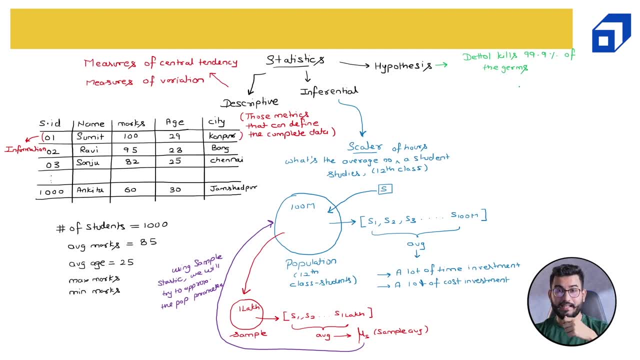 significance or not, Is it statistically correct or not, And that is where the power of hypothesis testing comes into picture. So we will try to test here. We perform test to check if a particular claim or statement can be statistically proven. Can be. 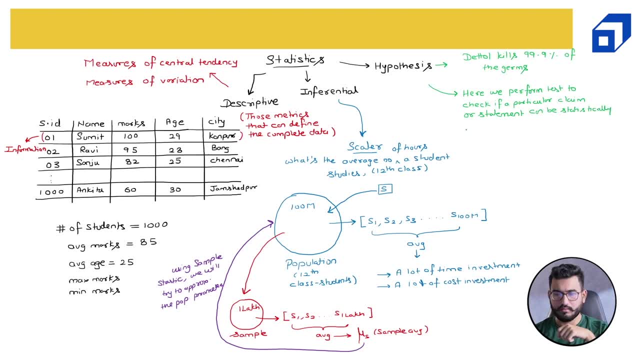 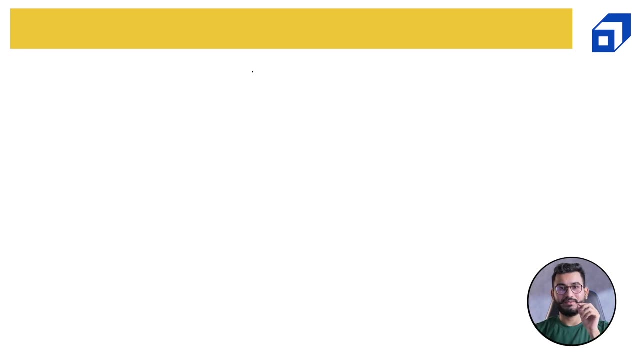 Statistically proven. So these are the three major segments which we are going to discuss Now. before we jump into any of these segments, we have to understand what kind of data we are working with. So we'll be briefly talking about how we can explain a data, And when. 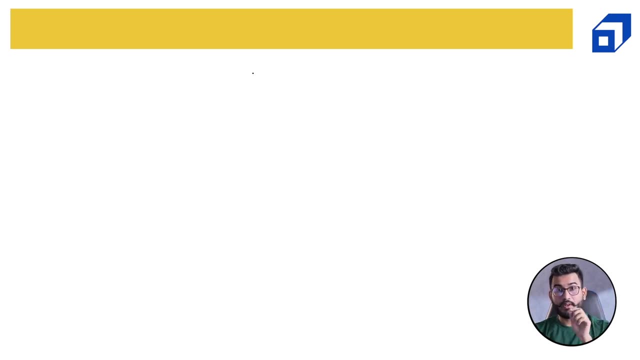 I say: explain a data. what are the various types of costs, What are the types of columns or variables we get in a data? So let's talk about it. We will be taking one very random example, So let's just quickly create a data Again. 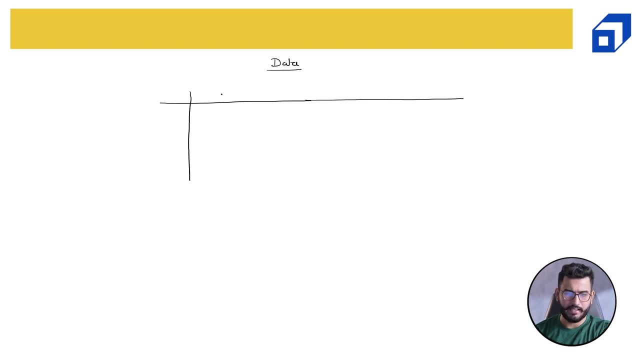 we can extend the same example that we have taken in the last slide. We were having a student ID, The name of the student, Salary, Age, Or instead of salary let's put marks: Age, Then city, Then we can go. 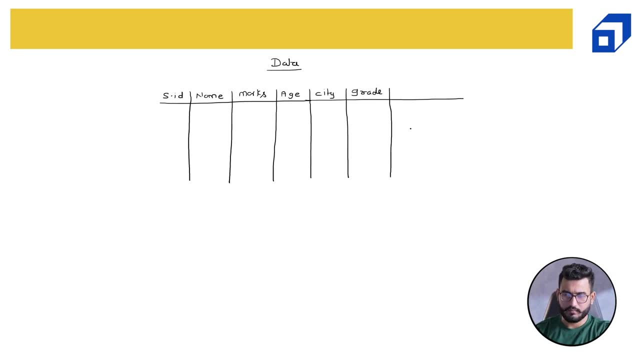 about writing grades And maybe subject, And finally we can talk about the gender. Let's fill this table with some few data points. So let's say we have 01, 02, 03, 04.. Name is Sumit Amit. 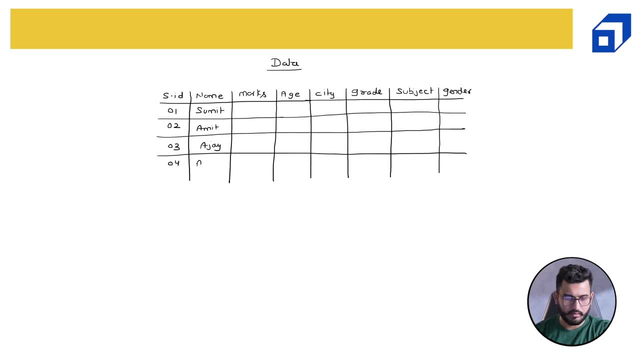 Okay, Ajay Ankita Marks is, let's say, 89,, 98,, 95, and 62. Age is 29,, 28,, 25, and 30. City is, let's say, K and P, B and G. 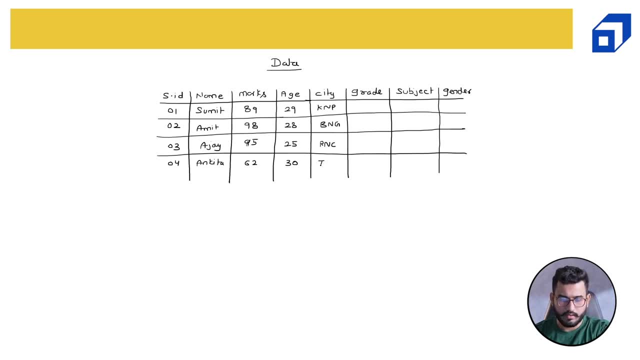 R and C And let's say TA, TA, Then grades A, B, C and B Subjects. So let's use S1 as subject number 1, S2, S1, S3.. Gender: Male male- male female. Now, this is my dummy data. 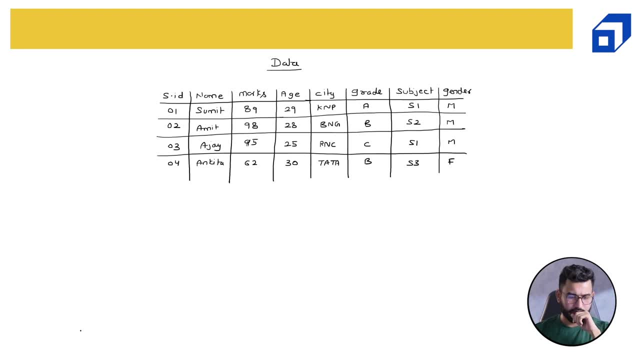 Now, if I ask you, are you guys able to observe any kind of distinction among all the kind of variables that we are having in this data? So remember, these are. these columns are also known as: So these columns are also known as the variables. So I mean I may be using 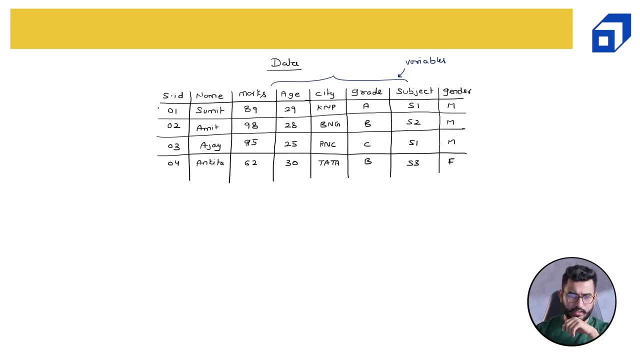 the term variables or columns, But I'm not going to be using the term variables or columns. I'm going to be using the term variables or columns, But I'm not going to be using the term variables or columns. And, as I have told you that each row is basically my group. 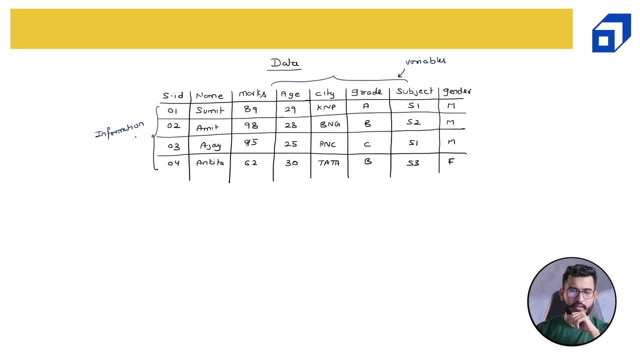 of informations, So each row is my information. Now, if I carefully observe, marks age. these two columns are my numerical columns. And why I'm calling it as numerical? Because the data which is which these columns are holding are the numbers. These numbers are something. 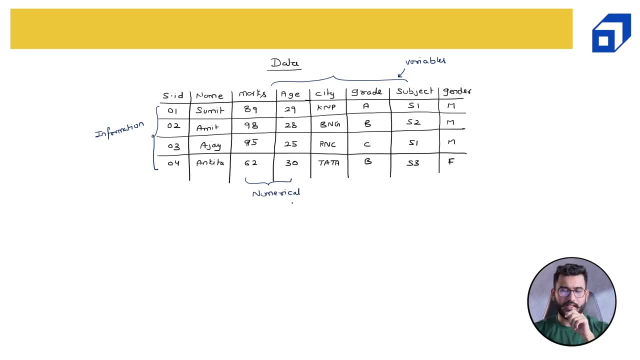 that lies between a minimum and a maximum right. So marks can be between 0 to 100.. Age can be between, let's say, since it is a school, let's take 25 to 35.. Then if I talk about city grades, subject and gender, let's say 25 to 35.. Then, if I talk about city grades, 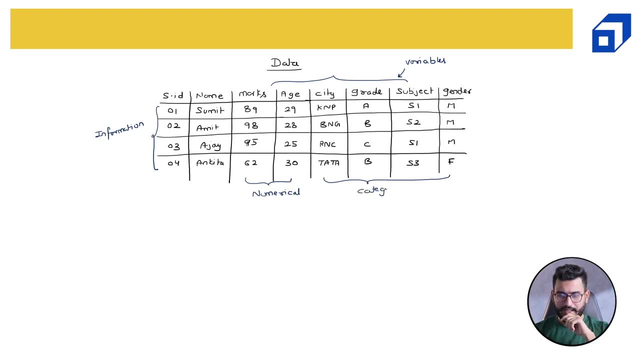 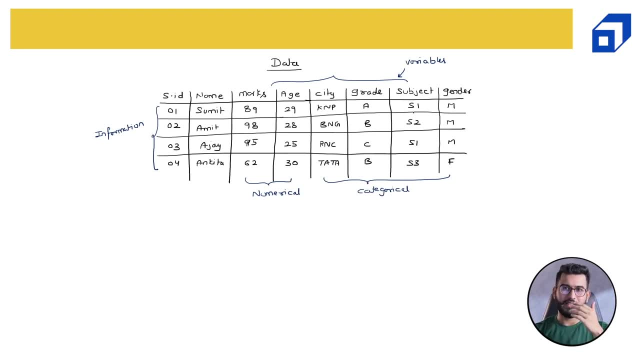 if I talk about city grades, subject and gender right, Then these categories are categories. These are all categories, right. Grades, ABCD categories, subjects S1, S2, S3 categories Gender: male, female category. Similarly, this name is a categorical column because 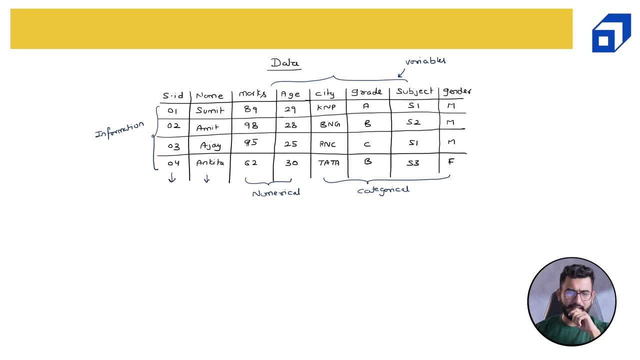 each name can be termed as a category. The student ID is a identity column. it is neither categorical nor numerical, so I can just simply call it as an identity column. Now there are like: in order to better explain these columns, we have a formal name given. 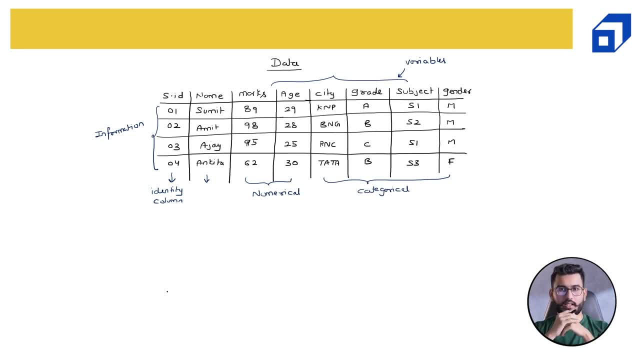 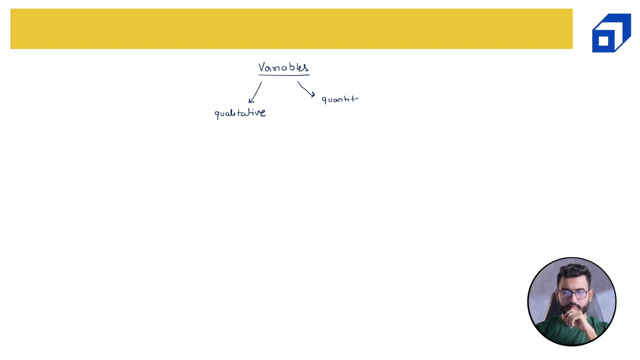 to all the numerical columns and all the categorical columns. Let's talk about it. So, when we talk about variables, it is formally divided into qualitative and quantitative. Now qualitative data is basically those columns which consist of non numerical data. So columns Which consist of non numerical data. 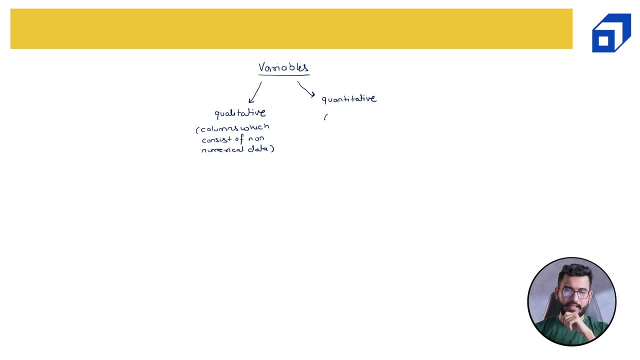 That's basically my qualitative data. Quantitative data is those columns which consist of numerical data. So, simply, I'll write numerical data, numerical data. Now, within qualitative, there is a further distinction, which is your nominal and ordinal. Now what is nominal? So when we talk about nominal, these are those columns which consist of categories. that does. 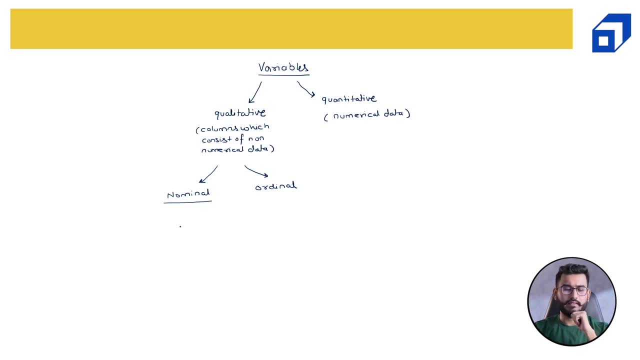 not comes with any kind of order among the categories, For example. So first take example, for example, city. let's say there is a column city, and the column is having categories as Kanpur, Delhi, and then Mumbai and Kolkata. Now I cannot say that Kanpur is better than Delhi, Mumbai is better than Kolkata, because 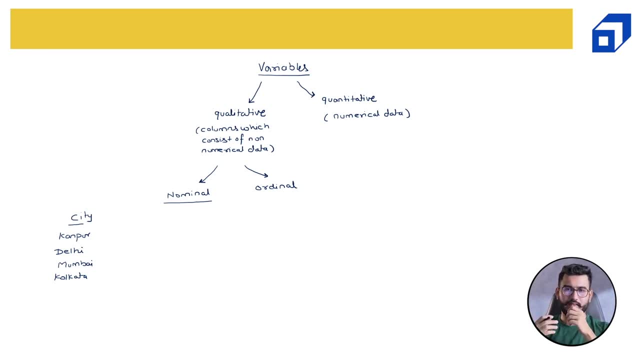 these are four distinct categories. They do not have any kind of orderness among them. So this is simply the nominal categorical variable or nominal qualitative variable. So I'll just write down the definition Categories. that does not follow Orders. Order among them are basically known as nominal data, ordinal data. 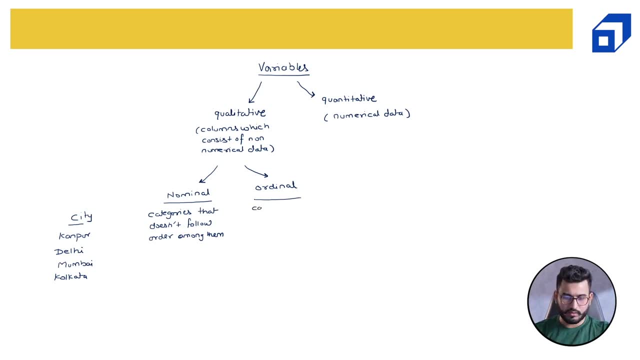 You guys would have already guessed it, It is basically those categories that follow orderness. orderness among them, for example, grades. or, for example, I will Let's say, Yeah, Great is the best example. So grades, So it, grades can be a, a, a plus. 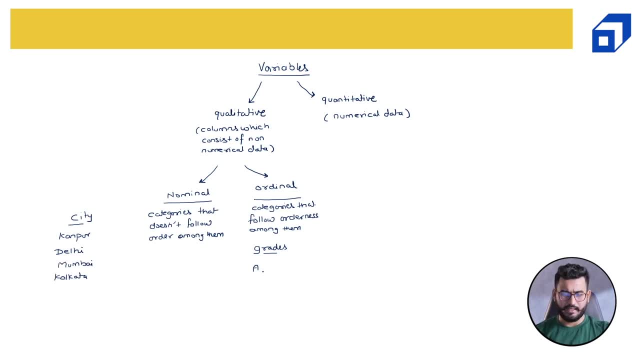 Maybe I should write a plus. first. Let's take ABCD. ABCD: Now we know that A is better than B, B is better than C, C is better than D, So there is some orderness among these categories, and that's the reason. ordinal data, we can also. 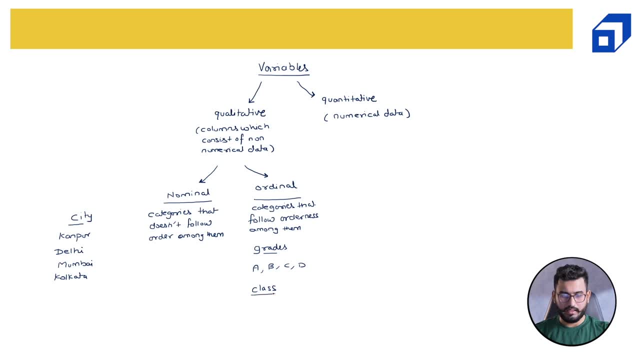 talk about class, Like first class, second class, third class, fourth class, So there is orderness. If I talk about, let's say, your educational qualification. educational qualification, So let's say a person is graduate, a person is a post graduate, a person is intermediate. 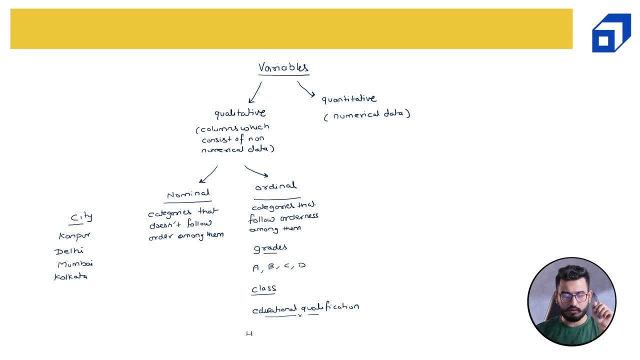 So I know that, So I know that High school, Then we can have intermediate, Then we can have graduation And then post graduation. So these are the four categories which will definitely have a order among them. So these are known as the ordinal qualitative variables. 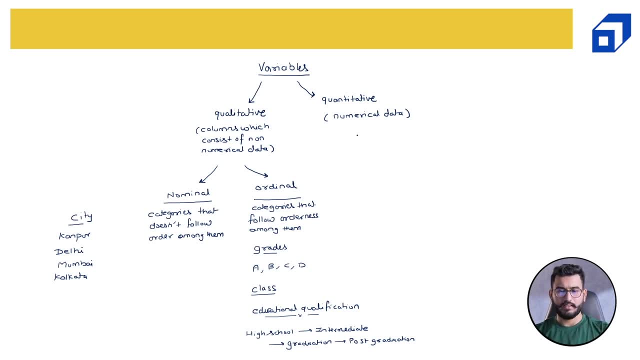 Now quantitative, As the name suggests, these are those variables which can be quantified. quantitative means quantified. we can extract some quantity out of it, For example minimum, maximum. we can perform addition, subtraction, So we can apply all those mathematical operations on these columns and after applying the mathematical 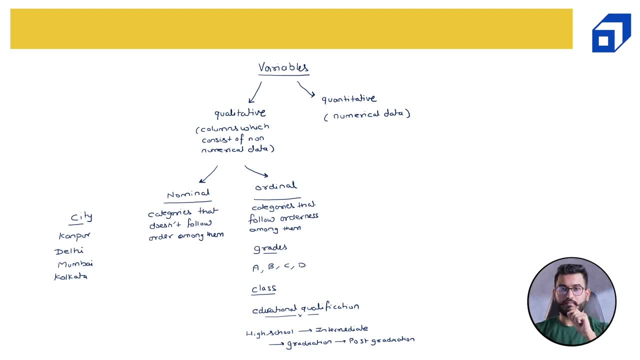 operations, The value will still make sense because they are qualitative, sorry, quantitative. Now, quantitative are further classified as number one: discrete and continuous. Now, when we talk about discrete, Now, these are those quantitative variables Which will have values That cannot take decimal values or that can only take integer or natural numbers. 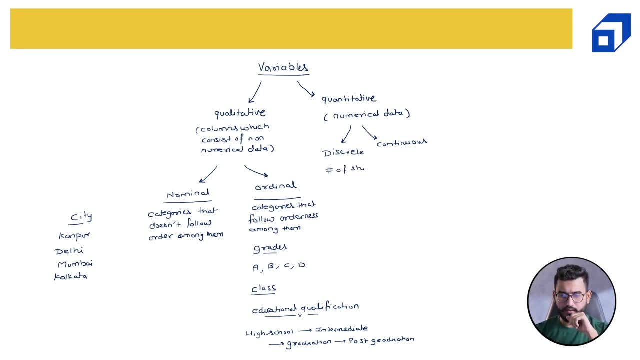 For example, number of students in a class. Now we know that a class can have two students, three students, four students, hundred students, two hundred students, but a class cannot have twenty two point five, seven, because this practically does not make any sense, right? So this is discrete quantitative variable. 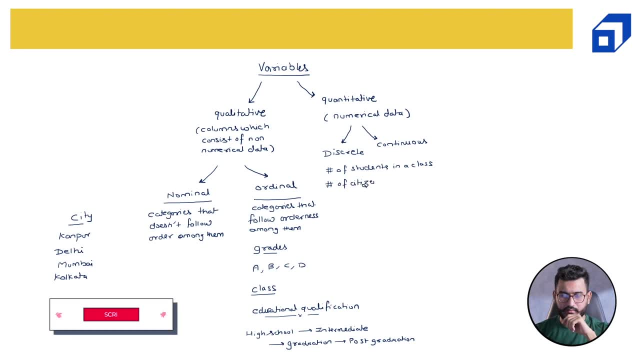 Similarly, number of Citizens in a country. Again, it will always be a natural number which is countable and finite, So I'll just quickly write it in a bracket: Countable and finite. When we talk about continuous, These Are those variables which are 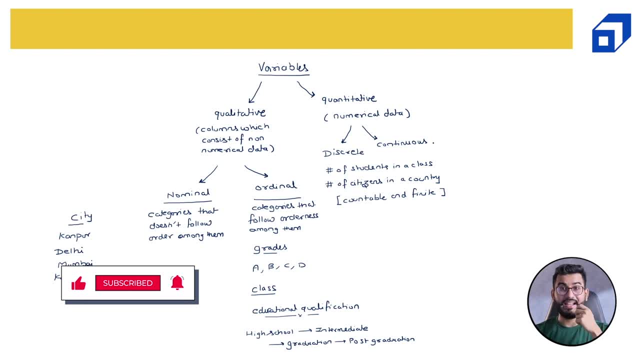 Non countable or uncountable and infinite, Uncountable And Infinite. Let's take an example and it will make better sense. For example, let's take income Now. income of a person can lie between a minimum and a maximum. 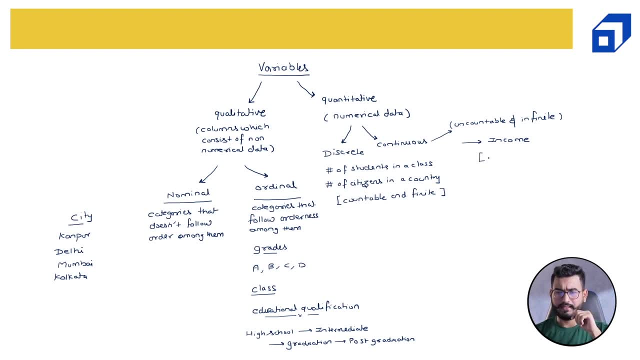 Value, For example, purpose. let's take the minimum income is hundred. The maximum income is, let's say, one million. Now, between these two numbers, I have infinite number of observations that are valid. Can a person earn? let's say hundred point one, five? 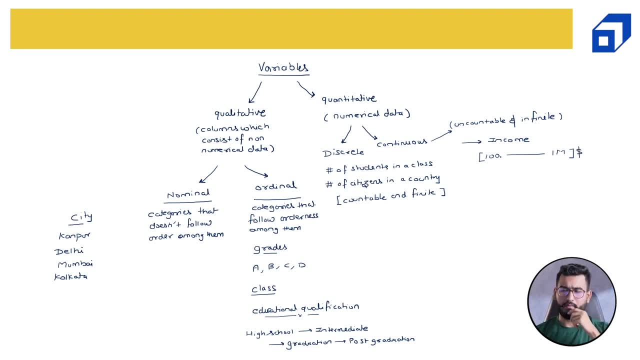 Let's say these are in dollars, So it will make more sense. So Is A person earning hundred point one, five of valid income? Yes, is a person earning, let's say one million, or Let's take a smaller value so that you guys can understand it. 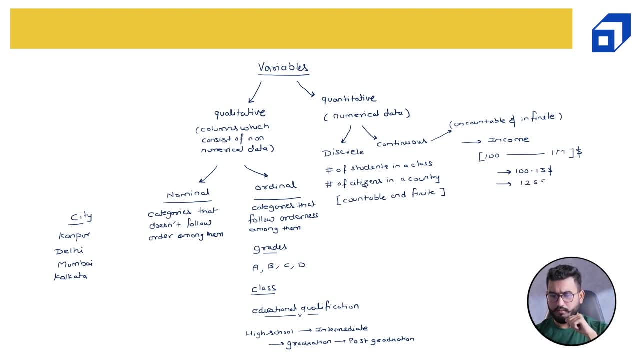 So let's say one thousand two hundred and sixty five point seven, seven, eight. I'm going very like I'm taking more decimal values just to make make you guys understand that this is also a Possible value, Which can, Which can Exist. 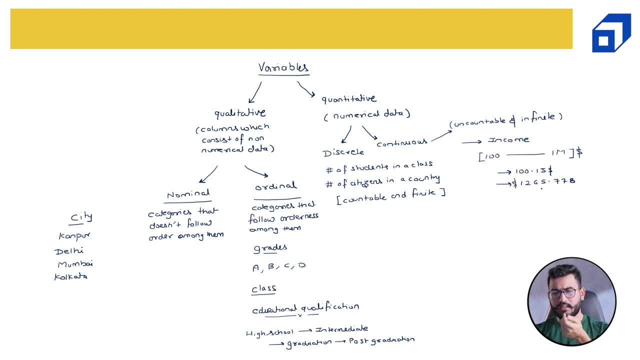 And which is practically possible. So a person can earn This number also right? So between hundred and one million, I have endless possibilities and each possibility or each observation Is possible to exist. Similarly, We have Age. Now let's say our minimum age is twenty seven. 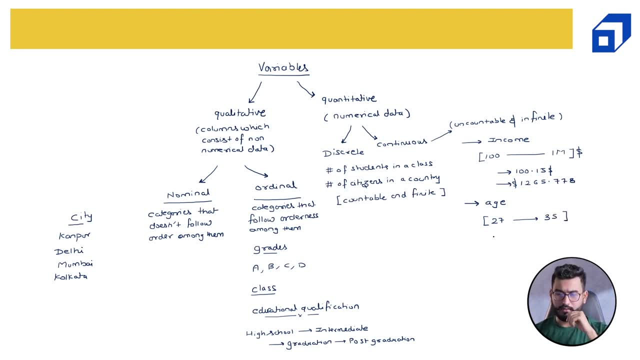 Maximum age is Thirty five. Can I have a person with the age twenty seven years, Five months, Six days, Four hours, Five seconds, Six milliseconds, Seven nanoseconds? Yes, Practically possible. So at every nanosecond I can have a particular observation that can lie in this scale. 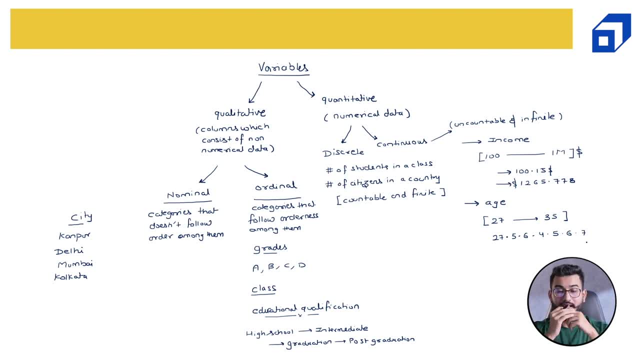 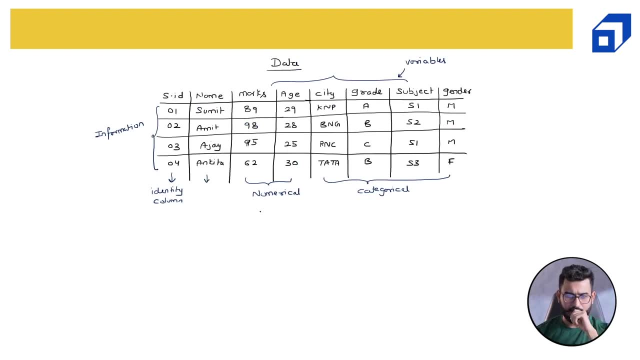 And that is the reason. age is also a continuous quantitative variable. If I go back to my example, We can see that both marks and age, They are Continuous Quantitative. Similarly, If I Look into Grades, They are qualitative. 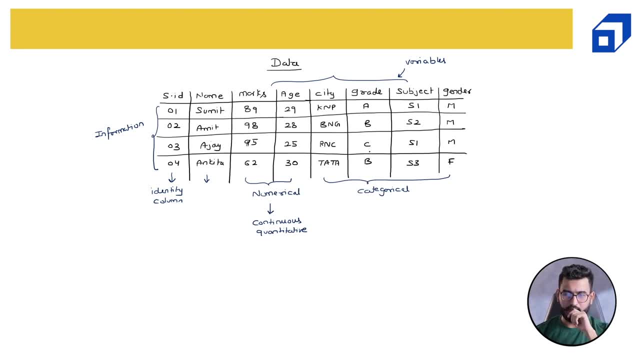 But It is Ordinal. So If I Look into Grades, They are Qualitative, But It is Ordinal, But It is Ordinal. Then Subjects, They are Qualitative, But 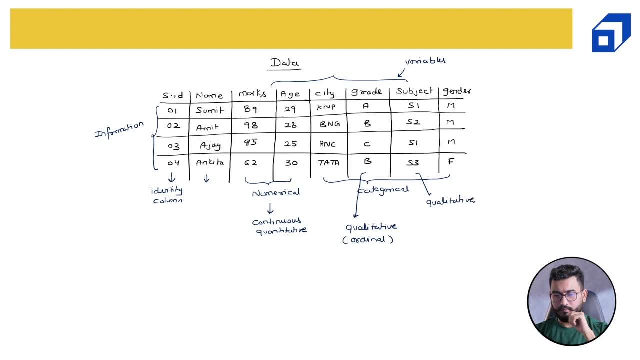 It is Nominal. Similarly, Grades Gender- Qualitative. Nominal Because I cannot say male is better than female or female is better than male. So These are two categories And it is Nominal City. 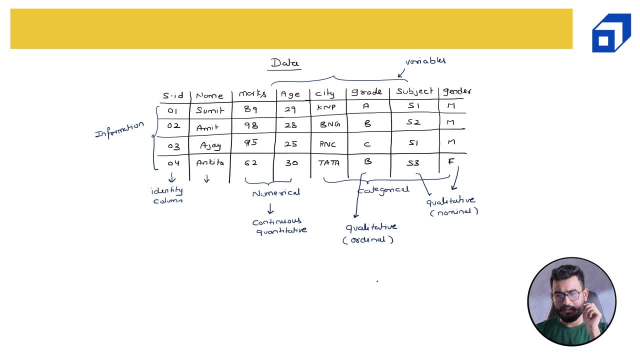 Again Qualitative Nominal, So I'll just Write Q, Hyphen N. So This Name Again Qualitative Nominal, And I Have Already Told You That. 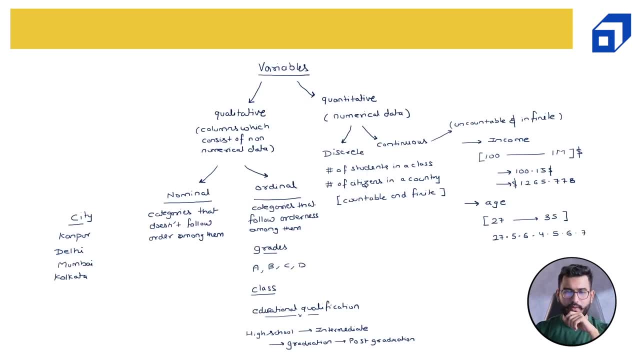 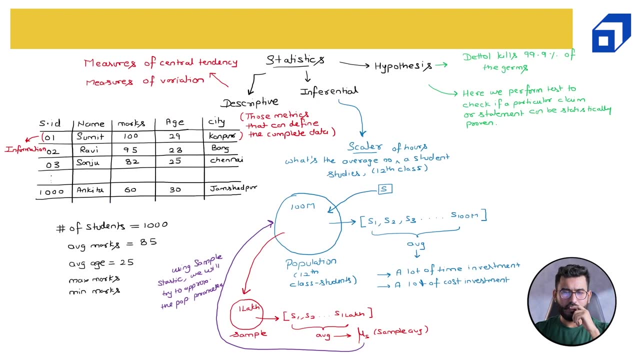 So Student ID Is Basically An Identity Column. It Is Neither Qualitative Nor Quantitative. So This Is How And What Are The Measures Of Variation? 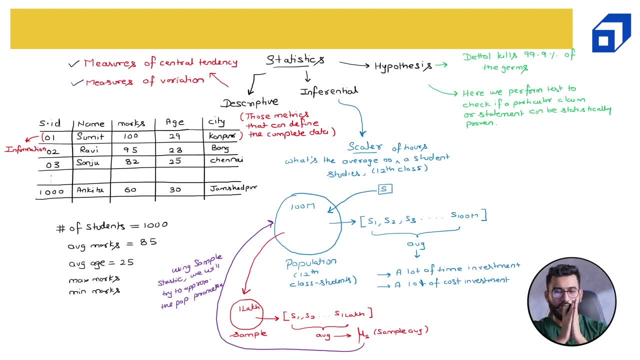 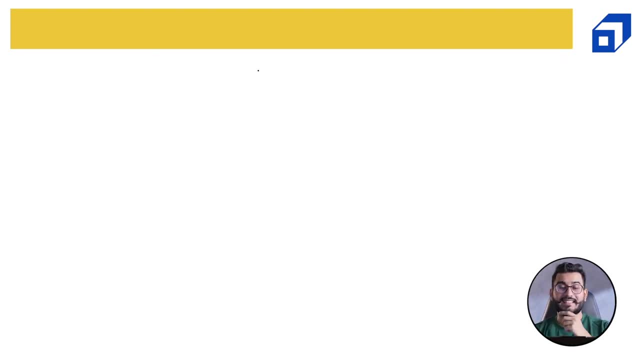 Is So With This Particular Topic We Will Initiate The First Category Or Maybe First Group Of Discussion Or First Branch Of The Data In 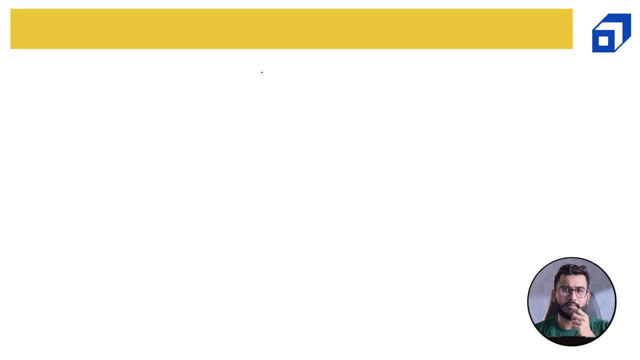 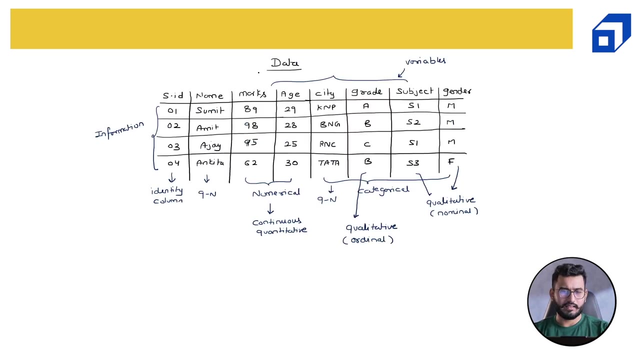 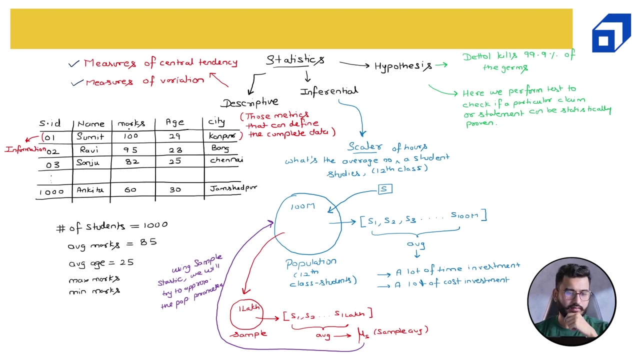 One Number Or In Few Statistics Parameters In Such A Way That It Can Describe The Complete Information. And If I Go Back To My First, 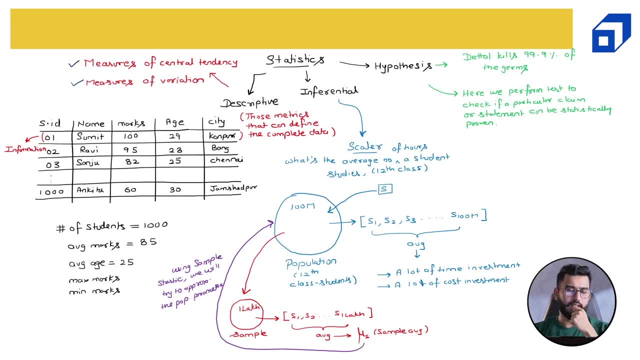 Slide Now. The Teacher Will Not Be Taking The Principle To Each And Every Row Or Each And Every Detail Of The Student, So Let's. 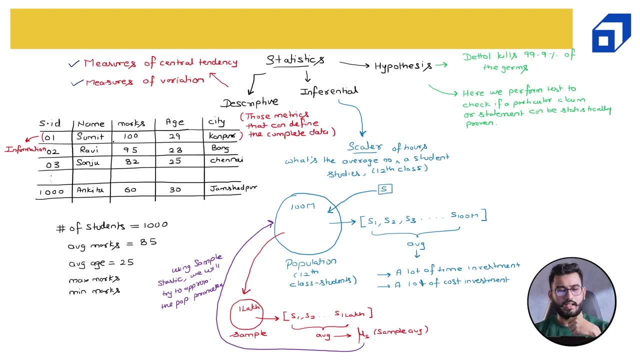 Assume That If I'm One Student Whose Name Is Ravi, Who He's From Bangalore, He's He's 28. Years Old, As You Can. 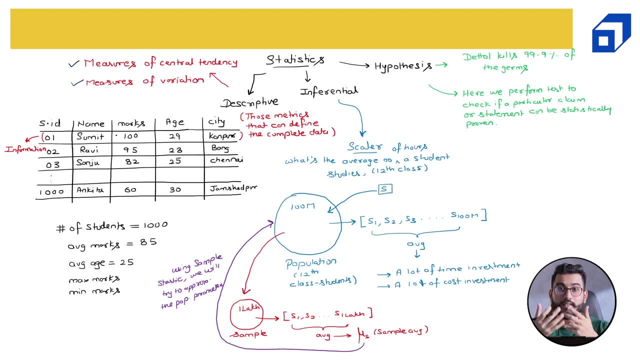 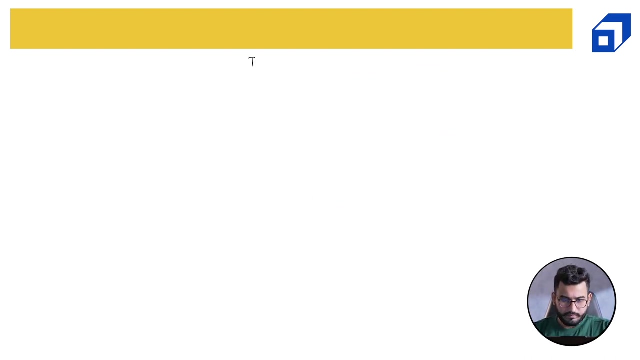 See That It Will Take A Lot Of Time, And I Would Have A Lot Of Time, So Let's Try To Now Deep Dive Into 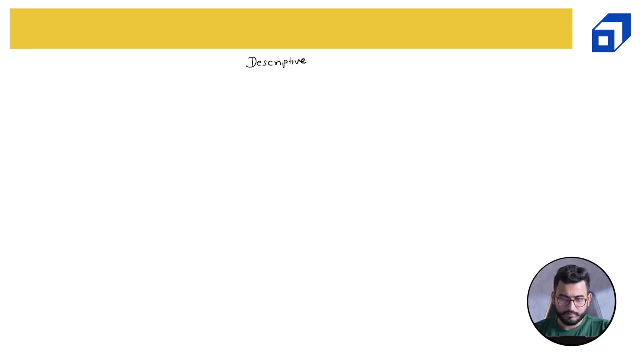 These Two Particular Topics. So Descriptive Statistics, As We Already Know That We Have Two Measures, Measures Of Central Tendency, And Then We Have 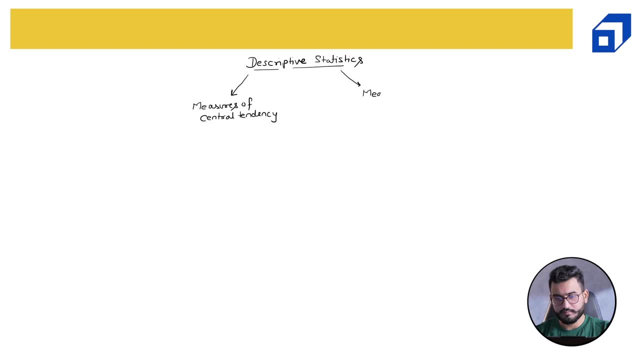 Measures Of Variation. You Can Also Say It Is Measures Of Variance Or Variation To Be, To Be In General English. We Can As You. 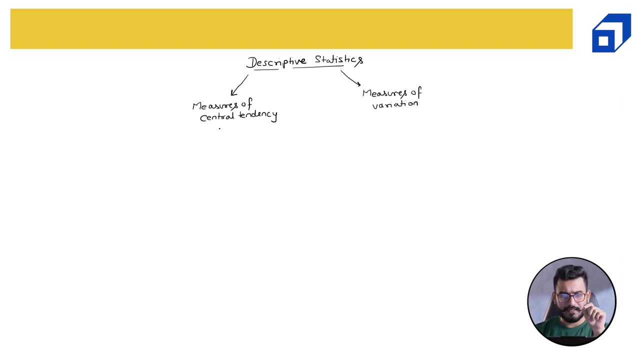 Know That If You Carefully Read The Name, It Says Measures Of Central Tendency. We Are Talking Something Regarding The Center. Now Is It The? 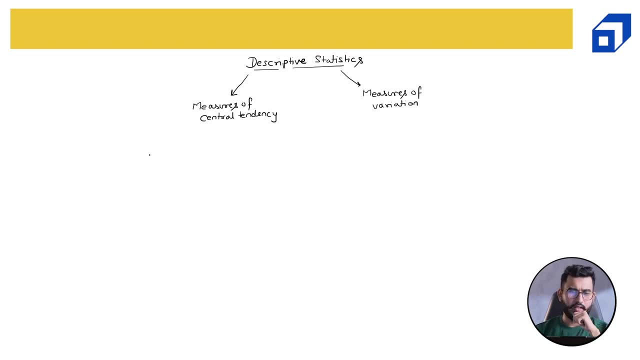 Center Of Class. So Let's Create Some Hypothetical Data Of A Class And We Have Age. So Let's Say We Have Age Of Some. 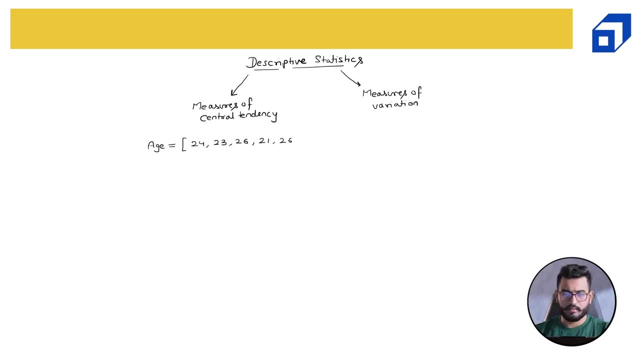 10. To 15. People, And Let Me Just One More 28.. One More 28.. Okay, Let's Make It As 26.. Then 32.. 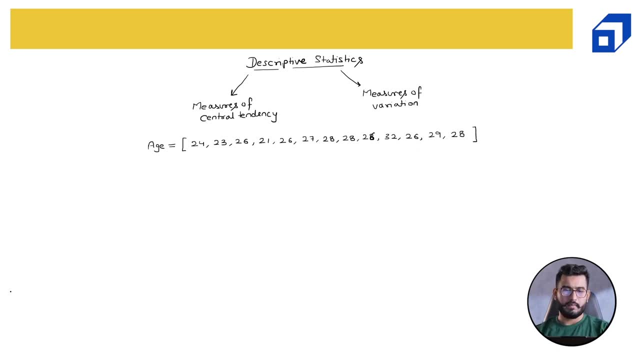 26., 29. And Finally, 28.. This Is The Data I'm Having. These Remember Each Data Point: 4., 5., 6., 7., 8.. 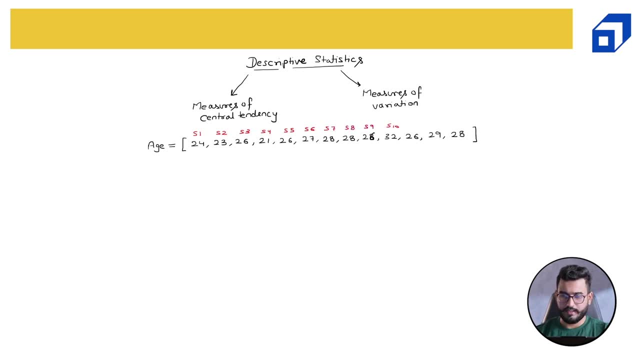 9., 10., 11., 12. And 30. So We Are, In Total, Having 13. Students In Our Class. Now How I Can Explain The. 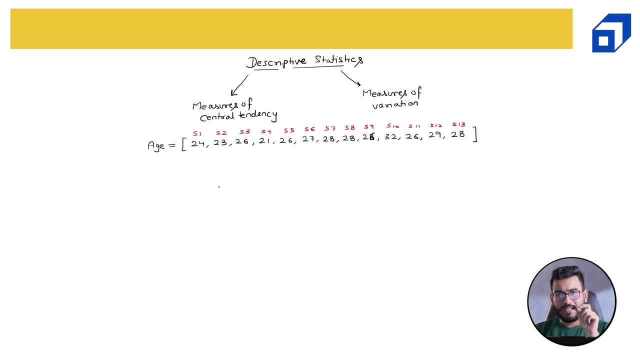 Complete Data Which Lies In The Center Of The Data, So That We Know That Below This Number. So Assume That This Pen Is The Center. 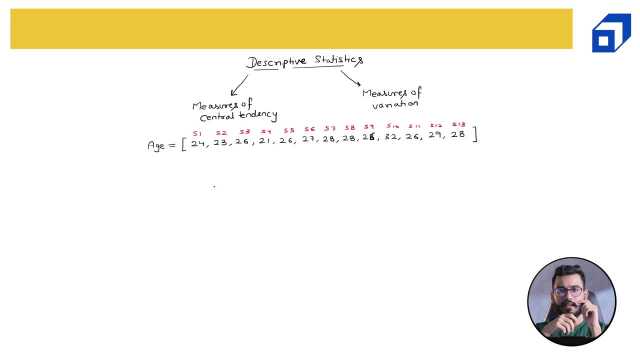 Of The Data. So I Think That This Is The Major Of Central Tendencies In This Particular Data, The Very First Major Of Central Tendency. 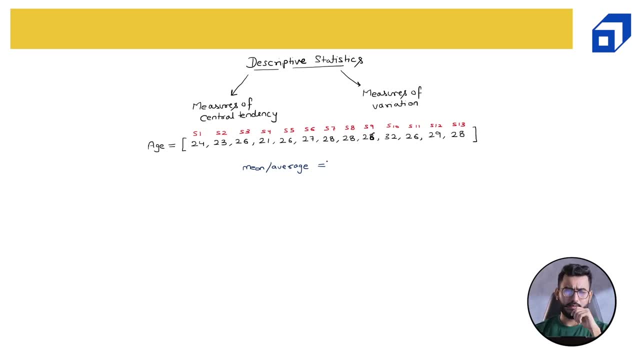 Is The Mean Or The Average And Many Of. Mathematically We Can Write Tab Summation Of So This: This Is A Greek Letter Again. 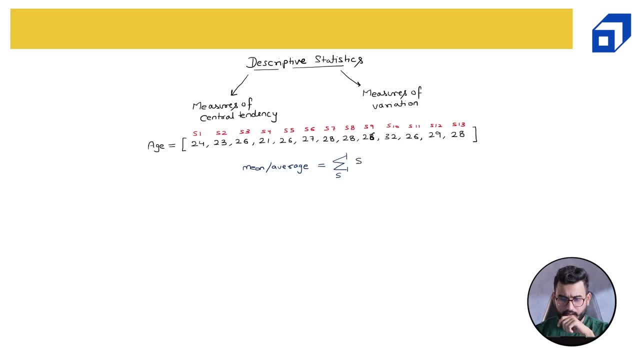 Summation. I'm Taking A Summation Over I Or, Sorry, Over S, And S Is Nothing S 3. And So On Till S 13.. 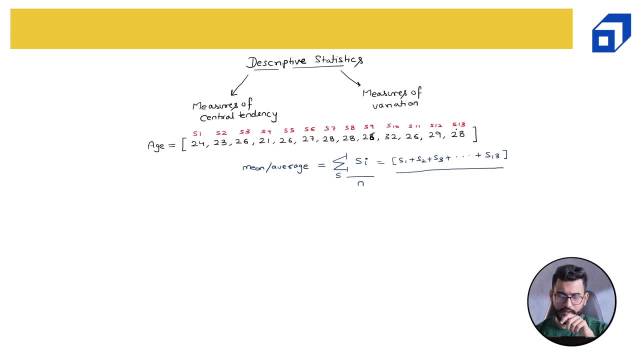 This Is My Sum Of All The Observations Divided By N. Now Here Are. You Already Known That We Have 13. And You Are? 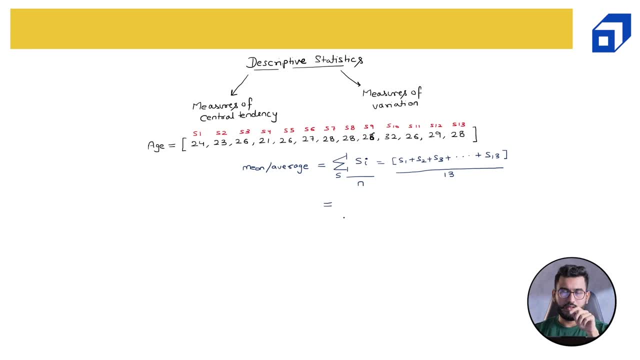 Watching This Video So That You Can Also Fully Understand The Complete Concept. So Please Watch, Please Stop The Video, Please Pause The Video And Calculate. 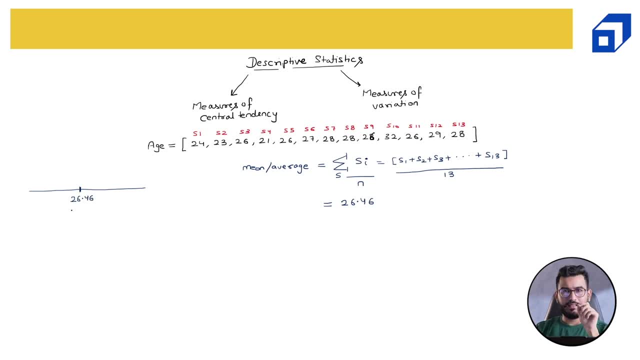 What You Want To See In This Video. Now You Are Watching This Video, So You Are Watching This Video. Now You Are Watching This Video. 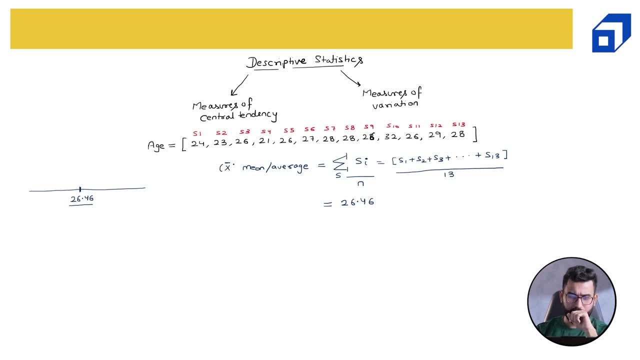 You Are Watching This Video. Now You Watch, You Can See That This Video How You Watch This Video. Now You Watch This Video, You Can. 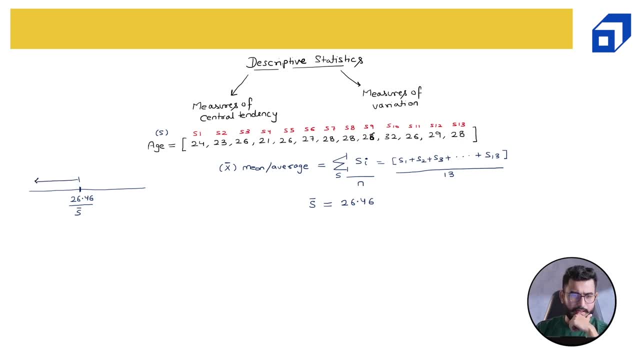 See. Now Watch This Video. observations: above this point I'm having few observations. now. you already know that in the class I'm having 13 people. so what we can conclude? we can conclude that in the class of 13 students we have few students above the age of 26, and I'm just taking 26 and few. 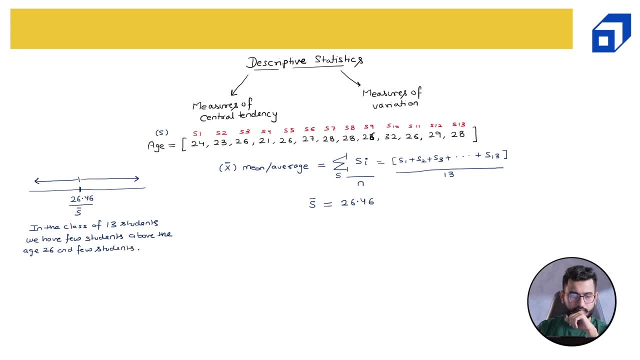 students below the age of 23. 26. So we are having few students above 26 and few students below 26.. And this 26 is basically describing the center of my data. Now, it might be exactly the center. it might not be exactly the center, Why? Let's try to understand this. Let's say, given this data, 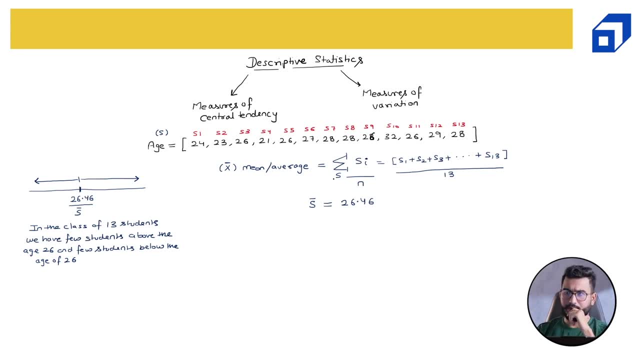 I intentionally add a particular observation. So let me add one particular observation: 40. Or let's add 50. So I'll write it over here and maybe let me change the color 50. So I've intentionally added a student whose ID is 14. And the age of this student is 40.. 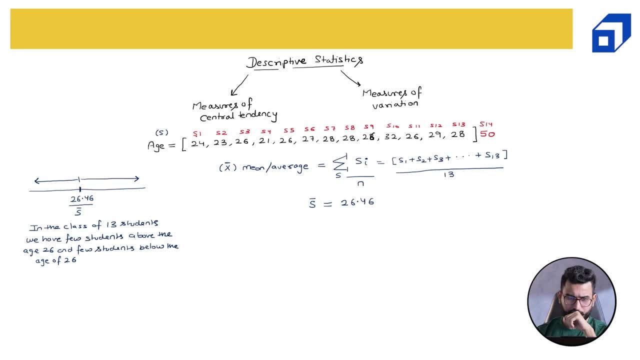 And into this particular data, which is having 13 students, you can see that almost all the students are having age in 20s, which is 21, 22, 23, 24 till 29. we have a lot of observations, but there is one student whose age is 32 right now. these observations are basically known as outliers. 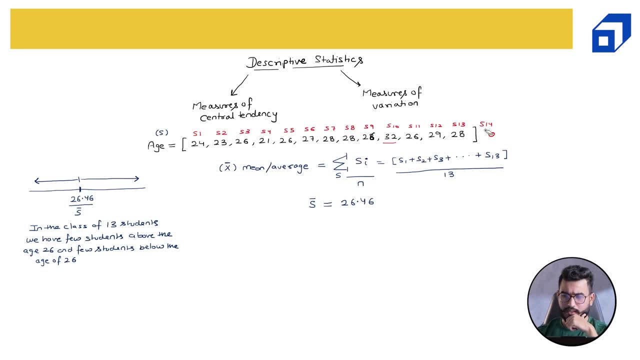 let me just remove this for a particular data point and let me write them in ascending order, and that would actually help us to derive the another measures of central tendency. so I'll I'll write: age is equal to now. the minimum number over here is 21, so I'll just draw a line over here. 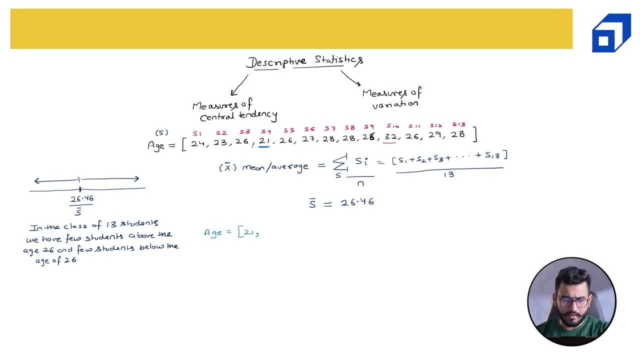 21, then we have. so we don't have 22, so we have 23, so i like 23 over here. then we have 124, so 124, then we have. uh, i don't think we have 25, so no 25. we have 1, 26, 2, 26, 3, 26 and 4, 26, so 26, 26, 26, 26, then we have. 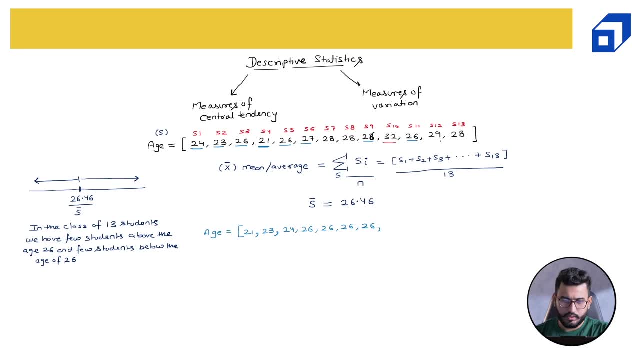 127 and only 127. then we have 28, 28, 28, 28, 28, 28, 28. finally, we have 129 and 32, 29 and 32. so all i have done is just rewritten all the age of all the 13 students in ascending order, where this is the. 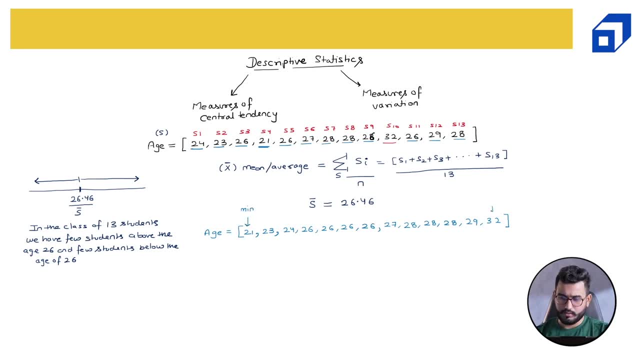 minimum age and this one is the maximum age. now, if you carefully observe, you can see that 32 appears to be 32 appears to be very different from majority of the data. now this observation is known as the outlier, so this is known as outlier. the formal definition of outlier is outlier. is that particular observation in my data? 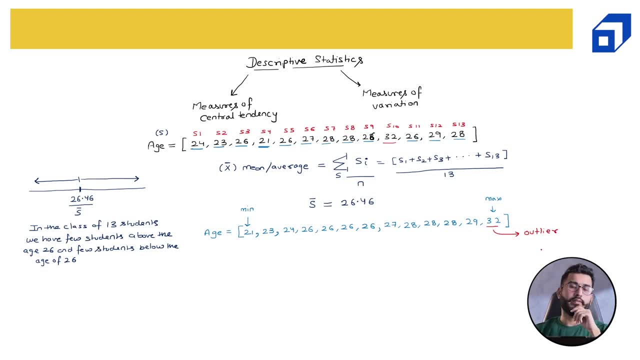 which is very different from majority of the data points. so let me just write it down. outlier is that particular observation in the data, that is, that is very different from majority of the data points. so if you carefully observe, here, majority of data points belongs to 20s, 21, 22, 23 till 29, but suddenly 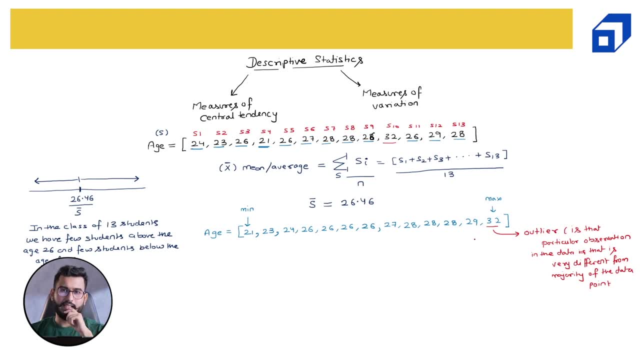 there is a number 32 and that is basically the outlier. now, what is the problem behind this outlier? why outliers are problematic? problematic when we talk about the descriptive statistics. If I try to look at the median, what is median? Median is another measure of central tendency. 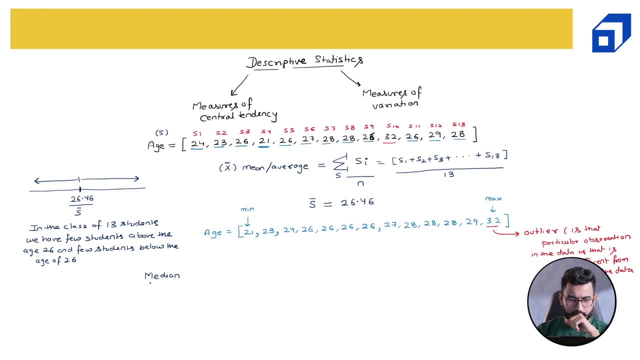 So what is median? Median is another measure of central tendency. So we have already talked about mean over here. then we have median. Median is exactly the center of the data, exactly center. So when I say exact center, that basically means above this. 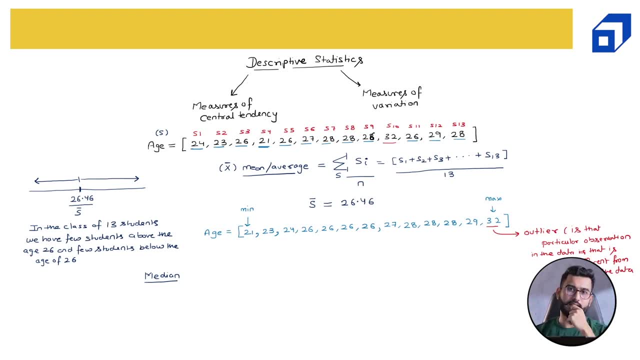 I will have 50 percent people. below this, I will have 50 percent people. So it is exactly the center how we can find out median. So there is a simple formula and plus one divided by two with the number of observations are odd. 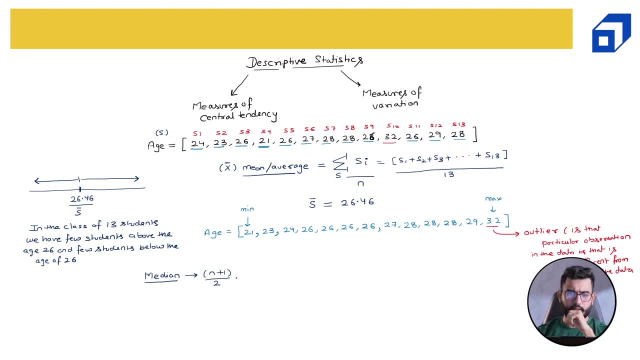 Here we have odd number of observations: 13.. So 13 plus one divided by two is 14 divided by two, which is seven. So my seventh observation is this: is the center of the data or is the middle point of the data? 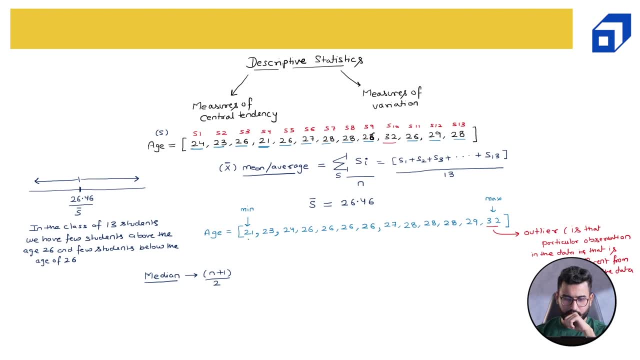 And let me just quickly mark it. So it is one, two, three, four, five, six, seven over here. This is my center. Now, if you just number, if you just calculate, if you count below this 26,, 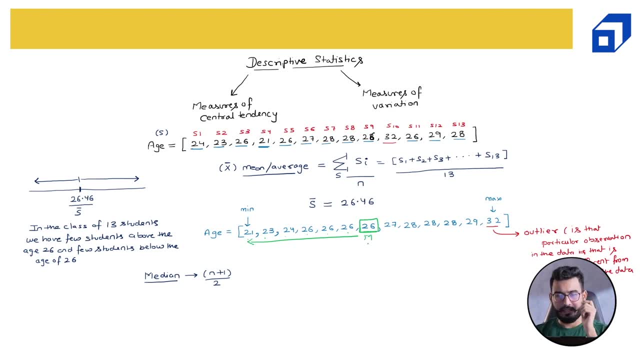 below this middle point. I'll just write M to depict that this is a middle point. I am having one, two, three, four, five, six. I'm having six observations above this: one, two, three, four, five, six. 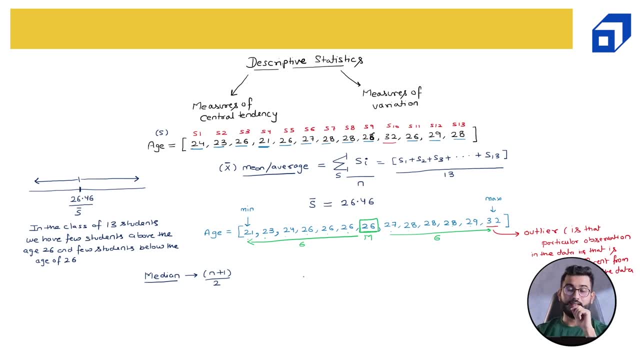 I'm having six observations. So median describes the exact center point of the data. So what is median? This value Lies Exactly In the Center of the Data In such a way, In such a way That we have: 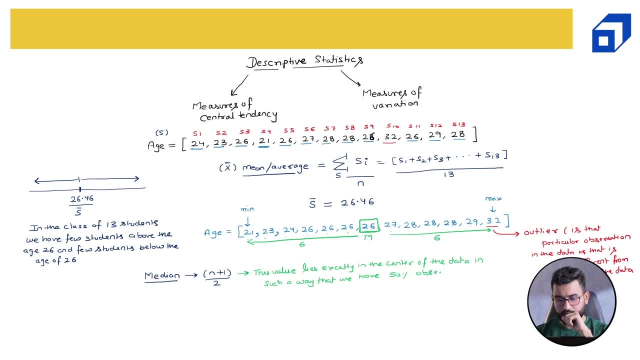 50 percent observations. 50 percent observations Above this point, above this point, and here we have taken M. so above this point, M and 50 percent, And again, this is M. so below this point, M. so median describes the center of the data. 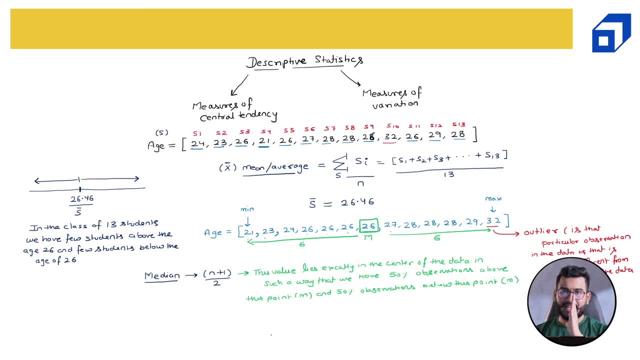 in such a way that it is lying exactly at the center, where 50 percent of the data is below this point. 50 percent of the data is above this point, while I cannot say the same thing for average. And you can see why. 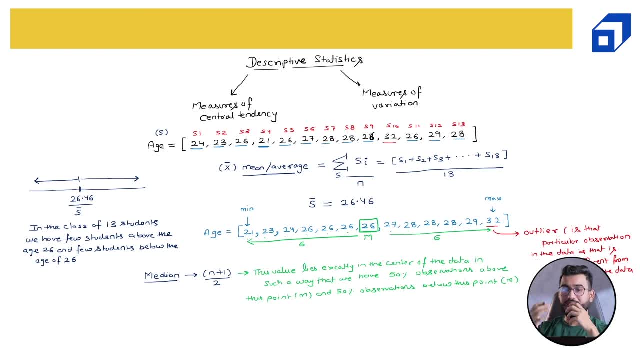 Average is basically taken out by considering all the data. When I have to calculate average, I am summing over all the data. Here you can see the formula. The formula is sum over all the data points divided by the number of data points. 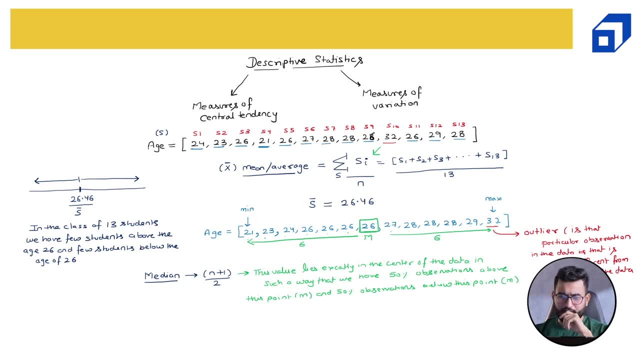 And due to these influential observations, which are known as outliers, my average can shift towards the outlier. Here you can see a mean. as I have told you, mean is also the center of the data, while median is also the center of the data. 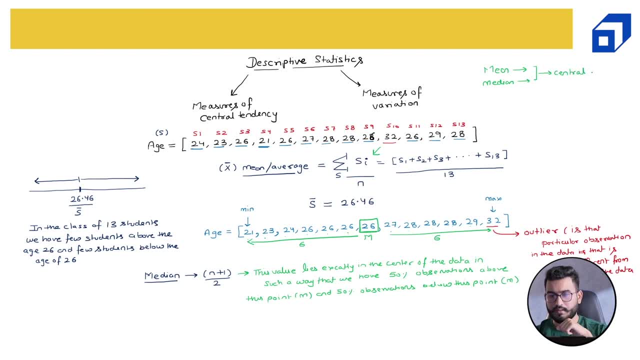 These, all these, both metric, describes central point Of my data. But why there is a difference, why my average is twenty six, point four- and why my median is twenty six. So my median is twenty six. Now, this is because of this outlier. 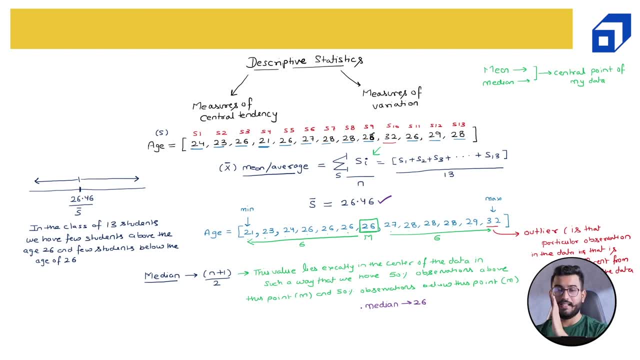 So where I'm having outlier, I'm having outlier on the higher end. This is my higher end. So what has happened to the mean? My mean has also shifted towards the, towards the outlier. Now, please remember this. I'll just write down as a note over here. 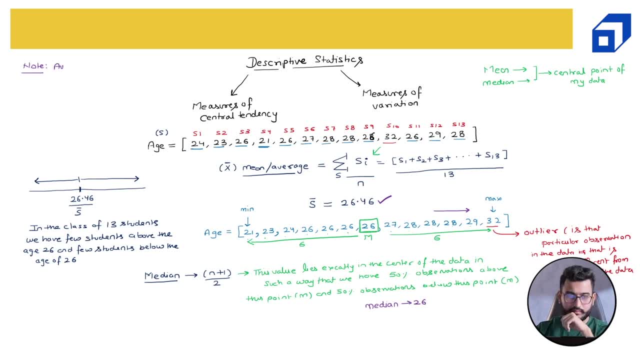 Here that your average Average gets impacted With the Presence of the outliers And will shift Towards the outlier. So if my outlier So, assume that if this is my number line and if my outlier is on the lower side, Then my average will shift towards the outlier. 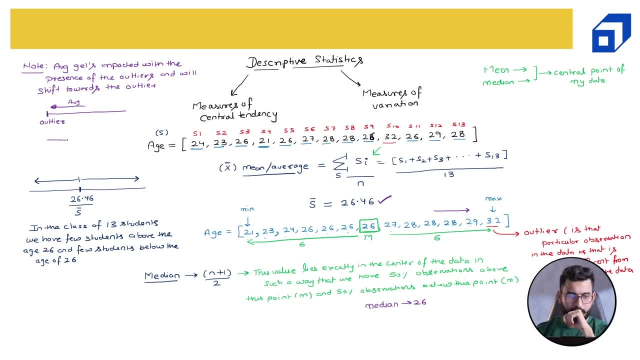 So my average will shift towards the outlier. If my outlier is on the higher side, Then my average will shift on the higher side, And we have already seen this example. My median was twenty six, But my average came out to be twenty six point four six because 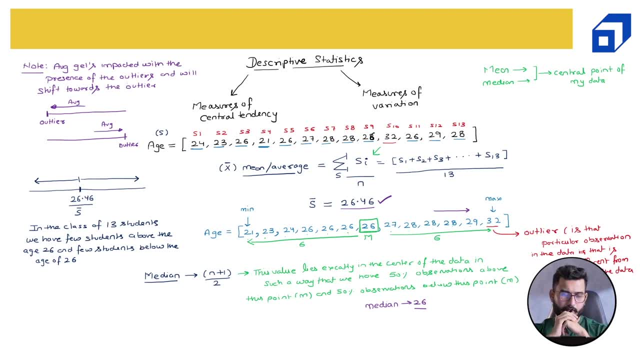 my average has shifted towards the outlier Right. Then we have one more major measure of central tendency, which is mode, And mode is very simple to understand. Mode is the observation with the highest occurrence in the data, So let me write the definition over here. 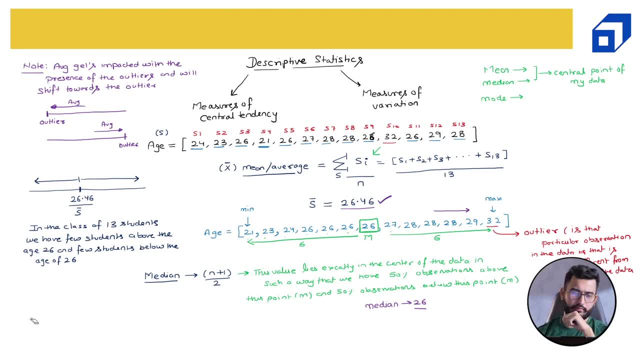 I'll just simply write it as observation with maximum frequency. Observation with maximum frequency. So if you carefully observe, in this particular data I'm having the observation number 26,, not number 26, observation 26 to have to do. This observation has appeared for. 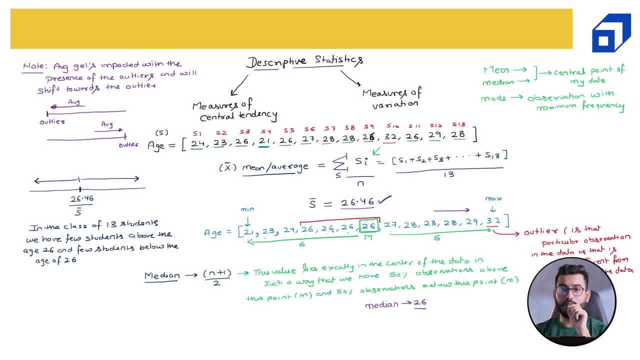 Four times. So the frequency is highest for the observation 26.. And hence my mode of this data is 26.. Mode of the data is 26.. Now there might be cases where you do not have any mode. For example, let's say I'm having four observations. 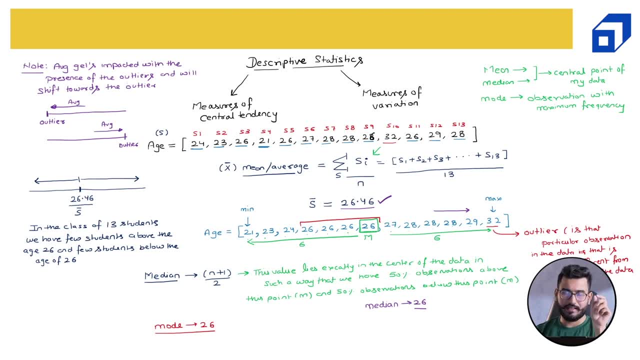 sorry, four observations. four observations 26. Or there are four students with the age 26. We also have four students with the age 28.. Now, in that case, when there is a tie, there is no mode, So you will simply write no mode. 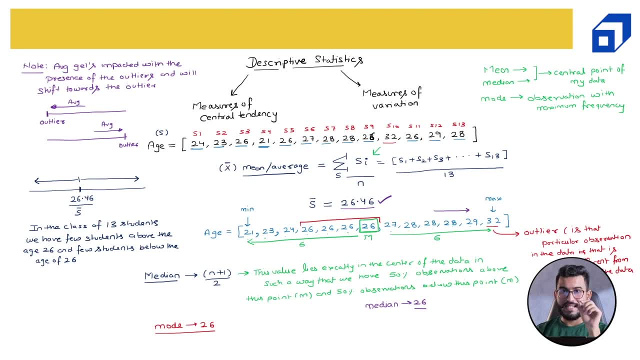 In that case you have to use mean and median to describe the center of the data. So I hope you guys are able to understand the measures of central tendency. As the name says, this or all these three measures which are mean, median mode. 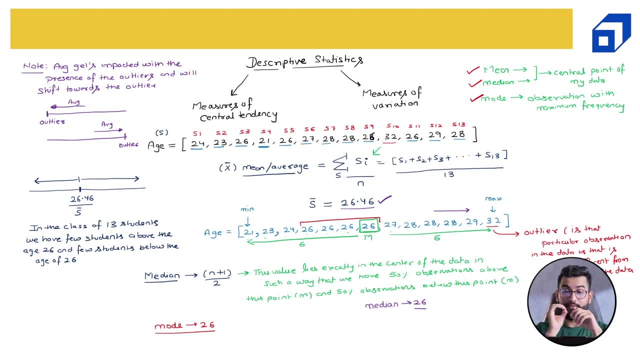 they basically describe the center of the data. And if your data does not comes with outlier- And here you have seen that 32 was the outlier- But if your data does not comes with outliers, maybe either on the higher side or on the lower side, we do not have any outlier- 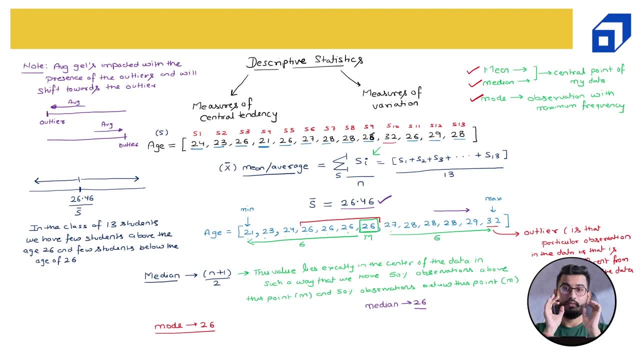 These three measures will fall very close to each other, or approximately they will be equal to each other. So your mean will be equal to more, equal to median. And here you can see, I was having average to be 26.46.. If I was not having this outlier, which is 32,, I would have got this value close. 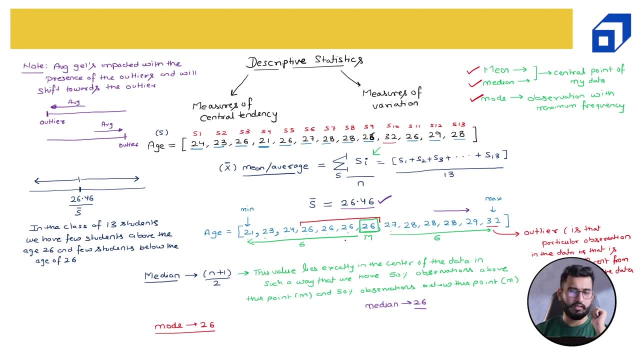 to 26 only. sorry. 26.46 is my average. My median is 26.. My mode is 26.. In this case, I can say that my data is having a center of 26.. Now, if I go to my principal and if I tell, 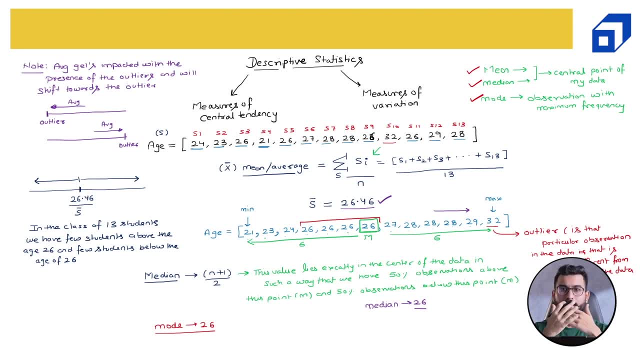 to my principal that the average age of my class is 26 with 13 students, then it gives the rough idea to the principal that, OK, we have a center point 26 and we have few students above this point, few below this point. 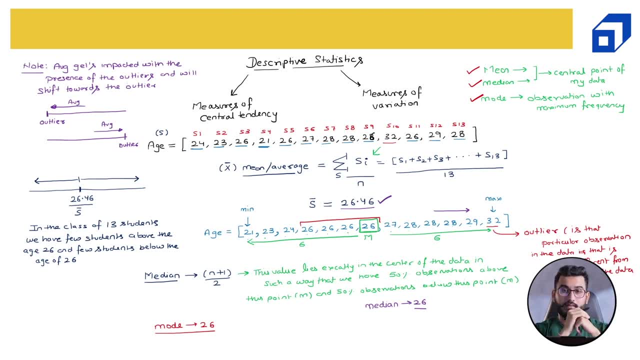 If I tell to my principal that the median is 26, with total number of students to be 13,, then in that case the principal will be able to do a little bit of math and he will be able to understand that. OK, we have six students below 26,. six students above 26.. 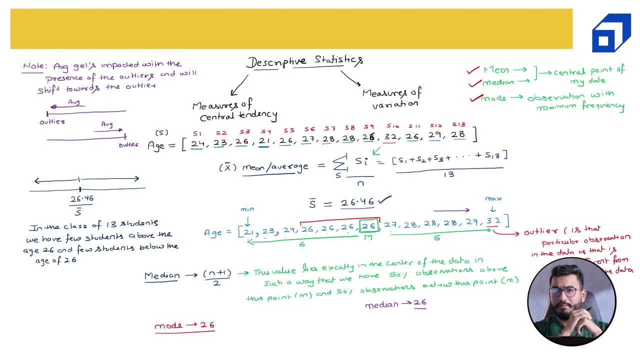 So I hope you guys are clear with measures of central tendency. but there is a problem. The problem is I'm still not clear How the values are varied. So I know that center is 26,, but how would the variation is there in the data. 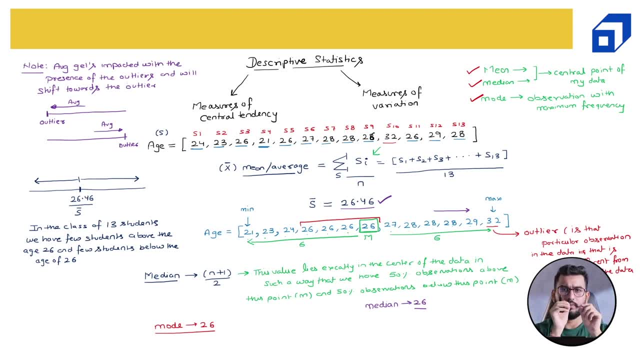 So am I having the age of the students to be very much varied? When I say varied, that basically means the values are very, very far away from the center. So let me just give you a very simple example over here. Let's say: 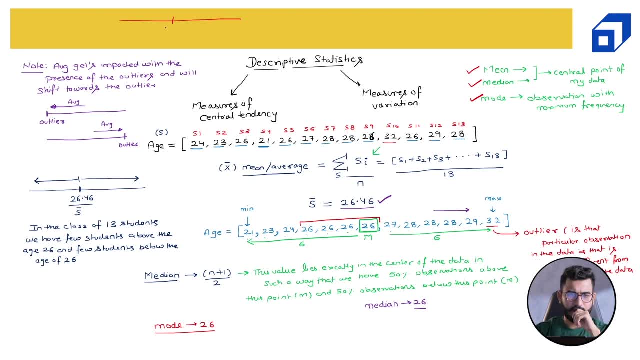 this is 26.. This is 26 and here also we have 26.. So in these two number lines the center is 26 itself, But in this number line on that is on my left of the side, left of my screen. 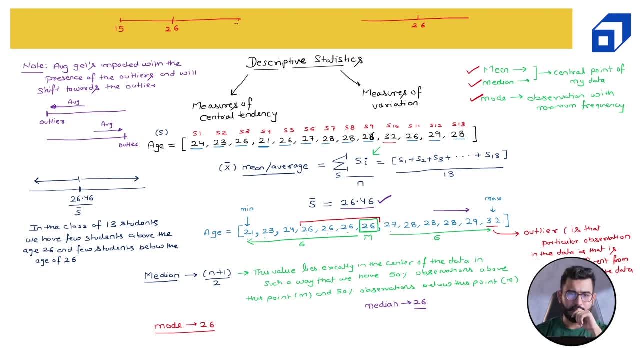 The minimum is 15.. Maximum is 30. Here you can see that the minimum is 20 and maximum is 30. Well, let's let's take it as 29.. Now here, if you see that the values are very far away from the center, there is a high variation. 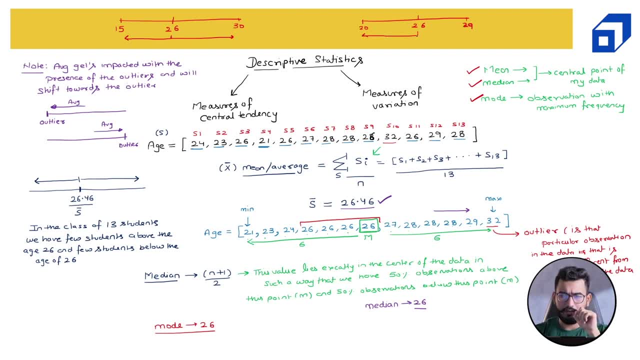 While here the values are not so far away from the center, The variation is low. So measures of variation tries to quantify this variation Given a particular data: how much values are scattered around the center? This is what we are going to learn in measures of variation, which is our next topic. 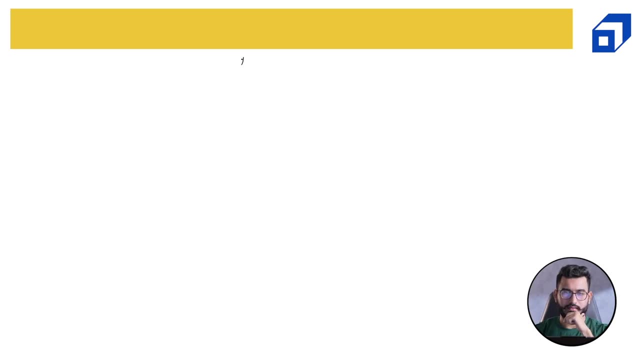 So now let's talk about measures of variation. Measures of variation- And I have already given you a very, very short example, I would say, in my last slide, But now let's try to Have a more insightful example which will clarify your doubt regarding what exactly is measures of variation. 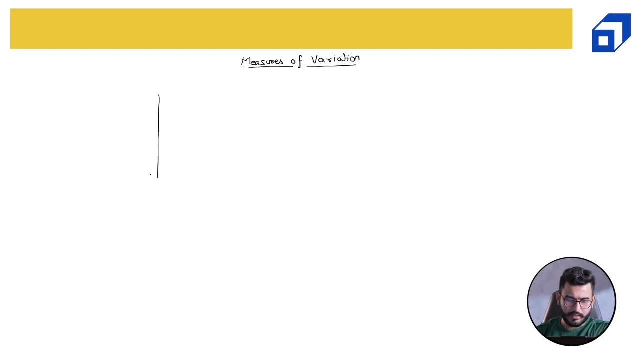 So let's try to Take two examples Or two subjects, And I'm just plotting these two subjects to get you a visual picture about what exactly I'm trying to explain. Assume that here the exact axis represents the student ID for both the plots and y axis represents the marks. 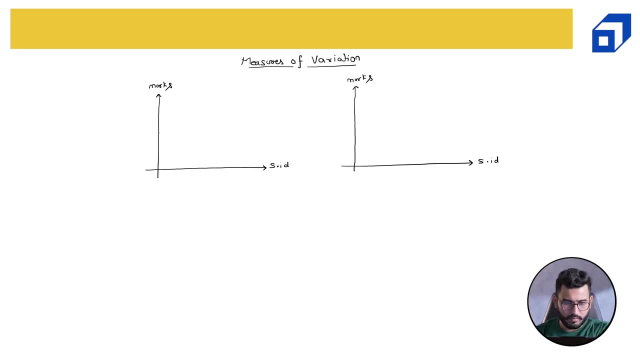 These are the marks. So let's say, the average marks are represented by this red color line, Red color dotted line. These are the average marks. This is the average marks. For example, you can assume that the average marks is 50 for both the subjects. 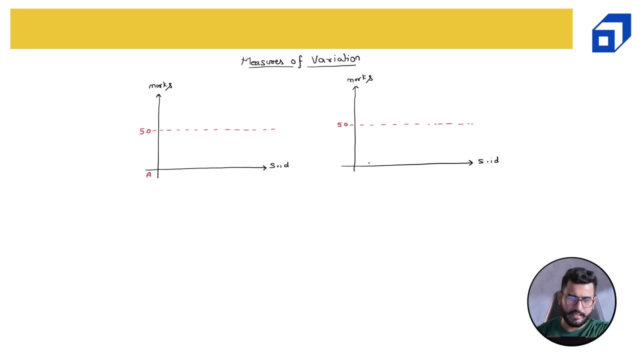 But for Subject A and this is subject B. I'm not just naming any subject, I'm just saying A and B. For subject A, The student marks are scattered like this: So this represents the marks of student number one. So this is. 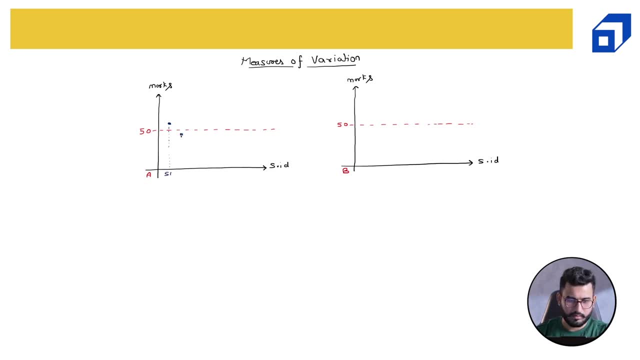 A student number one, then this marks of student number two, Then we have a student number three, and so on. So I'll just draw it now, because I hope this gives a clear picture about what I'm trying to explain. So this is basically the scatterplot for subject A. 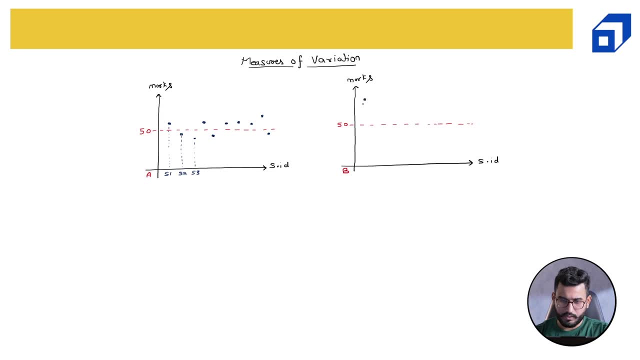 For subject B. This point represents The marks of Student number one, This for Student number two, then three, Four, Five, Six, Seven, Eight, Nine and let's say ten, Here also I think we have ten. 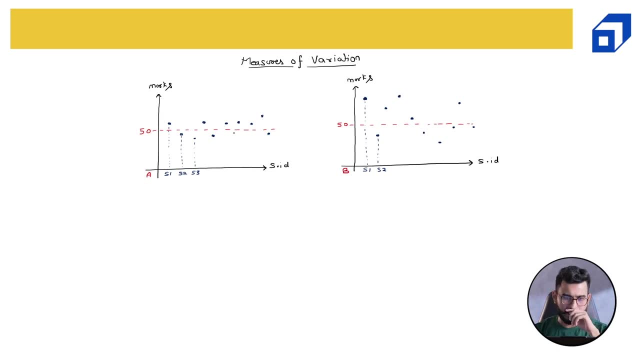 One, two, three, four, five, six, seven, eight, nine, ten. So you can see that, And in both A and B we are having ten students. But for subject A You can see that all the marks or all the students have scored. 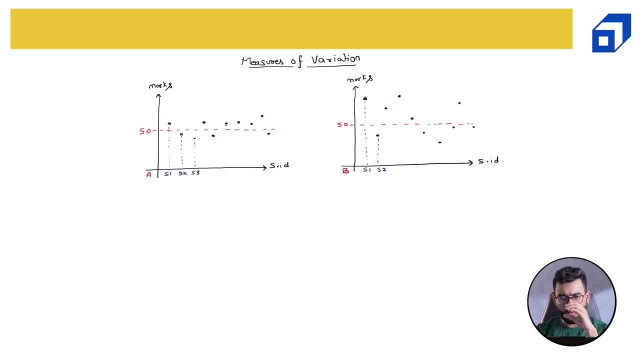 They have scored marks which are very close to the average Most of the people have scored. let's say, if I just create a band, let's create this band, a dotted band, So most of the students fall in under this band or within this band. 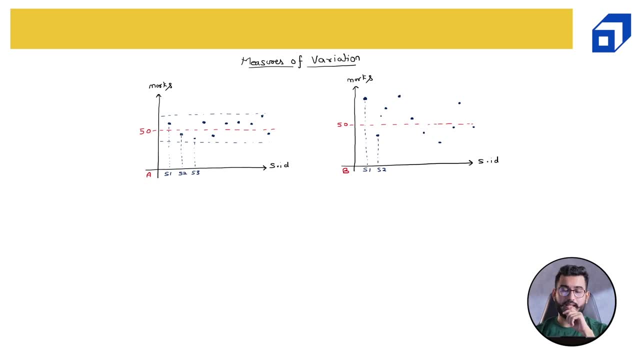 While here for subject number B, you can see that There is a lot Of scatteredness. You can see that there are data points which are very far away from the average line. there are data points which are also close to the average line. 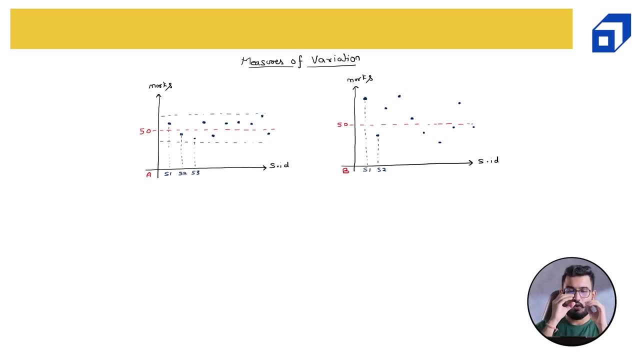 But in student, in subject A, all the data points are very closely scattered around the average line. Right now can I say that for subject A, the variation around the mean. So this is my Mean. The red color dotted line is my mean or the average line. 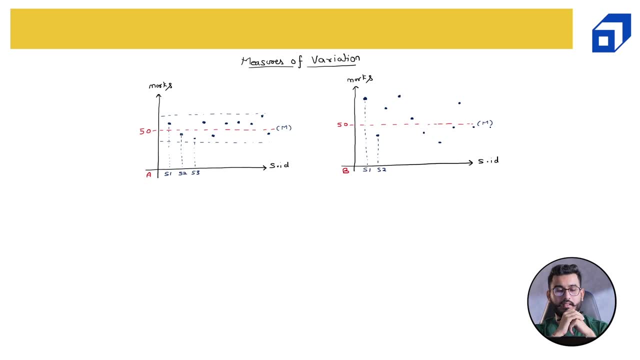 So M represents the mean or the average line. So for subject A The variation of the marks around the mean is low. For subject B, the variation of marks around the average line is high, So here The variation Around The average line. 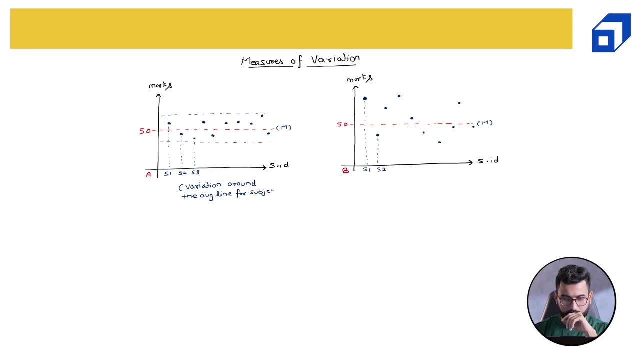 For Subject A Is low, While for this Variation Around The average line For Subject B Is high. Now the measures of variation tries to quantify this: How I can say this is low and how I can say this is high. 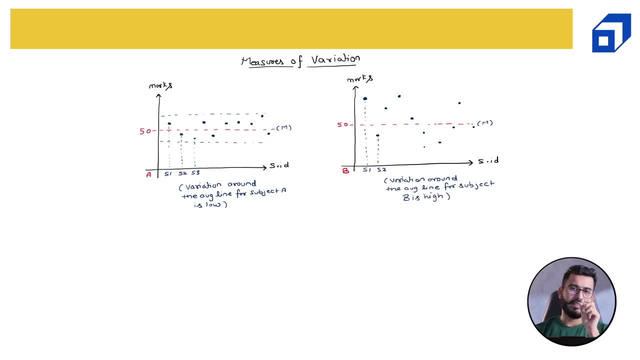 We need a number right, We need some quantity, We need a number that can describe this measure, or describe this scatteredness, or describe this variation. So measures of variations are those metric that describes the variation of the data around the center or around the average line. 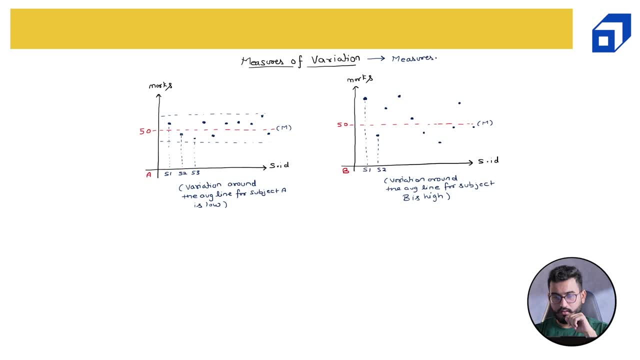 So measures, Or metric That Describes the Variation Of the data Around the center of the data Center, or the average. Now, what all measures we have? So number one, So I'll write it over here: We have: 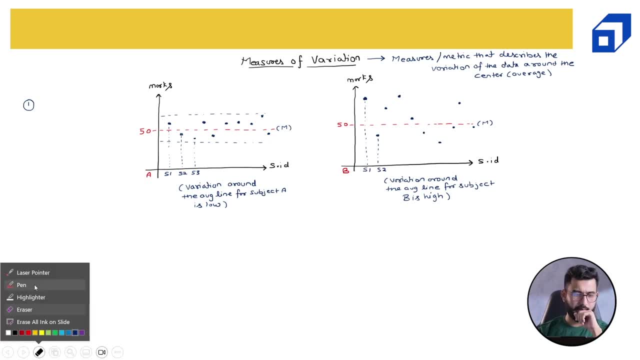 So we exactly have, I think, four measures. Let me write it down. So we have range, We have Variance, We have Standard, Standard deviation, Standard deviation And finally, we have the coefficient of variation. Coefficient of variation. 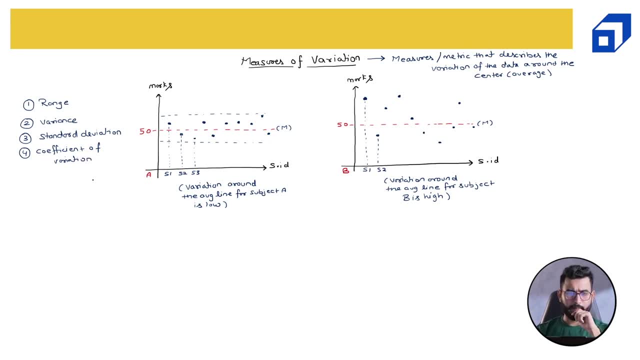 So let's talk about each of them. Now, in order to talk about any of them, we need the data. So let's create some random data. So let's say: here we have the data of The marks of a student in one particular subject. 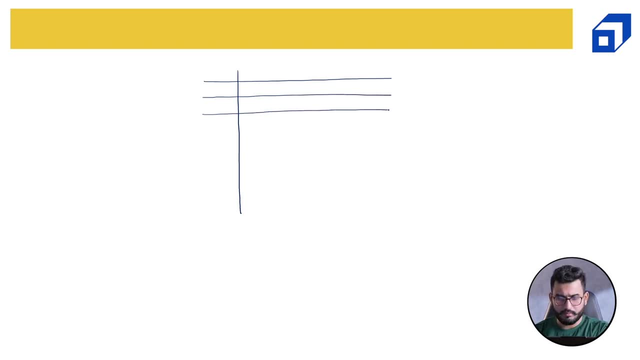 And I'm intentionally drawing this table a bit Large because we will be calculating a few Few parameters in order to arrive to the exact Quantity that we are looking for. So let me just quickly draw the table. So here we have the student ID, which again runs from one to, let's say, ten. 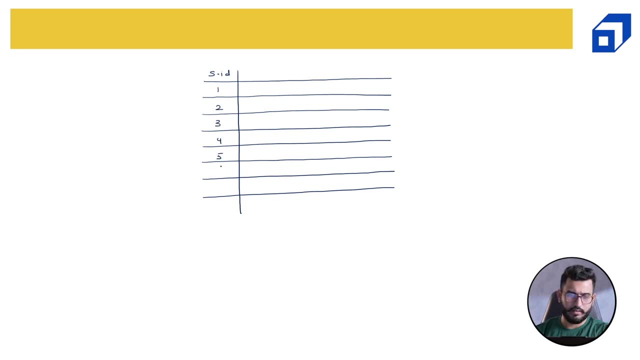 One, two, three, four, five, six, seven, And then these are the marks. So I will write XM. XM means marks of students. So let's say the marks are Twenty seven, Fifty two, Forty eight, Thirty, thirty three, thirty nine. 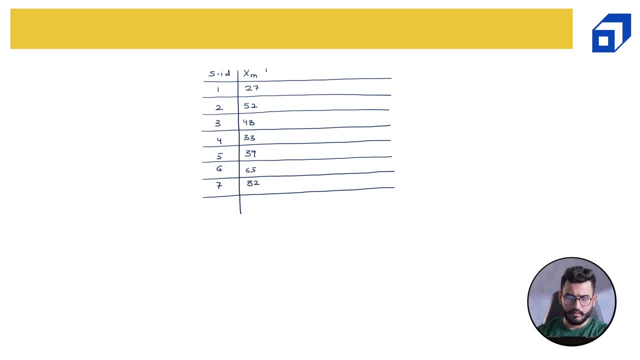 Sixty five and eighty two. So this is my marks of these students. Now, If I have to calculate the range, Range is nothing but The maximum minus minimum is. it gives you a very raw idea regarding What is the range of my. 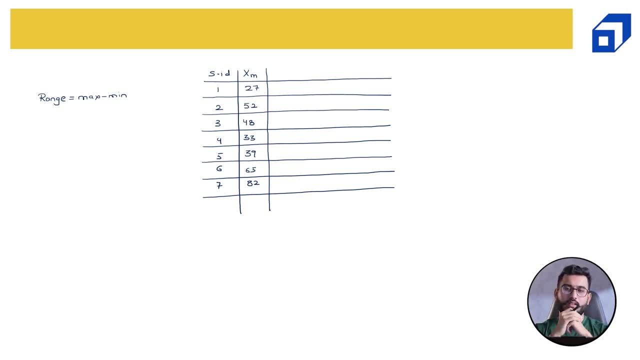 What is the range at which we are trying to work? Or If we are talking about the marks, then what is the minimum marks scored? What is the maximum marks scored? And the range is nothing but the difference between max minus min. So my max marks is eighty two minus minimum. 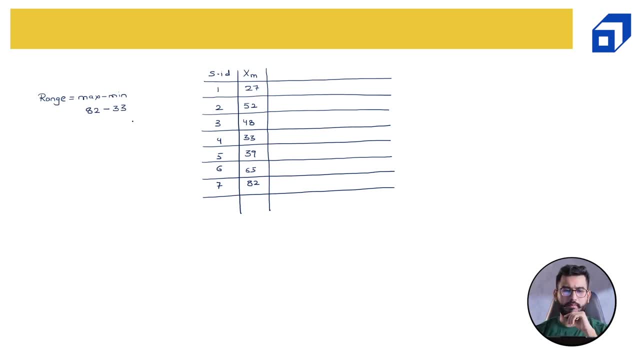 Which is thirty three, And if you subtract this you will get the range. The second major is variance, which is a better major to define the variation in the data. What is the problem with range? Range is again influenced by the outlier. 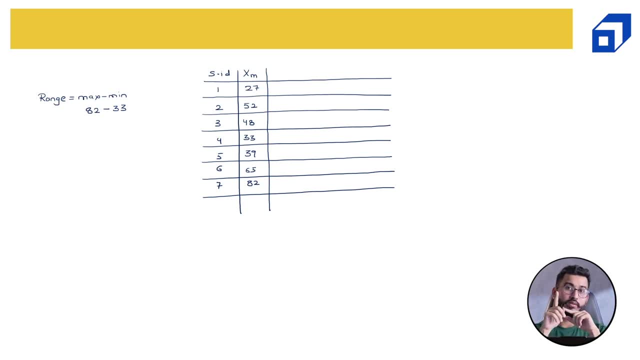 So let's say, if there is one student in the class who has scored 100, while most of the student has scored, let's say, close to thirty three, thirty three, thirty five, thirty, nine, forty, then in that case also the range would be very high. 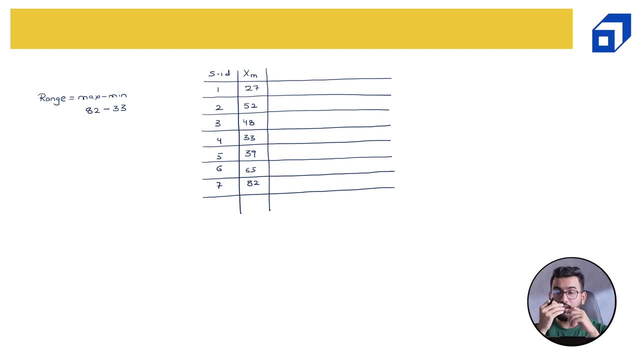 So it would. It would mislead you, It would give you, give you a misleading idea that students have scored in a high range. but that is wrong. range gets influenced by the presence of outlier And that is the reason we don't use the range as a major to to make or to. 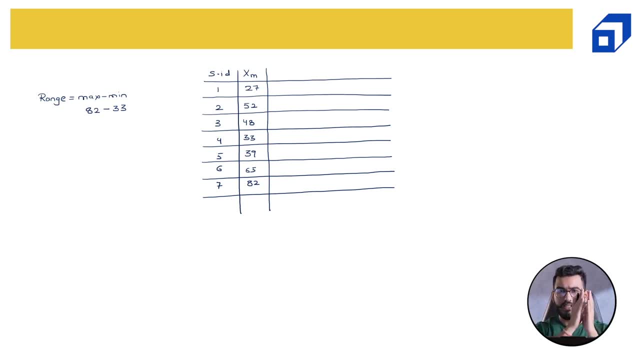 understand about how the data is, how the data is scattered around the center of the data, or center line. So let me write it down over here: Range is a metric that Gets Influenced With the Presence of Outlier. 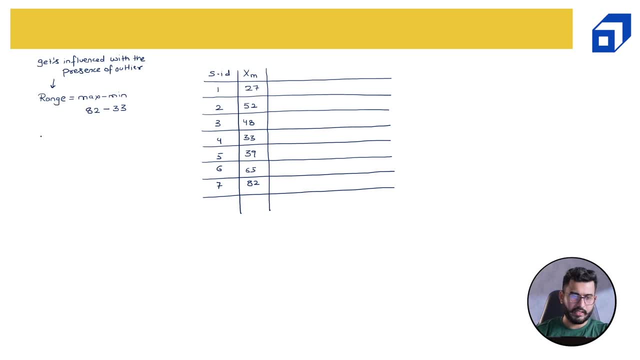 Now how to arrive to the variance. So we are talking about variance now. In order to calculate variance, We will first of all find out the center, because, as I have told you, variance is all about calculating the scatteredness, or calculating the variation. 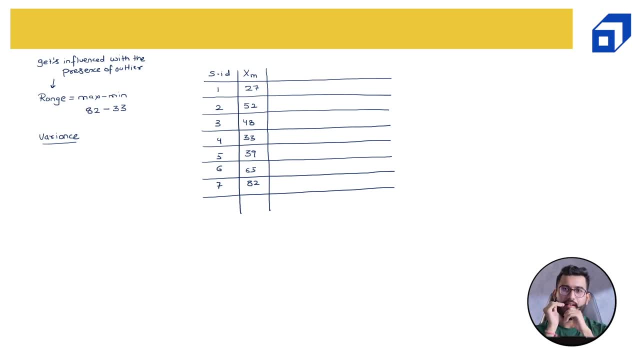 of the data from the center point, which is the mean or the average. So we have to find out the average, first of all the average, And if you guys want, you can pause this video and quickly calculate the average, because we have already learned about it. 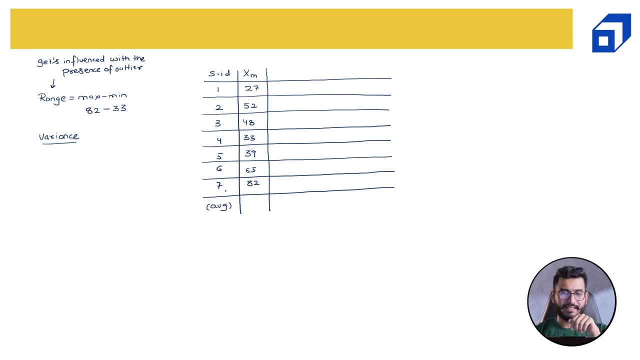 So just take the sum of all the observation divided by seven, because seven is the total number of students in the class, And that would give you the average. So the average of This particular marks for the students would came out to be forty nine point. 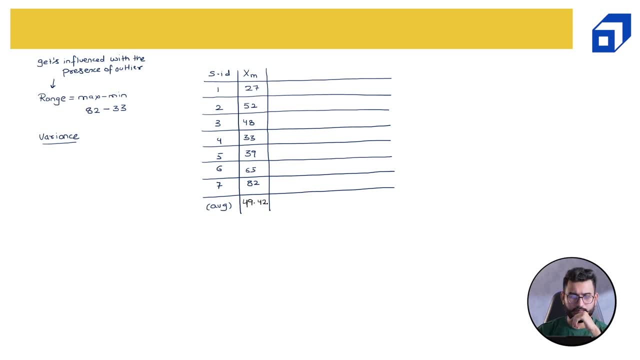 Forty nine point four to Now. for the simplicity purpose and for the for making all the calculations very simple, very clean, let's take this number as forty nine, So assume that the center is forty nine. Now we have the center, so let me just quickly draw the graph. 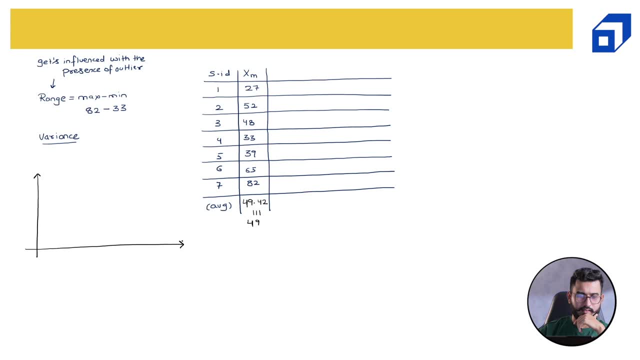 The same graph that we have seen in the last slide. This is a student ID. These are my marks and we have the center now at forty nine, So somewhere in the middle but one point below. So assume this is forty nine. So this is my forty nine. 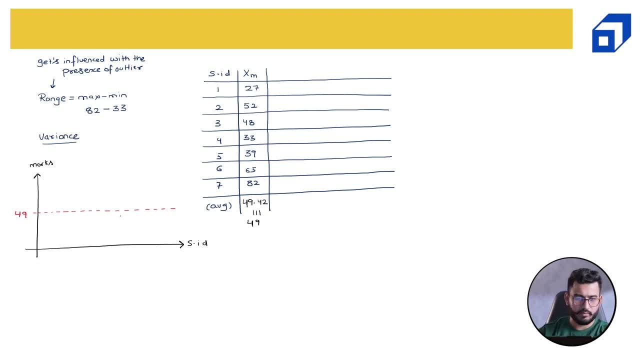 Now let's mark all these numbers. Twenty seven would lie somewhere around here, So this is student number one. Then we have fifty two, So this is my student number two. And then we have forty eight, which is very close to the average. 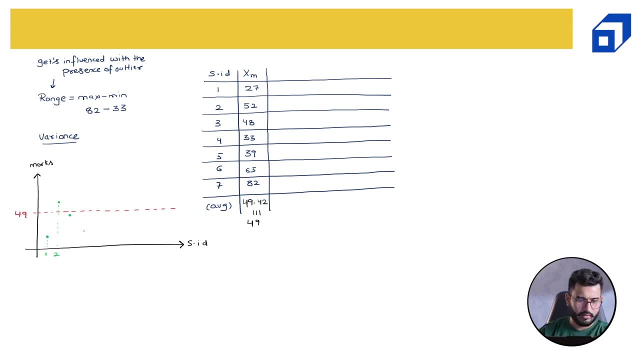 So this is forty eight and thirty three somewhere over here. Thirty three, then thirty nine, maybe over here, Then sixty five over and above the average line And finally Eighty two, which is again over and above the average line over here. 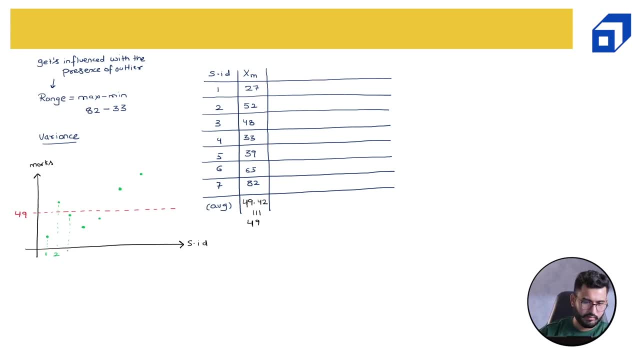 So these are my data points. This is my student number three. This is four, Five, Six, Finally seven. we have seven data points. Now we will calculate the distance of each of this data point from the center. from the center, which is average. 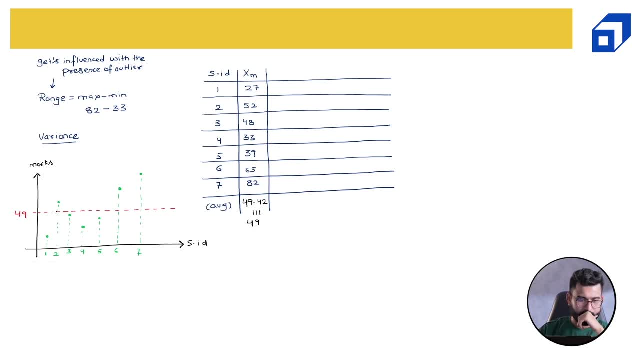 So when I say distance, I'm basically interested in This distance. This is D1, then this is D2.. Similarly, this one will be D7.. This one will be D6. So distance is nothing, But I'll take the data point. 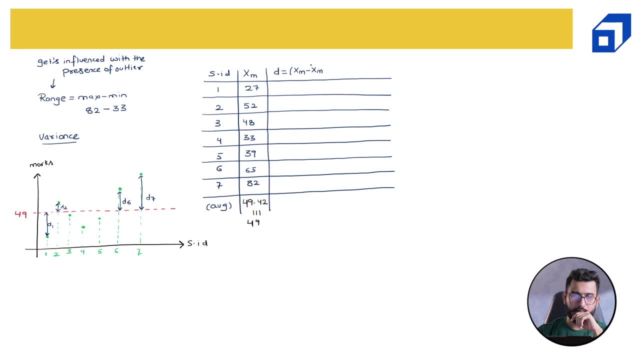 So XM minus XM bar. I hope you guys remember, if I put a bar on a variable it becomes the average. So this is my average marks, which is forty nine Average marks. So twenty seven minus forty nine, that will be my D1. 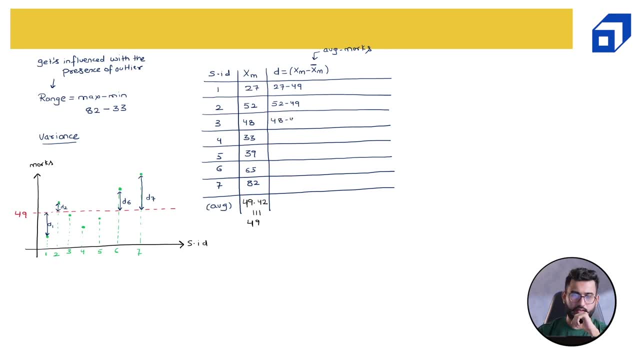 Fifty two minus forty nine, Forty eight minus forty nine, Thirty three minus forty nine, Thirty nine minus forty nine, Sixty five minus forty nine And finally, eighty two minus forty nine. Now, if I ask you, what is the average? 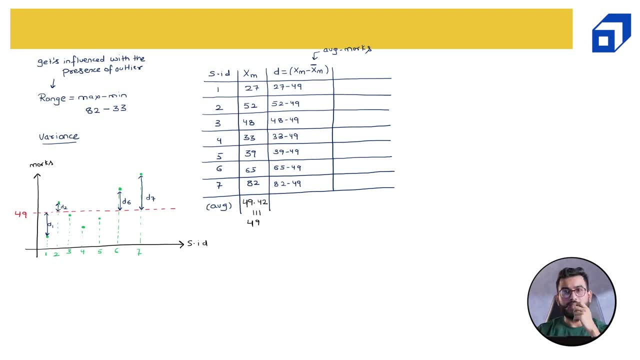 Now, if I ask you, what is the average? Distance from the center Basically mean how much, on an average, a data point is deviated from the center. Now, if I have to find out average, I have to take the sum of all these values, right? 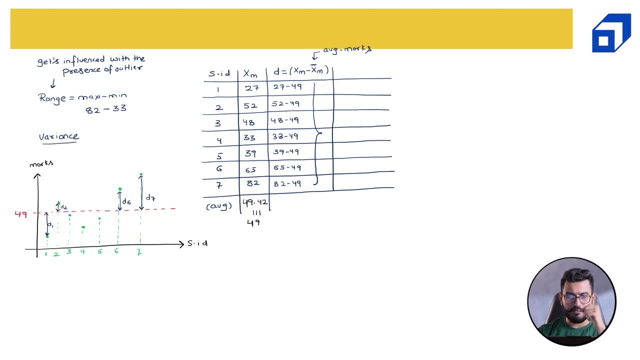 The problem is that Few of the values are above the average, which would result in a positive value, Few of the values are below the average, which would result in a negative value. And if I simply take the sum of all these data points, the positive will cancel out negative. 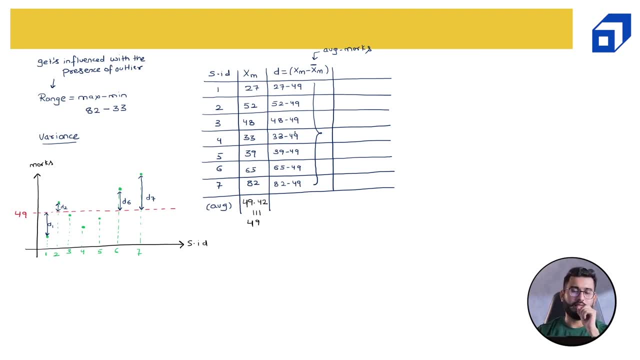 So we would get a very wrong value. And if, if I know that the center is zero and we have some positive value, some negative value, then everything will be, you will get a value close to zero, which basically mean there is no variation. 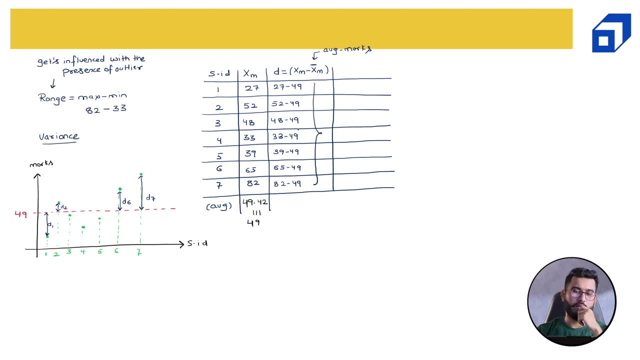 which is wrong, right? In order to This problem, I will take distance square. I will convert the positive, the positive error or the negative error into the square so that the positive and negative can be can be nullified. We can get rid of these positive signs and the negative sign. 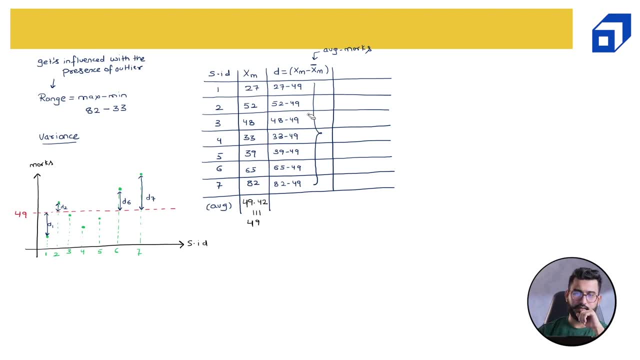 So let me just quickly write down what we are left with. So this will result in: I'll just quickly write down all the numbers, Because I have already calculated it. Now, here you can see that I'm having minus 16 and plus 16,. 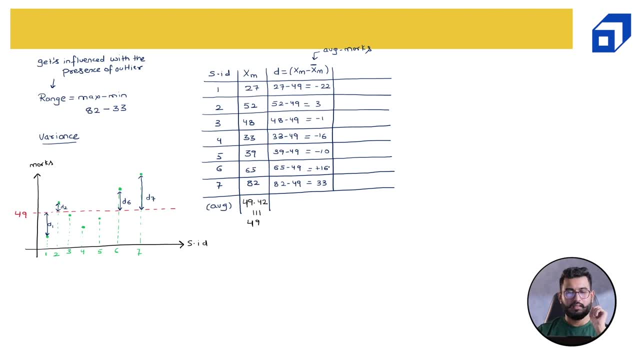 and if I simply take the sum over all the D, This minus 16 will cancel out plus 16, so I will not get the. I'll get the contribution of these two numbers. Similarly, you can see that I'm having minus 22 plus 33, minus one plus three. 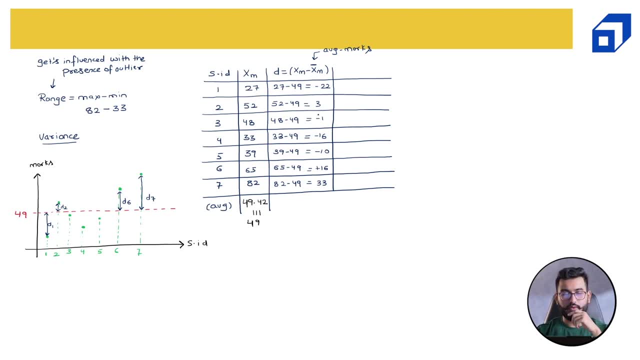 So we are having some values which are positive, some values which are negative, and we cannot simply take the sum, So we will take distance square. So 22 to the whole square is- I have already done it so- 484,, 9,, 1,, 256,. 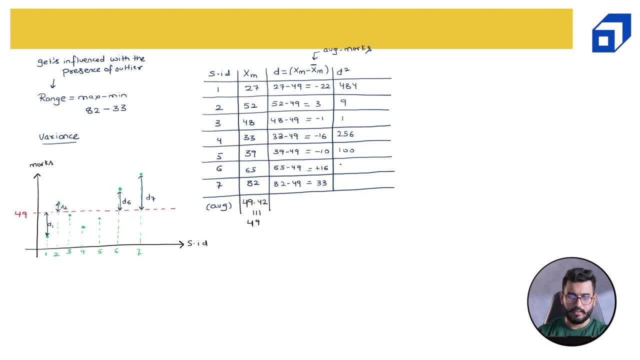 156, 100, again 256 and 1089.. Now we will take the average of the distance square. So what we have to take: average of distance square. Now you guys can ask me that Sumit why you have taken a square. 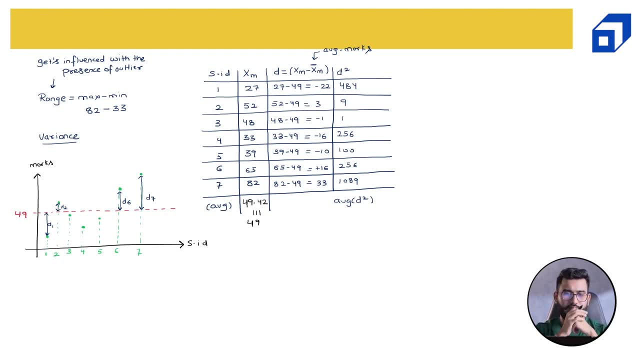 Why you haven't taken the absolute value. So I would have simply taken Minus 22 as just 22 and minus 16 as just 16.. Now please remember that when we are working with statistics, we are using a lot of calculus also, and as of now, I cannot show you where I. 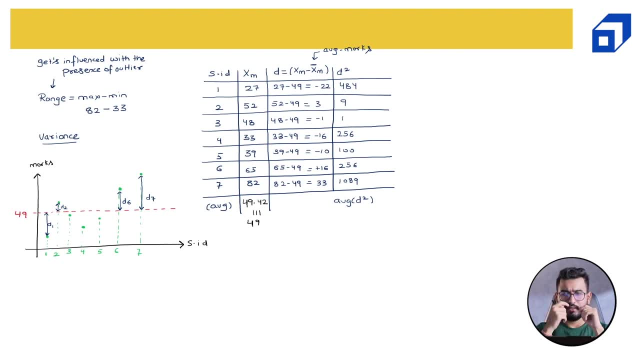 would be working with calculus. but as we proceed forward you would see that statistics is heavily dependent on calculus And when we talk about functions, the function or the derivative of a constant Is always zero and derivative of a square term which is d squared, or maybe. 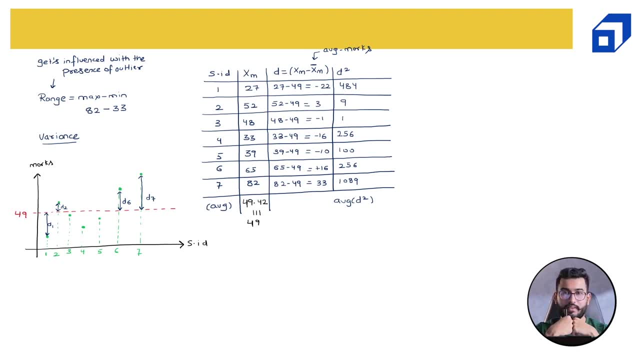 a derivative of a function which comes with a polynomial value can be differentiated. So your calculus does not work with constant, does not work with functions which are constant, And that is the reason we will not be using those. We will not be using the absolute term and we will be using the square term. 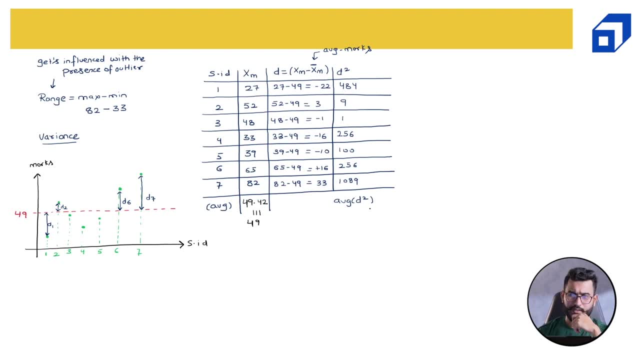 So we have to take the average of d squared And you already know the formula, which is summation over d squared And divided by n. so if I take the sum of all the observations which are present in the column d squared divided by seven, 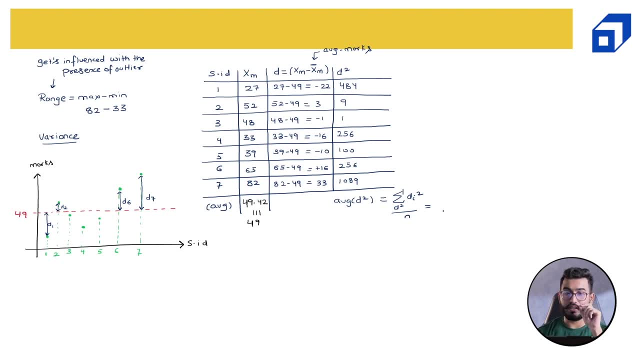 I would get the average distance, or not just the average distance. I would get the average of d squared. So this would be 2195 divided by seven, which is 313.57.. Now this value is known as variance Variance. 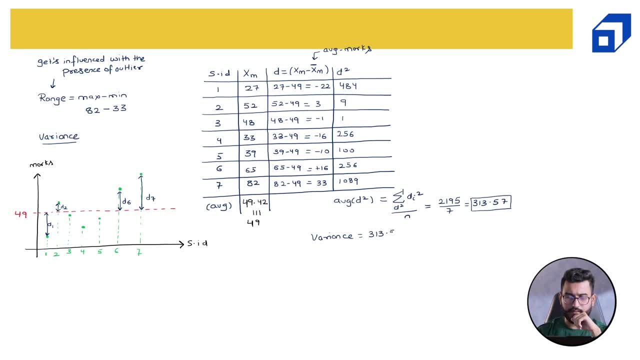 Which is 313.57.. The problem with variance is that you can practically not make sense out of it. I'm not able to understand what this value means, And if you remember, it was d squared. D squared is equal to 313.57.. 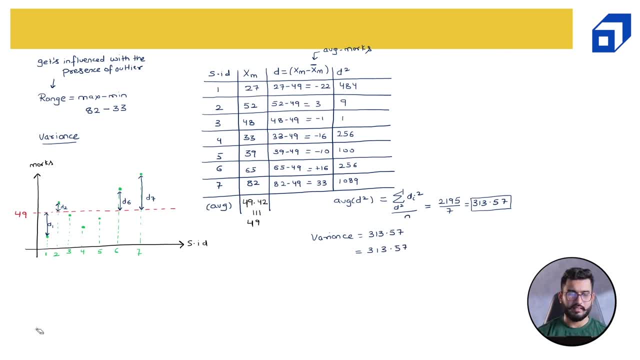 Variance is also known as sigma squared. It is known as sigma squared. This is a Greek letter, sigma, Sigma squared. So my sigma will be square root of 313.57.. And this would get us 17.65.. This is my sigma. 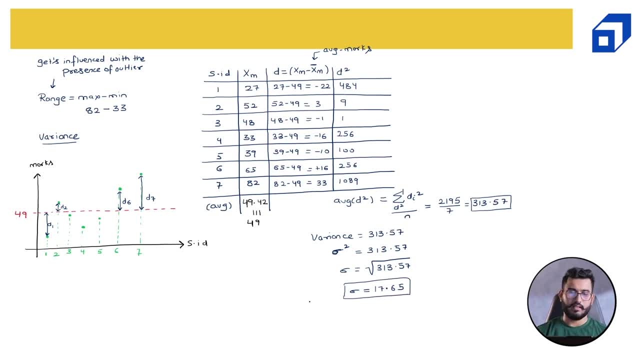 Now, what is the meaning of this? Now, sigma squared is my variance. Variance is basically my sigma squared, While sigma is my standard deviation. Standard deviation, Standard deviation, is my sigma. So standard deviation talks about the average distance that the data points are deviated from the center. 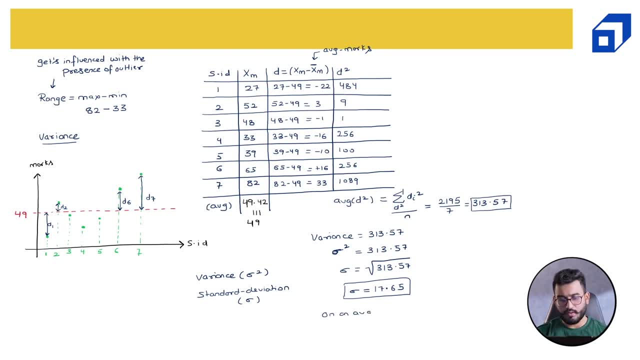 So, on an average, on an average, the data points, the data points are 17.76 marks above or below the mean, And that is what this standard deviation mean. How much, on an average, the data points are deviated from the center. 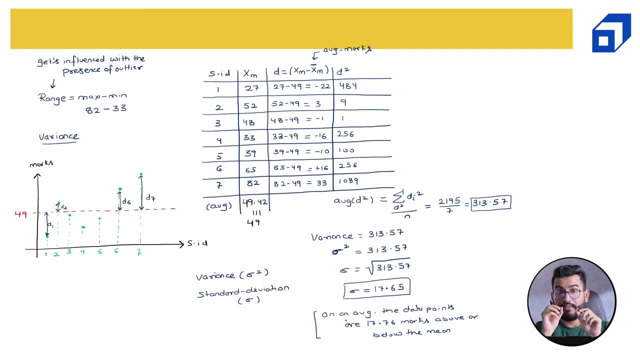 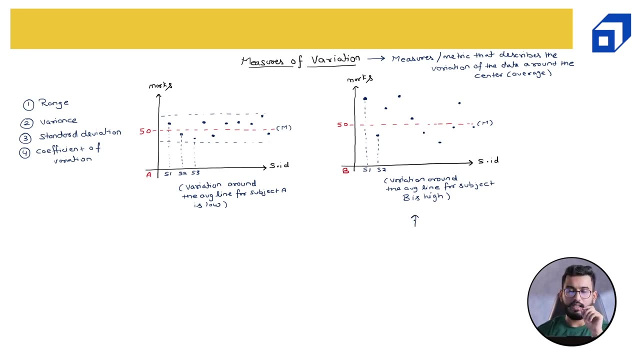 And that is 17.65.. Now, if this value is very low, which basically means the values are closely concentrated around the center point, for example, if I go back for this subject B, this one, you will get the value of sigma, which is my standard deviation, to be high. 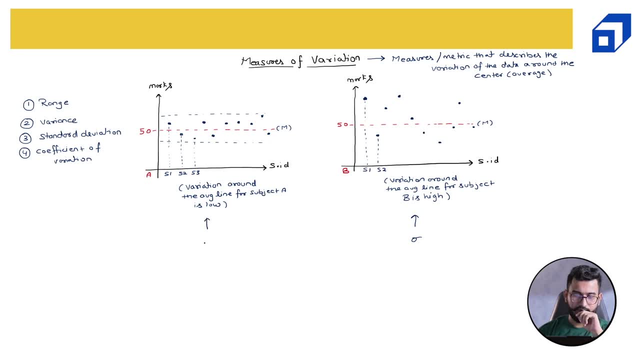 While for B- sorry for A, which is this case- I would get the value of sigma, which is standard deviation. This is going to be low. So if I call this as sigma A and sigma B, then my sigma A would be less than sigma B. 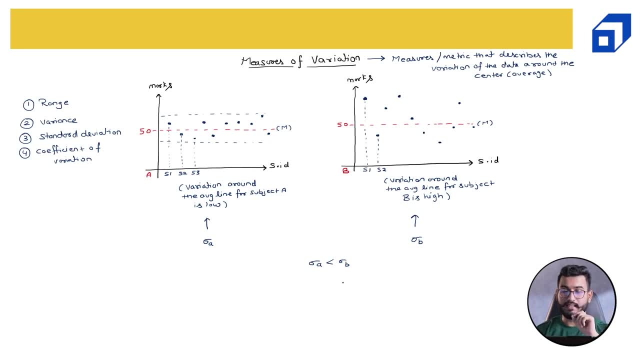 The standard deviation in subject A would be less than standard deviation in subject B. When I say the standard deviation is less, that basically mean all the observation or most of the observations are scattered very close to the mean, While when I say standard deviation is high. 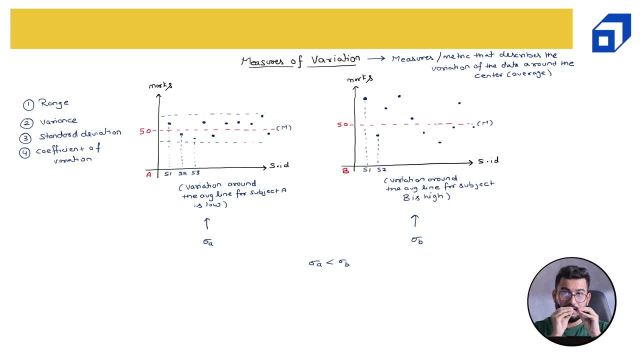 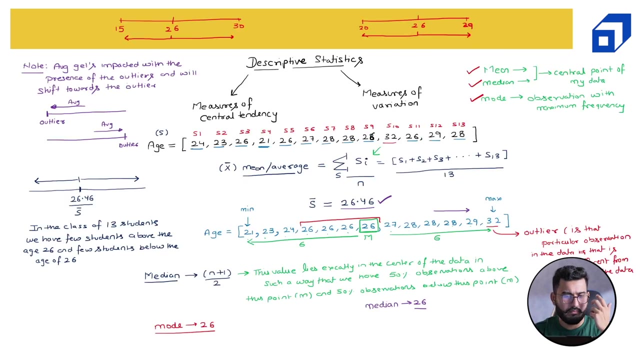 that basically mean most of the observations are scattered far away from the mean. Now, this gives you a better idea regarding how your data looks like. If you guys want to practice, you can see that we have already calculated the mean, median and mode of the age variable. 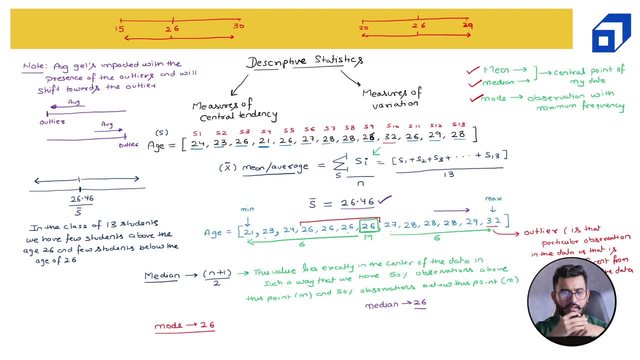 We were having 13 students and their respective age. We have already calculated mean, median and mode. Now for practice, what you guys can do. you can quickly calculate the standard deviation of this particular data and then you can try to understand it. 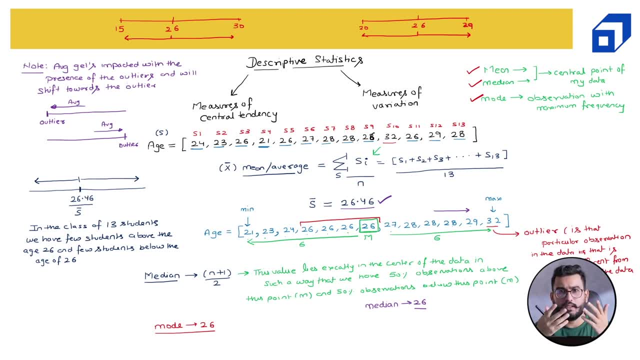 So if you have to explain to the principal or to any person about how this class looks like, So we have already seen one segment that this class is having The median to be 26,, which basically mean 50% people or 50% students fall below the age 26 and 50% fall above the age 26.. 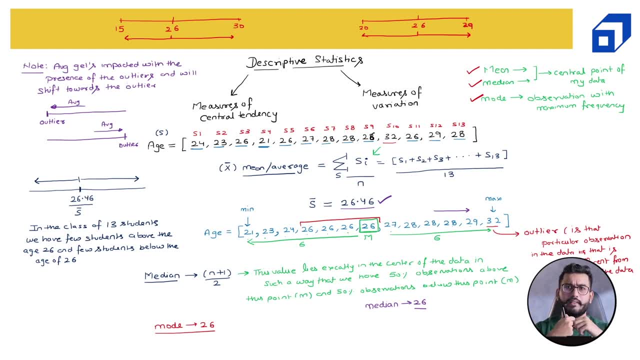 Now, if you get the standard deviation of, let's say, five years, I'm just throwing a value, I have not calculated it, So I'm just giving you this task to calculate this. But let's say, if the standard deviation of this data is. 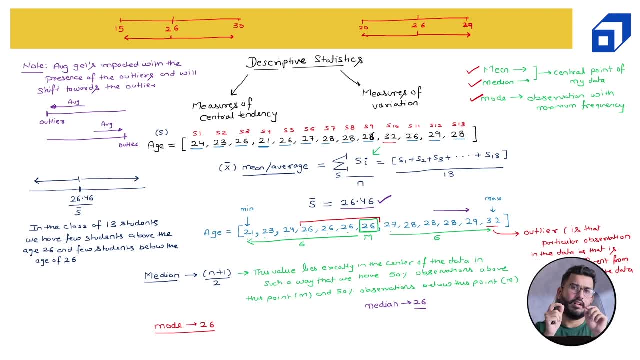 five years, then that basically means on an average, on an average, the students are having five years above the above the central point, which is 26.. So let me just quickly draw it. So let's say this is my student ID. 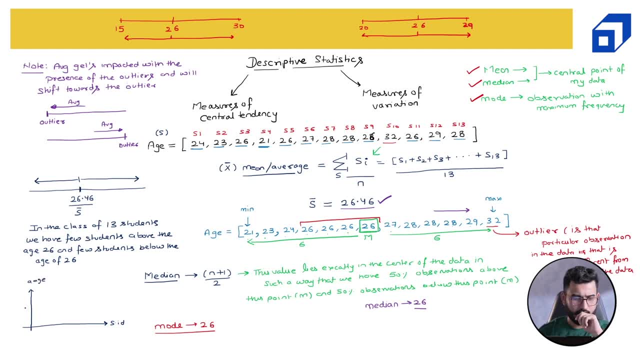 This is my age, This is my center, which is 20.. This is 26. And if I'm having a standard deviation of five years, that basically mean I'm having few students who are above the age, above the middle age, by five years. 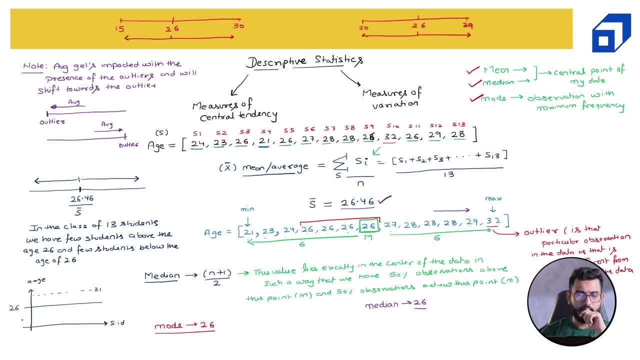 So 26 plus five will give you 31.. Right, And 26 minus five will give you Twenty one. So you can see that. you can see that most of the students in your data are between twenty one to thirty one Right. 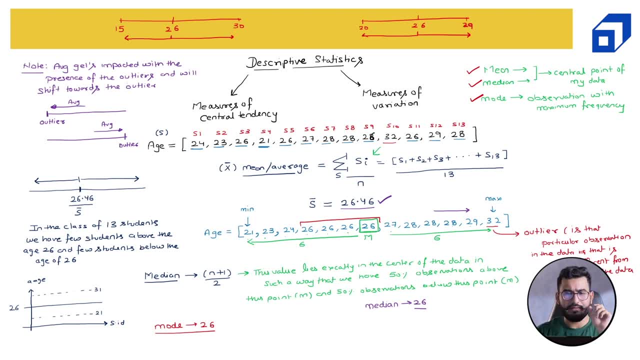 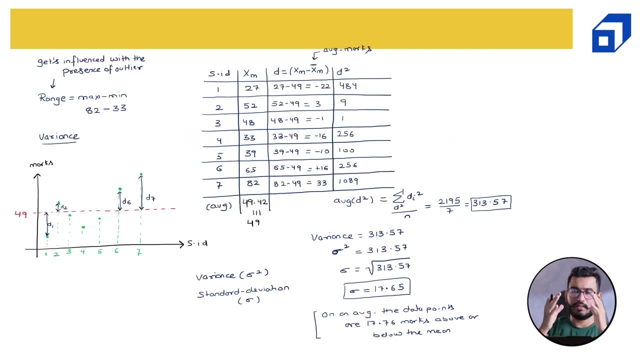 So, using the measures of descriptor, measures of central tendency, we get the central point. using the measures of variation, we get how the data is scattered around the central point. But there is a problem. The problem is, let's say, if I'm having two subjects, let's say I'm having a subject. 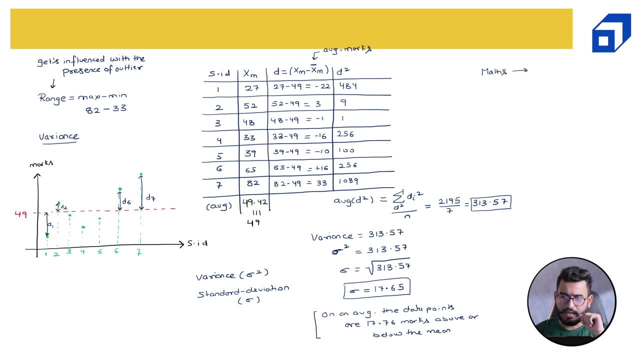 of maths, Oh, having a standard deviation of, let's say, 15 marks. And then I'm having age. Having a standard deviation of, Maybe- let's say I'm having another subject, Another subject, science- Having a standard deviation of, let's say, 20.. 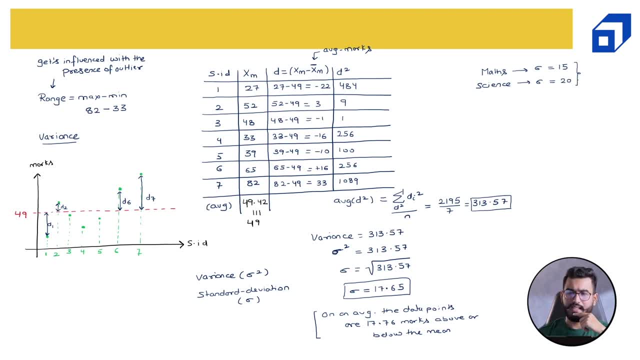 Now can I compare these two standard deviation? Can I say this is high and this is low? Well, we cannot do that using a standard deviation. We cannot compare the variations among the series. Now, please remember- this is a very important note- that a standard deviation 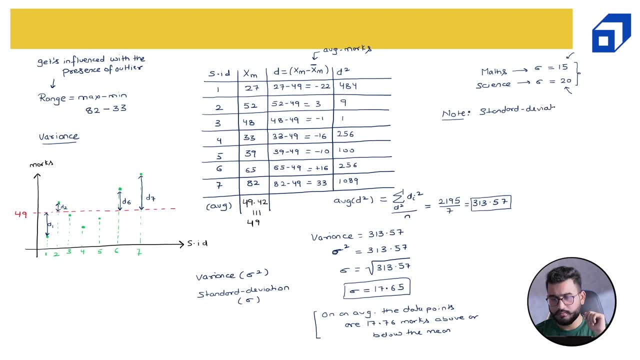 The standard deviation Talks about The variation In the individual series, Individual series, And we cannot Use it To compare The variation Among the series, The variation. So how we can compare the variation among the series? For this we have the next measure, which is coefficient of variation. 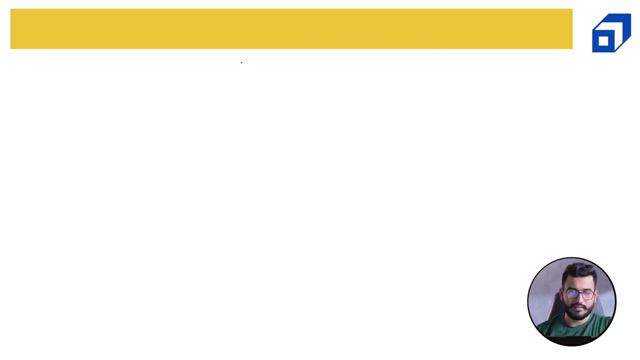 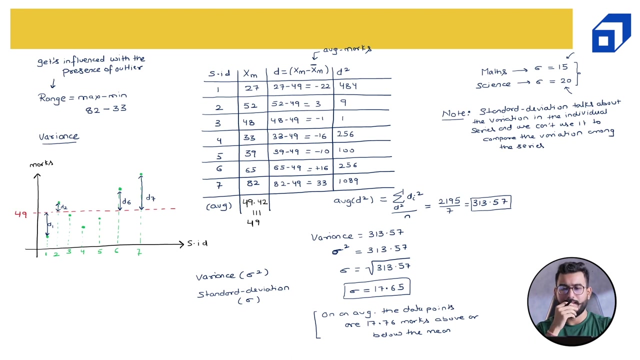 So now let's try to understand coefficient of variation. Coefficient of variation, As I've told you, the standard deviation is limited To describe the variation Within that series. So if I'm if I'm saying that the standard deviation of the maths marks is 50, 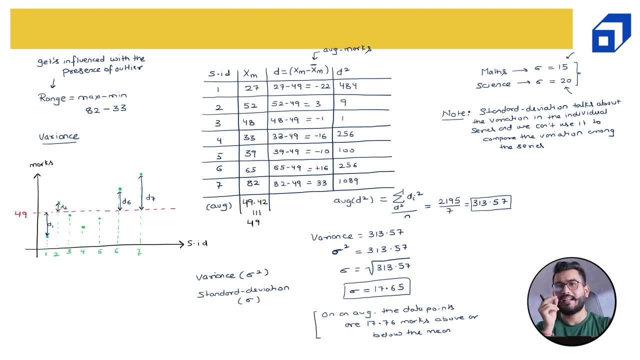 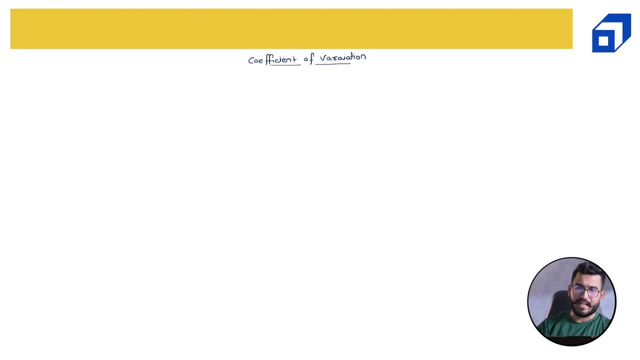 and the standard deviation of science marks is 20.. I cannot use these two individual standard deviations to compare the variation among the series. For that we have a different metric Known as coefficient of variation. Let's take one example. Let's take two series. 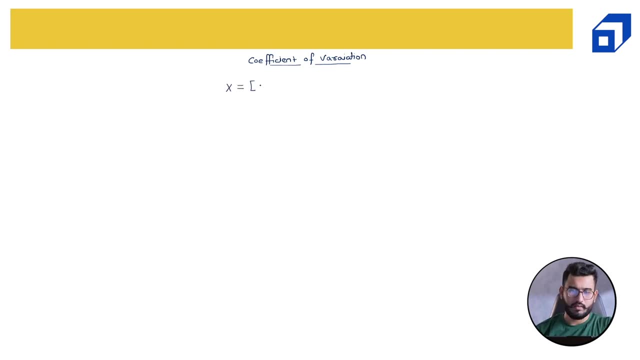 Series X, which is having One, two and three three data points. Series Y, which is having again three data points: One not one, one not two, one not three. Now, if I take the average of X, which it will come out to be to average of Y, 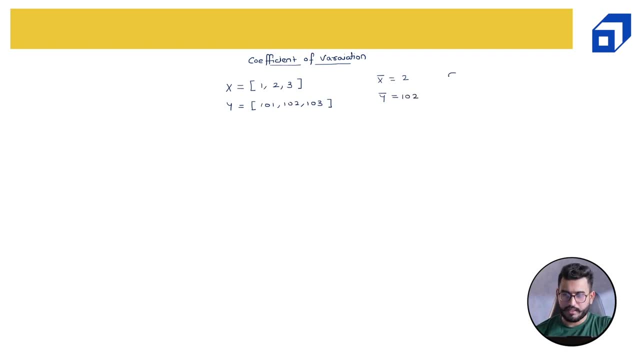 will come out to be one, not two. Similarly, standard deviation of X will be 0.8 to one. Standard deviation of Y will be 0.8 to one. Now, both X and Y are having the same standard deviation. Can I say that they have the same standard deviation? 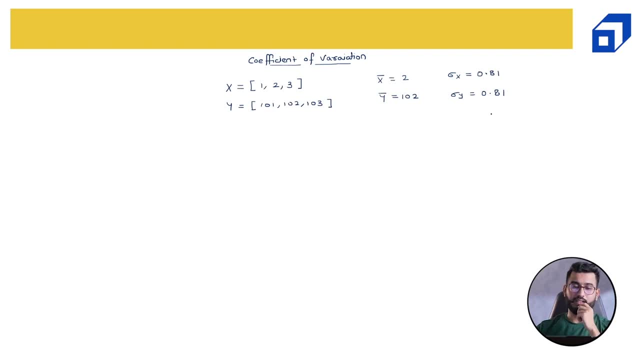 Or can I say that they are having the same variation? If you closely observe, you will find out that This is not true, While in the series X, you can see that the third element, which is three, is three times of the first, while in series Y. 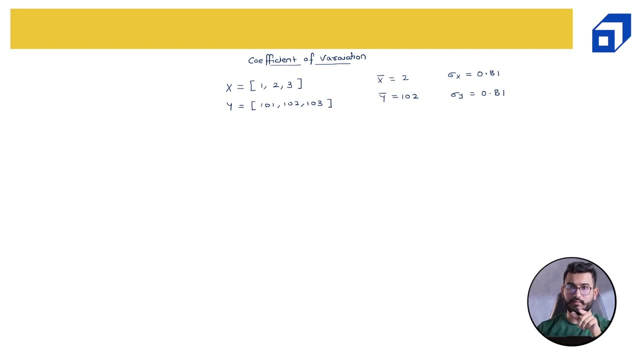 I cannot say. the third element is three times of the first Right, So they both are not having same variation. X and Y are not having same variation. How we can compare the variation, How I can see that X is having more variation, Y is having less variation. 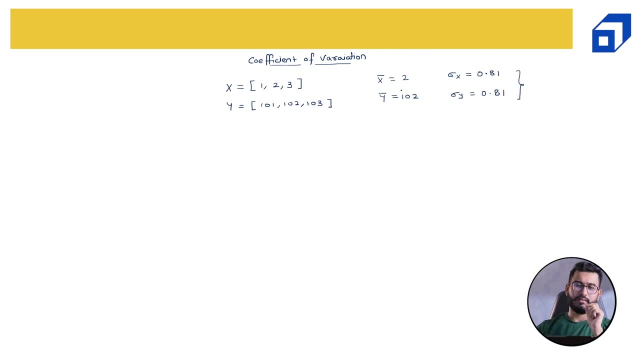 because the standard deviation is getting us the same value: 0.8 to one, 0.8 to one, How we can get or how we can compare. for this, we have coefficient of variation, which is nothing but the ratio between the standard deviation to the mean of the data. 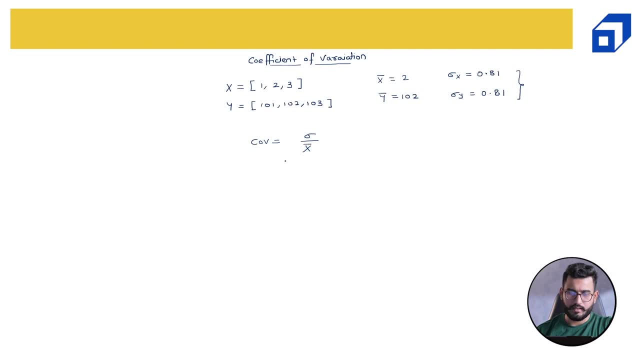 the standard deviation to the mean X bar For coefficient of variation for series X Would be 0.81 divided by two. for Y, It would be 0.81 divided by one, not two, So this would be 0.405.. 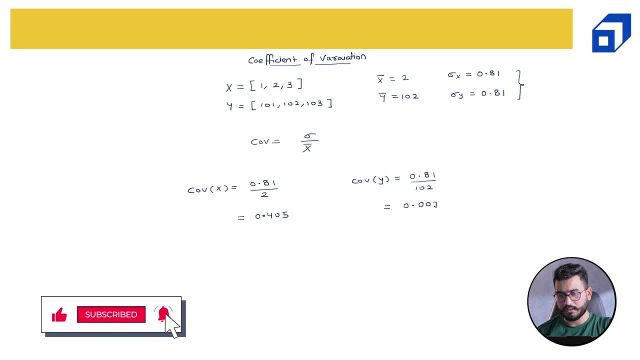 And this would be 0.007.. Now, if we closely look into these two values, which is 0.405 and 0.007.. This particular series, which is series X, is having the coefficient of variation of 0.405, while series Y is having the 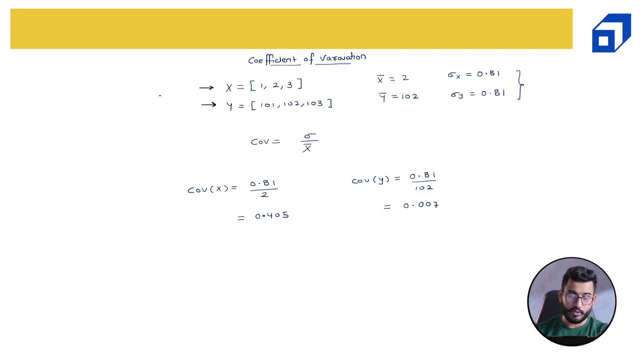 coefficient of variation of 0.007.. And I have already told you that the series X is having more variation than series Y, because in this series the third element is three times the first, While I cannot say the same thing for series Y, right. 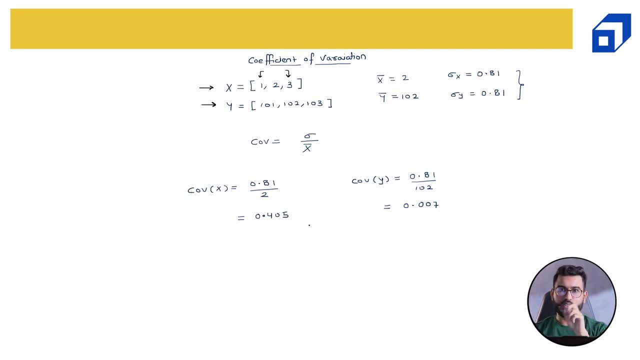 So when we have to compare two series or we have to compare the variation among two or more series, we look at the coefficient of variation. A higher value represents higher variation. So this series is having Higher variation When compared, When compared with. 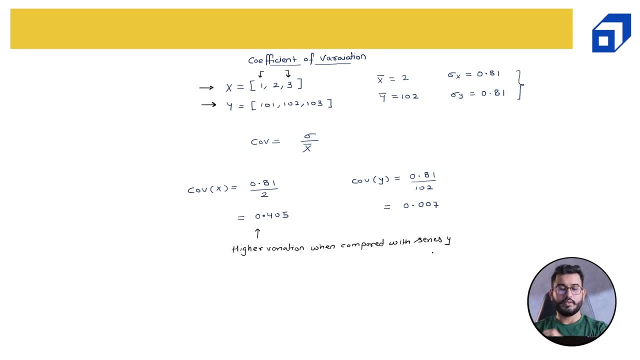 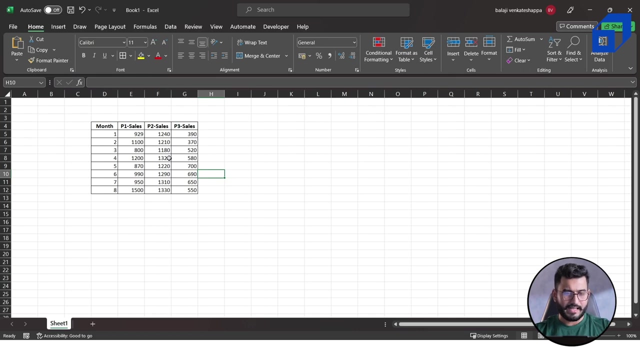 Series Y. So using coefficient of variation, we can simply compare the variation among the series and we should not be using a standard deviation. I hope this makes sense Now. here you can see I have taken one simple example and here we'll be using 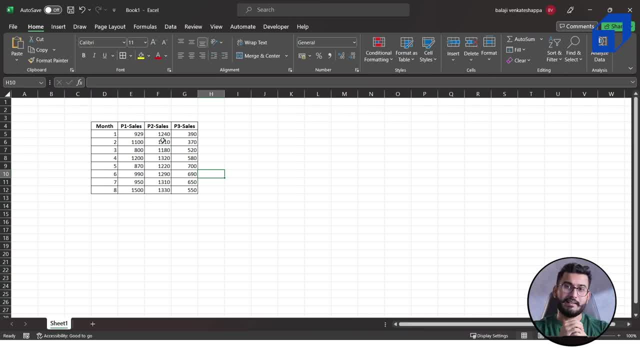 all the measures, which is, measures of central tendency and measures of variation, to understand how these three products are performing in terms of sale. And please remember, this is the number of units. So for product number one in month one, nine hundred and twenty nine units were sold. 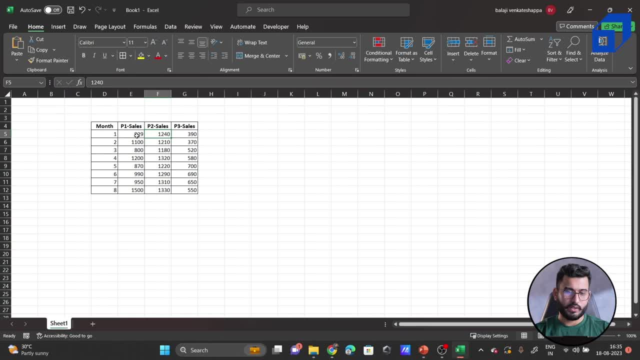 Similarly for product two in month, one, twelve, forty units were sold, and so on. So we can quickly find out. The average Median and mode for each of them is equal to average Average of this particular column And I can simply extend this formula to all other sales. 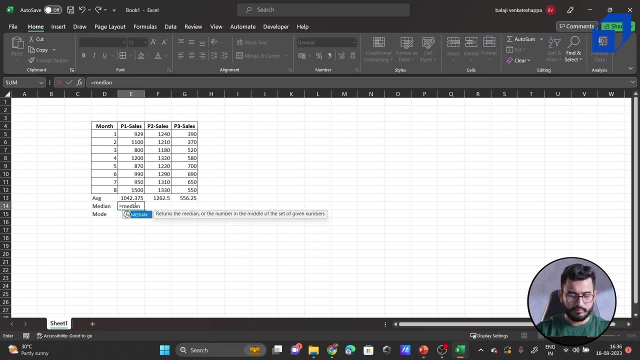 Similarly, median will be is equal to Median. I want median of all these Sales And I can simply extend This to all other sales, and then we have mode. so is equal to mode. Now, here, if you carefully observe, I do not have any mode. 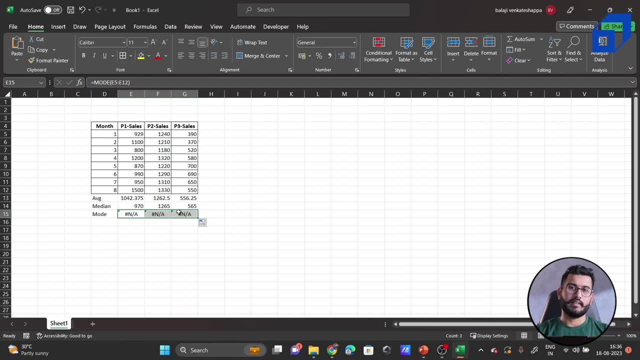 So my mode is not available and I have told you previously. So if I do not have any observation, which is which is duplicate or which is repeated for more than one time, which is having the highest frequency in our data, we will not be having a mode. so we only have average and median. 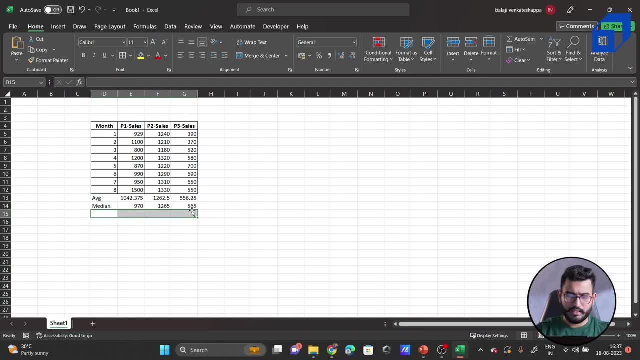 So I'll simply delete this because we don't have a mode, so let me delete this Now. if you compare the average and the median, you can see that for the sales of product number two, the average and the median is quite close. 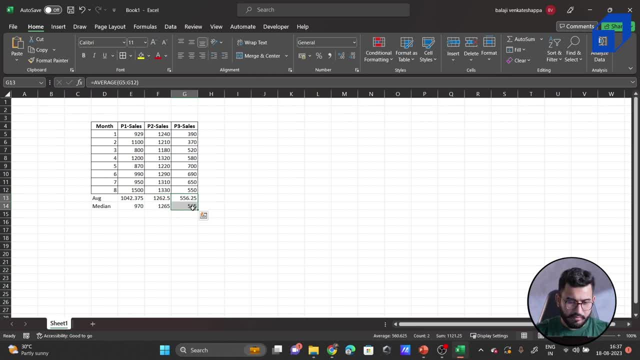 to each other, while the same thing can be viewed for product number three. But there is a difference. There is a vast difference. I would not say vast, but there is a quite a good Difference in the average and the median for product number one. 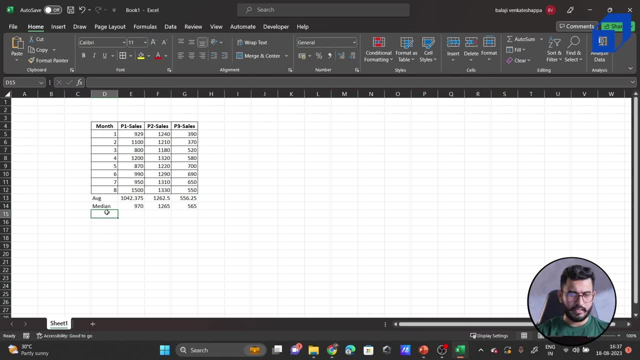 Let's try to look at the measures of variation also. so we will calculate the A standard deviation, So Is equal to SDDV, and we will use this SDDV, this one A standard deviation, And I can just simply: 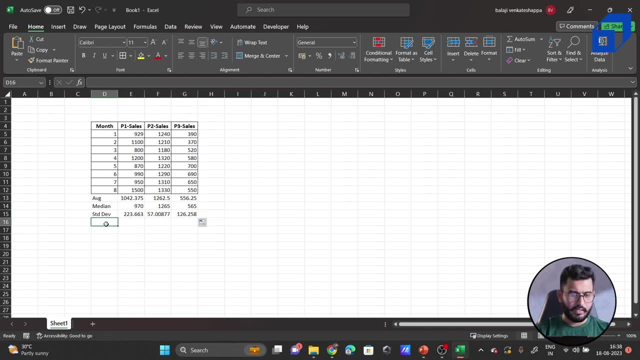 Extend this, And now we will calculate the coefficient of variation, COV. So this is given as the standard deviation divided by its average. Now, these are the numbers, which we have to carefully read and make sense out of them, What we can conclude about these three products. 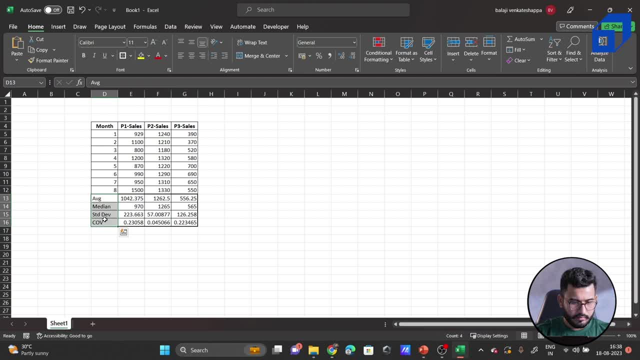 Let's try to understand them Now. if you carefully observe- and I would start with product number two first- In product number two you can see that the standard deviation is very small, While the coefficient of variation is also very small. Here also you can see that coefficient of variation is 0.23. 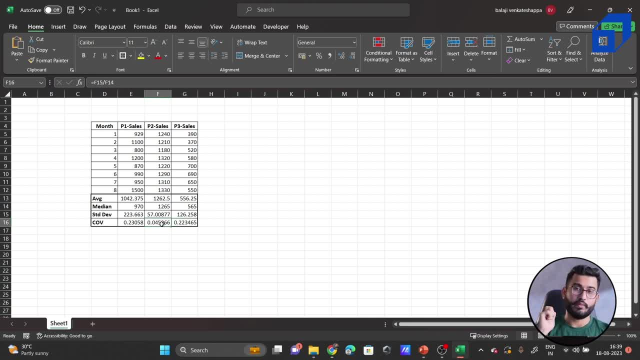 Here it is 0.22.. But here it is 0.04, which basically mean among all these three series, the lowest variation is with the sales of product number two. Also, if you look carefully, the median and the average is very close to each other. 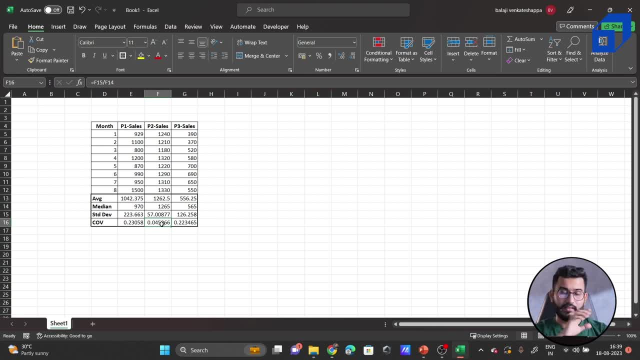 Also, the average is highest Among all the three products. So what I can conclude about product number two? number one: the product number two is very stable in the market because it is not. it is not having variations in month number one, same sale in month number two. 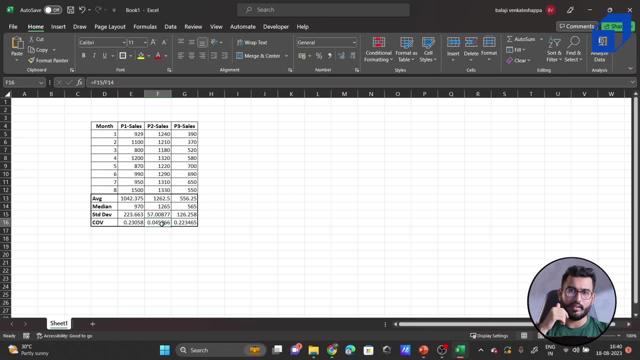 approximately same sale, month, three same sales, and so on. Also, it is always consistently high And that is the reason that average is the highest, at 1262.5 units. For product number three, a similar behavior can be seen, but on the lower side. 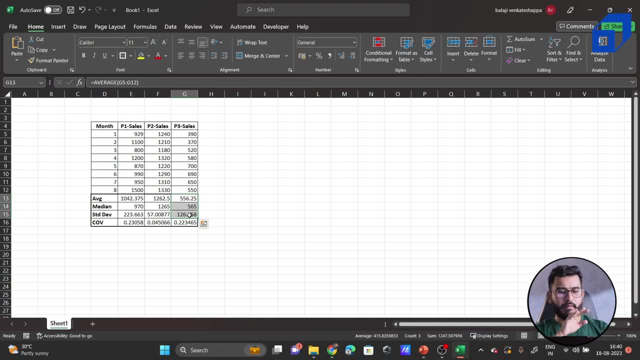 the average is 556,, which basically means, when compared with product number one, product number two and product number three, when compared with product number one and two, the sales of product number three is on the lower side or the lowest side, while the coefficient of variation for this, which is product three and product 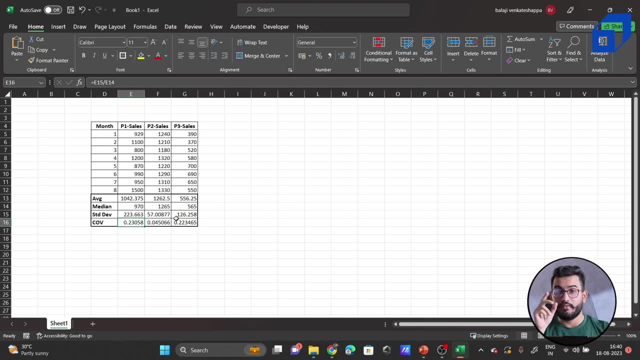 one is approximately the same, which basically means They both are varying at the same rate. The variation is approximately the same. So you can you can assume that one, which is product number three, is on the lower side and it is varying around that product number one is on. 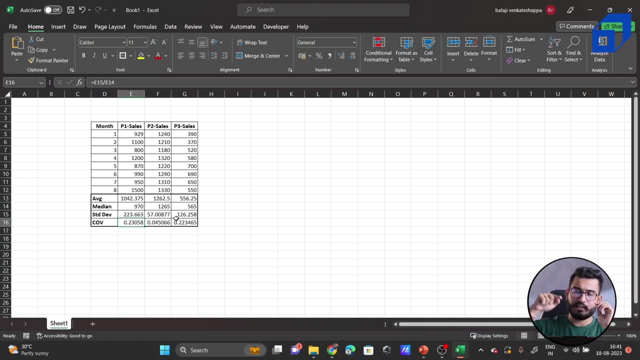 is on maybe second lowest and varying around that, And product number two is on the highest. So if I just color code them, I would say product number three would be coded as red product, one I can put it as yellow and two I can put it as green. 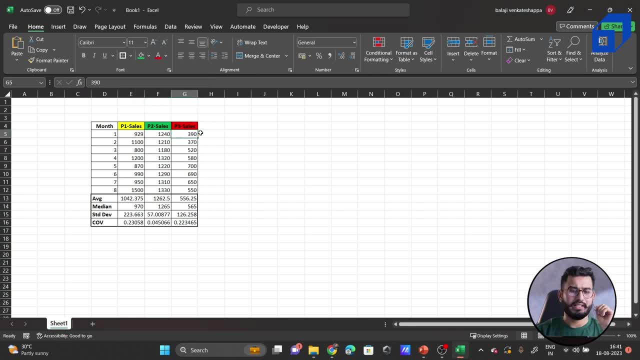 And the reason I'm putting it as green because it is the most stable product in the market, while sales of product number three is on the lower side. That's the reason we have assigned a red color, And product number one is having the sales between the highest and the lowest sale, which is product two and product three. 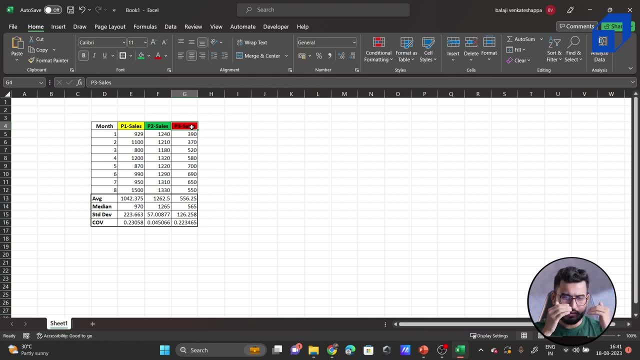 So we have assigned a yellow color. Now you can see that, using these measures, we can better make conclusions about the data, We can better explain the data, And that is the power of descriptive statistics. So you have seen that in this particular descriptive statistics segment, we have talked about how we can explain the data. 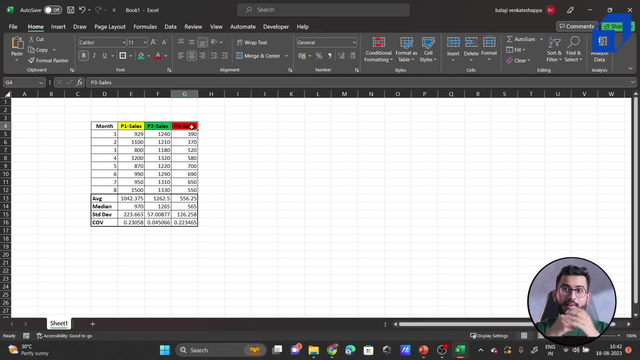 We have talked about the various types of variables. We have talked about qualitative, quantitative, right. Then we started our discussion around what are the various measures of central tendency. We talked about mean median mode, Then we compared all of them. Then we talked about measures of variation, where we looked into range. 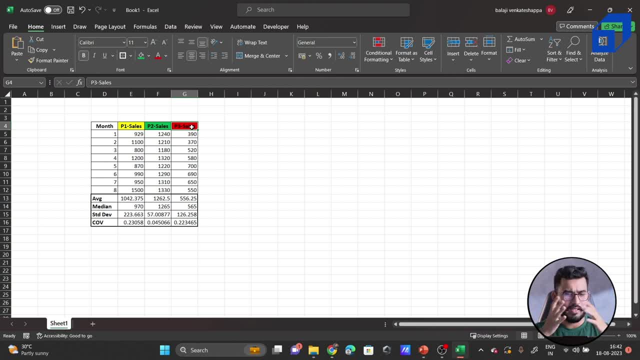 variance, standard deviation, coefficient of variation And, finally, we have concluded all our learning into this table, where we have compared the sales of these three products to conclude about which product is better and which product is not good. Now, this is what the application of descriptive statistics is. 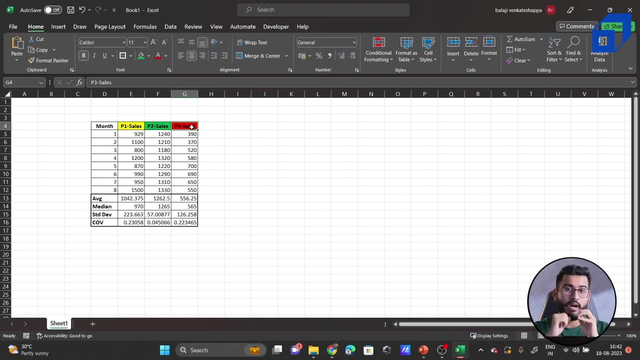 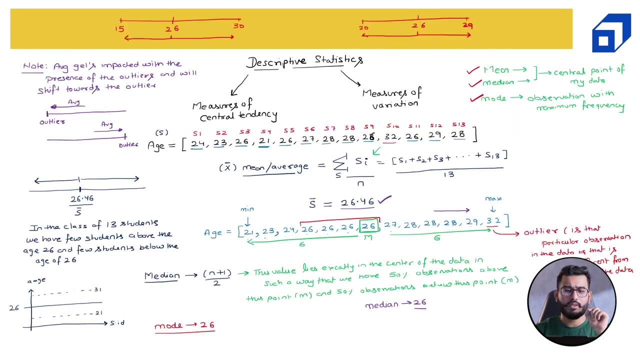 There is one small topic which is very related, related to outliers. I'll just quickly explain you that, Though that is not so much common in the in the descriptive world, but quite important to understand, I have told you about outliers right Over here. 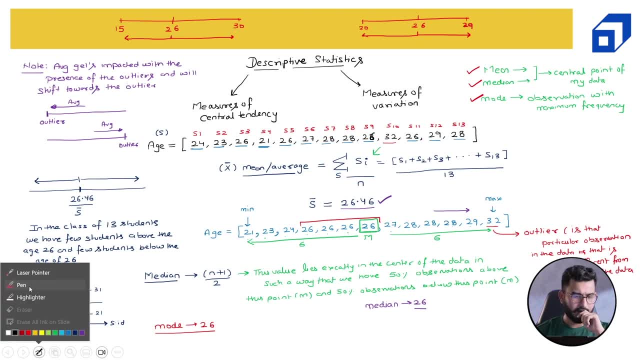 So I have told you that in this particular series where we have the age, 32 is considered as outlier. And what is outlier Outlier is that observation which is very different from majority of the data. Now, there is one particular topic which is known as the leveraging point or leveraging data point. 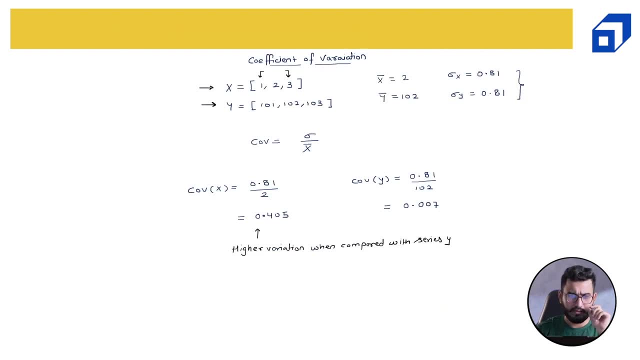 What is that? Let's take one very small example. So let's say I have this data And this is the stock price. So here we have the day of the month And here we have the stock price. Stock price of a particular stock. 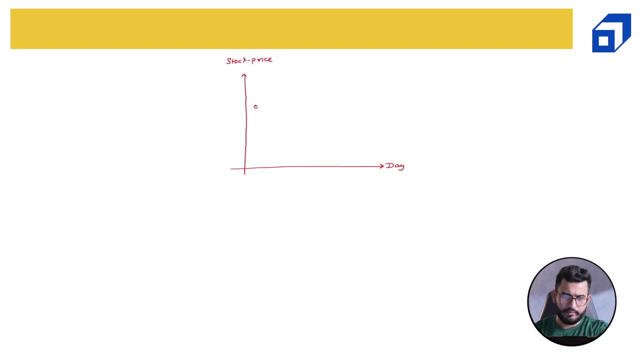 Let's say, on day one the stock price was somewhere around here, Then over here, then over here, then here, then here here, And one day it jumped over here, One day it jumped over here, then came back to its normal position like this: 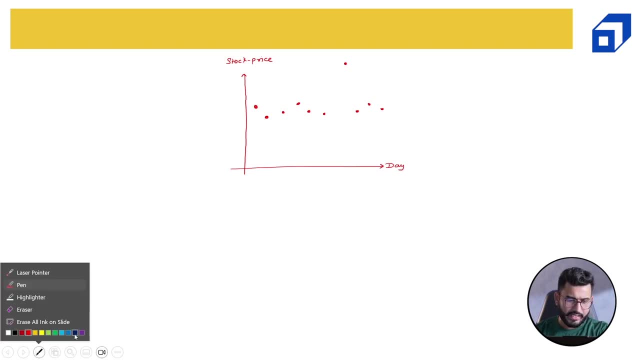 Now, at the very first like, if I provide you with this data, all of you will say that this is outlier, This is outlier. This is particularly the outlier data point, which is true, This is outlier. But as soon as I provide you one additional information, 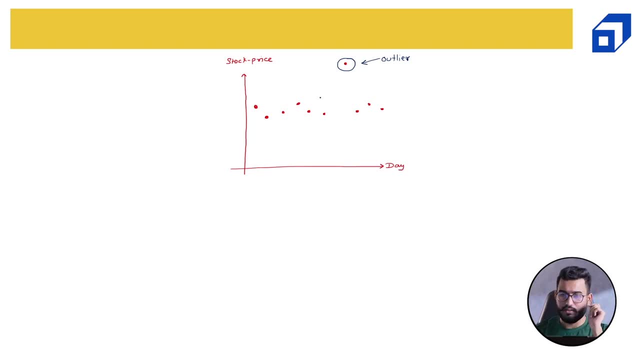 your answer will change. Now, if I told you, if I tell you that on this particular day, let's say this is day day number 15th, or maybe let's say day number 25.. So in the 25th day, 25th day. 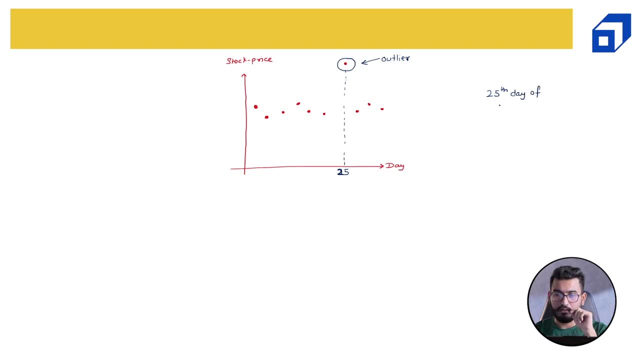 25th day of month. month, let's say March 2023,. let's say the stock market, or the stock exchange, Stock exchange. or let's not talk about stock exchange. let's say this company. let's say this is the stock price of the company Reliance. 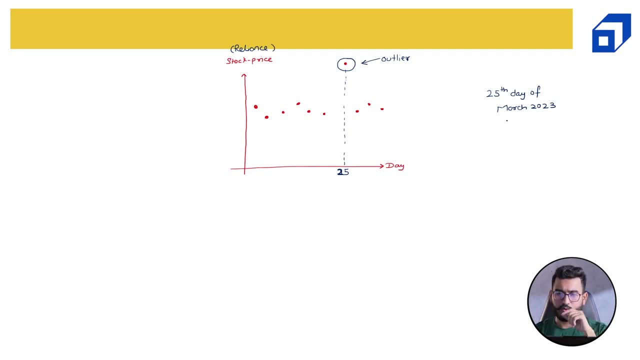 Reliance. So, on 25th day of March 2023, Reliance announced a major product, Announced a major product, announced a major product, or they made, they basically conducted a conference. they conducted a conference, they conducted a meetup in which they announced: 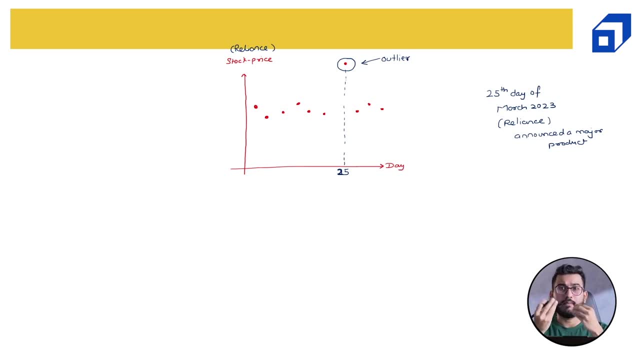 a major change in their policy, a major change in their product, due to which the stock price suddenly raised to this particular point. Now, this is not an outlier. this is the leverage data point, because it has been leveraged due to this event. 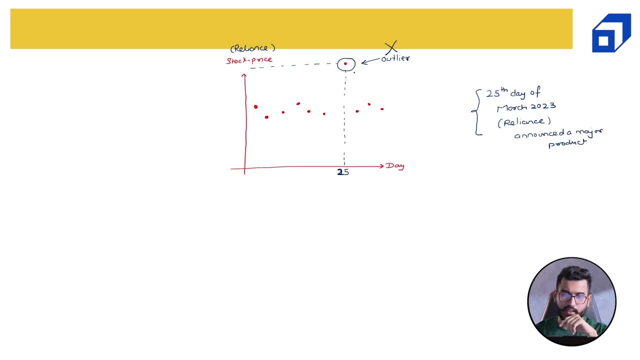 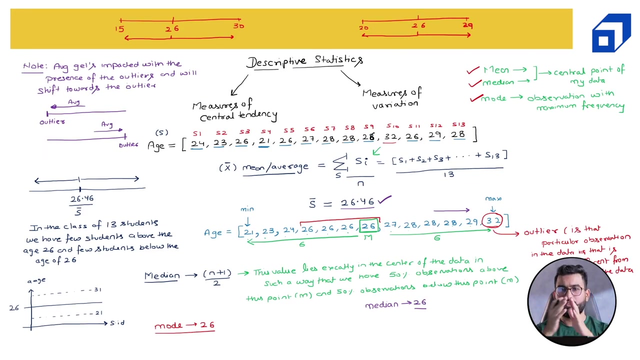 So I cannot say this is an outlier. I cannot say this is an outlier, This is a leveraged data point. So there is a difference between outlier and leveraged data point. If I go to this particular example of age, I cannot say this is leveraged data point because this person has not or the age. 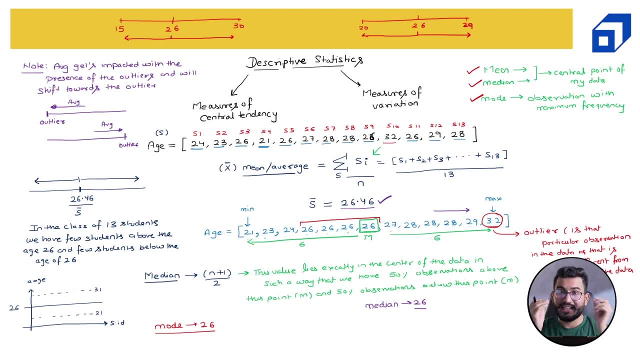 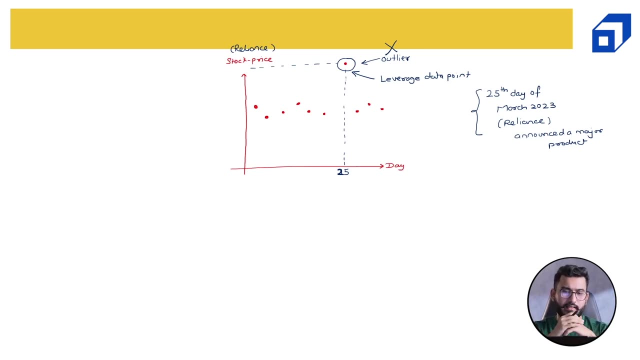 of this person has not been impacted by any external factor, So I cannot say this is an outlier. this is a leveraged data point. This is just an outlier. But in this case, where we are considering the sales of a particular stock price or stock price of a particular stock, let's say, Reliance- 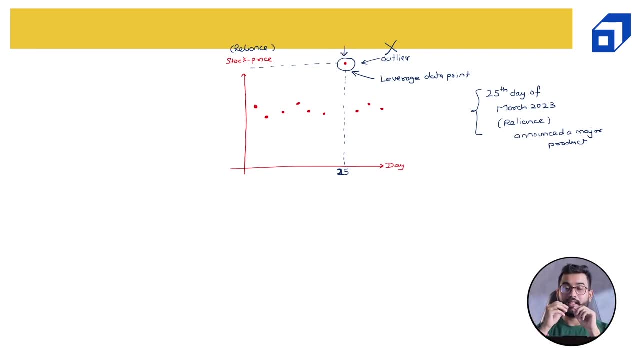 this data point is the leveraged data point because it has been, it has been influenced. the jump is because of a particular external factor which is nothing but the announcement Right. So I hope you guys are clear till this point. Now we will move forward to the next particular discussion, which is probability. 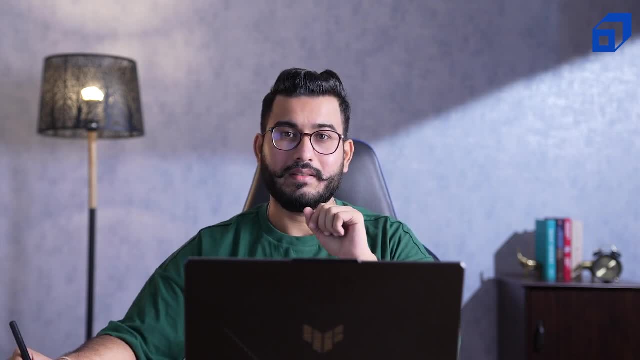 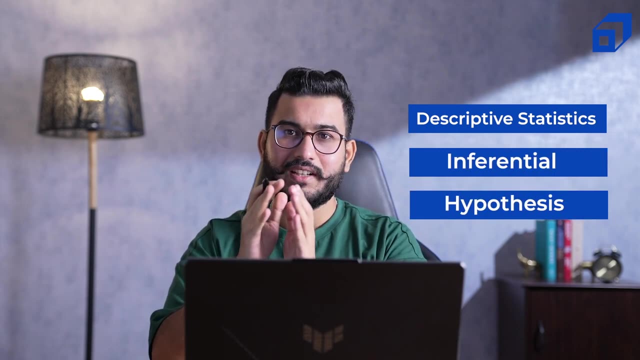 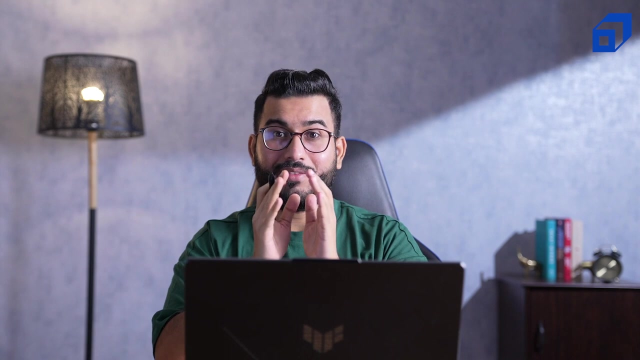 So now let's start with the topic probability. Now we started with descriptive statistics. We have to talk about inferential and hypothesis. But before we can move forward to understand inferential and hypothesis, we have to first of all understand what is probability. 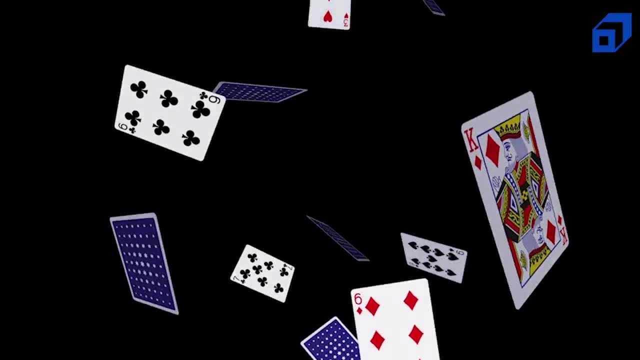 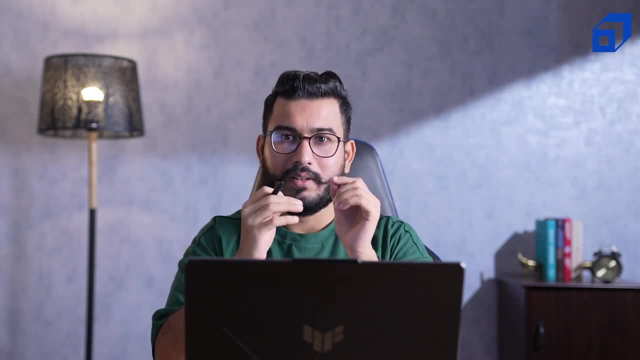 You guys must have learned about it anyway, Maybe in your 10th standards or maybe in your college days. But today we will try to understand the most important topics within probability, which will help you to understand inferential and hypothesis. So let's start understanding probability. 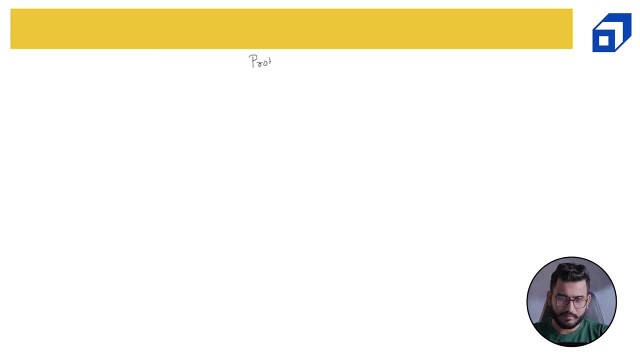 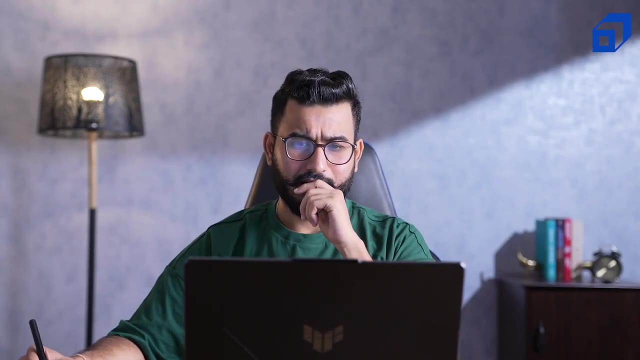 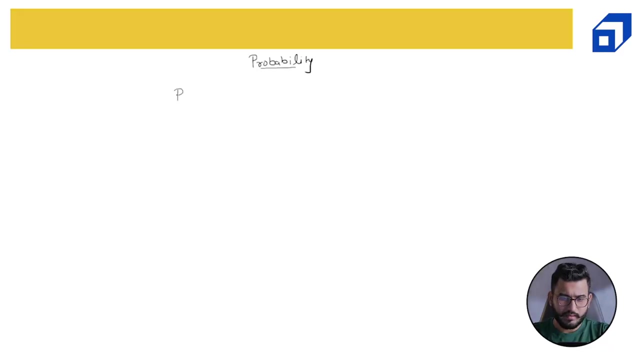 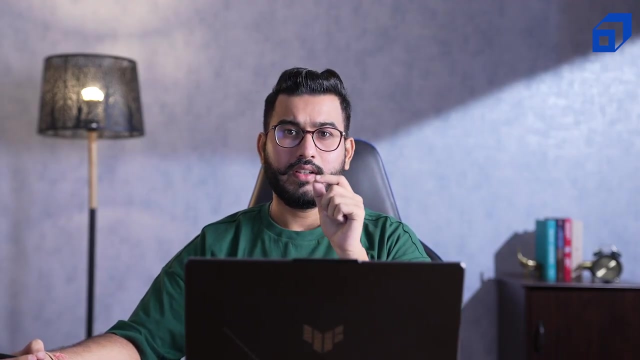 Now the term probability. Most of you are familiar with this, so before we talk about probability, we have to understand What is a random experiment, Random Experiment? Random experiment is a particular experiment in which you are not certain about the outcome. 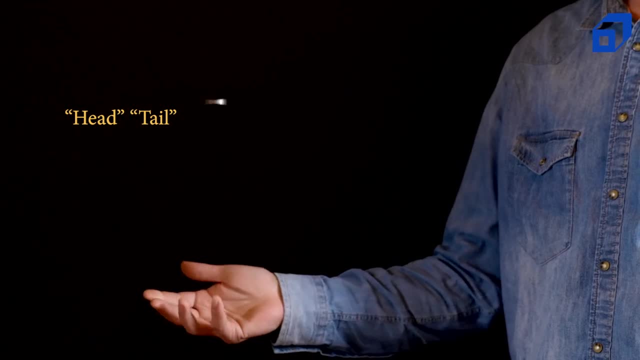 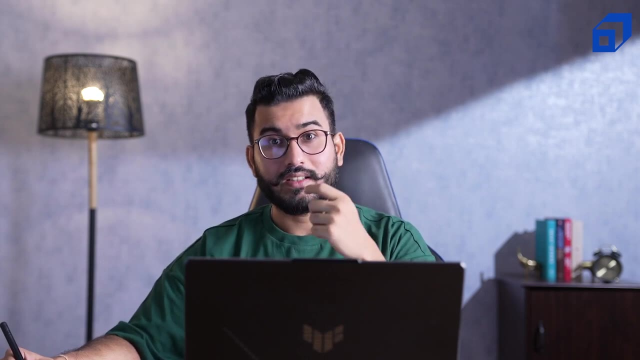 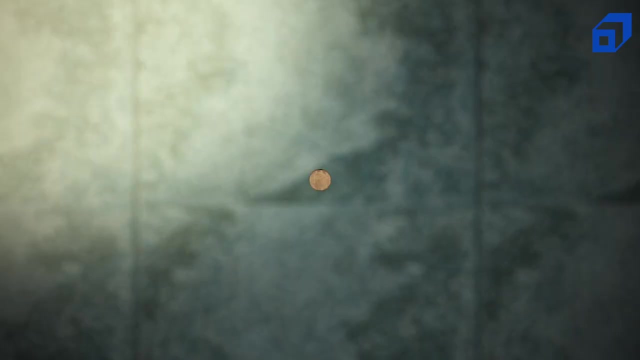 For example, if I toss a coin, I am not certain If I will be getting a head or a tail Right. If you are certain about it, then we don't need probability Right. So let's say, if I already know that the coin is going to land as head, 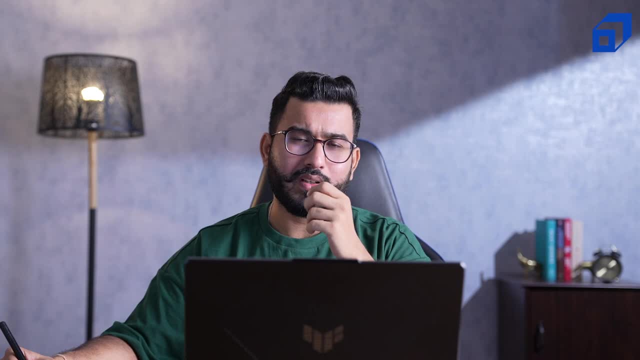 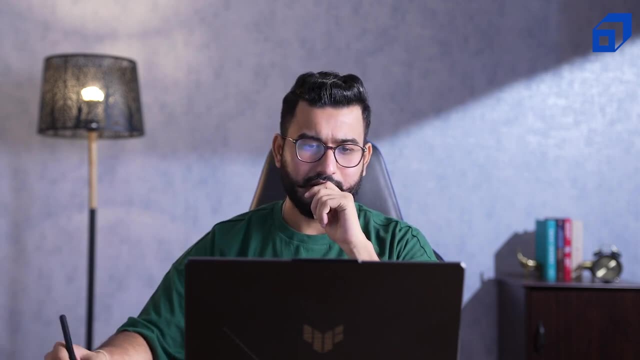 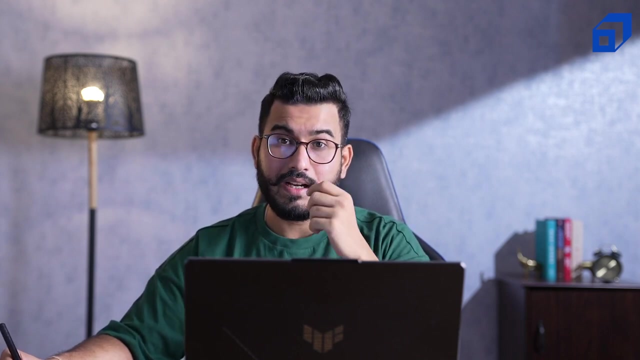 then I don't need probability, because probability is all about finding out what is the chances of getting a particular event Right. So what is a random experiment? It is something or it is. it is basically an experiment or an event For which I am not sure about the outcome. 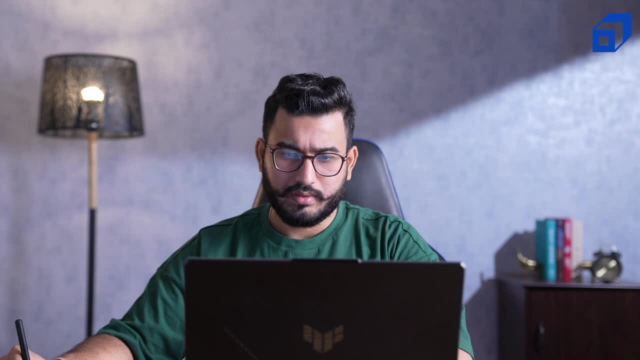 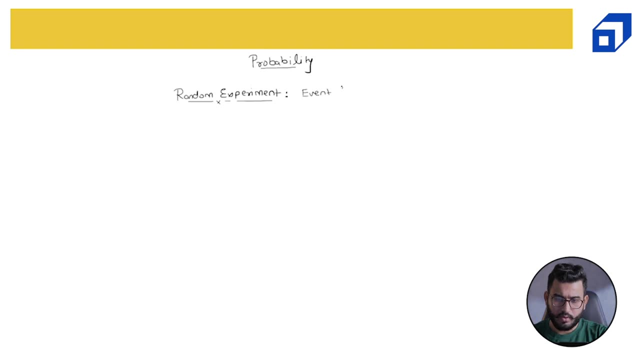 I am not certain about the outcome, So let me just quickly note it down. It is basically an event For which I am not Certain About the Outcome. For example: roll, roll off a dice, Roll off a dice. 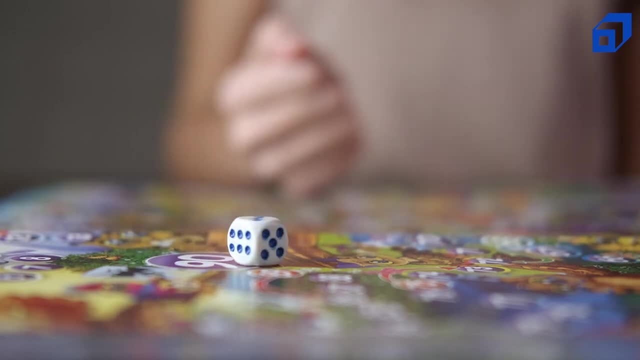 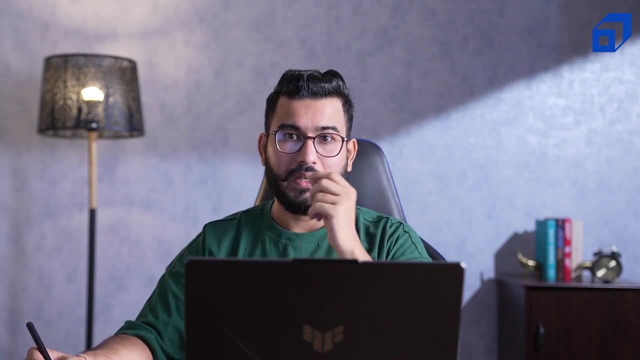 Now, if I roll a dice, I know that I may get one. So either one, two, three, four, five or six. But am I certain that I will be getting a one? No, Am I certain that I'll be getting a two? 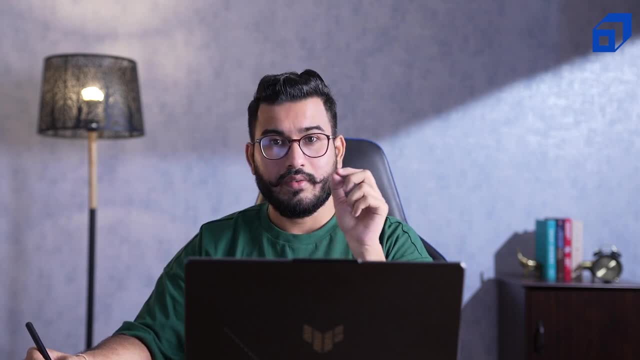 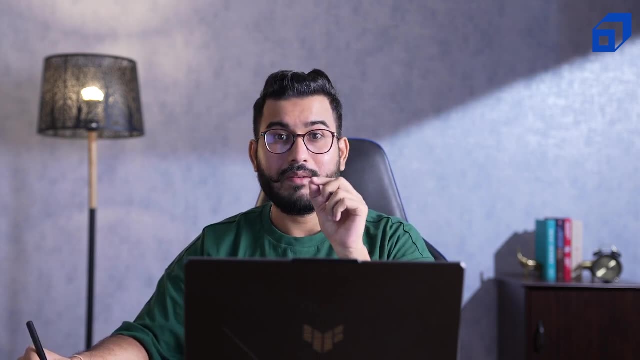 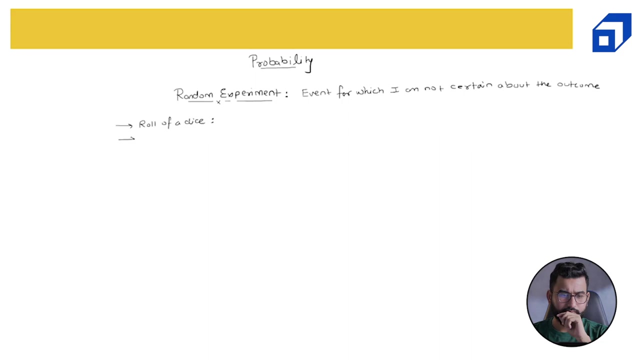 No, I may get any of the outcome within one, two, three, four, five, six. So rolling a die is particularly a random experiment because I am not certain about what is going to be my outcome. Similarly, let's say about my birthday. 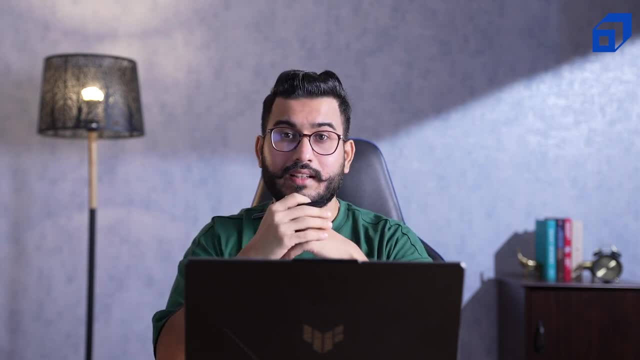 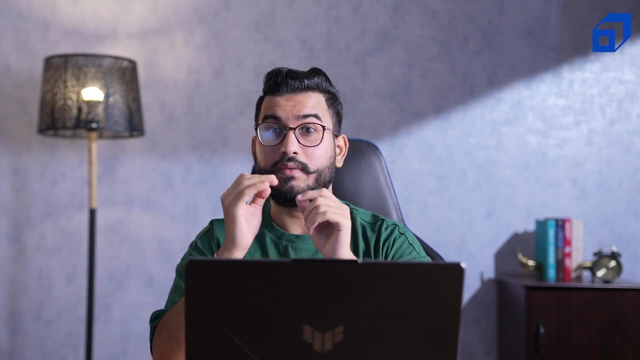 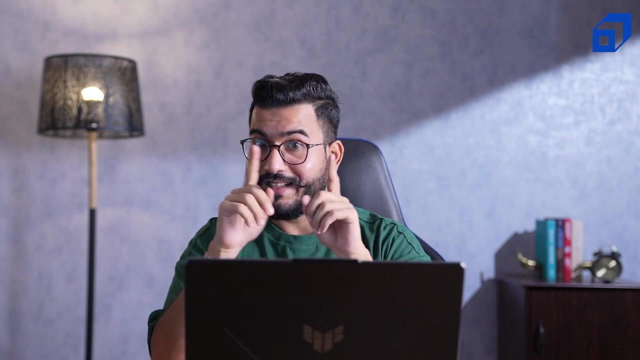 So now you are not certain about what is my birthday. but there is a difference. If I talk about my mother, she is very much certain about what is my birthday. So for my mother, My birthday's birth date is not a random experiment. but for all of you listening, 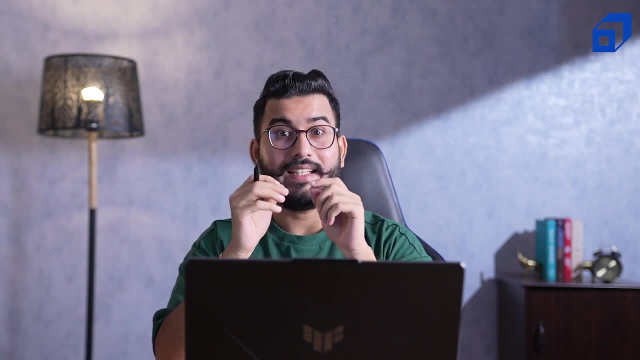 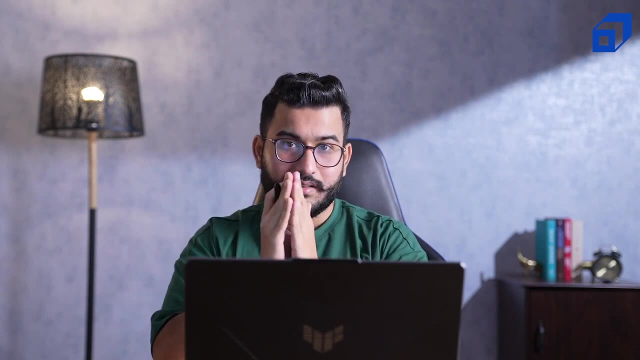 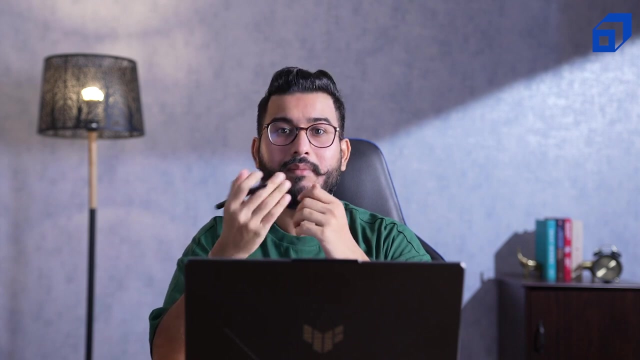 my birth date is a random experiment because it can be anything. It can be any year, it can be any month, it can be any day. So sometimes a random experiment, or the uncertainty is maybe because of the lack of information, for example, my birth date. 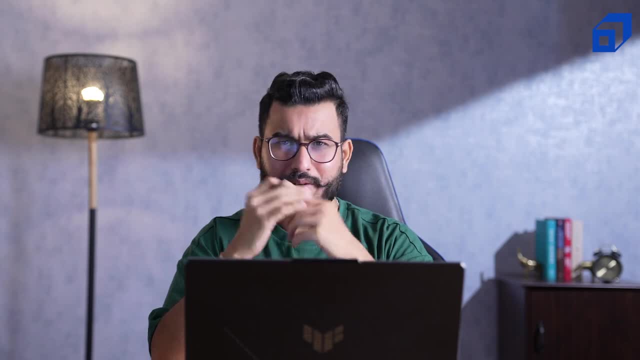 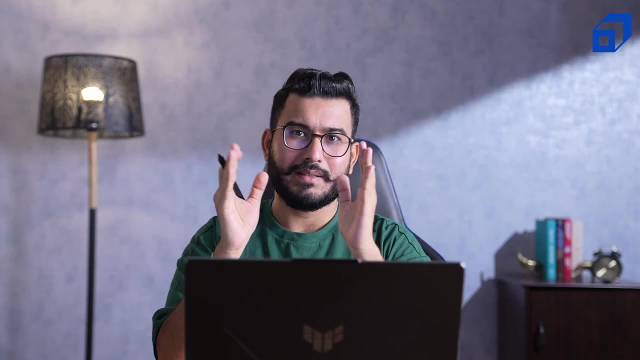 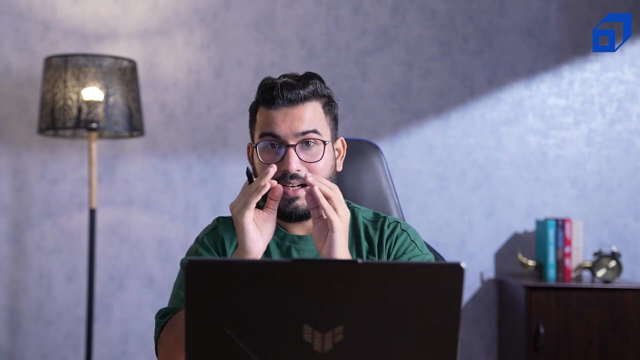 If you know about me, if you are my friend, then you might be very much certain that my birth date is in this year, this month and this date. So there is a difference between a random experiment, which for which you are uncertain about the outcome, and some event for which you are certain, like my birthday. 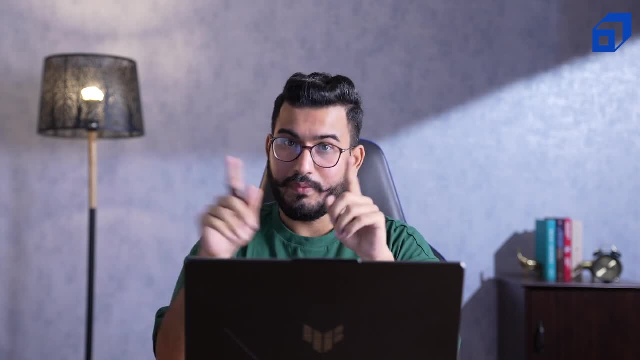 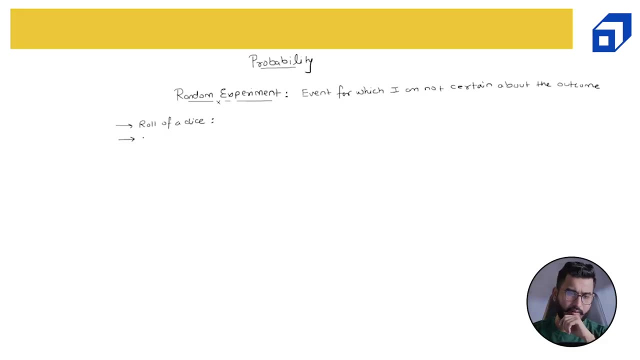 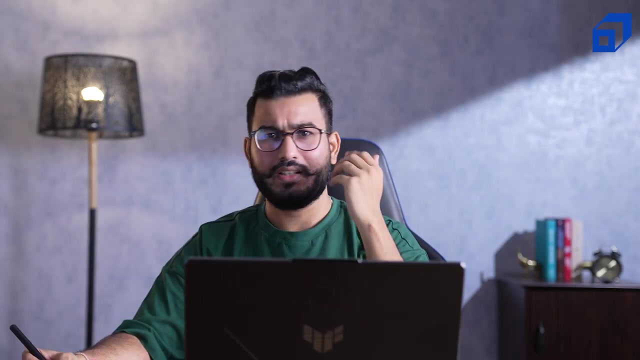 So that is not a random experiment for my mother, But for all of you it is a random experiment. So I'm just taking example of all the random experiments- Roll of a die or maybe Toss of a coin- And we can note down all such random experiments. 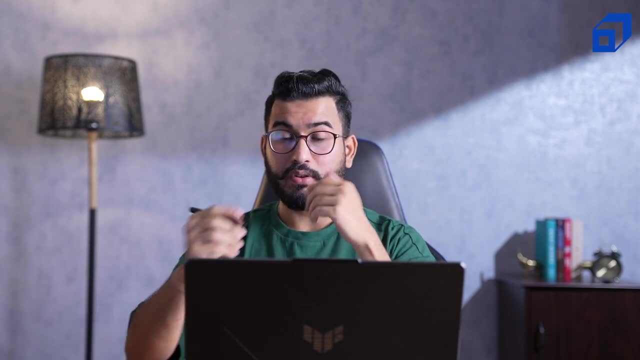 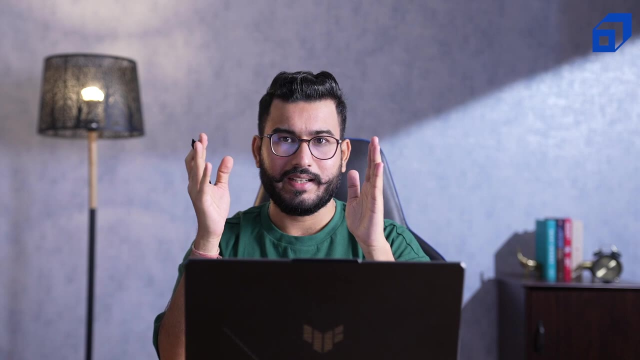 Now, what is a sample space? As I was talking about that, when you roll a die, you may get any of the outcome within 1 to 6, right? So 1,, 2,, 3,, 4,, 5,, 6, you can get anything. 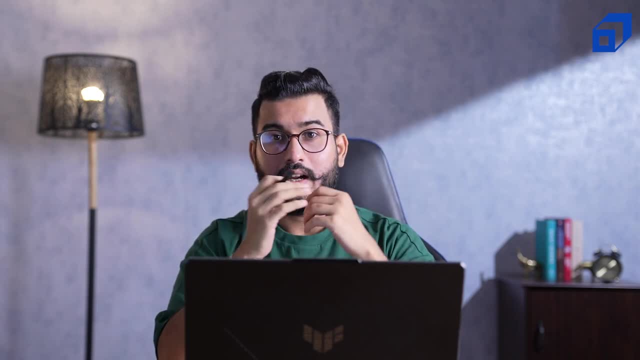 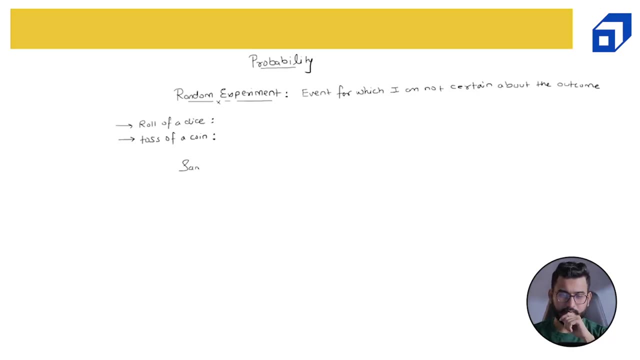 The set of all the possible outcomes out of an experiment is known as the sample space. So what is the sample space? The set with all the possible outcomes out of an experiment. So if I take the example of roll of a die, I may get 1,, 2,, 3,, 4,, 5,, 6, you can get any of the possible outcomes out of an experiment. So if I take the example of roll of a die, I may get 1,, 2,, 3,, 4,, 5,, 6, you can get anything. So if I take the example of roll of a die, I may get 1,, 2,, 3,, 4,, 5,, 6, you can get anything. 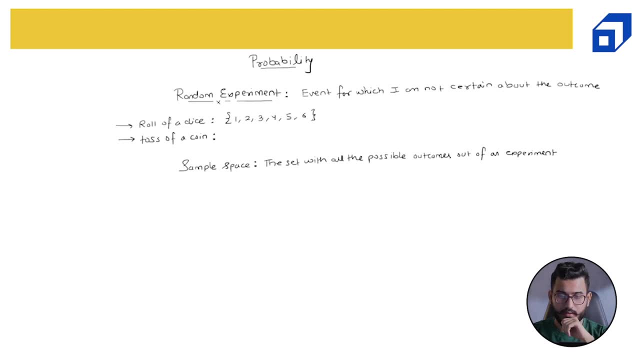 So if I take the example of roll of a die, I may get 1,, 2,, 3,, 4,, 5,, 6, you can get anything. So this is my sample: space for rolling a tie, for toss of a coin. 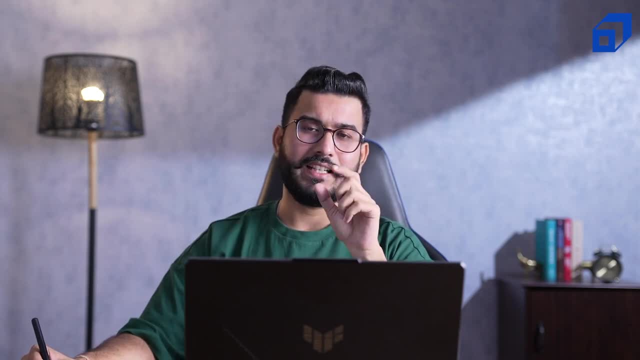 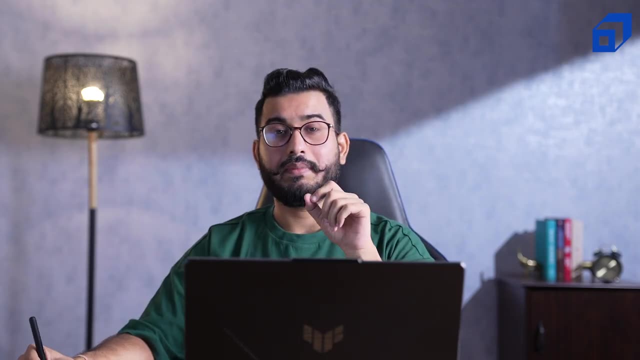 Now, if the coin is a fair coin, which basically means one side will be head and one side will be tail, So I may get either a head or a tail. Now, this is basically my sample space for the random experiment Toss of a Coin. 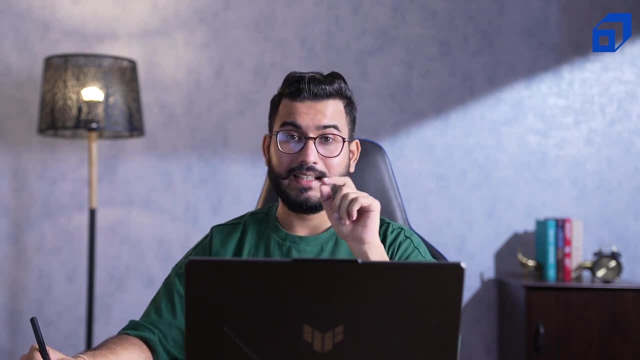 If I talk about my birth date, in that case all years maybe. let me not. let me just limit the sample space to 1996. so if you know that the birth year is 1996, then in that case the sample space will be all the. 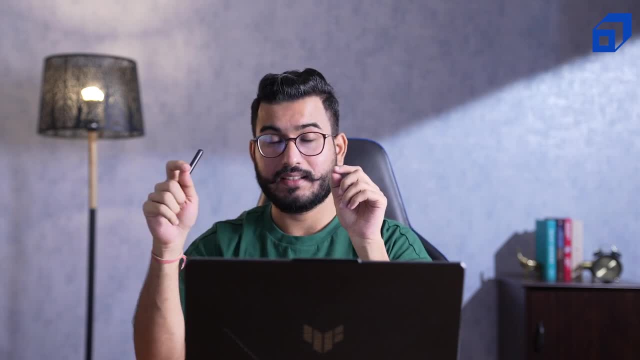 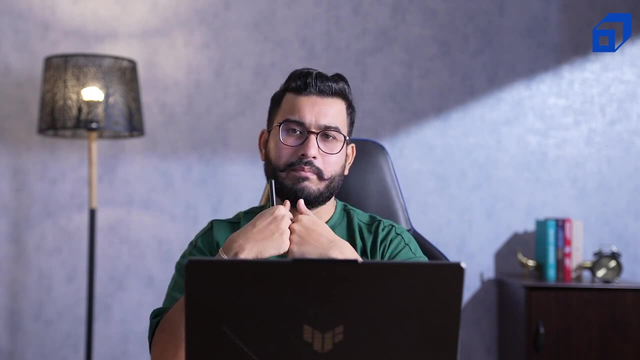 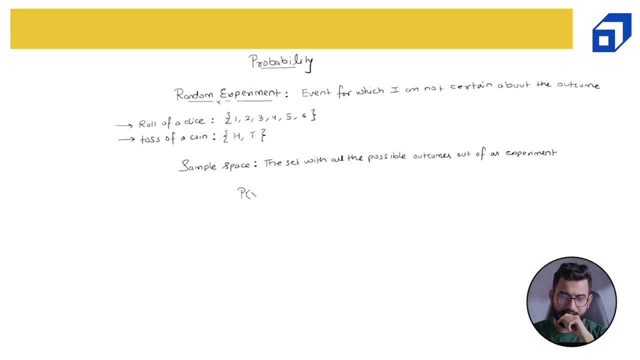 months, and within each month all the dates or all the days. so your sample space will have quite a good number of outcomes, right? so this is what my sample space is now. What is probability? so probability of a particular even X is basically how many times that event has occurred in your sample space. so number 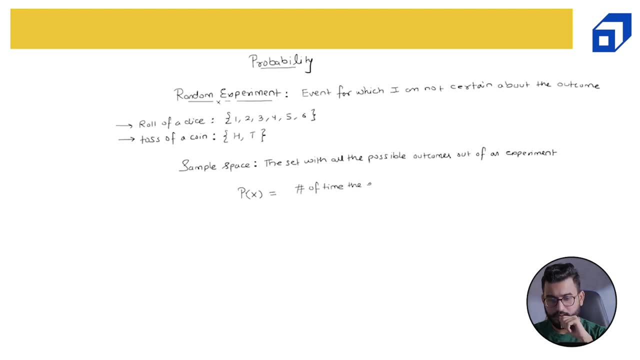 of times the event occurred in the sample space and we divide the time spent in creating the sample, then our number of times has occurred. this by the total size of the sample space. total number of outcomes. so total number of outcomes in my sample space. now please remember one thing: if I go with the definition, this 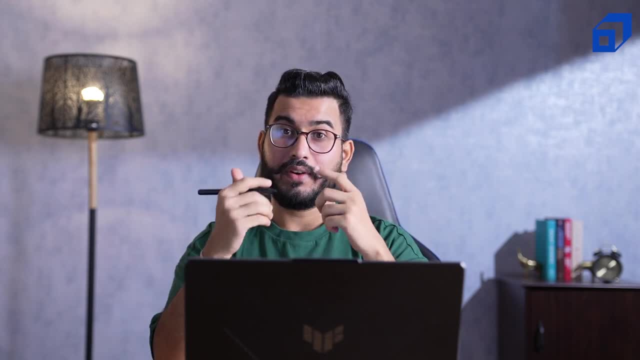 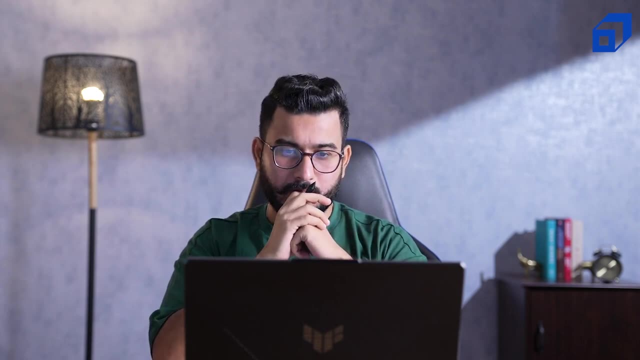 is the very accurate definition that the number of times a particular event has occurred divided by the total number of, or total size of the sample space. but there might or there may be various ways of writing a sample space. let's try to quickly understand the difference, because this: 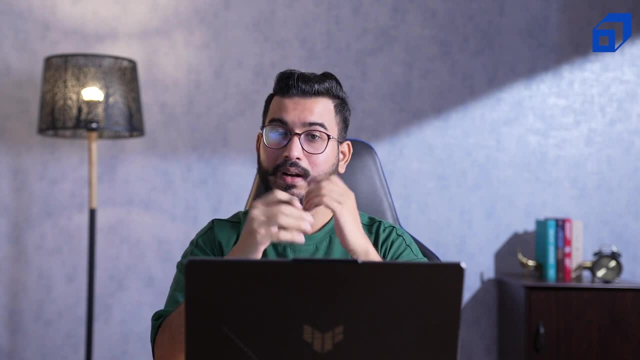 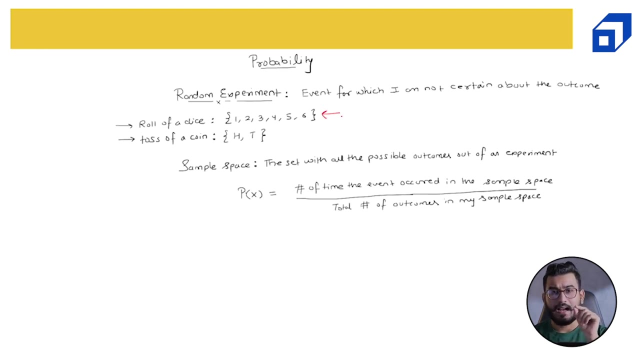 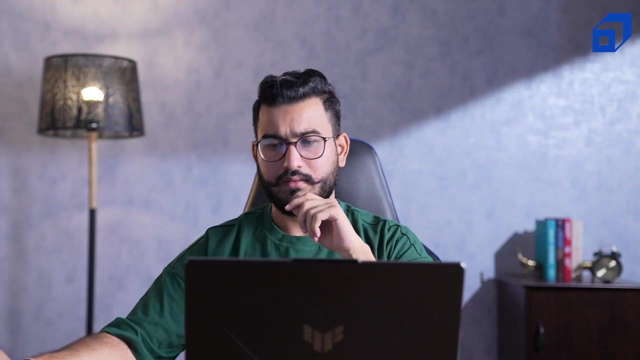 is the major mistake most of the students commit while calculating probability. so this particular sample space is having all the outcomes which are equally likely. so all the outcomes, all the outcomes in this sample space are equally likely. what is the meaning of equally likely? so if you already know about it, you can just pause the video. 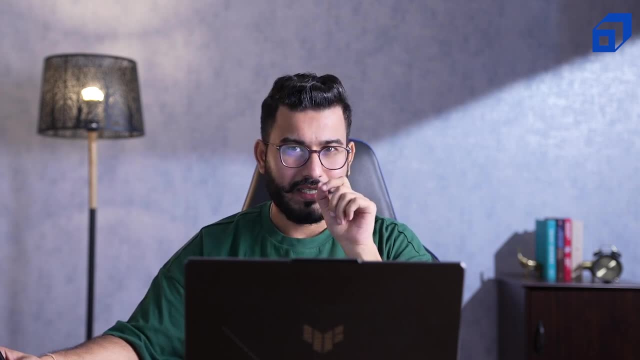 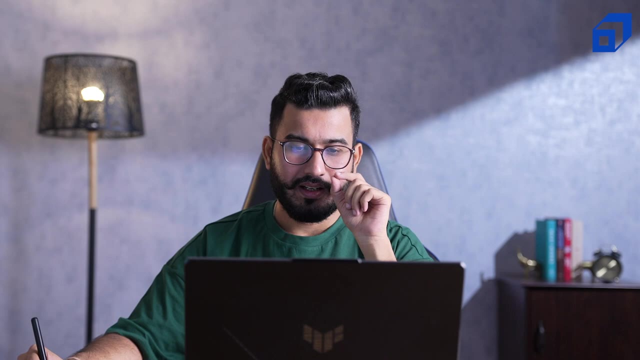 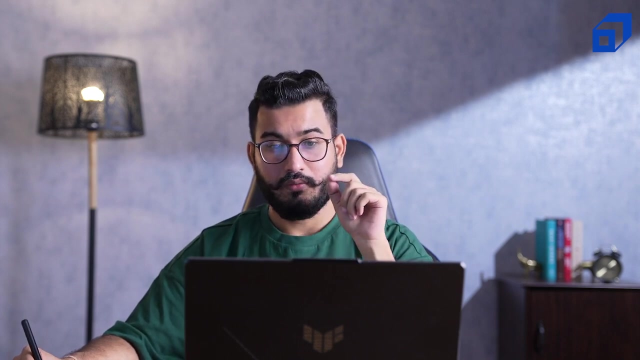 and comment on this particular video, but equally likely basically mean that if I choose any of the event, it will have the equal chance of occurrence. for example, what is the probability that I will get the number one if I roll a die? it is simply 1 divided by 6. what is the probability that I'll get 2 again 1. 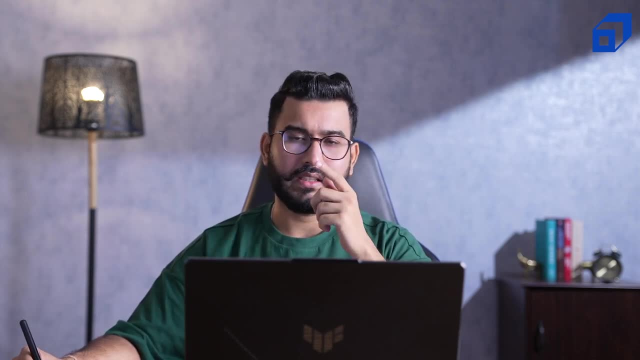 divided by 6: 3 1 divided by 6: 4 1 divided by 6: 5 1 divided by 6: 6 1 divided by 6, so all the events in this particular sample space are equally likely because each of them are having the probability equal to. 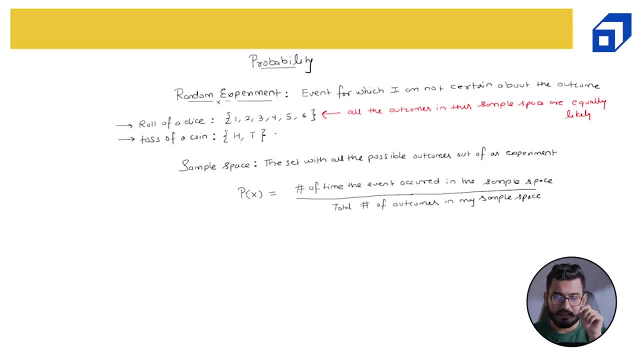 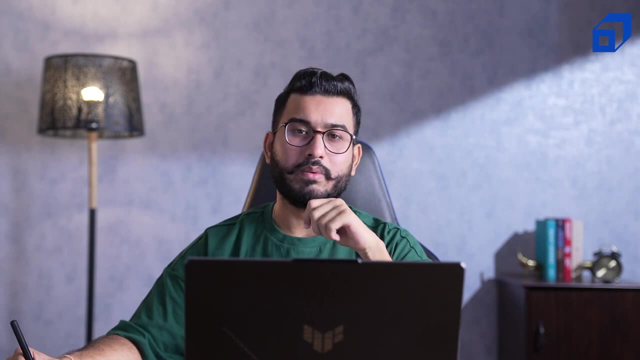 1 by 6. similarly, if I take this sample space- the sample is space- is also equally likely. so what is the probability of getting head 1 by 2? what is the probability of getting tail? again 1 by 2? so the probability of getting head and. 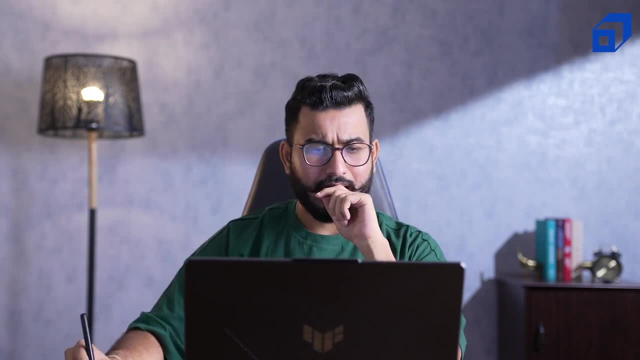 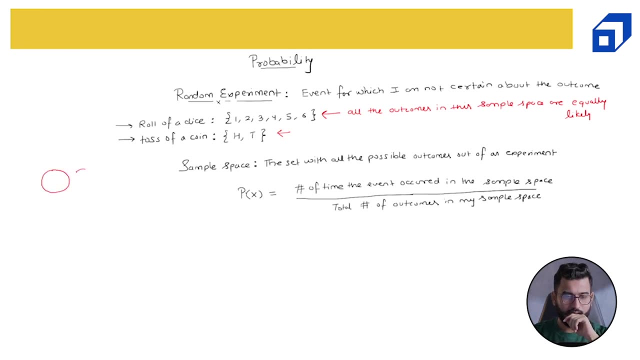 tail are equally likely. but now let's take example where I am tossing two coins. so I am having two coins. my drawing is really good, so I'll use my skill over here. so let's say: these are my two coins. now what are the possible outcomes? I might get a head. 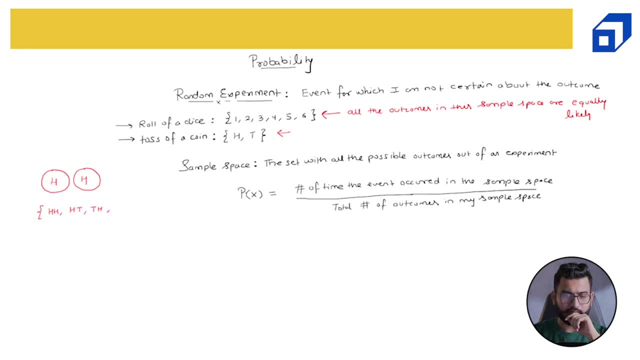 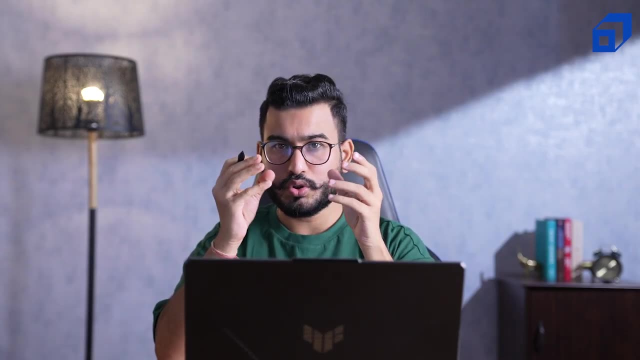 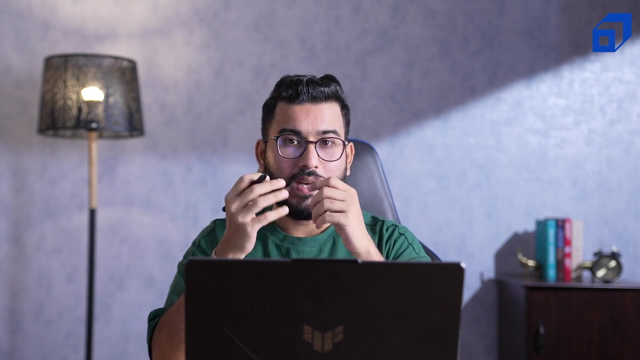 head, a head tail, a tail head or a tail tail. right now, what is the probability that I'll get a head and a head, like both coins land in two, both coins land with the face, head and head. this is one divided by 4, because here I'm having total four outcomes and the probability. 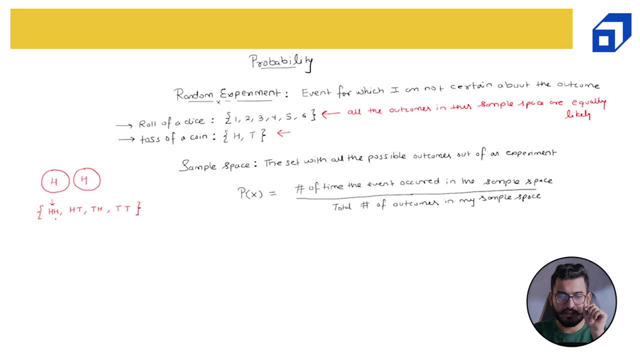 of getting headed is. only one event is there, so the probability of getting headed is 1 by 4. this is 1 x 4. this is 1 by 4. this is 1 by 4, so this sample space is also equally likely. can I write the sample space in another way? yes, we can. 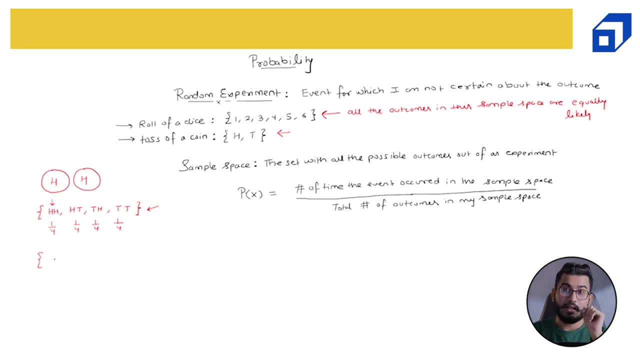 So let's say now, my sample spaces are the number of heads, so I can have zero heads, one head or two head. This is also a sample space, but there is a difference. this sample space is not equally likely. This Sample space is Not Equally likely. 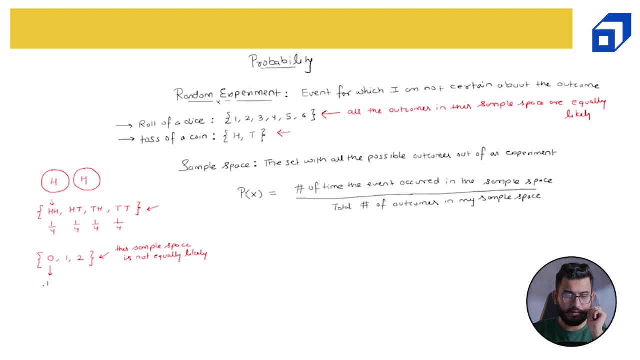 so the probability of getting zero head is 1 by 4 and please remember, here each number represents the number of Heads. so the probability of getting zero head is 1 by 4. probability of getting one head is This plus this, So it can be either head, tail or tail head. So 1 by 4 plus 1 by 4, it is 1 by 2 and 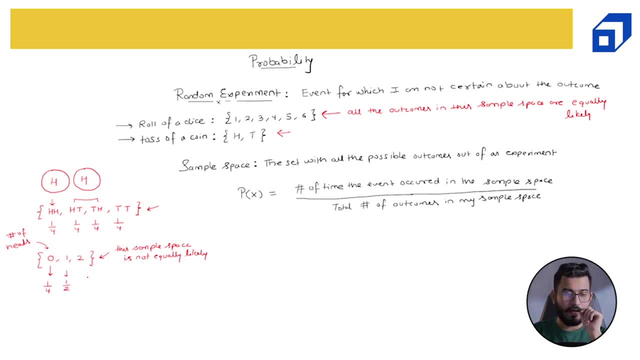 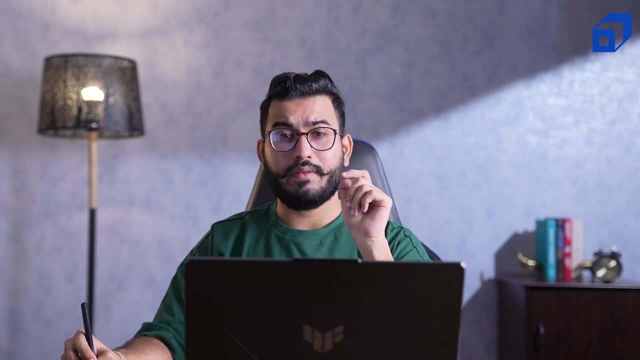 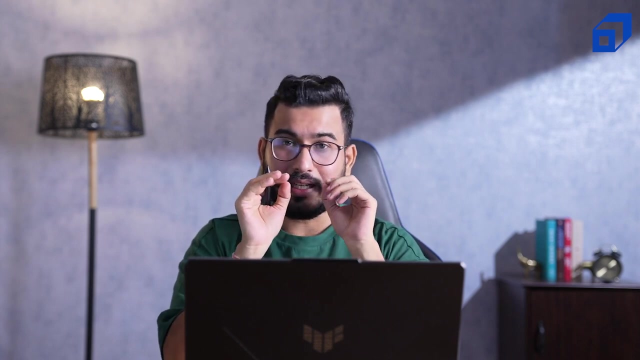 probability of getting two head is again 1 by 4. So here you can see that The probability of each event is not equally likely. So whenever you are calculating probability you have to make sure that your sample is sorry. your sample space Should be equally likely. if it is not, then you have to carefully. 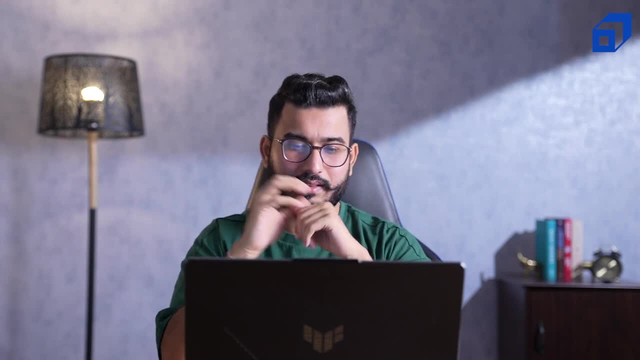 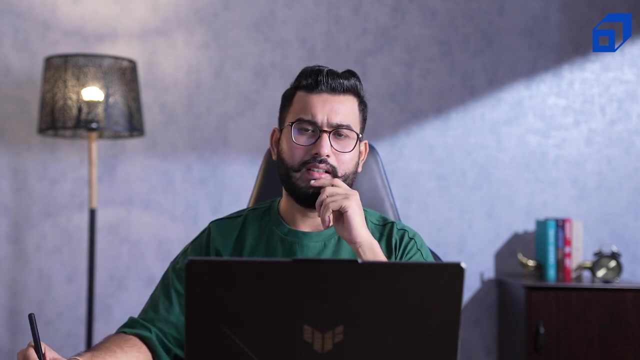 calculate your probability. I I hope this is making sense. So now let's talk about some of the rules of probability. So I hope every one of you are clear with the idea of random experiment and the sample space. There is one particular term which is known as. 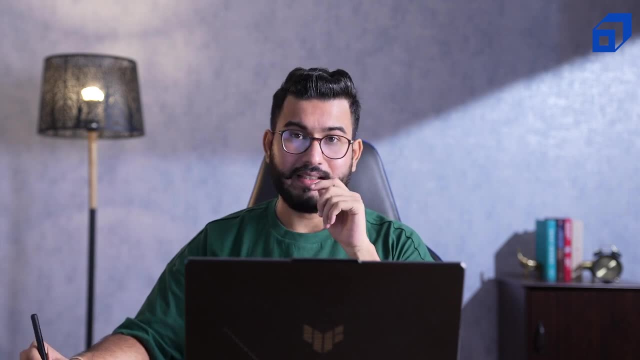 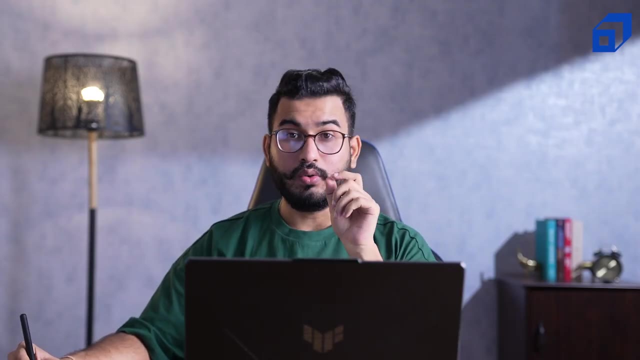 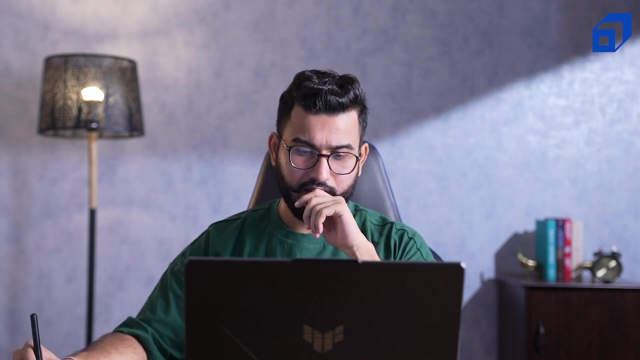 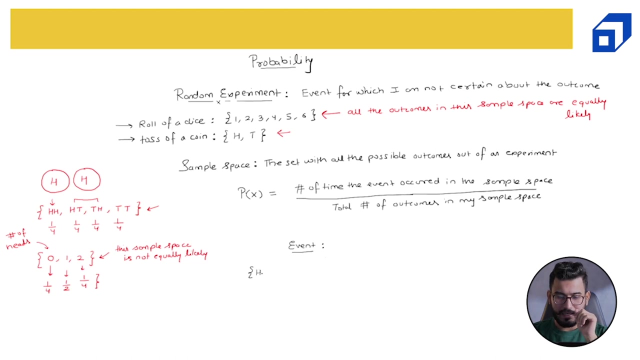 event. Now, what is an event? Any possible outcome or group of outcome out of a random experiment or out of a sample space is known as an event. For example, if my experiment is toss of a coin, then I may get a head or a tail. So out of this experiment, getting a head is. 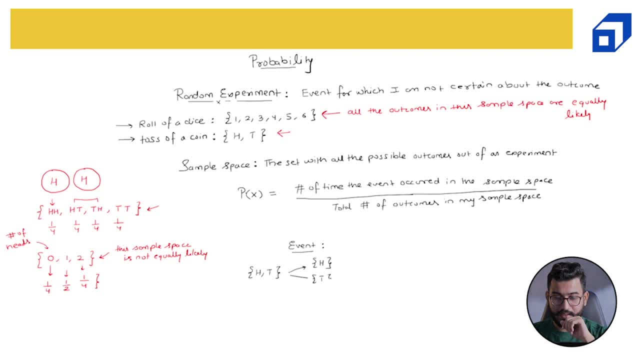 an event. getting a tail is an event. Similarly, if I'm tossing two coins, I may get head, head, head, tail, tail, head and tail tail. In this case, getting two heads is an event. getting one head is an event. 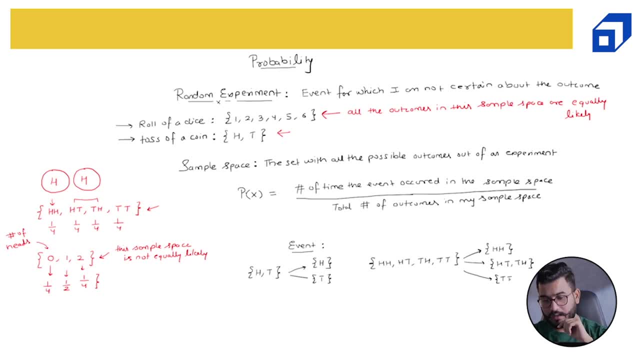 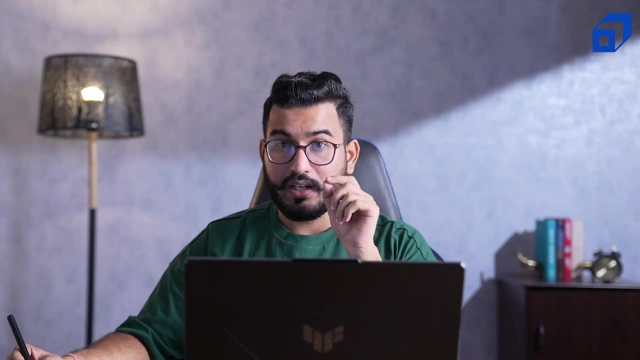 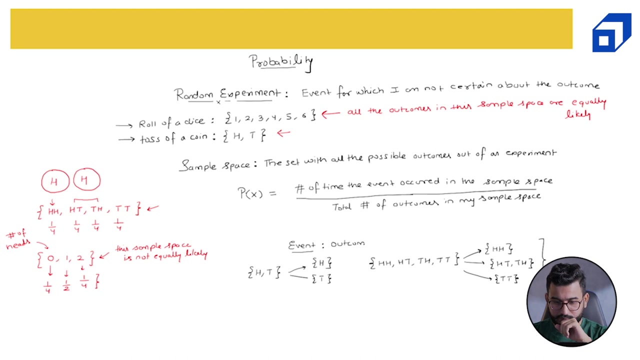 getting no head is an event. So all of these are my events. So event is nothing but a particular outcome or group of outcome out of a random experiment or a group of outcomes out of a sample space. so outcome or group of outcomes out of a 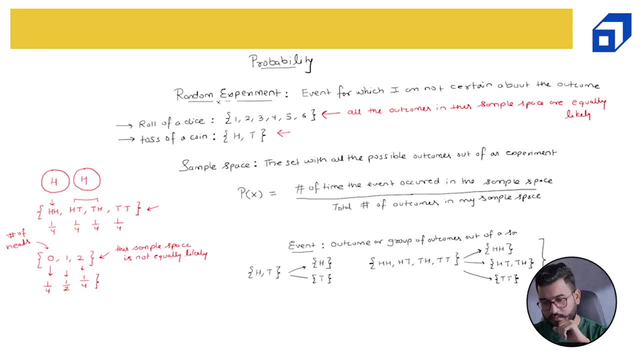 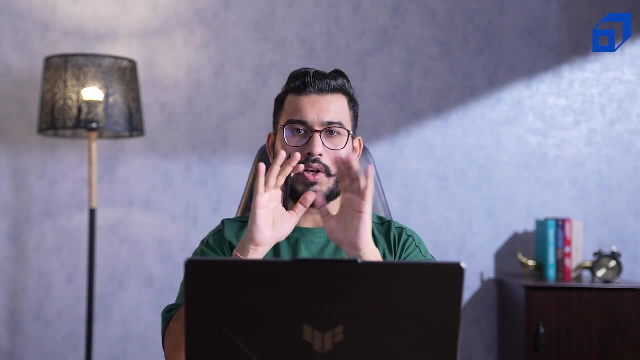 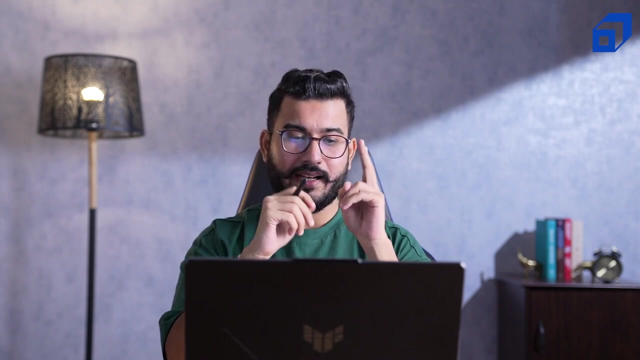 sample space. So this is the given event. So what all we have talked about? Number one, random experience. number two is sample space, and then we have collected different random experiments. Now, in order to the two ways in which we can write the sample space, one is equally likely. 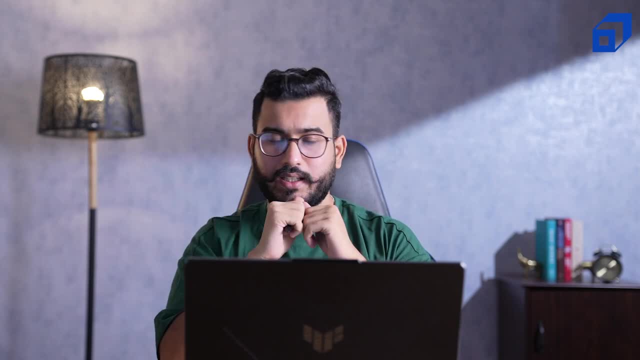 sample space, other one is not equally likely. the third topic which we talked about was event. now let's talk about the rules of probability. so when you are using probability as a measure or as a tool to basically calculate the possibility of probability of a particular event, there are some rules. 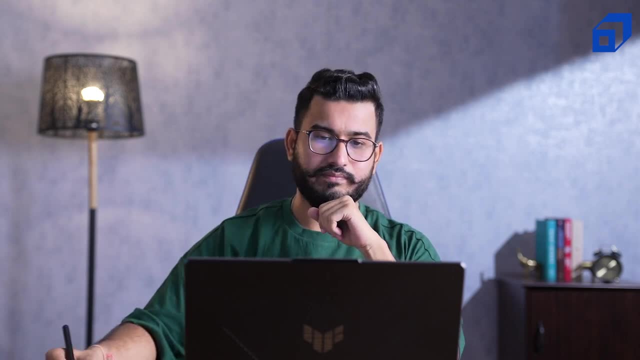 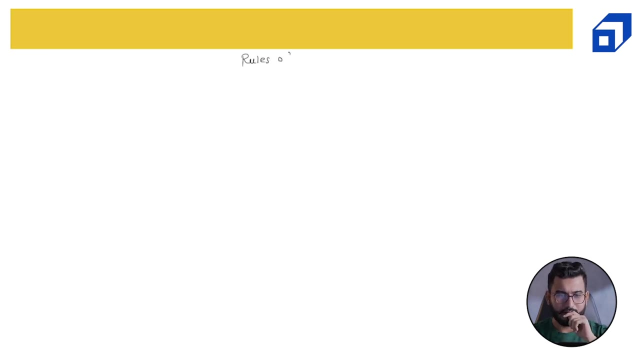 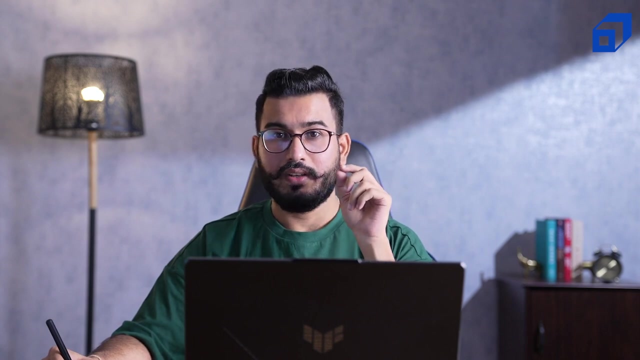 which we have to keep in mind. so let's talk about them. they are also known as the exams of probability. I'll just simply write it as rules of probability. so rules of probability. okay. the very first rule is: given a sample space, the probability of each outcome will always result to one. the total probability is: 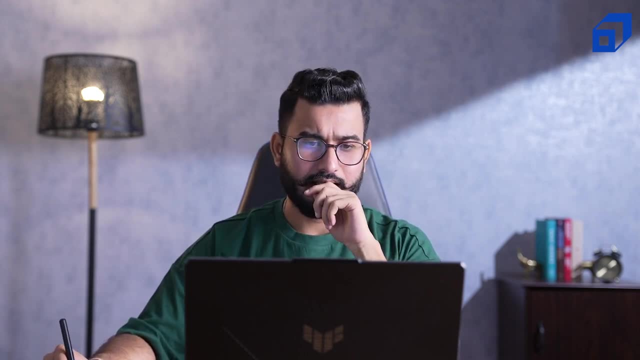 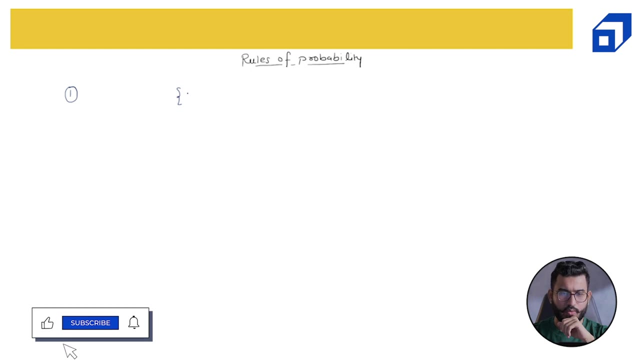 always one is equal to one. let's try to understand it. let's say I'm given with a sample, a sample space of rule of a dice, so when I roll our dice I may get one, two, three, four, five or six. we know that the probable probability of one is one by six. 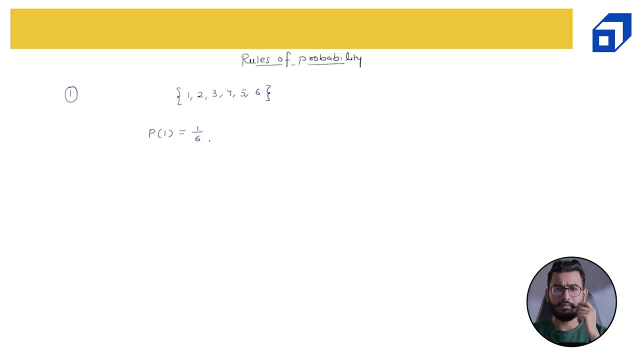 so what is the probability of getting one in the dice is one by six. what is the probability of getting two? it's again one by six, probably probability of three, again one by six, and this is equal to probability of four, probability of five and probability of six. all is one by six. now, if I take the 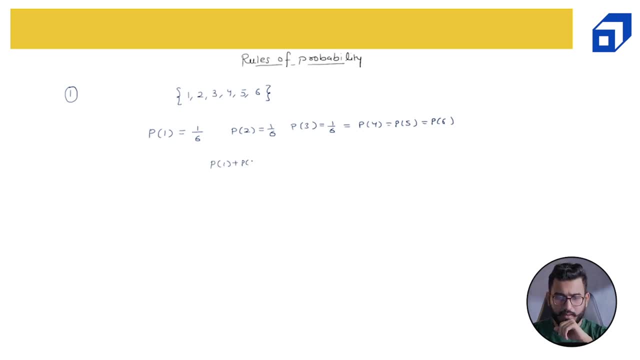 sum probability of 1 plus 2 plus 3 plus 4 plus 5 plus 6. if you do the quick math you will find out that it is equal to 1. that is my first, also summation of PI where I is running from 1 to n, or I is: 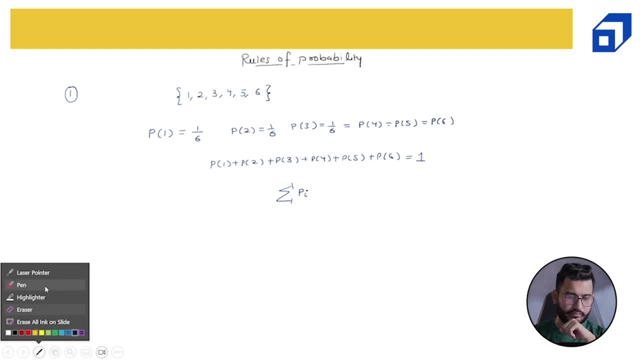 over my sample space. well, I'll just simply write where I belongs to my sample space. the sum of all the probability is always equal to one. this is my first rule let's talk about, so let me just formally write it down so that you guys are having all these notes and whenever you prepare for your interview, if you 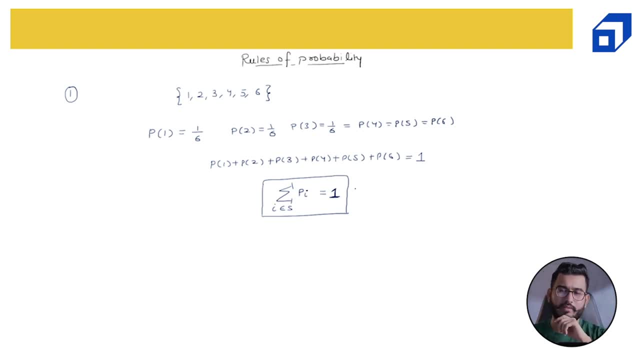 just read all the note, it will be very easy for you to pass your statistics around. So the sum of all probability over the sample space, or the sample space, is always equals to 1.. This is my first rule. Now let's understand the second rule, which is known as the rule of sum or addition probability. It 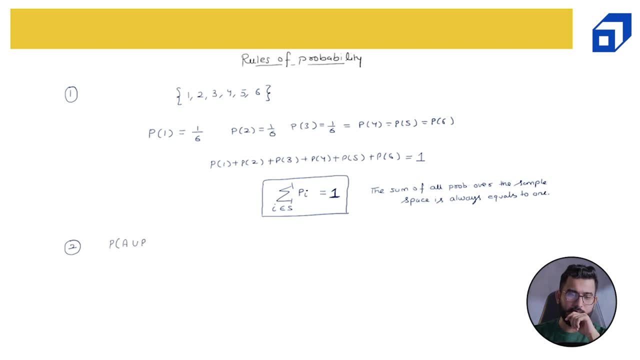 says that the probability of A union B is equal to probability of A plus probability of B If A and B are disjoned event. So there's are condition if A and B are disjoint. now, don't need to worry, I am not talking anything in German. this is very simple. 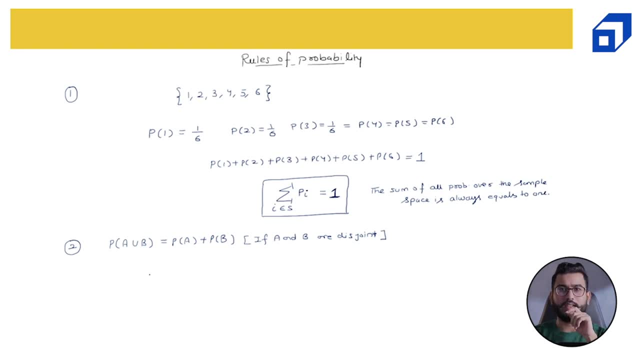 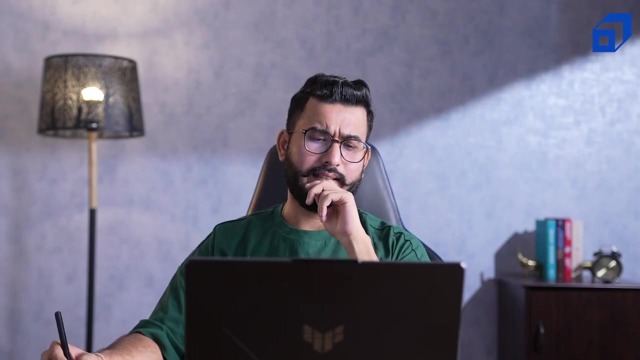 to understand. let's take one simple example. let's say I am tossing two points, so when you toss to points you might get two heads, two tails, one head, one tail and one tail, one head. Now, if I ask you what is the event of getting two head or so, let's take what is a. what is the event of getting two different? 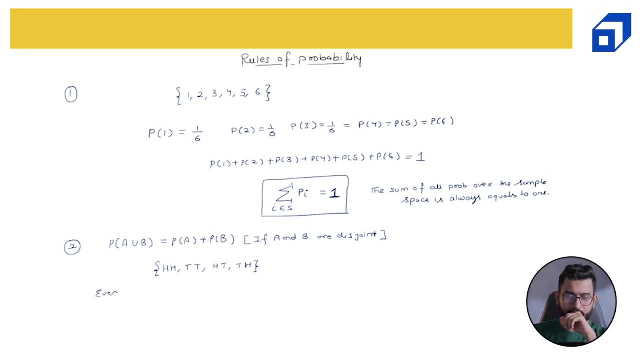 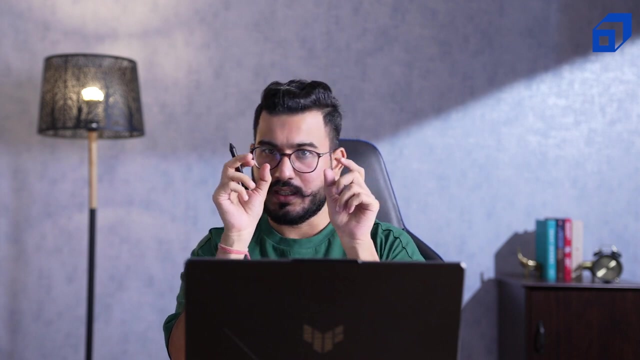 outcomes. let me write it down. what is the event of getting both coins with different outcome, which basically mean both coins land into a different outcome, so one is hit, so another one will be tail. if one is tail, another one will be head. and we already know that there are only two possibilities. 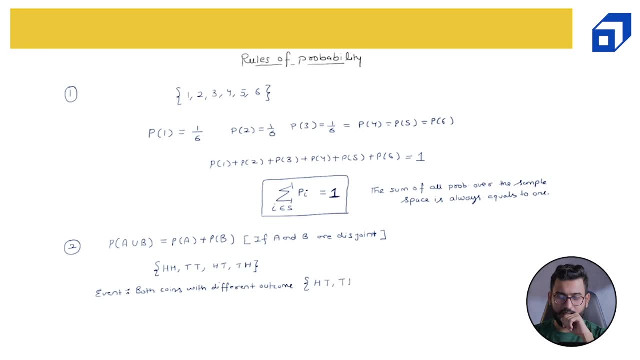 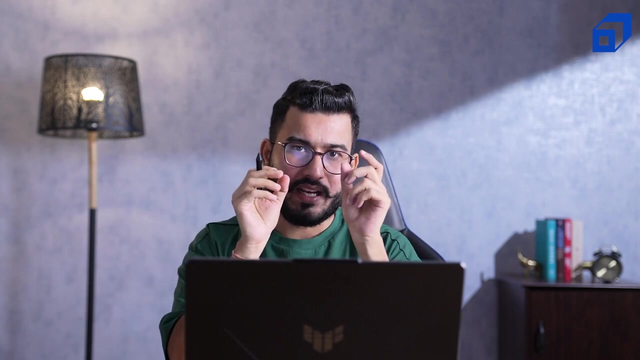 so my event would be head, tail or tail head. right, let's call this. I let's call this event as event a. now if we have another event where both coins lands into same outcome, which basically means it: if coin one is head, coin two is also head, If coin one is tail, coin two is also tail. So this is: 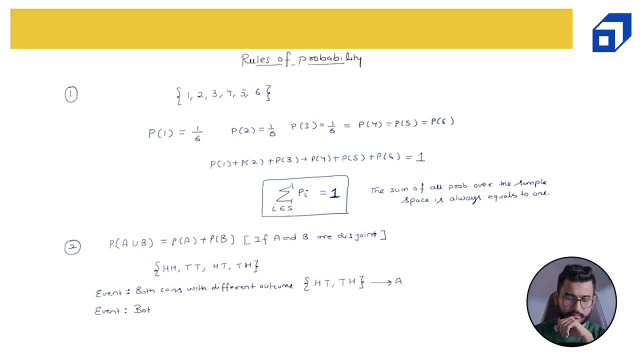 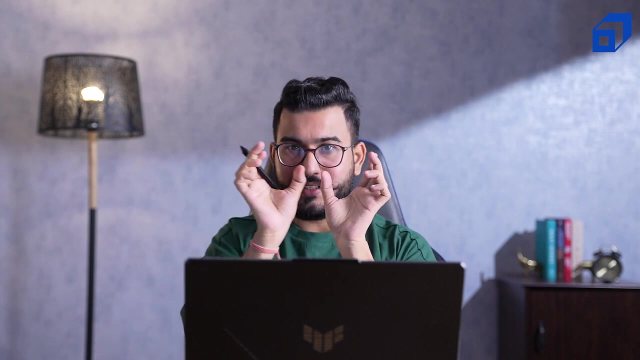 same outcome. So both coins, both coins with same outcome, and that would be head, head, tail, tail. and this is my event B. Now, if I take the union, union means addition. If I take the addition of these two set, then according to the rule, 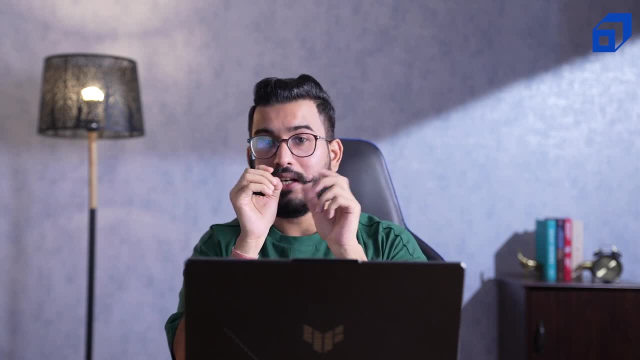 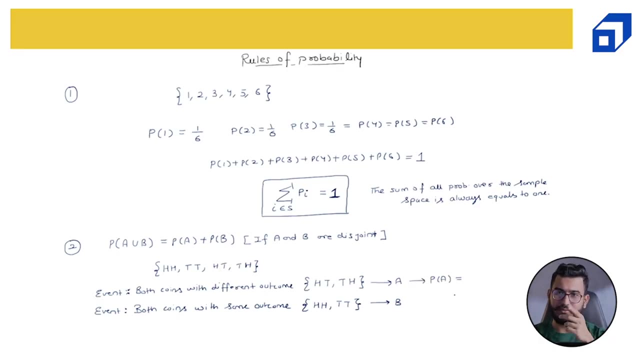 it is the sum of individual probability of the event. So what is the probability of event A? If you guys have understood, you can simply answer this and you can add your answers in the comment section. So the probability of A is there are two outcomes with which matches my condition. So head tail and tail head. 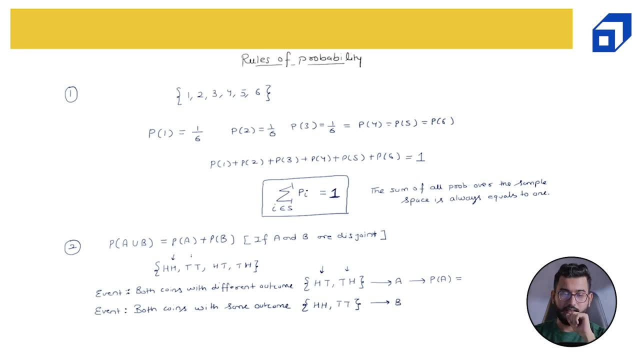 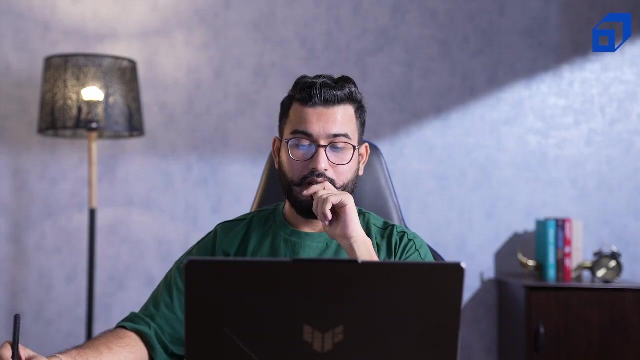 there are total of four outcomes in my sample space. So the probability is 2 divided by 4,, which is simply 1 divided by 2.. Similarly, probability of B is also 2 divided by 4,, which is 1 divided by 2.. Now, if I take the sum or if I take the union of these two events, 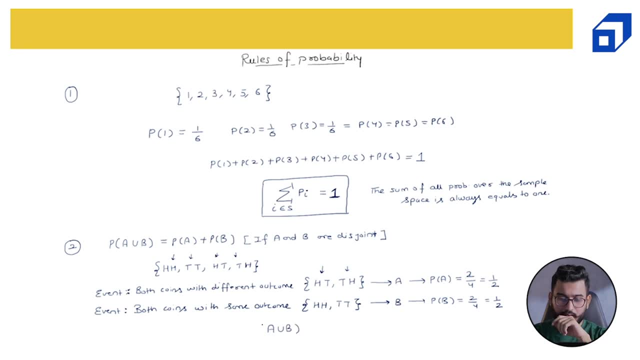 so what is the union of A union B? A union B means I will combine all the events in my sample space. Now, since we do not have any common element, my union would simply be head-tail, tail-head, head-head and tail-tail. And if I ask you, what is the probability of A union B? 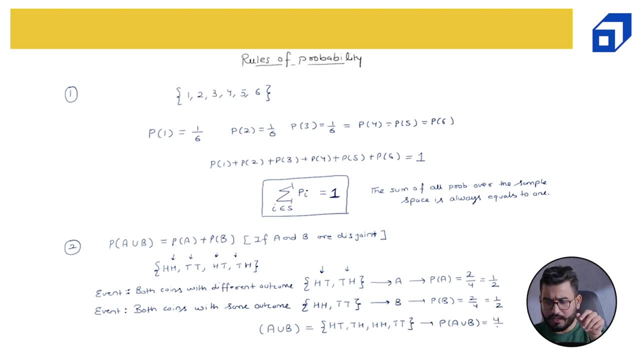 you will just simply say it is 4 divided by 4, which is 1.. Now, if I add up all the events in my sample space, I will get 4 divided by 4, which is 1.. Add these two probability: probability of A plus probability of B. you can simply add 1 by 2 plus. 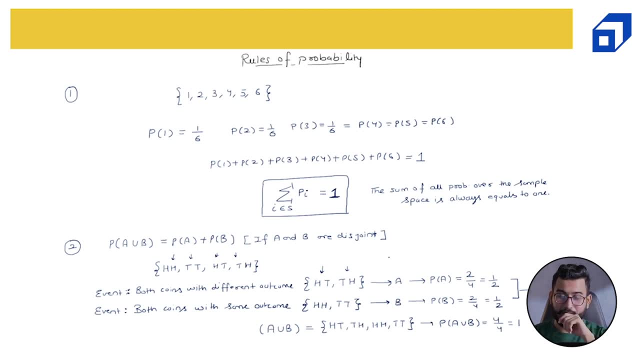 1 by 2.. This is also 1, right. So that basically means if two events are disjoint. so here you can see, event A and event B are disjoint. Why I am calling them as disjoint? Because they do not have any common event. You can see that in event A I am having head-tail, In event B I am having 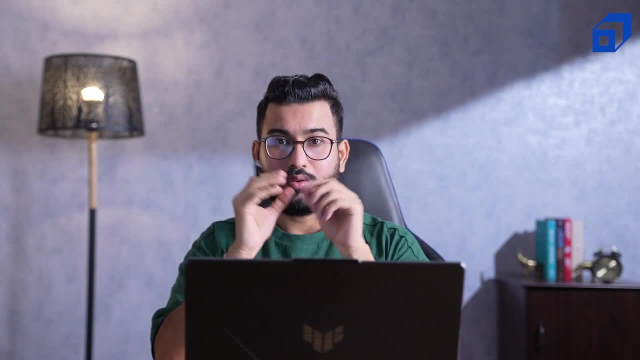 head-head-tail. In event C: I am having head-head-tail. In event D: I am having head-head-tail. There is no common event. So when two events- A and B- are disjoint, they do not have any common. 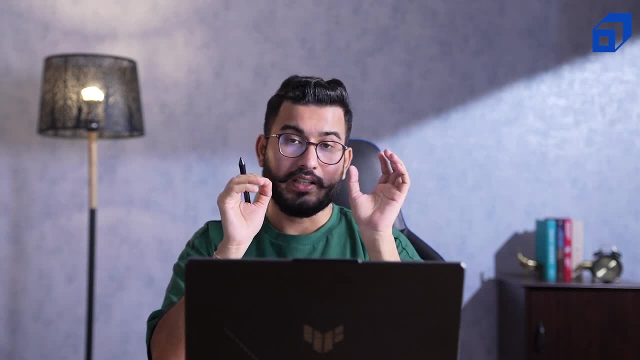 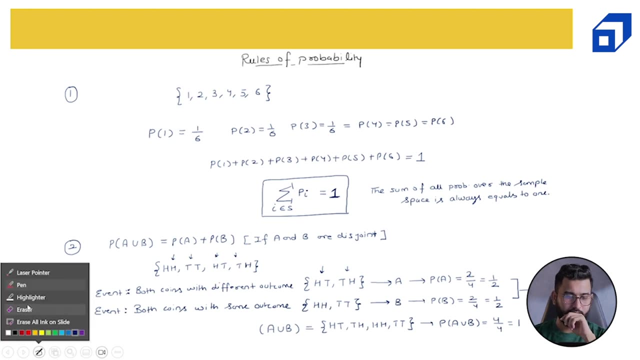 event, then the probability of the union is always equal to the individual sum of probability, And this is what we were trying to prove. So let me just quickly highlight this, And this is my second rule of probability. This was my first rule, This is my second rule, And 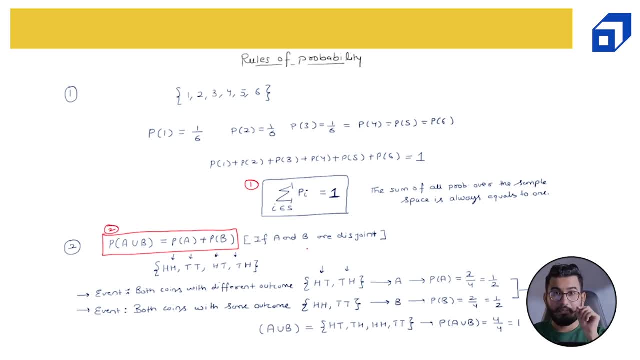 this rule is only applicable when your two events are disjoint. Where we have taken this example, A and B are disjoint because it does not have any common event among them. Right, Simple. Now let's understand the third rule, And third rule is also very much. 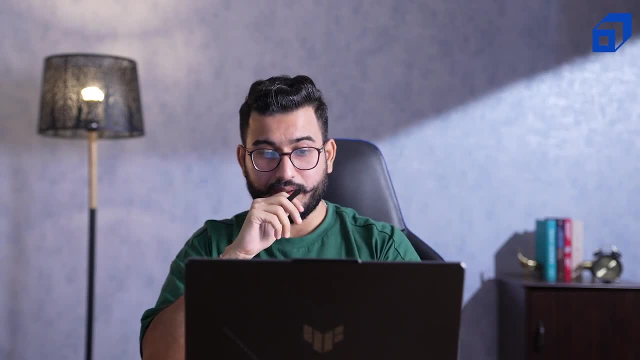 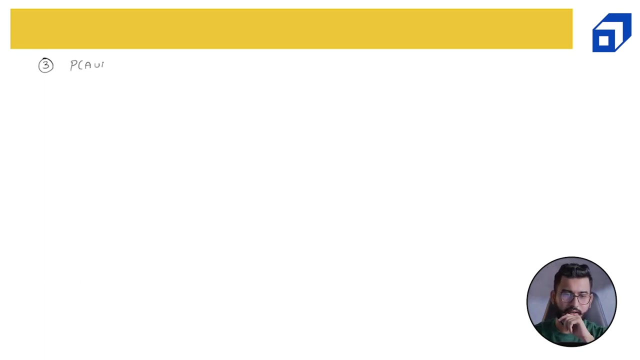 closely associated with the second rule, where we proved that probability of A union B is always equal to the probability of A plus probability of B, if A and B are disjoint. right Now there is one more rule: If they are not disjoint, then probability of A union B is probability of A. 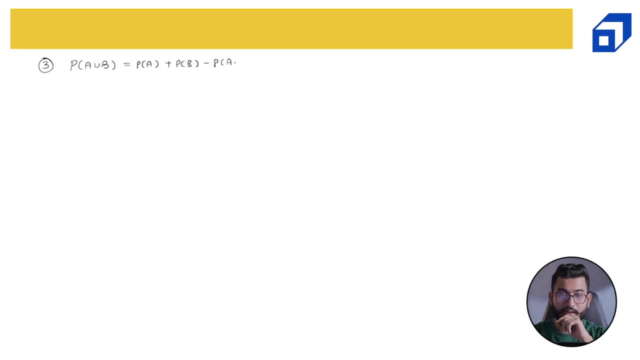 plus probability of B, Minus probability of A, intersection B. Again, you guys would be thinking that it is something German, but not. Let's try to understand it. In order to understand it in a better way, we will take the example of playing cards. Playing cards. 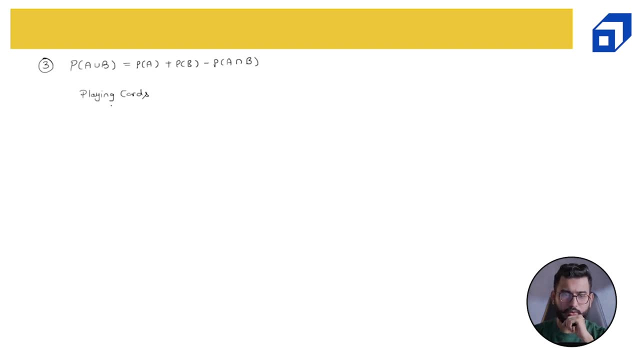 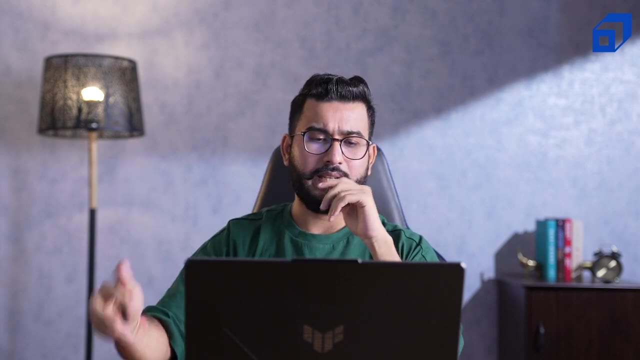 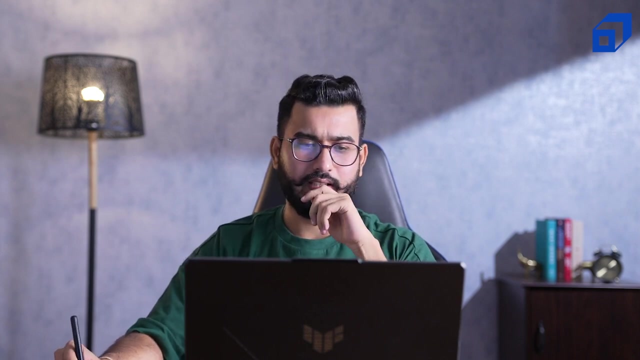 And I hope most of you would be aware about the playing cards, But if you are not, don't need to worry. Let's try to write down the complete details about how many playing cards we have, what are the various suits and everything. 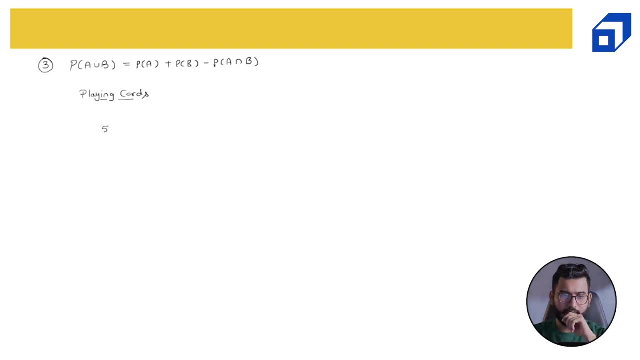 So in total a playing card or a deck of playing cards comes with 52 cards with four suits. So we have club spade, heart and diamond. Now, if you guys are aware about it, then you can easily point it out that. 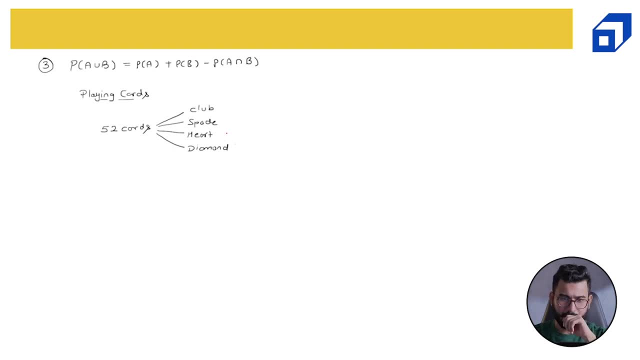 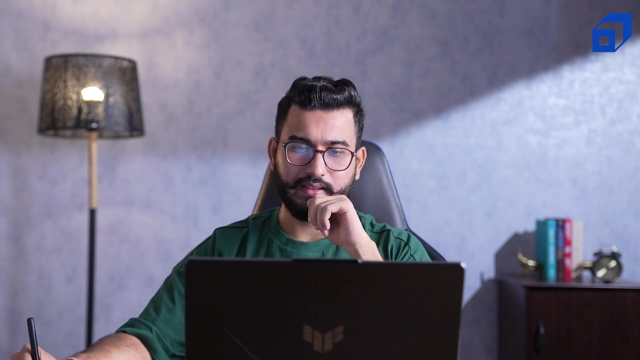 club and spade. These are two black cards, while heart and diamond these are my red cards. so club and spade are my black cards. Now club is having 13 cards, spade is having 13,, heart 13 and diamond 13.. So each of them, 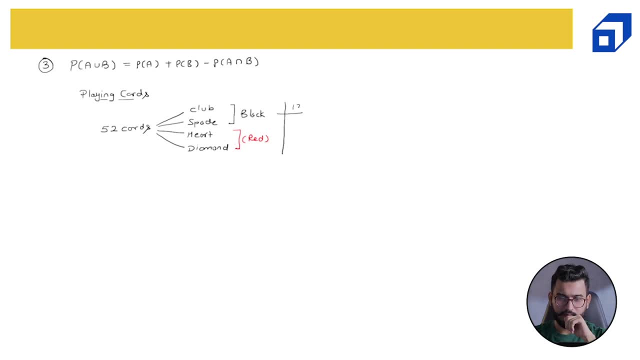 is having 13,, 13 cards Now. which all 13?? So let's write down the complete structure. So each suit comes with total of 13 card which starts with ace- a card of ace, then two, three, four. 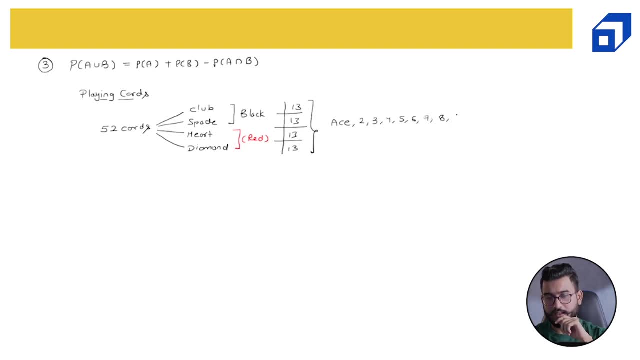 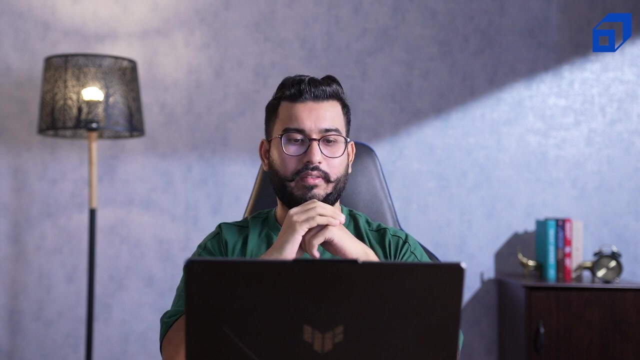 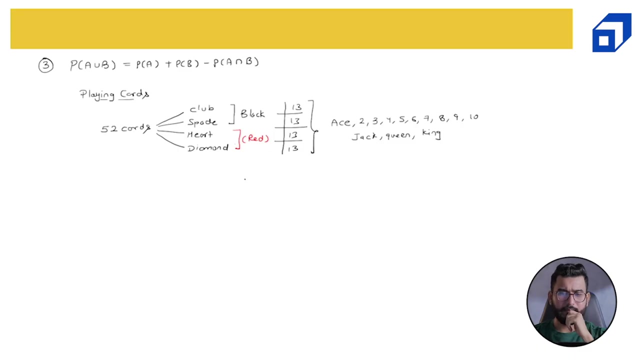 five, six, seven, eight, nine, ten and then three cards which are known as the jack, queen and king. Now this is the complete portfolio of your playing cards, or the deck of playing cards. Now let's try to calculate some probability of some events. So what is the probability of getting a jack? 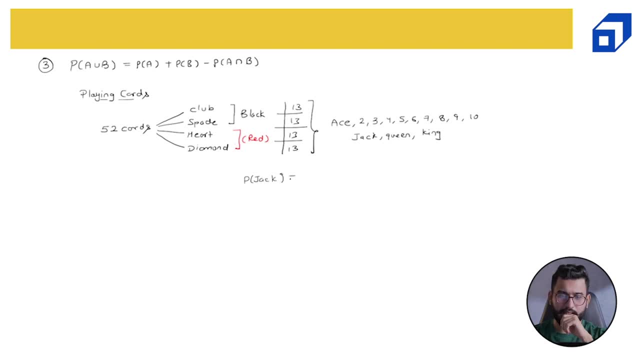 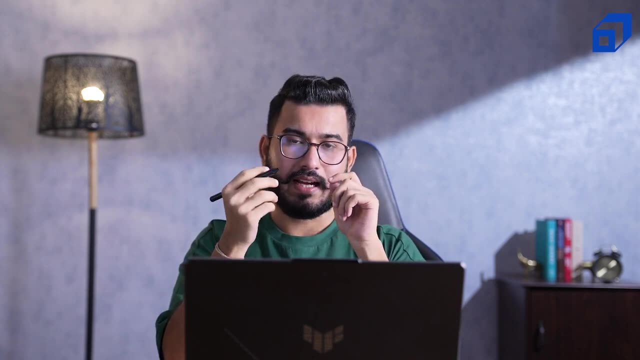 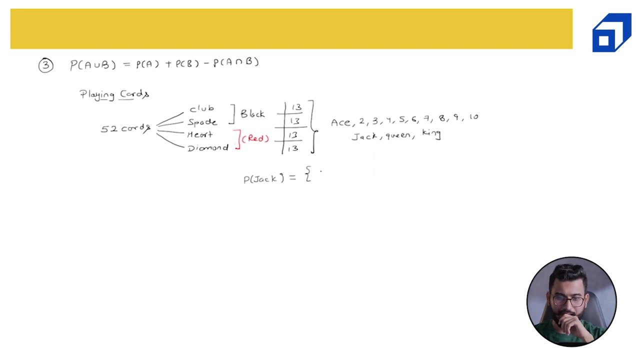 What is the probability of getting a card which is a jack card? Now we already know that a jack, a card of a jack, can come from any of the suit. So I may have a jack from club. So I write CJ, club of jack or jack of club. you can say anything. 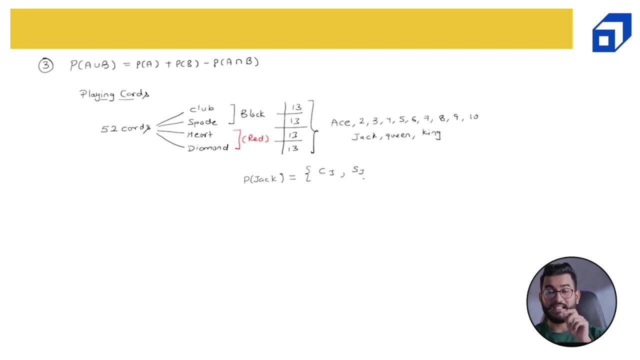 Jack of club, Jack of club. you can say anything, Jack of club, Jack of club. Then we have a spade. I can get a jack from a spade, I can get a jack from heart, I can get a jack from diamond. right, These are the total four outcomes, or total four favorable outcomes. 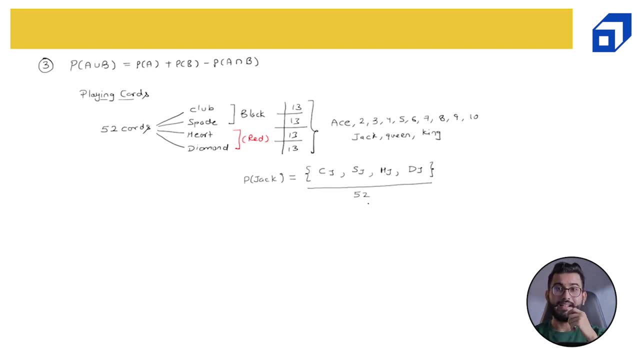 While the total number of outcomes, or total number of events in my sample space is 52, because each card is an outcome, right? So the probability of getting a jack is 4 divided by 52, right? What is the probability of getting a black card? Now we already know that club and spade, or let's 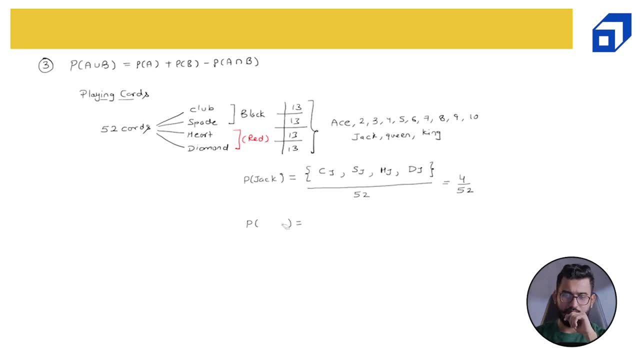 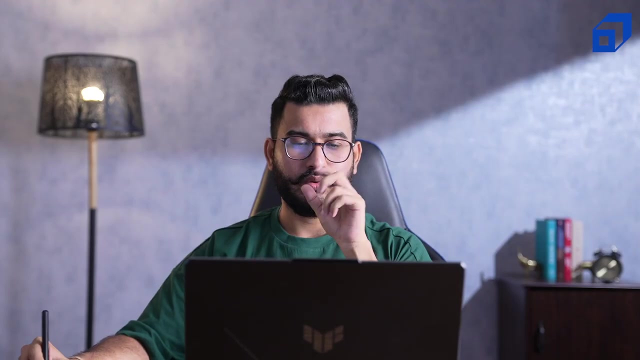 simplify the question so that I can demonstrate you the rule that we were trying to prove. So what is the probability of getting a heart? Now we know that there are total of 13 hearts, because heart itself is a suit, So we have 13. 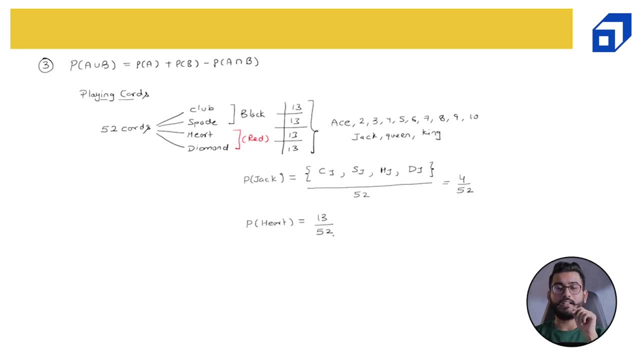 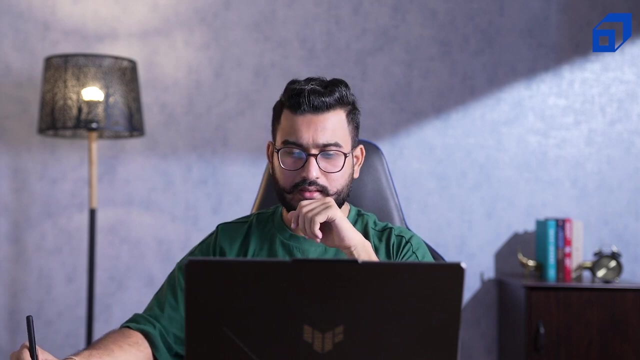 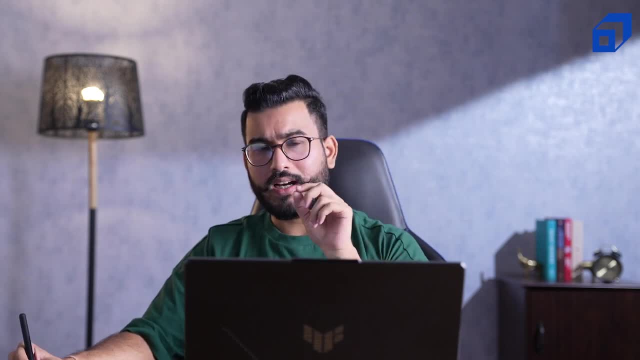 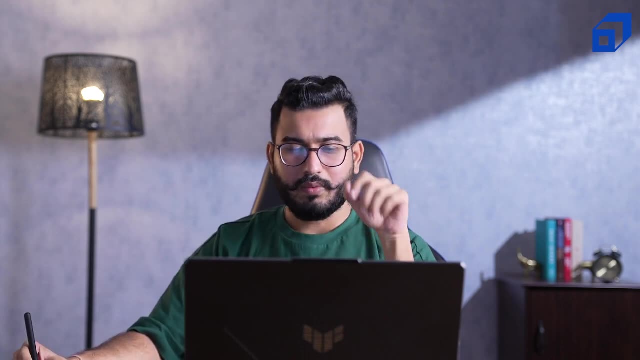 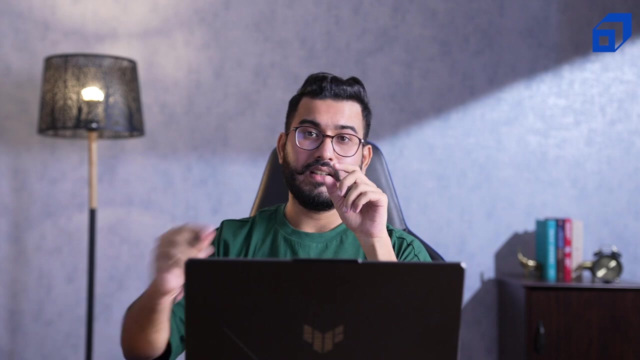 see. So let's see. So, let's see. We already calculated the answers. Let's try to note down all the outcomes. which matches this condition, and then it will be easy for us to understand if we are going in the right direction or not. Jack and heart, which basically means the card. 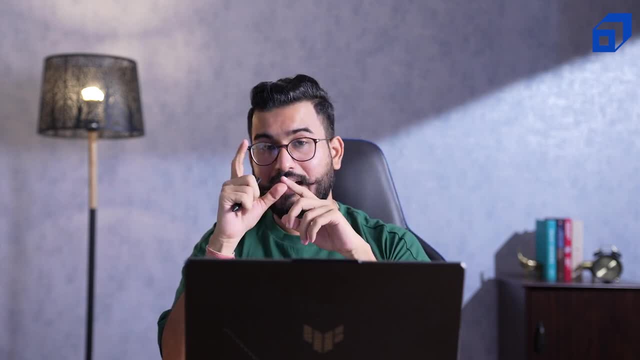 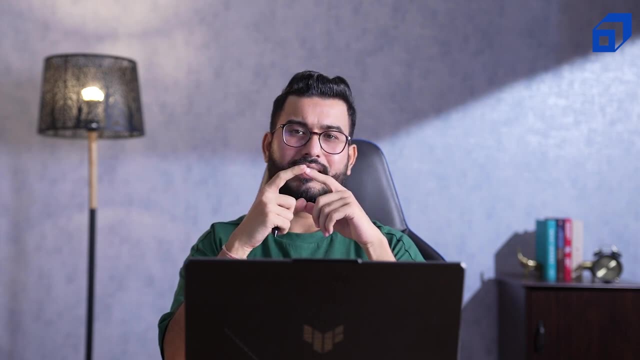 need to be a jack card and the card should be a heart. Now, if you closely try to understand this, you will find out that it is only one card that can satisfy these two conditions: A card which is jack plus it also belongs to a heart. 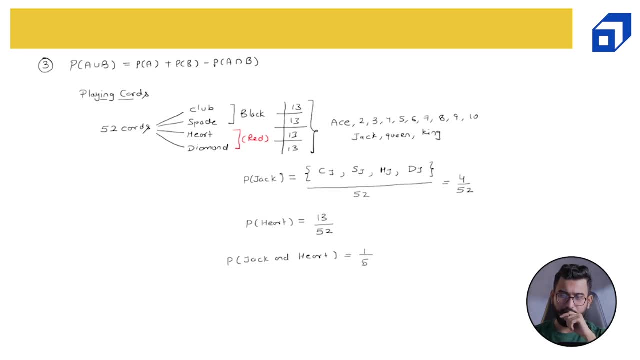 So the probability is 1 divided by 52, because I will have only one card, which is heart of jack or jack of heart. Now, what is the probability of jack or heart? Now, all means nothing but the addition. Before we calculate this probability, let's write down all the outcomes, or all the events. 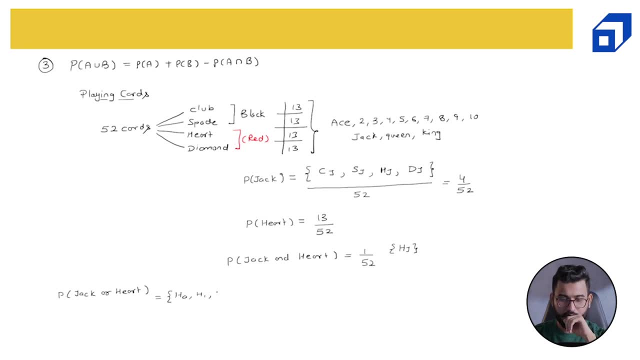 So it will be heart of ace, heart of 1,, heart of 2,, heart of 3,, 4,, 5,, 6,, 7,, 8.. 9,, 10,, then heart of jack, heart of queen and heart of king. 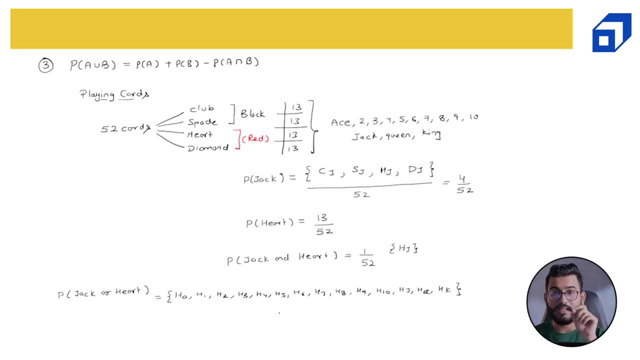 These are all the cards that belong to the suit heart. Now let's write down all the jack cards. So I can have a jack from heart. so hj, I can have a jack from club. so, cj, I can have a jack from club. 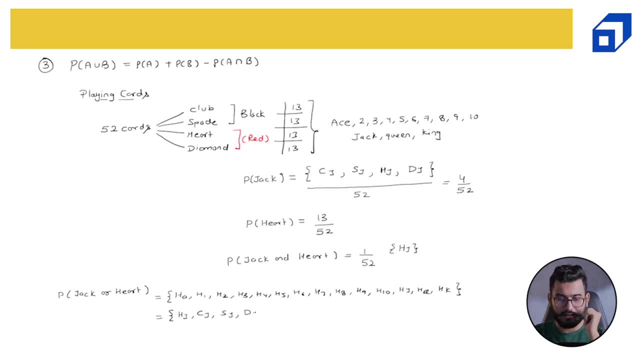 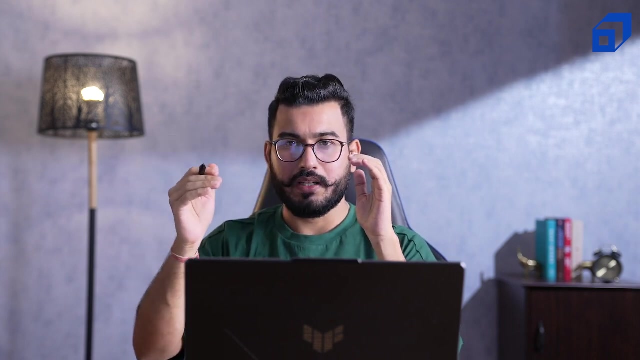 I can have a jack from spade, so sj and then dj. Now if I combine them, if I take the union of them, so let's call this as event B, this as event A. If I take A union B, A union B means I have to create a set which is having all the events from A and all the events from B. 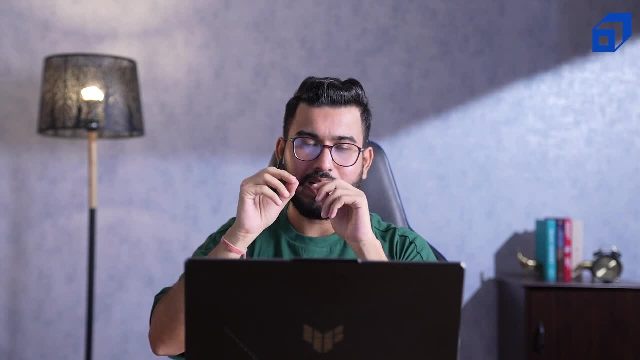 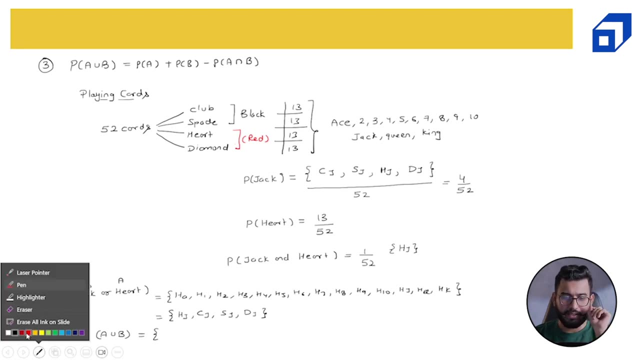 But if there is an event which is replicating for two times, I have to only pick one of them. So if I combine them, you will find out that there is one event which is common in these two sets, and this is this card. 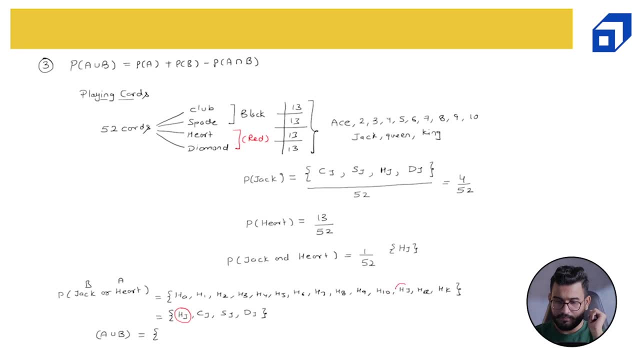 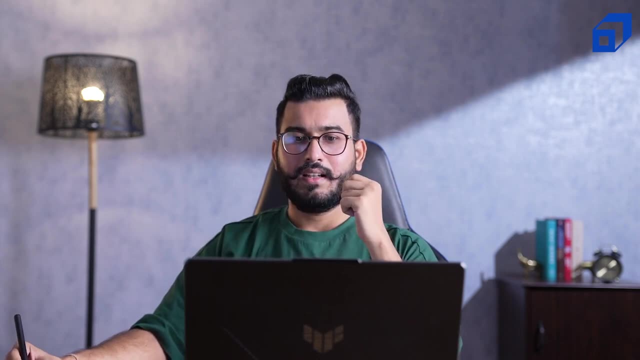 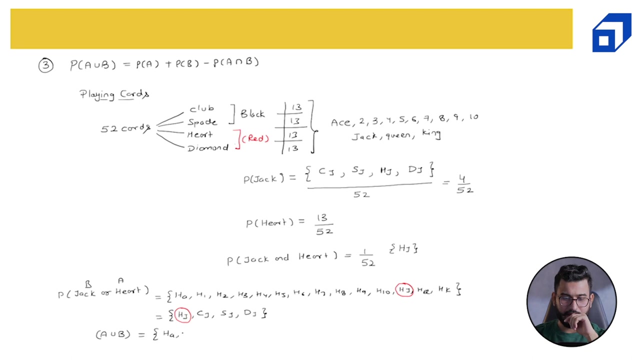 Let me just quickly circle it. So, heart of jack, this card is available in both these sets, and if I have to combine these two sets, I have to count this particular card only for one time. So if I write down All the combined event, it will be from heart of ace, heart of one, heart of two, heart of three, four, five, six, seven, eight, nine, ten. 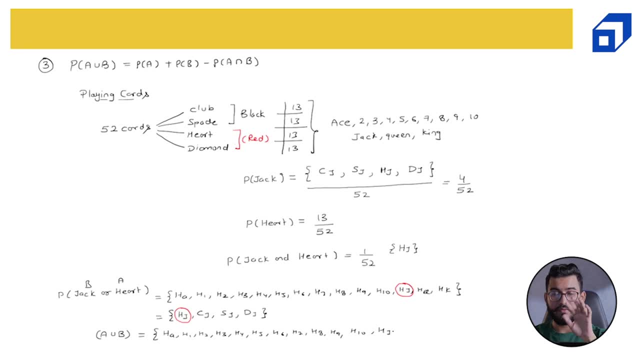 Then heart of jack- Now I have counted it already for one time- Then heart of queen, heart of king, and then I will write down these three cards, which is cj, cj, sj and dj. Now how many events I am having in this. 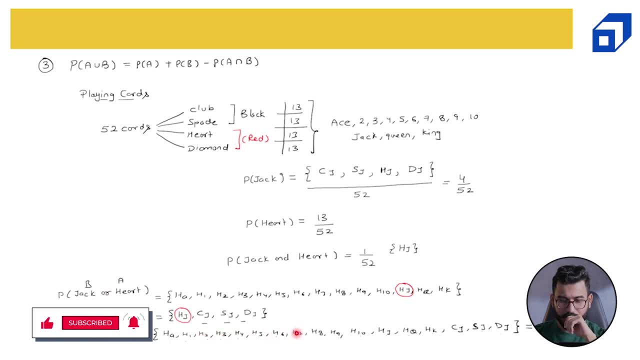 So one, two, three, four, five, six, seven, eight, nine, ten, eleven, twelve, thirteen, fourteen, fifteen, sixteen, seventeen. The mistake is: this is not h1,, this is h2.. So after ace it starts from two. 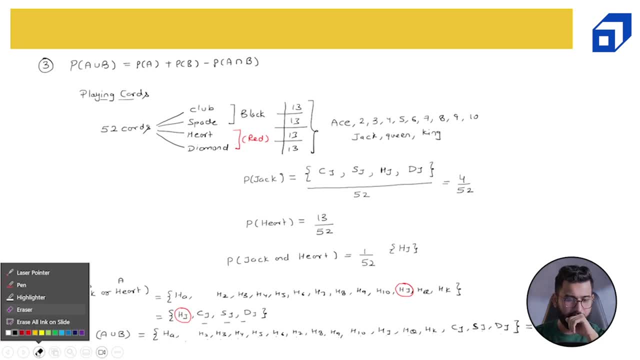 So I haven't read. I should not be writing this. In that case, my outcome will be 16 divided By 16, divided by 52.. Probability of jack or heart is simply 16 divided by 52.. Now, if I go with the formula, what is the probability of getting heart? 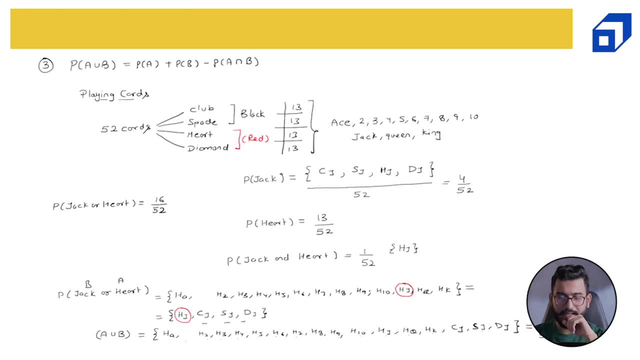 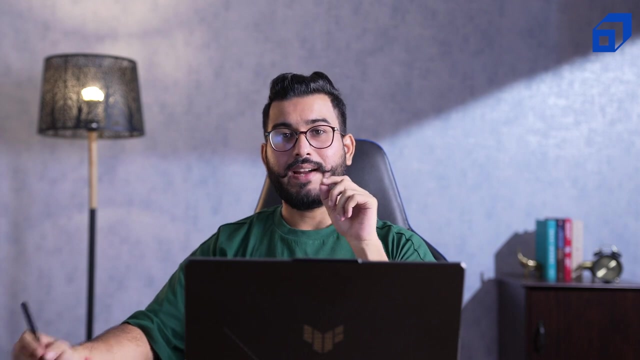 It is one, two, three, four, five, six, seven, eight, nine, ten, eleven, twelve, thirteen. So this is why 13 divided by 52.. This is four divided by 52.. Right, If I add them without subtracting this common event, I will be basically counting this card for two times, which is wrong. 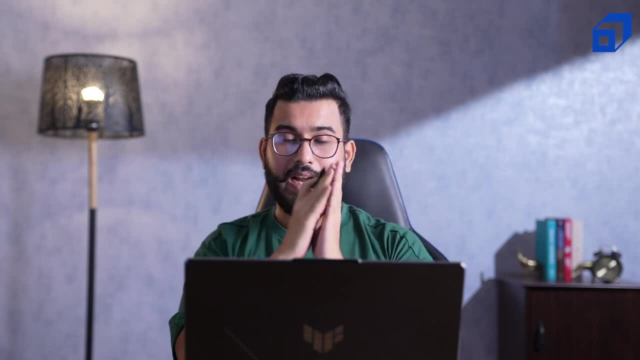 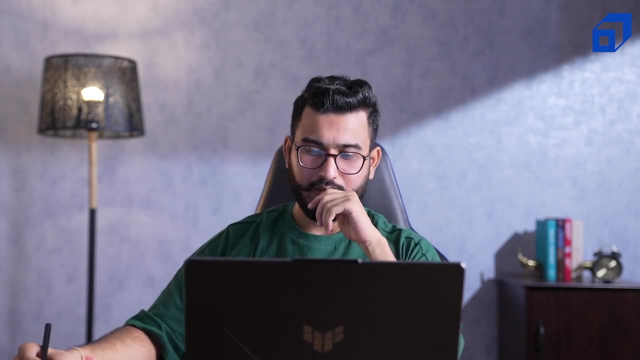 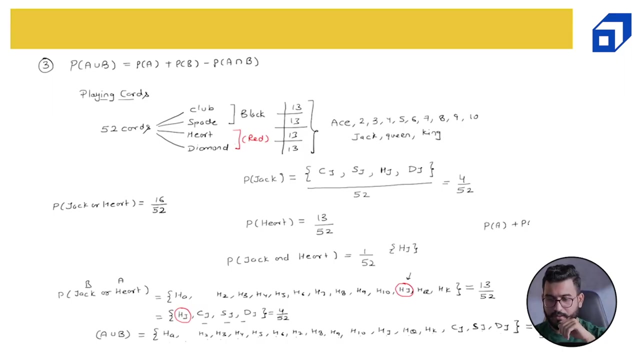 Right. If I have to add these two set, I have to make sure that I'm just counting this card for one time because, logically, I have only one card Right. So that is the reason when I'm combining them, I will write probability of a plus probability of B minus the common card. 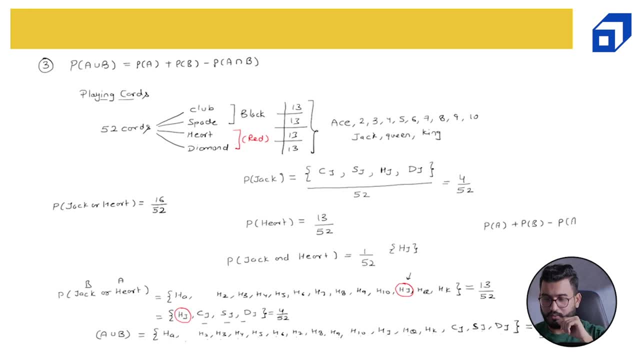 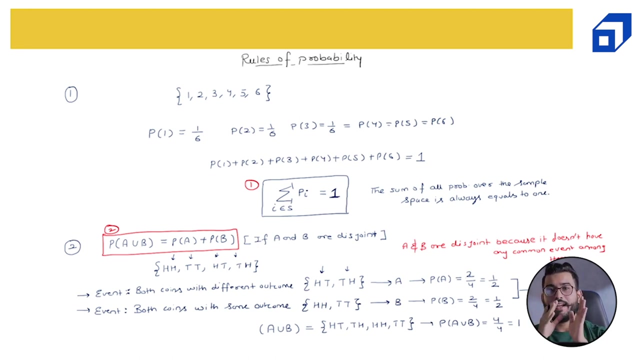 Or common event which occurs in these two set. So A and B. Now, if A and B is 0, A and B can only be 0 when the two sets are disjoint. I will go back to my rule number two. So if A and B are disjoint, probability of A intersection B is zero. 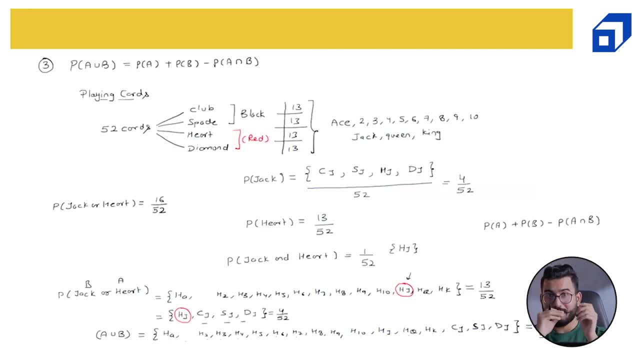 When A and B are joined basically mean they have a common event. Then my probability of A or B Pay A. You can go with this. B is equal to probability of A, which is 13 by 52 plus 4 by 52 minus 1 by 52. 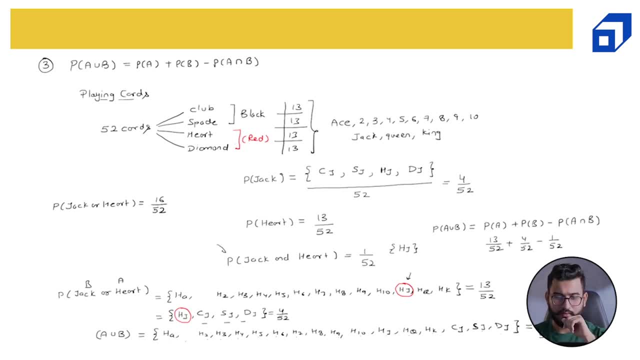 because I am having one card which is common and I have calculated it over here. So this will be total of 16. sorry, 17 minus 1, which is 16 divided by 52, which is my third rule of probability. I hope every one of you are clear with. 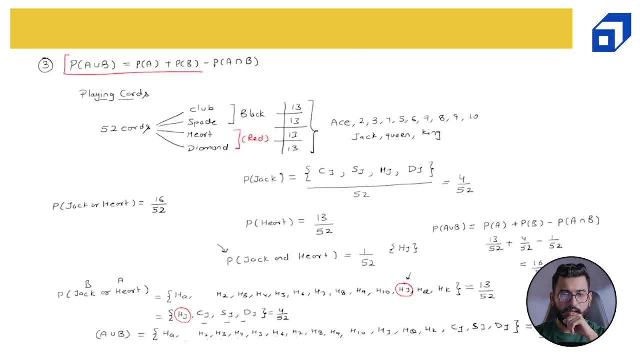 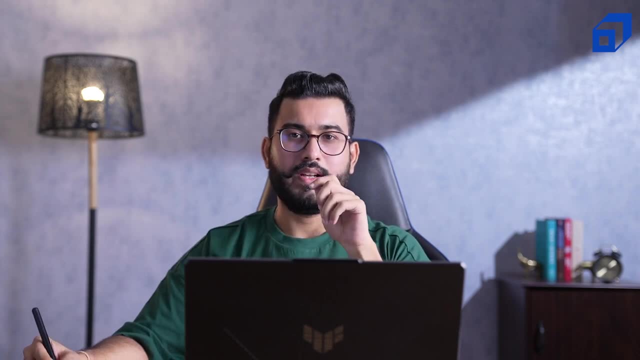 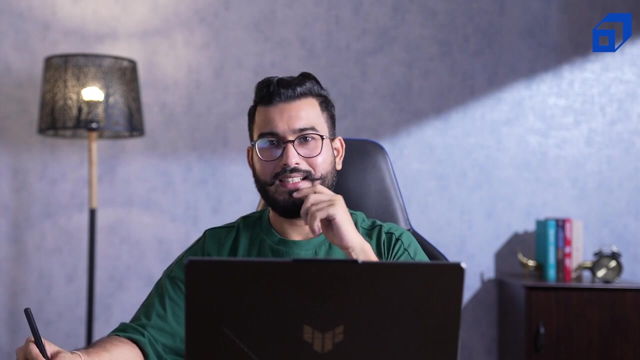 this. This is my third rule. Now let's look at the one final rule, which says: probability of A plus probability of A complement is always equal to 1.. Let's try to understand that. Now the fourth rule and the final rule is probability. 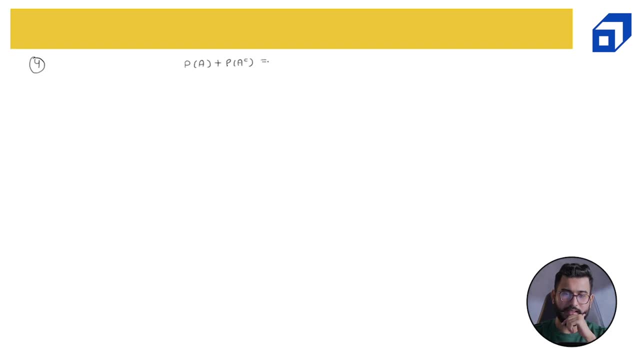 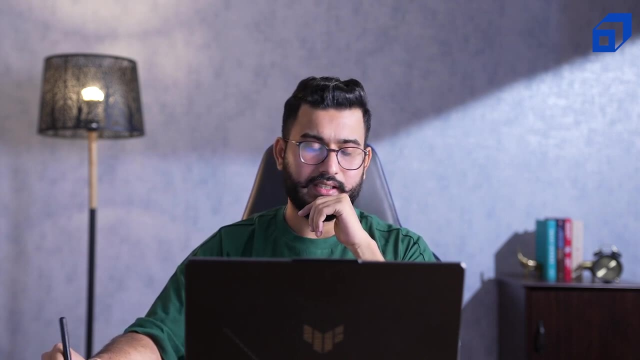 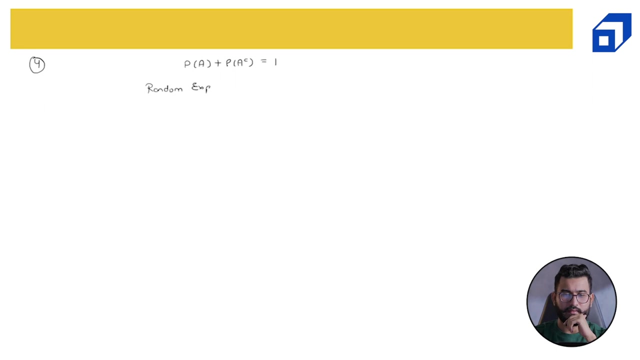 of A plus, probability of A complement is equal to 1.. What is the meaning of this? We have already seen this, but let's try to understand it again. Let's take an event or let's take a experiment: the random experiment where I'm tossing two coins, So toss of two. 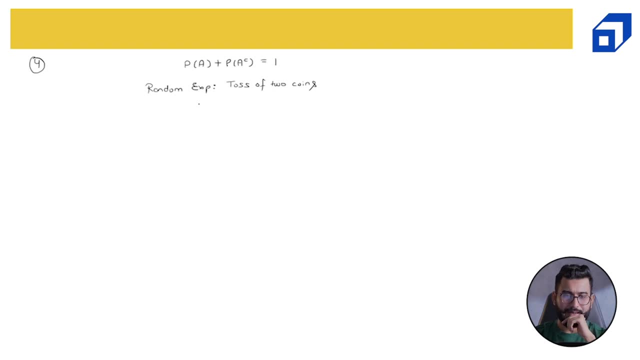 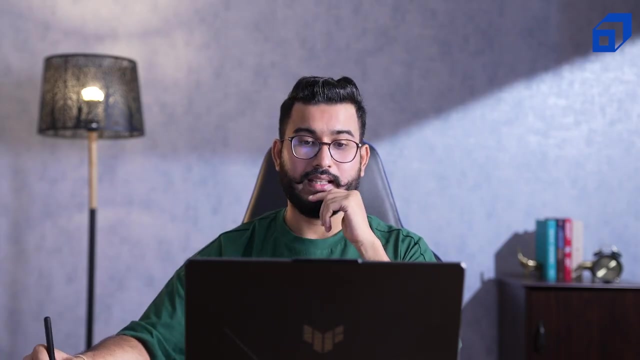 coins and I hope all of you are able to now build the sample space, which is we will get two heads, one head, one tail, one tail. one head, one tail and one head and then two tails. This is my sample space and this is a equally likely sample space. right, because? 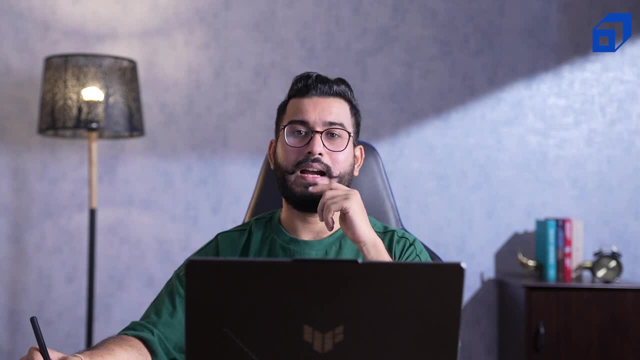 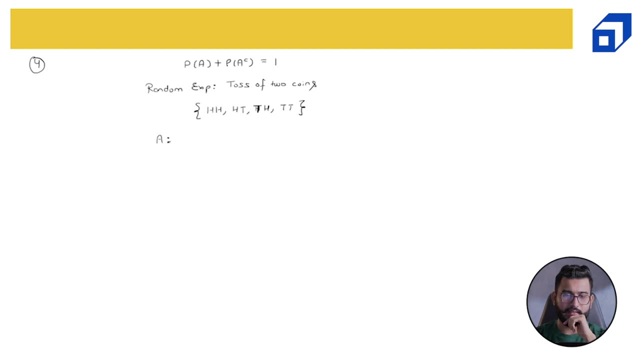 each event is having same probability. probability, right. Okay. Now, if I ask you so, let's say: event A represents both coins. both coins lands lands up with same outcome. both coin lands up with the same outcome. what is the complement of this? what is the meaning of? 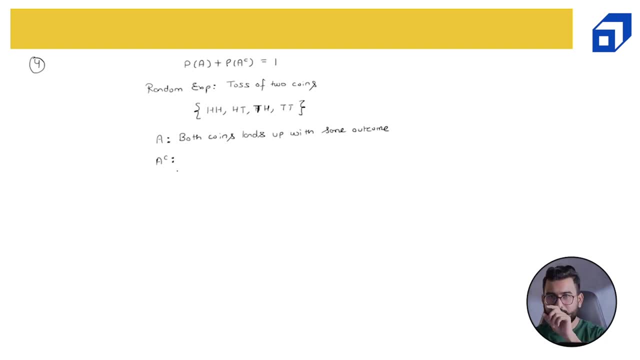 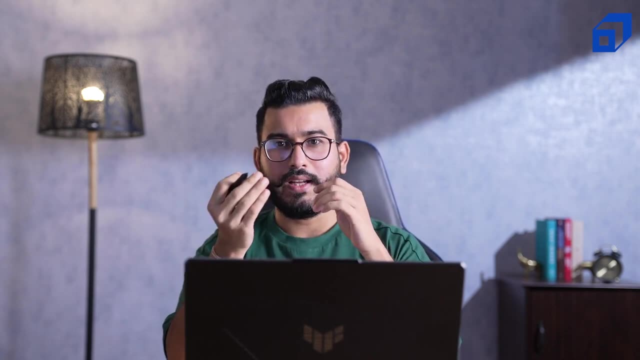 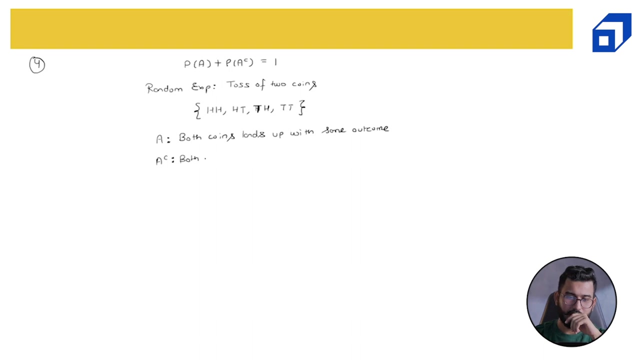 complement, the opposite of this, this, this statement. so I am saying both coin lands up with same outcome. so the opposite of this is both coins did not or does not lands up in the same outcome. so let's write the complement: both coins does not lands up with the same. 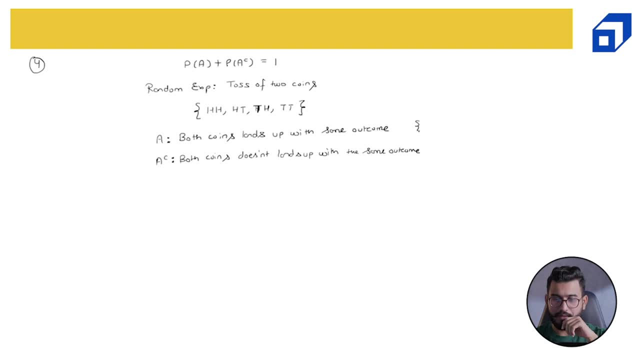 outcome. now, what is going to be the sample event for a? it will be H, H and tail tail. the complement of this will be H, tail head, tail and tail head. now if I add these two probabilities, so probability of A is one by two probability of a complement. 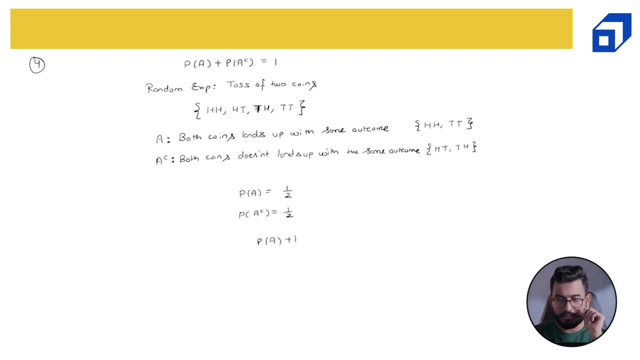 is also 1 by 2, so probability of a plus, probability of a complement is also equal to one. this is a very important rule, because sometimes you need to calculate the probability of a sample space and you just know one event, then it is simply. you can use this. 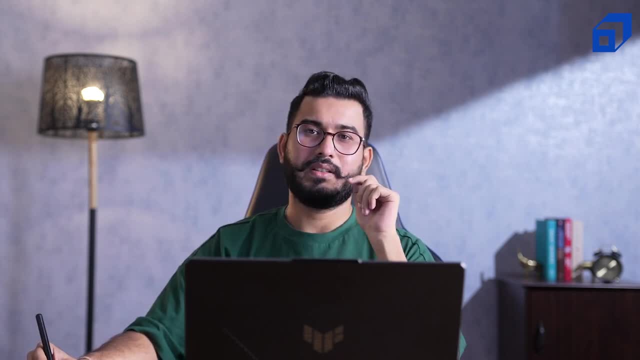 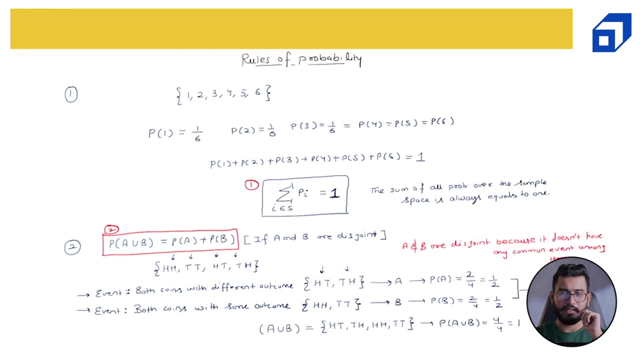 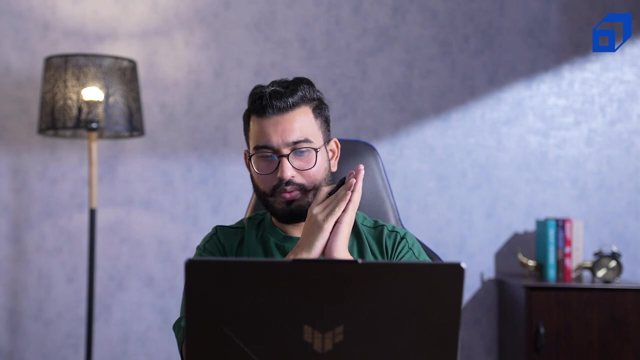 probability rule and you will be able to land up in the probability that you are looking for. i hope all of you are now clear with all the four rules of probability, which is the addition of or the sum of all the probability over the sample space is always equal to one second. one is: 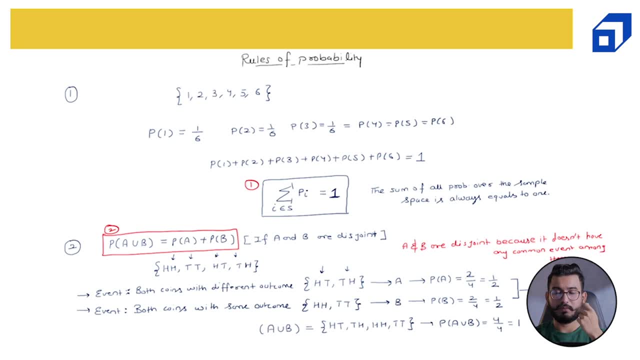 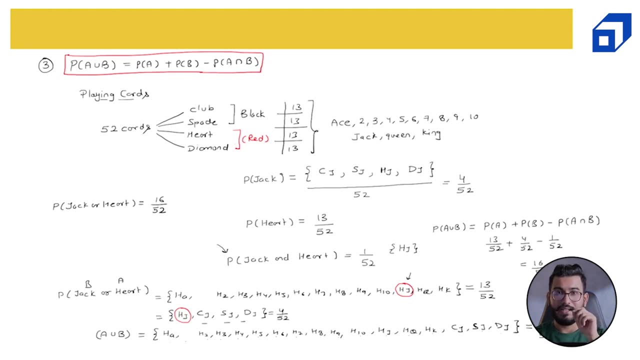 probability of a union b is equal to probability of a plus probability of b if a and b are disjoint. if they are not disjoint, then you have to subtract the probability of a intersection b and final one is probability of a plus. probability of a complement is always equal to one. 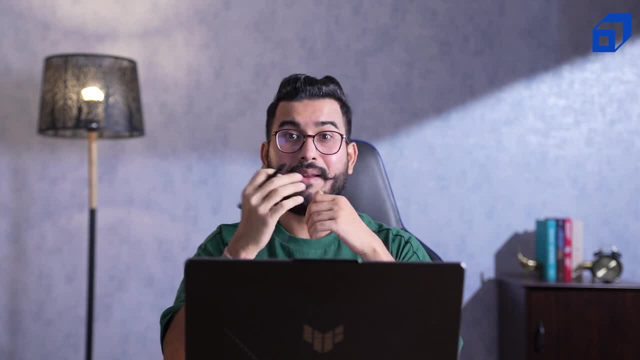 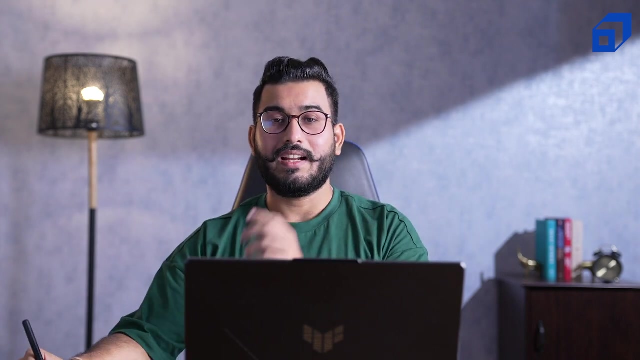 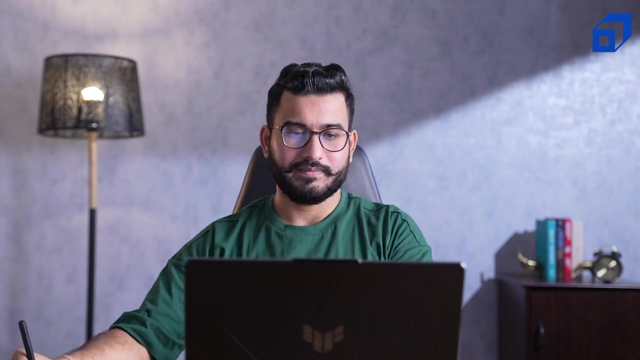 now let's try to understand the various types of events. a particular event or two events can be dependent or independent net. these two terms might be familiar with you, but now let's try to understand them with an example. so now let's try to understand what is particularly: dependent events and independent events. dependent, 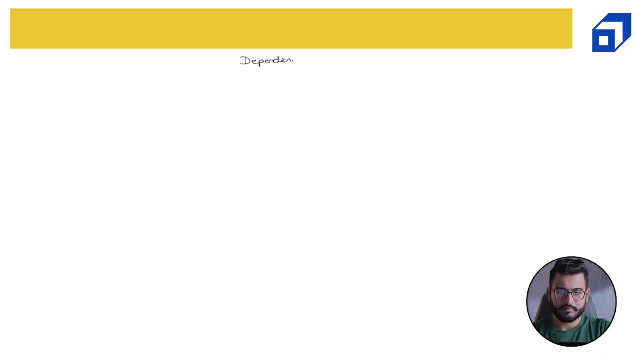 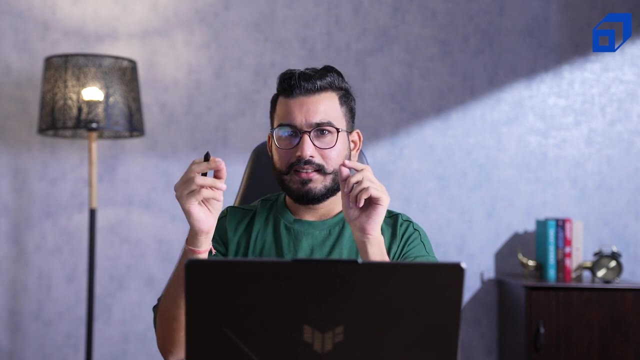 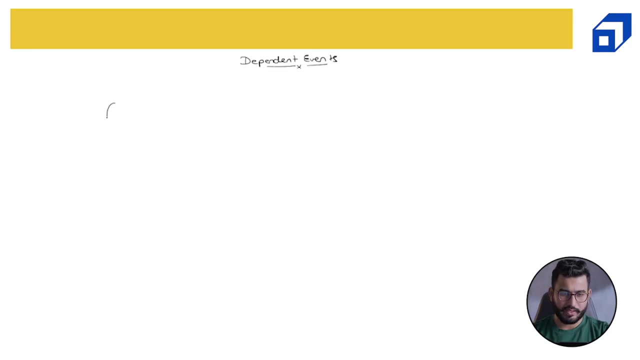 first, we will try to understand the dependent events. when i'm saying events, i'm basically talking about two events or two or more events, right? so let's take two events. i'm tossing a coin, so again my drawing skills, so this is, let's say, this is a coin and this is a fair coin. 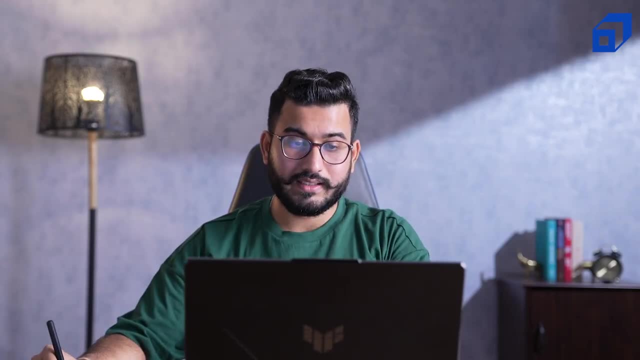 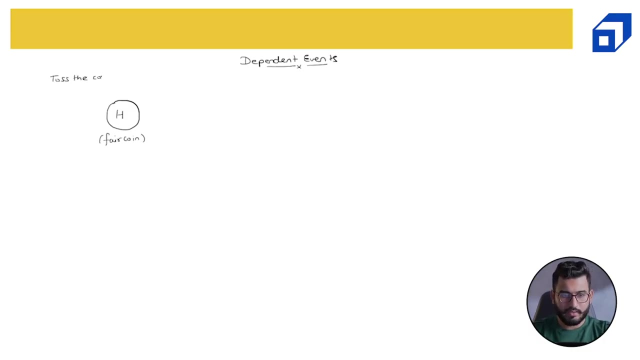 fair coin. now if i toss this coin for two times. so my experiment is to toss the coin for two times. now, when i toss it for the first time, so this is my first toss- when i toss it for the first time and, let's say, heads appeared, so let me write it down. when 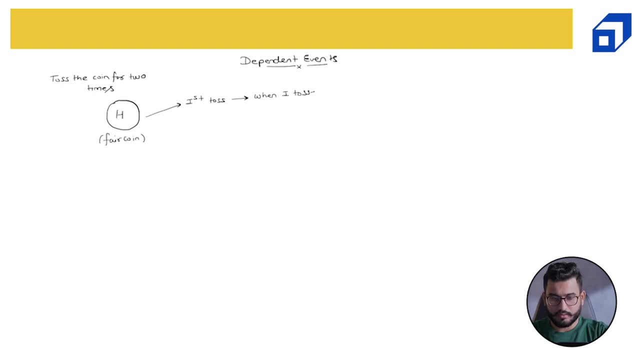 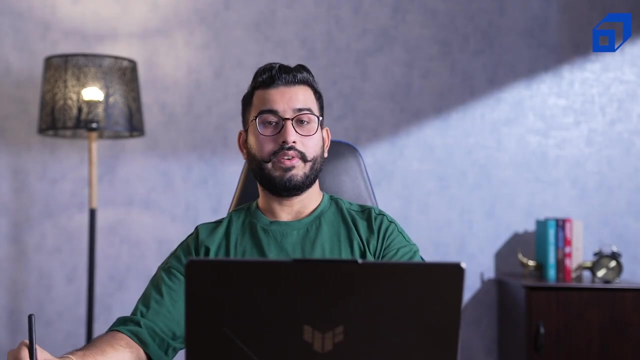 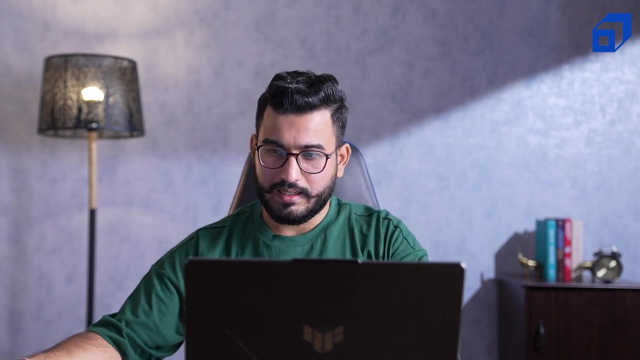 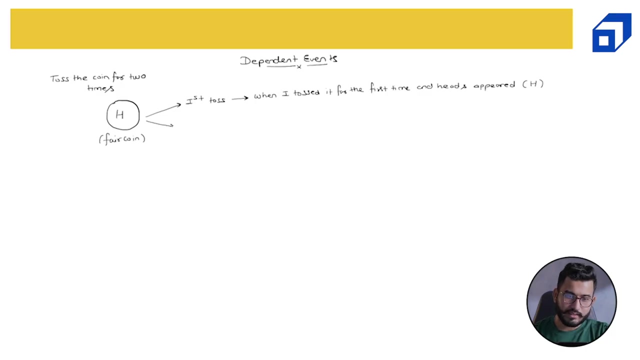 i tossed it for the first time and heads appeared. so we know that when i toss the coin and it lands up into head, you know this. so i'll let me write that the outcome of the first, the outcome of the first toss, is head now when i'm tossing the same coin for the second time. so second toss now. remember the coin is same. 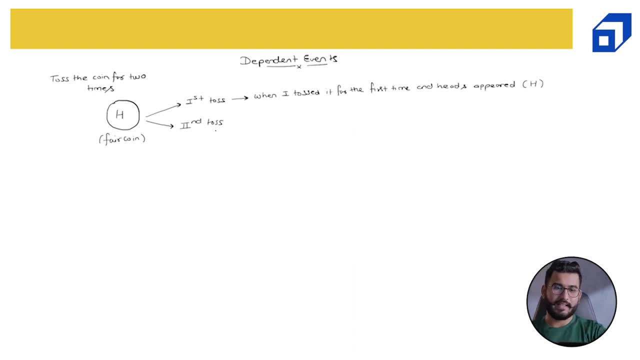 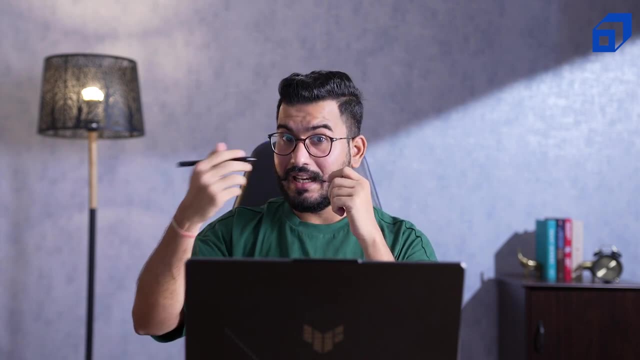 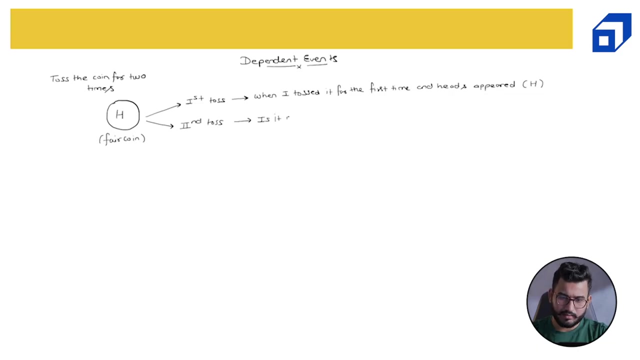 i'm having the same coin, but i'm tossing it for a second time. now, when i toss it for second time, is it more likely that i would get a tail, because the first one was head? so my question to all of you is: is it more likely that we would get a tail, since the first outcome was 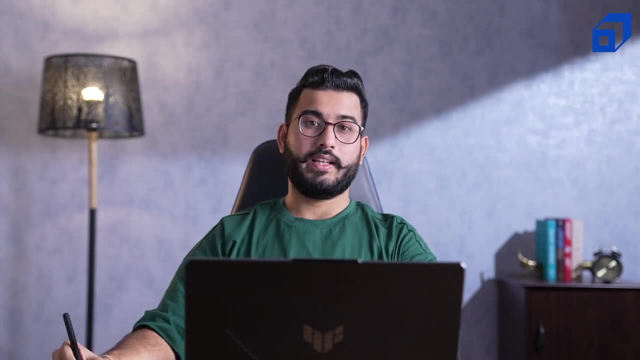 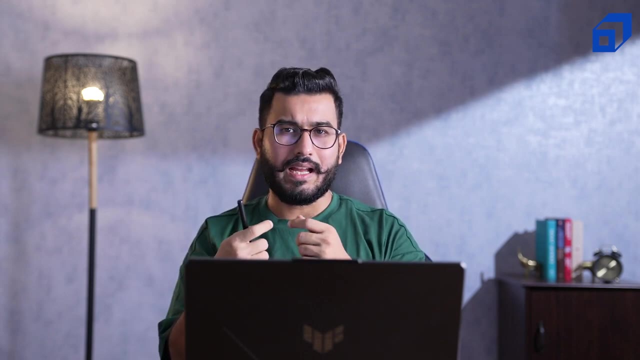 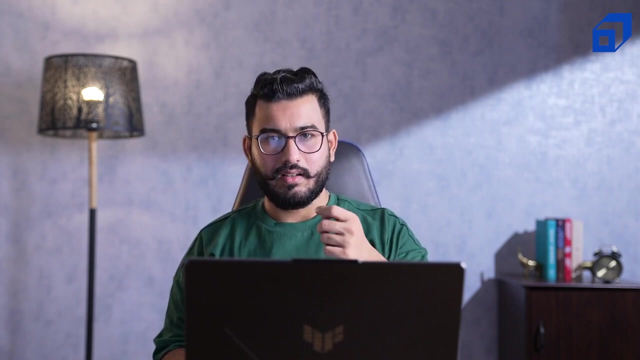 head. now all of you would say no, why? because the next outcome can again be having the probability of getting head and tail to be equally likely, which basically means, if I am tossing it for first time, I may either get a head or a tail. and what is the probability of getting head and tail? 0.5. 0.5, which is 1. 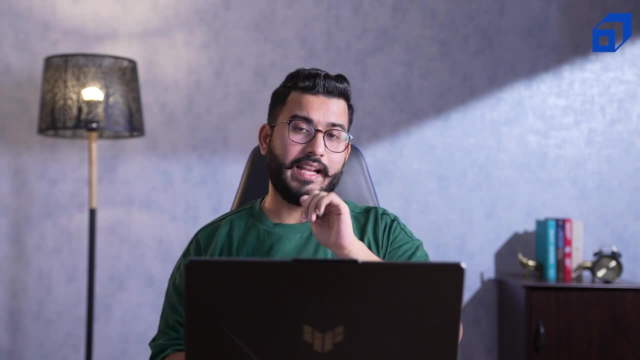 by 2. 1 by 2. if I toss the same coin for the second time again, the probability of getting head and tail is 1 by 2. 1 by 2, which is 0.5, 0.5. so what I'm trying to. 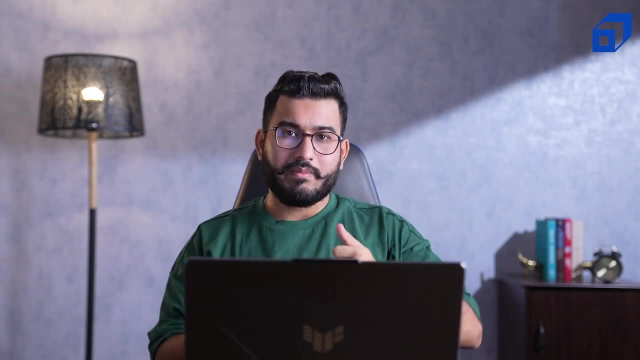 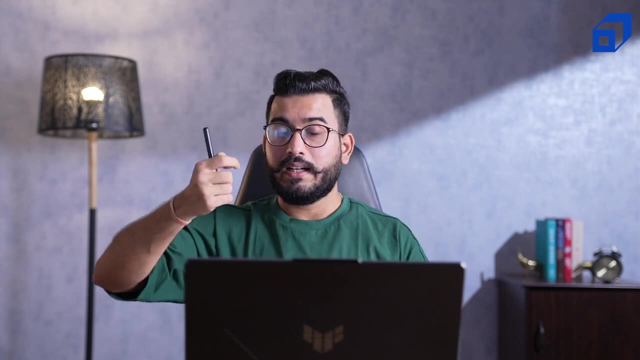 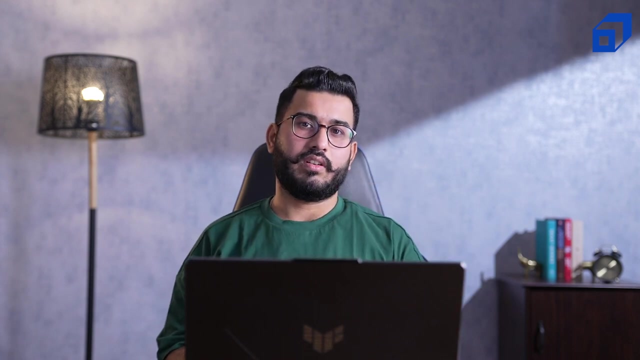 say is: if I toss the coin for first time and if I toss the coin for second time, these two tosses are independent of each other. the probability in my in the second toss is not getting influenced with the outcome of the first toss. okay, if my outcome in the first toss is head in the second toss, it does. it is, it is. 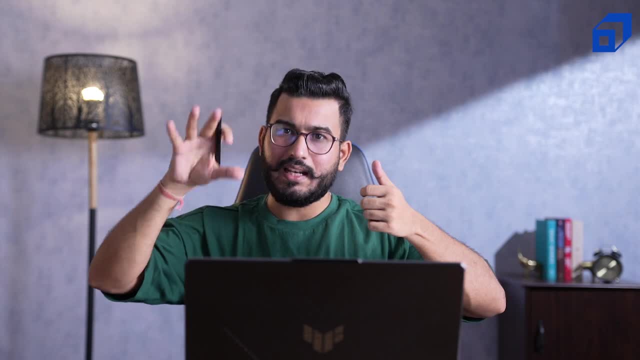 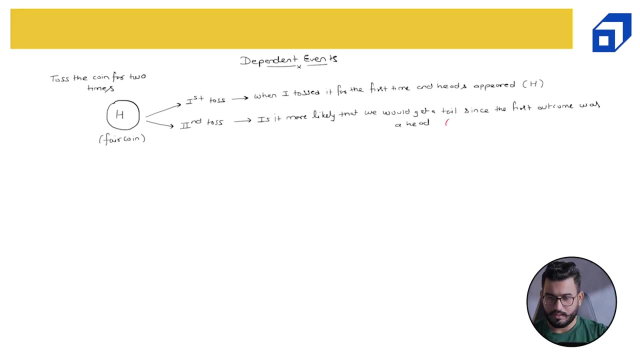 not influencing right in the second toss it is, it can be still be head or tail. so in simple words, first of all, the answer for this question is no, so I'll write a big no over here and the the rule is the outcome of the first event. 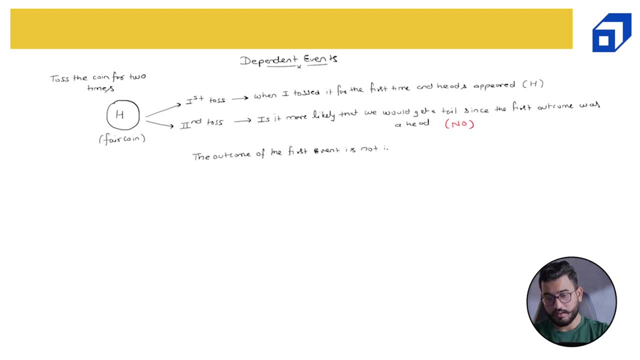 is not impacting the outcome or the probability- the outcome of the probability, probability of the second event or the second toss- and hence they are independent events. independent events, independent events. so if I toss a 10th time, another thing which is the probability of this game is being. postponed, then over a heltita I'll graduate Westma on how to get head or tail, and tail he says six, 5, 5, 11, 4, 10, 7, 8, 10, 7, 9, 10, 8, 11, 7, 9, 10, 8, 1, 2, 2, 3, 2, 2, 2, 3, 2, 2, 1, 2, 2, 2, 2, 2. 1, 3, 13, 8, 9, 9, 9, 9, 9, 9, 9, 1, 10, 9, 9, 9, 9. money. an thirds, he has not impacted the outcome of probability. the outcome of probability, the outcome or the probability probability of the second. 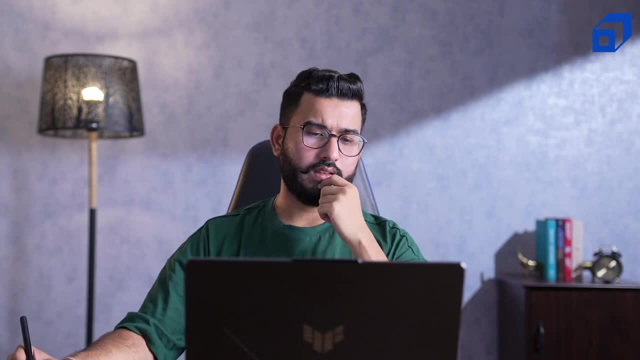 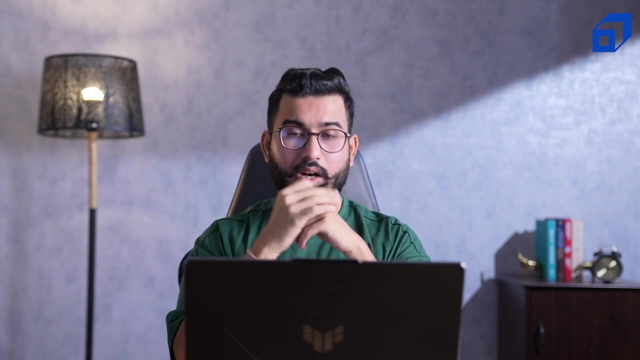 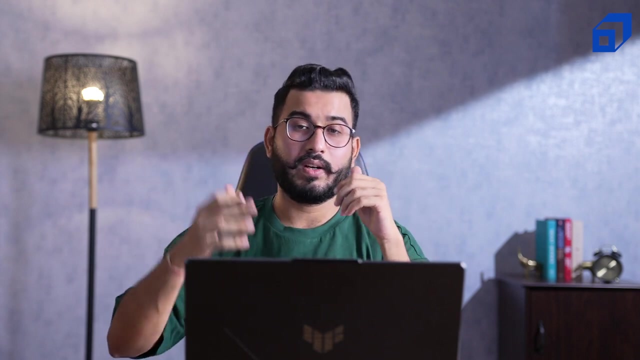 Now there is a very good. so in probability theory there is a topic known as gambler's fallacy. What gamblers think that? if so, let's say, if the game is of tossing a coin for 10 times, Now let's say there is a gambler who is given with the choice, who is given with 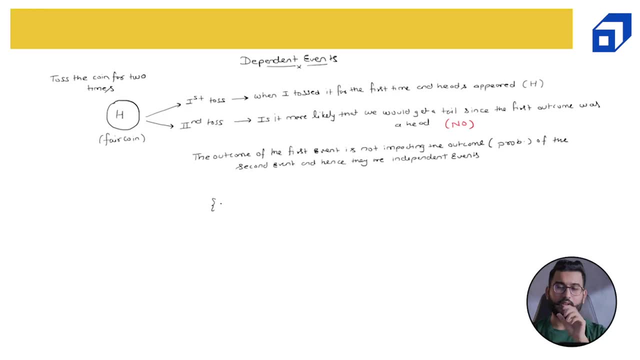 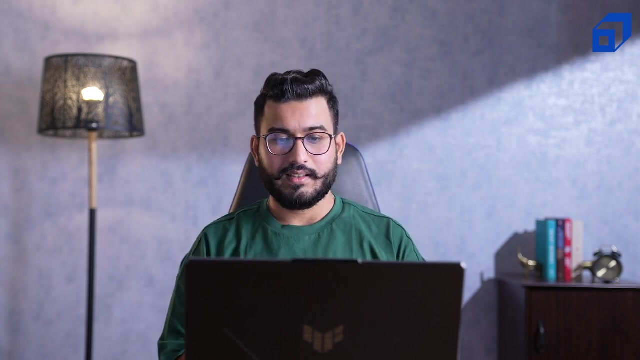 the game to toss the coin for 10 times. For the first five times, let's say, he has got all tails. So tail, tail, tail, tail and tail. So for the first five times he has got all the tails. Now what gambler's fallacy is that he will think that for the next five? 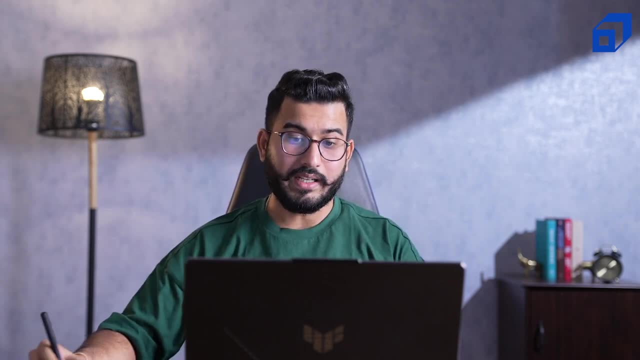 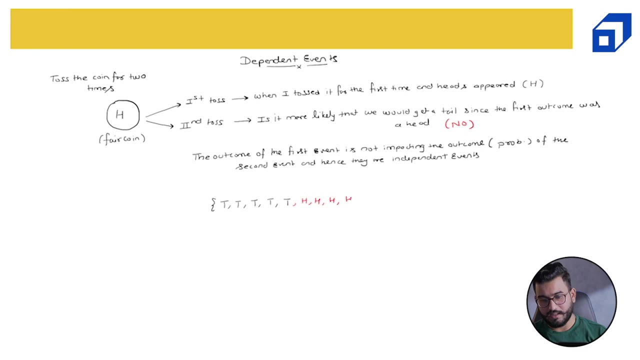 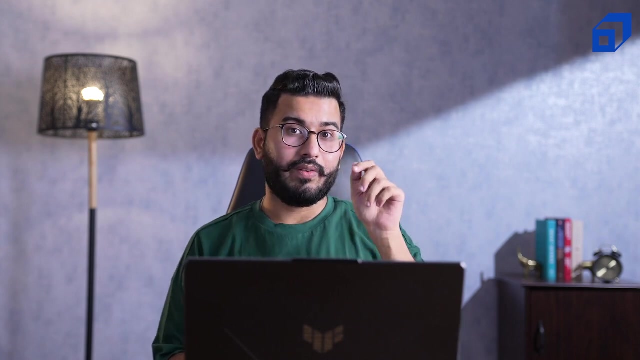 times he will get a head. So, according to gambler's fallacy, the outcome for next five tosses Should be head, head, head, head and head. Why? Because, according to the probability of head and tail, it should always be 0.5, 0.5.. No, that's wrong. It is only true when. 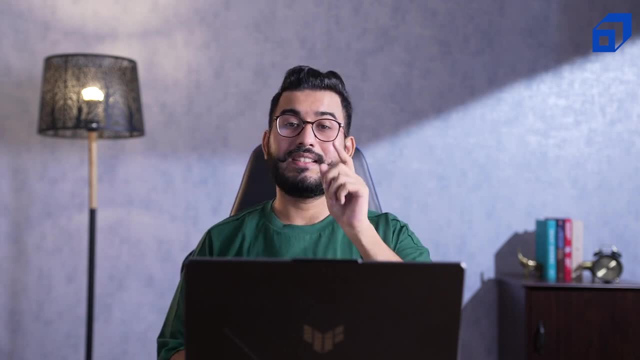 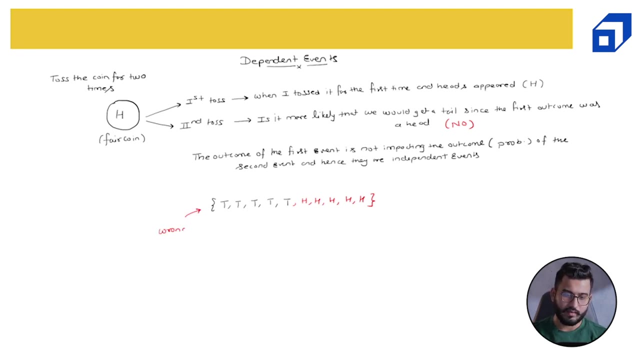 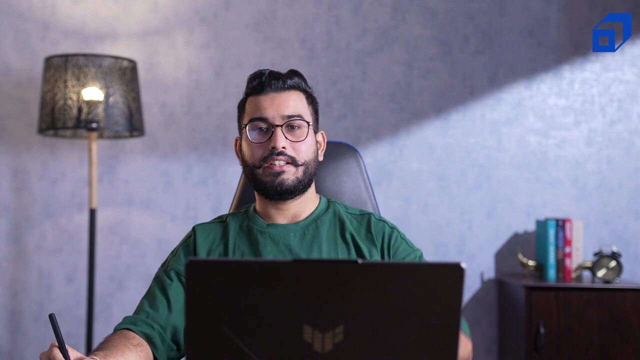 you are tossing the coin for very large time. That's known as the law of large number. So this is known as gambler's fallacy. This is wrong. This is wrong. This is only true when you are tossing the coin for very large time. So if I keep tossing the coin, let's. 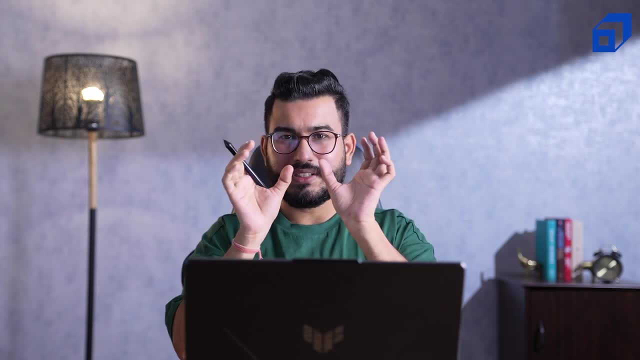 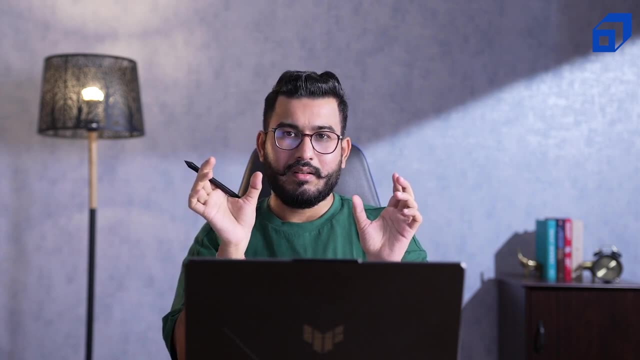 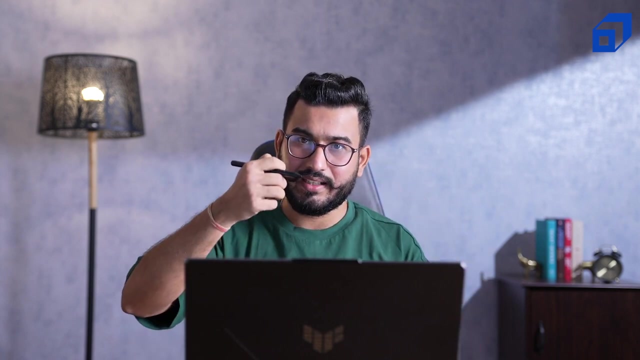 say, for 10,000 times, you will find out that approximately for 5,000 times you obtained a head and 5,000 times you obtained a tail. But if you are tossing the coin for two times and you expect that I will definitely get head for first time and tail for second time, 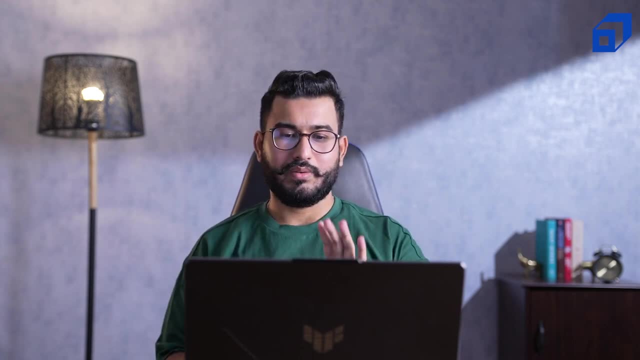 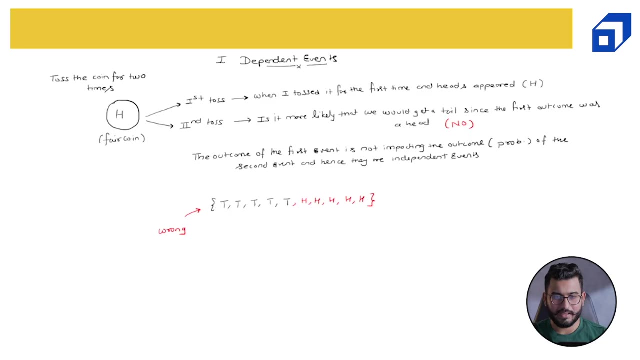 that is wrong. That is the gambler's fallacy. So I hope you guys will not be disappointed. Thank you, You will not be landing into the gambler's fallacy and I hope you are clear with the dependent event: Independent event independent. So when two events are independent, the probability 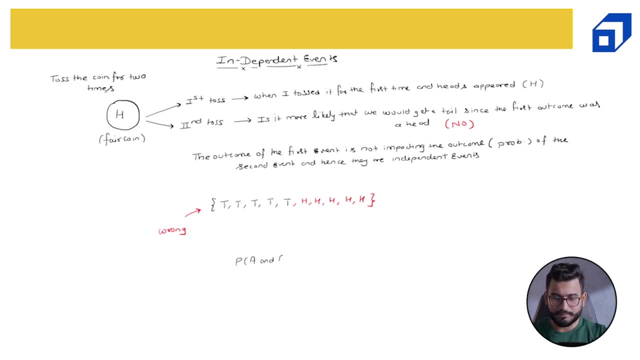 of A and B is simply as probability of A multiplied by probability of B. So, for example, probability of getting head in first time Toss and probability of getting head in second toss is simply can be written as probability of head in first toss multiplied by probability of head in second toss, And this will be equal. 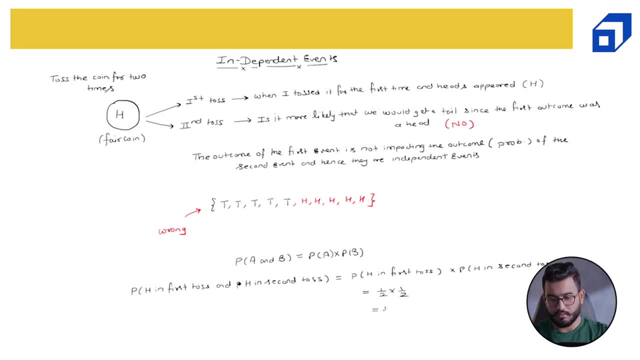 to 1 by 2, multiplied by 1 by 2, which is 1 by 4.. So that is what you are going to get. You will get head and tails. head and tails will be equal to 0.5.. 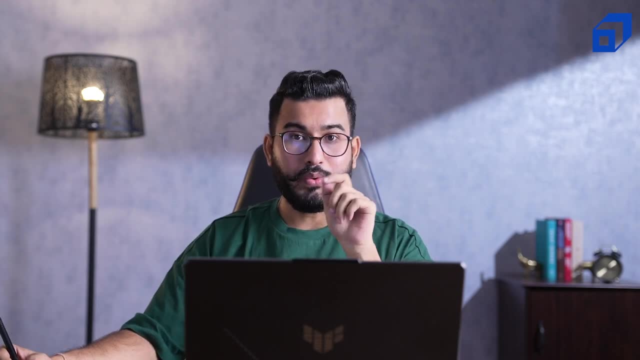 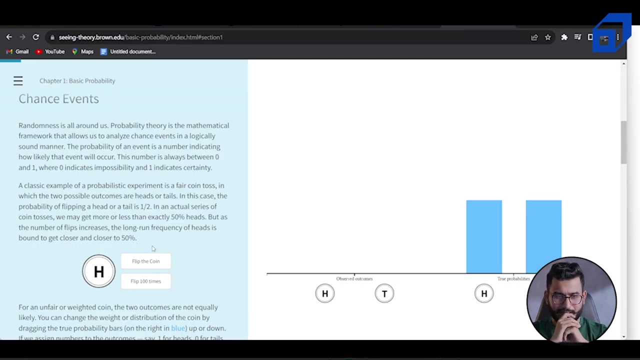 I hope you guys are clear. Let me just quickly show you one example of gambler's fallacy which proves that when you toss a coin for a very large time, then only the probability of head and tail will be closer or approximately be equal to 0.5 and 0.5.. Now here you can. 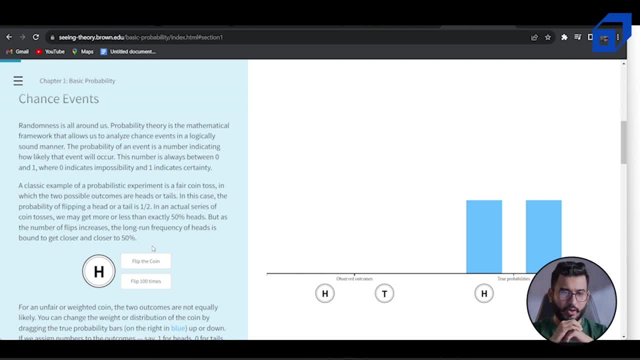 see, there is a very cool website which is seeingtheorybrownedu. this is open-source website. Now it shows these are the true probabilities. basically mean the probability of head is 0.5, for tail it is 0.5.. Now I can flip the coin. so if I flip the coin for the one time, 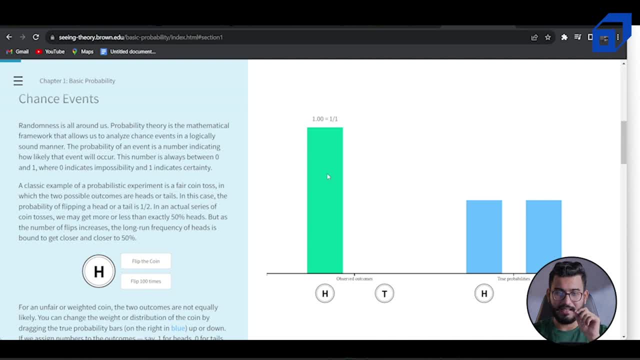 you can see that for the first time, I obtained a head, so my probability of getting head is 1 by 1.. If I flip it for one more time, I obtained a tail. so 1 by 2, 1 by 2.. If I flip it for one, 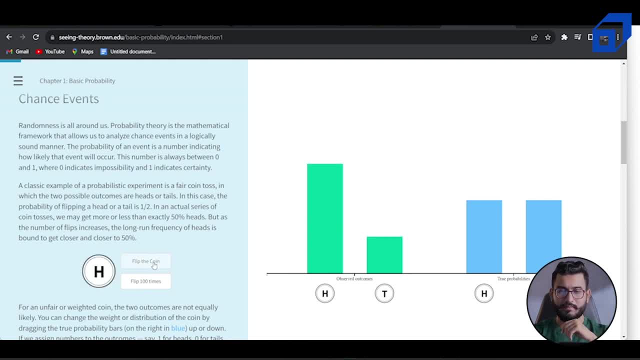 more time. I obtain a head for one more time again. a head for one more time, a tail for one more time, a tail for one more time, a head. Now, if I do it for 100 times, I obtained out of 107 times. head came for 57 times, tail came for 50 times. Let me do it for one more 100 times. 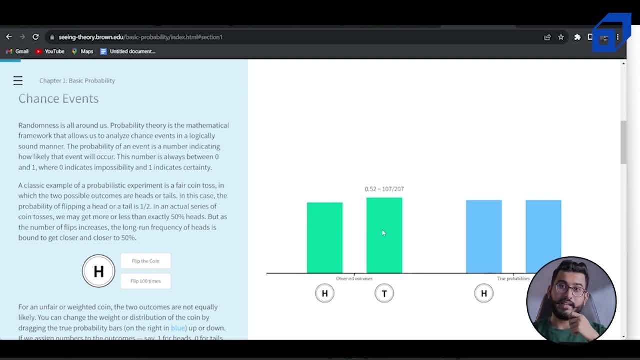 Now you can see that now the probability of tail is more than the probability of head If I do it for 1000 times. so, which basically means I have to hit this button for 8 more times. so 1,, 2,, 3,, 4,. 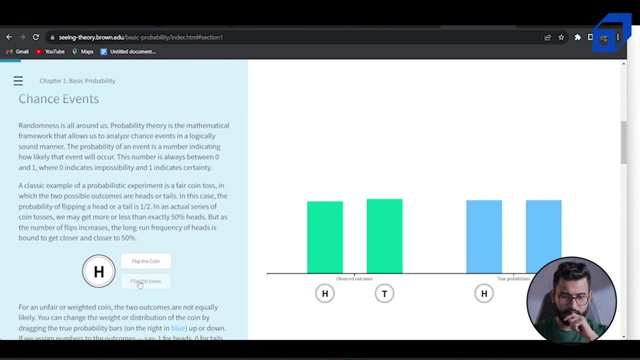 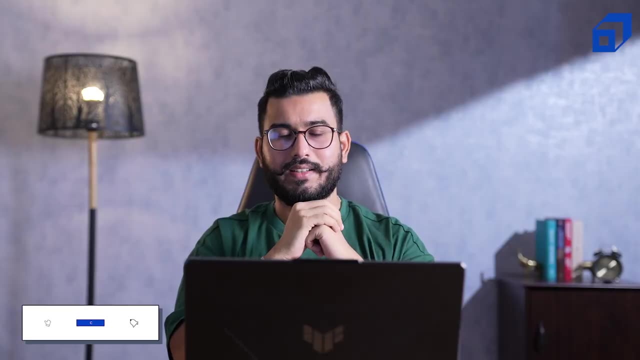 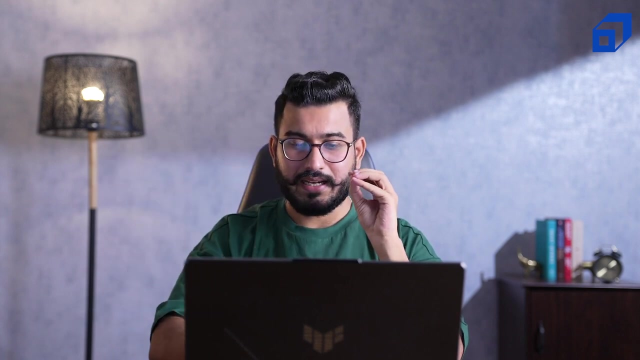 5,, 6,, 7, and 8.. Now just look at this: 0.49, 0.51- very close to 0.5- and 0.50, right. So this is the law of large numbers. if I perform the experiment for very large time, then my observed outcome, or observed- 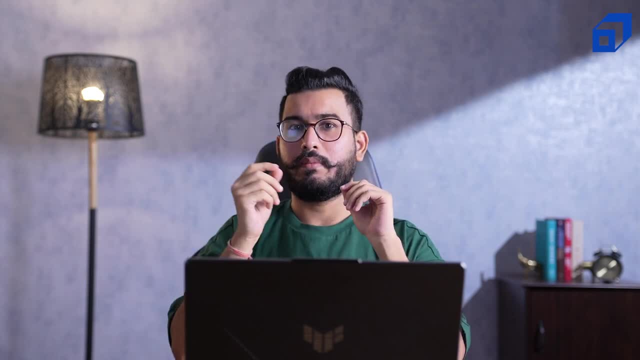 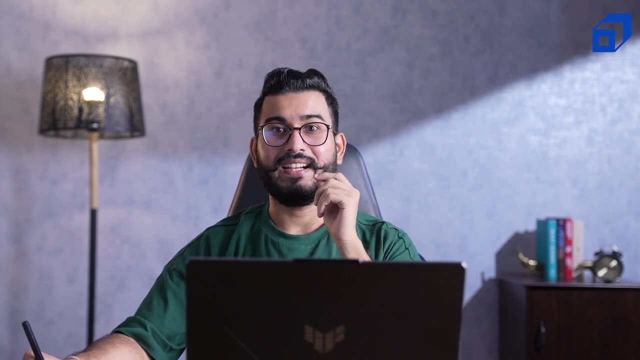 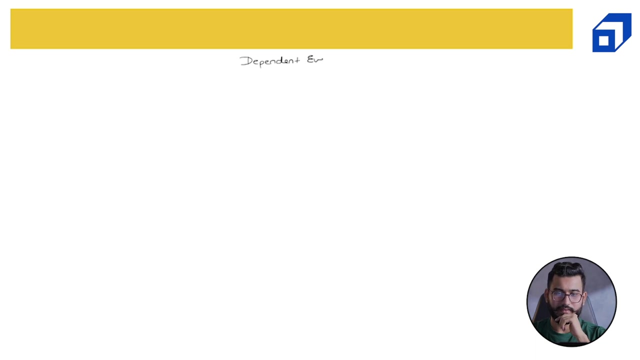 probability will be close to 0.51.. to the true probability, which is 0.5 and 0.5.. I hope this makes sense to all of you. So now let's talk about dependent events. So dependent events. Now for dependent events. 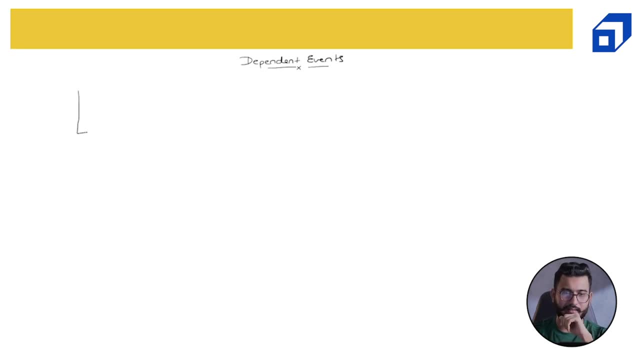 we will take a very simple example. Let's say I'm having a bag And this bag is having, let's say, two orange balls. We have two orange balls And, let's say, some white balls For white balls. I'll draw it like this: One white ball, two white ball and three white balls. 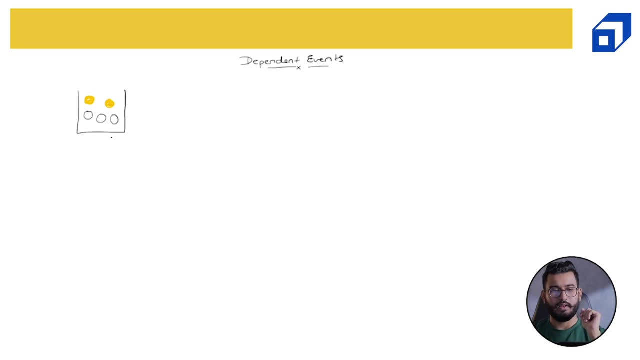 So, total, I'm having 5 balls in which there are two orange, three white. So let me write it down: two orange and three white. Now the experiment is: we take a ball out of the bag. so take a ball out of the bag. we have to note the color. so note down the color. 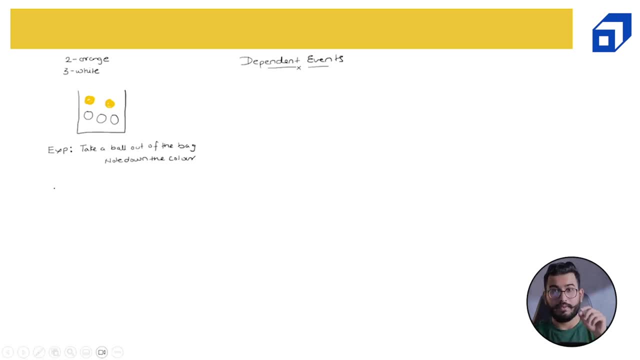 and we put another ball. we'll take out another ball out of the bag. so take one more ball out of the bag and then we note the color of that ball also. note down the color. Now please carefully remember that this experiment is without color. 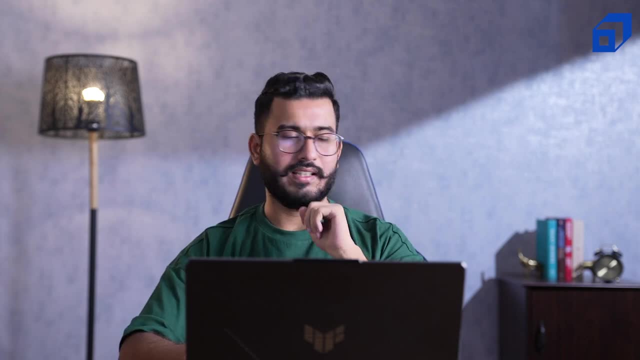 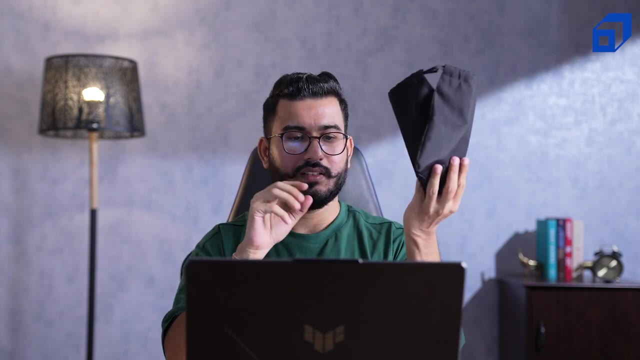 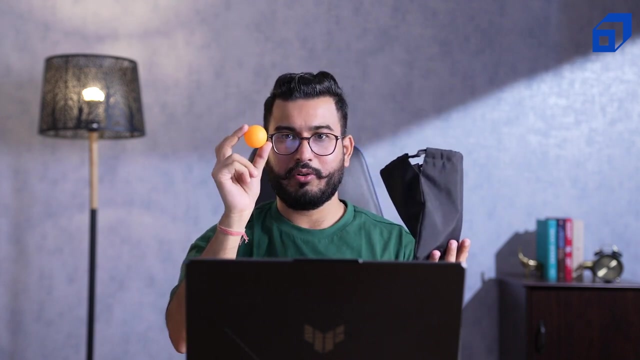 So let me just quickly demonstrate this example. Let's say this is my bag and this bag is having two orange balls and three white balls. Now what is the experiment? I have to take a ball out of the bag. so this is my orange ball. 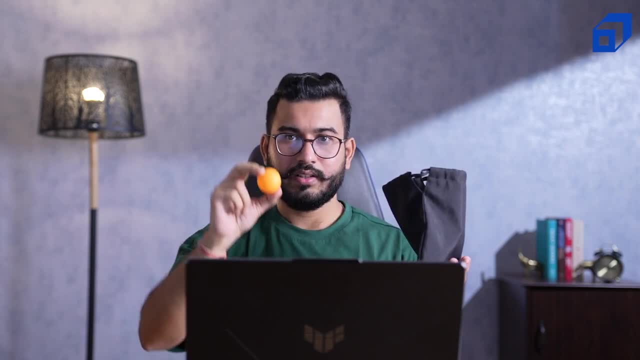 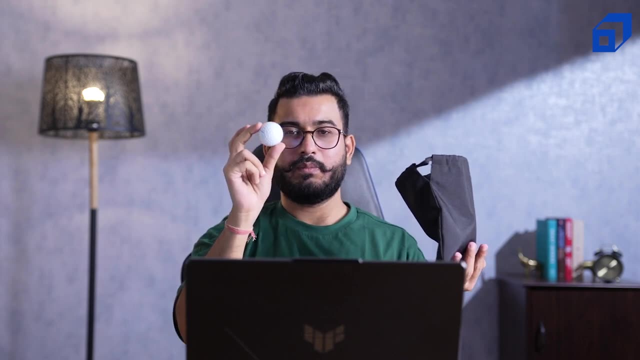 and I note down the color. so we will write orange and we keep it outside. Then we again take a ball out of the bag. this is a white ball. we will note down the color and we will keep the ball out of the bag. 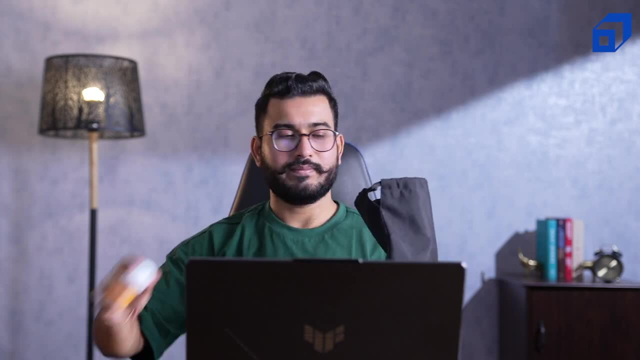 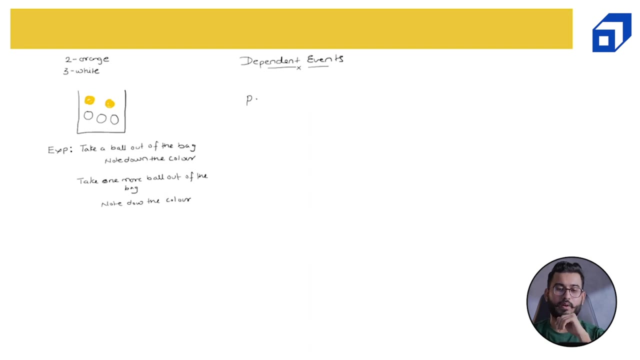 So this is what is my experiment. I hope everyone is clear. Now my question is: we have to calculate the probability that I get a orange, so O. so first ball happens to be orange, second ball happens to be white. So what is the 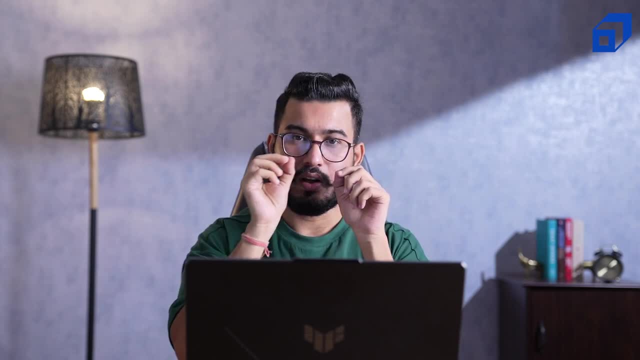 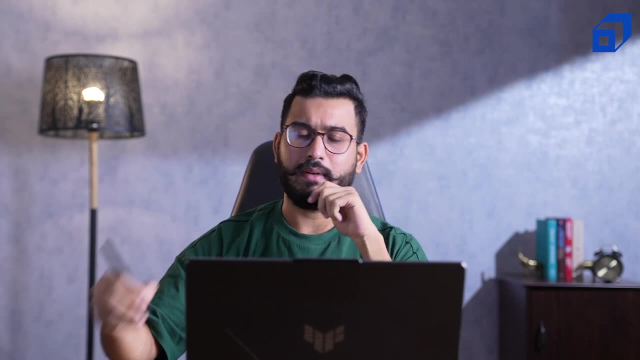 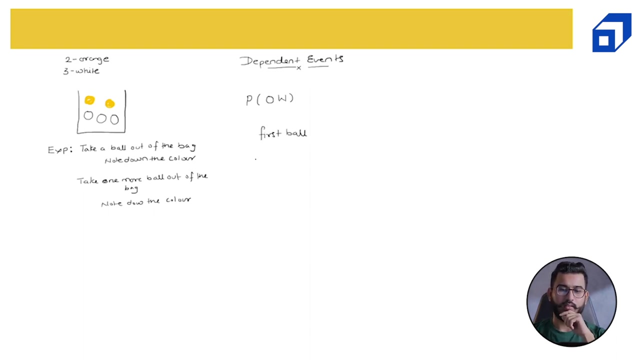 probability that I will get first ball as orange and second ball as white. Now let's solve this problem step by step. When I am taking out the first ball- so this is my first ball, first ball- when I am taking out the first ball, the bag is having three white and two orange. 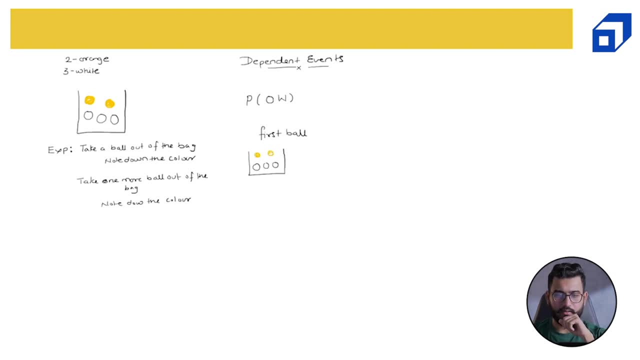 so initial is three white, white and 2 orange. Now what is the probability of getting a orange ball or an orange ball? Probability of getting an orange ball? This is simply be 2 divided by 5. Why? Because I have 2 orange balls and there are total of 5 balls. Now I have taken this ball out. 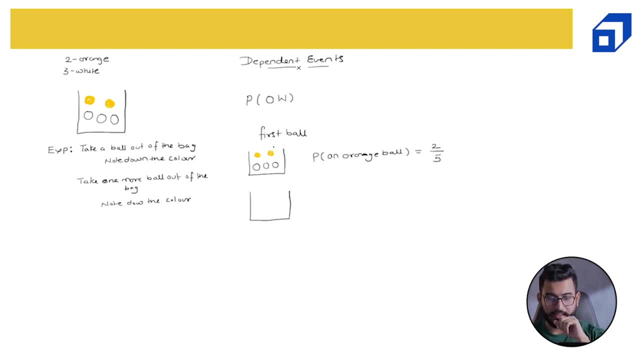 of the bag. So the bag is now. so I will take this ball out of the bag. This ball is out of the bag now. Now the bag is left with 1 orange and 3 white balls: 1,, 2,, 3.. 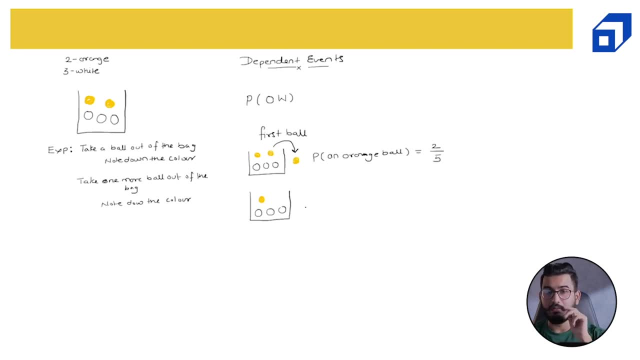 Ok, Now what is the probability that my second ball is a white ball? So, probability of second ball is a white ball, but there is a condition given to us. So, given that, given that, so this symbol means, given that the first ball was orange, 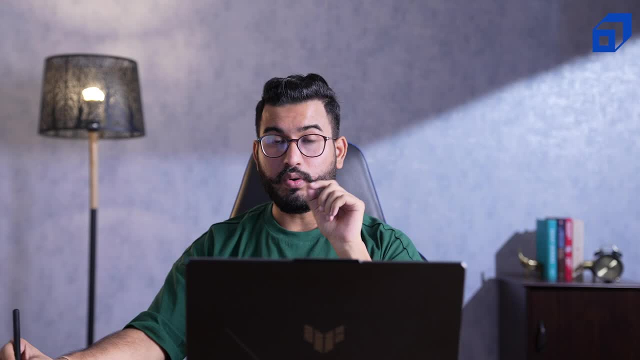 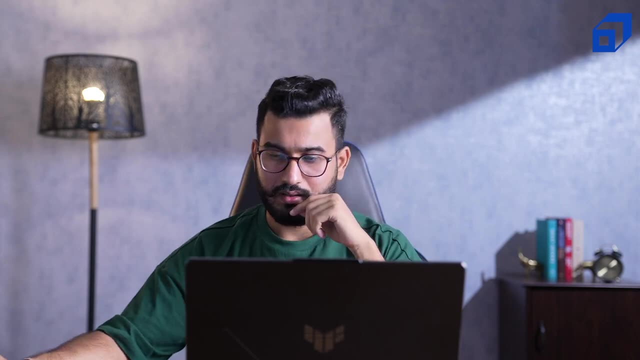 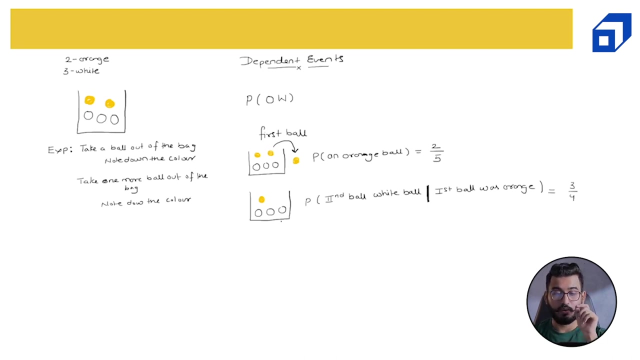 So we know. we know that first ball was orange. Then what is the probability that my second ball will be white? This will be 3 divided by 4.. Because we have 3 white balls and total are 4 balls. Now, if I ask you, what is the probability of getting orange and a white? So what is the 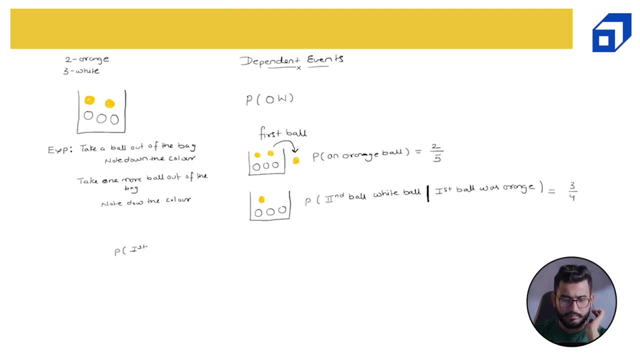 probability of a first ball. Ok, Ok. So what is the probability of getting orange as orange and second ball as white? Now, this will be simply as probability of first ball as orange multiplied by probability of second ball as white. So this is my probability of getting 1st ball as orange and the second ball as white. 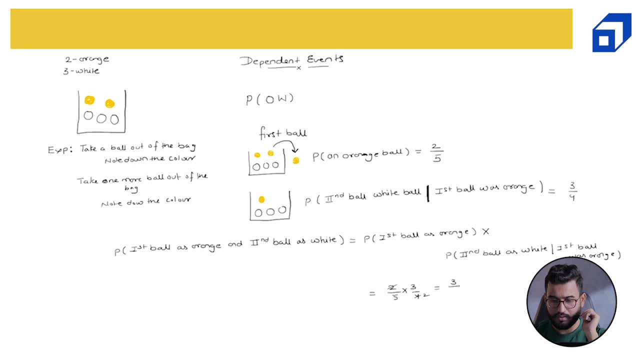 So this will be 3 divided by 5 and 3 divided by 4.. So this is my probability of getting first ball as orange and second ball as white. So this is 3 divided by 10.. Now here, if you carefully understand the experiment, the probability of second ball being white will be 3 divided. 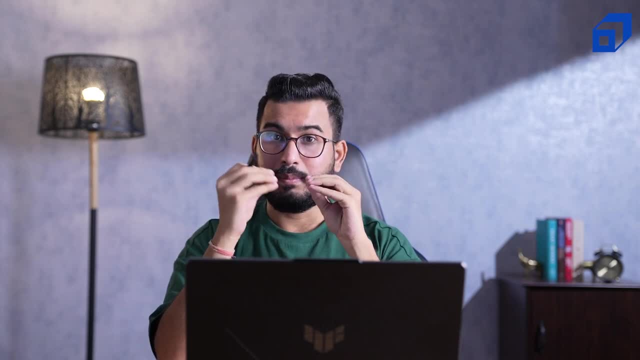 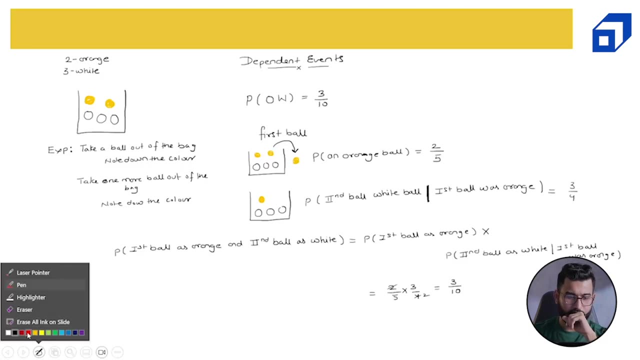 by 10.. What is the probability of getting orange? Ok, is dependent on the outcome of the first trial. So here is a note: the probability of second ball is dependent on the probability or the outcome of the first toss, or first trial, or first. I would say. first trial is a correct word. So this is what is my 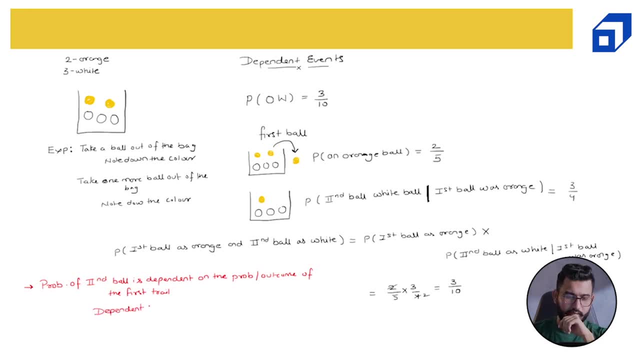 dependent event is dependent events. So when two events- A and B- are dependent on each other, if they are dependent, then the probability of A and B is given as probability of A multiplied by probability of B, given A has already happened. this is my probability of A and B. this is the dependent rule. When two events 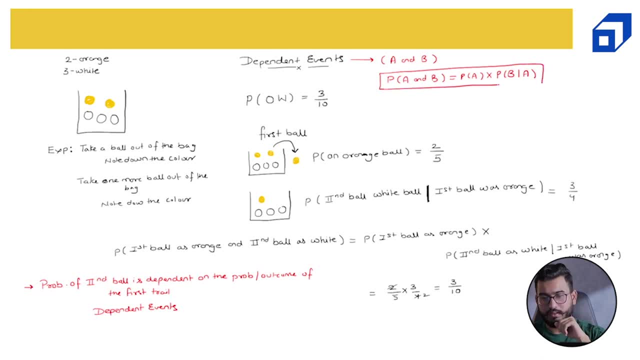 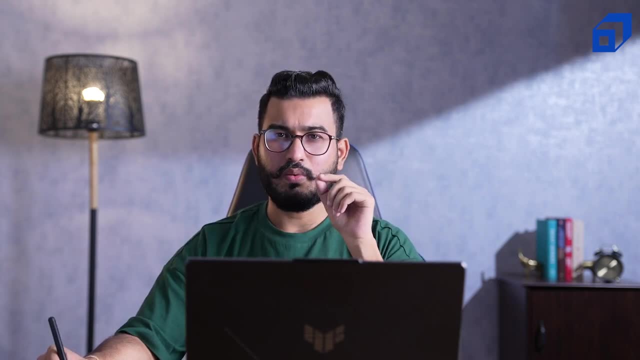 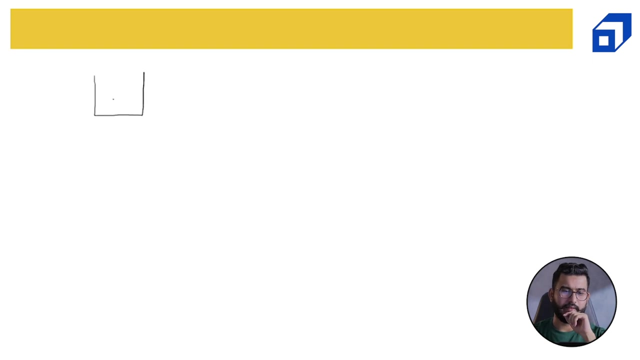 are dependent on each other. I hope this experiment, this example, make sense to all of you. Let's take one quick example to understand the dependent case in a better way. let's say: I'm again having a bag. this bag is having three black and I want all of you to 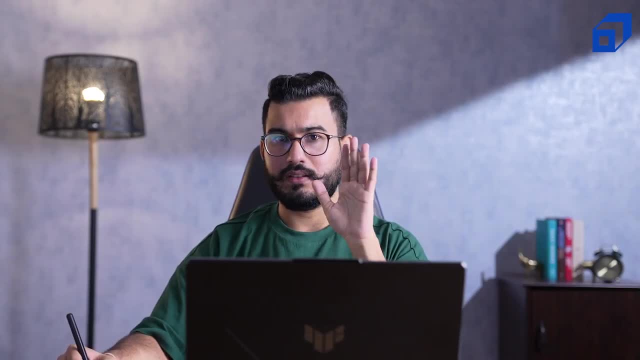 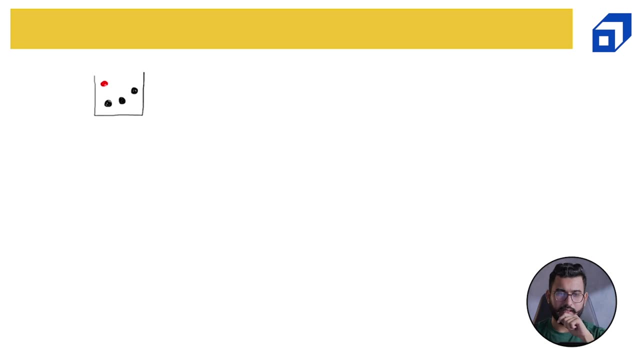 take out pen and paper and try to solve this. pause the video, try to understand the logic and solve it. so the question is: the bag is having three black and two red balls. what is the probability of getting red, red, which basically means probability of red in first draw and red in second draw? this 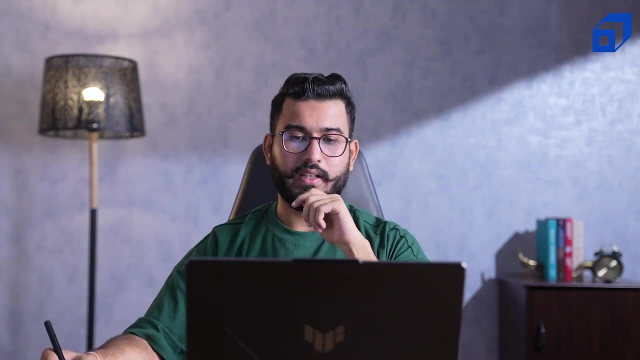 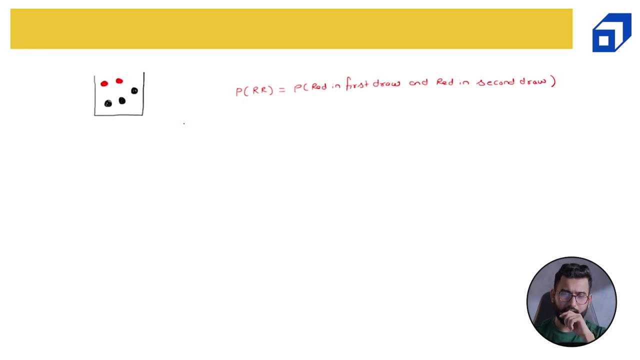 is my question. now let's try to logically solve it. I want all of you to pause the video and try to solve it by yourself. I hope you guys would have solved it already. so let's say, initially, the bag is having two reds and three black balls. three black balls. 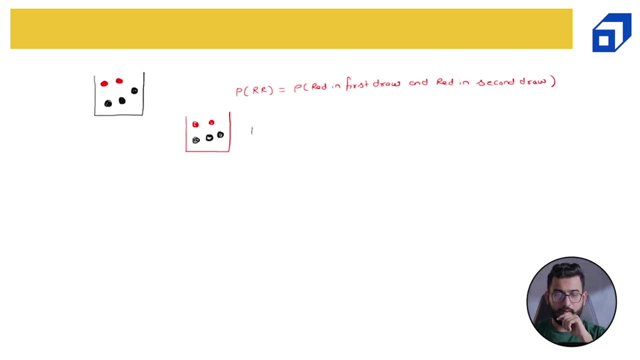 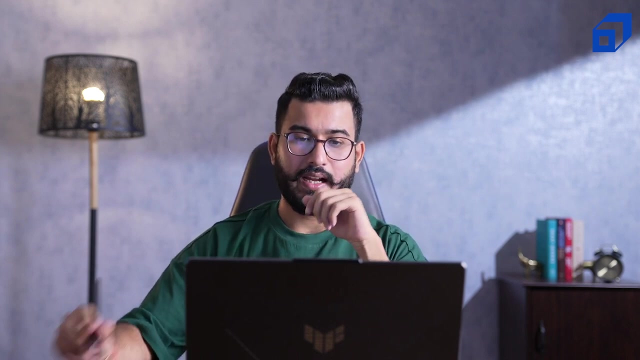 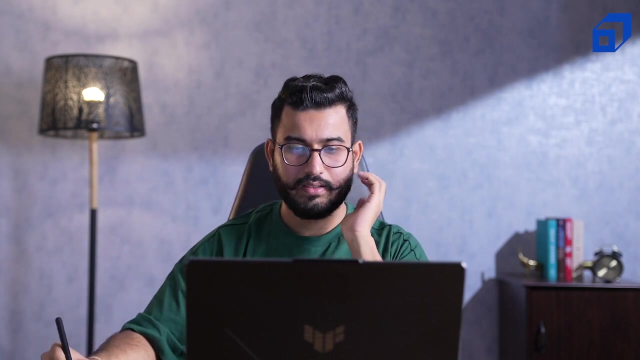 now, the probability of the first ball being red is 2 divided by 5. right now, this ball is out of the bag now, so I have taken out the ball and I have kept it outside, so the bag is now left with one red and three black. 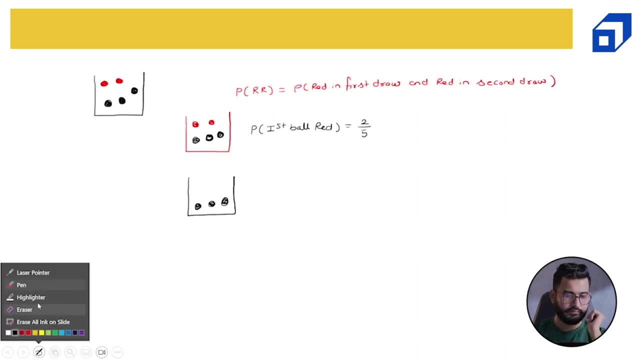 so one red and three black. now what is the probability of getting the second ball as red, given that I have already taken out the first ball as red? given that first ball taken out was red, Now this would come out to be 1 divided by 4, because I am left with. 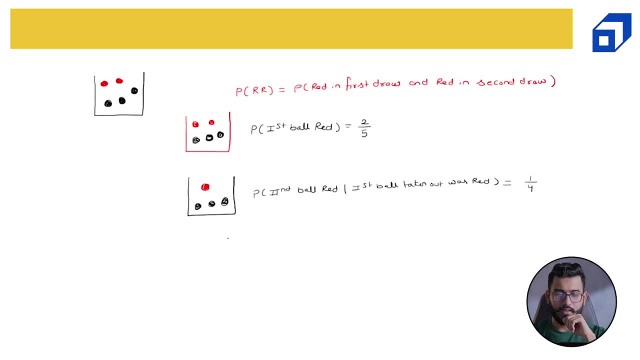 one red ball and total balls are left are 4.. So what is the probability of getting a red red, which basically means red in first trial and red in second? This will be probability of first ball as red multiplied by probability of second ball as red, given first ball. 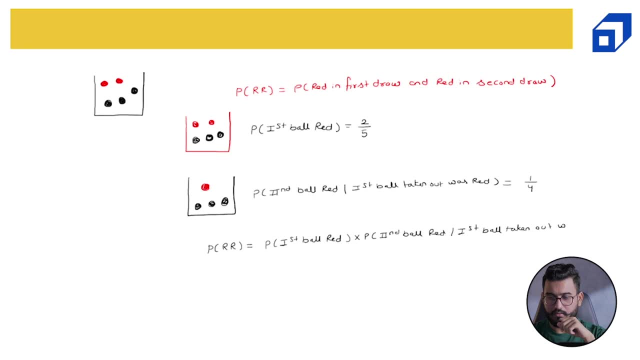 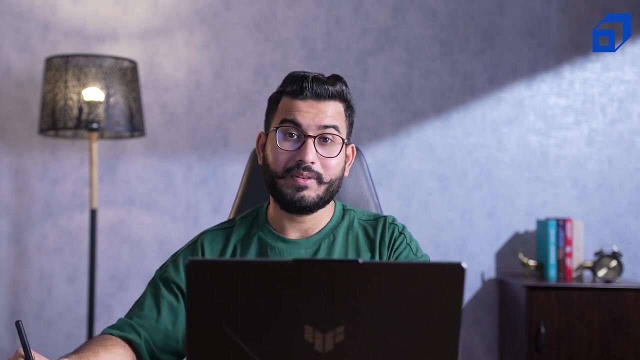 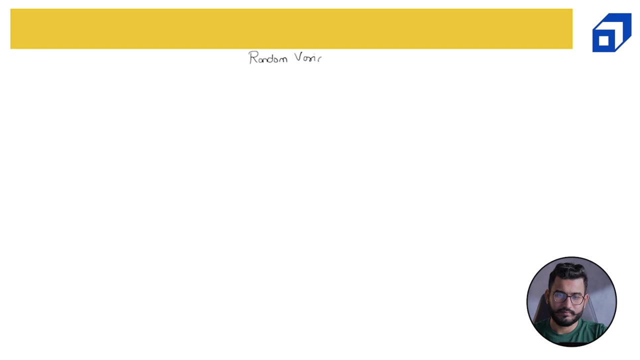 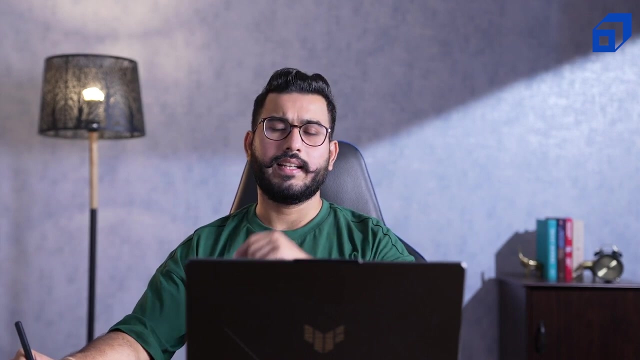 taken out was red. So this would be 2 divided by 5, multiplied by 1, divided by 4.. This is 1 divided by 10.. I hope you guys were able to solve this question. Now let's talk about random variables. Now, random variables is something that quantifies the outcome of an 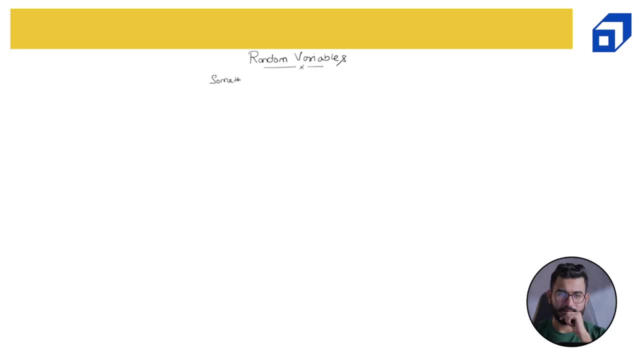 experiment, Something that quantifies, something that quantifies the outcome of an experiment. The outcome of an experiment. Now let's try to understand it in a better way. So let's say I am tossing two coins, So my experiment is toss of two coins. Now the sample space for this would be: 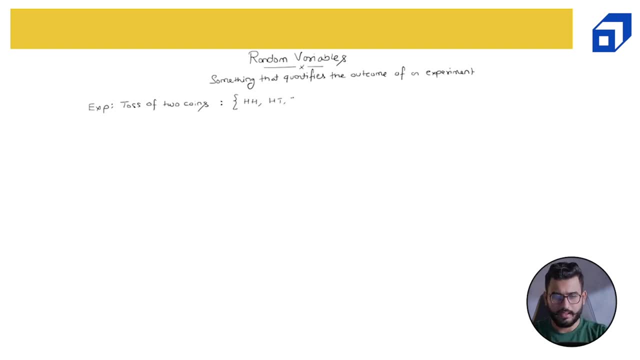 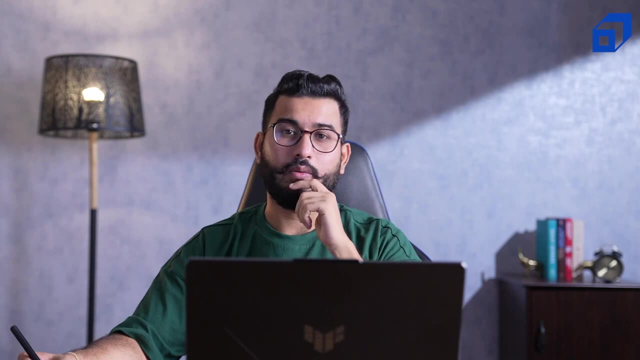 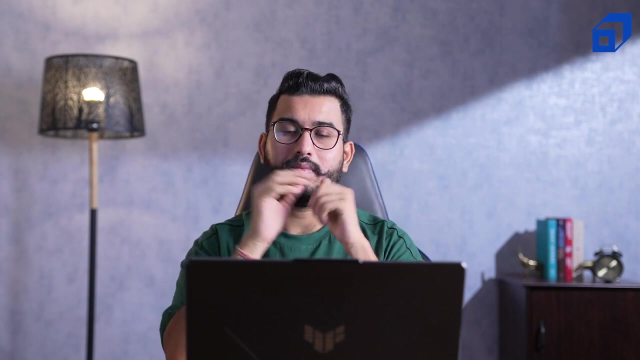 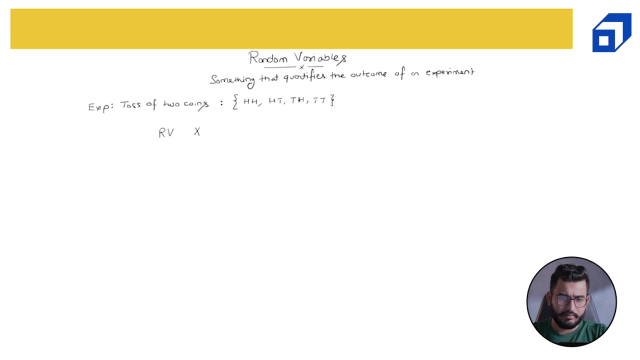 two heads: head, tail, tail, Head and tail tail. Now how I can quantify the outcome. What is the meaning of quantification? Converting the outcome into a number or mapping outcome into a number? So, let's say, my random variable can be. so are we assigning the variable with a sign or alphabet, x? So my x can be number. 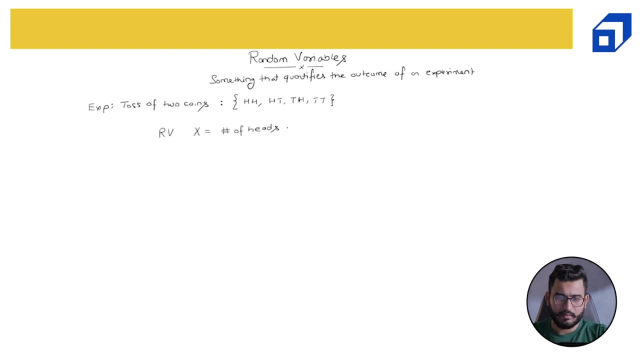 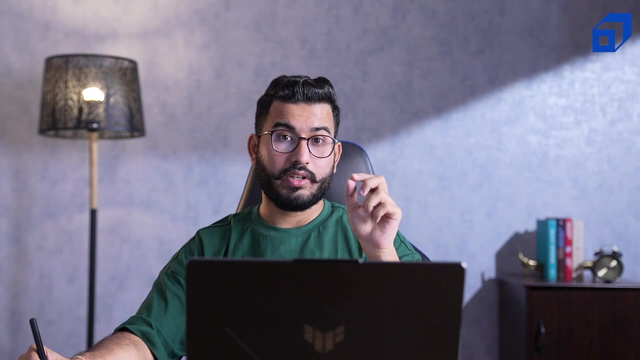 of heads in a toss of two coins. So my random variable can be number of heads in a toss of two coin in a toss of two coins. Now, this is my random variable and this will map the outcome of the random process, which was toss of two coins, into numbers. I will 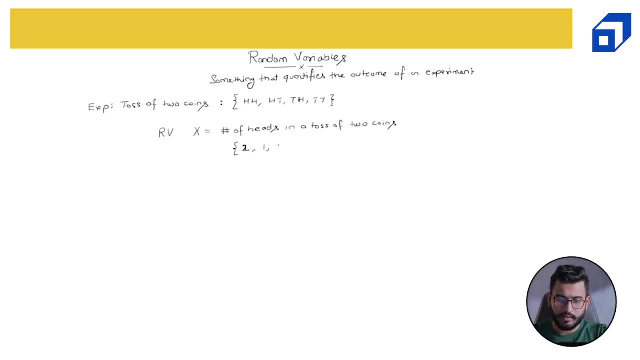 get 2, 1 and 0.. How So, if I write head head, head, tail, tail, head and tail tail, Now this corresponds to two heads. So the number of heads when you toss two coins can be two heads. This. 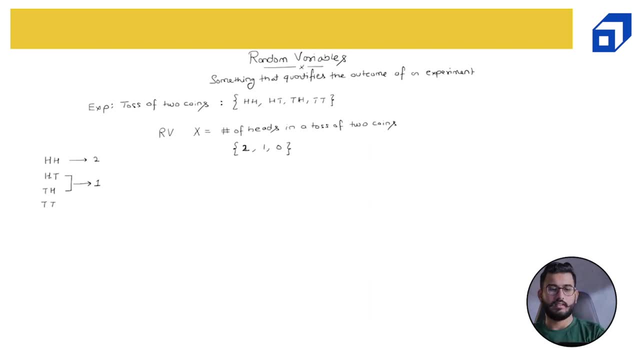 both quantifies to 1, because in both of these outcome I am getting one head and this is mapped to 0.. Because there is no head, So 2, 1, 0. This is my random variable x. Similarly, I can have a. 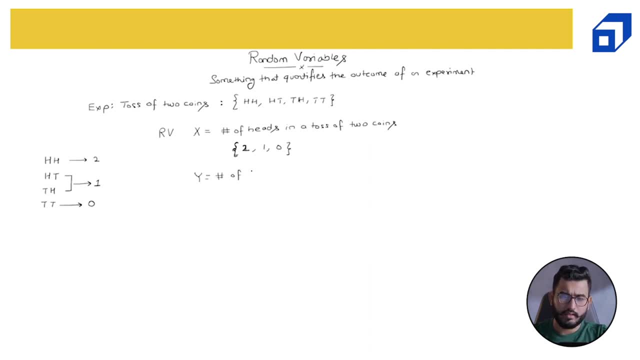 random variable y with number of tails in a toss of two coins. In a toss of two coins. So let's say y will also represent 2, 1, 0.. I can have two tails, one tail or zero tail. I can also have a random variable y with number of tails in a toss of two coins. So let's say y will also represent 2, 1, 0. So the more heads, the more settings. so 2, 1, 0, 1, 1, 1, 1, 2, 1 keep. 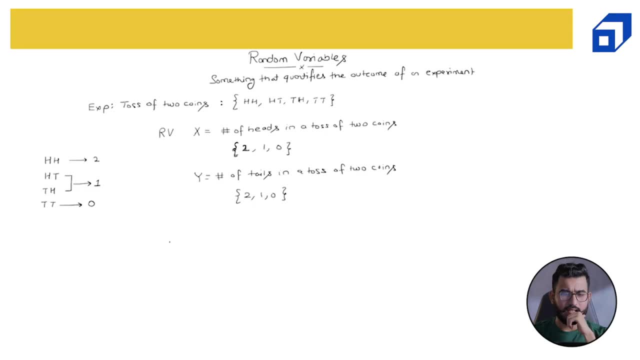 in process. So this is my random variable, where I have taken a random number. For example. let's say, I would state that if you get so, there is a game. let's say there is a game which says: if you get two heads, I will give you 10 rupees, So you win 10 rupees. 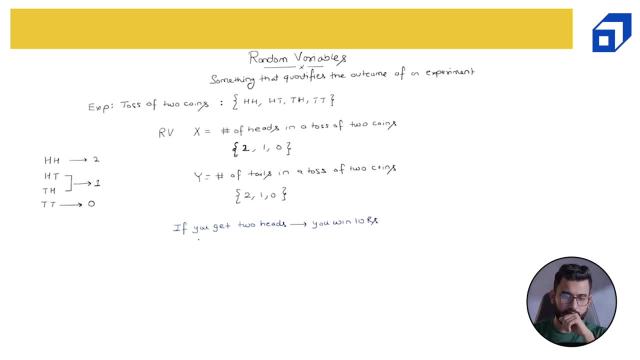 you win 10 rupees, Then I can have another right. if I use it the other way, I give an outcome. So for any other outcome, much better than 1, 2, 1,, 1, 0. I'm sure. much better than 2, 1, 1. in that case, you should choose the right outcome. So I have now. so this is my random variable, where I, where I have taken a random number, For example, let's say I have stated: 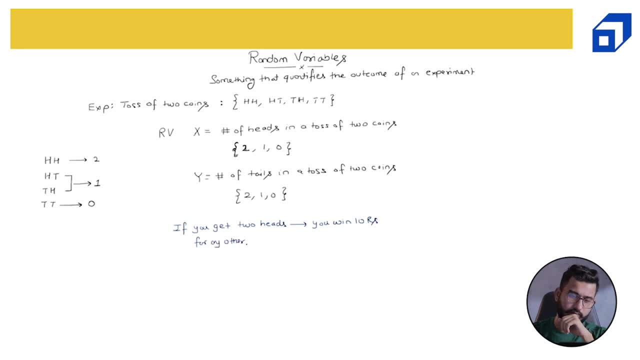 for any other outcome. you have to give me. you have to give me 5 rupees, So you pay 5 rupees. Now, in this case, let us say, I am interested in the amount I can win, So 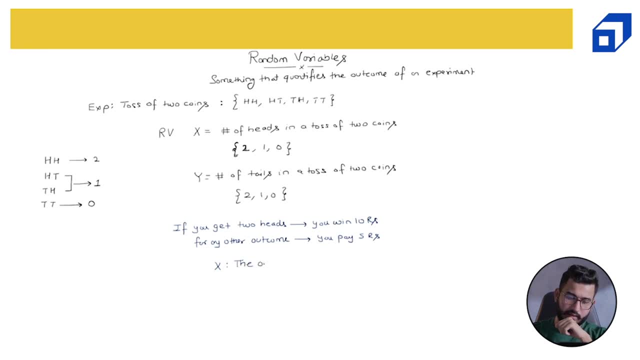 x is my random variable. x represents the amount or the total price, So the amount I can win, and it can either be 10 rupees. so I will write plus 10 because it is a gain for me. so plus 10 and minus 5 because minus 5 represents loss. So here what I. 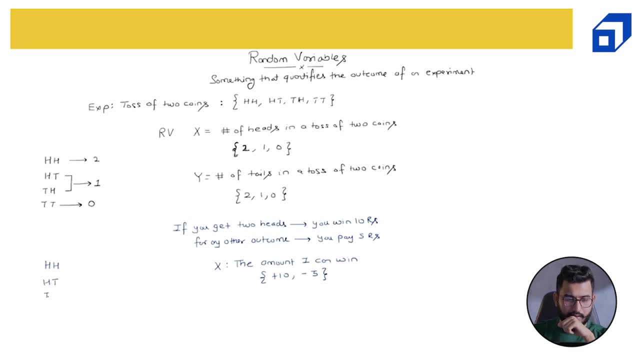 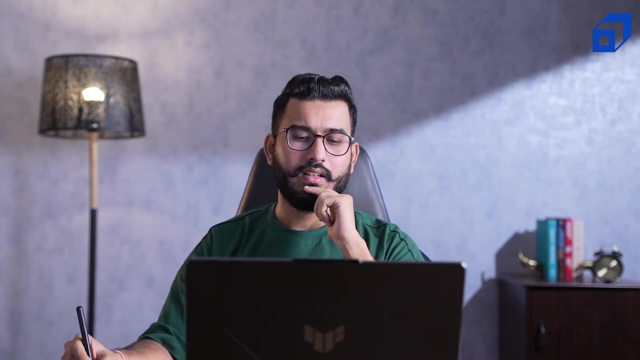 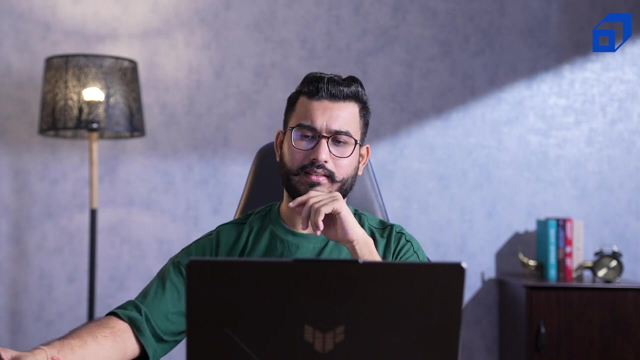 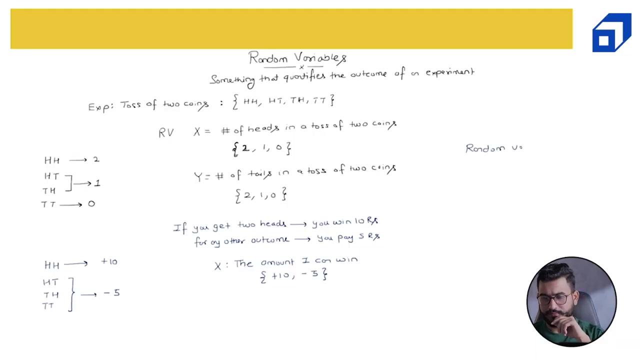 have done. if my experiment is having these four outcomes, then this is mapped to plus 10 and all of them are mapped to minus 5.. This is also a valid random variable. Now, random variables are essentially divided into two categories. A random variable can either be a random variable can. 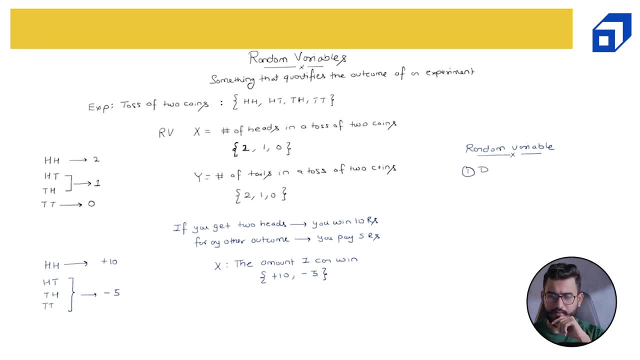 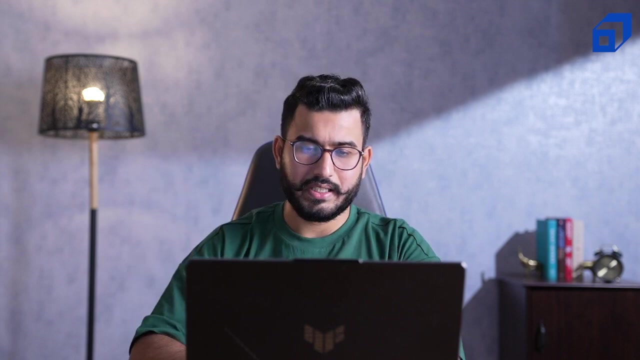 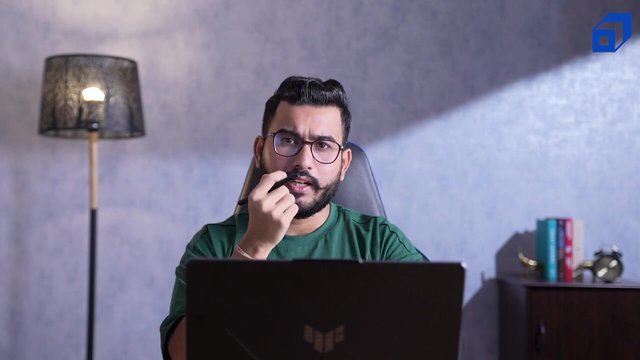 either be discrete or it can either be continuous. Now, what is discrete random variable, or what are the discrete random variables? Well, discrete random variables are those variables for which the outcome can be quantified into integers which are countable. For example, number of heads in a 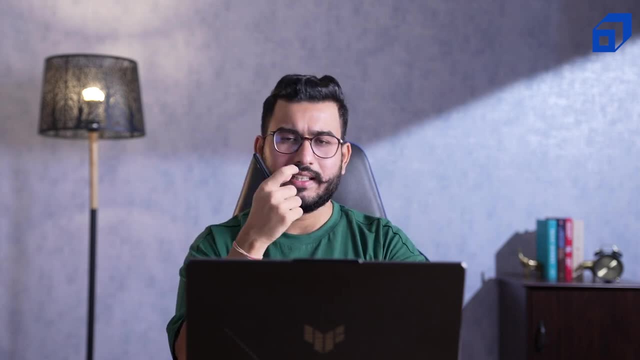 toss of two coins. I know it can be either zero, it can be either one, it can be either two, but if I ask you about you completing watching this video, so how much time you will complete take to watch this video? Now, it can be anything from minus infinity to plus infinity you can take. 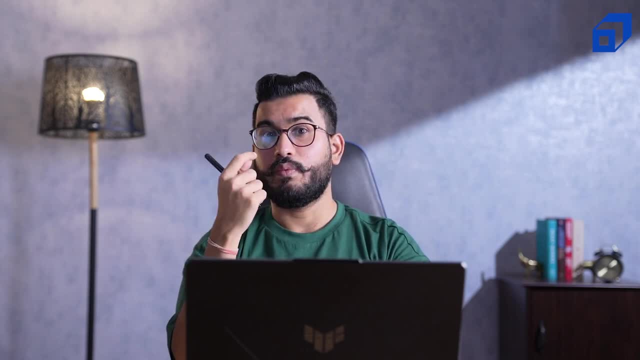 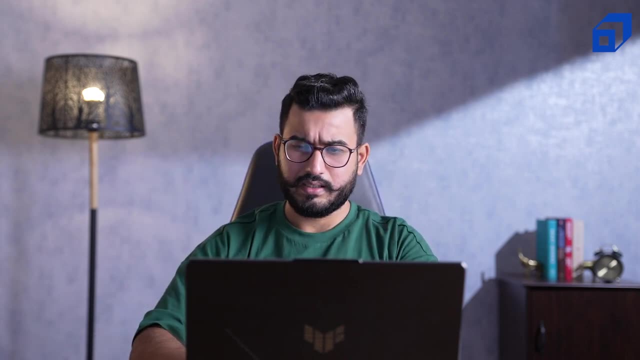 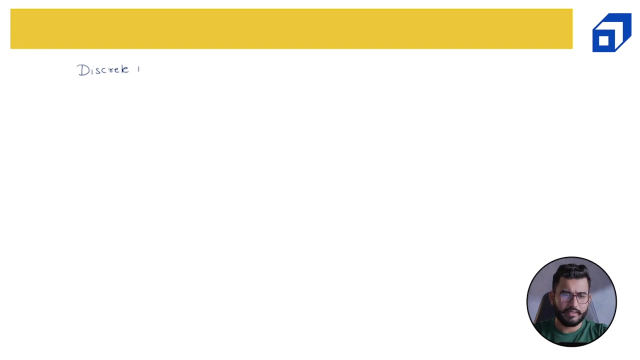 one hour. you can take one hour five minutes. you can take one hour five minutes 50 seconds. there are endless possibilities. right, Let's take a simple example. let me just go to a next page for discrete. first of all, we'll take example for discrete: random variable: the outcome. 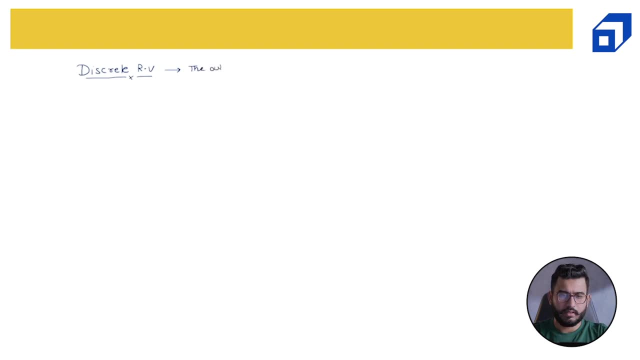 the outcome is the outcome are mapped to integer numbers which are countable. you can simply count them. for example, number of heads in a toss of two coins. or let's take one more example. let's say there is a person who is trying to shoot a particular. 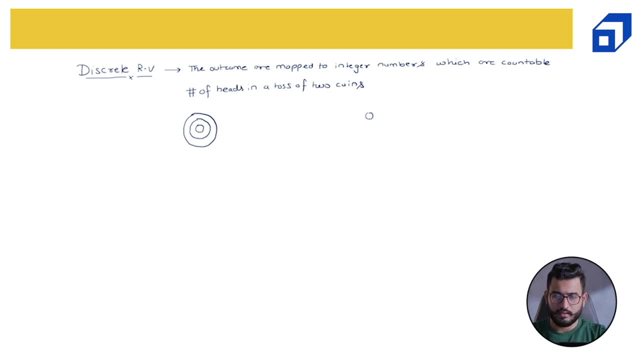 target. so this my target. here I'm having the person and this person is trying to shoot the target. so here is the target. now let's say this person is trying for 10 times. so the person try to shoot the target for 10 times. then what can be my random? 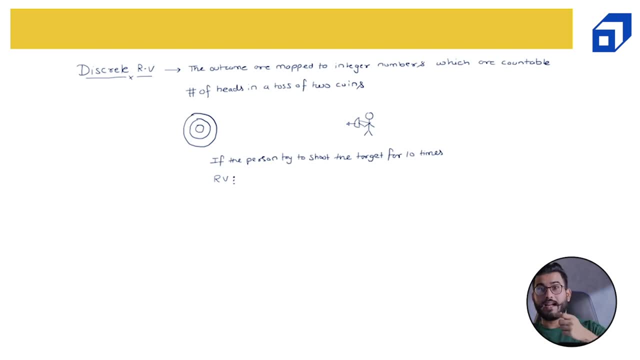 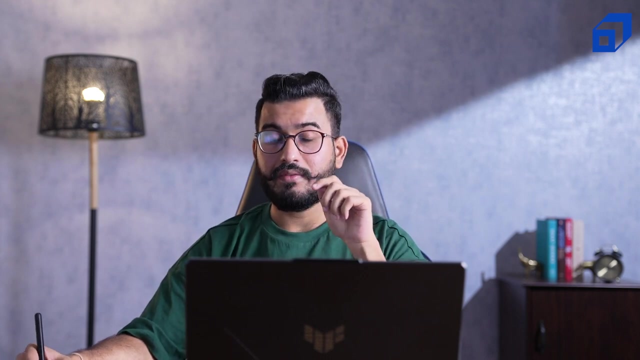 variable. my random variable can be the number of times the person hits the bull's eye. so my random variable, x, can be number of times the person hits the bulls eye. now, if you closely observe, this can be a. this can only take. this random variable can only take integer numbers. so I can only only 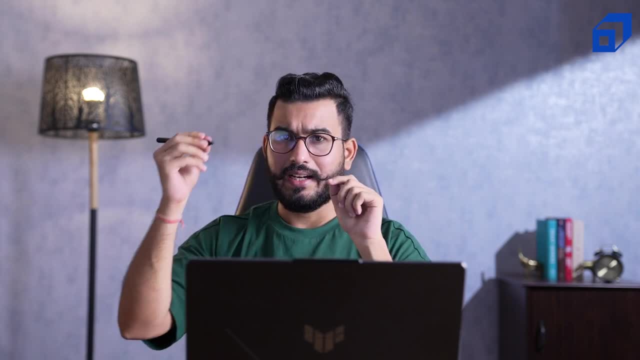 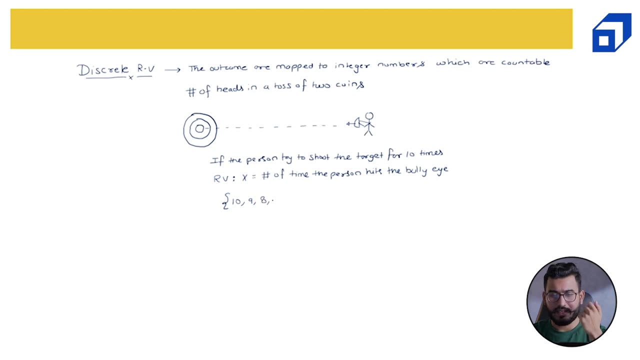 get the number of times the target of the a bull, but the random variable can. So the person can either hit the target or hit the bullseye for all the 10 times, maybe for 9 times, for 8 times, for 7,, 6,, 5,, 4, 3, 2, 1 or 0. 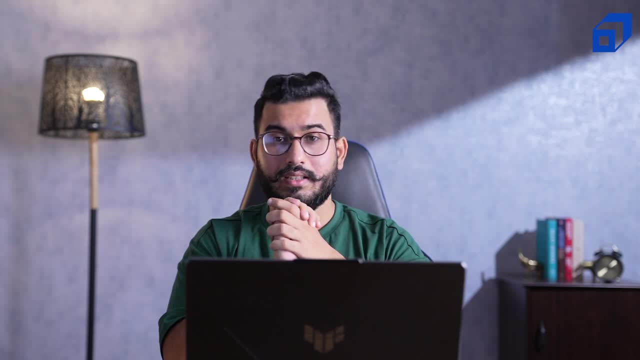 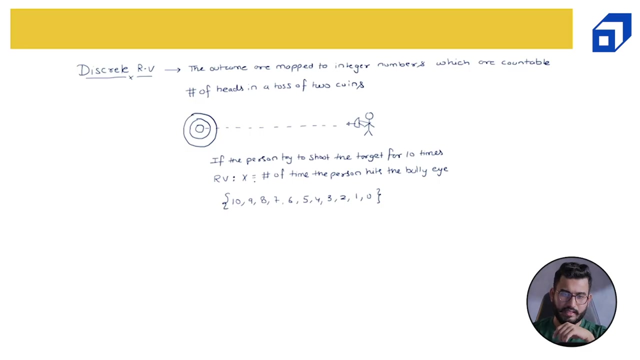 0 means the person was not able to hit the target for any time. This is my discrete random variable. Can this variable take any value other than all these possibilities that I have written? Can the random variable x that you can see on your screen, can this variable take 1.7?? 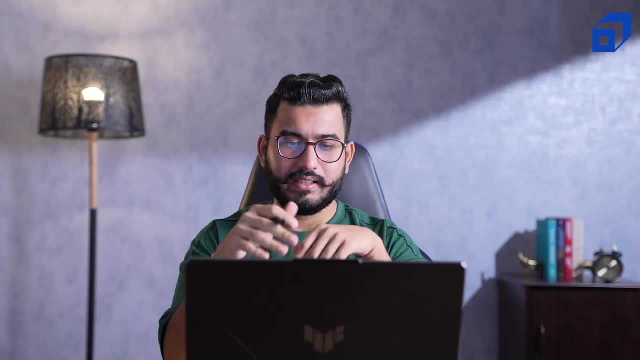 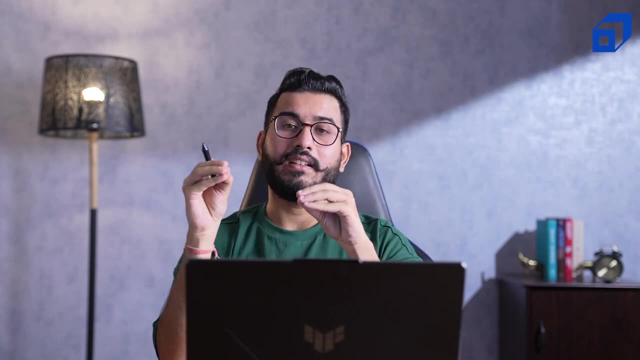 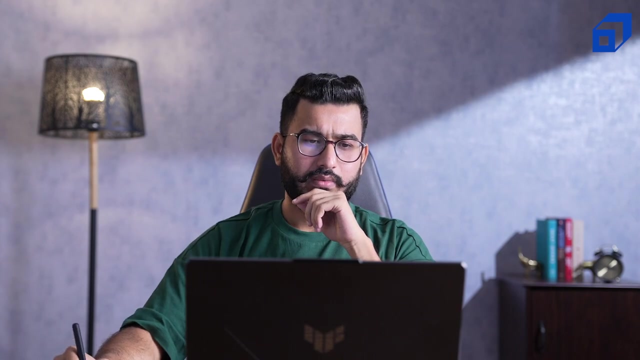 No, it cannot take 1.7.. Similarly, this random variable cannot take 10.5 or maybe 9.11.. So it can only take these limited numbers. So this is why this is known as a discrete random variable. Let's talk about continuous random variable. 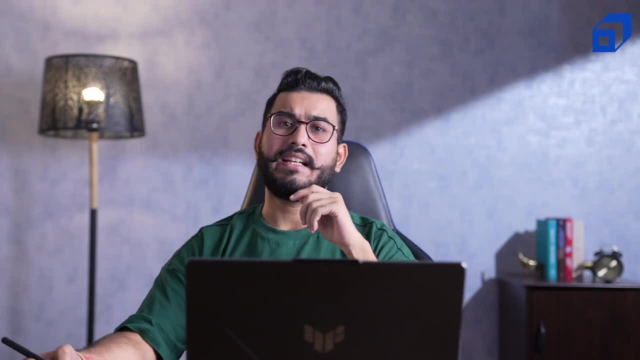 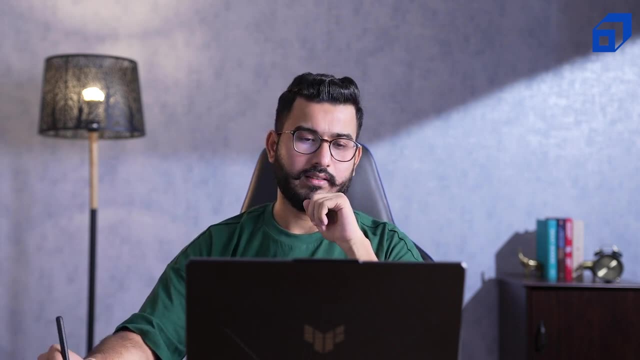 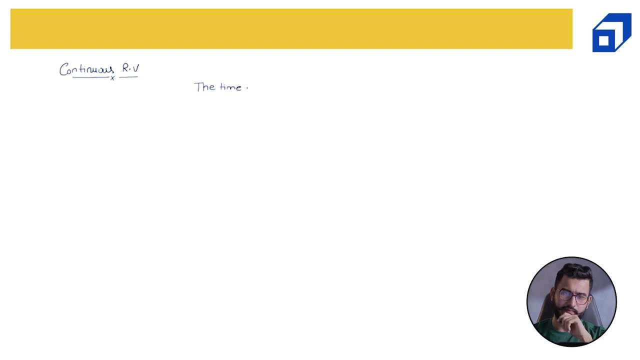 Now, continuous random variable can take many values. The outcome are many possibilities. So, for example- let's take first of all an example- The time. the time an employee Takes to commute from home to office. Now, this is my random variable x: the time an employee takes to commute from home to office. 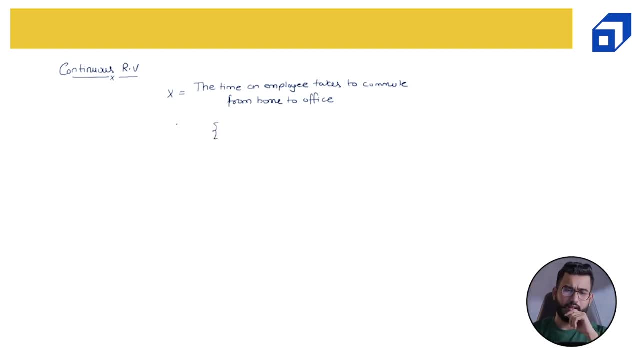 Now this can be anything. let's say we have defined a range. minimum is the person Minimum takes 10 minutes. Maximum is, let's say, one hour. or let's say we will keep the scale in minutes itself. So we have written 10 minutes. 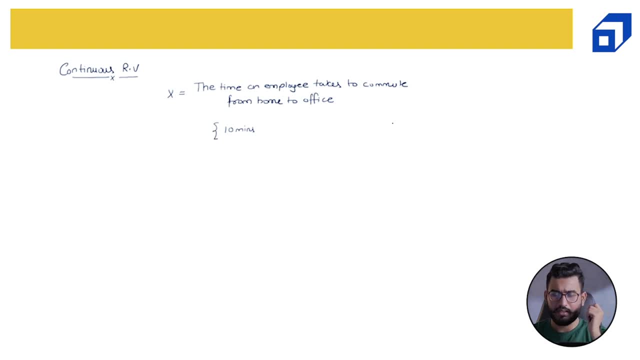 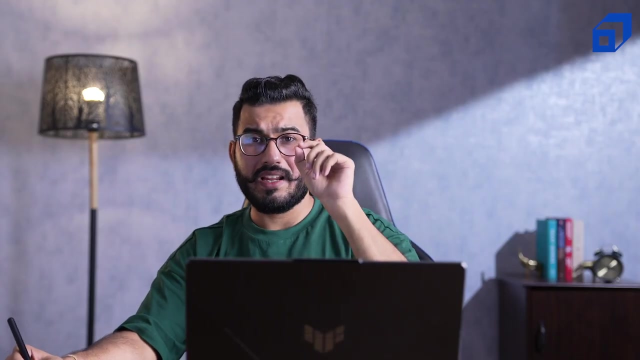 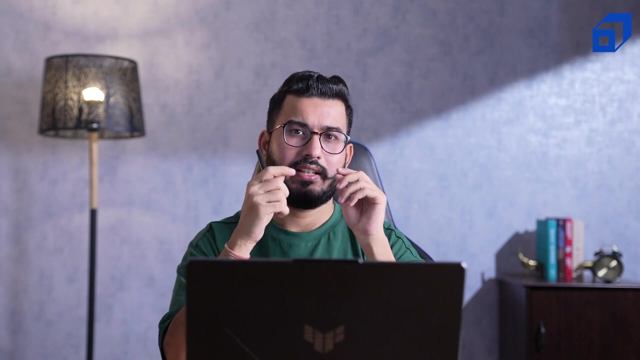 So this is 10 minutes and the maximum is 60 minutes. Now, between these two minimum and maximum, between this range, I can have endless numbers, endless right. There can not be a particular point That I can pinpoint. I can not say the person would take 10 minutes, 5 seconds, or 3 milliseconds, 2 nanoseconds. 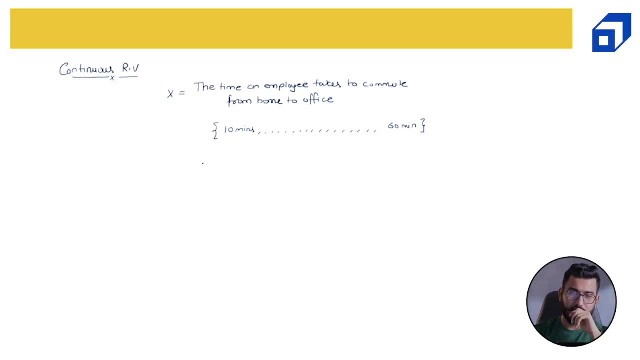 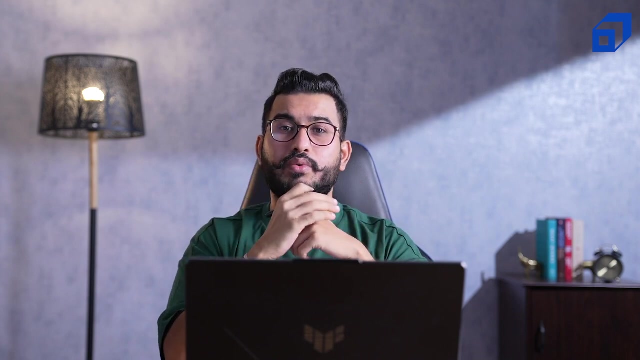 It can be endless possibilities, right? So this kind of random variable is known as the continuous random variable. So here x represents my continuous random variable. When I talk about discrete random variables, there are some properties and distributions associated with it. There are some properties and distributions associated with it. 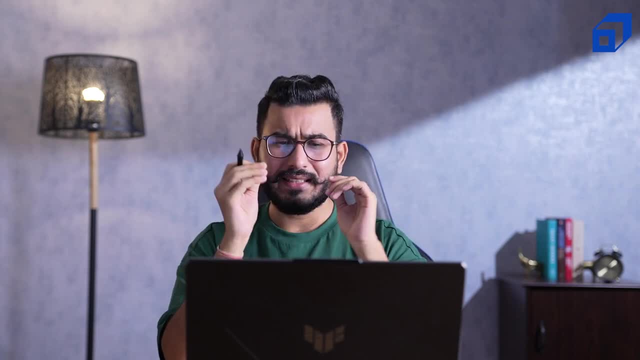 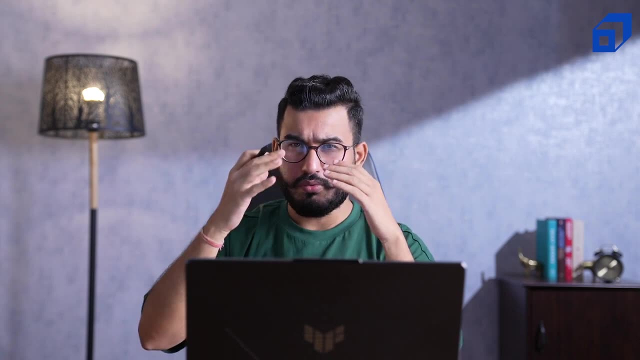 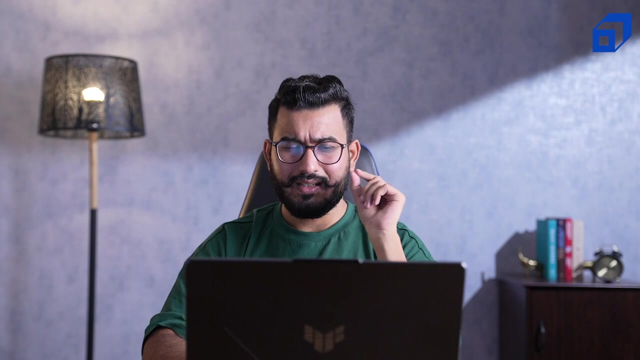 Similarly for continuous random variables. the reason we are talking about it is because we wanted to generalize them. I will talk more about them. I will talk more about how we can generate a distribution out of them, But before that, let's briefly talk about a very important topic known as expected value. 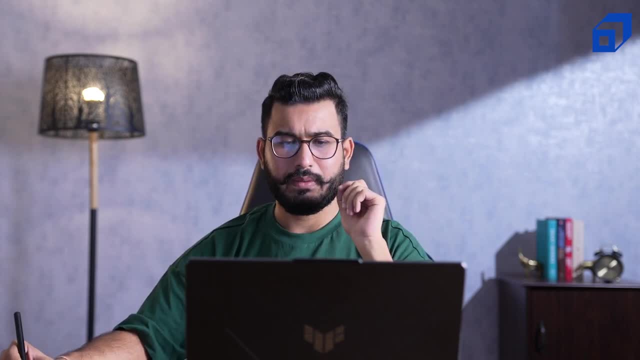 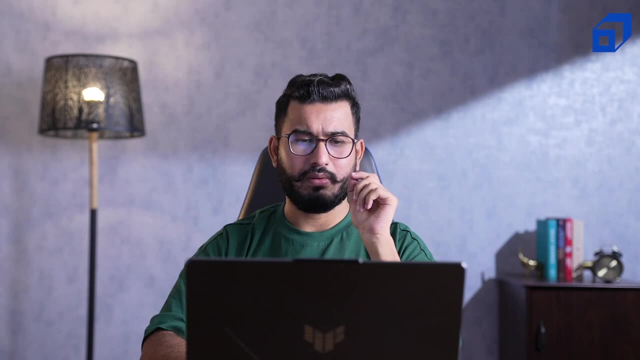 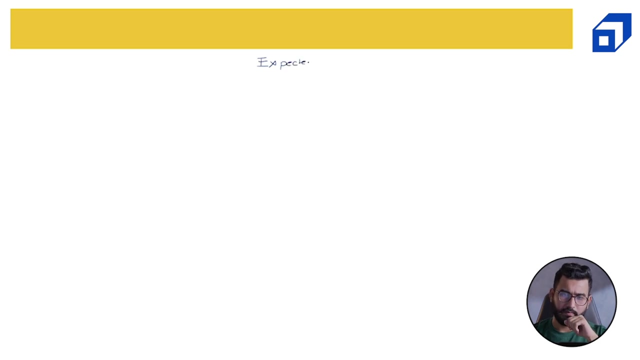 And we will take this example for to calculate the expected value. What is the expected value? So I'm just taking a topic out of the random variable to talk briefly about expected value And then we will jump to distributions. So expected values: 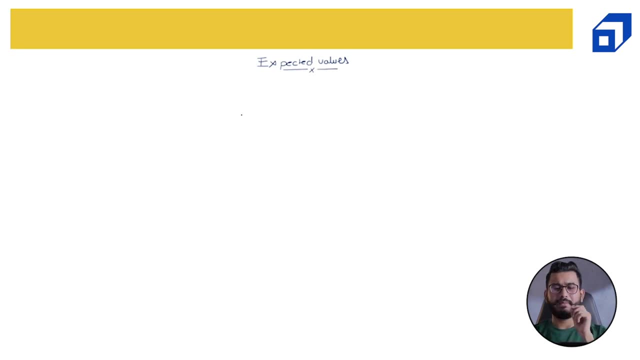 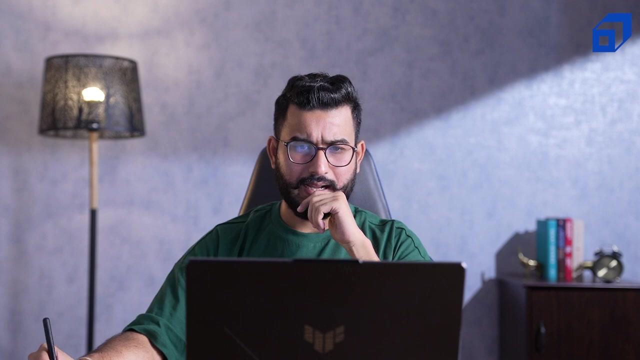 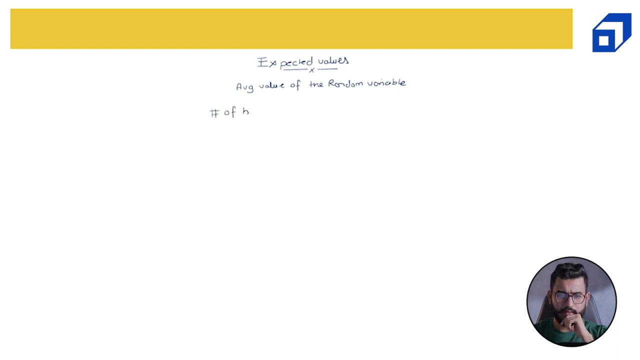 Now, when we talk about expected values, it is basically the average value of the random variable. Average value of the random variable. Now let's say- I'm taking one example- Let's say the number of heads, The number of heads in a toss of two coins. 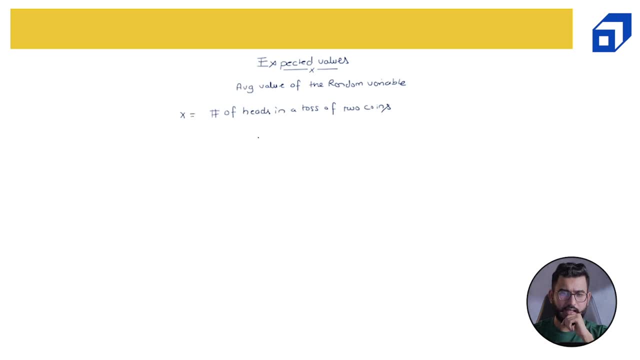 Now this is my random variable x, And this random variable can take 2, 1 and 0. So either I can get two heads, one head, or zero head. Right, I have already shown you this. Please remember this. Now, what is the expected value of this random variable x? 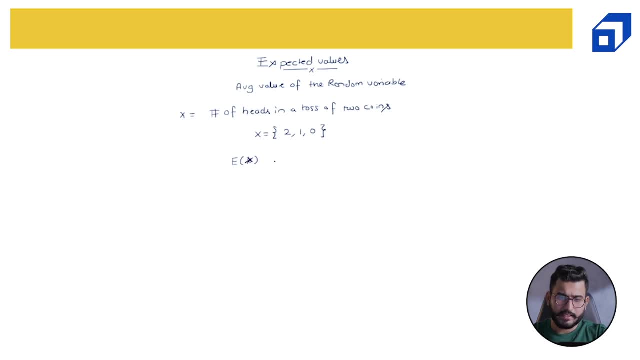 So what is the expected value of x? Expected value is nothing but given as summation of i over x, pi into xi. I would write it formally as xi into pi, And then the probability of x is equal to xi. What is the meaning of this? 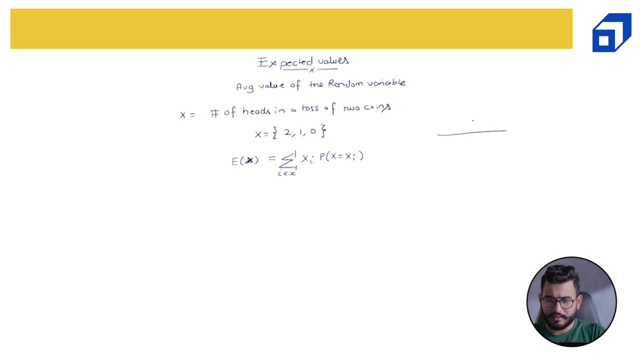 So what is the probability? So let me just quickly create a table with the random variable x and the probability of x. So random variable x. Probability of x is equal to xi. So the random variable can take value 2, 1 and 0. 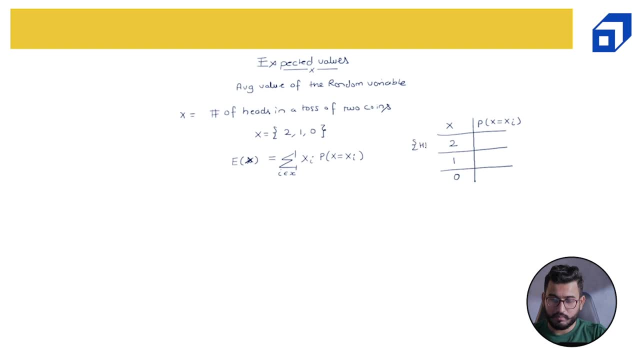 Now 2 can come out from this event: head head, 1 is the event of head, tail, Tail and tail head, And 0 is the event of tail tail. So the probability of getting 2 is 1 divided by 4.. 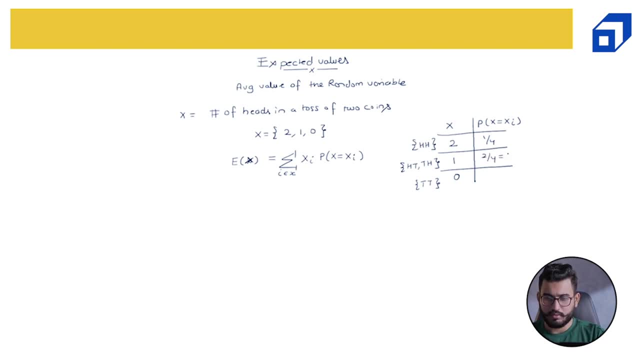 This is 2 divided by 4.. Which is eventually 1 divided by 2.. And this is 1 divided by 4.. These are the probabilities. So the expected value of x is nothing but the random variable multiplied by the probability of that random variable. 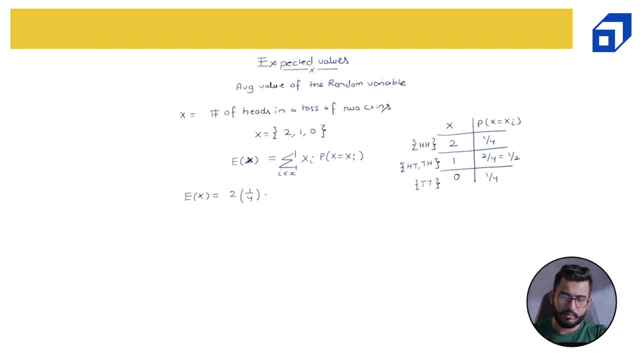 So 2 multiplied by 1 divided by 4 plus 1 multiplied by 1 divided by 2 plus 0 multiplied by 1 divided by 4.. So this will be 2 times. So I will get 1 divided by 2 plus 1 divided by 2.. 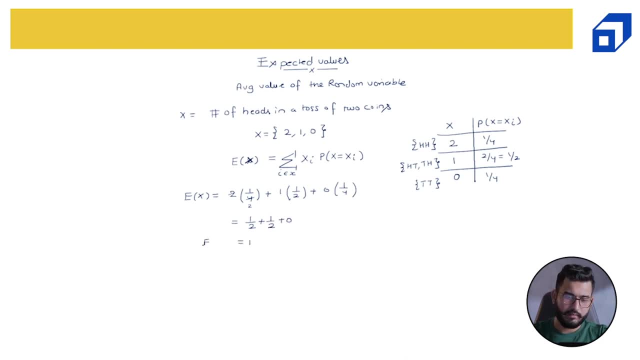 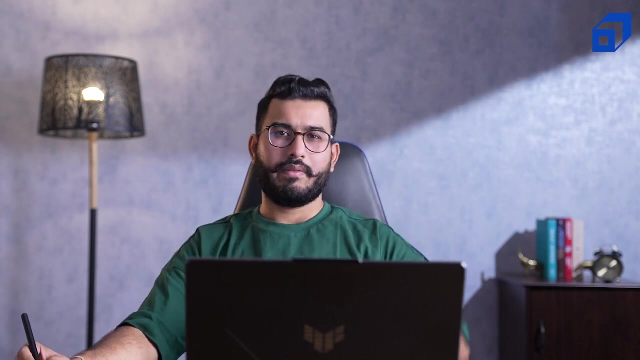 And this will be 0.. So the answer is 1.. Expected value is 1.. What is the meaning of this? This means On a long run, If I perform this experiment for a very long time, If I keep on performing this experiment. 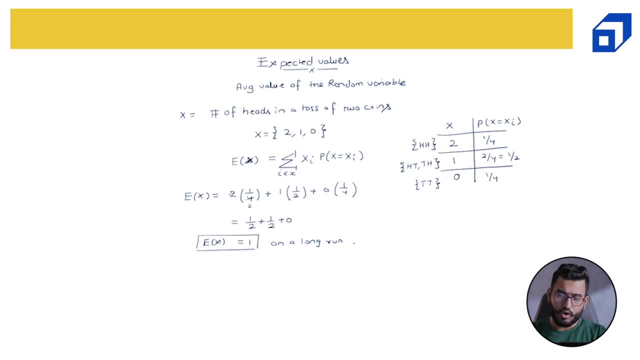 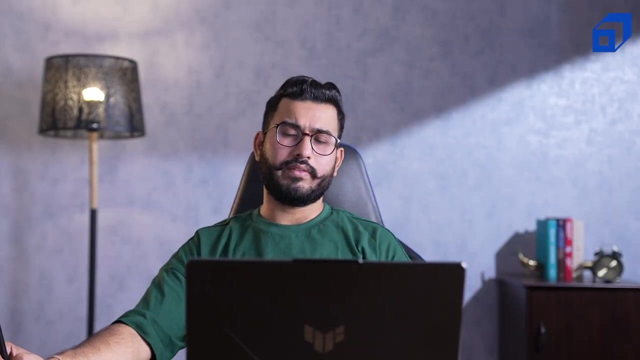 I am tossing 2 coins again and again On a long run. On an average, This experiment, This experiment would result In 1 head. So on a long run, you will observe that You are getting 1 head. This is the mean of this random variable. 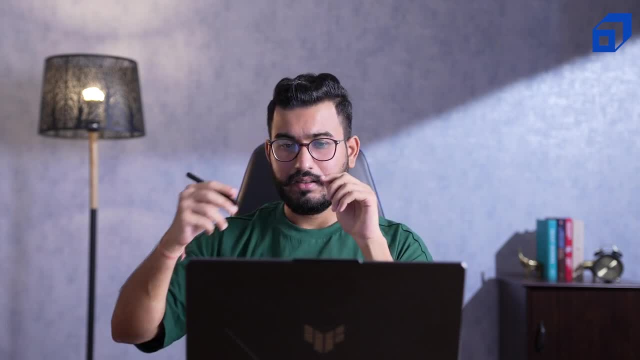 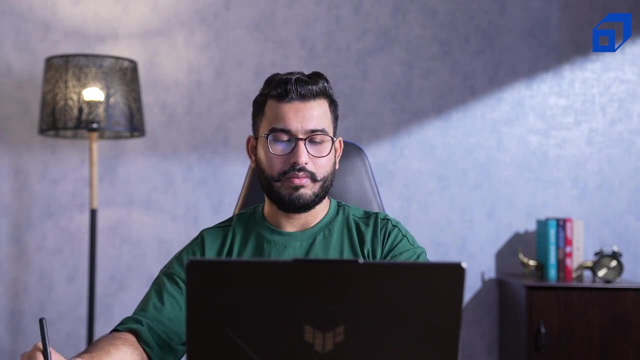 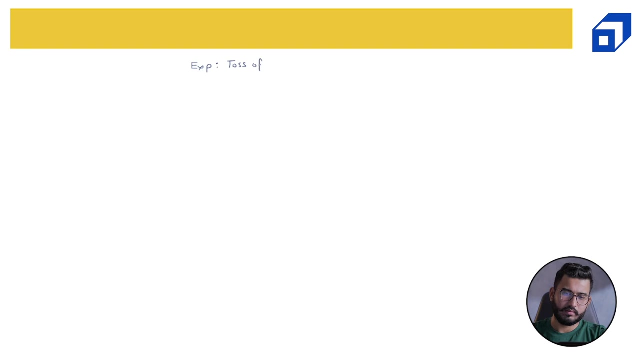 If this is not making sense, Let's take an example in a game format, And then you will be able to connect with it. Let's say: Now I am having the same experiment. The experiment is Toss of 2 coins. 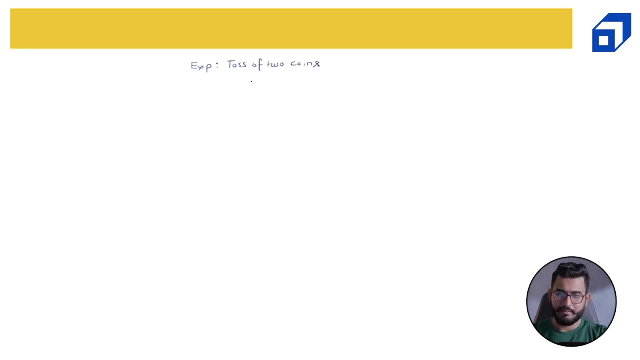 Toss of 2 coins. I may either get Head head, Head tail, Tail head And tail tail. Now We are mapping, So my random variable x is now The amount I can win. The amount I can win. 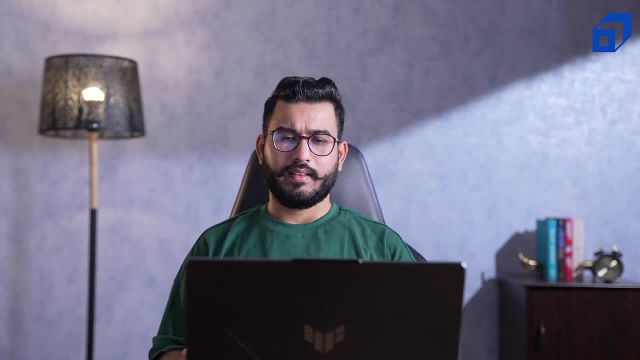 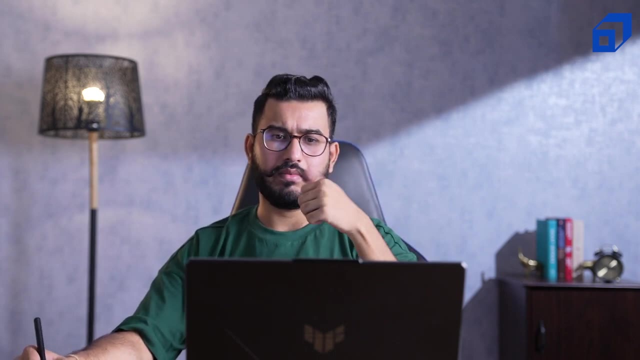 Let's say 2 people are playing Some game And the condition of this game is: If the person tossing 2 coins, Or if the person tossing a coin for 2 times Gets both of them are head, The person wins 10 rupee. 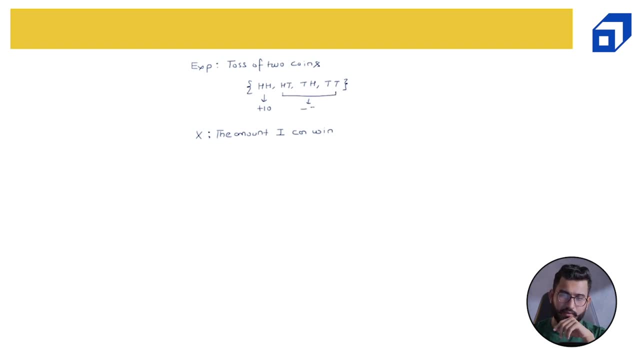 For any other combination The person has to pay 5 rupees. So the random variable x is Plus 10 or minus 5.. Now I will quickly create a table. This is my random variable xi. This is probability of X is equal to xi. 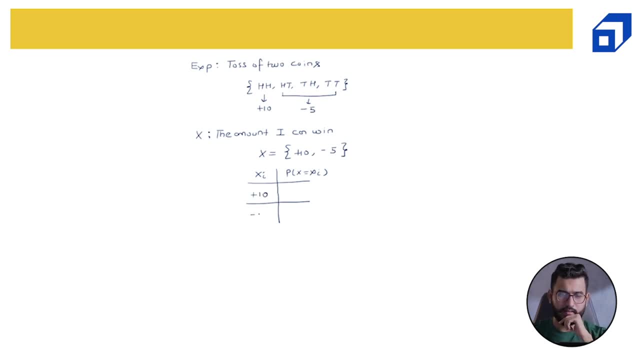 So person can win 10 rupees, So plus 10.. Person can lose 5 rupees, So minus 5.. What is the probability of Winning 10 rupees? You can see The probability of winning 10 rupees. 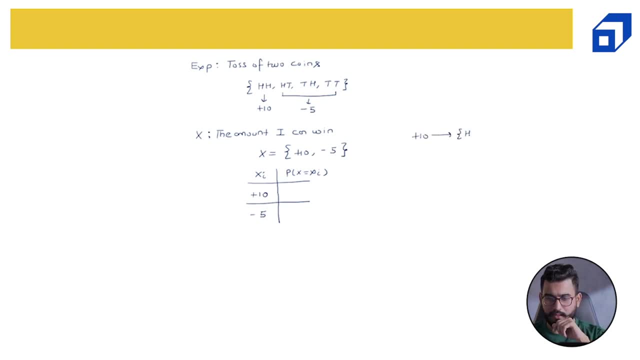 Plus 10. Can only come When the person has obtained both head, Which is 1 divided by 4. Right Probability of losing 5 rupees Is Getting either of the Either of the event, Which is head, tail, tail. head and tail tail. 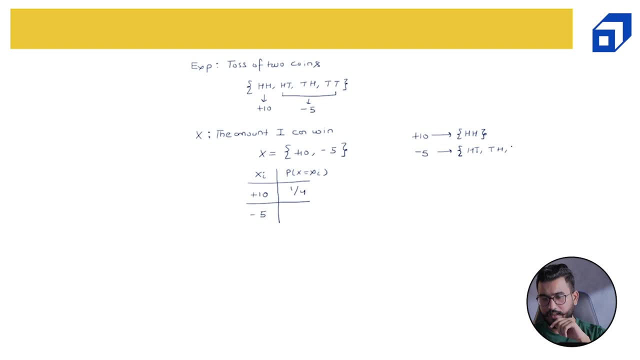 So head, tail, Tail, head and tail tail, And this is 3 divided by 4.. Now I will calculate the expected value of x, Which is 10.. 1 divided by 4.. Plus Minus 5.. 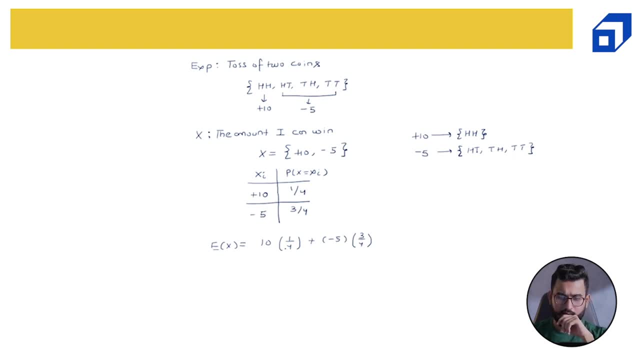 Into 3 divided by 4.. Now this will be 2 times 2.. 2 times 5.. This will be 5 divided by 2.. Minus 15 divided by 4.. Or For easy calculation: 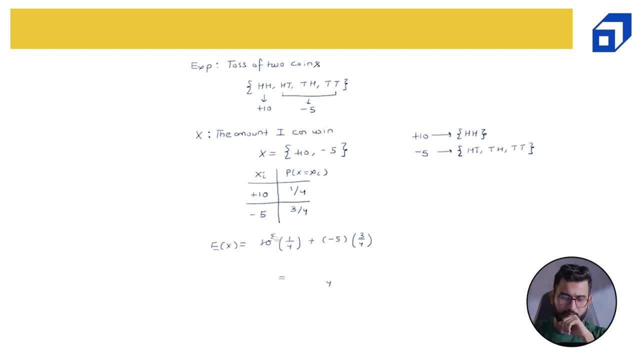 Let's Keep them, Let's Let's not cancel out The 4. Because the numerator is Denominator- is both 4.. So I will get 10 divided by 4.. Minus 15 divided by 4.. 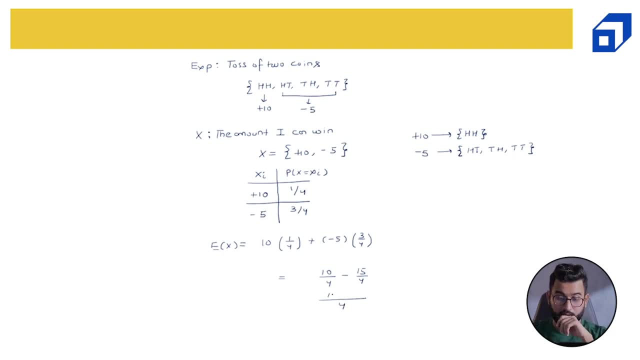 This would be 4. Denominator. Denominator is 4.. 10 minus 15 is Minus 5 by 4.. So Minus 5 divided by 4. Which is Minus? 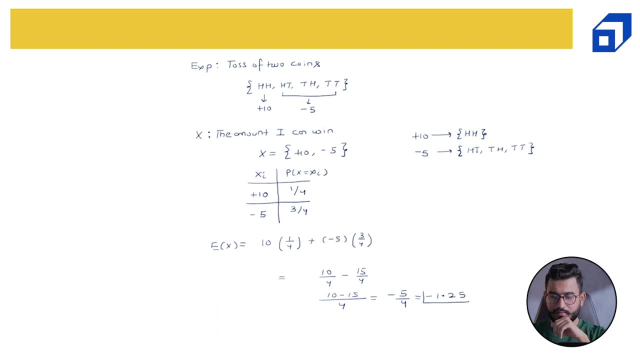 1.25.. Now what is the meaning of this value? This value basically mean On a long run. If you play this game for very long time with your friend On a long run, On an average, You would End up. 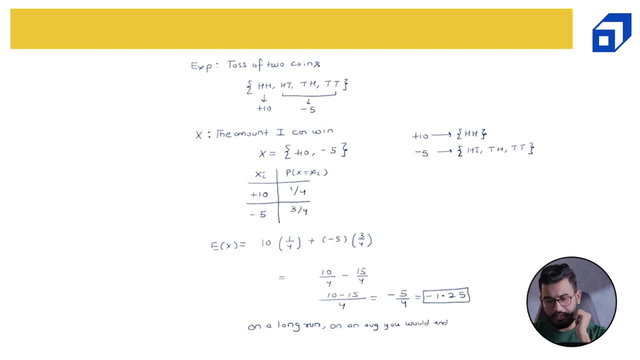 Losing 1.25. Rupees Per Game. So this is Our Loss For you. What was my random variable? The amount I can win? The random variable ends up in a negative value, Which is Minus. 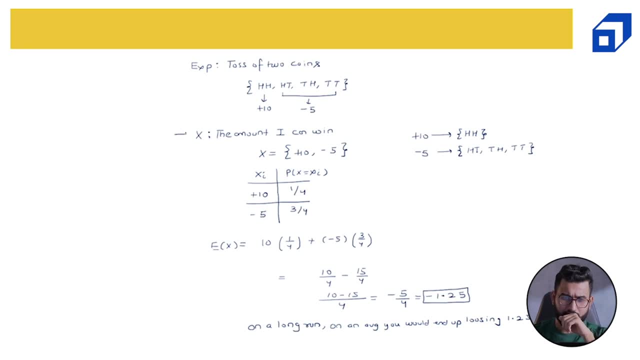 1.25.. So on a long run, If you Perform This experiment, You will Lose 1.25. Rupees Per Game. So This: If you perform this experiment for a very long time. 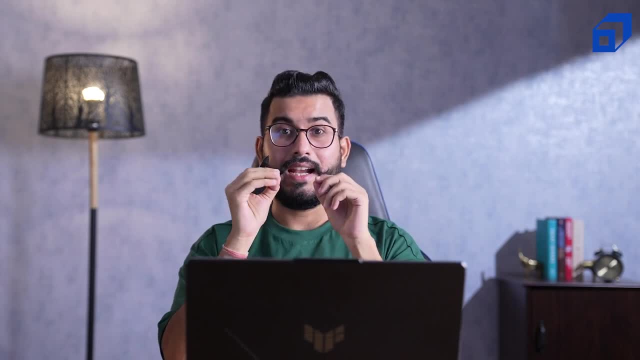 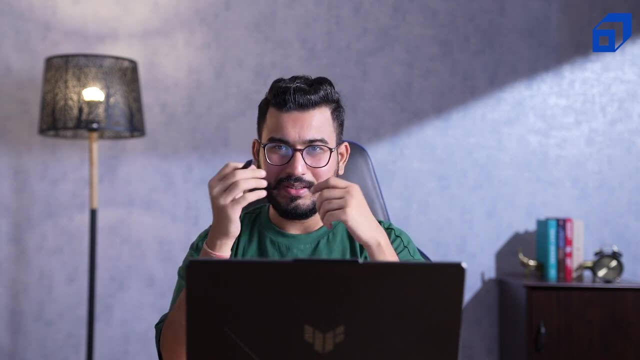 And you play this game with your friend, Then you will End up losing 1.25. Rupees Per Game, And that is what You should do. So when you are Playing a game, Please make sure. 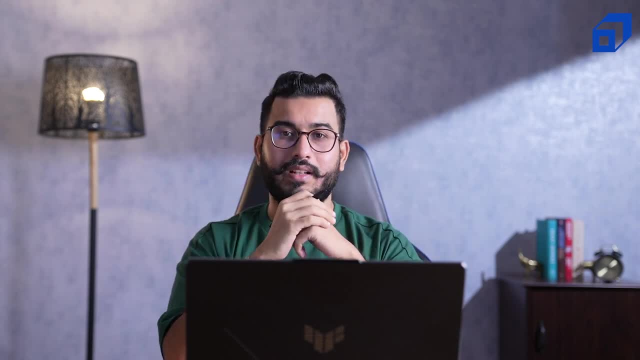 The expected value should always turn out positive for you And You. You would have Heard about this term: The house always wins. The house always wins, Which basically mean In Gambling, Whenever you go to Any casino Or any gambling house. 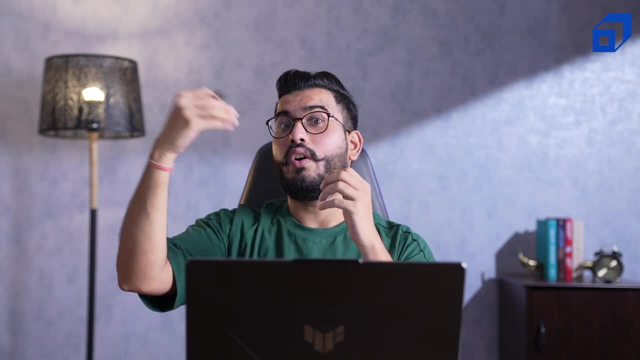 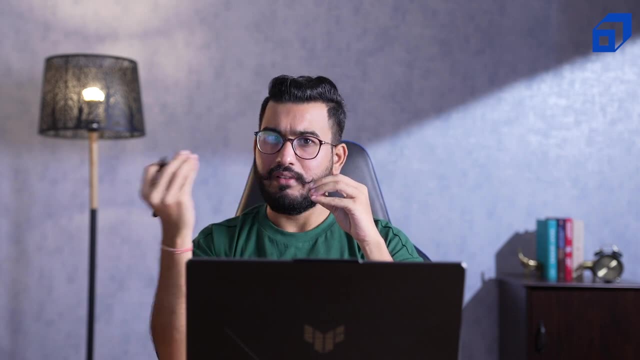 They always win On the long run. So If So many people Are playing the same game, Some are, Some of them Will win, While Most of them Will lose. So on a long run It is a profit. 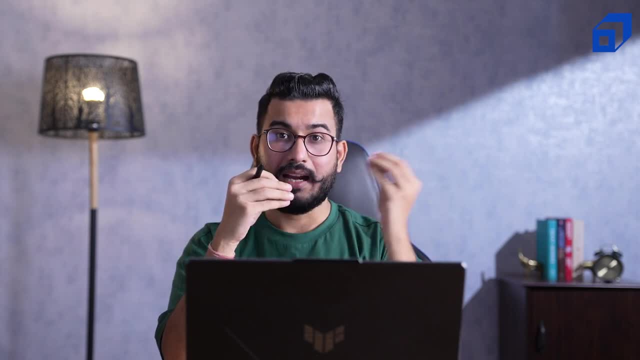 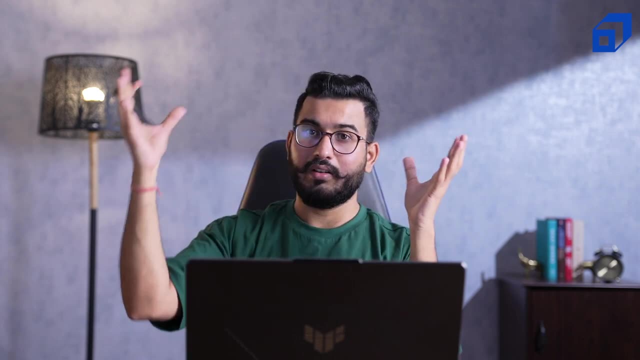 For the, For the gambling house Or for the casino. So Some of them May win, Some of them May lose, But on a long run, When Many people Are playing The game In the casino, The house, 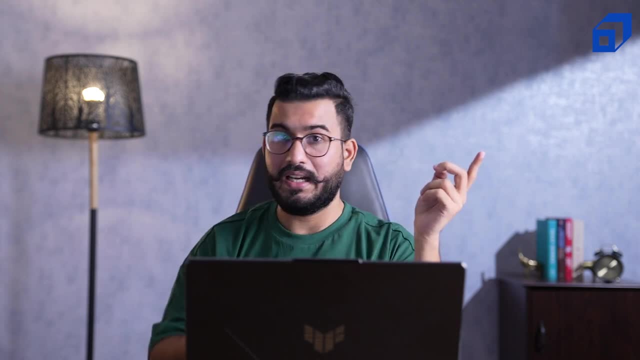 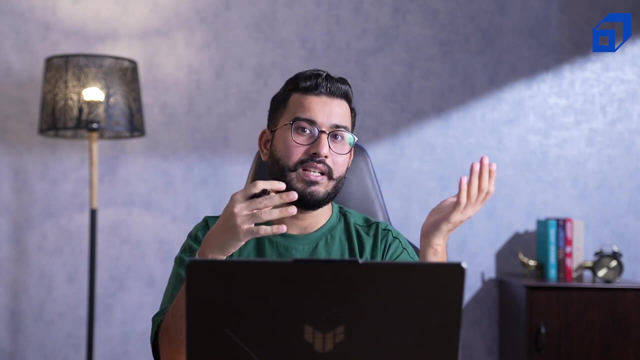 Will always win Because Their expected value Is positive For them And negative For you, And all The games Are Made In such a way That the expected value Is favorable To them. So Now, 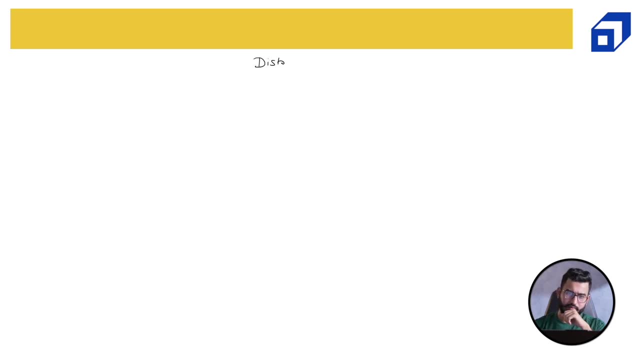 Let's Talk About Distributions. What Is Distribution? So, When We Have A Random Variable, I Hope You Already Know A Random Variable Can Be Of. 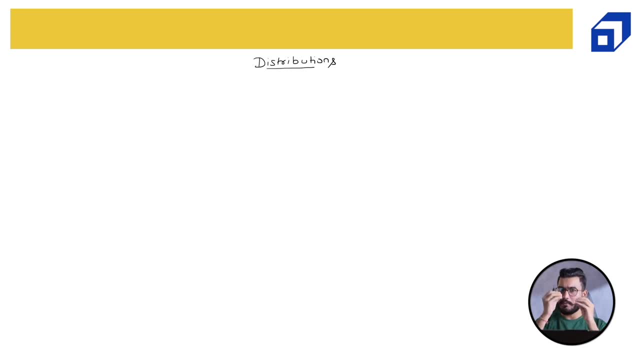 Two Types, Either Discrete Or Continuous. So Let's Say, I'm Having A Discrete Random Variable. So When We Talk About Discrete Random Variable, 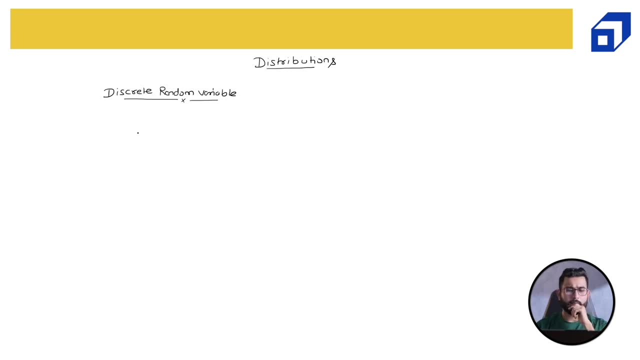 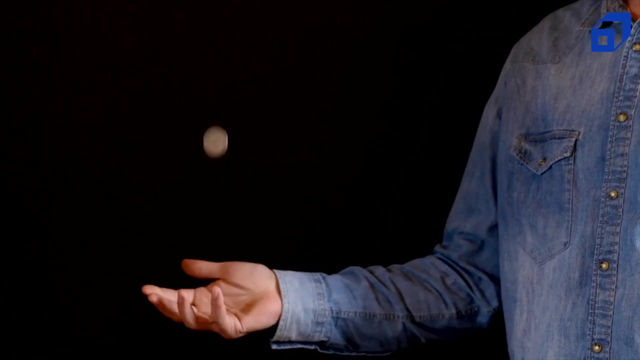 We Know That The Outcome Can Be Discrete. It Can Be Integer, Right. So Let's Take One Example: Two Coins, And I've Taken This. 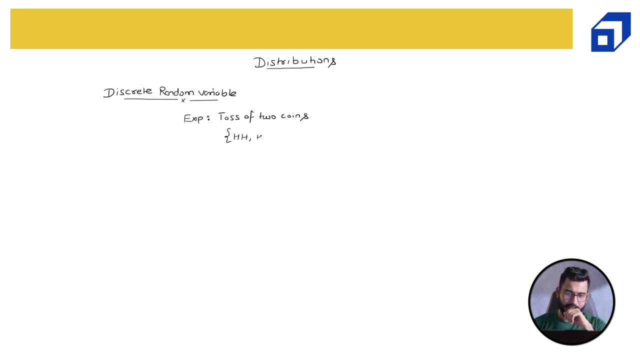 Experiment For So Many Times, So You Already Know That The Outcome Can Be: Head Head, Tail Tail Head And Tail Tail Right. The Outcome If 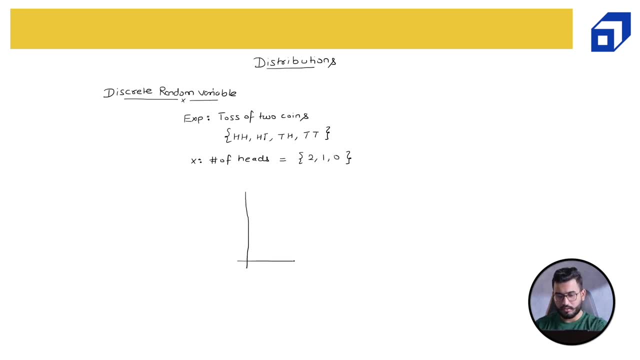 I Plot This Distribution. So I'm Having A Plot In The X Axis, I'm Having The Random Variable And I Already Know This Random Variable. 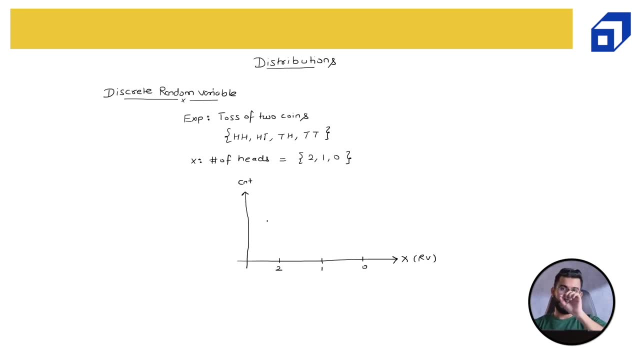 Can Either All Time Or What Really Is The Opportunity To Live Forever. So We Have To Live Alone Now, You Will Know, Not For Time. 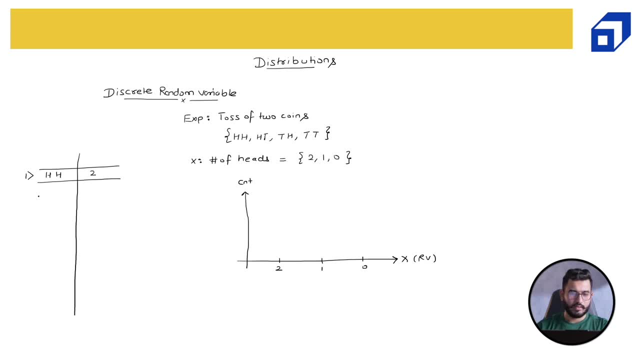 To Live In Your Home. you obtained head, tail, so 1.. In trial number 3 you obtained tail, head, so again 1.. In trial number 4 you obtained tail, tail, so again 0.. In trial number 5 you obtained tail, head, so 1.. In trial number 6: 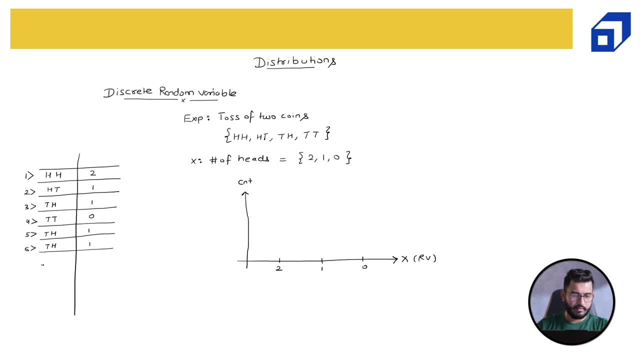 you obtained tail head, so again 1.. In trial number 7 you obtained head, tail, so 1.. In trial number 8, you obtained head, head, so 2.. In trial number 9, you obtained tail, tail, so 0.. In trial number 10, you obtained tail head, so again 1.. Now this is my 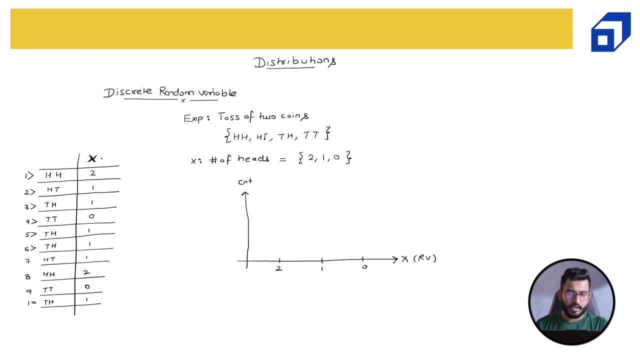 outcome or random variable X. Now I will just count and create a variable X. Now I will just count and create a plot. so how many times I have obtained two heads? so one time, two time. so I'll assume that this is one, this is two, this is three, and so on. so for two times I 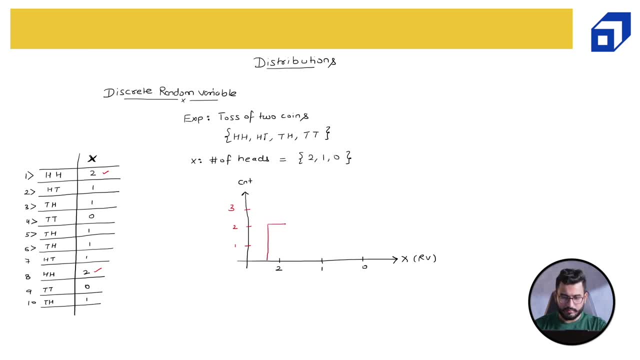 obtained head head, so I'll create a bar over here. then how many times I obtained one head, so one time, two time, three time, four time, five times, six time, so six time, let's say it represents like this: and then how many times I obtained no head, so one zero and zero, so two times. 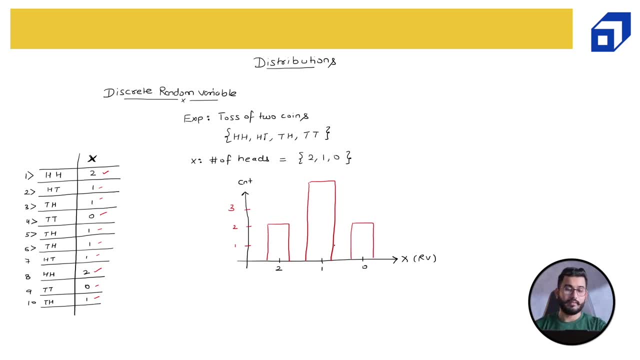 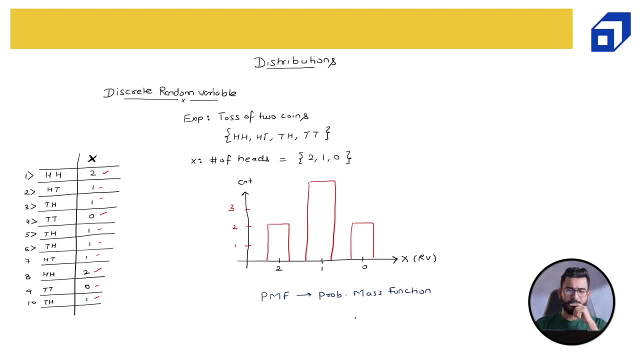 known as the probability mass function. This is known as the probability mass function. Now, please remember this: that if I'm tossing one coin, so let's say, if I'm just tossing one coin and we have already created this probability mass function. I hope you remember. I have shown you one website seeing theory dot edu. In that. 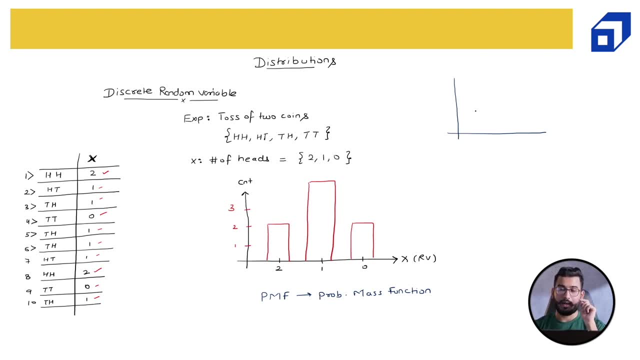 website. you have seen that for the true probability. so the true probability of getting head and tail when you toss one coin is half and half, one divided by two and one divided by two. so the probability of mass function of the true probability when you toss one coin will be 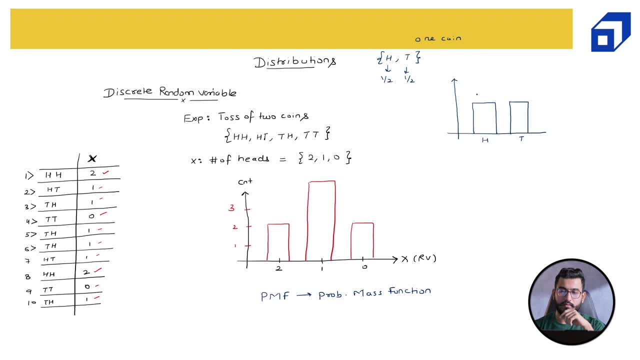 0.5, 0.5. so this is head, this is tail: 0.5, 0.5. but you, when you actually perform the experiment, this can change, this can be anything. this can be. let's say, I'm having more head and less tail, so let's. 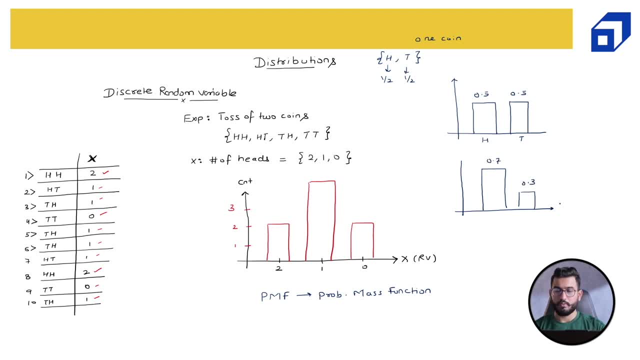 say: this is 0.7, this is 0.3 when you tossed one coin for 10 times. so seven times you obtain head, three times you obtain tail. quite possible, right? this is known as the observed. this is known as the observed. so this is known as the observed. so this is known as the observed. 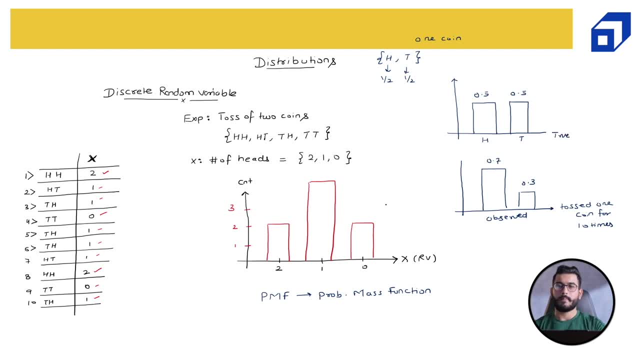 known as observed. This is known as true. Similarly, for this example: the true. so what is the probability of getting two heads? It is 1 by 4.. Probability of getting one head: it is 1 by 2.. Probability of getting zero head: it is 1 by 4.. How? Because I have mapped them. 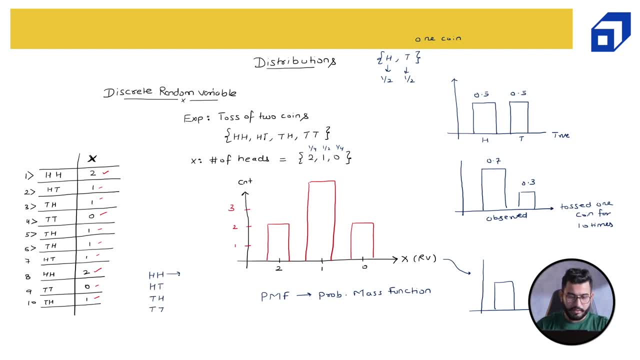 Please remember this probability is 1 by 4.. Probability of one head will be 1 by 4 plus 1 by 4, which is 1 by 2.. And this will be again 1 by 4.. So the true a PMF for this would look. 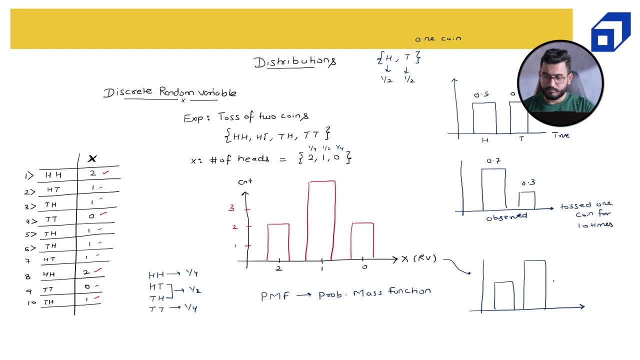 something like this, Where this would be 1 by 4, which is 0.25,, 0.5, and 0.5.. Again, 0.25.. This is the PMF for my random variable X, which is a true probability. 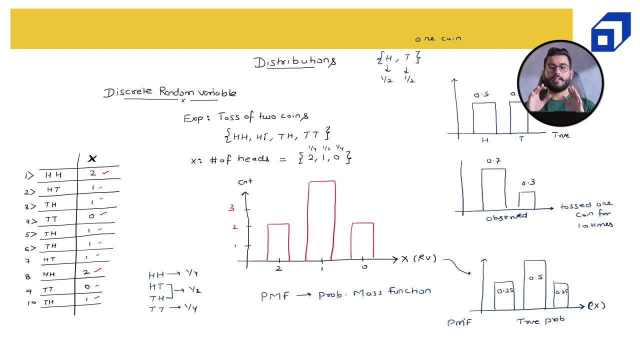 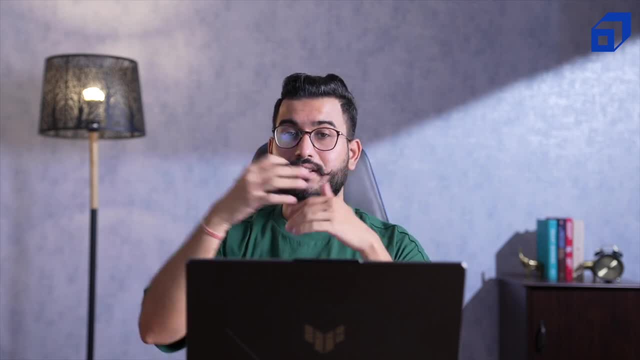 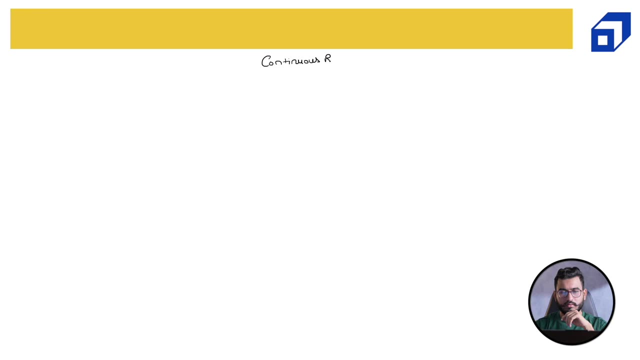 This is the PMF. This is for the discrete random variable. Now let's talk about the continuous random variable and how the distribution looks like For continuous random variable. if you guys carefully try to understand the continuous random variable, we cannot have the discrete type values or integer values, but we can have range also. We can have range right. 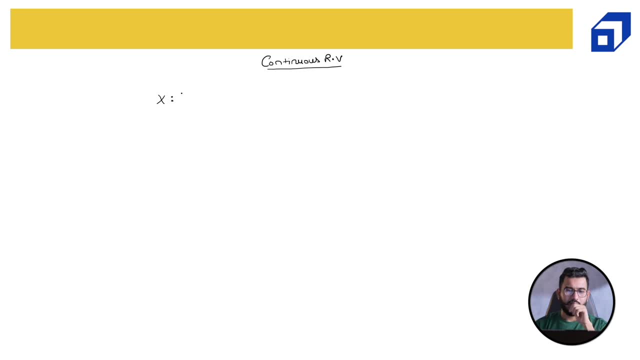 For example, let's say the random variable is time an employee takes to commute between home and office. Now let's say we have defined the minimum and the maximum range. Let's say: minimum: the person takes 10 minutes. Maximum, the person takes 60 minutes. Now I can. 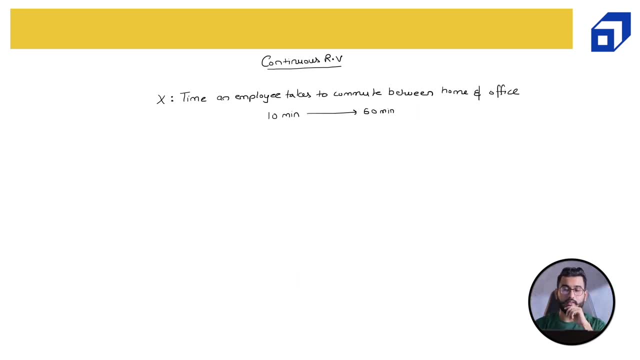 have endless possibilities between these two numbers, right? Let's say we have observed this. So let's say I have 10 minutes, I have taken one employee. or let's say I have taken myself And every day I'm just taking down. 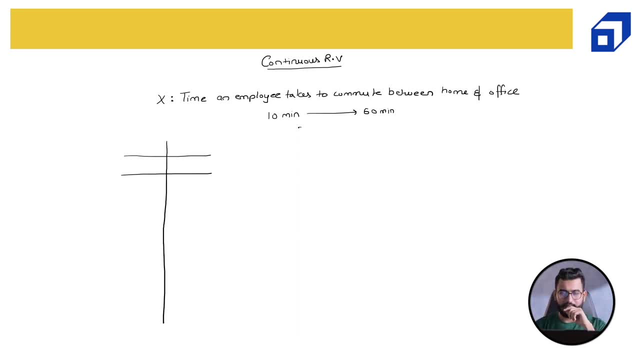 the number of minutes I took. So let's create a set over here. This is my observed set for X, So X observed. The observed set for X is: let's say, in the first day I took 11 minutes. Second day I took 32 minutes. Then let's say 20.. 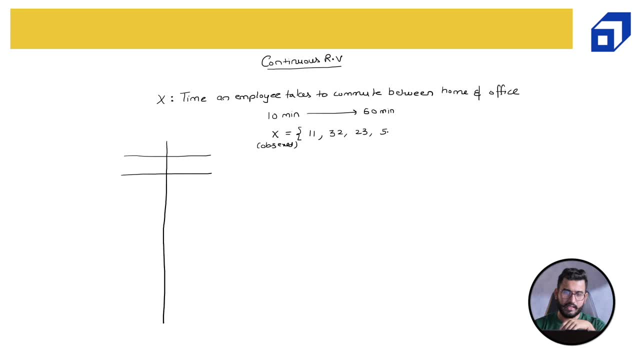 Then let's say 53 minutes, Then let's say 59 minutes, Then let's say 43 minutes, Then let's say 29,, 33,, 48,, 57 and 12.. So 1,, 2,, 3,, 4,, 5,, 6,, 7,, 8,, 9,, 10.. 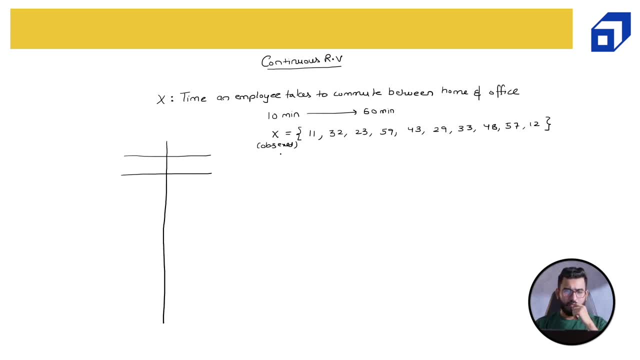 For 10 days. I observed the number of minutes I took. Now can I take each advantages over each of the previous set? asaret you of them as a random variable? No, because this is a continuous random variable. So my question to: 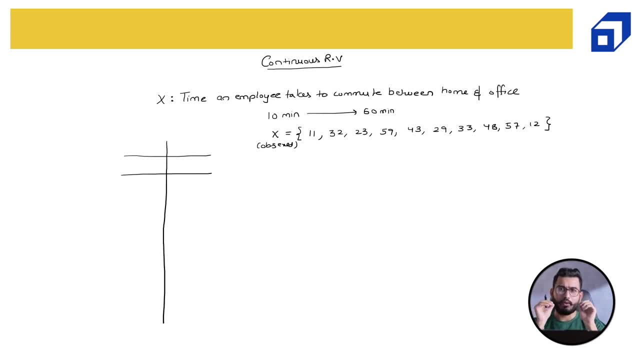 all of you is that: are these the only possible outcomes which I can get from this experiment? No, We can have more outcomes. If I perform this experiment for another 10 days, I can get more values. Let's say someday I took 23 minutes 2 seconds, So 23.2.. Let's say someday I took 11. 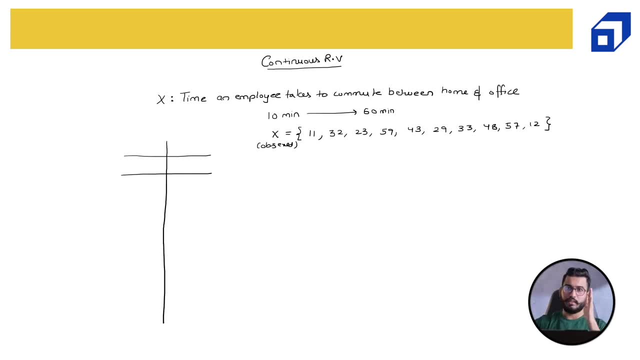 minutes and 5 seconds. So there are endless possibilities. So I cannot take each entry or each outcome over here as one random variable. Then what is the solution? I would go with the range. So let's define the range over here. So range would be, let's say, from 10 to 15,. 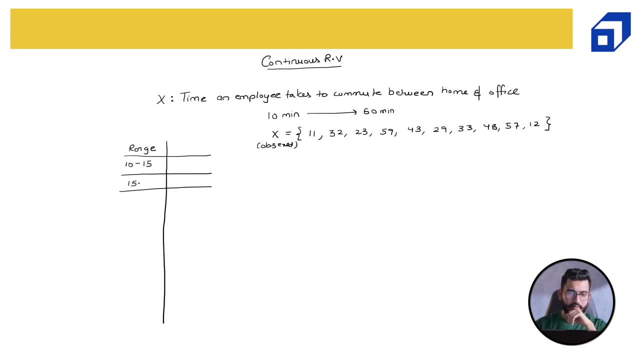 15 to 15.. So let's define the range over here. So range would be, let's say, from 10 to 15,, 15 to 20,, 20 to 25,, 25 to 30,, 30 to 35,, 35 to 40,, 40 to 45,, 45 to 50,, 50 to 55.. 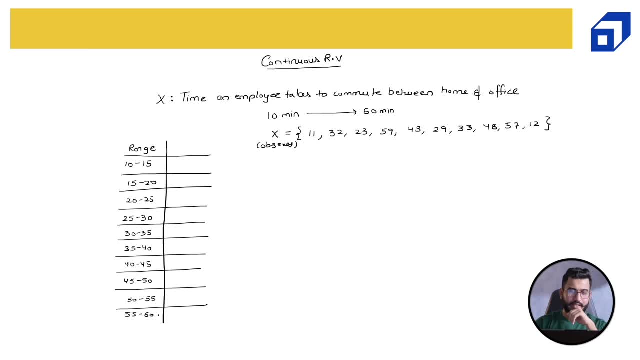 And finally 55 to 60. And I will now just write down number of times I observed a value between this range or in this range. So let's write the count. So in between 10 to 15, I was having this value which is 11 and 12. So I write 2 over here. Between 15 to 20, I don't have a value. 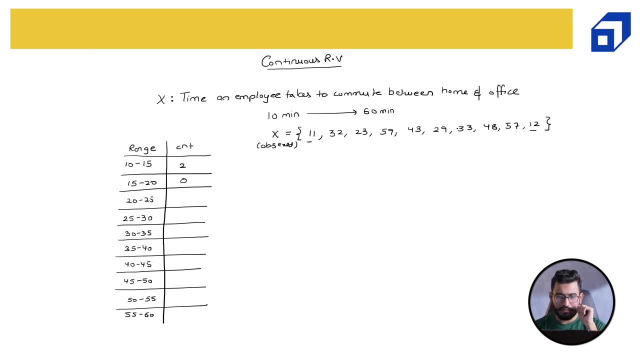 zero: 20 to 25,, 20 to 25.. I'm having one value, So I write 1 over here: 20 to 25,. I'm having 1.. 25 to 30,, 25 to 30, I'm having 1 value, so I'll write 1 over here: 30 to 35,. so 1 value. 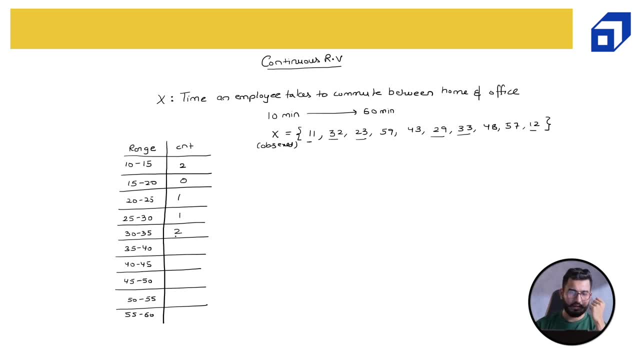 over here. 1 value over here, so 2 values 35 to 40, 35 to 40, I don't see a value, so, okay, 30 to 35,. I was having no value, so I should write 0 over here, 30,, no 30 to. 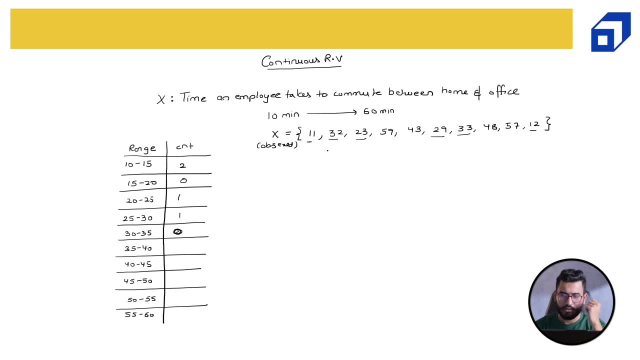 35,. I'm having 33 and 32,. yeah, 2,. this was correct. ignore if I'm doing something wrong, because I'm just trying to quickly fill this table. 35 to 40, 0,. 40 to 45,. 40 to 45, 1. 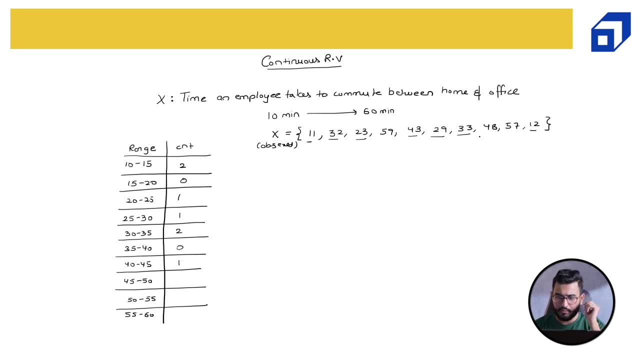 value over here, so 1, 45 to 50, 1 value over here, 50 to 55, I don't see a value 50 to 50,, 55 to 60, 1 value over here, 1 value over here, so 2 value. now, when I plot this, I 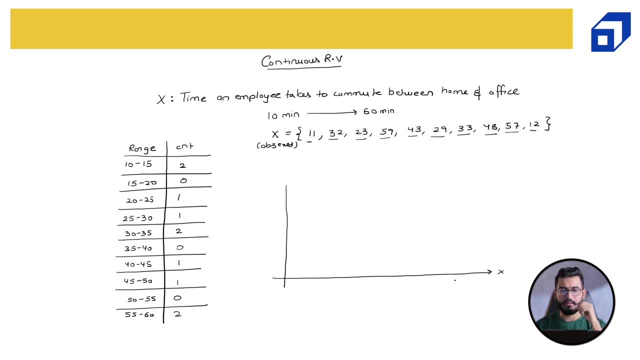 will plot it as a range. so my x is over here, which is again the time taken by an employee to commute between office to home. here I'm having the same count, but here I will have the range. so starting from 10, 15,, 20,, 25,, 30,, 25,, 30,, 30,, 30,, 35,, 30,, 30,, 30,, 30,, 30,. 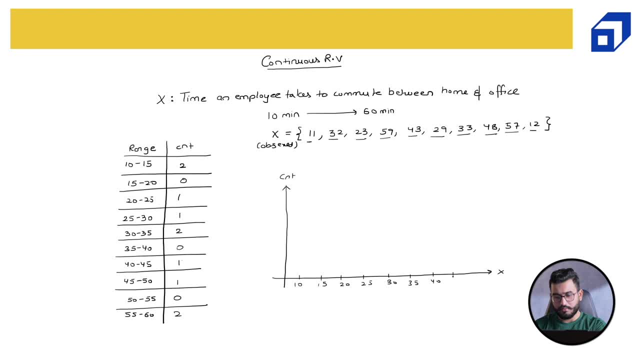 35,, 40,, 45, and so on till 60,, and then I will have this bars, which is known as the histogram. this is not the bar chart, this is the histogram. so 10 to 15, let's say 2,. 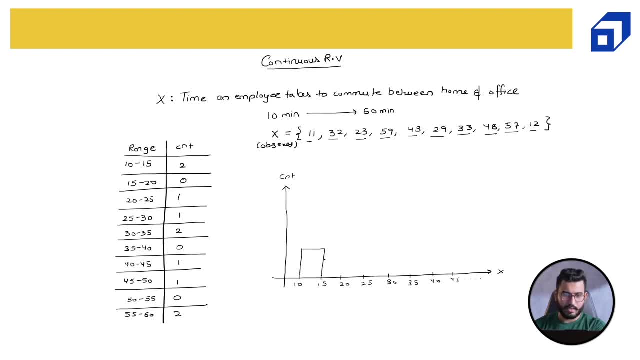 like this: then 15 to 20, I'm having 0, so a line like this: then 15,, 20 to 25, I'm having 1 and then 1, so let's say like this and then: 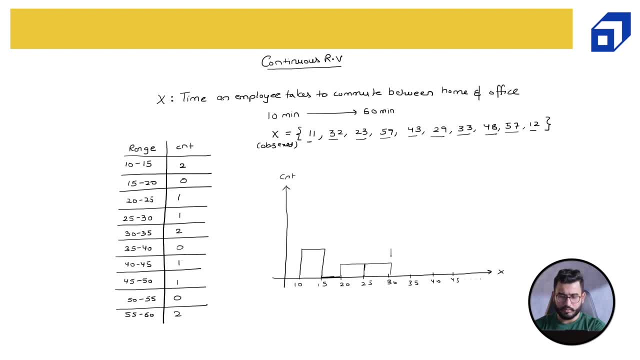 then again I'm having 2, and then again I'm having 0, then again 1 and 1, and so on. now this is basically my probability density function- pdf- probability density function. now why I'm calling it as a density? because if I ask you, what is the probability of a person takes 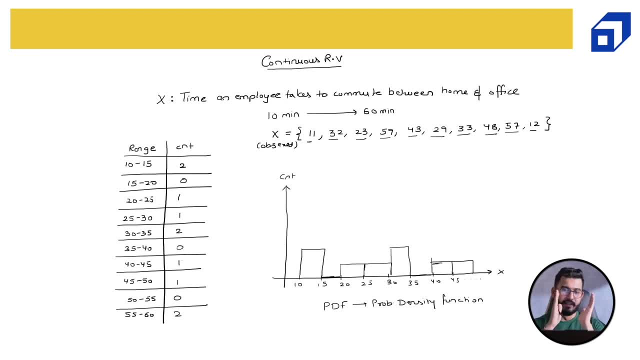 the time between 10 to 15 minutes. I'm not talking about one point, I'm talking about a range which is density. so that is the reason. here the distribution is known as the density, and please remember the probability of a 1 point- 1 point- compared to density. 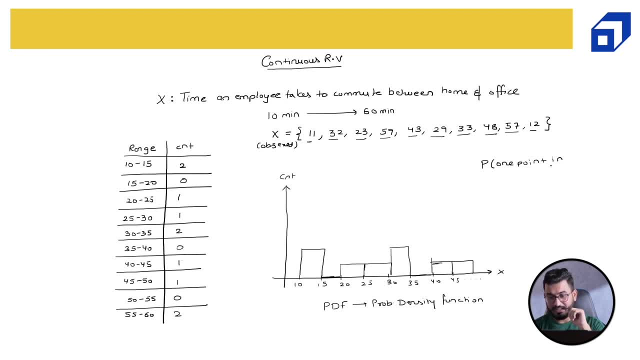 one point in a continuous distribution or continuous random variable is always equal to zero. If I ask you what is the probability that a person will take 10 minutes? That would be zero. The probability is zero. The reason is: we cannot calculate it. We cannot calculate. 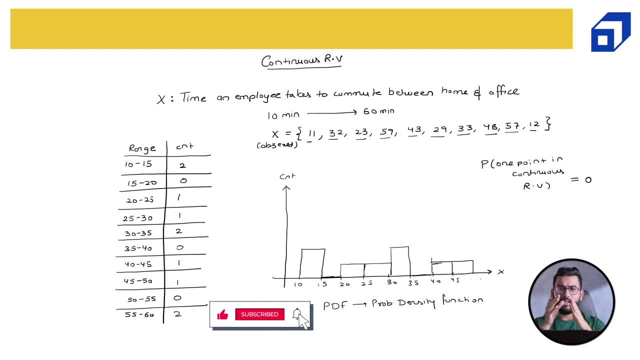 it because the way we are calculating the continuous random variable is by using a measure. Here we are using a measure as the time taken by a person, right And 10 minutes- is something that a person can take endless number of time, So we don't know how many times a person can. 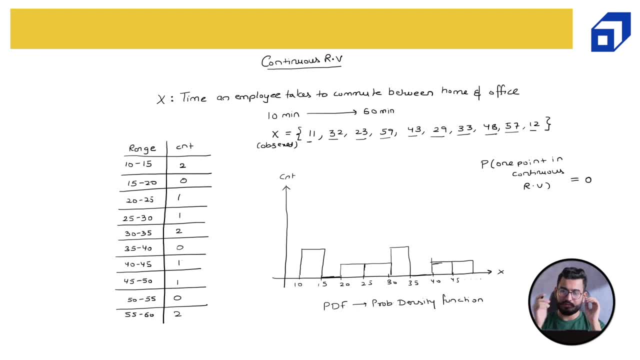 take 10 minutes divided by we know So how many times a person can take 10 minutes, The probability of 10 minutes is zero. That would be number of times the person takes 10 minutes divided by total time. So total time. we know total time is 60 minutes, but how many times the person has taken 10 minutes? 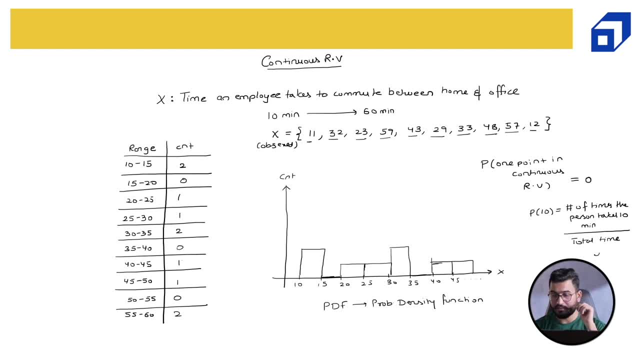 I don't know the answer. This can be infinity also, right, I don't know that. So the probability will end up zero, Becoming zero. So the probability of a point in a continuous random variable is zero, And the reason we call it as a probability density function is because we are not talking about 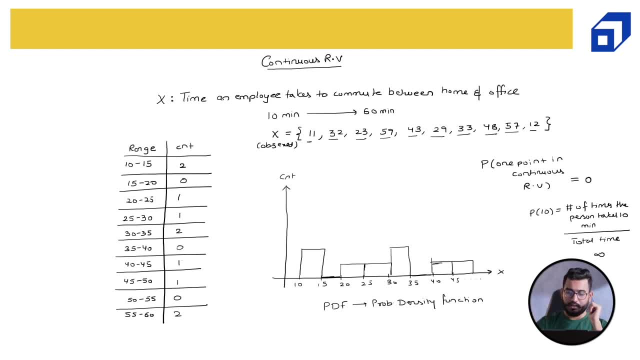 one point: probability. We are talking about a range Now within discrete random variable, the distribution for discrete random variable and the distribution for continuous random variable. we have some very general distributions, some standard distributions That are very important in the field of statistics and probability. So that is what we are going. 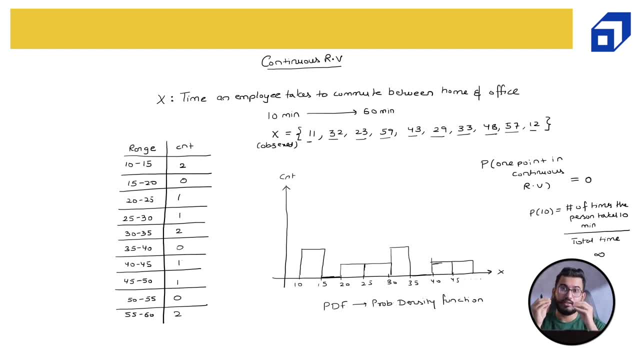 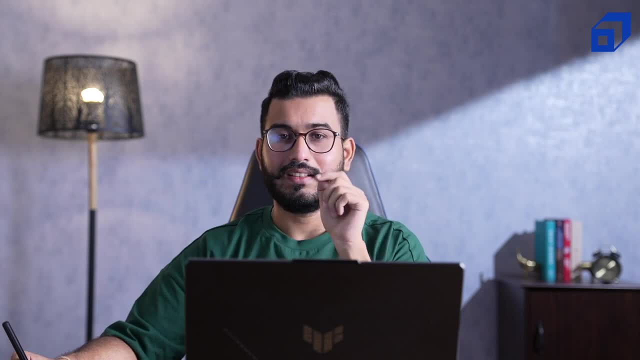 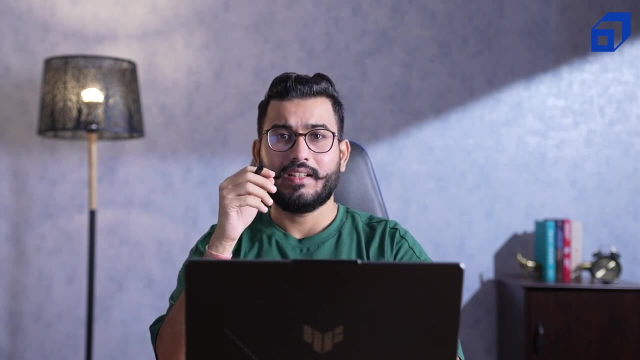 to learn next The various type of standard distribution that comes under both discrete and continuous. So we have talked about discrete random variable and continuous random variable and we have seen very simple example of how we can create distributions for discrete and continuous. Now there are some standard distributions. 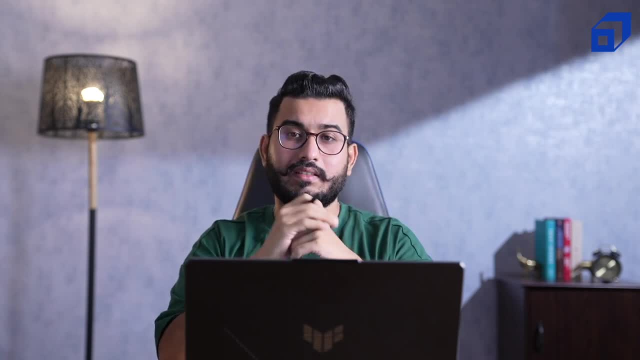 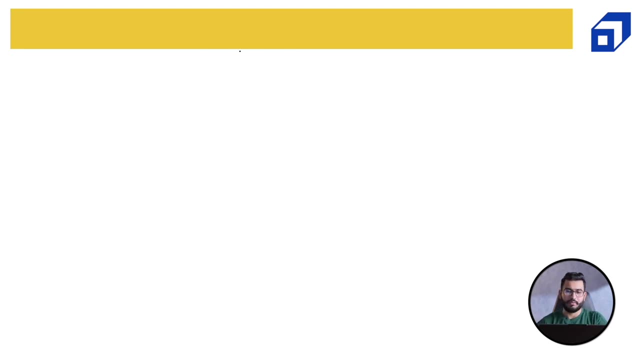 Okay, Okay, Okay Okay. that comes under discrete and continuous. So what we are going to do, we are going to talk about these standard distributions. So the very first, we will first talk about discrete. So within discrete, the discrete random variable, we have two very important distributions: One: 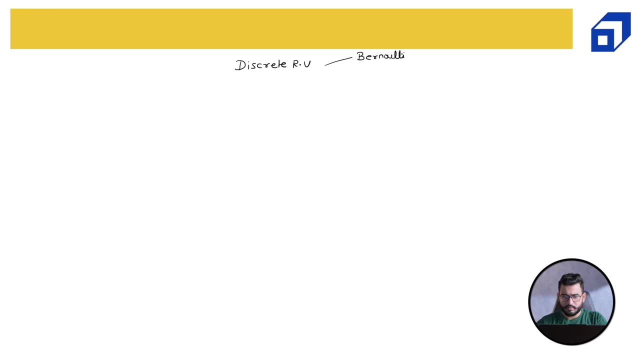 is known as Bernoulli and the second one is known as binomial. So Bernoulli distribution and binomial distribution. Now, what is the Bernoulli distribution? or we will first talk about the Bernoulli experiment. So when we talk about the Bernoulli experiment, the Bernoulli experiment is a particular experiment. 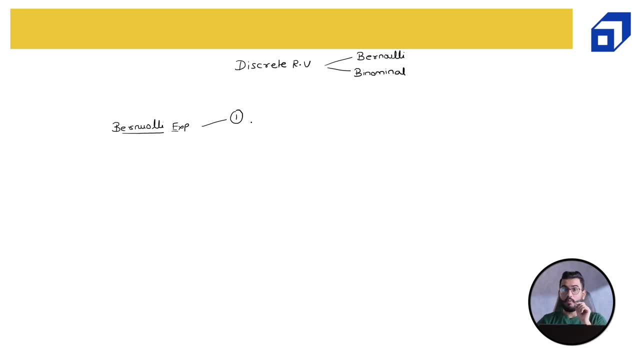 in which number one, the outcome is always binary. So the outcome is always binary, which basically means the outcome is always binary and, as you can see here, the outcome is always binary and, as you can see here, the outcome is always binary and, as you can see here, 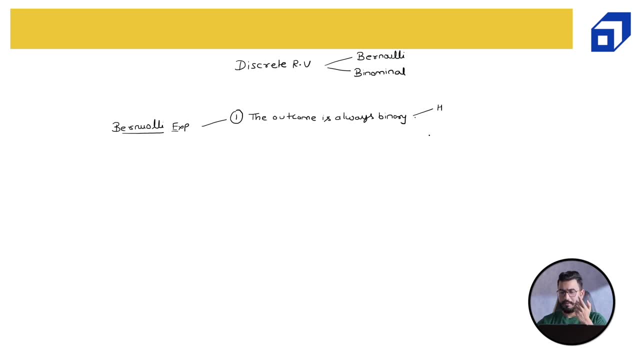 as you can see, here the outcome is always binary, which basically means thiscell og the outcome is either head, or maybe win or loss, head or tail. So let's say head or tail, win or loss, or maybe one or zero, So it will always be binary. The second one is the number of trials. 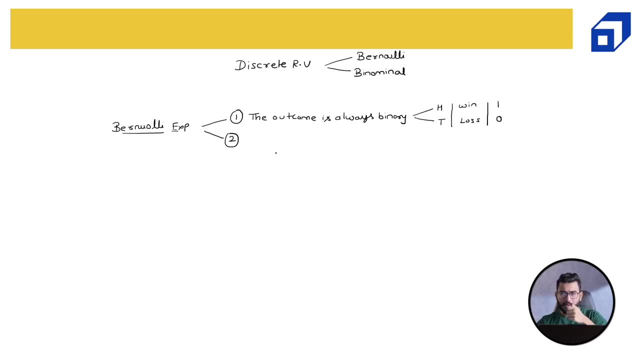 is only one. So we are just performing the experiment for one time, So the number of trials is only one. So, for example, let's say I'm having a coin and I tossed this coin for one time, So toss off this coin. 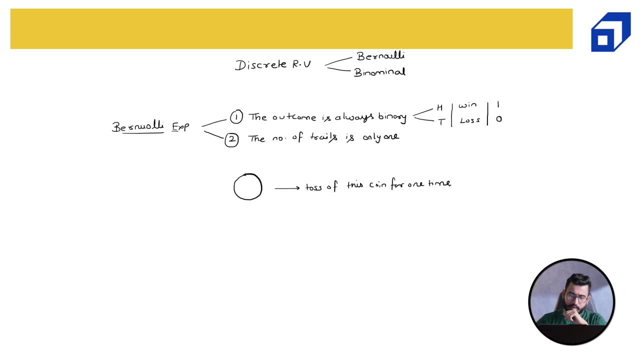 For one time Now, can I consider this as a binary Bernoulli experiment? Yes, Why? Because when I toss this coin, I may either get a head or a tail, So the outcome is binary. Now, since the outcome is binary, this experiment is the Bernoulli trial. So why I'm calling it as a trial? 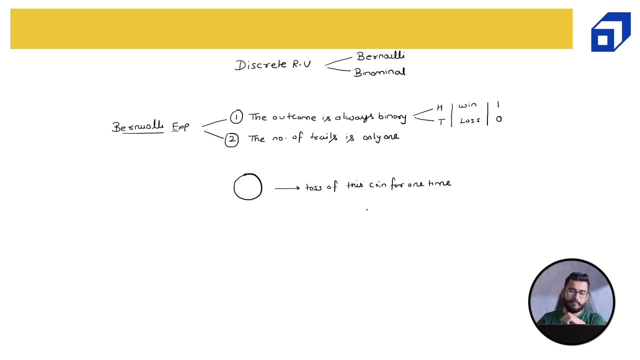 because I am performing the experiment for one time, So I can either get head or tail. So the Bernoulli trial is the Bernoulli trial, So I can either get head or tail. So the Bernoulli trial distribution looks like very simple. We have already seen it, but I'm drawing it again. 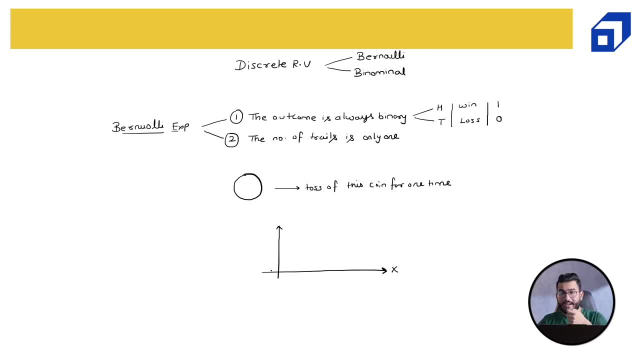 Let's X represent the number of heads when you toss a coin for one time. So you may either get a head. So let's say I obtained a head and for tail it is nothing. So this is basically my Bernoulli distribution, Bernoulli distribution. Now, please remember one thing: There is nothing. 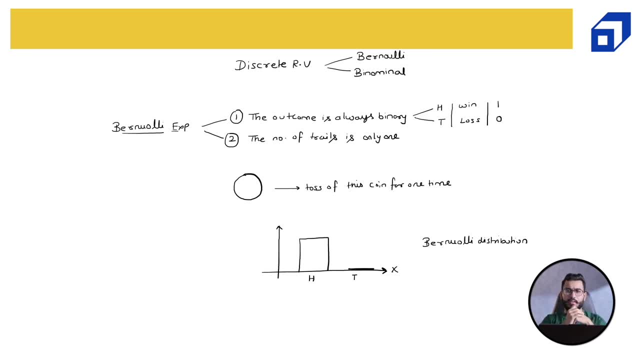 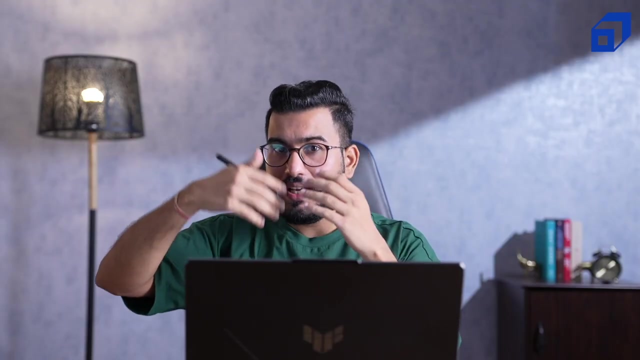 difficult to remember about Bernoulli distribution. It is just a particular experiment which is having binary outcome and one trial. binary outcome, one trial, Now binomial- is something very much Associated with Bernoulli. So when I perform the Bernoulli experiment for N number of times, then we get a binomial experiment. So what is binomial, Binomial, binomial experiment? So when? when the Bernoulli experiment? So when? when the Bernoulli experiment? So when, when the Bernoulli experiment, When the Bernoulli experiment is performed for N times, we get binomial experiment, We get binomial. 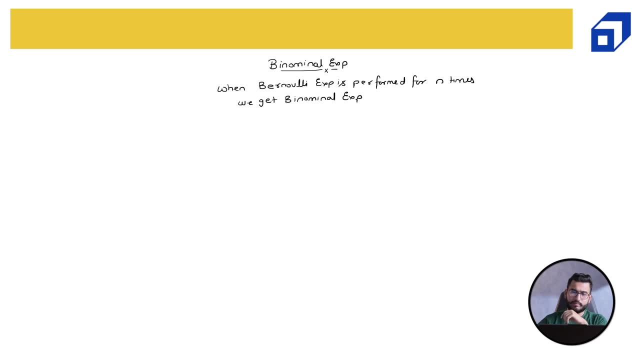 experiment. This is my binomial experiment. Let's take one example. Let's say I'm having a bag and we will try to understand the binomial experiments. So binomial experiment is nothing. but when I am performing the Bugün experiment for N times and becomes binomial Again, the outcome of 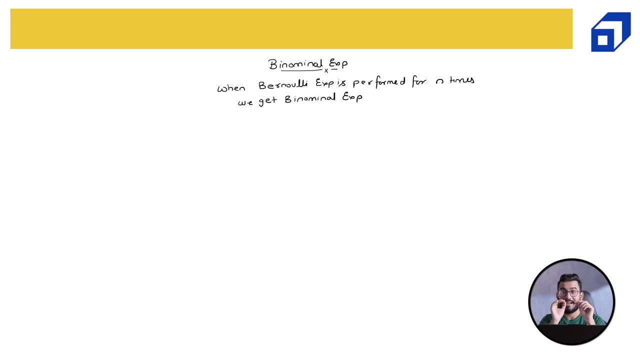 each trial in binomial experiment is binary. So again, as you know that you are having a coin and you are tossing it for 10 times, So since I am tossing it for 10 times, it becomes binomial, But the outcome 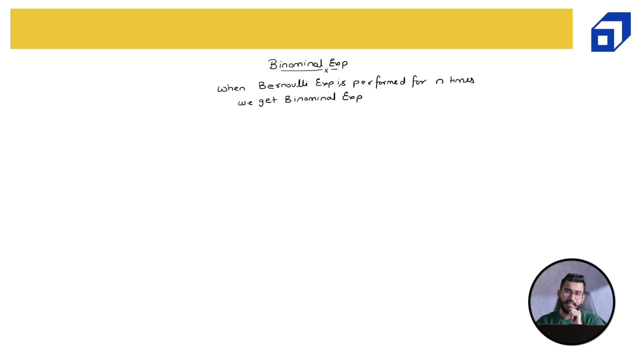 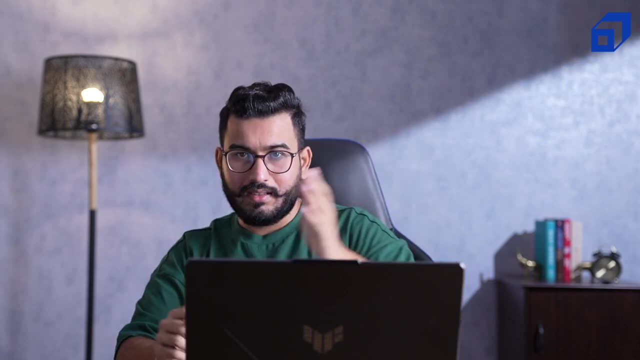 Of each Tomorrow Of N times, It becomes binomial, but the outcome of each bomb- higher For this question style- is going to be either head or tail, which is binary, and that is the reason it is a binomial experiment. so we have n Bernoulli experiments when I combine. 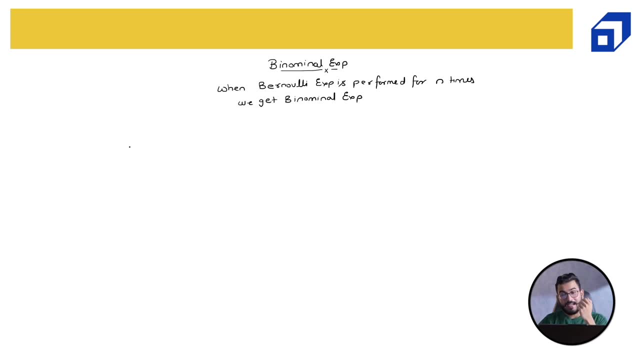 them, it becomes binomial. now let's understand how to calculate the probability of binomial experiment. so probability of binomial experiment. okay, now let's say I'm having a bag and this box is having, let's say, two orange balls. so two orange balls, so let's say the bag is having three orange ball and 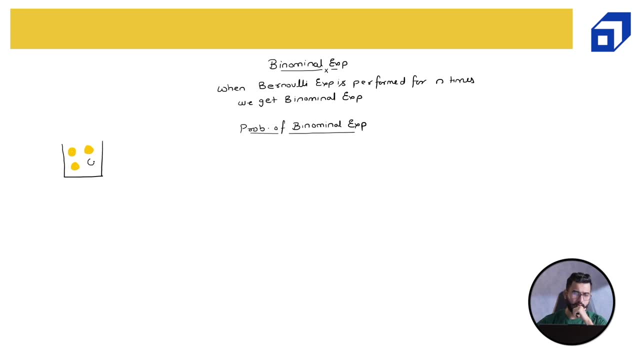 two white balls, so one white point, two white one, so three orange and two white. Now my random variable X is the number of heads. oh sorry, my random variable X is the number of orange balls I may get out of this bag. Number of 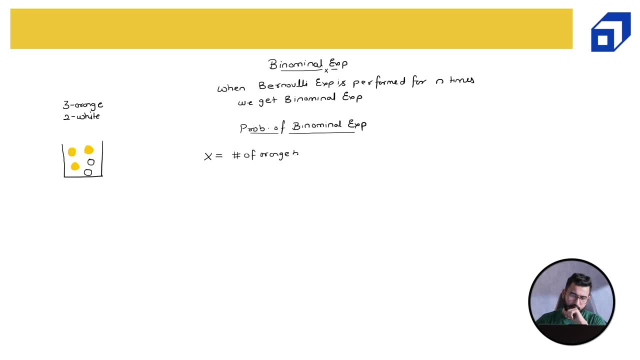 orange balls. I may get out of this bag if, if the experiment is performed for three times. Now, if you are not able to understand it, let's try to take the example. So the experiment is: we have to take the ball out of the bag. 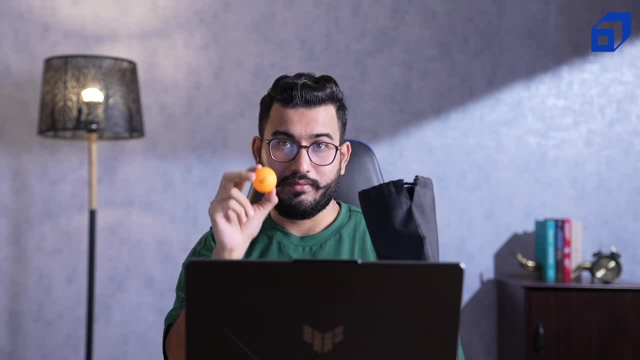 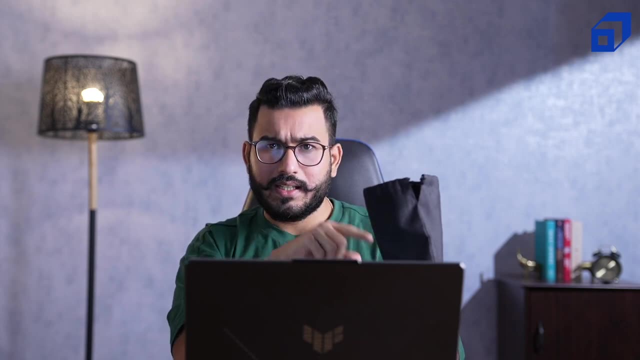 note down the color. So what's the color Orange? We will note it down and put the ball back to the bag, And I will do this for three times. Now is this a Bernoulli trial When I'm taking the ball? 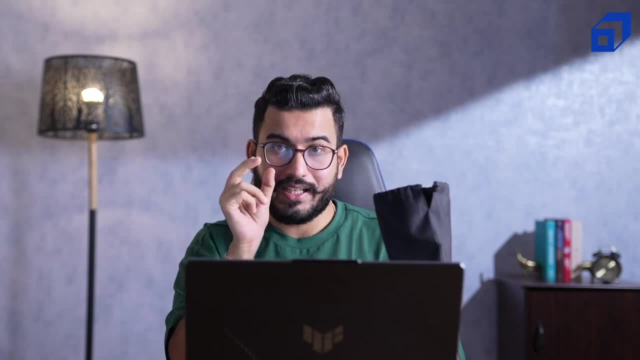 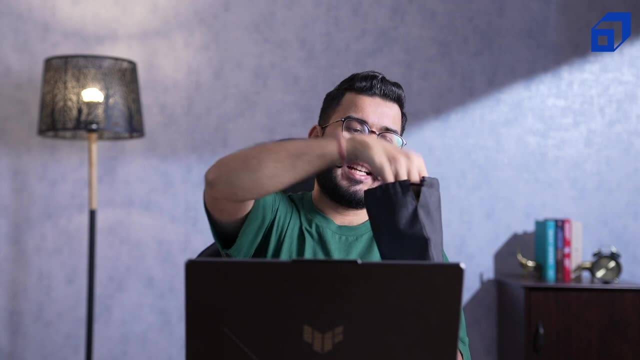 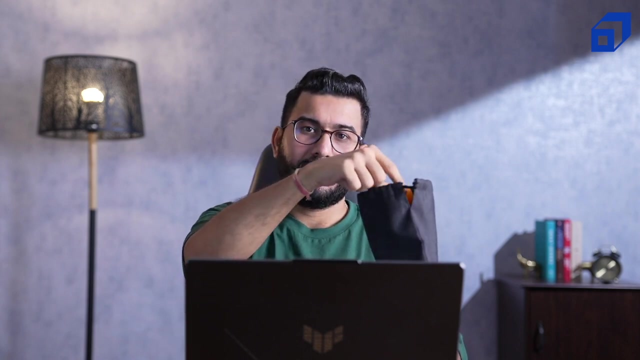 out of the bag for one time. is it a Bernoulli trial? Yes, Why? Because I can either get an orange ball or not get an orange ball. So first time I obtained an orange ball. this is my four one Bernoulli trial- and I place the ball back to the bag Again. 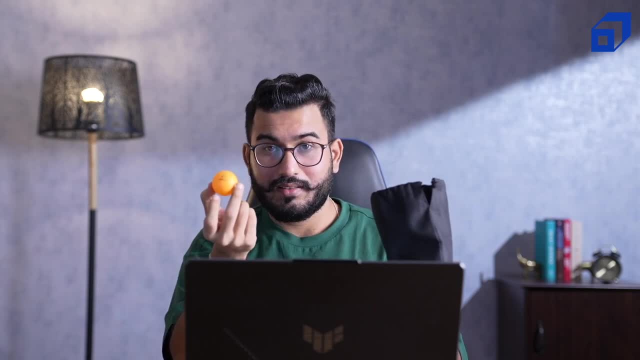 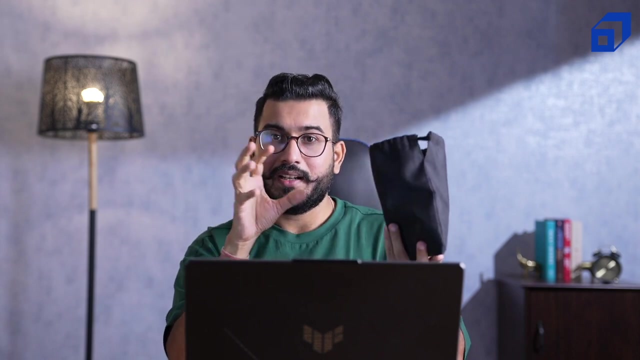 I did the experiment. I obtained again an orange ball and I note down the color. I put the ball back to the bag And I did it again. I again take a ball out of the bag. It came out to be orange. I note the color and I put the ball back to the bag. Now what is happening? 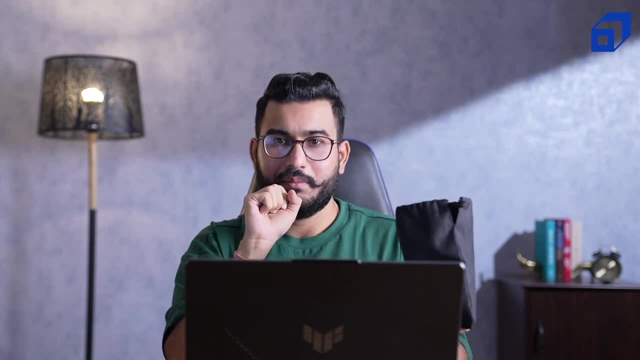 have performed the Bernoulli experiment for three times. so each time I was taking the ball out of the bag it was a Bernoulli trial, and I have performed the Bernoulli trial for three times. so let me just note down the outcomes, first of. 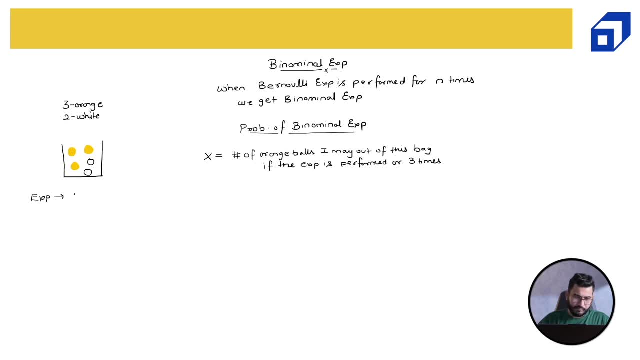 all, let me note down the experiment. the experiment is: take a ball out of the bag, then note down the color of the ball and then put the ball back to the bag. back to the bag. now we have to perform this experiment for three times. now we have understood the experiment. right now, let's say I'm interested in finding out. 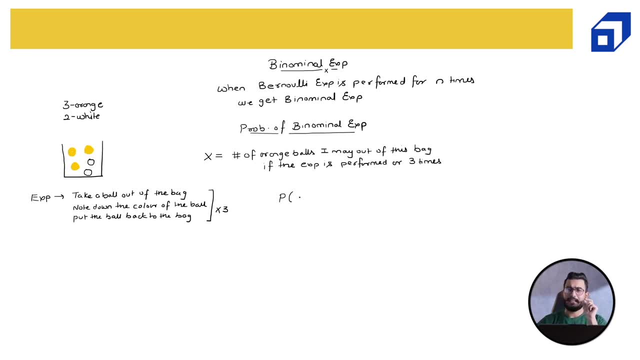 the problem that I will get exactly two balls when I am performing this experiment for three times. so two orange balls, two orange balls in three trials. now what are the possible combinations in which you can get two balls or two orange balls? let's note it down. so this is my trial number one. 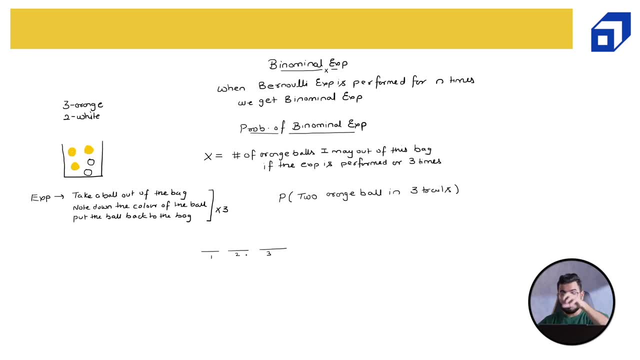 two and three. let's say, for the first two trials I obtained orange, so let me write O, O, and then you obtained a white ball, so white. then for the first you obtained orange, then white, then orange. then for the third you obtained white, then followed by orange and orange. so now these are the three possible. 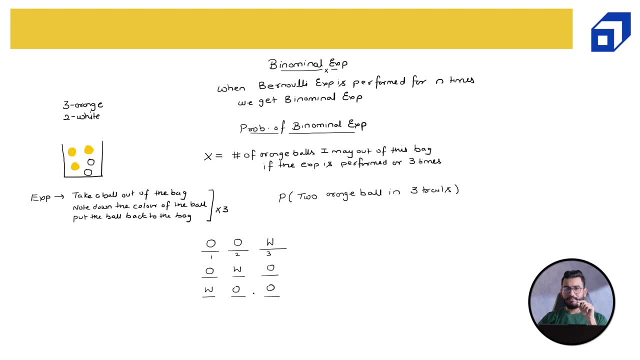 combinations I may get out of this experiment. now, what is the experiment? I am taking a ball out of the bag, noting down the color, putting the ball back to the bag, performing this experiment for three times. my objective is to find out the probability that I will get two orange balls in three trials, when I'm 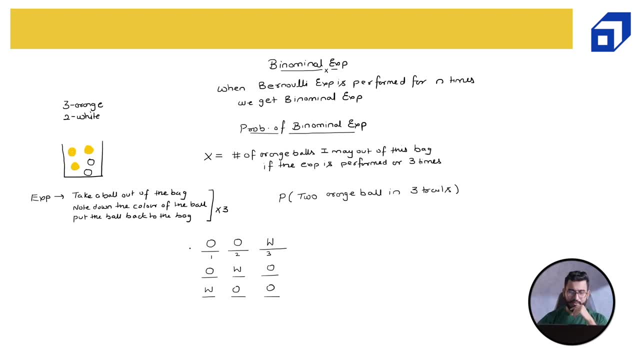 performing this experiment for three times. these are the three possible combinations. now, if you carefully observe, each trial is independent of the other, because every time I am taking a ball out of the bag, the bag is still having five balls, because we have total of five balls, right? so what is the? 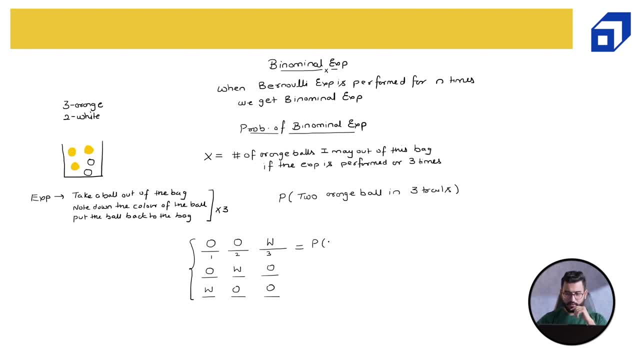 probability of getting orange, orange, white, it will be simply probability of orange multiplied by probability of orange multiplied by probability of white. similarly, for this orange, white, orange would be probability of orange multiplied by probability of white, multiplied by probability of zero, sorry orange, then white, orange, orange would be probability of white. 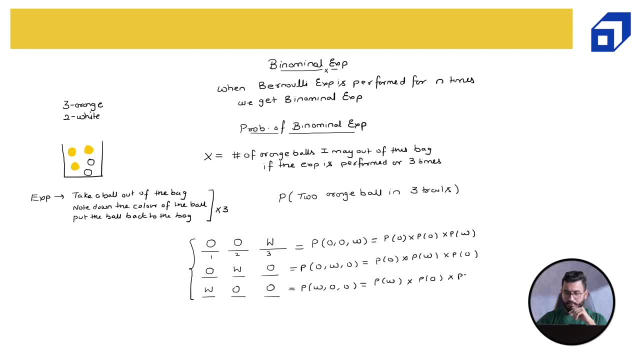 multiplied by probability of orange. multiplied by probability of orange: now, probability of orange is three divided by five. probability of oranges 3 divided by 5. probability of white ball is 2 divided by 5. so this will be 3 by 5 into 3 by 5, into 2 by 5.. This will be 3 by 5 into 2 by 5, into 3 divided by 5.. 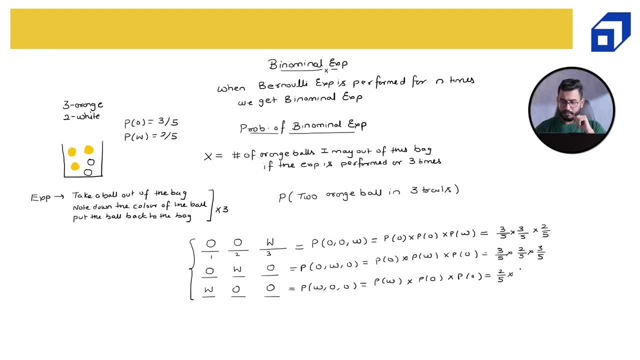 And this will be 2 by 5 into 3 by 5 into 3 by 5.. So if you carefully observe, I can write each of them as 3 by 5 to the whole square into 2 by 5.. 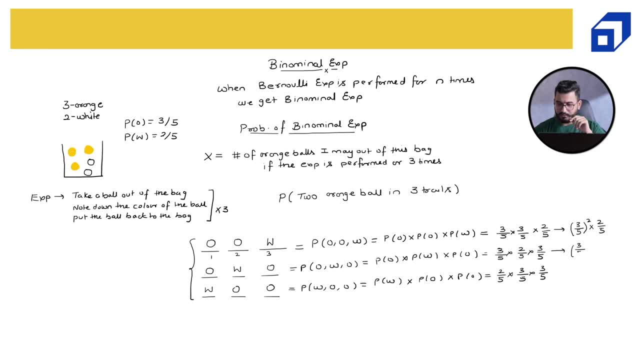 I can even write this as 3 by 5 to the whole square into 2 by 5.. I can write this as 3 by 5 to the whole square into 2 by 5.. Now, what is the probability of getting 2 orange? 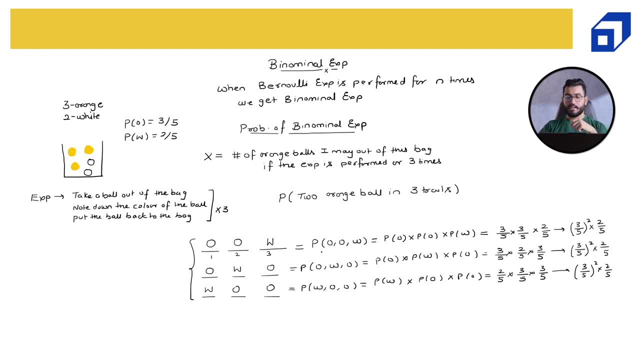 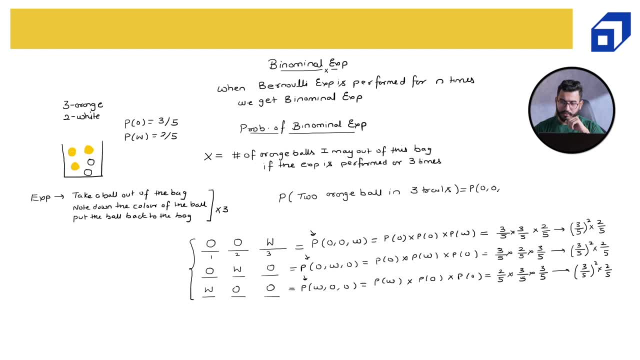 So it will be probability of O comma O comma white, which is plus probability of orange comma white comma orange, plus probability of white comma orange comma orange. Now we have already calculated everything, So it is- I'm just taking it over here- So it will be three by five to the. 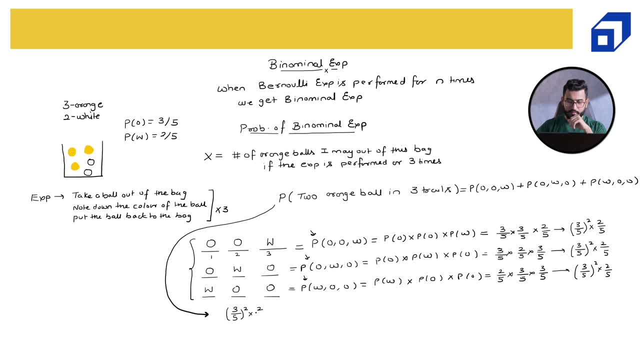 whole square into two by five, plus three by five to the whole square into two by five, plus three by five to the whole square into two by five. Now all the three terms are similar, So we can just simply write it as three times of three by five to the whole square into two by five. 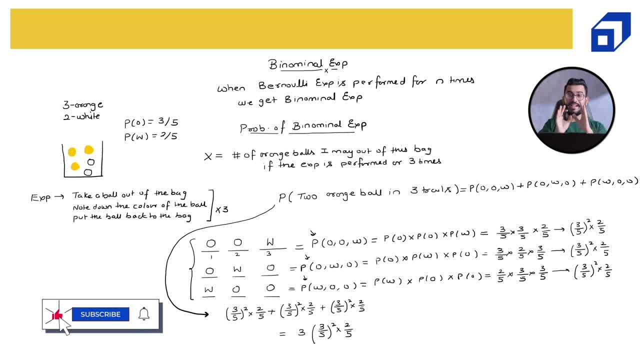 Now this particular equation can be generalized for any binomial experiment. How Let's see The generalized equation is N, CX, PX, Q to the power N minus X. This particular equation can get you the probability of any binomial experiment. What is N? N is the 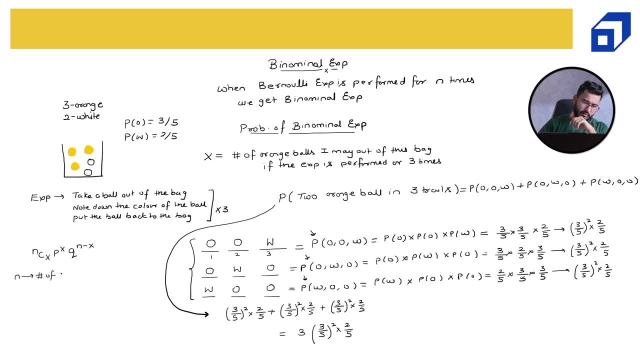 number of Bernoulli trials. Bernoulli trials X is the number of success and N trials, P is the probability of success And Q is the probability of failure. So if I try to map this equation for this particular experiment where I have calculated, the probability is three. 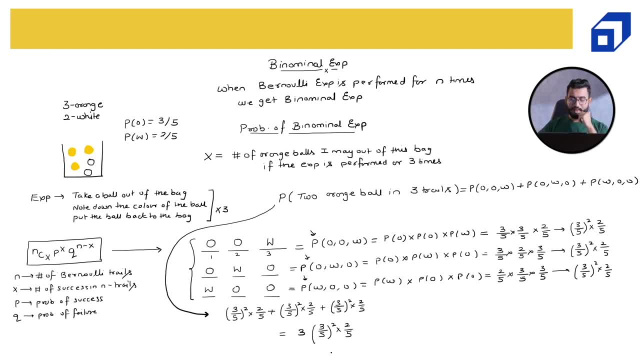 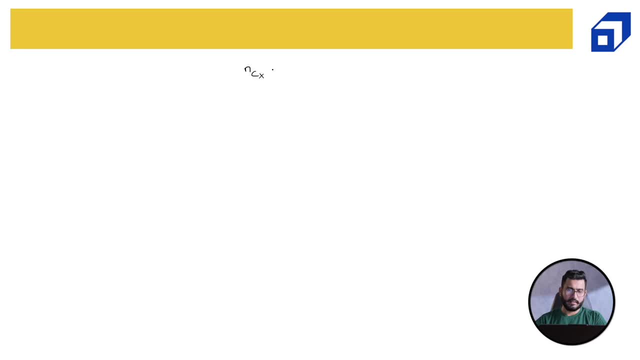 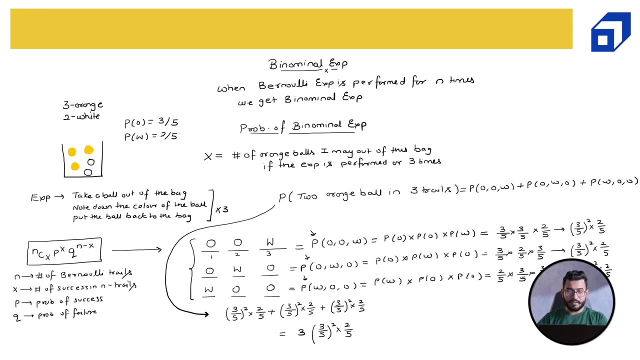 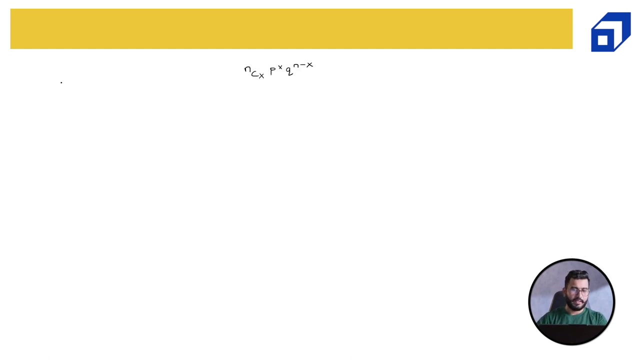 times of three by five to the whole square into two by five. Let's try to do it in the next slide. So the formula is N, CX, PX, Q to the power, N minus X. Now in the last experiment we were performing the trials- Bernoulli trials- for three times. Here I have written it right. So my value of N is three. 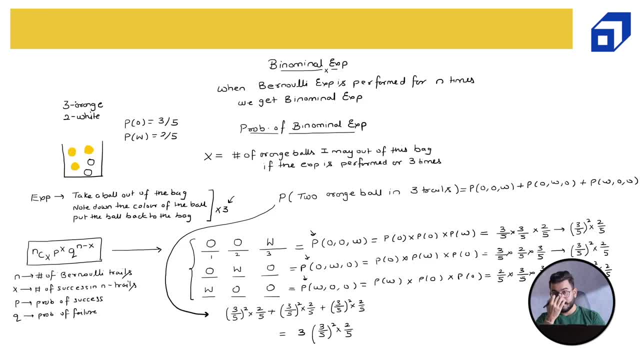 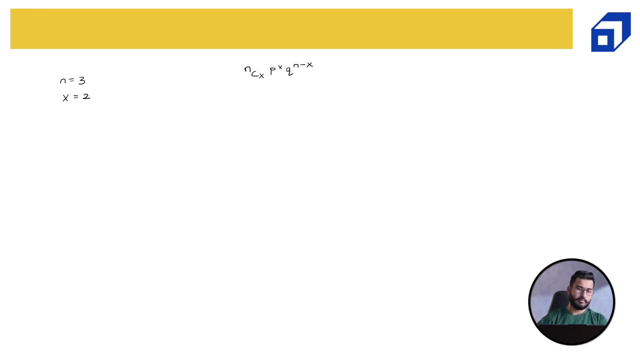 Now, what is X? X is the number of success. X is the number of success. X is the number of success. Now, if I consider getting an orange ball as a success, then I was interested in getting two orange balls. So my X is two because I'm interested in getting two orange balls. P is probability. 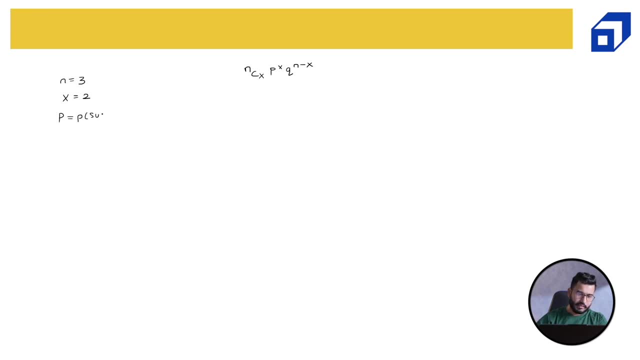 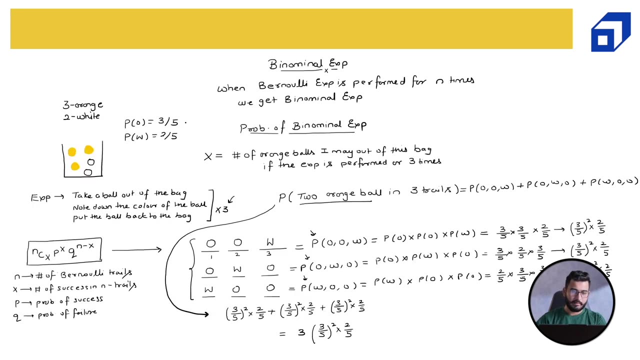 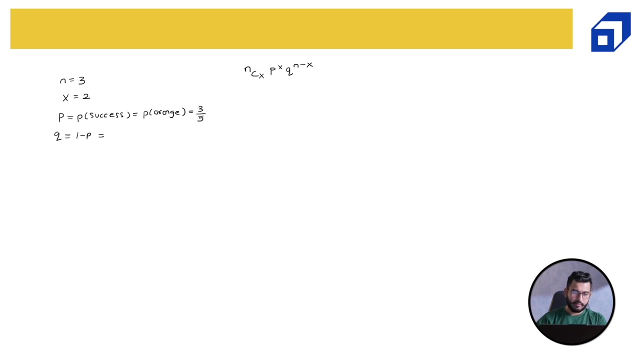 of success, which is nothing but probability of orange, And orange probability is three by five, And Q is the probability of failure, which can be also written as one minus P. This is given as two by five. Now if I put everything on the formula, this will be three C, two, three by five to the two. 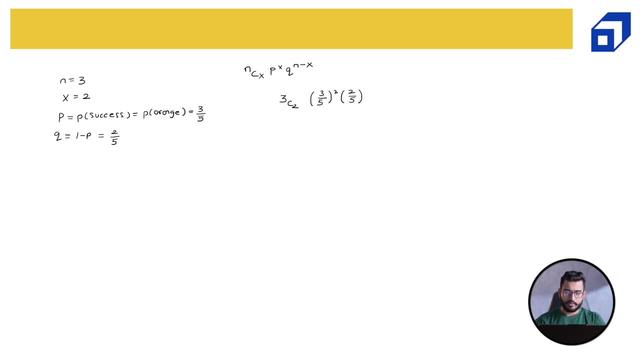 into two by five, to the power of three minus two, which is one Now the N CX factorial. this particular term can be expanded as N factorial upon X, factorial minus X factorial. So three C two would be three. factorial upon two. factorial three minus two. 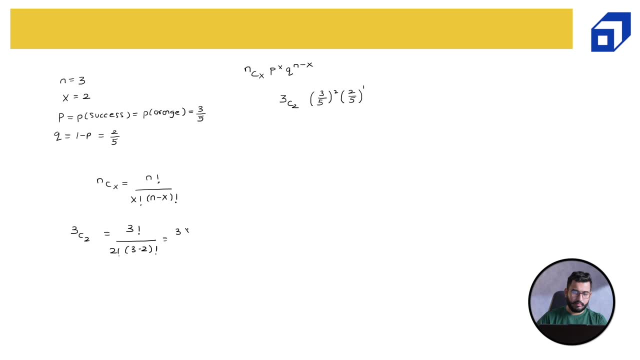 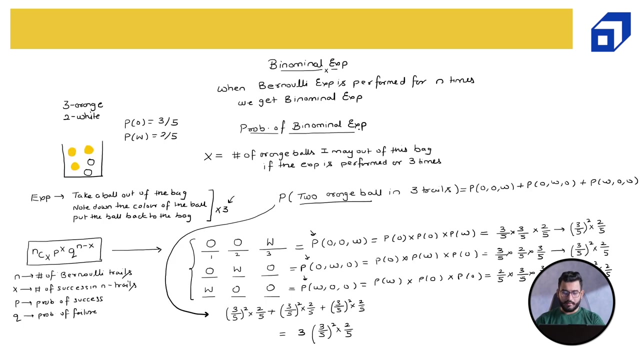 factorial, which is three into two factorial divided by two factorial into one factorial. Two factorial will cancel out two, So we'll be left with three. So three times of three by five to the whole square and two, two by five. And here you can see we have already done this manually. 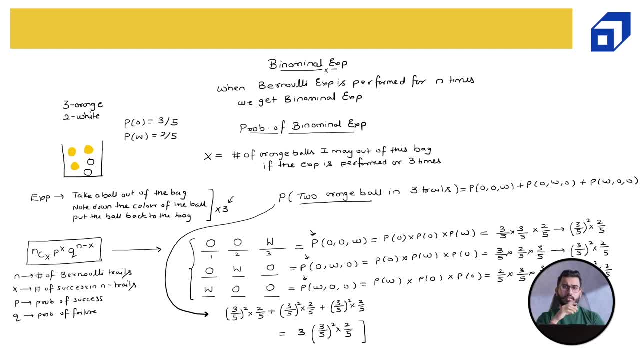 So using this formula, you can find out the probability of the number of success in N Bernoulli trials, The number of success, which is X, in N Bernoulli trials, which becomes binomial right. Let's take one more example. 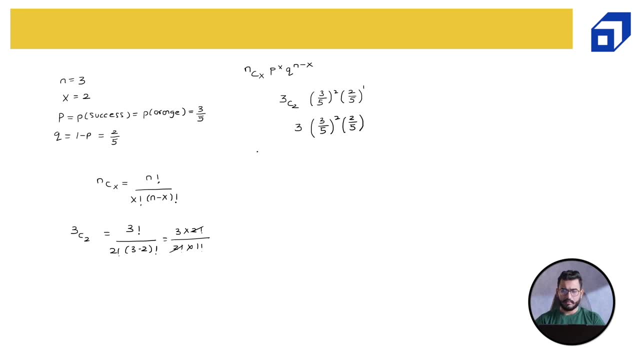 a quick example to help you understand this. So I'll just create a portion over here. So let's say there is a person who is trying to shoot a target. Here we have a person this person is trying to shoot a target for for 10 times. for 10 times, So N is 10.. Now is this: is this particular experiment. 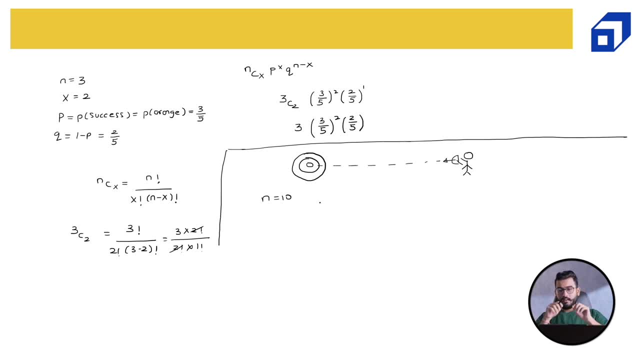 consists of a Bernoulli trial. Yes, because when the person is trying to shoot the target, it will either hit or miss. So it is a binary experiment, which is the outcome is binary And if I consider the experiment to be performed for one time, it is a Bernoulli trial, Since I'm performing 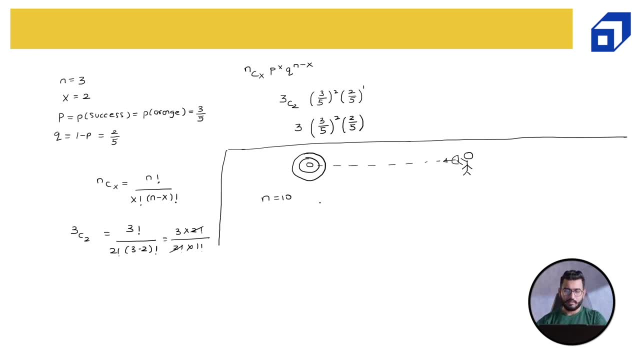 this experiment for 10 times, it becomes binomial experiment. So let's say the person is trying to hit the target for 10 times, The probability that he will make a hit is, point, let's say, 0.4.. So there are 40% chances that if a person tried to try to make a hit to the target, 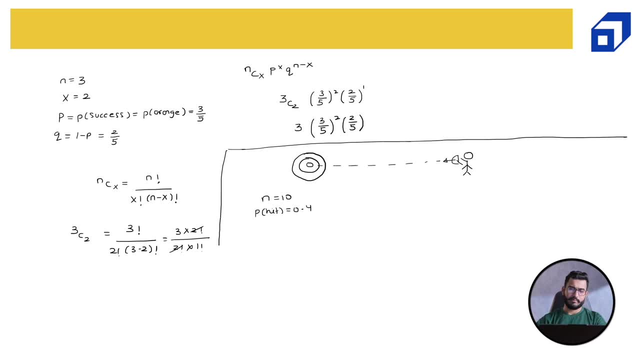 it will hit the target 40% of the time. So the probability of miss will be 0.6,. right Now I'm interested in probability that he hits the target exactly 0.6.. 0.6. 0.6.. 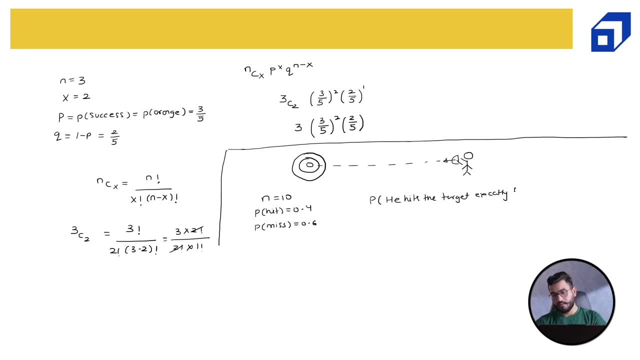 0.6.. Exactly for five times. So I'm interested in five successes in 10 Bernoulli trials. so my x value will be five. I quickly apply the formula ncx, pxq to the power n-x, n10c5: probability of hit is point 4 to the power 5, and then point 6 to 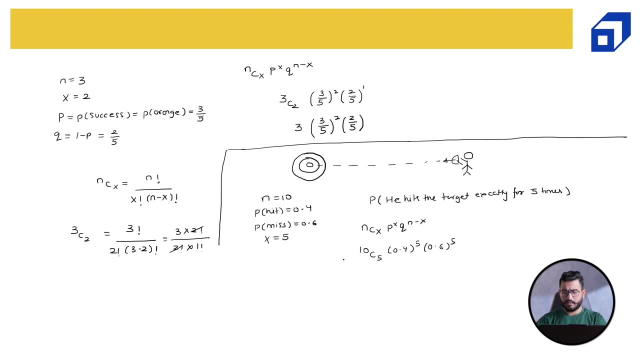 the power of 5.. 0.6. 0.6. 0.6. 0.6.. you can solve this and you will get your answer. What is the probability that if the person is trying to hit the target for 10 times, he will make a hit? He will make an exact hit for five. 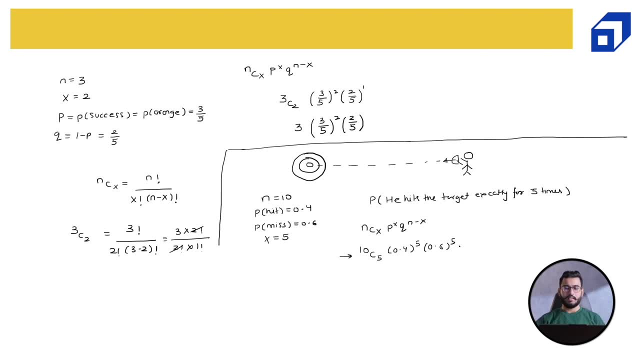 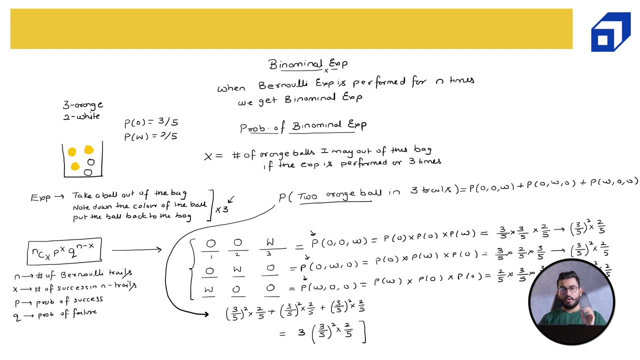 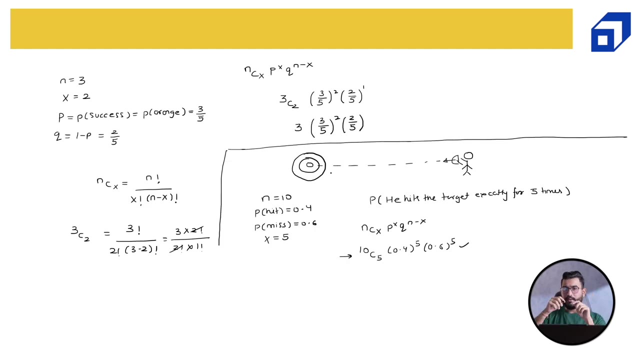 times And this will be your probability. This is the binomial probability. Now, if I calculate all the probability for all the random variables, in this case, in the case of hitting the target, what is my random variable? My random variable X is the number of times this person 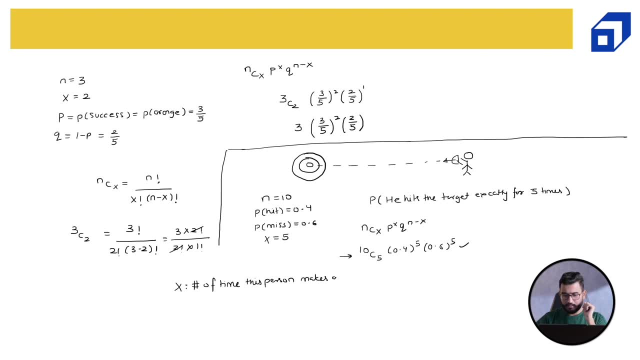 makes a hit. Now the person can make a hit for all the 10 times, for 9 times, for eight times, for seven times, six times or maybe for zero times. So these are all the random variables. Now, against each random variable is why calculate the probability and I plot them. 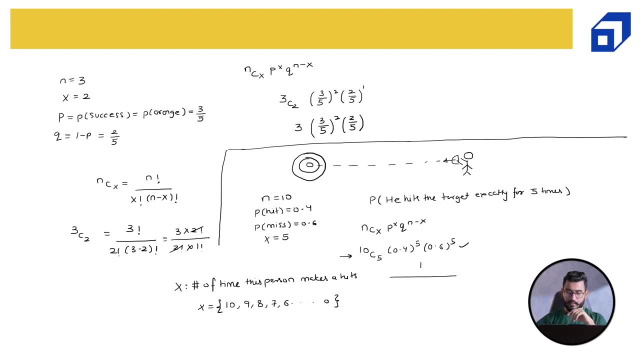 So let's say: here I'm having X, here I'm having probability of X is equal to XI. And if I calculate all the probability, what is the probability that he will hit the target? for exactly 10 times, for nine times, for eight times, for seven times and so on? And if I plot it in a 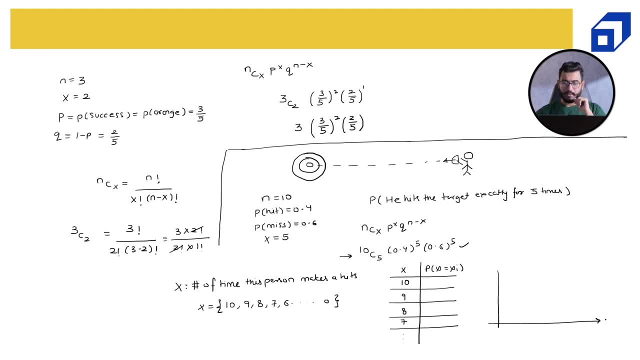 mass function. so here I'm having X, here I'm having, let's say, probability P of X is equal to XI, then this will become my. this will basically become my PMF of binomial probability or binomial experiment. I hope everyone is clear about this. We can have a quick Excel example to demonstrate you how this. 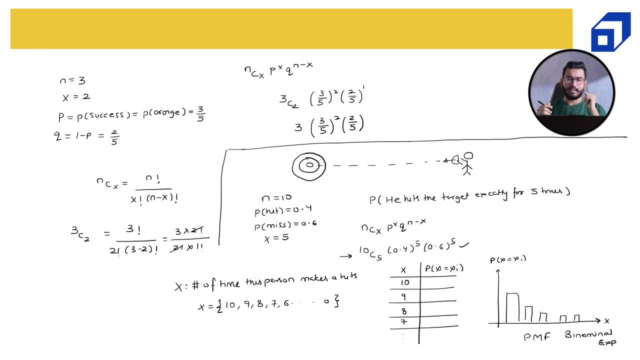 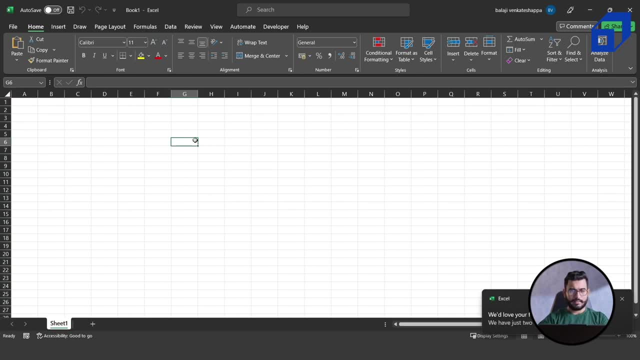 particular PMF looks like. So let's look at an Excel example. Now, here I'm having an Excel worksheet. Let's say, this is my X, which can be 0,, 1,, 2,, 3,, 4,, 5,, 6,, 7,, 8,, 9, and 10.. 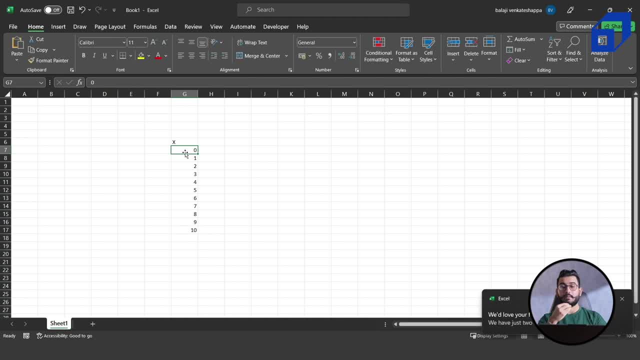 What is the meaning of 1, 0?? That basically means a person was not able to make any correct hit. So if the person was trying for 10 times, he was not able to hit. for any time The number of successful hits was zero. What is the meaning of 1?? 1 basically means when the person was trying to. 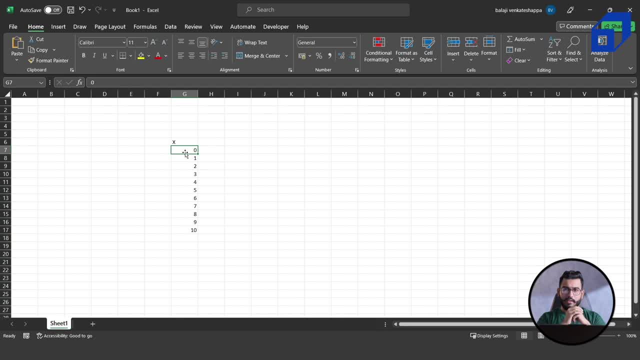 hit for 10 times, or maybe shooting for 10 times. he was able to hit the target only for one time. So that's what my X is. I'm now interested in calculating. the probability of X is equal to XI. So let's do that. We will use the formula, the combination formula. So combine is the 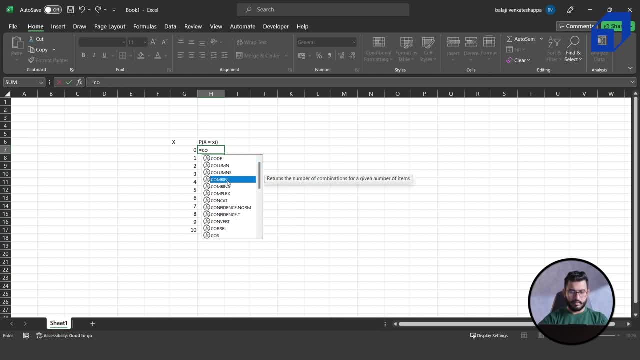 function that we have in Excel, And the total number of trials are 10.. X is this multiplied by so NC? Probably, probability of success was 0.4,. want four to the power of X. point four with the power of X. 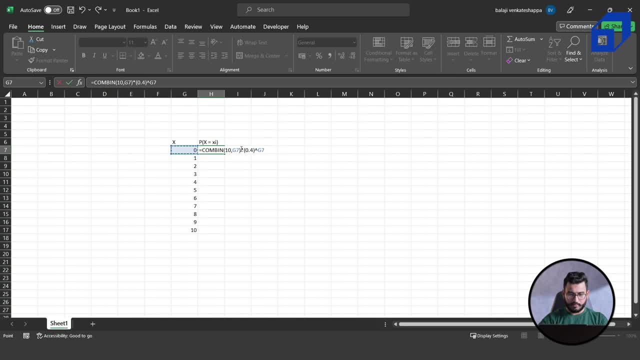 And I would put this in idea, so that nothing is getting wrong. And this is multiplied by failure, So Q, So 0.6 to the power of X, to the power of n minus x, So 10 minus x, and I close the bracket and I think everything is fine. 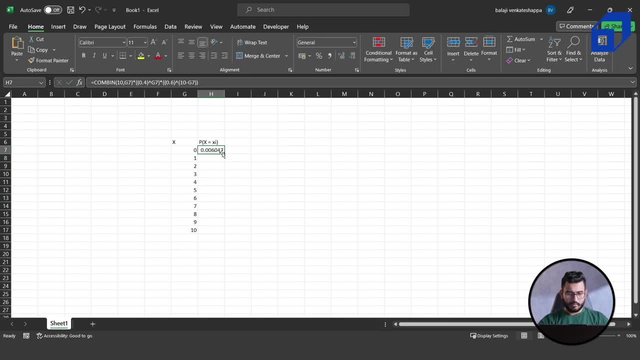 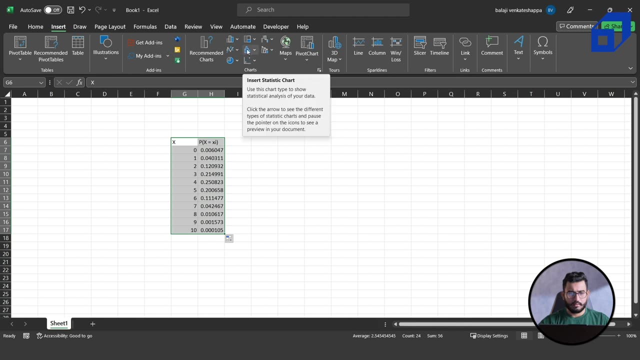 Let's expand this formula. I have the probabilities, Now let's plot it. So I'll go to insert: I'll choose a chart, maybe a column chart, And here we have the probability, which is wrong. Actually, it is plotted very wrong. 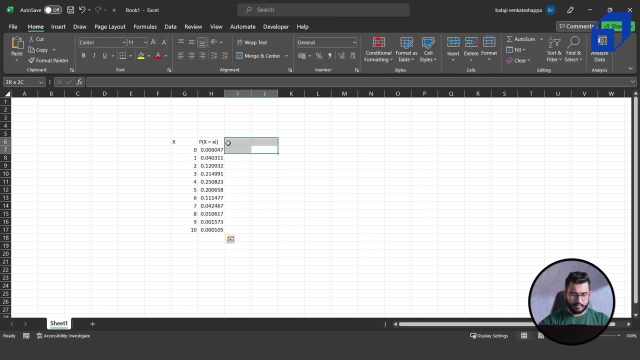 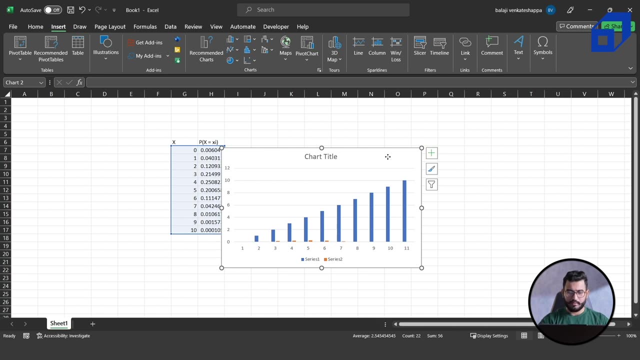 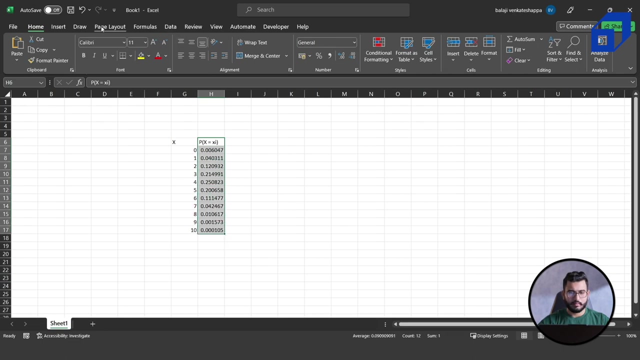 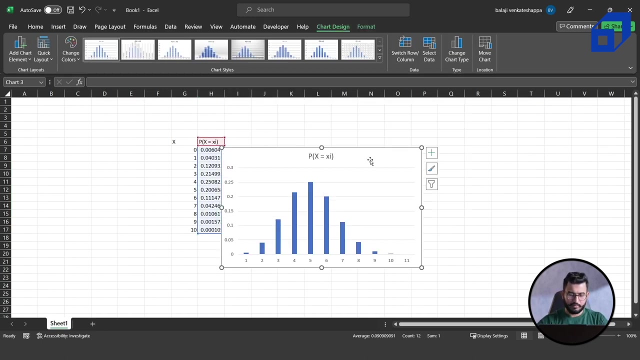 I should choose only. I think, if I choose this also, Let me try it for one more time. Otherwise we have to manually do it. Okay, that is not coming correctly, So let's choose only this. So this one insert and this chart Now here. first of all, this is not 1, this will be 0. 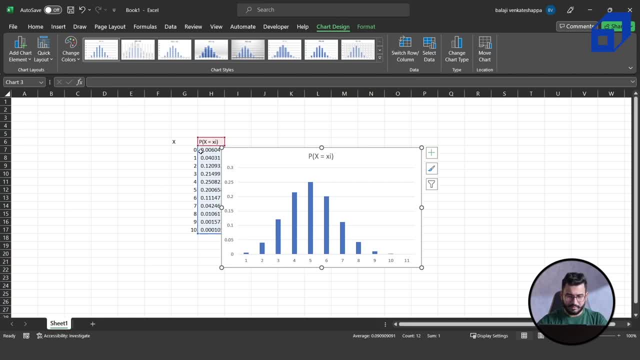 This will be 1 because we haven't selected the x, So assume this is 0. Then this is 1, and so on. Now you can see that the probability that a person will hit for 4 times is highest. 4 times is highest And here you can see in the result. 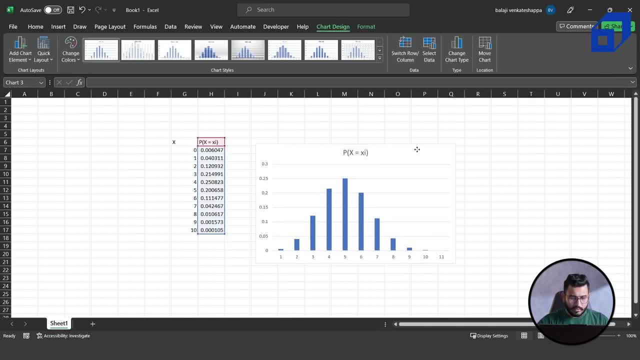 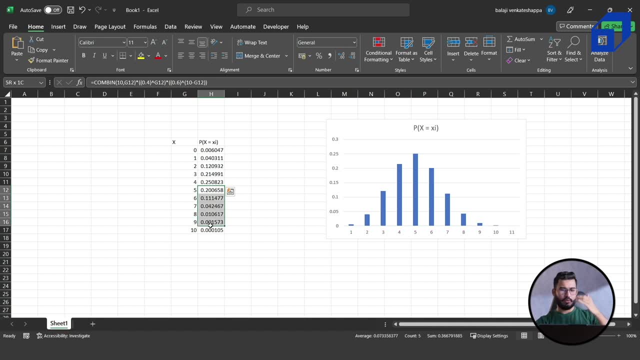 also that the person hitting the target for four times is highest. And then as we move forward it becomes lower and lower and lower. And if I go below four, it is becoming lower and lower and lower. So, using the probability mass function of any discrete random variable, 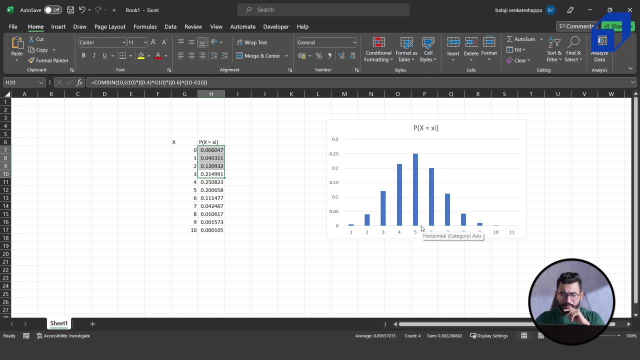 we can answer a lot of questions. So if I ask you, what is the probability that the person will be able to hit, or the person will be able to make at least five, at least five correct hits or at least five successful hits. So at least five means I'm interested. 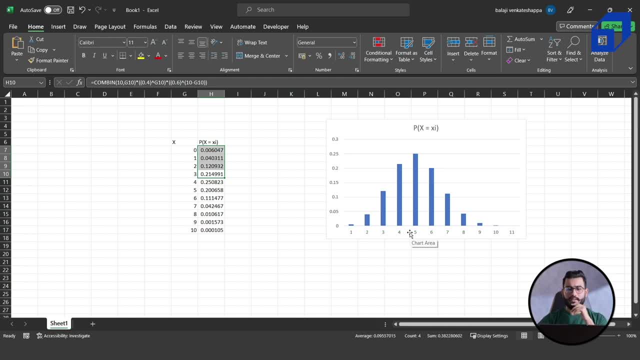 in the probability of X greater than or equal to five, which basically means- I'll just simply take the summation of all these probabilities, which is equal to 0.36.. So there are 36% chances that the person will hit at least four or five times. What is the probability that the person 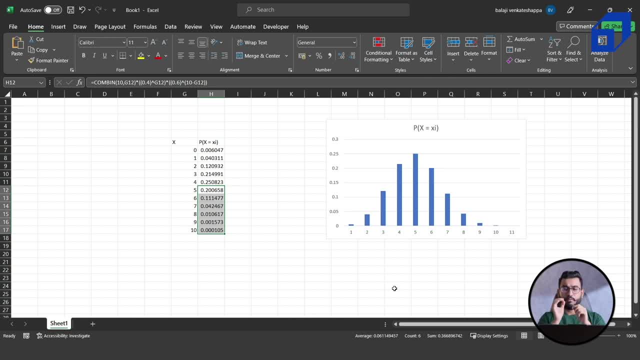 will be able to make the correct hit at most five times. at most means less than or equal to five, which basically means I'm interested in all these probabilities, which is 83%, which basically means the person will be able to make at most five correct hits 83% of the time Right now, using this. 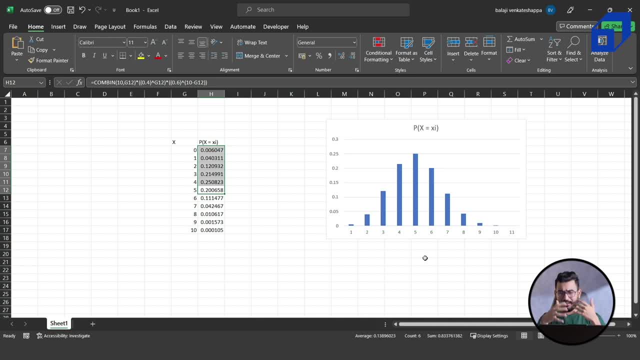 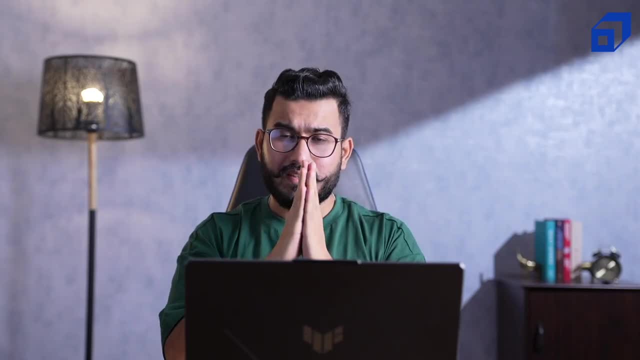 of various distribution, various discrete random variables. we can answer a lot of questions right, And that is the reason these distributions are created, but we are interested in one such distribution, That is the. I would say that is a very important distribution. 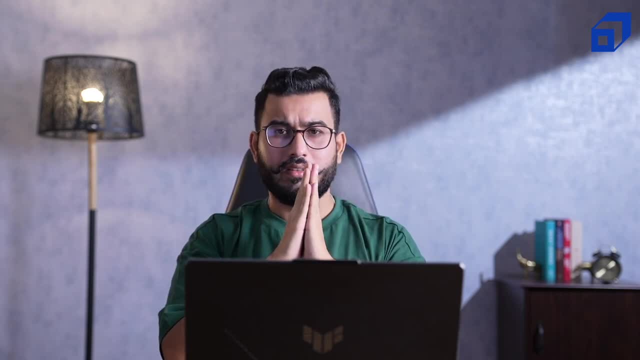 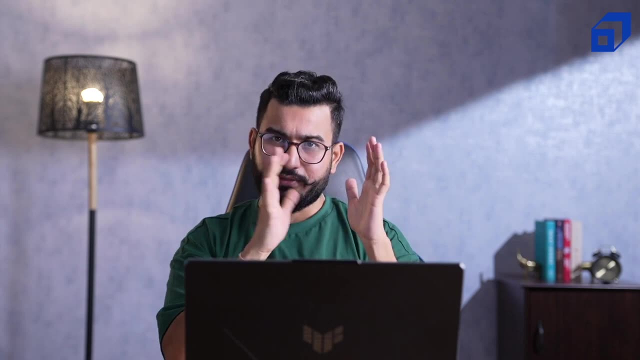 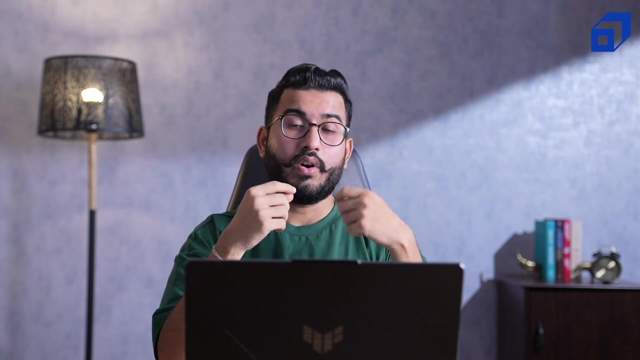 in the entire statistics and entire machine learning that is known as the normal distribution, which comes under the continuous random variable. So we have completed a discussion around a discrete random variable, under which we talked about Bernoulli experiment and the Bernoulli distribution, then binomial experiment and the binomial distribution, And this is the 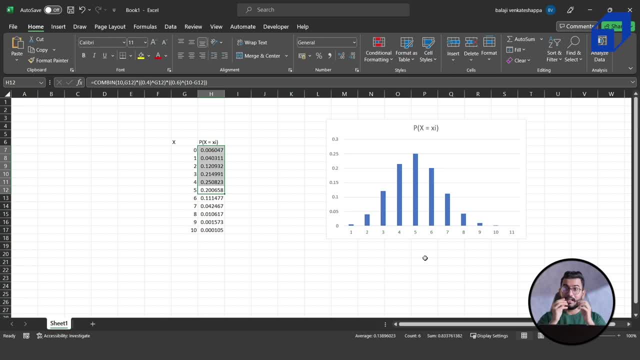 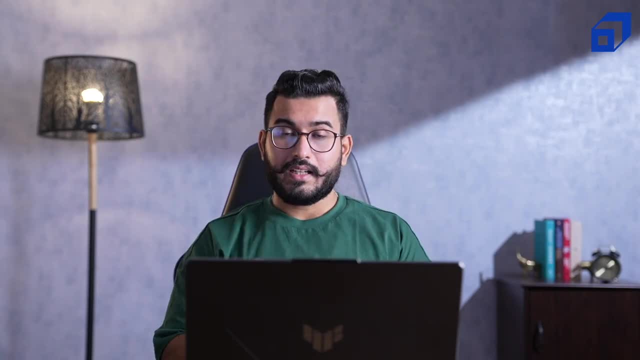 binomial distribution. Now let's talk about the continuous random variable, And within that, the most important distribution is normal distribution. If you guys are targeting for any data science job- and you have to- you have to attend your interview for the data science field. 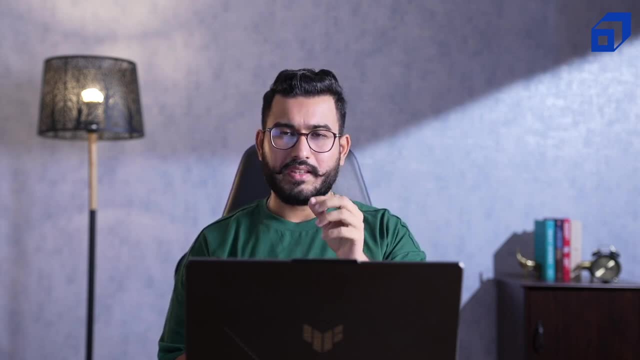 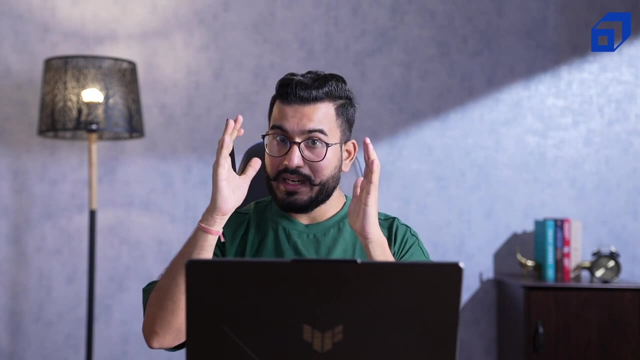 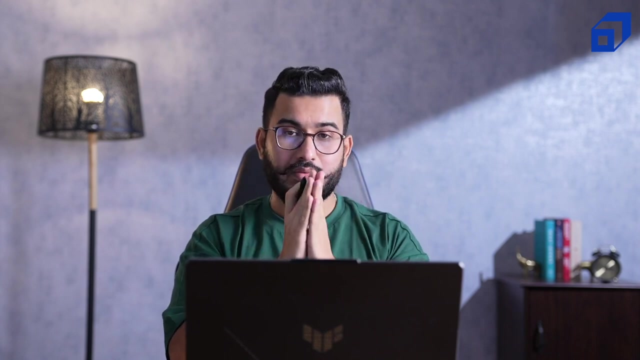 then this topic is one such topic that you will a hundred percent find out in your interview. It can be in any way, but it will be around this topic. So please listen to me very carefully, because this is really important when when it comes to data science interviews. So when it 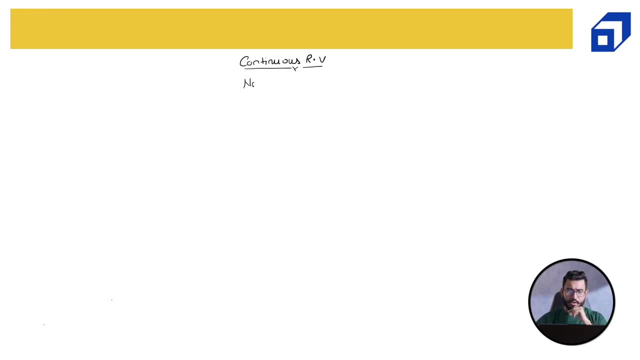 comes to continuous random variable, we have a distribution known as the normal distribution, And normal distribution is something that looks like a bell shaped curve, something like this. Now, what is the meaning of this? So if I, if I assume that the X axis represents our income, 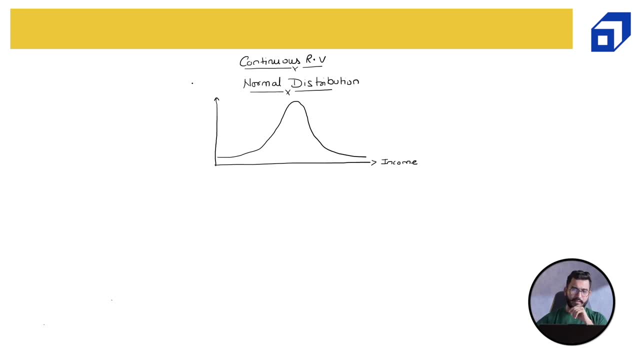 and the Y axis represents the count or the probability, then within this distribution we have a bell shaped curve. So if I assume that the X axis represents income and the Y axis represents the count or the probability, then within this distribution, within this range, within this range I have highest number or the highest occurrence of the. 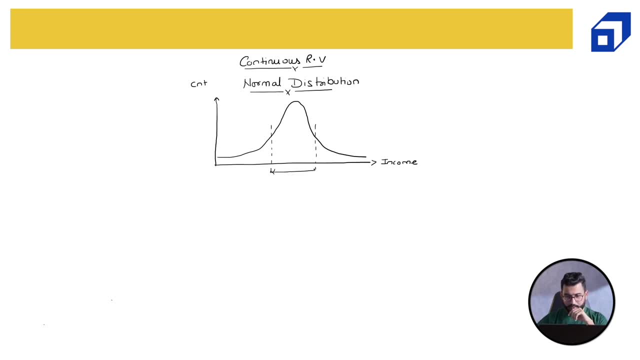 observations. So I have maximum number of people in the, in the mid range, in the mid income range. This is known as the center of my distribution. Now, what I have drawn right now is a normal distribution, but in reality it's just a normal distribution. So I have a maximum number of people. 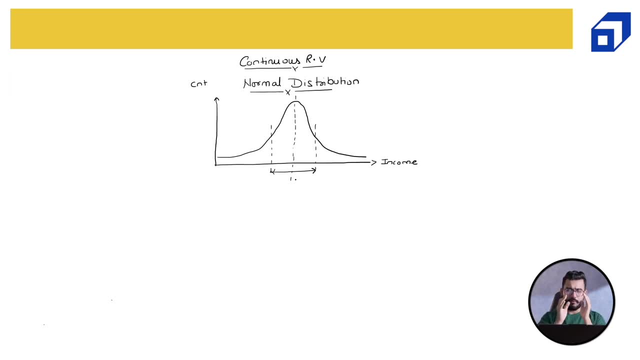 in the middle range And then within this, schwbucks fans- is a normal distribution. So I am essentially drawing that the past year on right, basically right, from my distribution, arius shift, and then you are just going to be one of the six today. So in reality, normal. 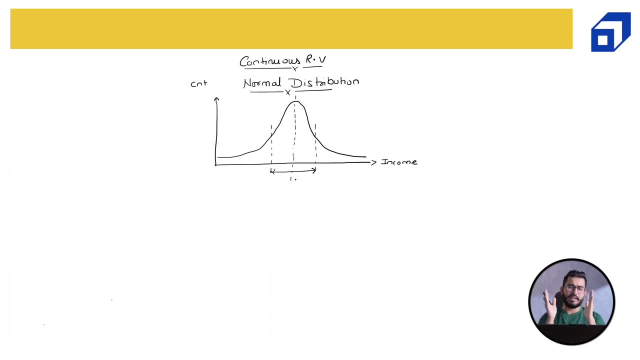 distributions can be of variety of shapes. creatives with commemorative count and arrays. as of now you can see it as a very symmetrical shape, But in reality you might get a very symmetrical shape of a normal distribution or you might not get. So in order to understand, 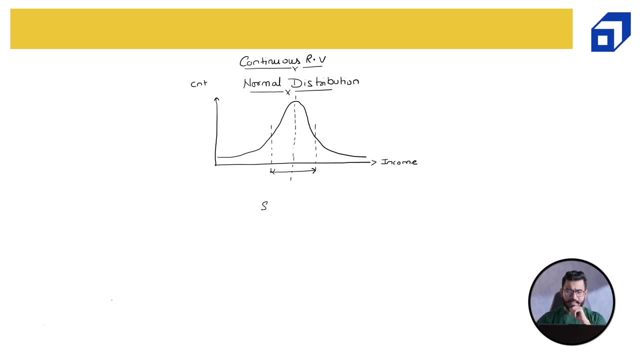 whether your data is following our normal distribution or not. we have something known as Jez quan difficult difference between both Storeroll and the data science aurait distribution. now why we have a standard normal distribution. a standard normal distribution will help you to compare few properties in your original data. so let's first of all type, let's 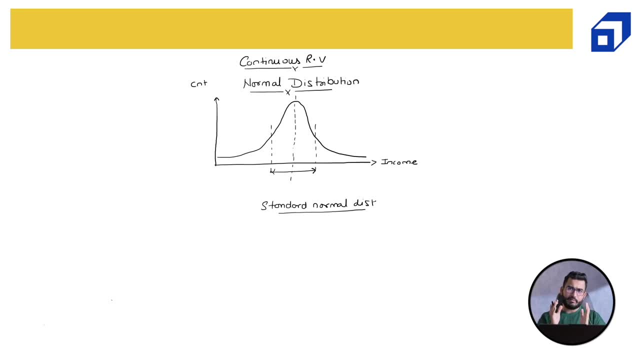 first of all understand what is a standard normal distribution, what are the properties of standard normal distribution, and then we will try to compare our data with the standard normal distribution to generate some insights. let's try to understand the standard normal distribution now. here I'm having a particular standard normal distribution, the advantage of standard normal. 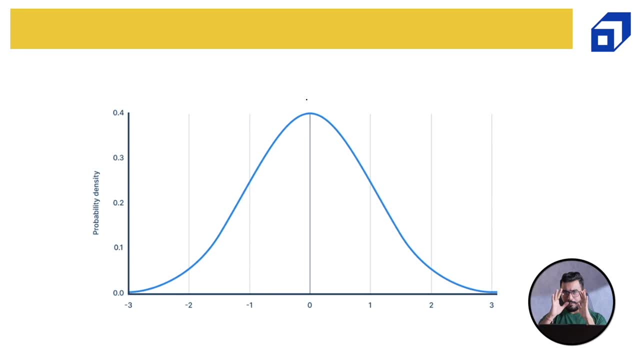 distribution is that it is perfectly symmetrical, which basically means: this is my Center, this is my center or this is my professional level, this is my percentage. protects means ours, is our data, our distance is exactly the same as ours. so now, if I prove my scale in my x and x and reading it, 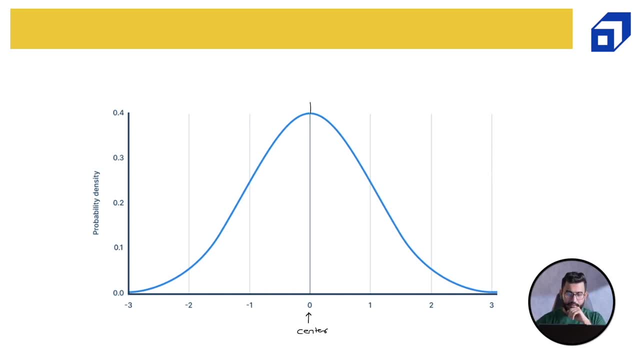 center, which basically means this is having the mean. this is my mean point. So mean, median and mode, all the three quantities fall in the center. I'm having 50% data below this, 50% data above this. So it is perfectly symmetrical. half here in the left side. 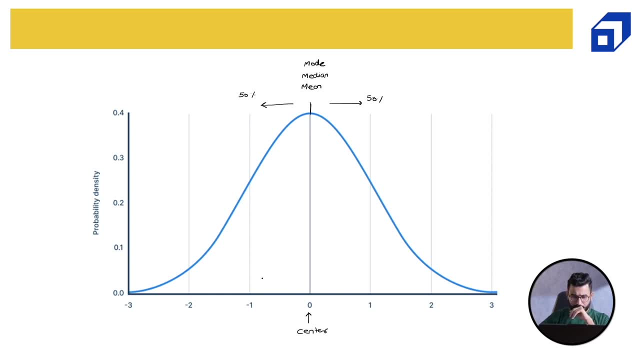 half here in the right side. Now the numbers you look into the X axis are known as the Z scale. We will talk more about it. Don't worry, I will explain you everything. What is Z scale? How we got these numbers? Don't worry, As of now, just try to understand what is the standard normal. 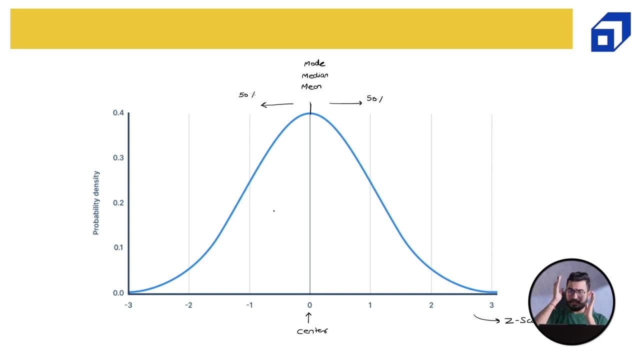 distribution. So number one is the mean is the mean and the median and the mode. all these three properties lies in the center. It is perfectly symmetrical. Okay, 50% on the left, 50% on the right, which basically means 50% data is on the left, 50% data is. 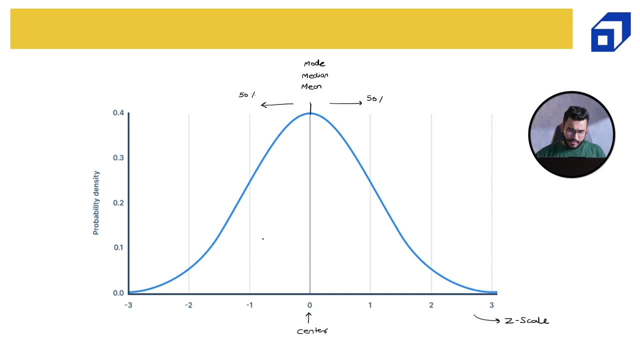 on the right. According to the standard normal distribution distribution property, 68% of the data lies between plus minus one standard deviation, 95% data lies between plus minus two standard deviation and 99.7% data lies between plus minus three standard deviation. 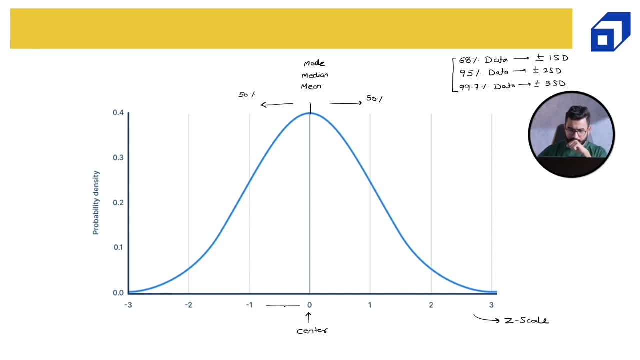 Now, what is this? This is one standard deviation, one standard deviation below, one standard deviation above. So between these two points, I'm having 68% of the data. between these two points, I'm having 95% of the data Right. 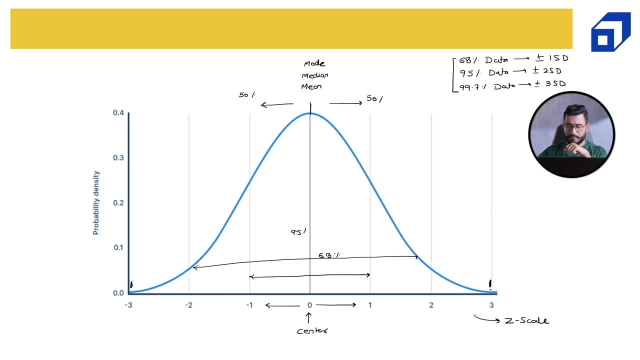 Okay, between these two points, from this point to this point, I'm having 99.7% data. If you're not able to understand how I obtained the Z scale and what I'm talking about- 68,, 95,, 97,- let's try to understand it with a real example. First of all, let's try to understand. 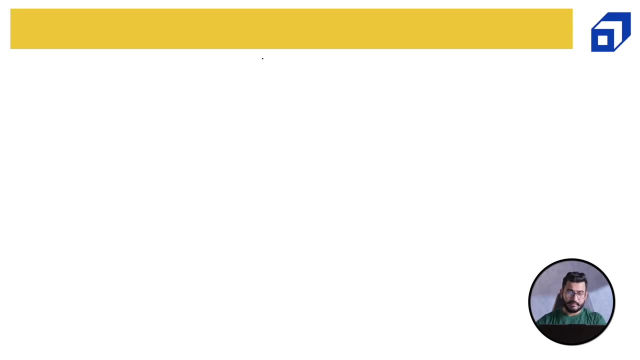 the Z scale. So what is Z scale? For this, we have to jump into the topic of scaling. Scaling Now, don't worry, We have a topic which we are talking about, which is normal distributions. We have talked about a standard normal distribution. We have looked into some. 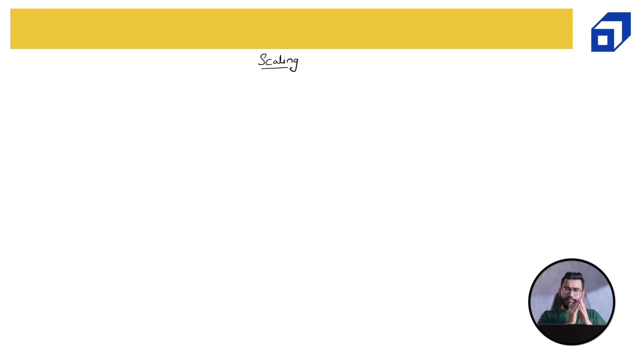 of the properties. but there is one confusion. The confusion is what is Z scale and what, how we have obtained these numbers and what is one? is standard deviation below one standard deviation above? So we will pause this topic as of now, just. 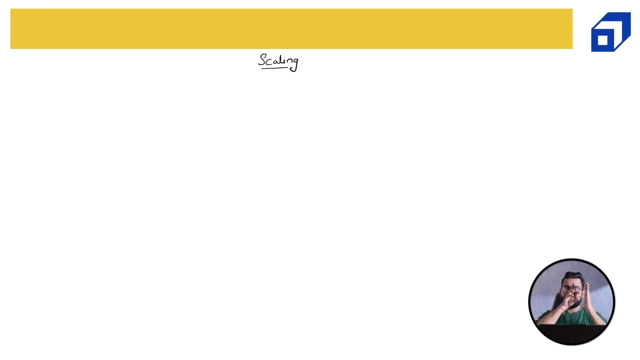 just create a barrier over here. We'll try to understand this as small topic, which is scaling and the Z scale. Once we are understood, when we are clear with this, then we will bind everything and you will be very much clear. So stay with me for another 10 minutes and you will be clear with everything. 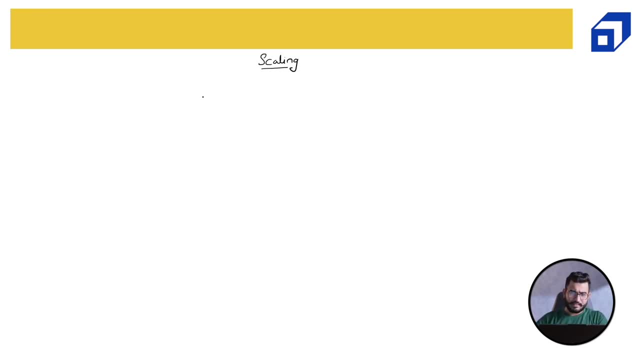 So what is scaling? Now the problem is: let's say I'm having two variables: age and income. Let's say age is a person is having age of 27 and income of Thousand dollars, something like that. Now can I compare these two values? 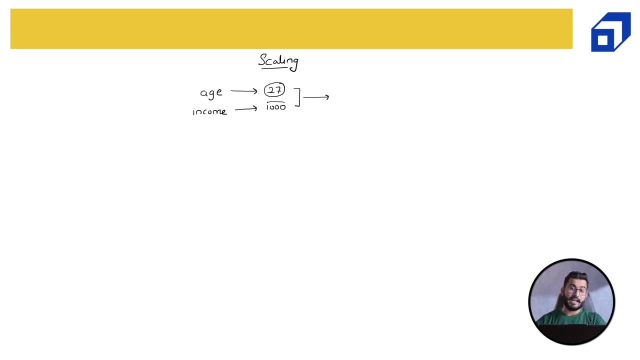 Can I say this is a very low value and this is a very high value? No, essentially we can not Why? Because both of them are having a different scale. Age isn't. the age is in the scale of year, while income is in the scale of dollars. So I can not compare these two values. They belong to. 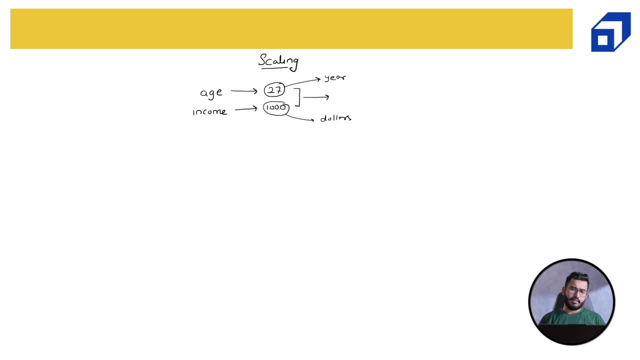 two different scales and we can not compare them, Right? But what if I want to compare them, then we have to make them into a common scale, right? And that is what scaling is known as. So scaling is a process of converting the data into one common scale. 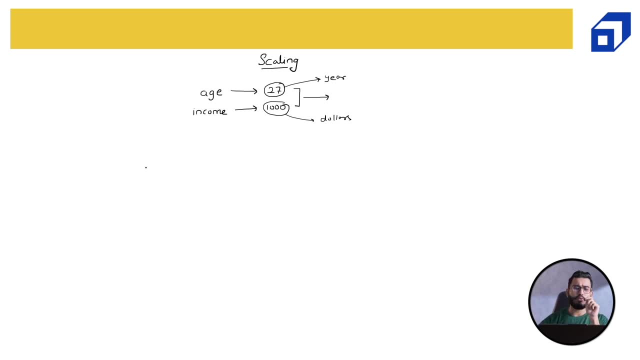 using which I can compare various values. There are two common approach which we fall in scaling. One is known as the min max scaling, also known as the normalization Scaling. The second one is known as the standardization of the Z scaling. The Z scaling. 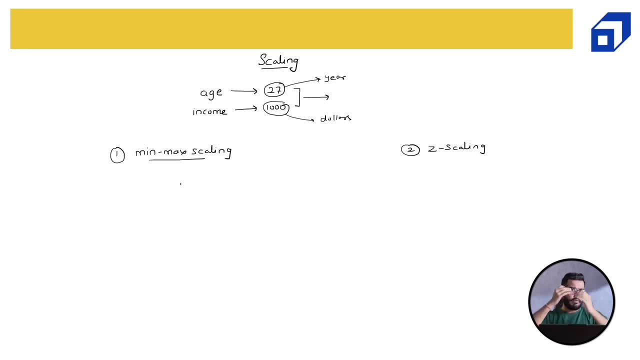 in the min max scaling I tried to con convert the complete data into a scale of zero to one. Their minimum is zero, Maximum is one. The formula is very simple: X minus Min divided by Max minus Min. I'll show you. I'll show the show you the example in: 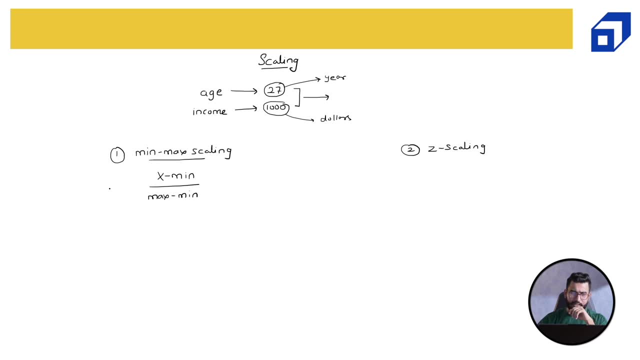 as of now. just look into the formula, where X is the value I want to convert. So X is the value we want to transform or convert. Now here, Z in Z scaling. the formula is X minus standard division, sorry, X minus mean. divided by Sigma. What is X? X is the value we want to convert value. 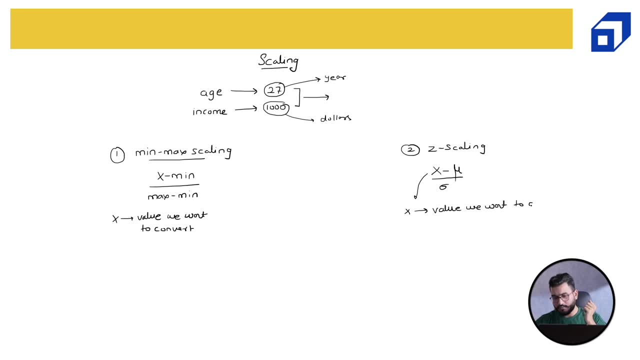 We want to convert: Mu is the mean of the column mean of the variable and Sigma is the standard deviation of the variable. So we have this formula. Now let's try to apply this formula in the actual data in the Excel file to make sense out of it. 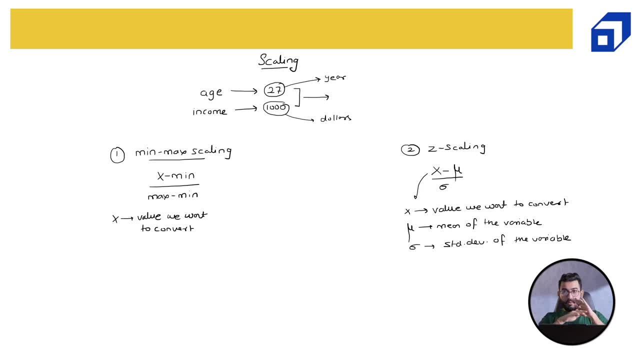 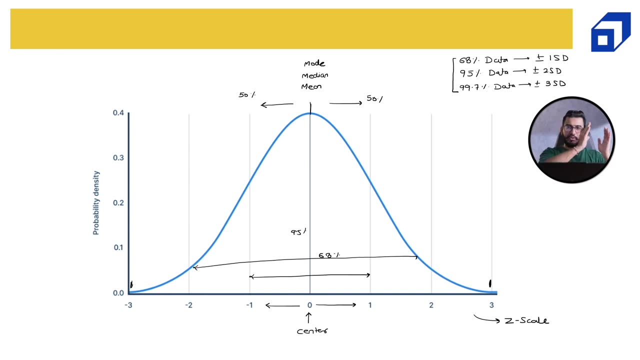 And then you guys will be very clear about how we obtained this Y axis. This is the major question. right, We have the normal distribution, a standard normal distribution topic parked As of now. we are trying to understand the scaling And the main question that we are trying to answer, right. 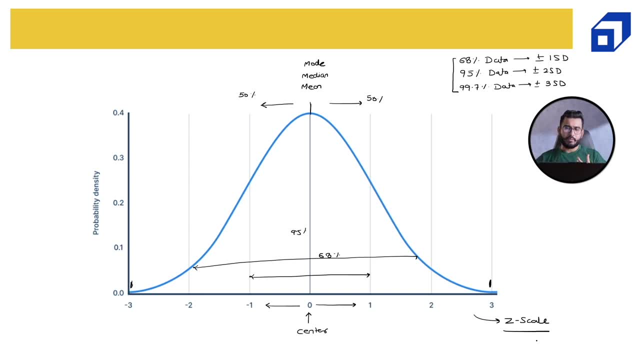 now is how this Z scale came into picture, And once we are clear with this, then this is standard normal distribution will make more sense to you, right? So keep this topic part. we are talking about this topic And now we are moving forward to understand the scaling topic. 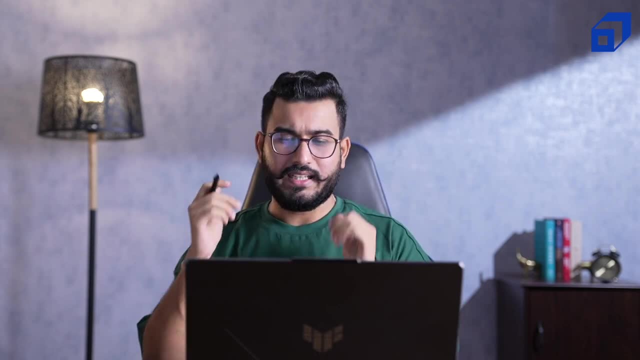 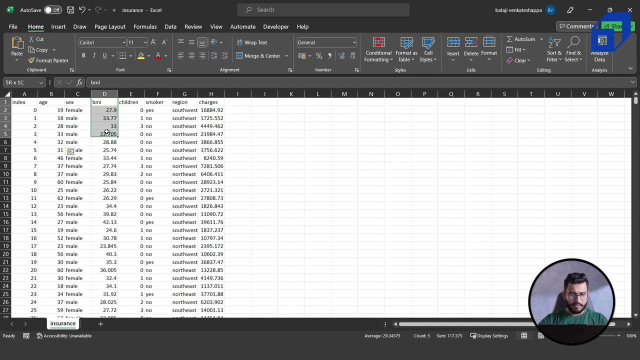 in Excel with particularly a data example. So let's do this Now. here you can see, we have a data which is having age, BMI and charges, the insurance charges. I cannot say that this value is very low. This value is middle and this value is very, very, very high. Why? Because age is in. 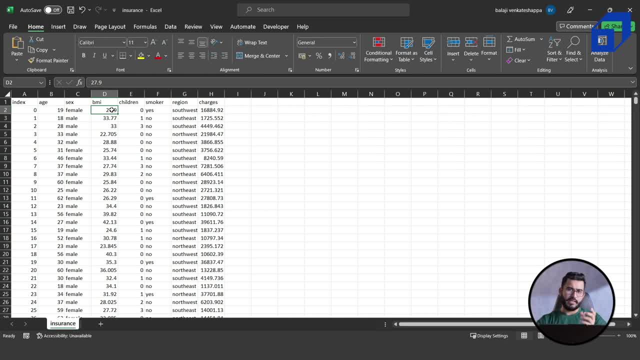 meter, BMI is in kg per meter square. if you know, BMI unit is kg per meter square and charges are in dollars. These all three are in different scale. I cannot compare them right. Let's try to use min max scaling. So for min max scaling I need the minimum value. So let me insert quickly some rows. 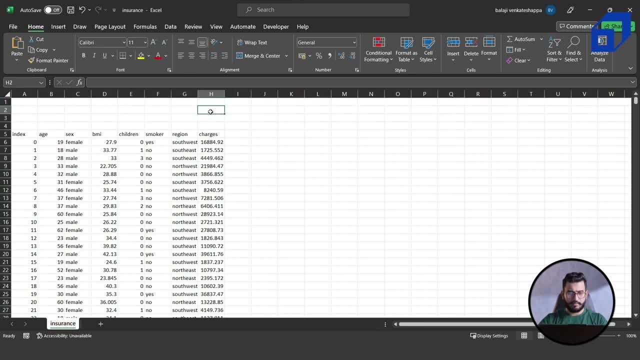 So let's say here I'm having minimum maximum, So I'm just calculating the minimum for age. oh sorry, is equal to minimum of the column age. So I'm having the minimum value to be 18, then calculate the maximum of the column age. 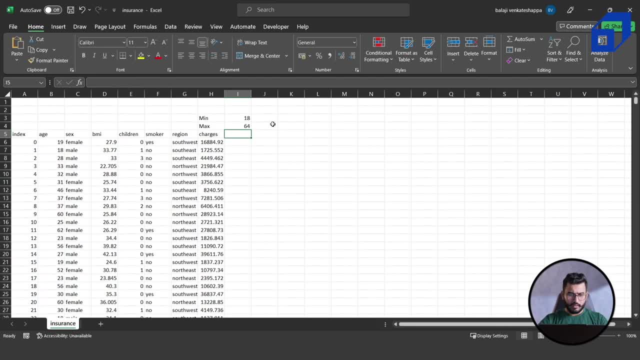 The maximum value is 64.. Similarly, I'll call this column as age- underscore normal. Similarly, I'll do it for BMI- BMI underscore normal. And then for charges- charge and underscore n. I'll just find out the. also, let's quickly do one thing. Let's. 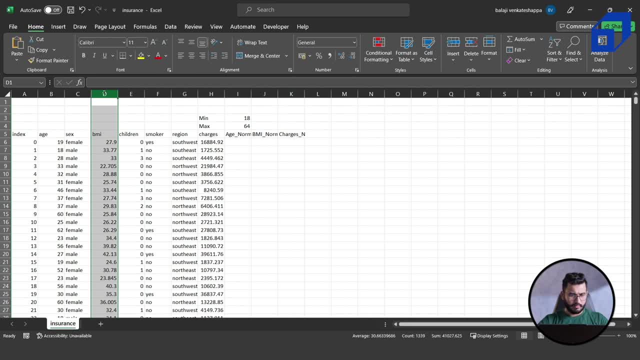 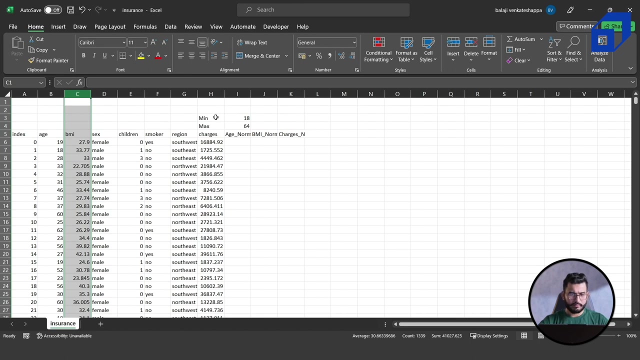 shift these columns And let's shift this column also. So let's see how it works, So that I can simply just extend the formula And I do not have to write it again and again. Now, if I just simply extend this formula, I get the minimum of age, BMI and charges, And this will give 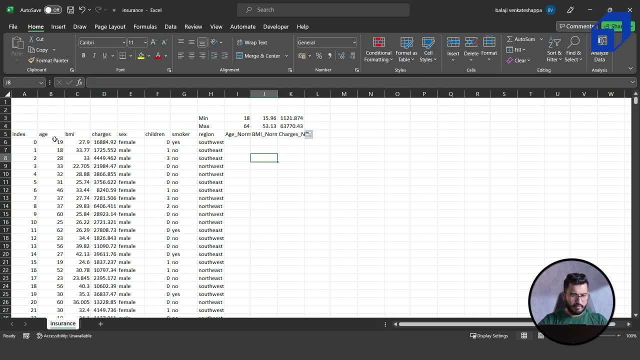 me the maximum of age, BMI and charges, because age, BMI and charges are one after the other. So I just extended the formula. right Now let's apply: the formula is equal to X, which is this value I want to convert, minus minimum, So I'll just freeze this value. So 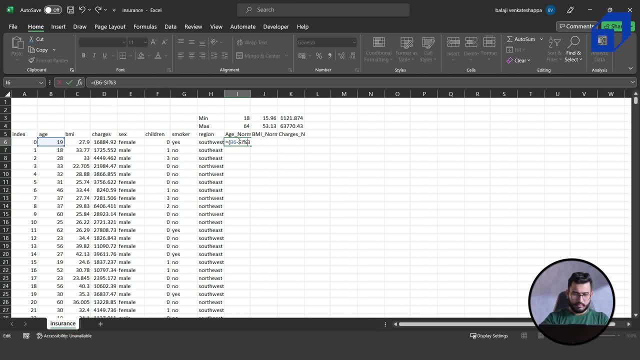 I won't. I will put a dollar X minus min, divided by the value max and then minus and then minimum, and I will. so let's do one thing: let's not freeze I, so that if I extend the formula, this is not getting fixated. I'll just fix the row $4 and 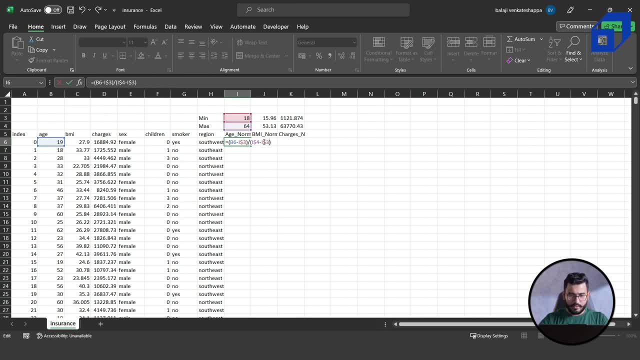 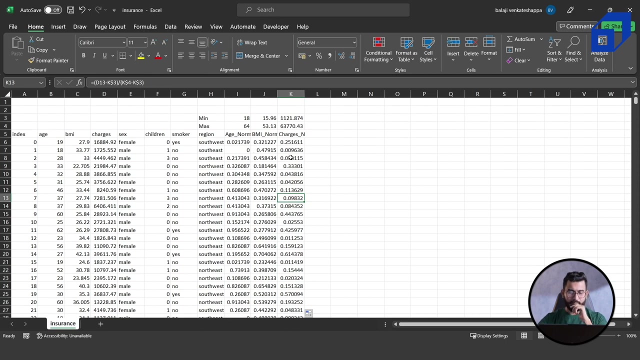 $3 and let's enter, let's try to apply it on the entire column and let's try to extend it to PMI and charges also, and let's try to extend it to all the rows now. now, all these three columns are in a scale where minimum is 0, maximum is 1, so, as you that, 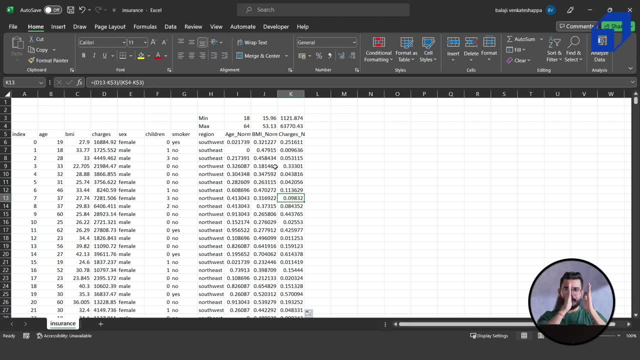 you have a number line. minimum is 0, maximum is 1. now the middle point will be 0.5, so the mean is 0.5. so any value which is close to 0, you can assume that the value is very low. any value which is close to 1, you can. 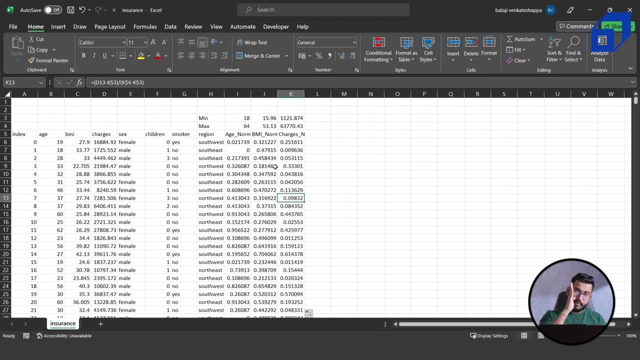 assume that the value is very high. any value which is bit around 0.5 is the average value. right now. the scale is very clean and all these three columns- age, BMI and charges- are now in this scale, the normalized scale. let's try to compare the value. if I look at this person, the age of 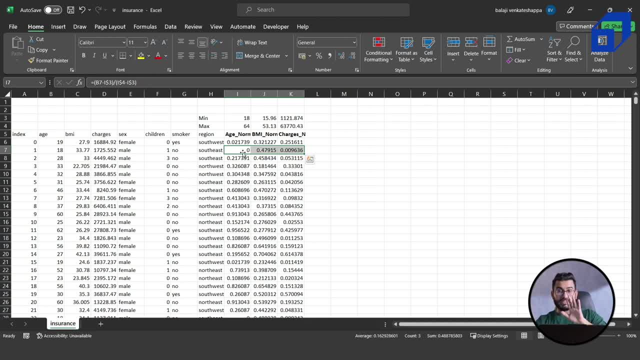 this person is 0, which basically means this person is. this person is the person who is having the lowest age. in my data, the age 0 means the person is having the lowest is the minimum age. then 0.47 is the BMI, which basically means the BMI is around. 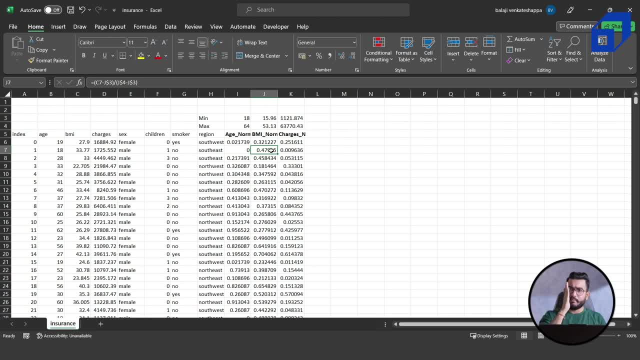 mean I told you 0.5 is the middle, 0.47 is near to 0.5 rise. so BMI is around average, while the charges to zero. right, so what i can conclude for this person? this person is a young person, very young, having average bmi and very low charges. right, let's take one more person, let's say this person. 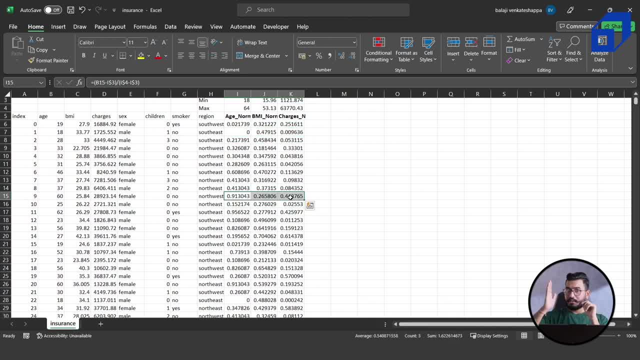 the age is 0.91, which is close to one. right 0.91 is close to one, so age is 0.91. bmi is 0.26, close to one, 0.1, so 0.26. and then charges are 0.4, which is close to the middle value. so if i 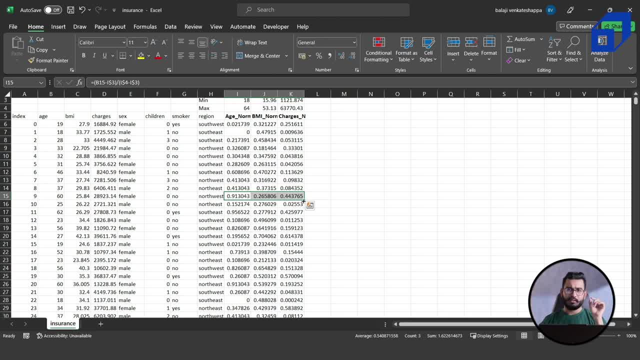 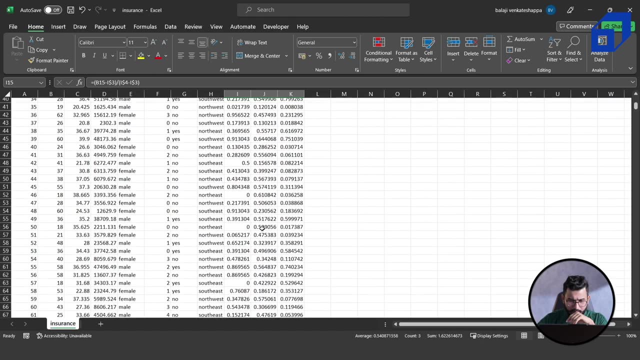 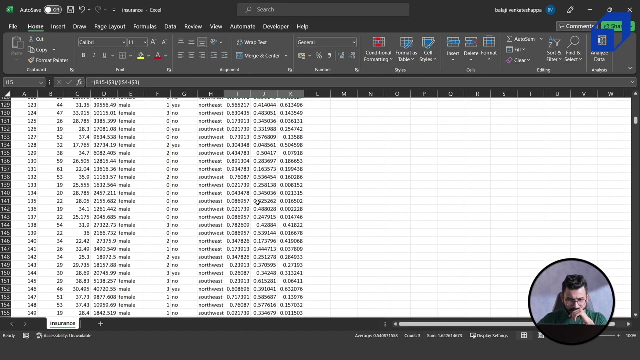 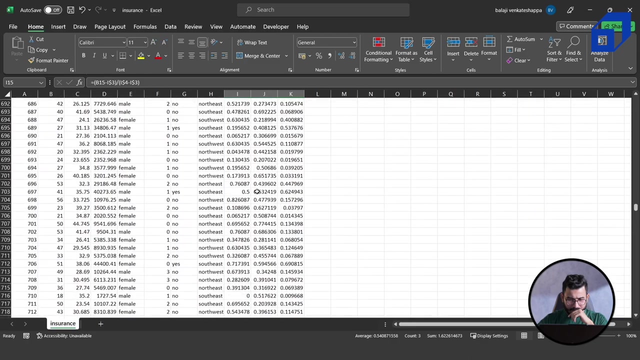 talk about this person. this person is having very high age, uh, not very high bm, so bmi is below average, but charges are around average, right? uh, let's talk about a person who can be a outlier. say something. let's see if i can find out some interesting value so that it makes some real sense. 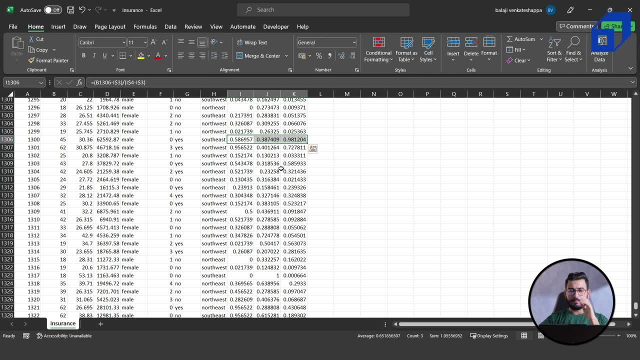 okay, if i look at this person, this person is having 0.5 as age middle age. the bmi is for this person is below average, but the charges are very high for this person. you can see this person right. so i hope now you guys are able to understand how to read values in a normal scale, normal means. 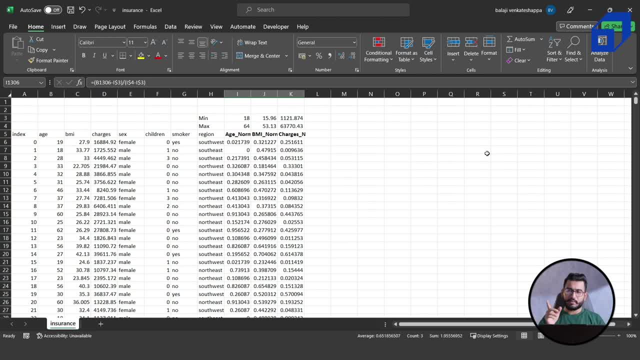 minimum is zero, maximum is one and the formula is x minus min divided by max minus min. in the z scaling, which is a standardization, we need the average, we need the standard deviation and once i do this, let's do this first of all. so this will be my 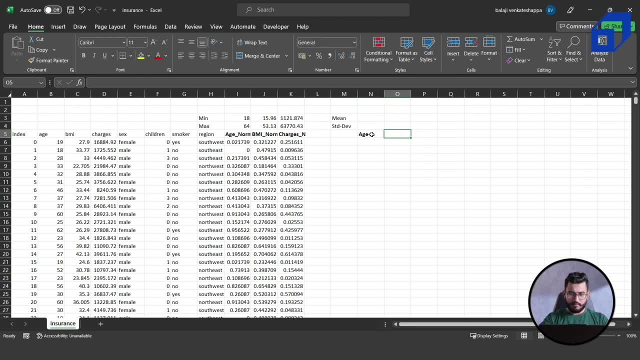 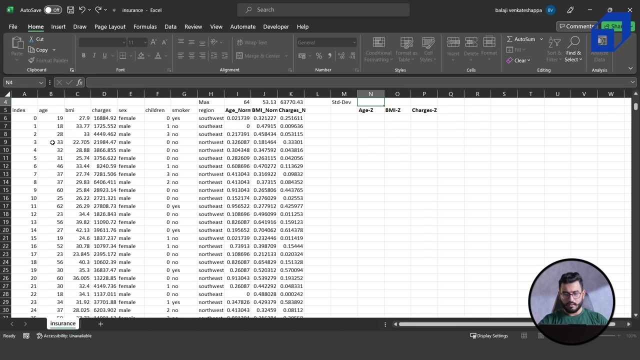 age hyphen z, and this will be my bmi- hyphen z and then charges hyphen z. now let's apply. the formula is equal to, so first of all we have to calculate the mean. so is equal to average. i need average of the age column. i will just extend this formula. 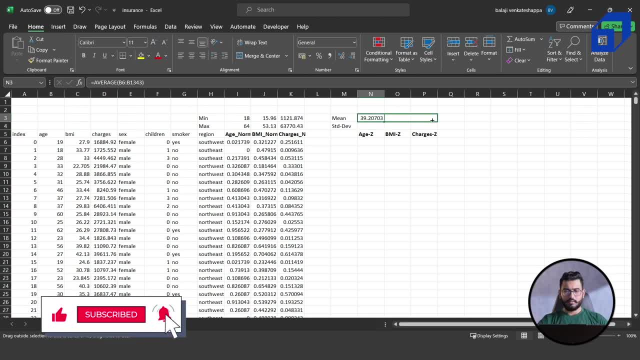 to the next cell, next two cells. then i need the standard deviation. so i'll just use this standard deviation of the bmi h column. then i will extend this to the next cell and now we will apply. the formula is equal to x minus mean, so x minus mean, and i will again just freeze the row x minus mean. 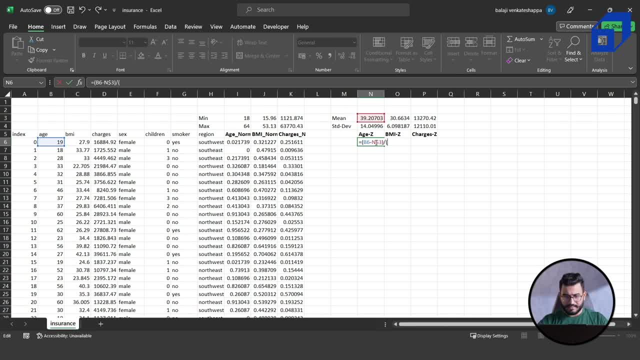 and divided by standard deviation. this is my standard deviation. i will freeze the row and enter. now let's extend it to all the rows. i don't know why it's not happening. let me try it one more time, okay? i don't know why it's not happening, so i have to do it manually. 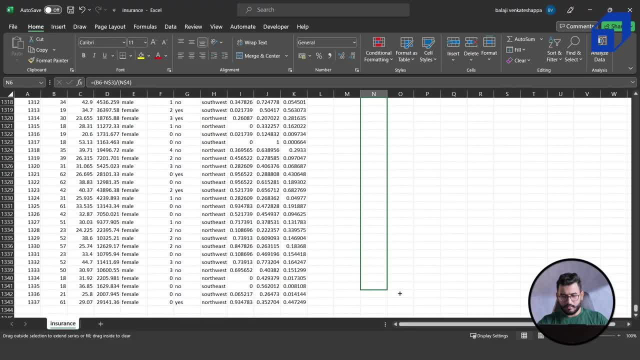 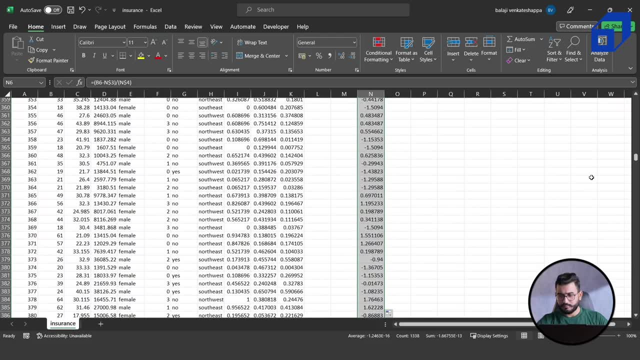 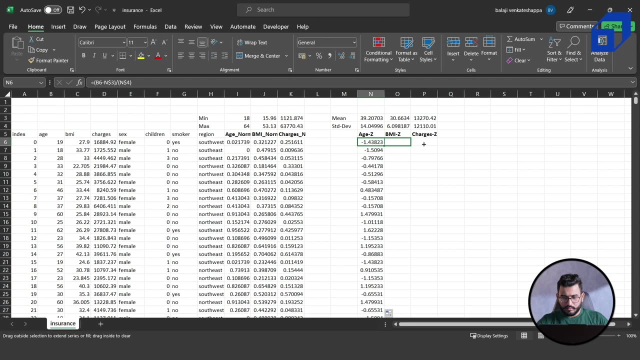 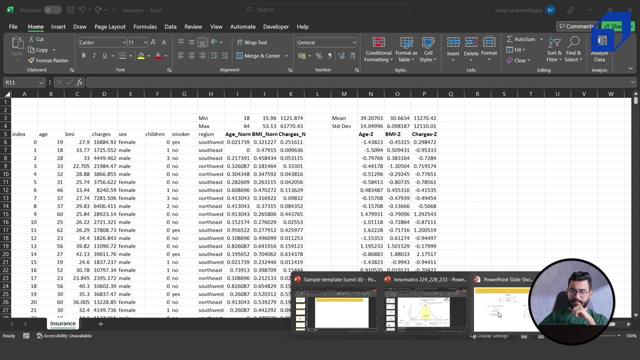 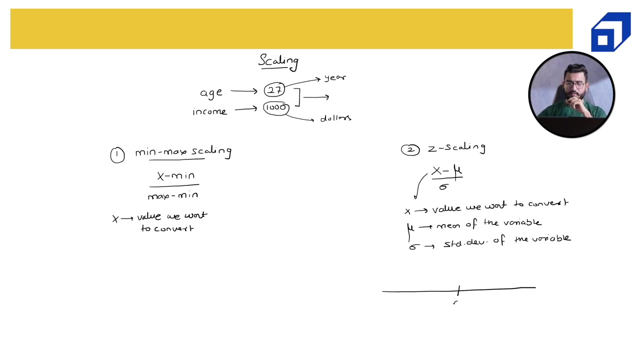 and then i will extend this formula to the next column also. so let's do it like this, and this one also. okay, now in the z scale. so what we can do here is this: the z point is in the z scaling, my middle point is zero, then i'm having minus 1, minus 2 over here, plus 1 plus 2 and plus 3 over here. 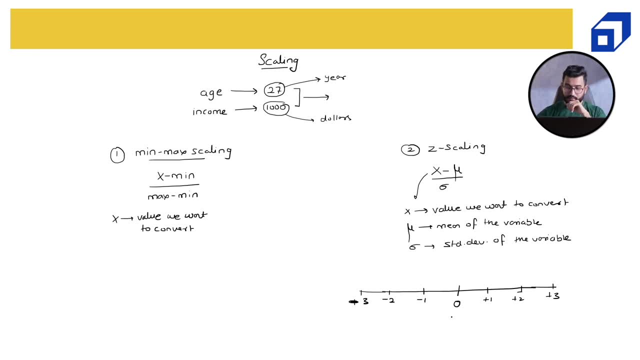 and minus 3 over here. what is these values? what are these values? these are known as my standard deviation. this is my mean, or Z scaling will convert your data in such a way that now the data is having a mean of zero and the standard deviation of one. So if you get a value close to zero, that basically means you. 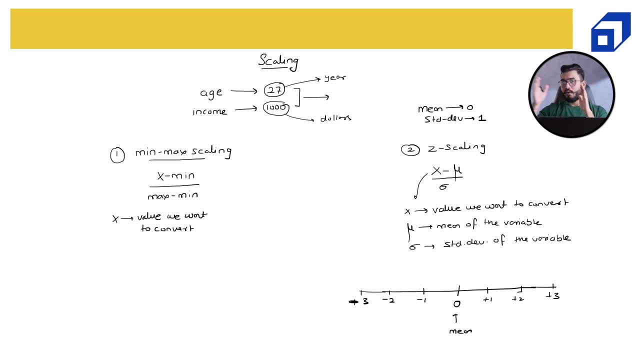 are an average. If you go on the positive side you are moving above average and the higher you move, that many standard deviations you are above the average. So let's say the value is plus 1.2, which basically means you are one standard deviation above the average. If let's say the 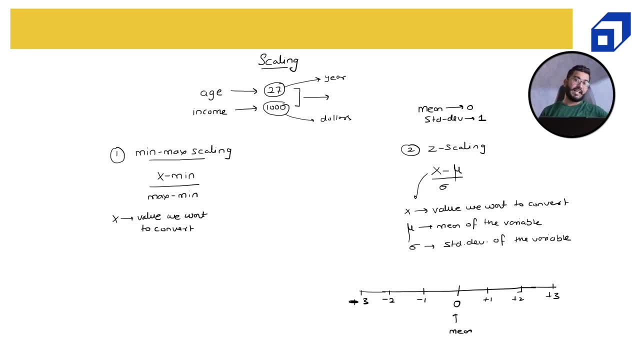 value is minus three. that basically means you are three standard deviations below the average. So Z scaling will convert your complete data into a scale where the center becomes zero, the mean becomes zero and the standard deviation becomes one unit. one unit on either side. 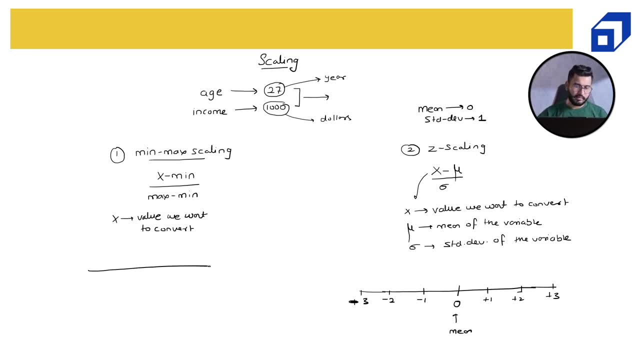 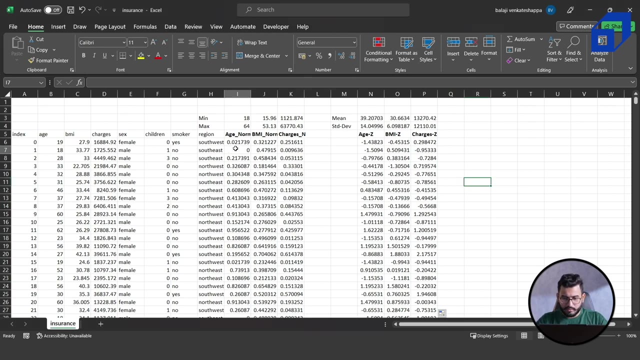 For min max scaling. it was something like this: zero, one and middle is 0.5.. Let's quickly compare it and try to check the Z scale. So here, if I look into this person, this person is having BMI of 0.5.. 0.5 means very close to zero, right? So zero is the middle, 0.5 is very close to zero. 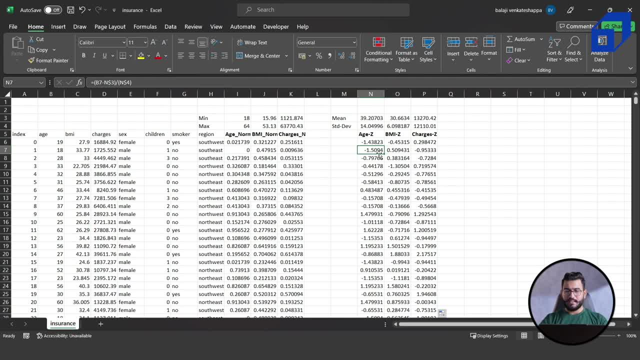 Then minus 1.5 is the age, which basically means from zero, the person is 1.5 standard deviation below the mean. Then minus 0.9 charges from the mean, the person is 0.9 standard deviation below the mean. So this person is having normal BMI because the value is close to zero, very low. 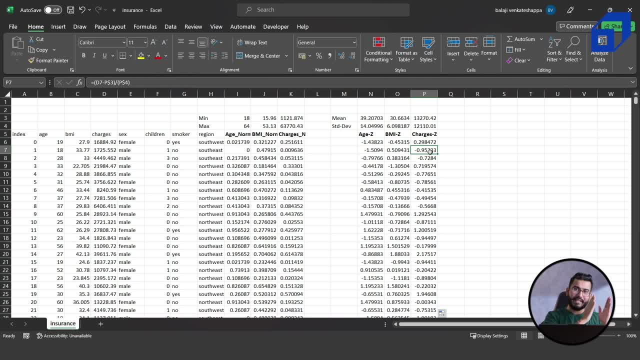 age and very low charges, because both the values are on the negative side. So you can see that with standardization, since I'm having positive negative sign and middle is zero, it becomes very easy for interpretation. If the value is positive- I know this is above average. 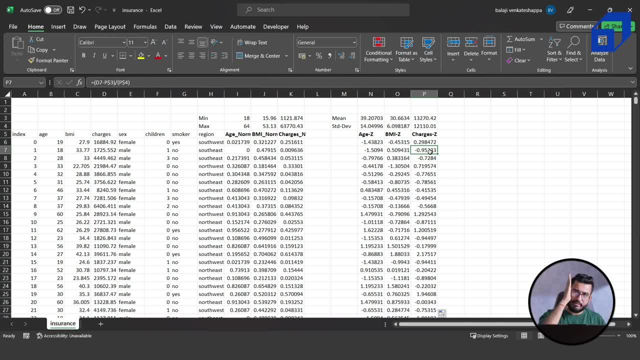 If the value is negative- I know this is below average- The value is positive, which basically means it is close to zero. That is the advantage of standardization. Now, this is the Z scale which you guys can find out in my standard normal distribution. 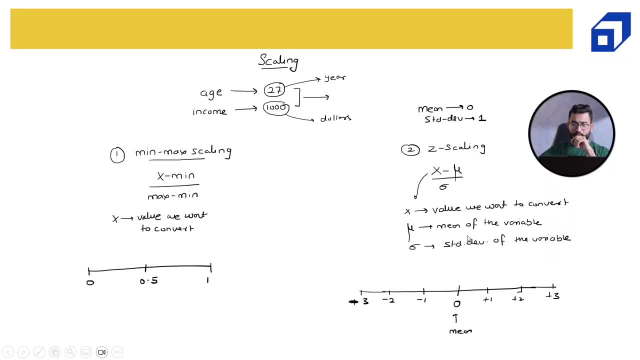 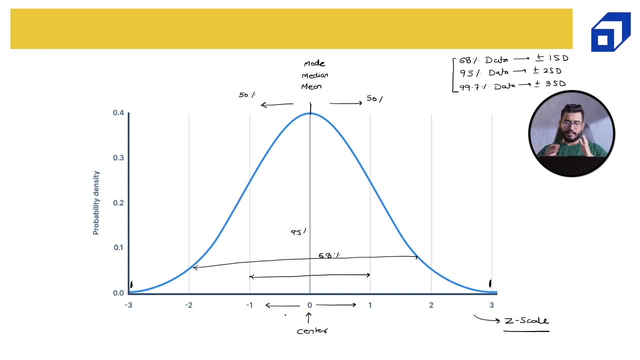 So if I go back to my standard normal distribution, I can see that I have a standard normal distribution. This is what the Z scale is. So the middle is zero. I have one standard deviation below the mean, one standard deviation above the mean, and so on. Now, according, 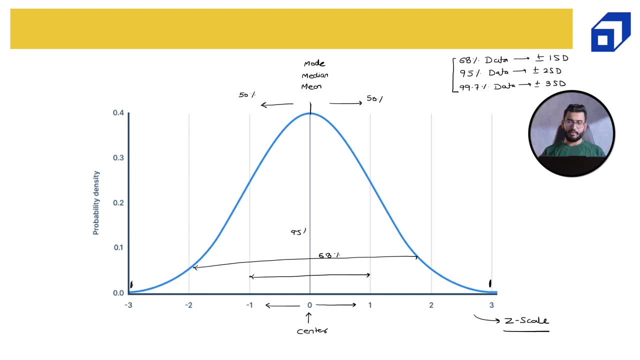 to the property of a standard normal distribution. it states that 68% of the data is plus minus one standard deviation above or below the mean. 95% data is plus minus two standard deviation. 99.7% data is plus minus. 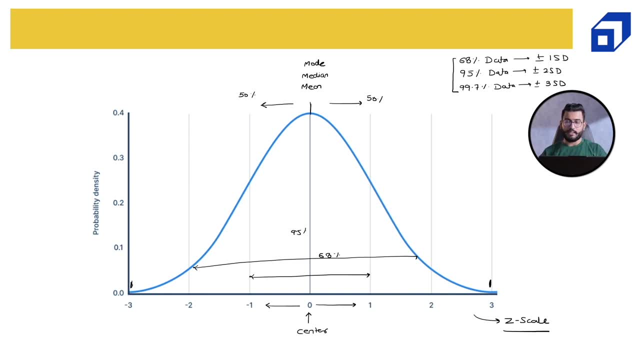 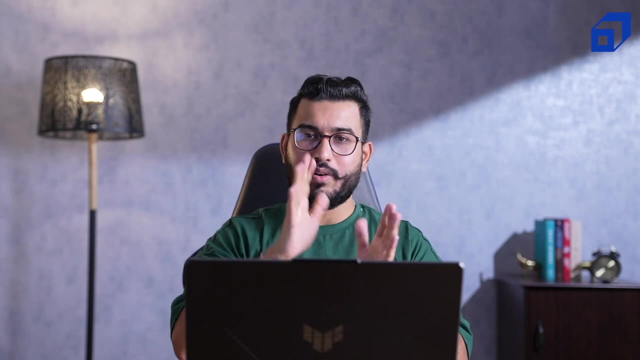 Let's try to quickly prove it. For that, first of all, we have to check which particular column among each BMI in charges follow normal distribution. So I already know that BMI follows a normal distribution, which basically means when I plot it it would resemble a. 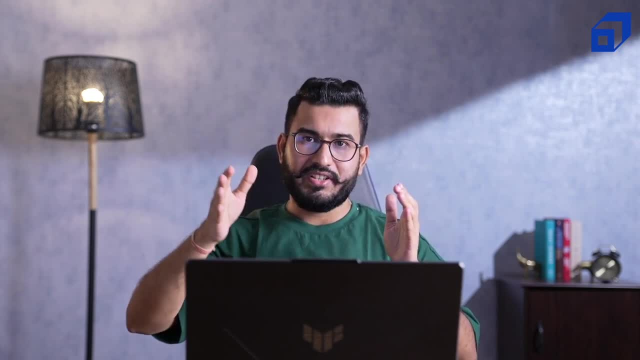 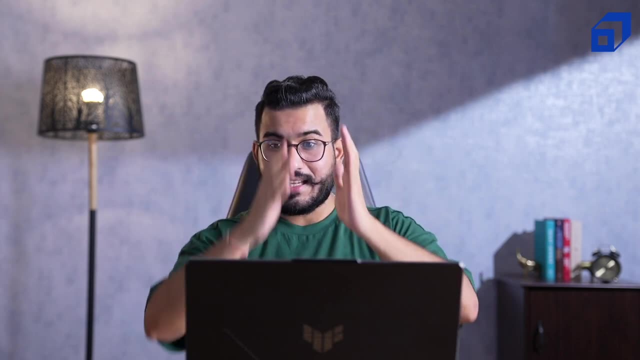 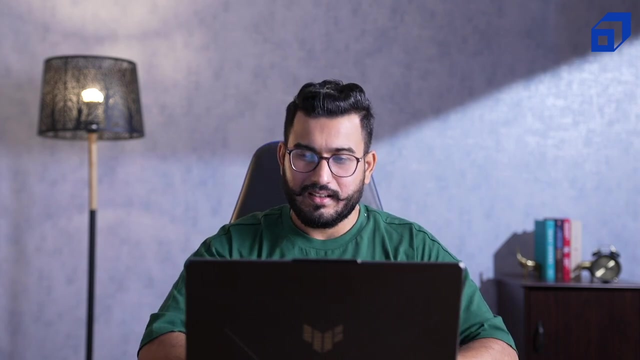 normal curve, a bell-shaped curve which is symmetrical. You will get half data from below the center and half data above the center. and since I have converted the BMI column completely into a Z scale or standard scale- now just see the magic- I have selected the BMI column. 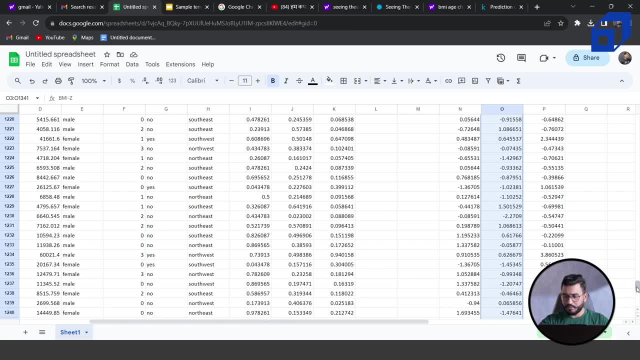 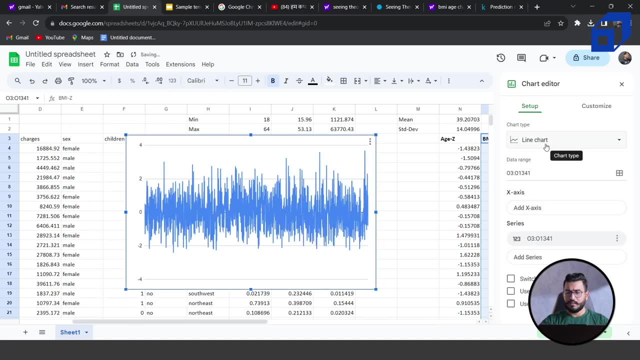 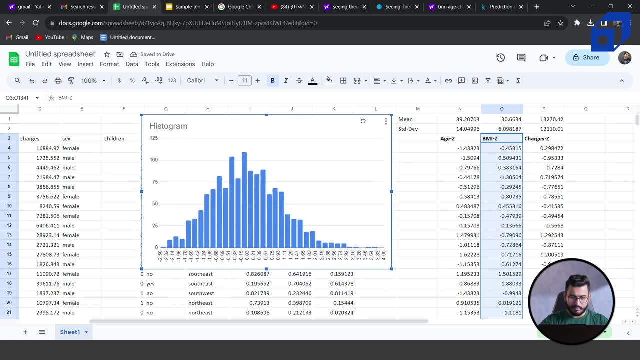 and now we will go to the insert option in this Google sheets, go to chart and we will select the histogram. now, if you closely observe this histogram, you can see that this point is the center: 0.00 point 0, 3 is the center and below this value I am having negative points above. 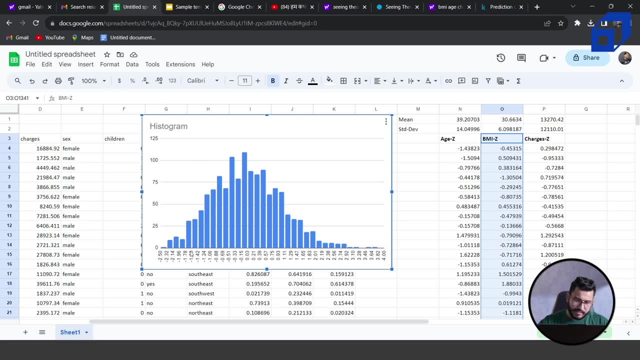 this value. I am having positive points. now you can see that the data is spread around minus 2 standard deviation, which basically means below it will. it is distributed to standard deviation below the mean and for standard divisions above the mean. now you can. you can see that it is not perfectly distributed to standard deviation below for a standard. 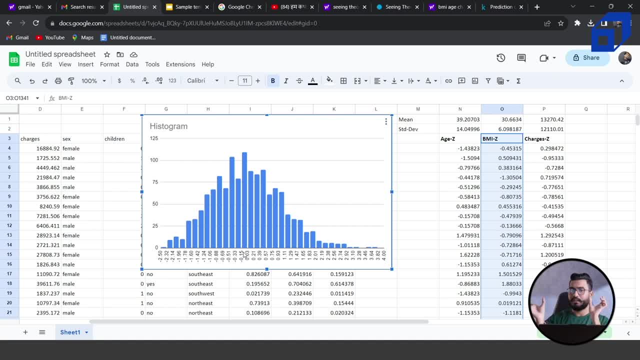 division above. so here I am having less data, here I am having more data, or the spread is more on this side, the positive side. this is one thing which can understand. this is a normal distribution, but this is not standard normal. so in order to you compare this distribution with something, we need a standard thing. right, let's say, if I have to, 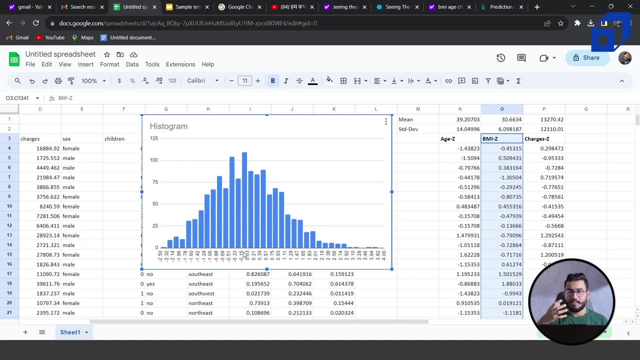 compare my performance in any exam, I need some standard score right. standard score is 100, so maximum is 100, the best is 100. so whenever we try to compare something, we need a standard right. similarly, in order to compare the distribution of a continuous random variable, which appears to be: 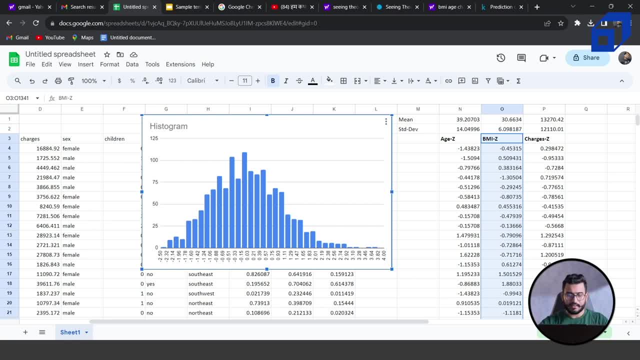 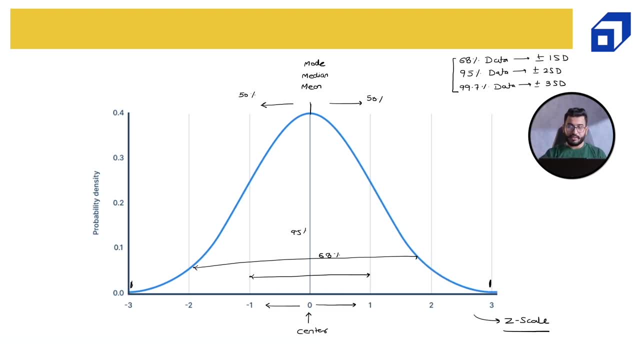 normal. I need a standard normal distribution and this is where my standard normal distribution comes into picture. this is my standard normal distribution. now, standard normal distribution says that your mean, median and mode will lie in the center. and if it is not lying in the center, if your mean is. 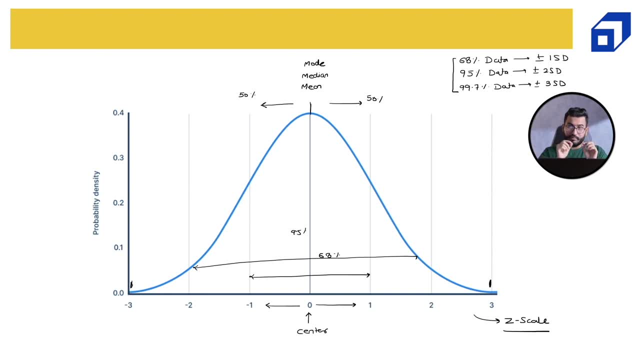 not equal to mode, is not equal to median. your distribution is not a standard, normal distribution. it will be either left skewed or right skewed. these are the two terms which I am introducing. I will explain that later you as we move forward, don't worry. but as of now we are trying to understand the properties of 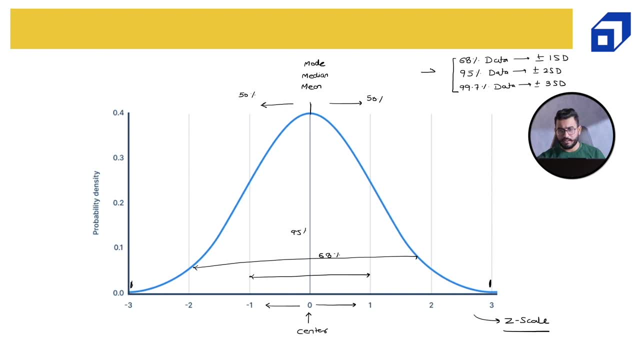 normal distribution, and here I have already written the three properties, which is 68% of the data lies across one mind plus minus one standard deviation above or below the mean. similarly, 95% to standard deviation above or below the mean and 99.7% data lies across plus. 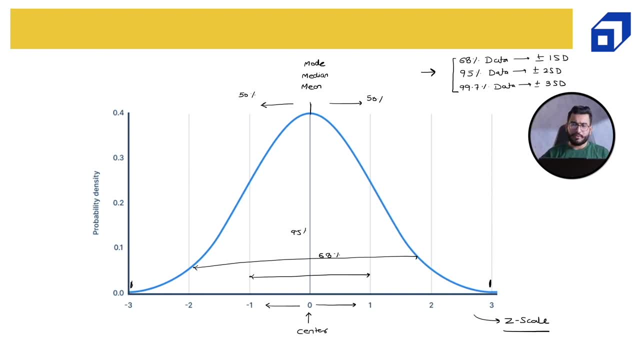 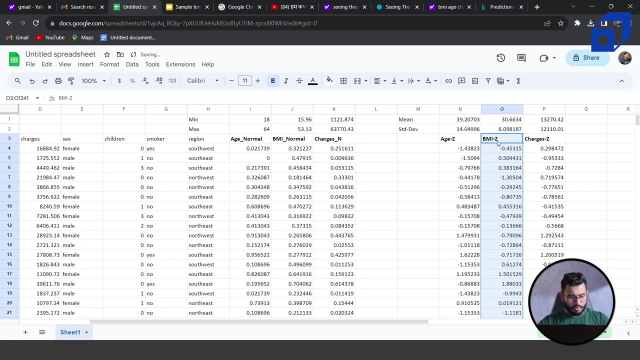 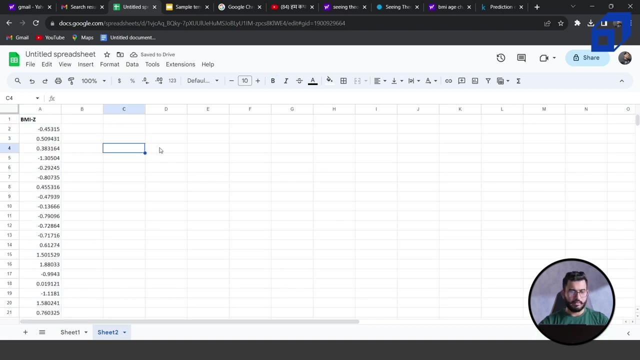 minus three standard deviation. right now, what we are going to do, we are going to quickly prove it. so here we have the data. I'll just quickly close this. I'll copy this data into a new sheet over here now. we will calculate the mean, median and mode and for simplicity purpose, let's not use 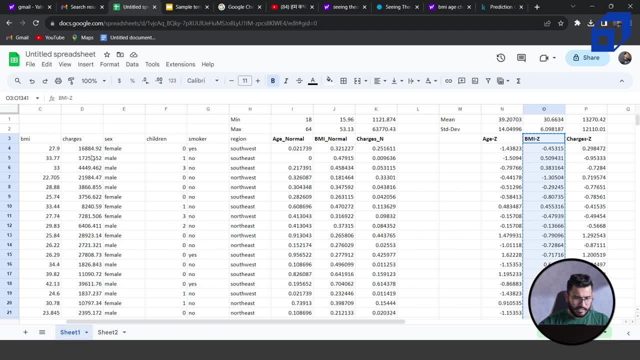 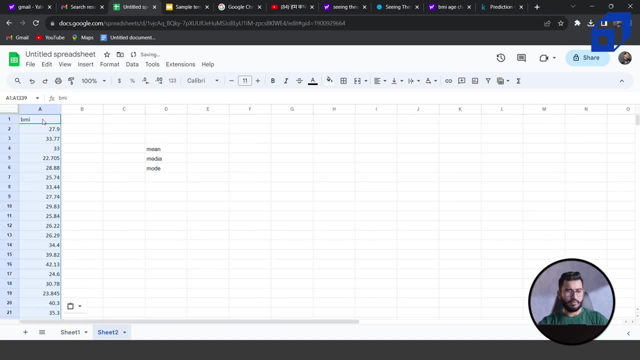 the Z scale. let's use the original scale so that you guys are able to understand this. so I'll just replace this column with the original data: BMI. what is the average? BMI is equal to average of this column. what is the median? so a medium is a median of this column and what are the modes and the mode of this column? and here I have a. 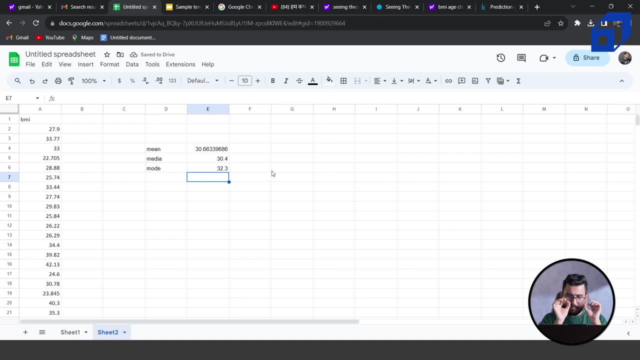 we have. So now you can see that mean is 30.6,, median is 30.4,, mode is 32.3.. These values are approximately close to each other, not exactly same. So first impression about this distribution is that it is not standard, normal distribution, but it's something close to standard, right. 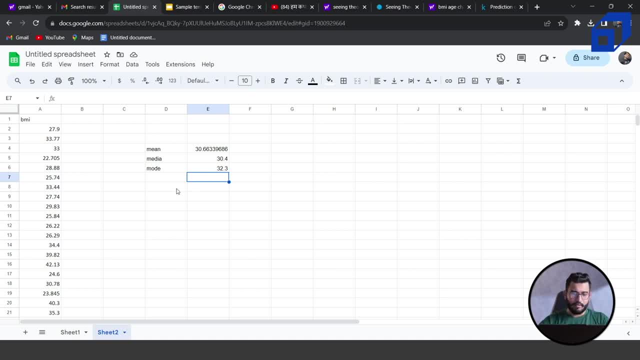 But how much close? Let's try to understand that. First we will prove the property. The property is that 68% of the data falls across, plus minus one standard deviation, right? So let's quickly find out the standard deviation. So STD DEF is equal to STD, So this is my standard deviation. 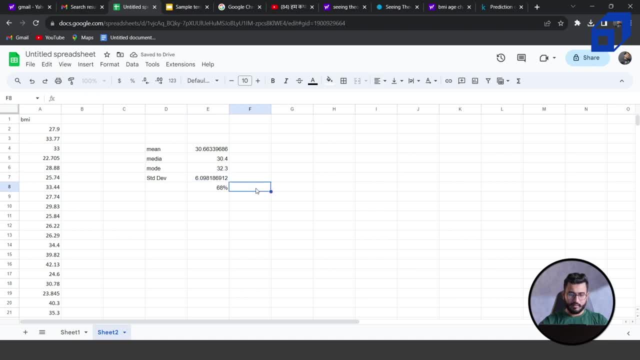 of this data It is 6.09 standard deviation If I go plus one standard deviation below the mean. so let me create a table over here: 68% I go. so this is my mean minus minus. let's say this is my lower limit, This is my upper limit. 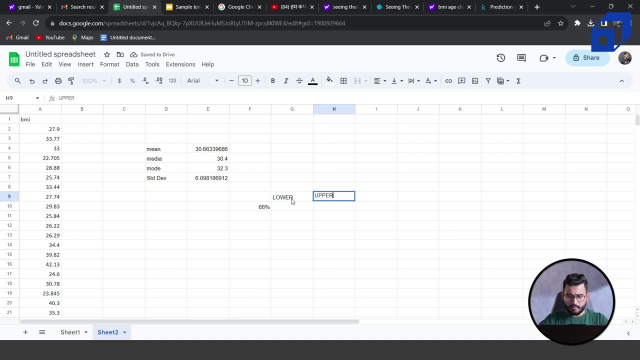 I'll explain you everything, Don't worry, Don't get overwhelmed. And this is my count. This is my total, And let's write 68% over here. And this is my total, And let's write 68% over here. 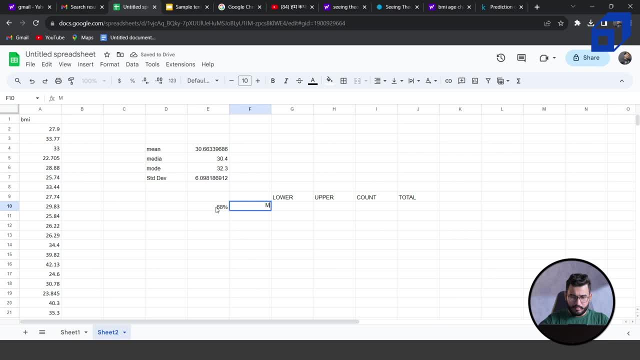 And this is mean. So one standard deviation. So now what we are going to do? we are going to take mean and subtract one standard deviation. So one standard deviation. So mean minus one standard deviation. The lower limit is 24.5.. Then mean plus one standard deviation. The upper limit is 36.. Now 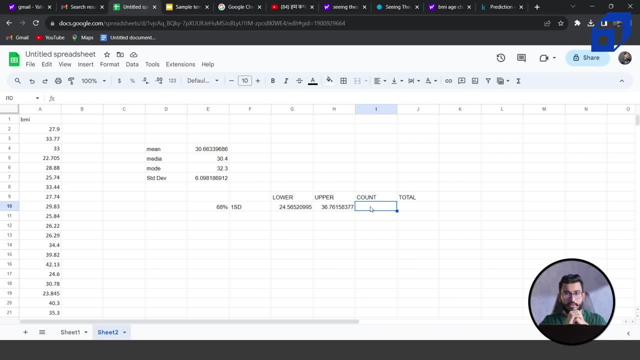 those are falling in this range, because my objective is to find out the percentage. So I'll quickly apply a filter over here and I will create a filter by condition, And my condition is: is between: is between: the lower value is 24.5.. And upper limit is 36.7.. So my upper limit is 36.7.. So with that I am done, I'll take a look. Now let me add one more name to the table. This is my total, So I am going to take a look at my total. So the final and my total. So that is my total. So this is my total. So the put and cut, so current, and I have to create a filter over here And I will create a filter by condition and I will add a condition And my condition is between the lower value is 24.5. And upper limit is 36.7.. 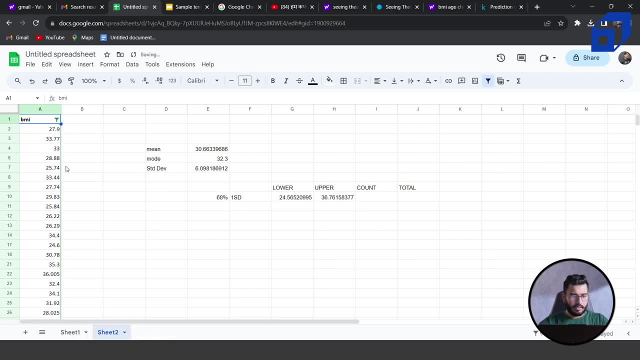 and I'll just quickly create a filter. Now. I'll just simply count it. If you carefully look over here, the count is 900.. So there are 900 values. that falls in this range. What are the total number of values for that? I have to remove this filter, So I'll say none. 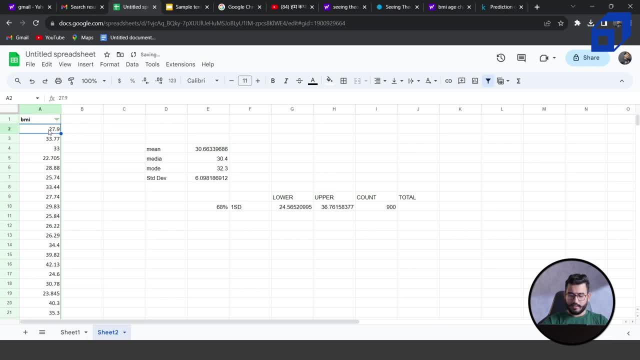 I'll say okay And I will calculate. So 1,338 is my total, So 1,338.. Now let's calculate the percentage Percentage. Sorry, Percentage. My percentage is equal to count divided by total And this is 0.67.. If I convert this into percentage, it is 67.2%, The standard. 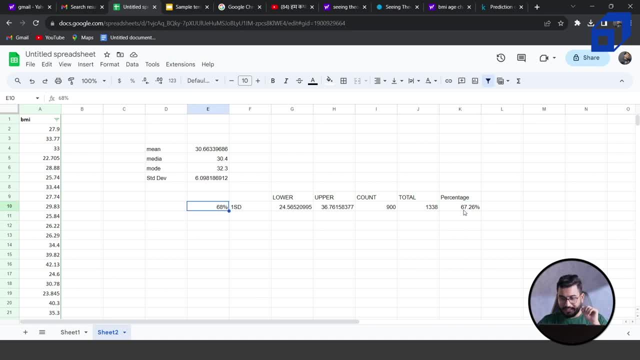 value is 68%, My data is resulting in 67.2%. This is the first proof of the first property. The first property says that 68% data lies between plus minus one standardization. I'm getting 67.2 because it is not a standard, normal right. The second property is: 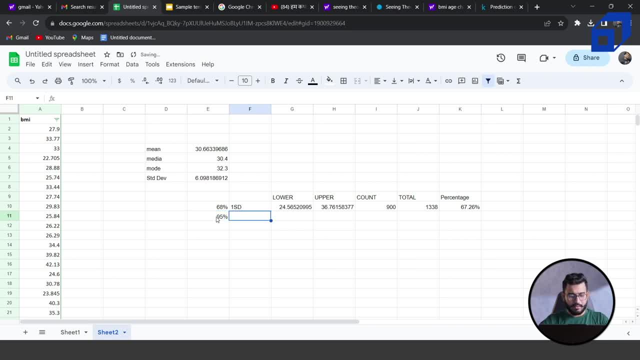 95%. So 95% data lies between plus minus two standardization. Let's check the lower limit. So is equal to mean minus two times of the standard deviation. Then is equal to mean plus two times of a standard deviation. And now I will count. 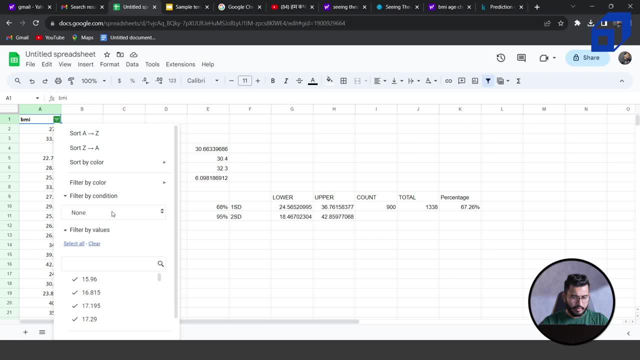 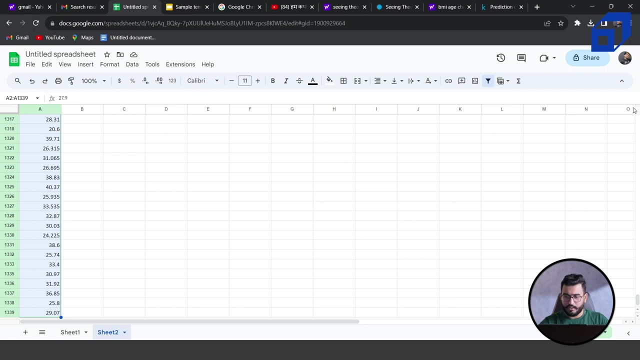 So I will go over here. My condition is between: My lower limit is 18.4.. Upper limit is 42.8.. I'll click okay And I will now count. The count is 1,281, data points 1,281.. So let's. 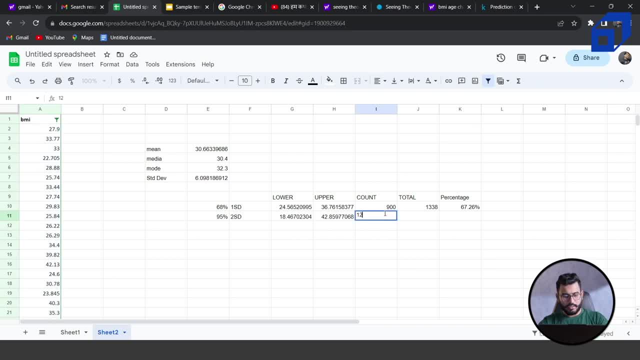 quickly write it down over here: 1,281,, 13,, 38 is my total. I'll just extend this formula to the next, the below cell: 95.74.. What is the standard value? 95%. What I'm able to achieve: 95.74.. Why there is a. 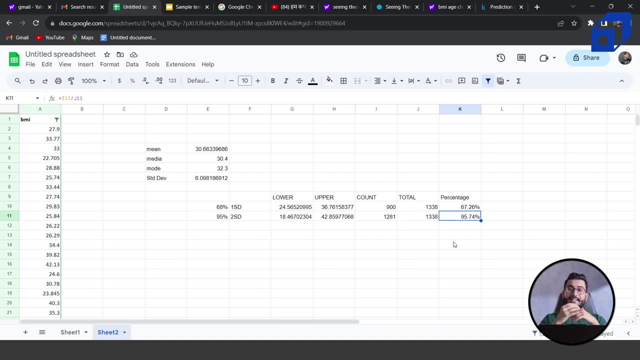 difference Because BMI is not my standard normal distribution. According to the standard normal distribution, around 95% values in my data point will lie between plus minus two standard deviation- And here you can see final one is 99.7% of my data falls between 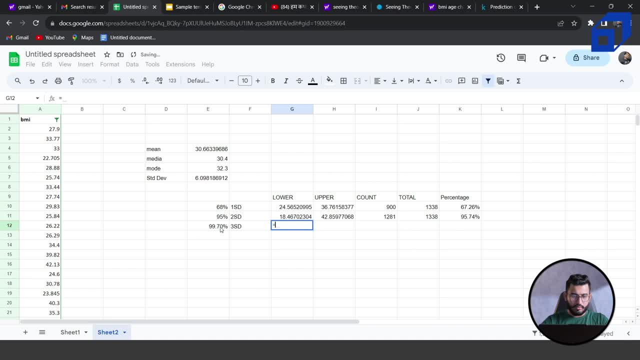 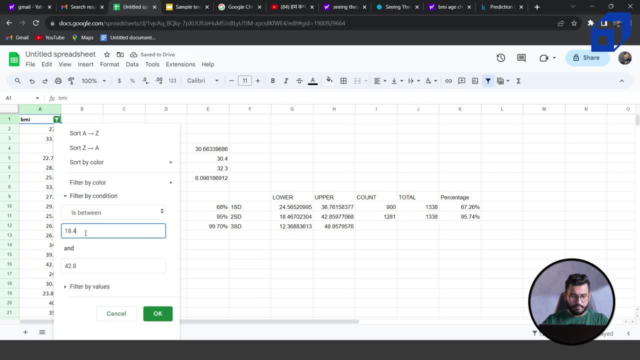 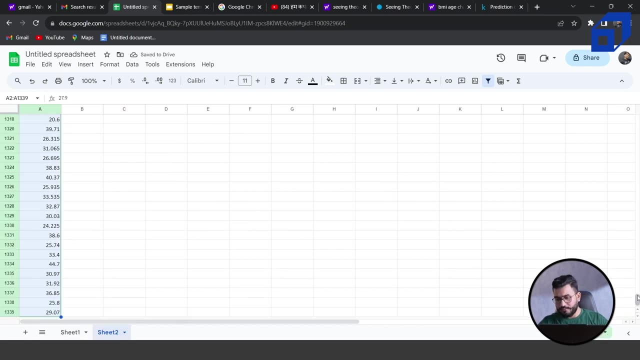 how many data points I'm having in this range. So 12.3 to 48.9, and I'll click OK. I'll just quickly count: It is 1334 and total is 1338.. So 1334, this is 1338 and I will extend this. 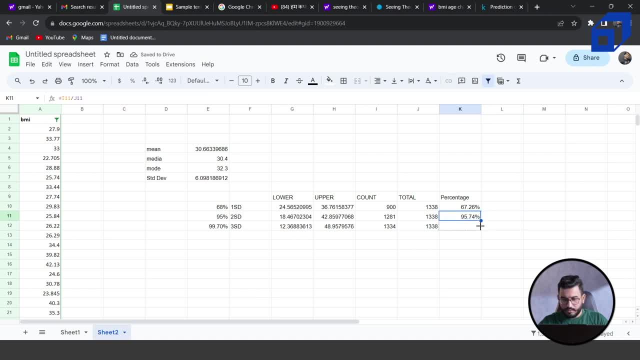 formula to the next row And I'm getting 99.7, which is exactly the same right. So this is the proof of these three properties: that 68% of the data lies between plus minus one standard deviation. 95% plus minus two standard deviation- 99.7 in plus minus three standard deviation. Now 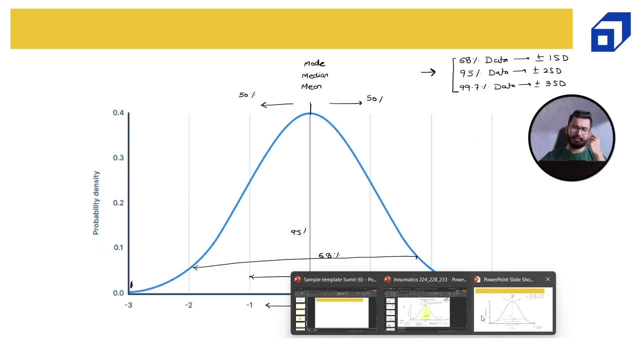 if I am given with a particular value- so let's say I'm given with a particular value- how I can find out that? what is the probability at that point? if you're not able to understand my question, don't worry at all. Let me try to make you. 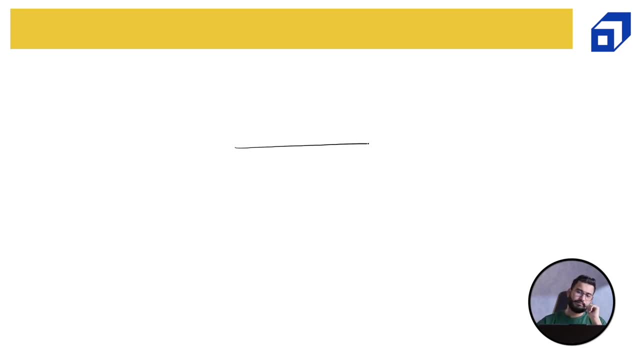 understand what I'm asking you. This is my standard normal distribution. This is my middle point. This is my standard normal distribution. This is my middle point, Which is zero. Zero means the mean is zero. What is the probability that a data point will lie? 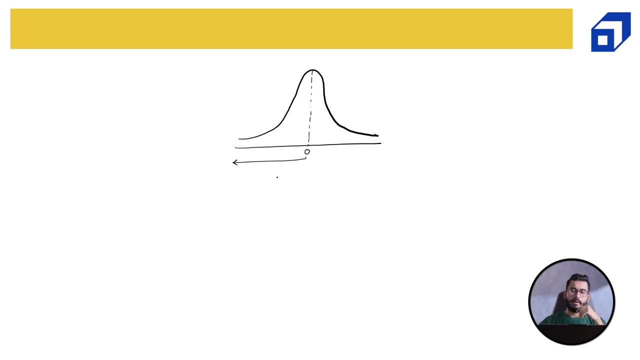 below this point, What is the probability? It is 0.5 and above this point, it is 0.5.. Because, as you already know that if I'm having, if I consider the complete probability, so what is the probability that a data point will lie anywhere in this particular? 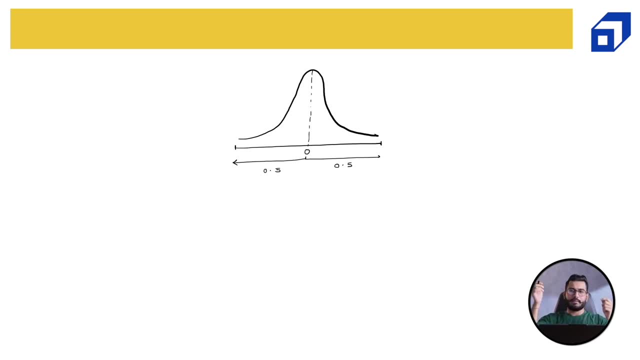 range. It is one, right. We know the minimum range. We know the maximum range. I know the probability that my data will lie somewhere in the middle, So I know it is going to be one. What is the probability that it will lie below mean 50%? above mean 50% if it is a standard? 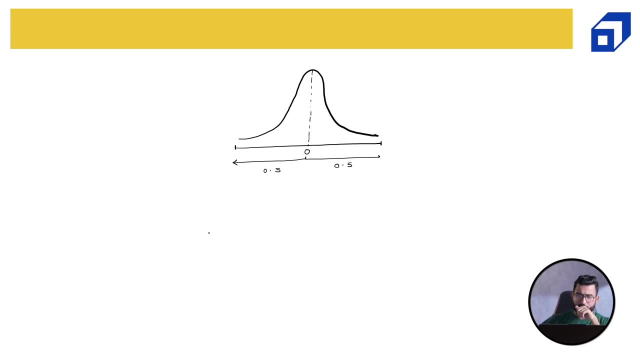 normal distribution. So, in order to find out the probability at any point from the left, we have something known as a Z table. Z table is basically a standard normal distribution table, standard normal distribution table, which helps us to find out the cumulative probability from lower point to this point. 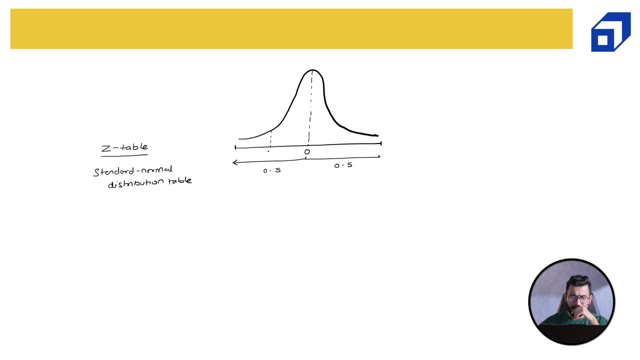 If I ask you what is the probability that a data point will have will lie below this point. So using the Z value, so let's say the Z values over here is minus one, So using the Z table, we can find out this probability, which is the area under the curve. Now let's 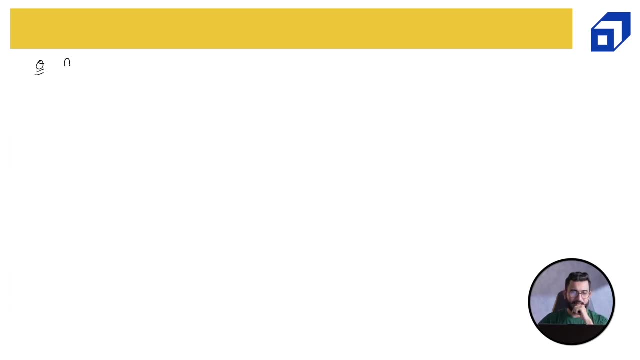 see one example. Let's say a set of biology marks in a class are normally distributed: Okay, Okay, Okay Okay, With a mean of 70 and a standard division of six, A standard division of six points. Now, led X represents something like 2, 3, 0, 6.. 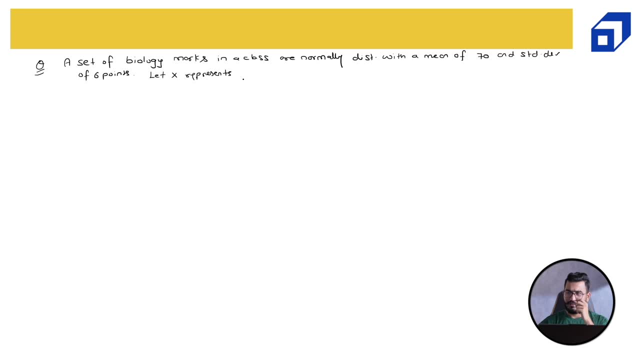 The score on now randomly selected person. So let X represents the score of a randomly selected student, Then what is the probability that the marks of this student would be between 64 to 79.. This question is very simple to solve. We just need the properties that we have learned. Let's. 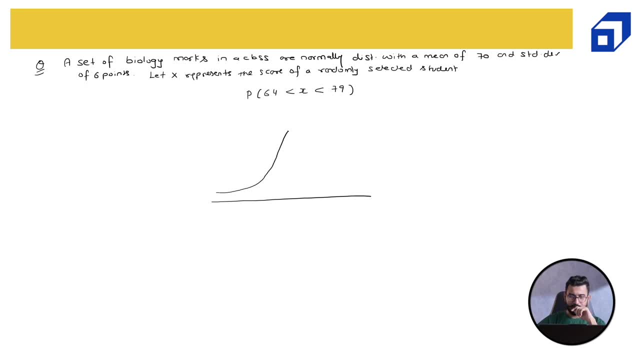 create the normal distribution. First of all, this is my normal distribution. The mean is 70.. A standard deviation is six, which basically means I'll go one standard addition below, So I'll get 64, one standardization above, So I'll get 76, to standard division below 58,. 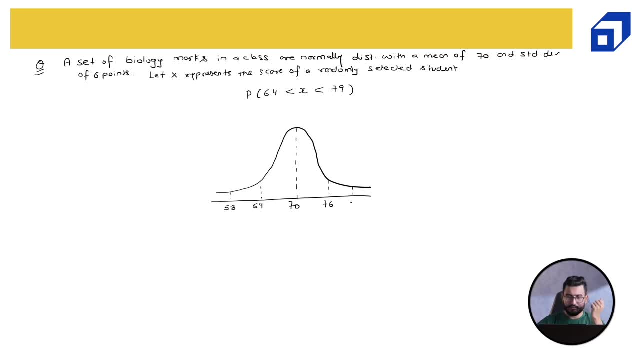 two standard division above 82.. Now what I need? I need the probability between 64,, which is this point, 64,, which is this point, to 79,, which is between 76 and 82,. right, So, from 76,. 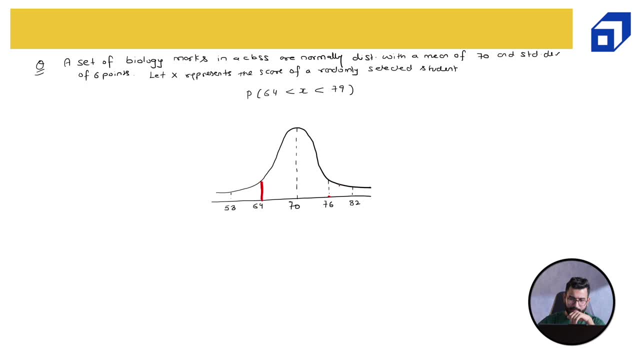 if I go half a standard deviation above, this will be 79, right? So this is the area which I'm looking to find out. Let me just highlight the area. This is what I'm looking to find out. I hope you guys are able to look at the area. 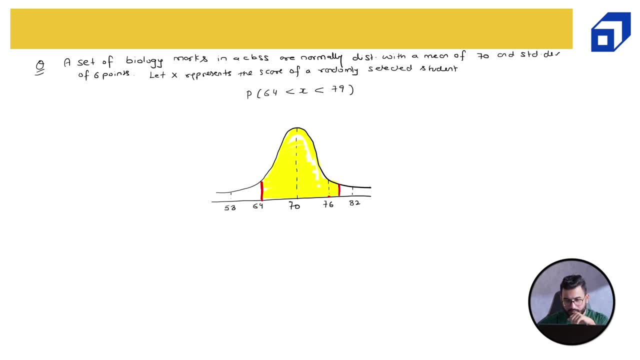 It looks like I'm coloring a book, but I hope this makes sense. Now, this is the area which I'm interested in. Now, if I go with the logic and the um, the properties that we have learned, so, from this point till this point, my uh, the percentage of data points, or the probability. 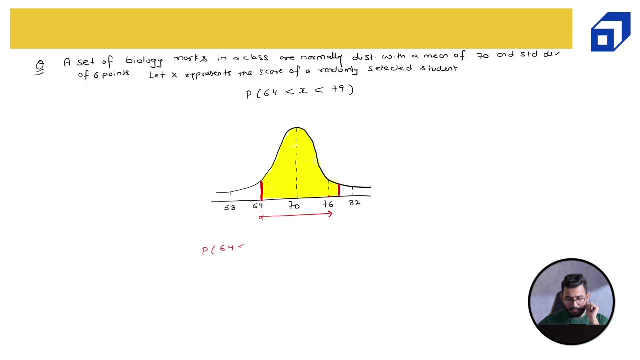 of a data point between 64 to 76 is 0.68, 68%. We know the property right Now. from this point till this point, from this point till this point, and from this point till this point, what is the uh area under the curve? So, if this is 68,, then 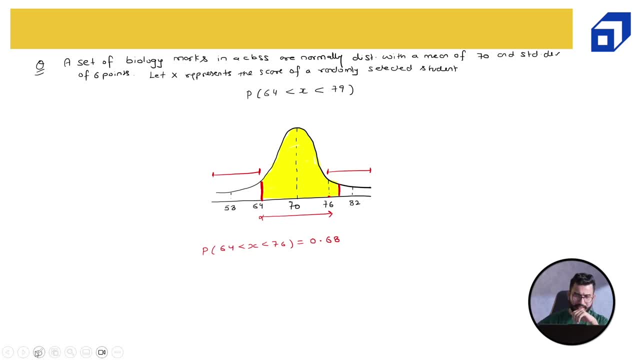 this point will be, or let's. let's not look at the complete curve, Let's look at the middle portion only. So from 58 to 82, from 58 to 82. So probably probability of data point between from 58 to 82 is 0.95, 95%, right? If I subtract this middle portion, this point, I will get. 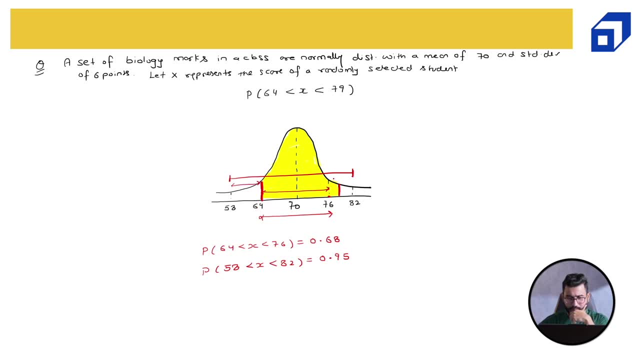 this portion and this portion, And I need the half of this portion, right, As we know that this part and this part is going to be exactly the same, right? So let's call this as C. and let's call this as C. Let's say 0.68 plus 2C is equal to 0.95.. So 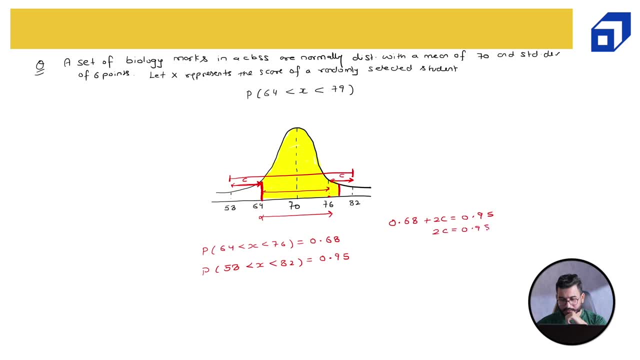 2C is equal to 0.95 minus 0.68.. C is equal to 0.95 minus 0.68 divided by 2.. This will give me C, this part right. So let's calculate C. So this will be 0.135. 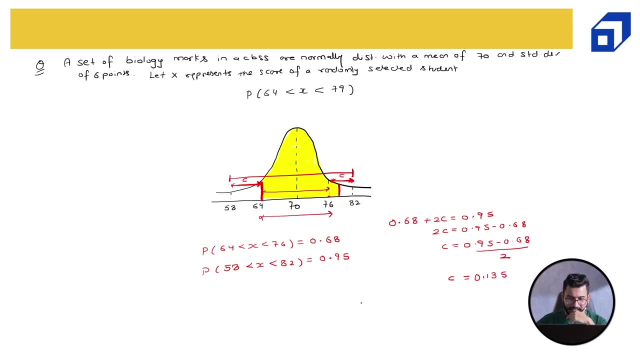 Now I'm interested in half of it, right? So my final answer will be probability of a data point between 64 to 79.. I'm interested in this point will be 68, which is 0.68 plus 0.135 divided by 2.. 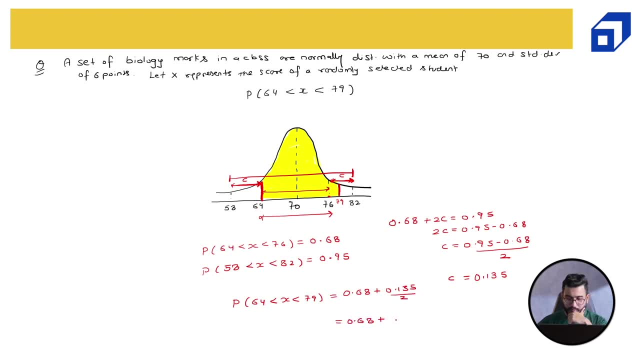 So 0.68 plus 0.675, which is 0.7475.. This is my final answer. So there are 74.7% chance for answers. I don't know whether one is right Or one is wrong. I expected few. I'm curious as to. 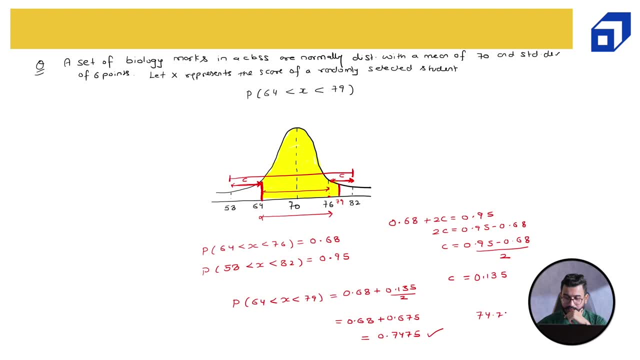 which ones are correct. I determine it on my 잘izing technique. There are Пощ with which one is right, But it's only happens often that there's Camera out there, But it is not so that there may not be any chances that a person who is randomly selected in the class will have the marks between 64 to 79.. 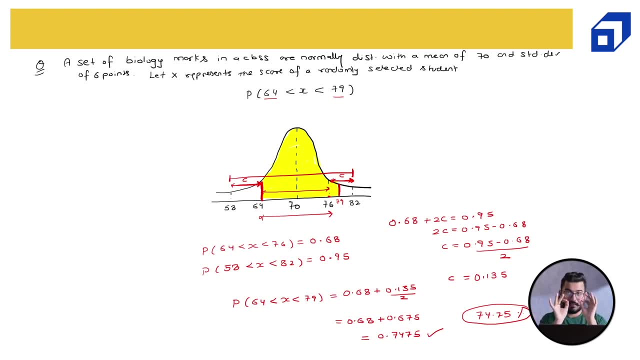 Now, in order to solve this question, we have used just the property of a normal distribution, which states that 68% of the data lie between plus minus one standard deviation, 95% between plus minus two and 99.7% plus minus three. I hope this is making sense, right. 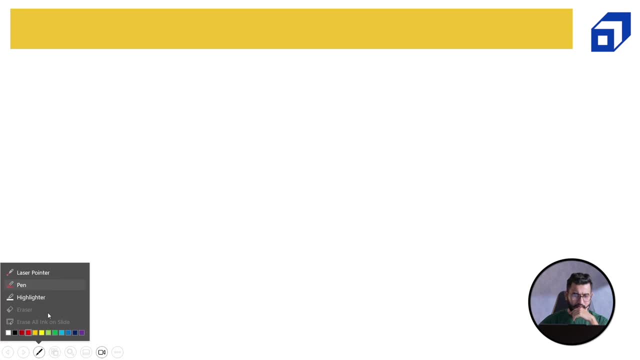 Now let's take one example which will utilize the Z table, for which, in order to solve this, we need the Z table. So the question says: the scores of ZMAT or GAMT. ZMAT are roughly normally distributed, So the score of ZMAT or GAMT will be ZMAT, with the mean of 527 and a standard deviation of 112. 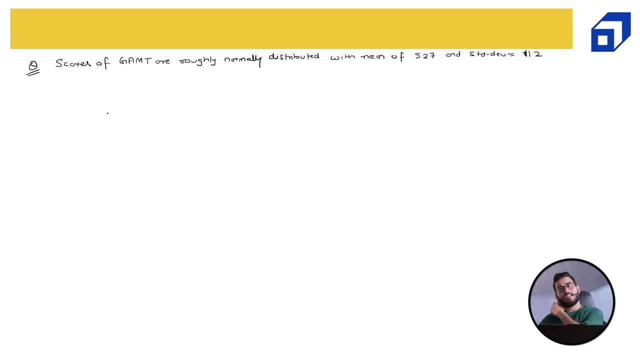 What is the probability that a of an individual is scoring above 500?? So my first question is: probability of an individual scoring above 500.. Now, in the previous question we were able to solve it because it that the question, the numbers that was given in our 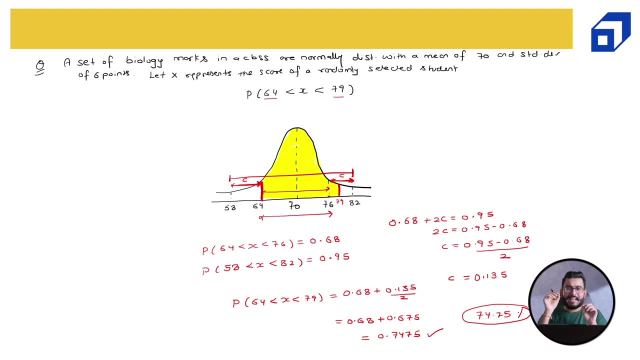 question was in the terms of any standard deviation. So the standard deviation was six units. I was given that the minimum and the maximum range in such a way that I was able to make calculations. I was able to use elementary math to get to the point right. But now we are not. 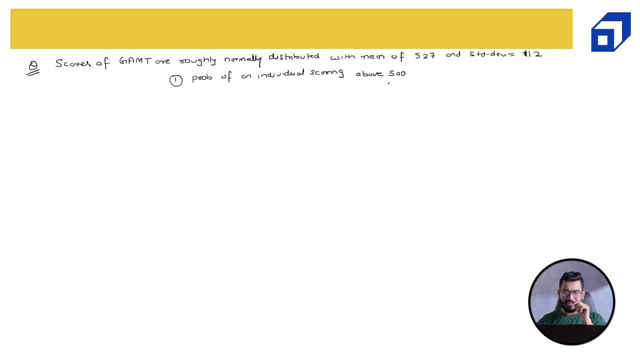 able to adjust it, because 500 and then standard deviation is 112.. It is really difficult to use the logic and use elementary math to get it done. In this case, Z tables are very useful. Let's solve this question. I know that the Z math scores are normally distributed with the mean. 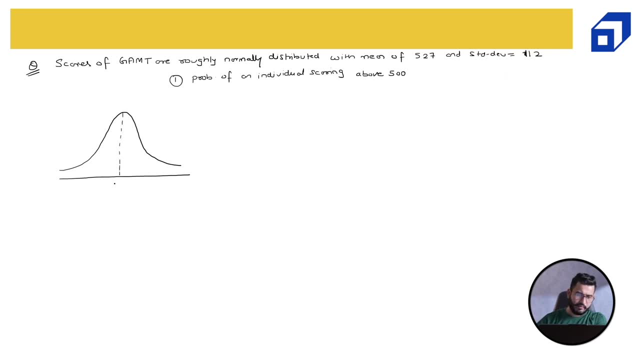 which is 527, and standard deviation is 112.. Now I will find out how many standard deviation above or below this value is lying at. So we'll use the standardization formula. We will find out the corresponding Z value, which is nothing but X minus mean. 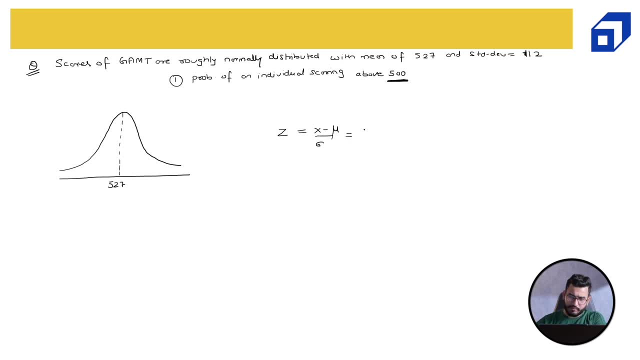 Divide by Sigma X is 500.. The value to be scaled minus mean 527 divided by 112, which will be minus 0.24.. So if I consider the Z scale, this value will be zero and minus 0.24 is over here. 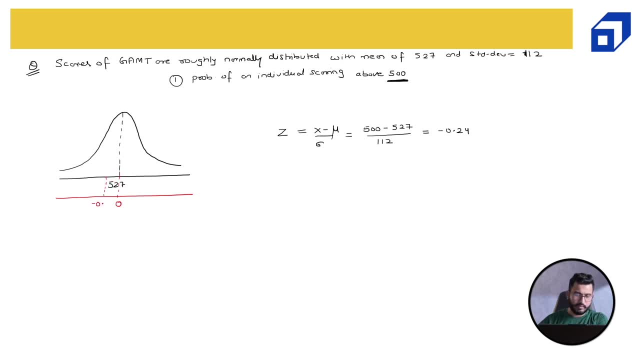 below me minus 2.5.. Now what is the probability that the person will be able to score above 500, in which area I'm interested in? So if this point is minus 0.24, then I'm interested in the area above this, which. 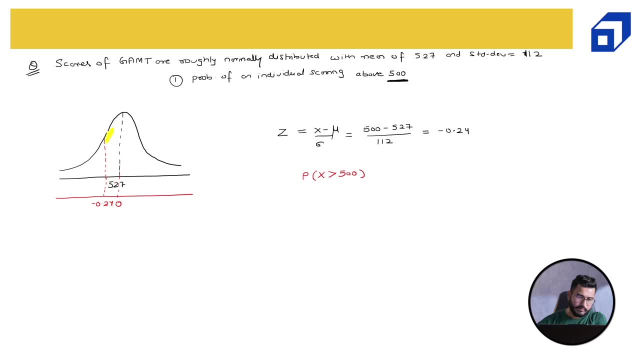 is this area the probability that the person will be able to score above 500.. So I'm interested in this area, this particular area. Now, how we will find it out? So using the Z table. Z table will provide me the area under the curve. 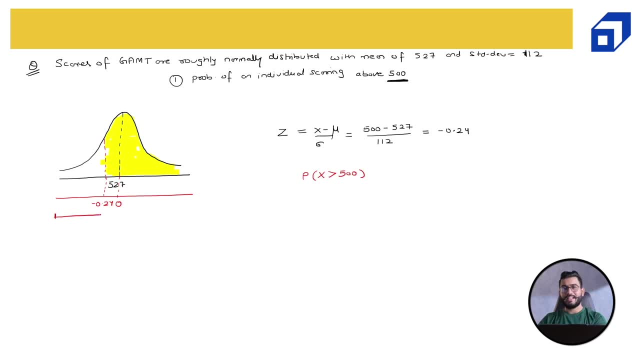 from this point all the way up to this point. Remember, AUC that you will get from the Z table will always be from the left. So once I have the area, which is the probability, from this point all the way up to this point, I'll subtract it from one and I'll get my required answer. Let's 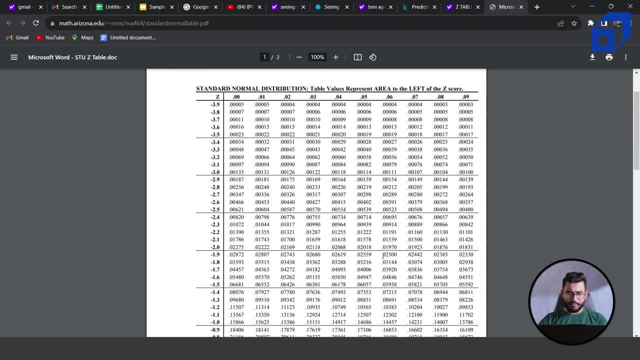 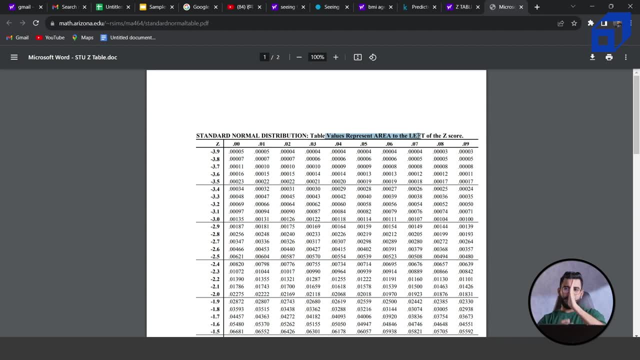 check the Z table. Now here we have the Z table And if you read, this is the standard normal distribution table. value represents area to the left of the Z score. So if I, if this is my Z score, left of the Z score. 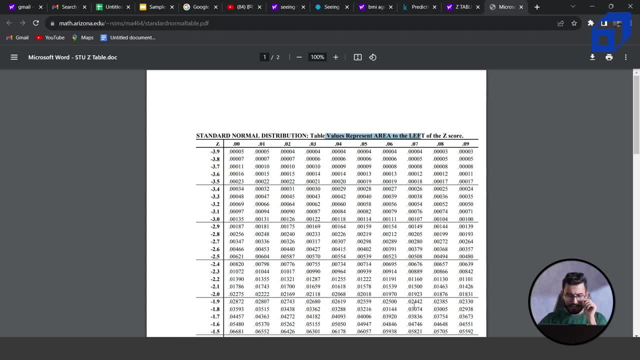 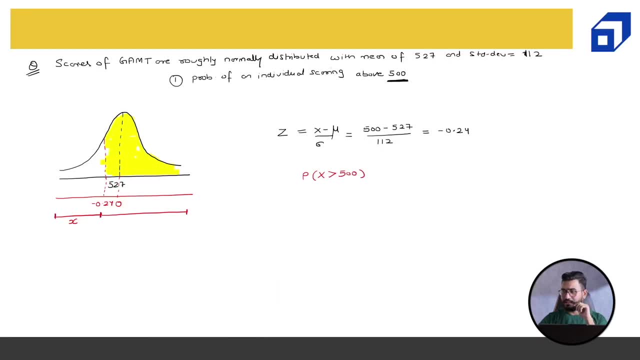 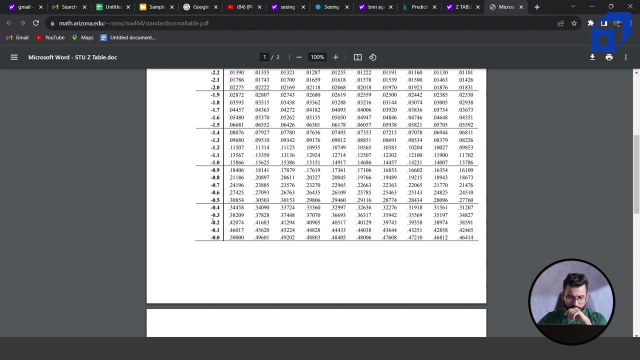 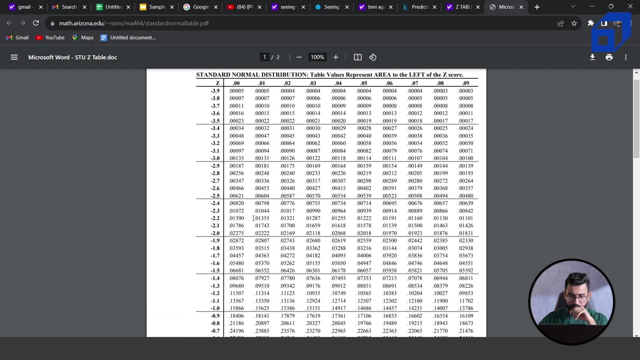 I'm interested in the value which is minus two zero points. So let me just cross check it: minus 0.24.. Let's check the area under the curve. So minus this is 0.2.. So my, we have to first read the row and then the column: So minus 0.2, and then four this value. 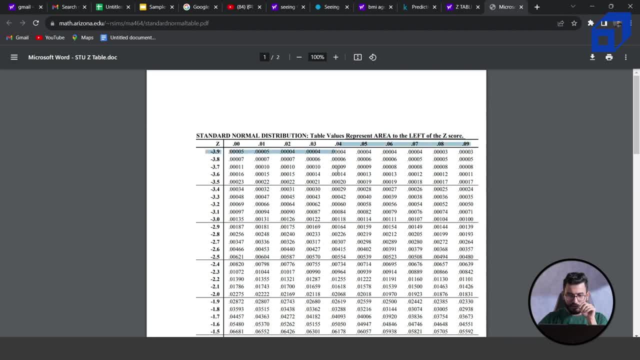 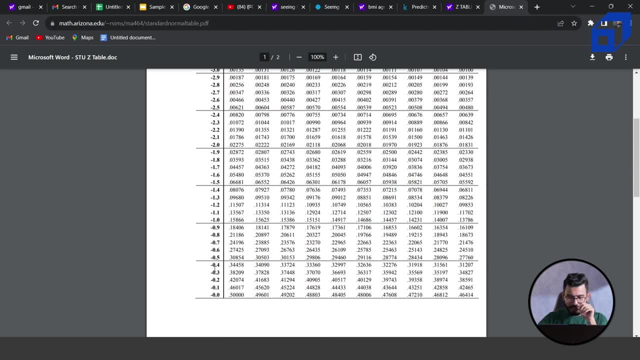 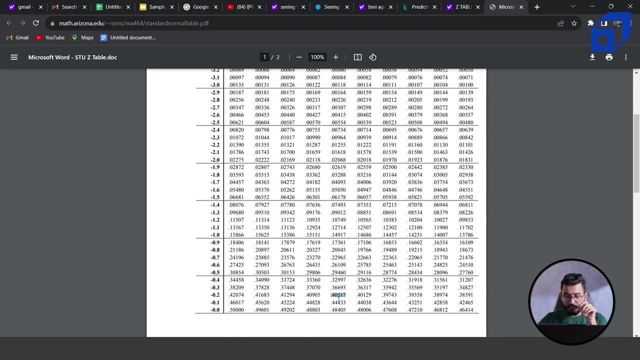 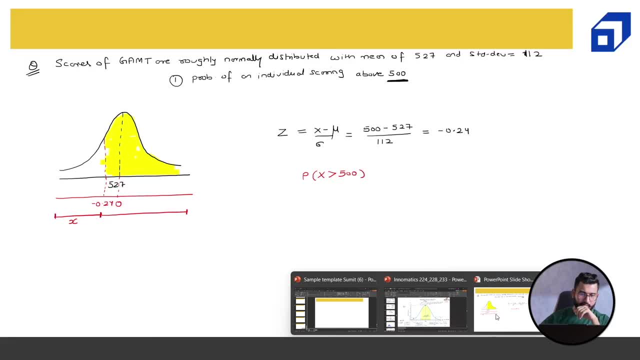 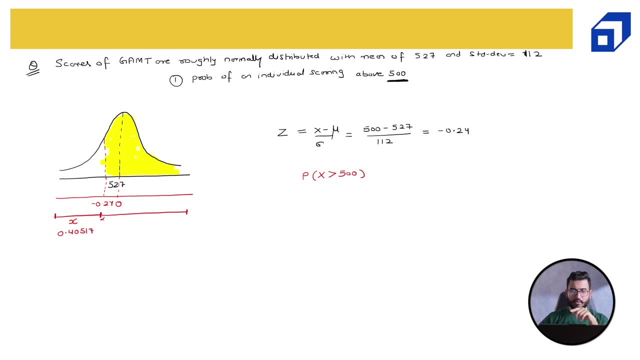 .40517.. .40517.. .40517.. .40517.. .40517.. So this, this X is .40517.. I'm interested in this. So what it would be is equal to one minus probability of X, less than or. 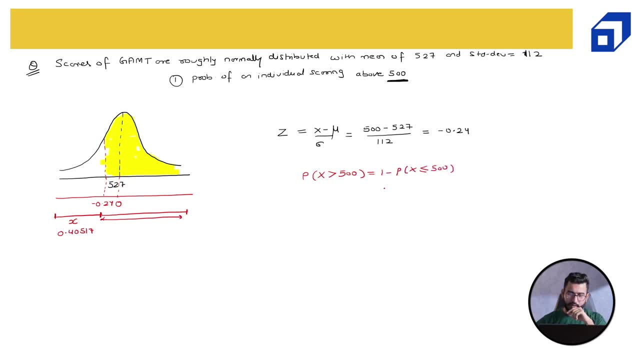 equal to 500, which is one minus probability of 0.40517.. The answer will be .59.. There are 59% chances. .50517.. .50517.. .50517.. Let's say there is one more question. 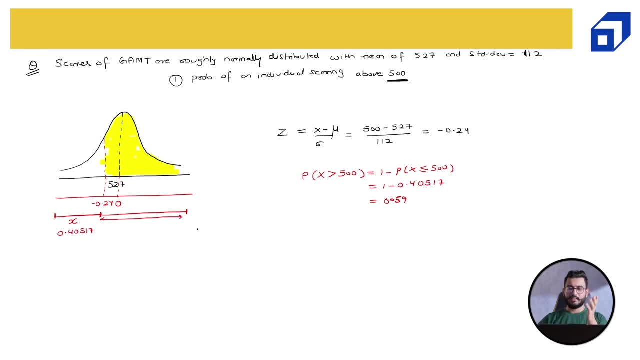 .50517.. in the same, in the same example, how much minimum marks should the individual score in order to be in the top 5%? now, this is a very interesting question and if you guys can understand it, you have understood the complete normal distribution: top 5%. if this is my middle value, top 5% means 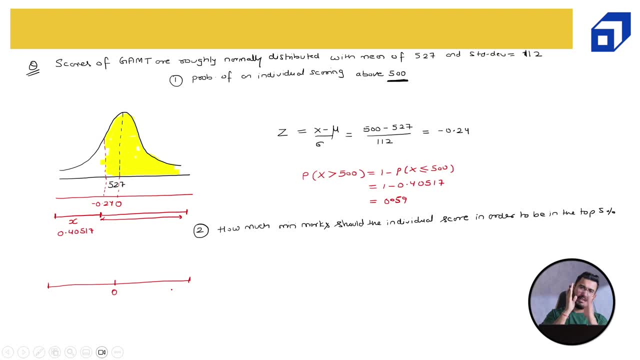 below me or below that point, 95 percent data is there. so if I draw the normal distribution and below, so let's say this is the point which I want to find out, and below this point I'm having 95 percent of my data right. so I know that I want to find out that Z value X minus mu, divided by 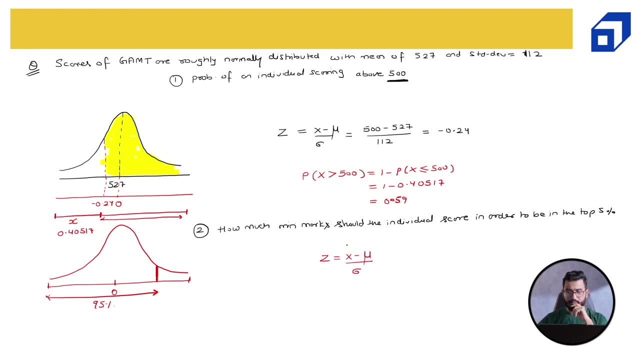 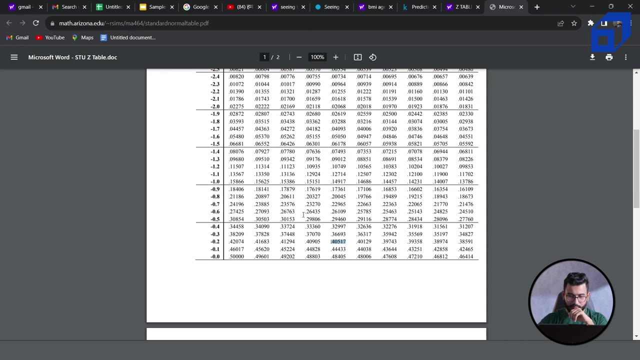 Sigma. I need to find out that X where the Z value is this. so what is the Z value at 95%? let's look into that. the Z value at point nine five. so I have to look at the area now to find out the Z value. so nine five zero five is. 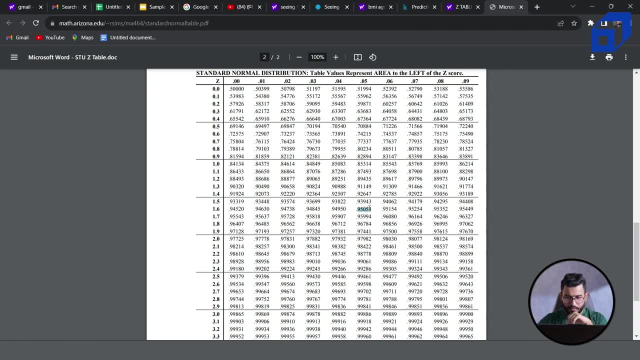 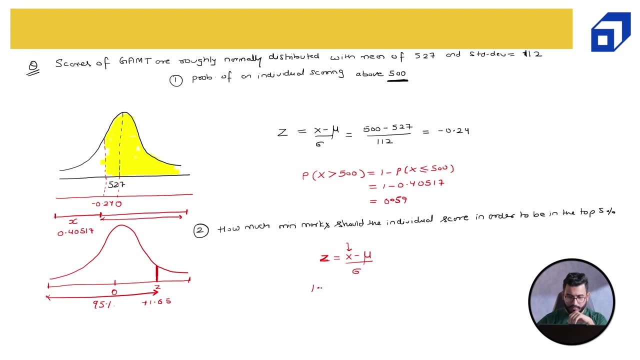 over here. this is one point six and five. so one point six five is my Z value. so it's a Z value plus one point six five. so I know the Z value plus one point six five is equal to X minus. mean is 527 divided by studying division is 112, again the elementary math, 1.65 multiplied by one hundred. and 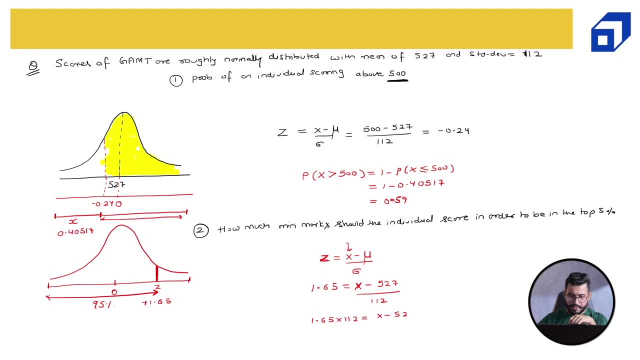 twelve 12 is equal to X minus five hundred and twenty seven. so my X will be 1.65 multiplied by one hundred and twelve plus one hundred and twenty seven, and two of that takich's in this will be five hundred. aliages game all the time and we get it. 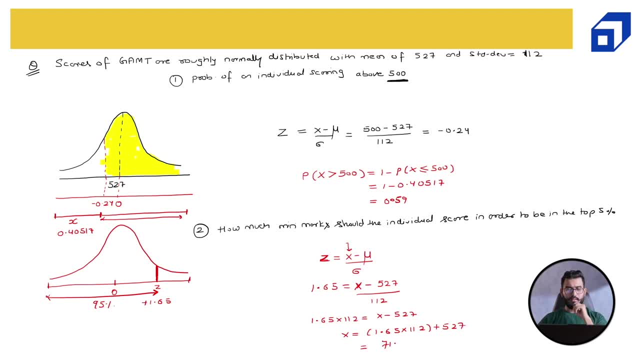 be 710.6,, which basically mean the person has to score a minimum of 710.6 in so that the person can lie in the top 5% And below that person I'm having 95% of the observation Now. this is the. 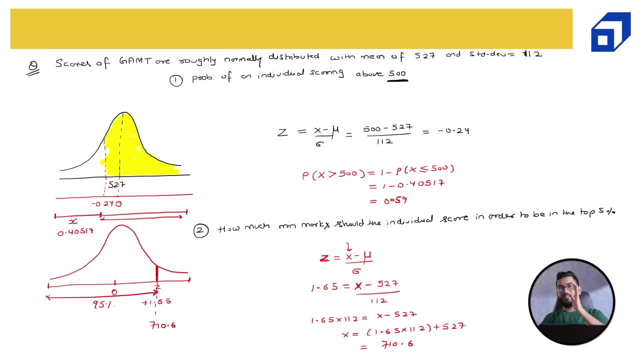 application of Z table. how Z table can help you to find out the Z values and how Z table can help you to find out the area under the curve, which is essentially the probability. What is the probability that I will have a data point below this point, below this Z value? That's what the 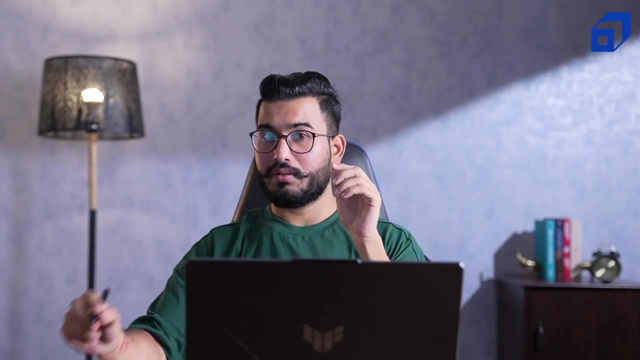 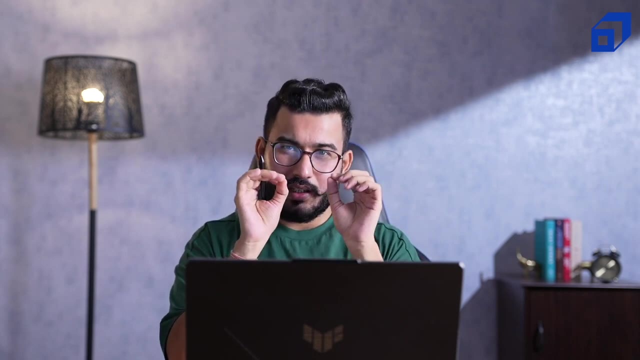 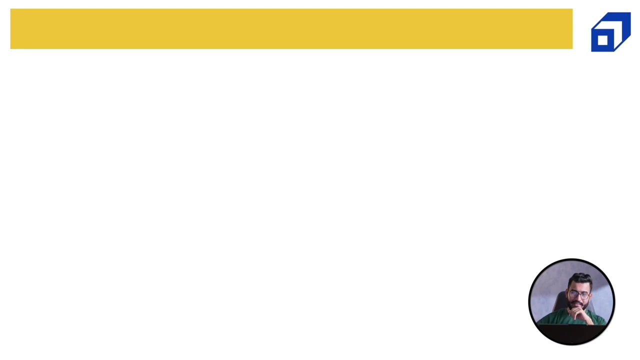 application of Z table is Now. we have learned about a lot about a standard normal distribution. right Now, what we are going to do, we are going to learn last property of a standard normal distribution, which is the analysis of skewness. We know that as standard normal. 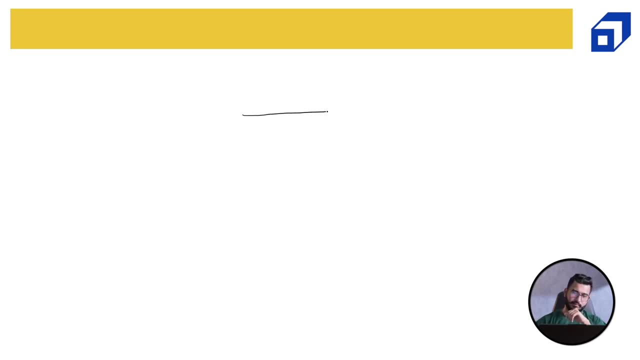 distribution. we know that as standard normal distribution. we know that as standard normal distribution looks something like this: a bell shaped curve which is symmetrical, which basically means 50% data below mean, 50% data above mean. but this is a standard And in reality it is very. 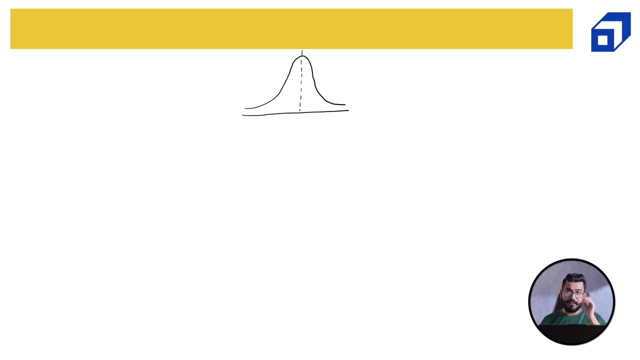 difficult or close to impossible to find out a random variable, a continuous random variable which appears to be a standard normal distribution. So we use standard normal distribution as a benchmark, But in reality you may get a distribution which is either left, skewed, 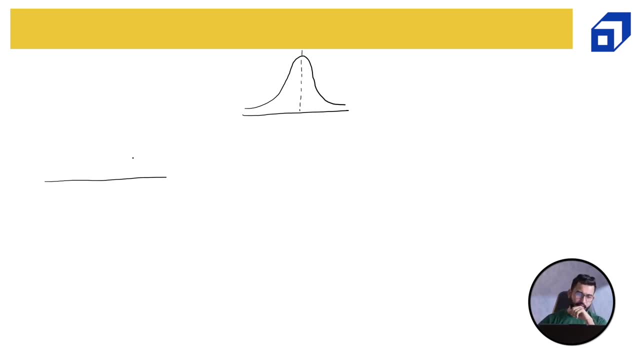 right skewed or no skewness or near skewness. Let's look at all the three types. This is known as the left skewness. I apologize, This is known as the right skewness, Right skew. Why I'm calling it as a right skew? because the skewness is on the right side. So right skew In the case of right. 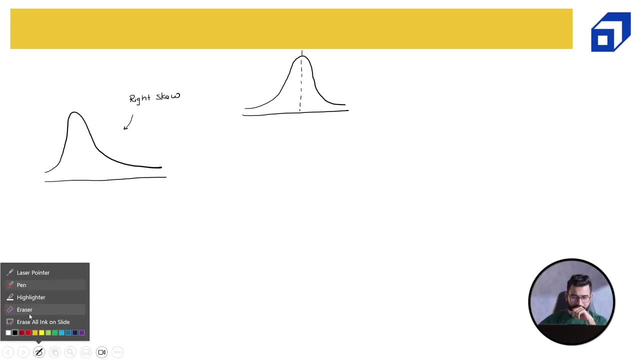 skewness. This tail happens to be because of the presence of outliers, the presence of outliers, presence of outliers, while most of my data is on the lower side. So here I will get the mode, followed by the median, and then I will have the mean. So I hope you guys remember that when we were talking about the 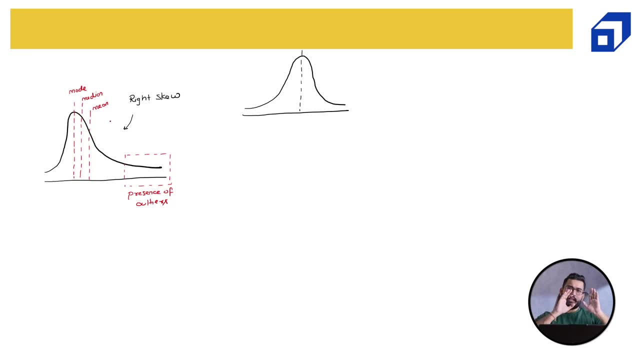 descriptive statistics, we have learned that if I'm having outliers on the higher side, my mean will shift to the higher end And that is the reason you can see that the mean has shifted to the outliers or towards the outlier. Now, below this point, below the median, I will have the 50%. 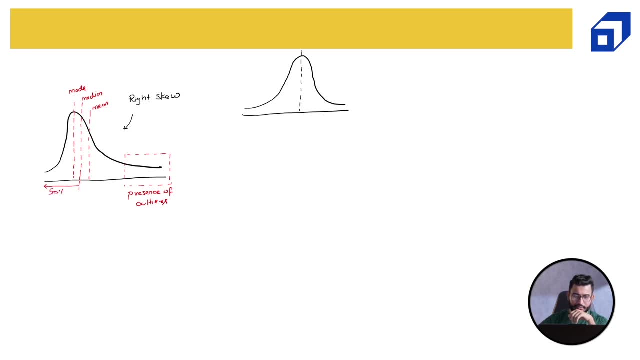 of my data And above this I will have 50% of my data. This is known as right skewness. I can also get a distribution which is left skewed or something like this. Now, here again, you guys can easily understand this tail is because of the presence of outliers. 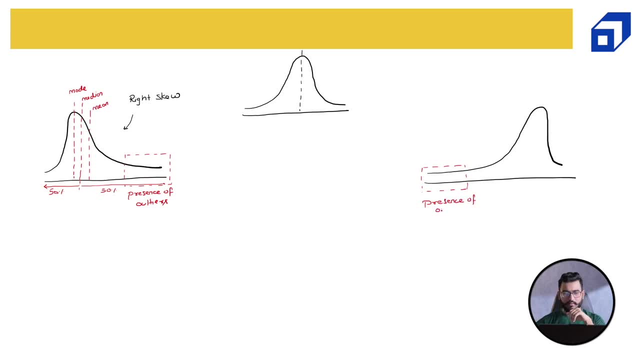 presence of outliers, outliers, And then again, this is the mode, the mode We have the median somewhere around here and finally the mean. So mean again shifted towards the outlier. Now, here most of my data is on the higher side. If I consider this X axis to be my income, then this left. 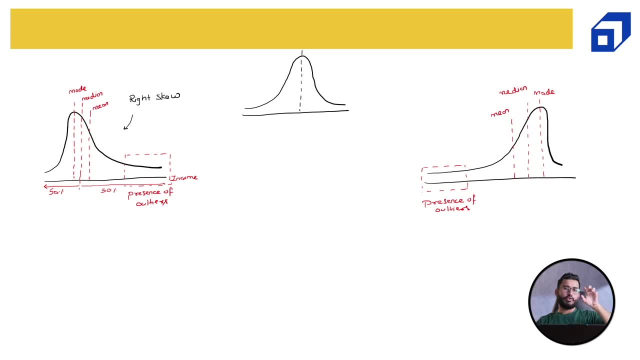 side graph represents that most of the people are having low income, While in the left skewed graph- a left skewed distribution, we can understand that most of the people are having high income, But due to the due to the presence of few people who are having low income or 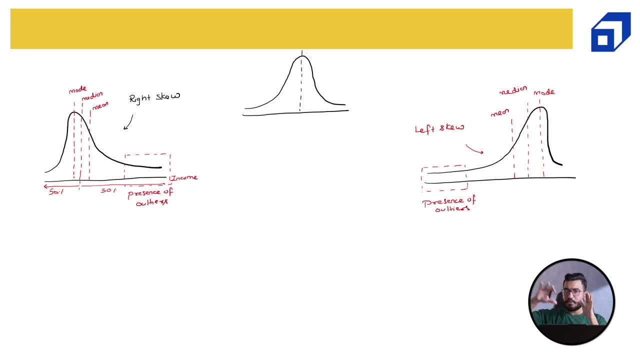 very low income. uh, the graph has been on. the distribution has been skewed and we obtained a left skewed graph. Now, in the case of right skewness, my mean is greater than median, is greater than mode. This represents the presence of right skewness. In the left skewness, my mode is greater than. 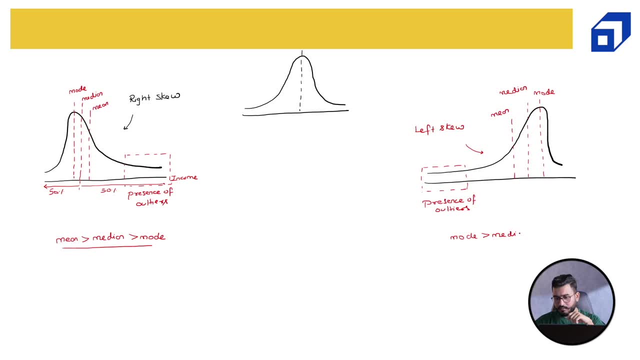 median is greater than mean. This is the presence of left skewness And in the case of no skewness, mean will be equal to or approximately equal to, median will be equal to, or approximately equal to mode. If you are getting something like this, you can say your distribution is. 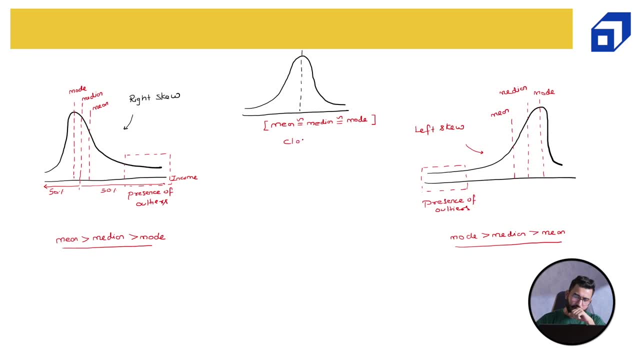 close to normal distribution. close to normal distribution. Now, please remember the properties that we have learned: 68%, 95%, 99.7%, which is also known as 1,, 2, 3 rule. it will applicable. it will be. 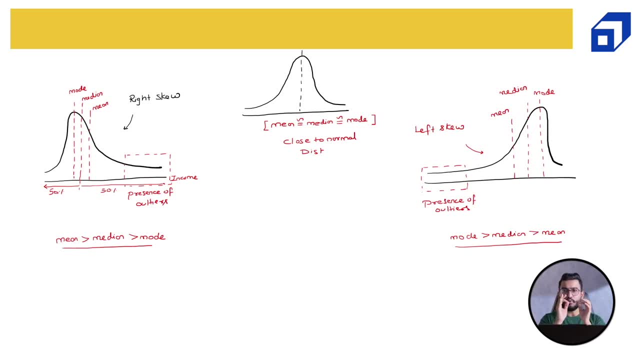 best applicable if your distribution is close to normal distribution, While if your distribution is having left skewness, right skewness, well, those properties will not be 100%. true, it will be close, it will be very close, it sometimes it will be very different. So, whenever you 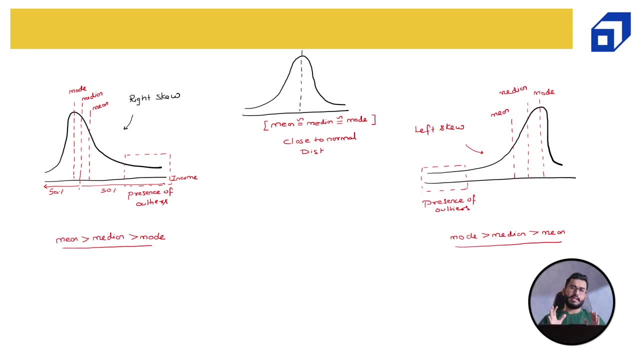 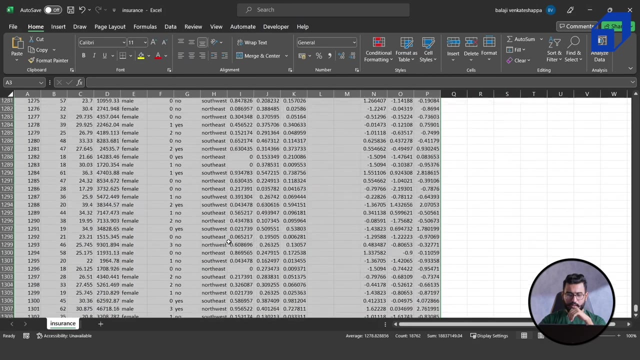 are applying the property, please make sure that your distribution is close to normal distribution. The example of BMI that we have seen was close to normal distribution. So we can just go back to the same, the same sheet. So let me go back to the same sheet. 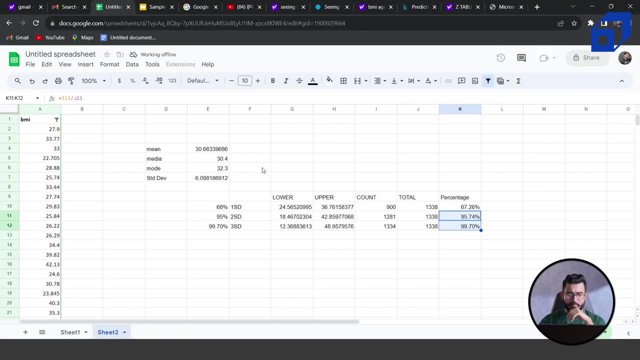 Here we have the data And here you can see that the mean median and mode were very close to each other. So this distribution was close to normal. it was not perfectly normal, it was close to normal And that is the reason these properties hold true. Otherwise, if this distribution was not normal, 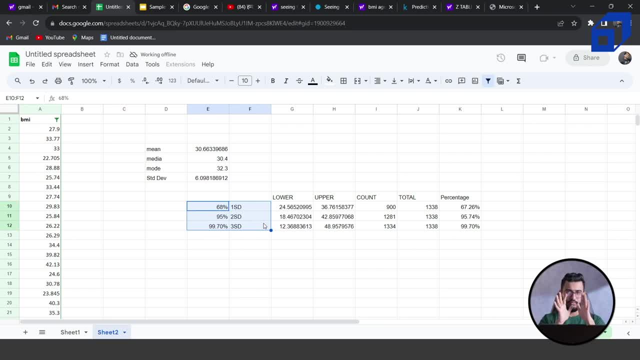 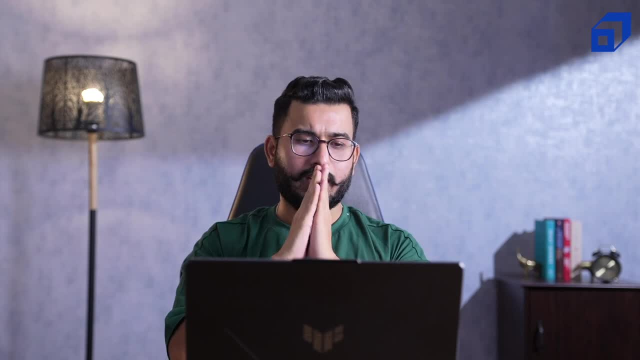 this property is would not have held true. I hope this make sense. So we have covered a lot of topics And the most important important topic that we have covered till this point was the normal distribution. the analysis of Z table. how to read a Z table? 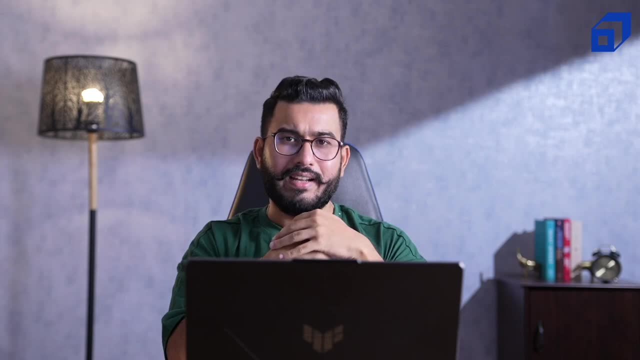 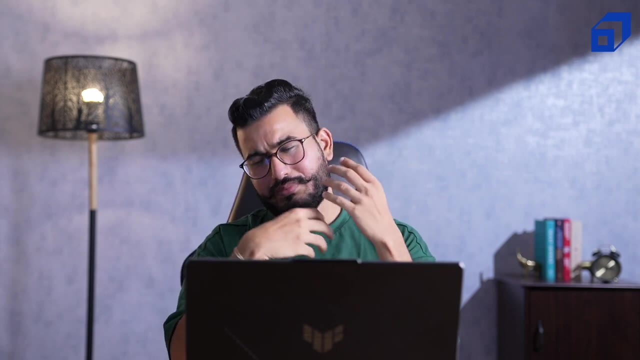 how to make use of Z table to find out the probability values, And we have also learned about descriptive statistics and a bunch of probability: The random variables, consecutive, continuous expected value. we have learned a lot. right now, we are going to start with. 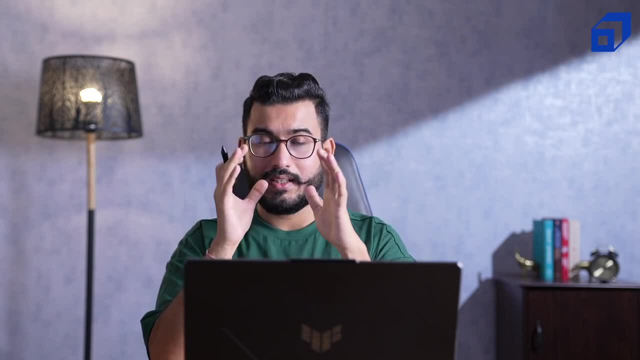 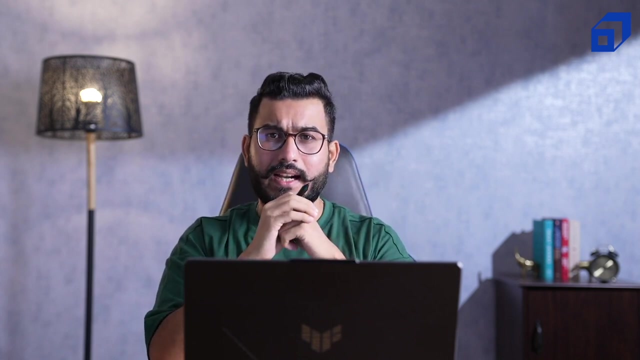 the second very important topic under our statistics and probability framework, which is inferential statistics. i have already given you the essence of what inferential statistics is and why we need it when we were discussing about descriptive statistics, but now we are going to understand it completely and also we are going to utilize the power of inferential 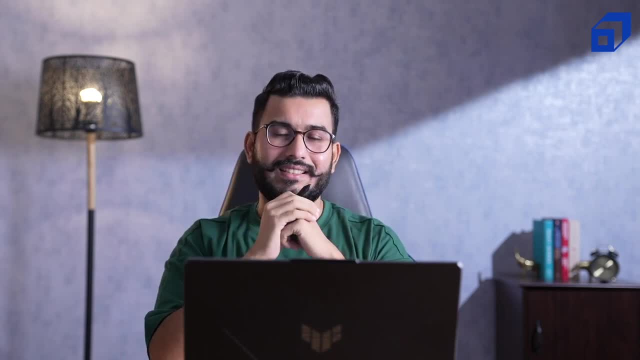 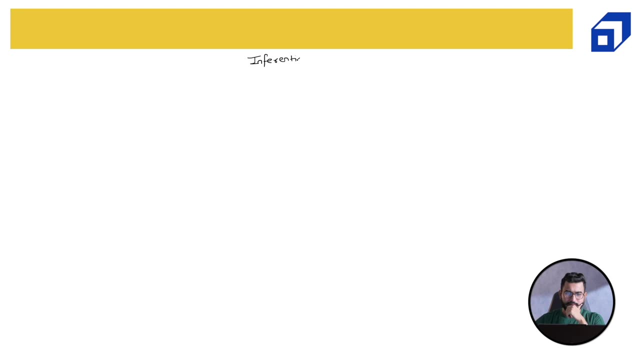 statistics to make estimations. so let's start our discussion. so when we talk about inferential statistics, in order to understand inferential statistics, we will take one example. let's say you work for a marketing company and your manager wants you, wants you, to find out on an average how many recharge, or maybe the 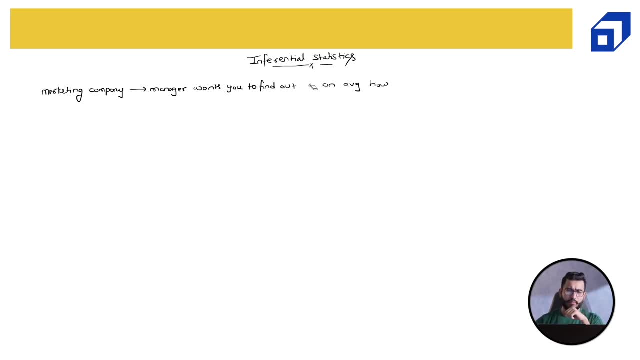 average recharge. so your manager wants you to give able average recharge and when you give able average, you you to find out the average internet recharge, the average internet recharge made by the Indians, So I'm talking about the complete Indians in last year. Now just look at the scope of the 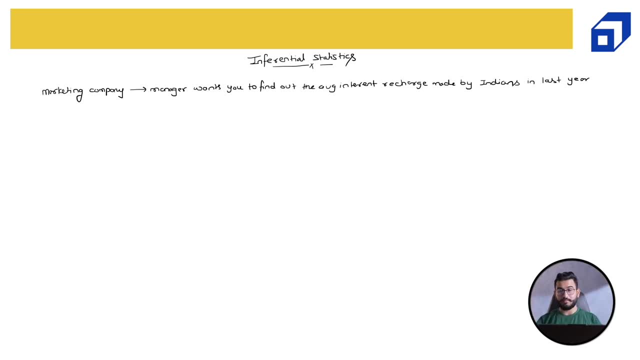 problem. We are talking about complete India And your task is to find out the average, the average internet recharge that was done by complete Indians in last year. It's a very big, challenging problem, right? So let's assume that we have the circle representing the complete Indian population. 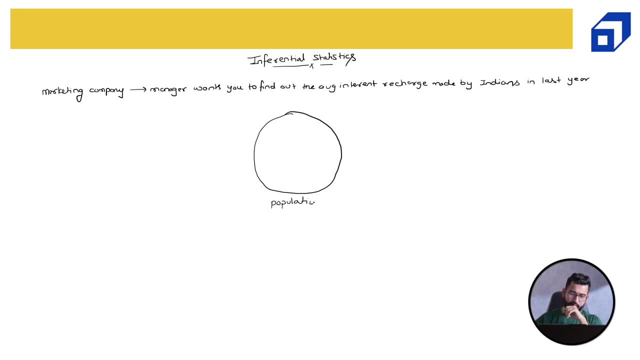 So population? And now, in order to find out this answer, what you will do? so let's say: this is you, this represents you. you will basically reach out to each and every individual, you will collect the data. So let's say the, the recharge done by person number one. 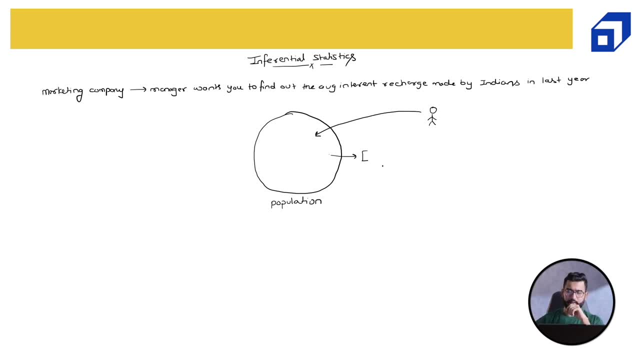 So, let's say, the recharge done by person number one isr One, then r two, then r three, and so on, till are, let's say, 150 crore. Now, First of all, it is impossible, or not impossible, to near to impossible, for you to collect the data of this much size and it will be impossible to connect the data of this much size and it will be impossible, in order to work out a percentage. 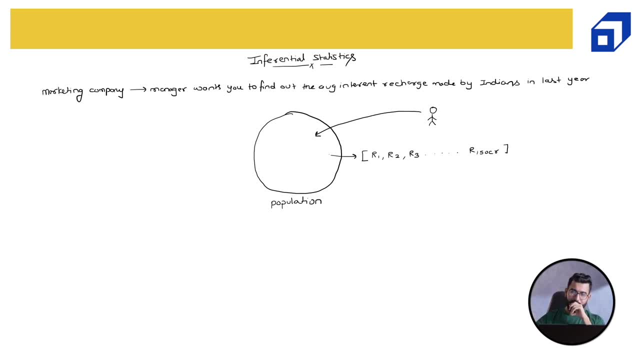 So that's the hidden information is that? And let's say, you heard about companies. R 보시면, In India a company могу Directly data banget r R A for you to perform survey in such a large scale. so what is survey? let's say, if I'm having a group, 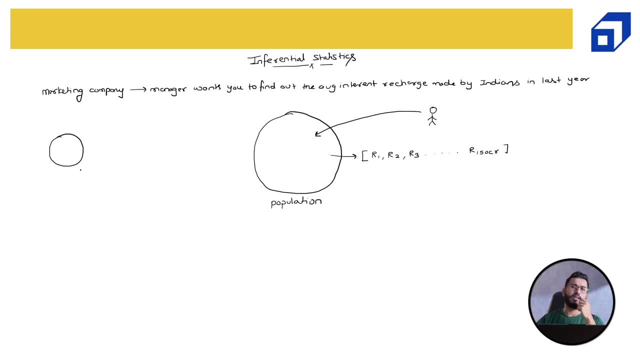 of people and I want to ask whether they prefer tea or coffee. so what I will do? I will perform a quick survey. I will perform a survey. so survey basically mean I will go to each and every individual. so reach out to each and every individual then ask them about their opinion. 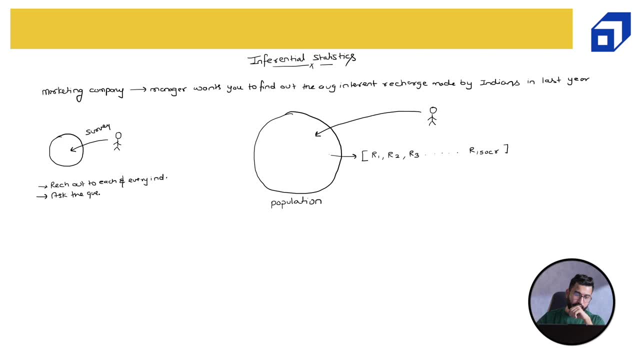 so ask the question. ask the question, then collect the data, collect the data and finally we perform the estimation. so estimation estimation means we calculate the average, minimum, maximum, whatsoever you want to calculate. this is the process of survey. now, if I have to perform the same thing on a population which consists of 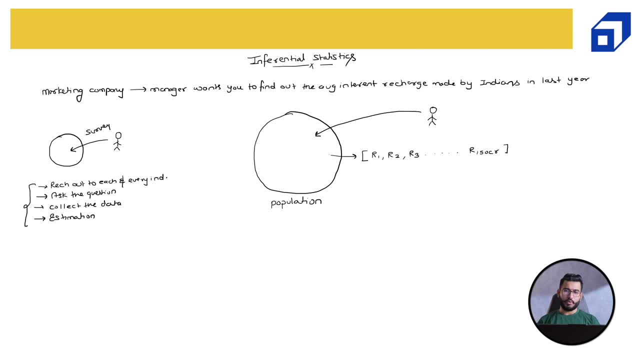 150 plus crowd people, don't you think? for a individual like you, it is near to impossible, not impossible to near to impossible and the I would say it is impossible. even for me, or even for a get along and organization. it is impossible for anyone to perform a survey in such a large scale, Even if it is possible. 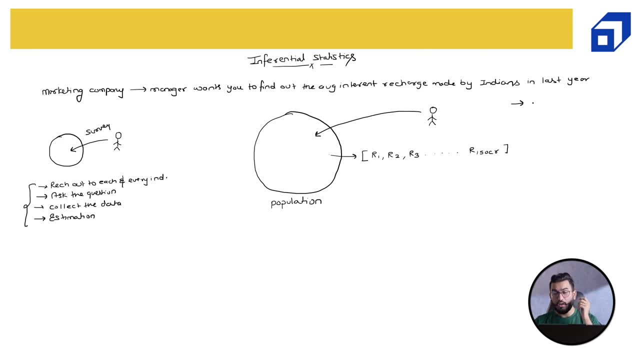 even if it is possible by a government organization, it will take a lot of time, a lot of time, and it will take a lot of investment. A lot of investment means lots of money is required, A lot of people is required. So lots of investment, investment. Now, what is the better solution? 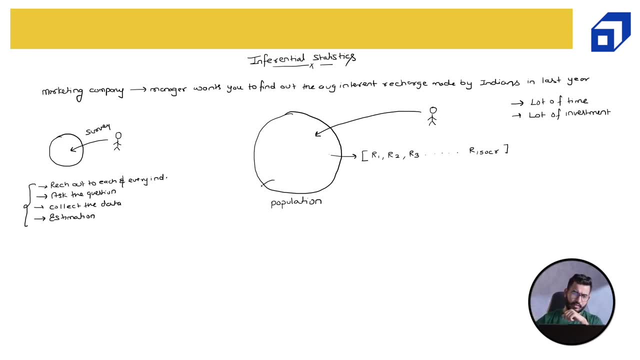 for this? We have already discussed about it. The solution is: I'll take a small sample. We call this as a random sample. Now I'll talk about what random sample is all about. But we take a small sample, We take random people. Let's say, I have taken one lakh random. 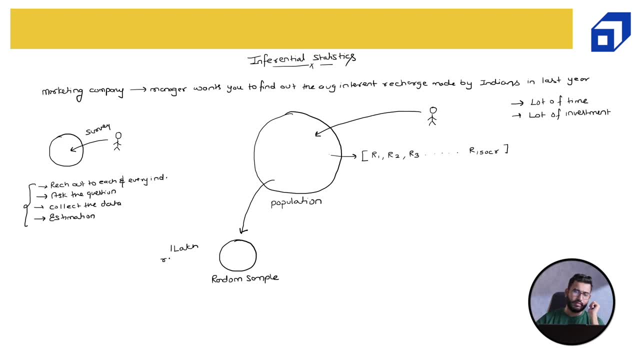 people, One lakh random people from the population of 150 crore plus people. Now, as an individual, it is quite possible for you to perform survey on one lakh people. So you have performed survey, you calculated or you collected the data. So R1, R2 till R1 lakh. then you take. 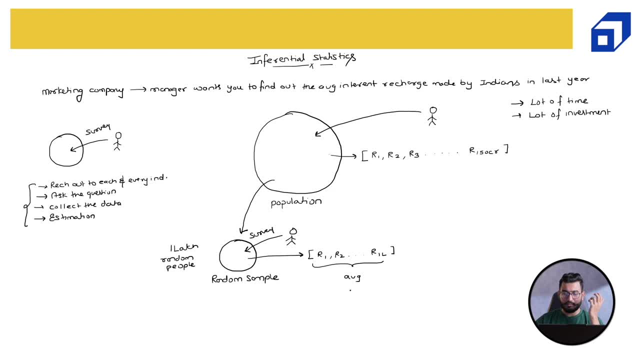 the average. Then you took the average And this is my sample average, Sample average. This is known as the statistic Sample statistic. Now, using this, I will try to approximate my population parameter. So using sample statistic, a sample mean. 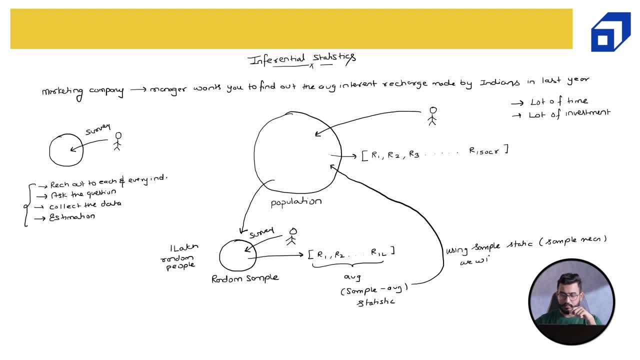 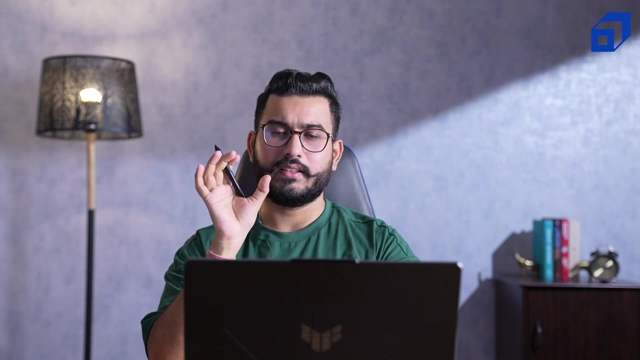 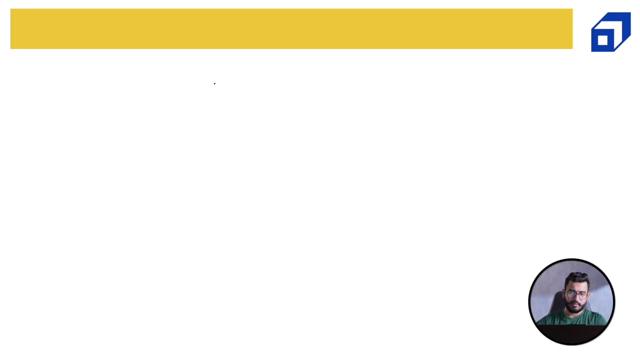 we will try to approximate the population parameter: a population mean, population mean, and this is basically known as your, this is basically known as your inferential statistics, inferential stats. now, before we talk about how to estimate the population parameter, let's try to quickly understand what is sampling and random sampling. so when we talk about sampling, it is 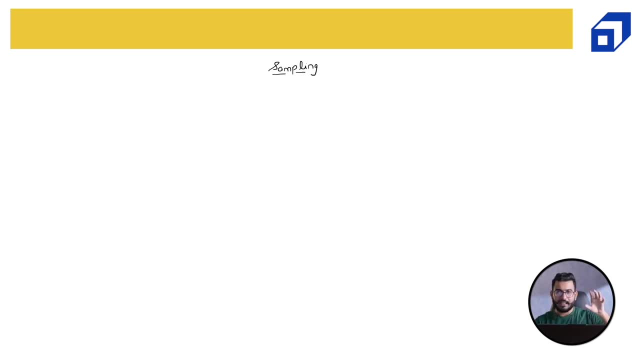 basically the procedure of collecting few observation from a bigger subset, or you may say population. so I am having a population, I'm having a population and now I want to collect a smaller sample of smaller group of observations. this is another sample. now this process is known as sampling. there is one very popular sampling technique, which is known as random sampling, and 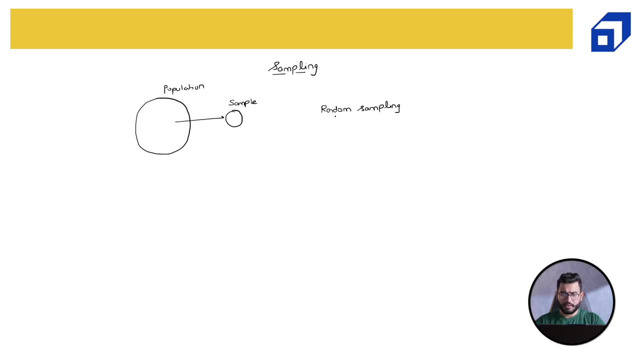 this is a very important interview question. what is that sampling? Random sampling is nothing but assume that if I'm having a population having, let's say, numbers 1,, 2,, 3,, 4,, 5,, 6,, 7,, 8,, 9,, 10,, 11,, 12,, 13,, 14,, 15,, 16,, 17,, 18,, 19 and 20.. So I'm having 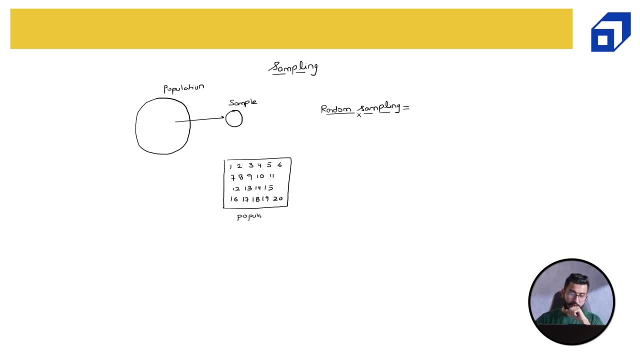 a population which is having twenty people, and the roll number of twenty peoples are written over here. Now, if I have to select a random sample of five people, so select random sample of five people. So what we will do, we will. we can select any five people, but according to the 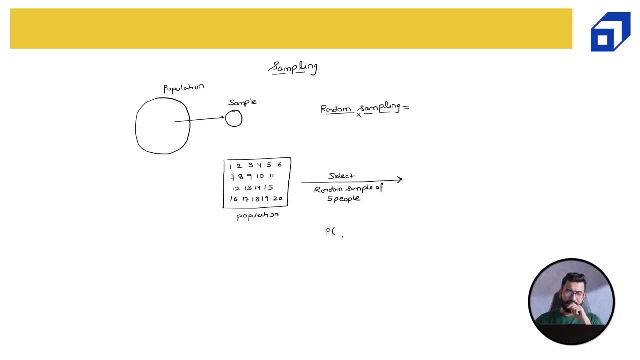 random sampling, the probability of selecting any observation is equal to 1 by n. So probability of selecting 1 is 1 divided by 20.. Probability of selecting 2 is 1 divided by 20.. And this is same for selecting any number: is 1 divided by n. 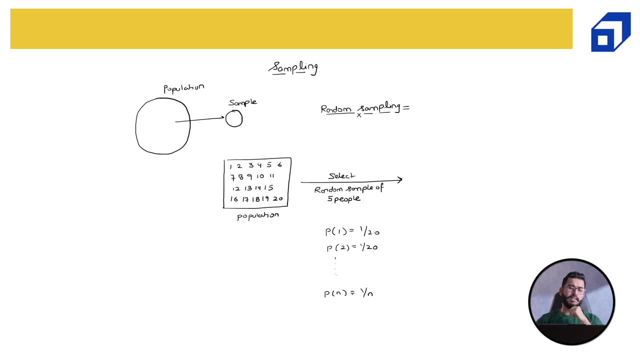 Which basically means in simple random sampling there is no bias. We will just randomly select any observation from a population, and the probability of selecting any observation in my population is 1 divided by n, Which is the same probability for every observation. So each observation in my data comes with same probability of 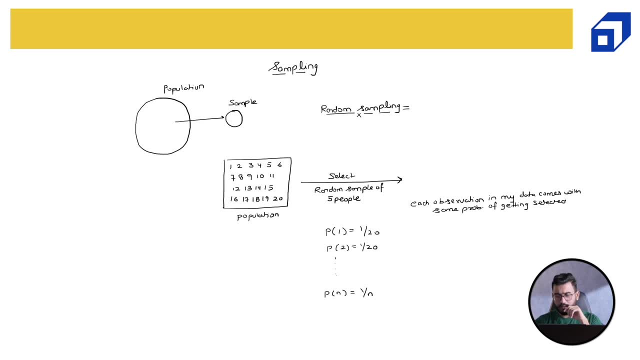 getting selected into the sample. So here my sample can be 5,, 9,, 2,, 7 and 10.. Now why I have written 5?? Why I have written 9?? I have just randomly selected these 5 numbers. 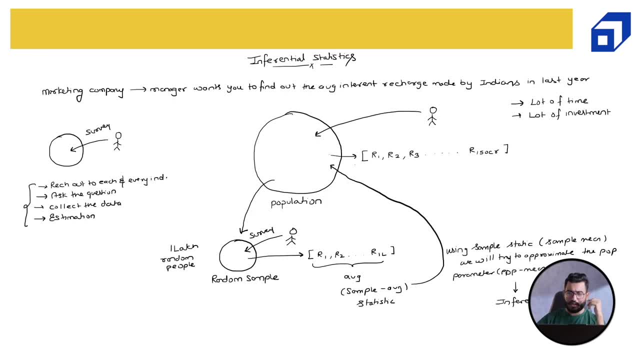 So this is simple, random sampling, And that is what I was talking about here: The simple, random sample. Okay, Now let's talk about how to perform, essentially, Estimation. In order to perform estimation, we use a particular algorithm, which is known as the central limit theorem. 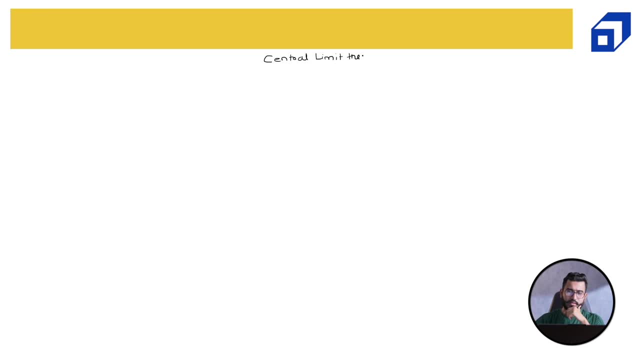 Central limit theorem. Now what this theorem talks about. This theorem states that if I am having a population- let's say this is a population of Indian people- Let's say I took one simple random sample of 1 lakh people. Now, when I calculated the average, 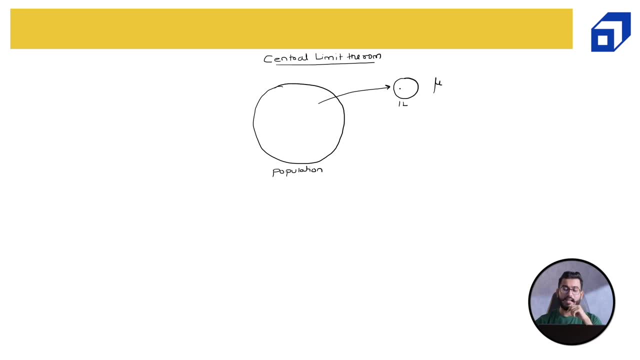 the average recharge amount for these 1 lakh people for sample number 1 came out to be, let's say, 250 rupees. For again, I took another sample, sample number 2, of another 1 lakh people. the average came out to be, let's say, 220 rupees. 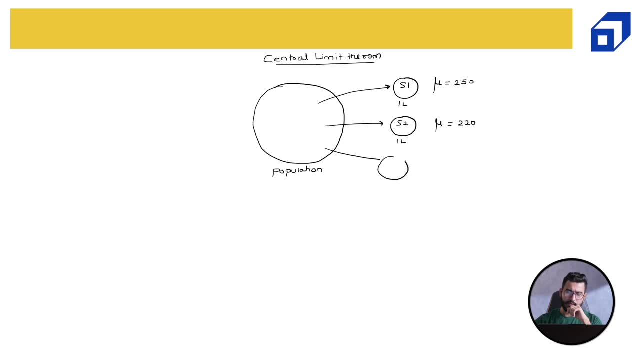 I again took one more sample, sample number 3,, again with 1 lakh random people. the average came out to be, let's say, 210 rupees. And like this, if I keep on doing, if I take enough simple random samples from my population, 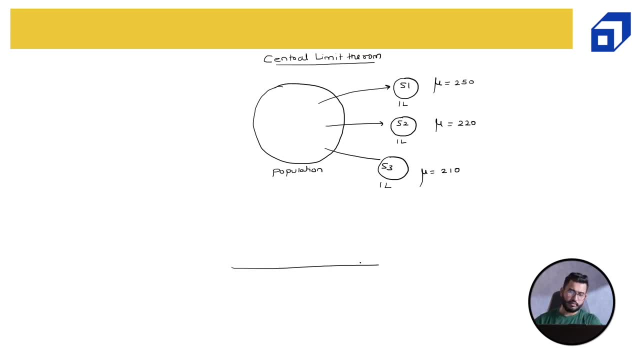 and I quickly plot them in a particular histogram, I'll get a normal distribution like this: I'll get a normal distribution where the average of this normal distribution is my population average And the standard deviation is given as sigma divided by root of n. 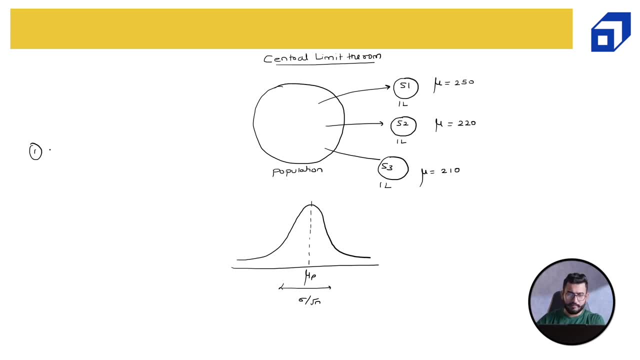 So the first property of central limit theorem is the average of all of all sample average. sample average will be approximately equals to the population average. The second property is the standard deviation of the sampling distribution is given as sigma divided by root of n. 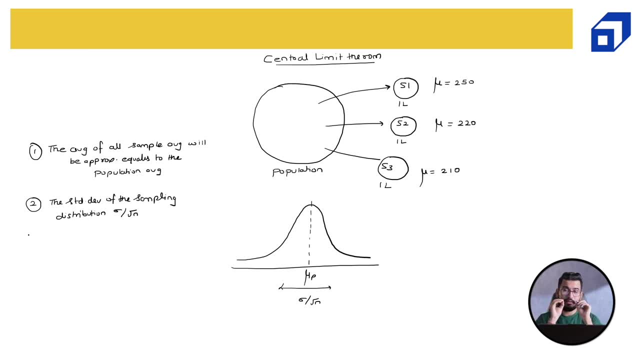 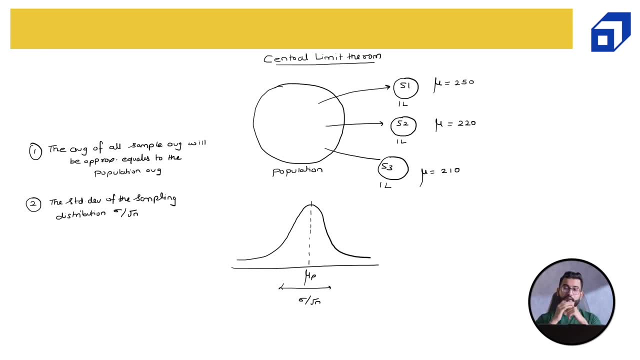 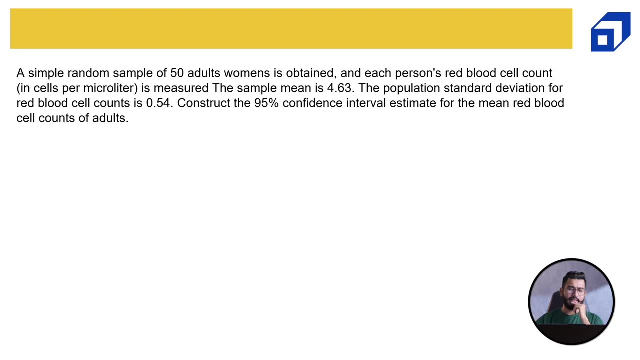 Using these two properties, we can estimate the population range. Let's try to understand how we can estimate the population range. Let's say this is the question that is given to us. In a simple random sample of 50 adult women is obtained. 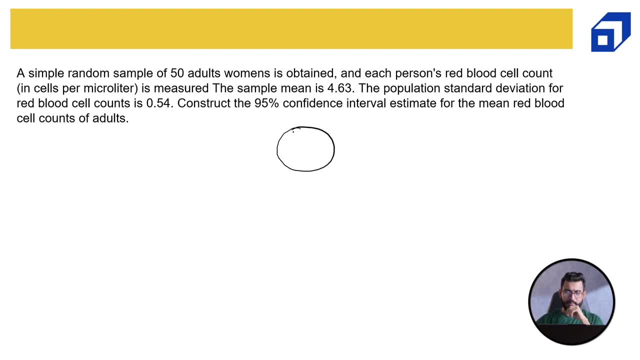 So I have a simple random sample. this sample is having. n is equal to 50 women, And when the red-blade cell count was made, And when the red-blade cell count was made, cell count was measured for them, this sample average came out to be 4.63.. The population: 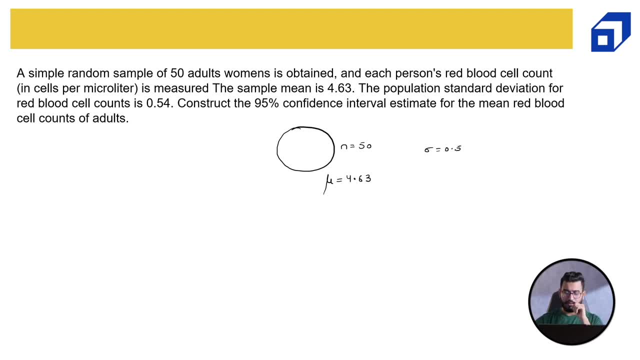 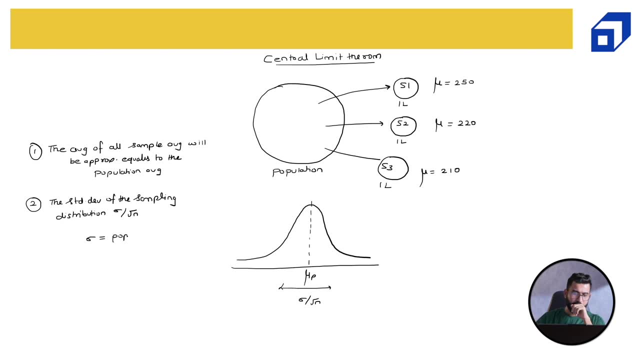 standard deviation is 0.54.. Now let me go back, and I was. I did not specify that this sigma represent population standard deviation And this n represents the number of observations in the sample. So in this case it would be 1 lakh. So central limit theorem states that the average of 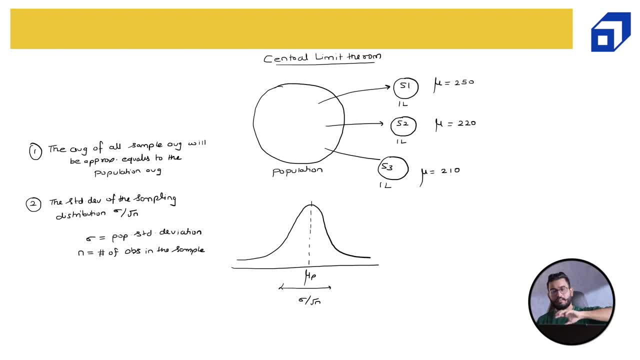 all these sample average. so I've taken multiple sample sample, I have taken multiple samples from my population. These are my multiple samples. These are my multiple samples- 123, and so on, And if I take the average of all these sample average, it will be closely equal to the. 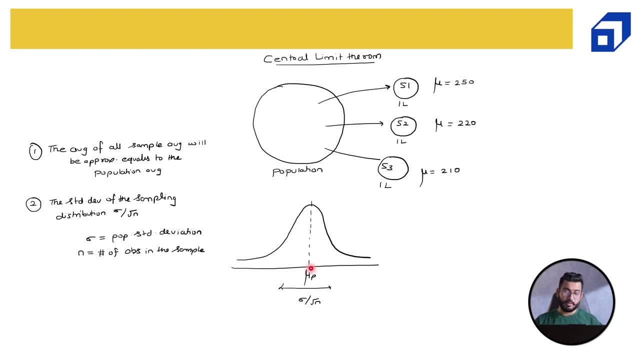 population, mean a population average, And if I plot them, if I plot all these sample means in a distribution, in a histogram, it will closely resemble a normal distribution And the this, this is this distribution- is known as the sampling distribution. This distribution is known as the. 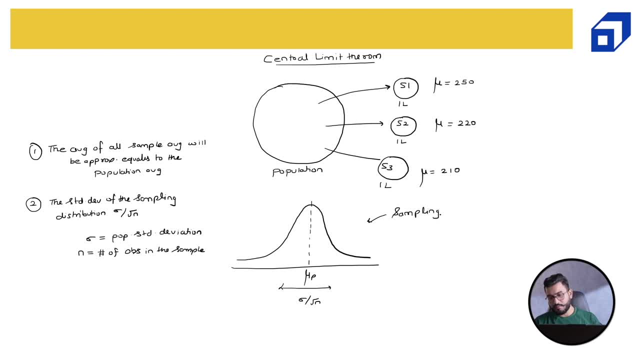 sampling distribution. by sampling distribution because we have obtained it using the sample means. So these are my sample means. Now, central limit theorem states that the average of all the sample mean will be closely equal to the population mean And the standard deviation of the 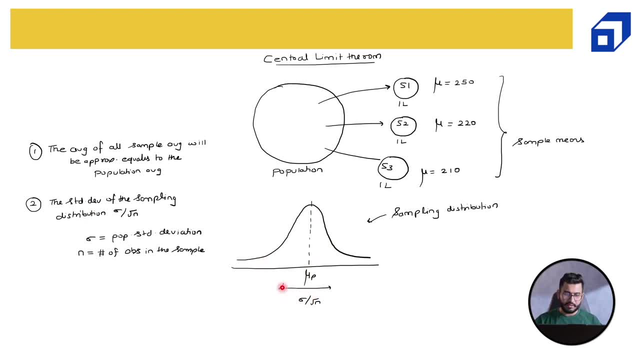 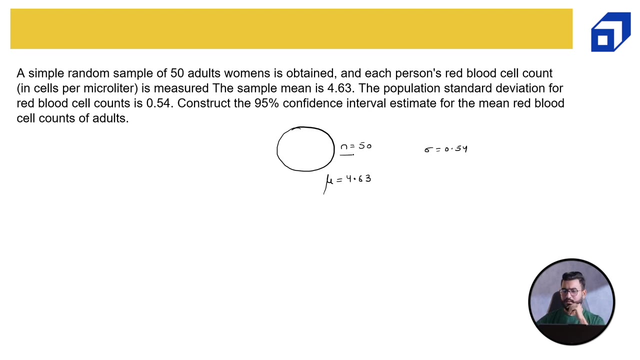 sampling distribution is sigma divided by root of n, where sigma is a population standard deviation and is the number of observations in the sample. Now this property is very important and very useful to estimate the population range. So I'm given with n as 50.. My sigma population standard deviation is 0.54.. My average sample mean is: 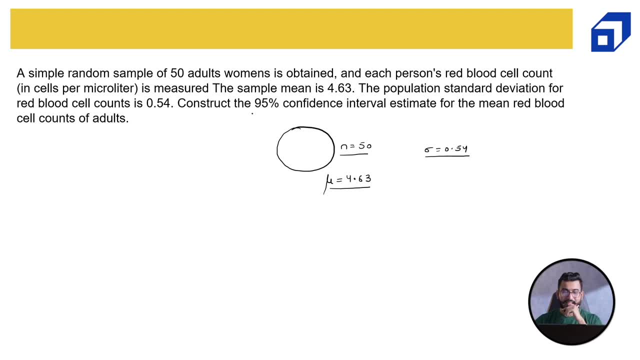 0.4.63.. Now I have to construct 95% confidence interval estimate. We already know that a sampling distribution follows a normal distribution. This is my sampling distribution for this particular, for this particular event. So I know that my sampling distribution follows normal distribution. Let's say this is my mu, which is sample mean, And I want 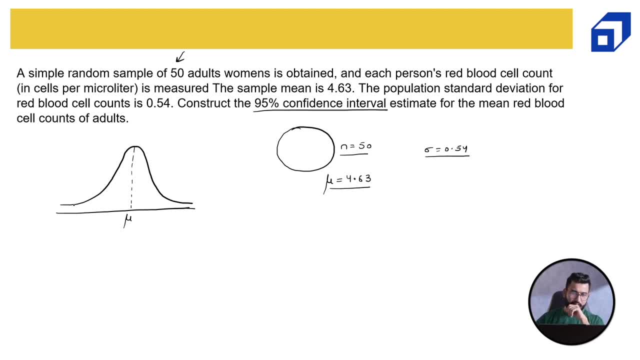 to estimate this range- lower value, upper value- in such a way that between these two I get, between these two I get 95% of my data. Now, don't worry, I'm not rushing. Don't worry, I'll explain you everything, But this is my, this is my problem statement. 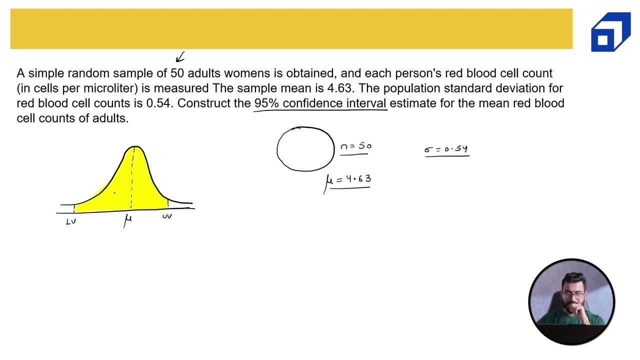 I have to estimate the lower value and the upper value in such a way that between this I have 95% confidence. I've right now. we are using the word confidence, But as of now you can use the term that I need lower value and upper value in such a way that 95% data is between these two values. 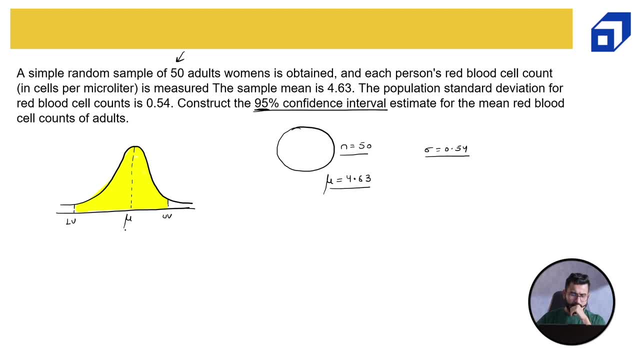 As of now, you can use the term that I need lower value and upper value in such a way that 95% data is between these two values. two values, Now, we already know this. actually that from the mean, if I go below two standard. 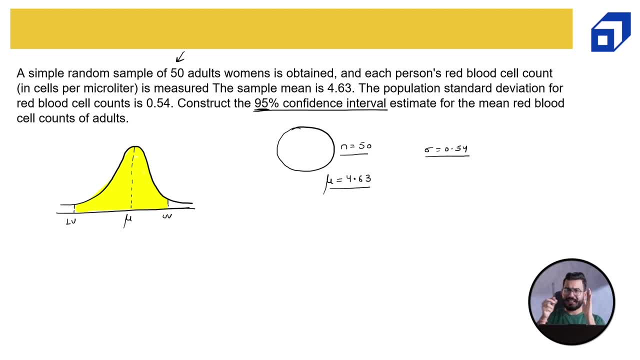 deviation and above two standard deviation. I can get 95% of my data using the second property of my normal distribution, right? But that is not exactly two standard deviation below the mean. I'll just tell you. assume that. assume that this is my standard normal. 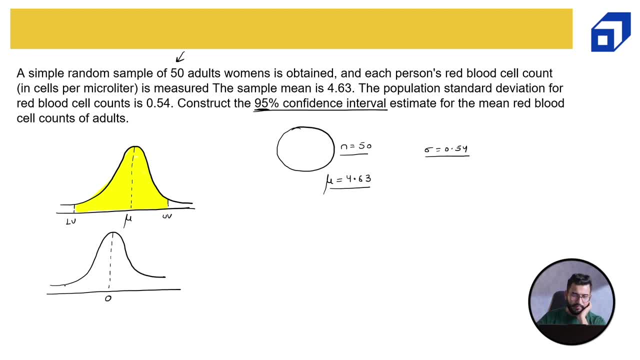 distribution mean zero And I have to find out. I have to find out the Z value over here. What is the Z value over here And what is the Z value over here, Z1 and Z2.. And assume that between Z1 and Z2, the area is below the mean. 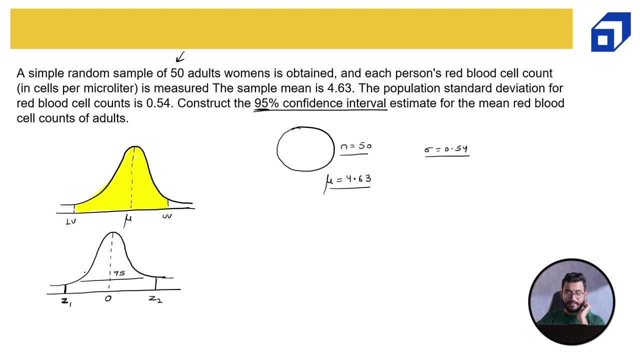 If the area is 95, so if the area is 95, between Z1 and Z2, this area, this black color area, what that will be, what that will be. So the total sum of these two black area will be 5%. So this will be 0.025 and this will be 0.025.. How So total is one Between. 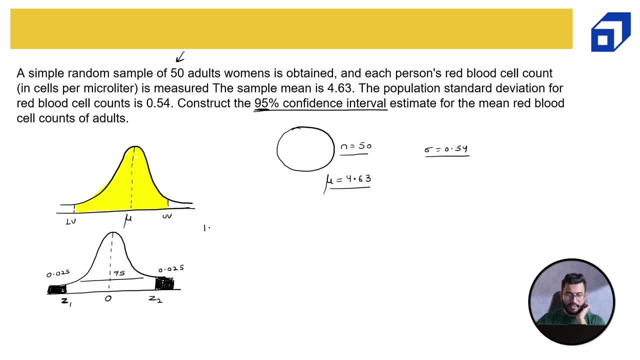 these two data points, Z1 and Z2, my area is 0.95.. So I'll subtract, So I'm left with 0.05.. Now, since I'm having two shaded regions, I will divide it by two, So I'm left with 0.025.. So half is over here. 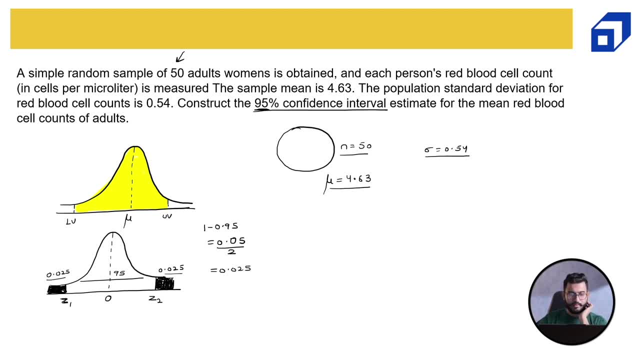 and half is over here. Now I have to find out the Z value over here. So from here to here, the area under the curve is 0.025.. Let's quickly use our Z table. So 0.025, I have. 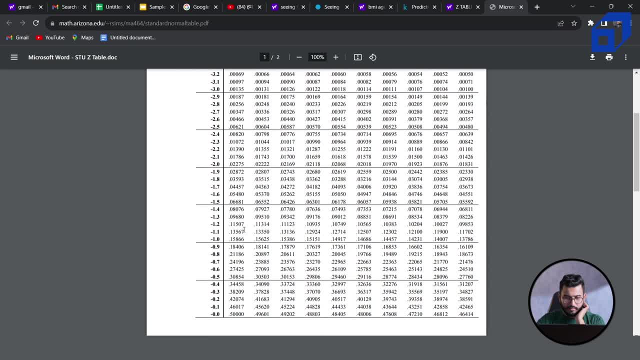 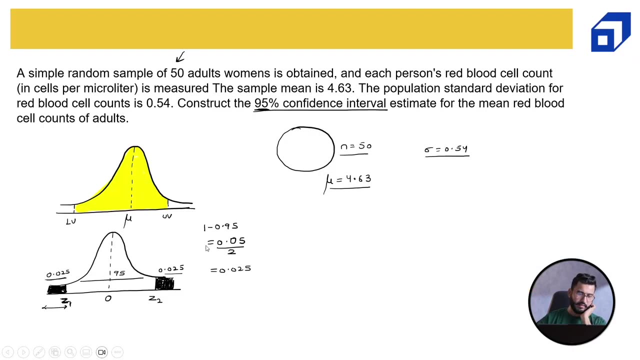 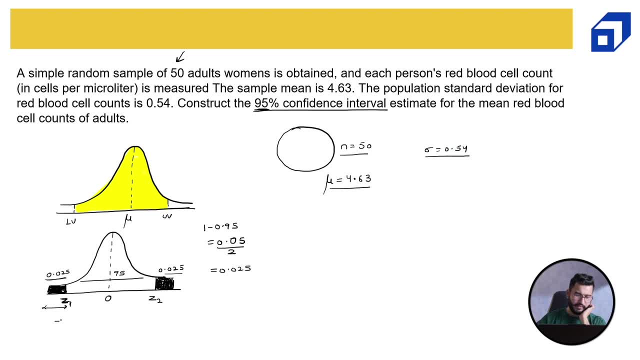 1.96.. This point, Z1, is minus 1.96.. Similarly, to find out Z2, I have to go from here all the way up to here, So that will be 0.95.. This is middle region plus 0.025.. So that. 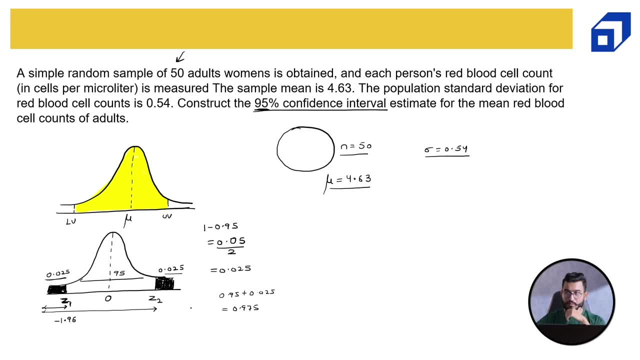 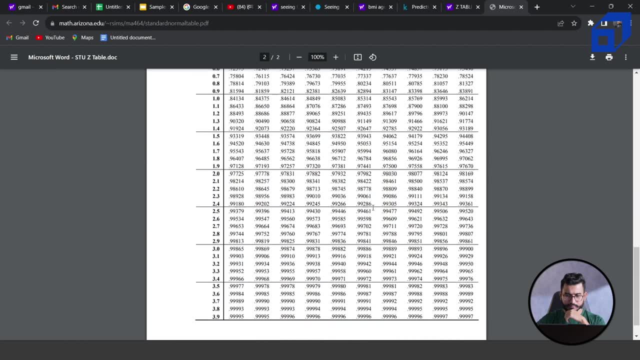 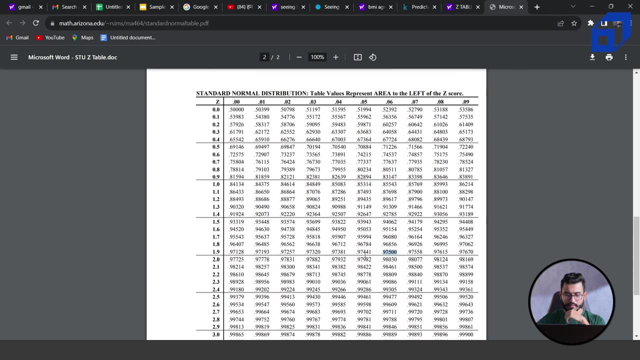 will be 0.975.. So let's look at 0.975.. So 0.975.. 0.975 is over here. This is plus 1.9 and 6. So we have plus 1.96.. Now we have the lower. 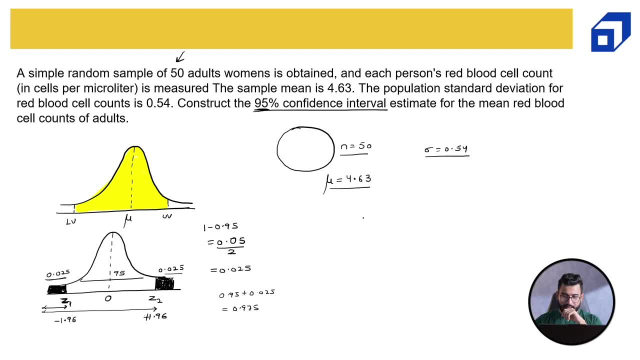 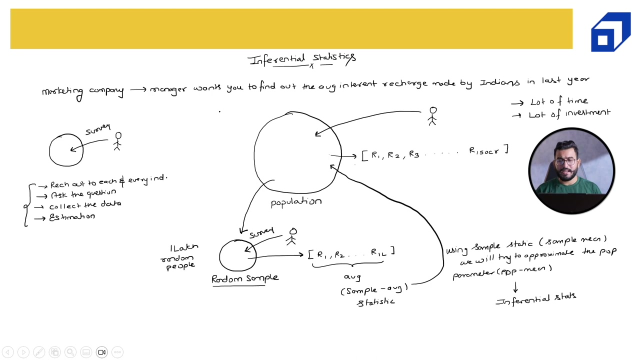 Z value and upper Z value From the sample mean to estimate, to estimate population range or population parameter range. Why am I estimating a range? Because if my manager is asking me to find out average recharge made by the Indians and if I'm using sample mean, I'm not 100% sure right. So I cannot tell my manager that the sample mean was for, let's say, 280 rupees. 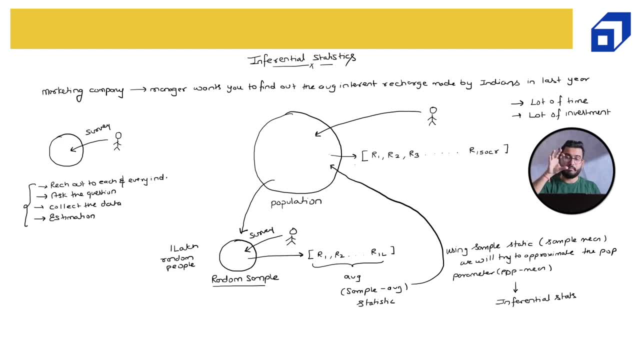 Because I have just analyzed one sample, I have just surveyed one sample, So I have to tell my manager, with a range, that I can tell to my manager that, okay, sir, I don't know exact value, but I'm sure I'm 90% confident, or I'm 95% confident that my population mean lies somewhere between these two values. 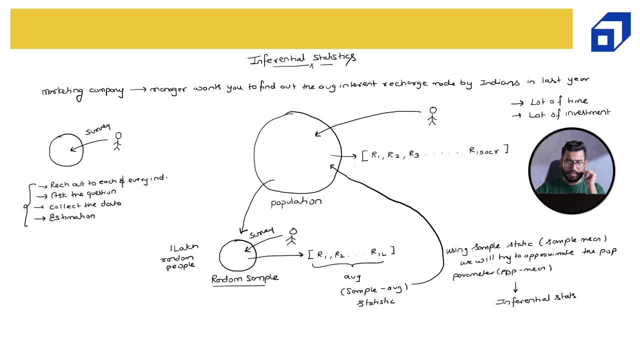 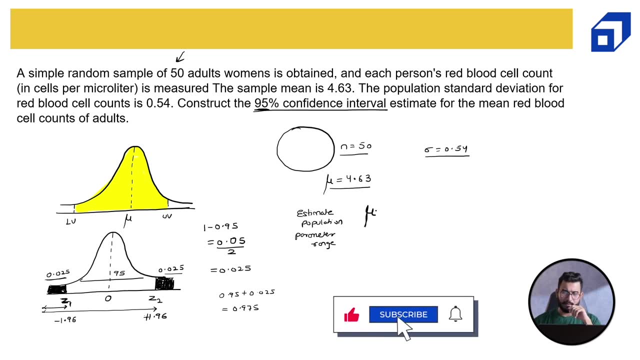 So that is what we are trying to estimate. So if I go back to my question, To estimate the population parameter range in my sample mean, this sample mean, we will add and subtract the z times of sigma divided by root of n, What is z. So from this value I'm moving 1.96 standard deviation below the mean, 1.96 standard deviation above the mean of the standard deviation of the standard deviation of my sample. 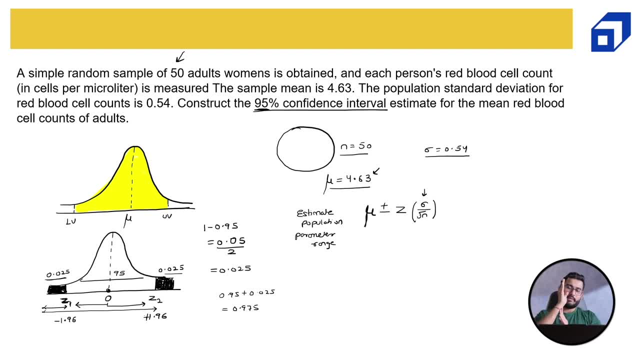 So essentially what we are trying to do, from the mean, from the sample mean, we are just moving below and above, below and above. So to get this lower value and the upper value- So this is my mean- In order to get 95% confidence I will move minus 1.96 standard deviation below, plus 1.96 standard deviation above the mean and that will get me the population range. So mean is 4.63. 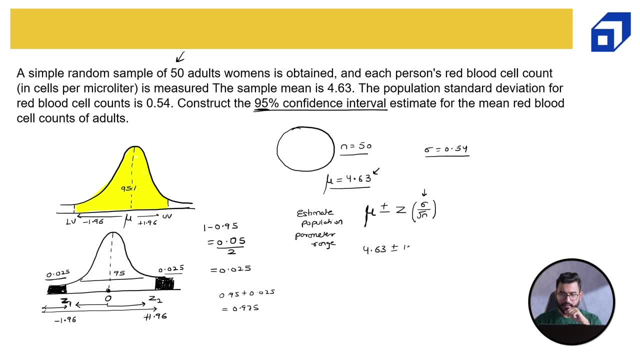 Plus minus 1.96. standard deviation is 0.54 divided by sigma of root 50.. If I solve this- 4.63 plus minus so- this will come out to be 0.149 and the range would be 4.481 comma 4.779.. What is the meaning of this? This basically means that there are 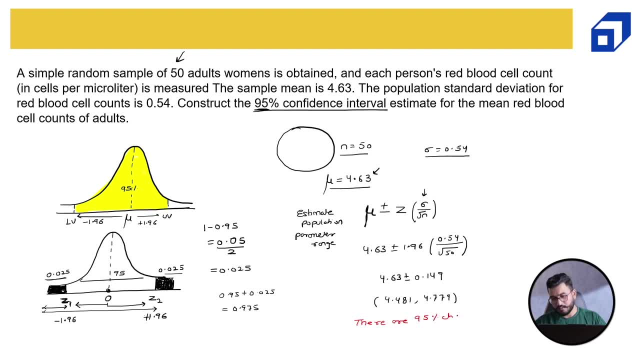 90% chance of that the actual population mean would lie. 95% chances that the actual population mean would lie somewhere between 4.481 YouTube 7, 4.77 9.. between 4.481 YouTube 7, 4.77 9.. 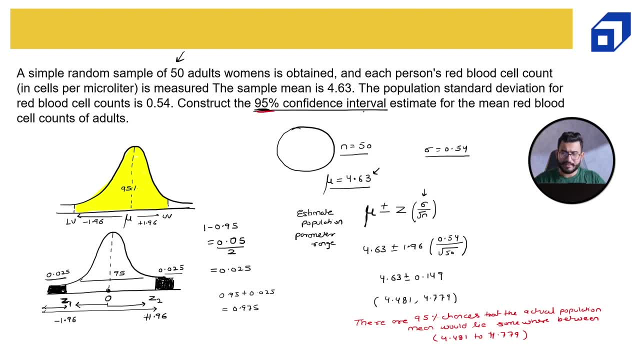 was asking me construct 95% confidence interval estimate for the mean of red blood cell count of the adults. so right now, 50 adult women's were taken and their sample mean was 4.63. but if we talk about the complete population, complete population of adult women's, then this range states that there are 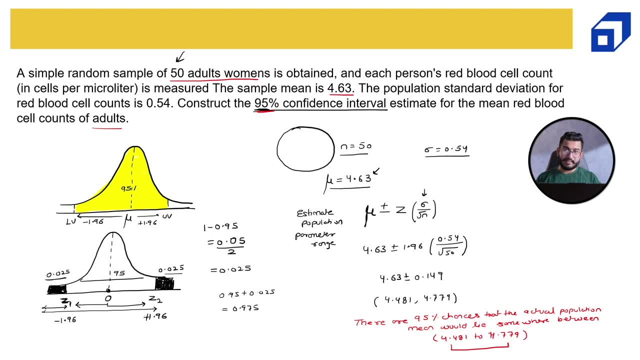 95% chances that the red blood cell count of the complete adult one woman population, which would lie between 4.48 to 1 microliters, to 4.779 microliters. that is what this range is. let's look at one more question and then it will it. 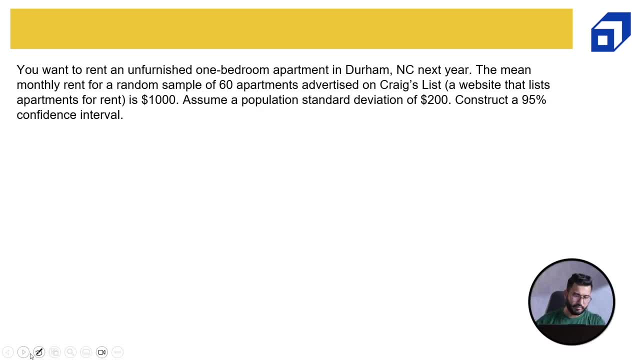 will clear all your doubts and it will be very clear to all of you. so the question says: you want to rent an unfurnished one-bedroom apartment in New York City. the mean monthly rent of random sample of 60 apartment advertised in some website came out to be $100. so what you did? you are trying to estimate what is. 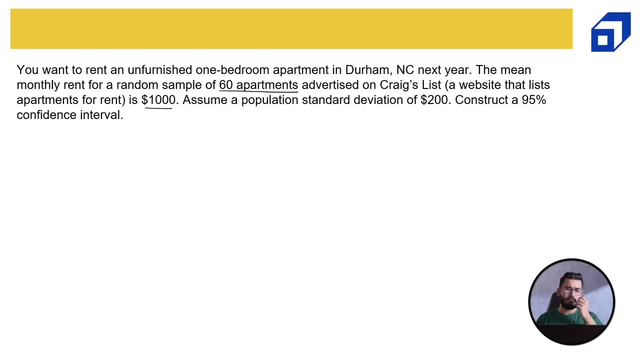 going to be the average one bedroom cost or average one bedroom rent in New York City. so what you did? you googled and you searched through some website. you sampled 60 apartments in the same city. so 60 apartments- my n is 60- and after looking at all the all the rent, the average of this sample came out to be: 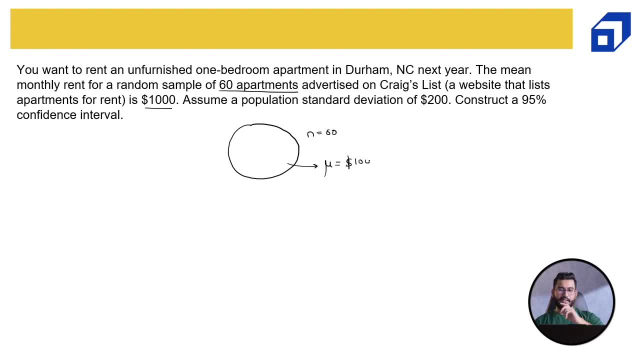 $1,000 and the standard deviation was. you assumed that the population is time deviation to be $200. so this is just an assumption. population standard deviation is $200. this is population. now we have to construct 95% confidence interval. again for 95%, we have already calculated the Z values. so 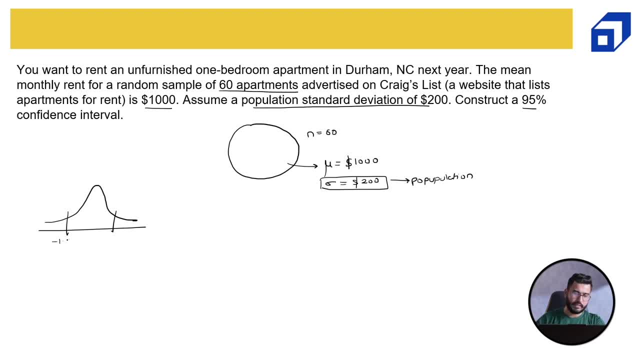 the Z values is minus one point nine six plus one point nine six. so we will just apply the formula: mean plus minus Z times of Sigma divided by root of n. mean is 1000 plus minus one point nine six. Sigma is two hundred divided by root of 60, and if I just quickly solve this, it will came out to be nine. 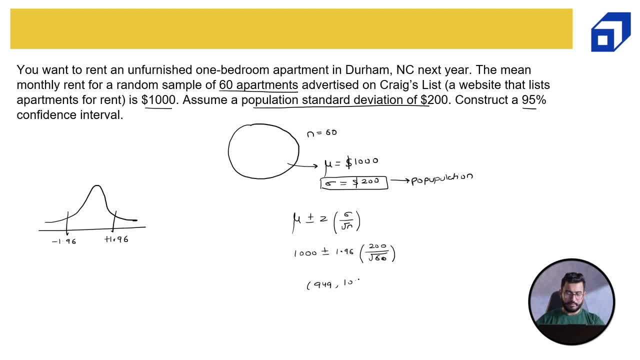 forty nine, comma one zero, five zero, which basically mean there are 95% chances that the actual rent of one bedroom, one bedroom apartment in New York City would be somewhere between nine, forty, nine dollars. two one zero, five zero dollars. and this is what the application of inferential a statistics is. I hope you guys. 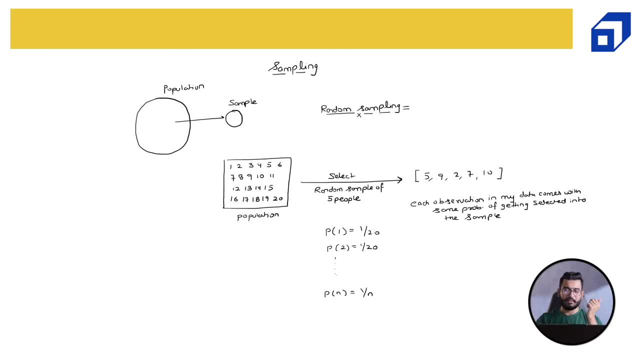 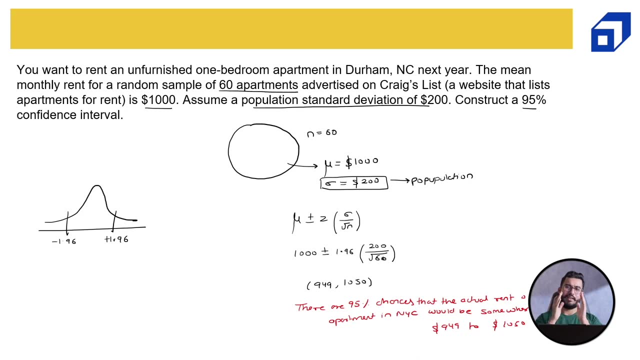 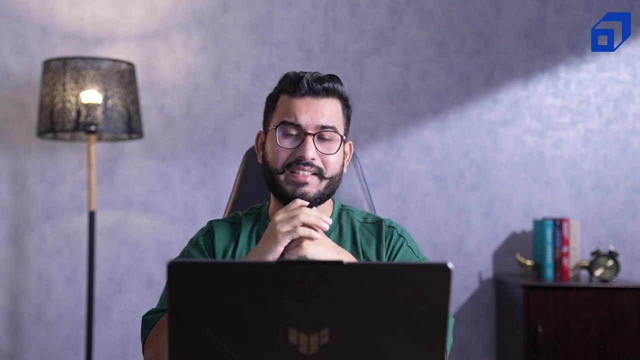 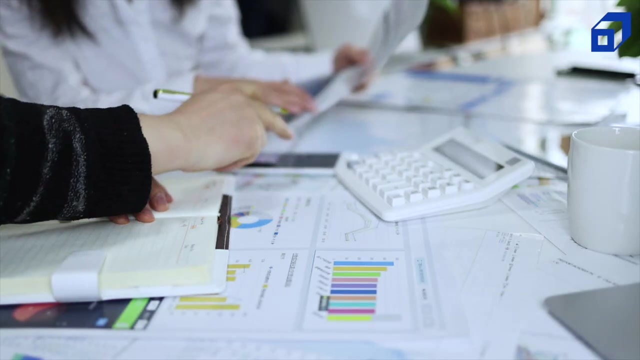 are able to understand this, to connect all the dots, and able to understand how we have arrived to this particular point Now. this concludes our discussion in inferential statistics. So till now, we have talked about descriptive statistics, we talked about probability and we have also looked at how we can use inferential statistic to approximate the population parameter. 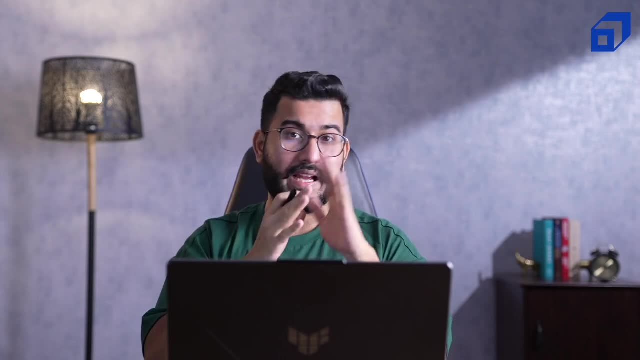 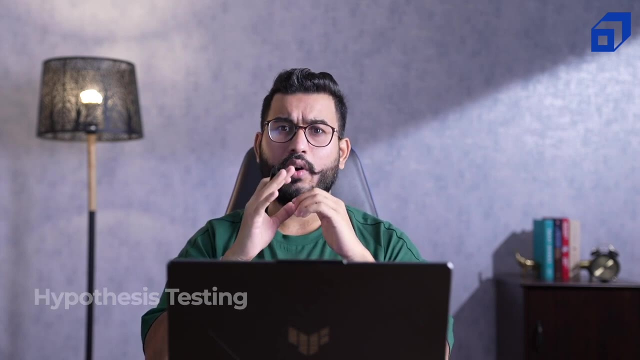 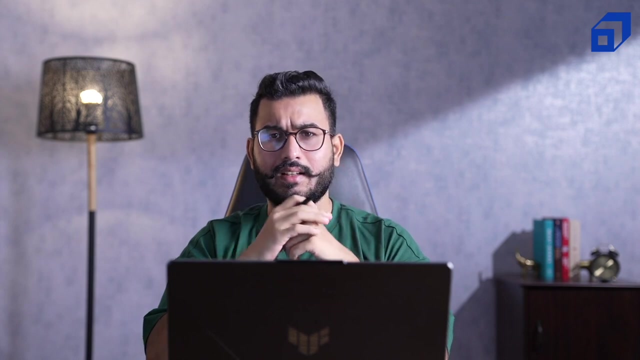 given the sample statistic. So this is all what we have covered. Now we are going to start with hypothesis testing. Now I have already given you a brief idea behind what hypothesis testing is. So when we started this video, we briefly discussed about all the three major buckets. 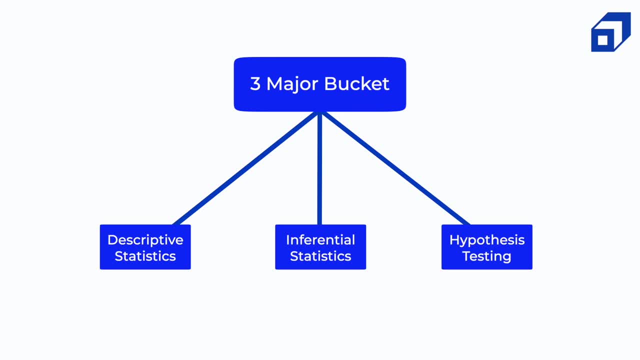 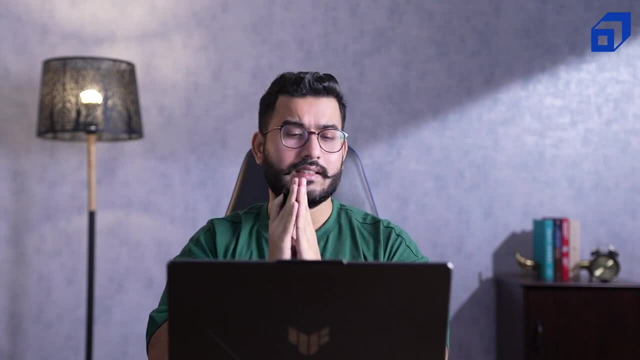 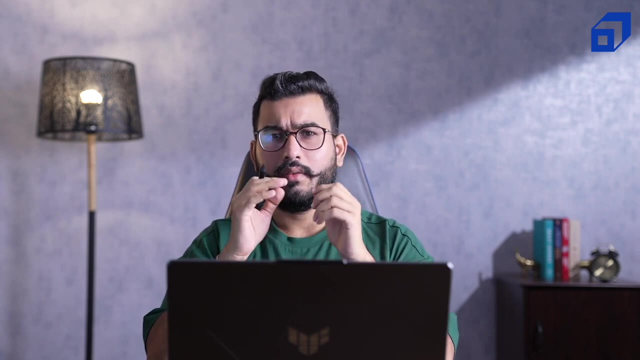 What is descriptive statistics? What is inferential statistics? What is hypothesis testing? But in this section, we are going to have a detailed conversation regarding what exactly is hypothesis testing and how this can be useful when it comes to data science or when it comes to data analysis. 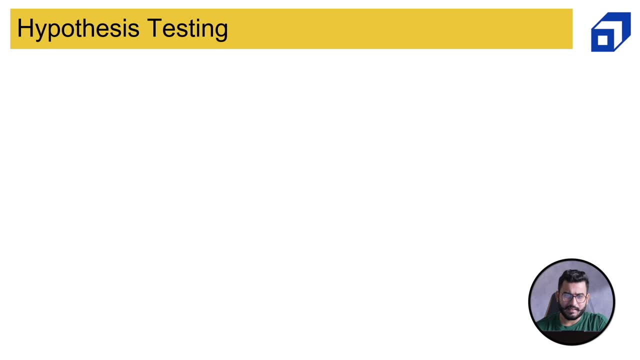 So let's start this discussion Now. to understand hypothesis testing, we will take one example. So let's say there is a code, So let's say this particular person is a judge sitting in the code, So judge in the code, and we have two lawyers and we have the person who has been convicted. 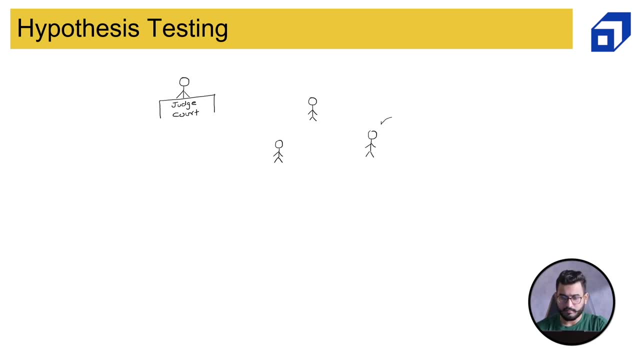 So this person is being charged, charged for some crime. Let's say this person is talking in English. Let's say this person is talking in English. Let's say this person is talking in English favor of the convicted person and this person is the against the person. Now, if 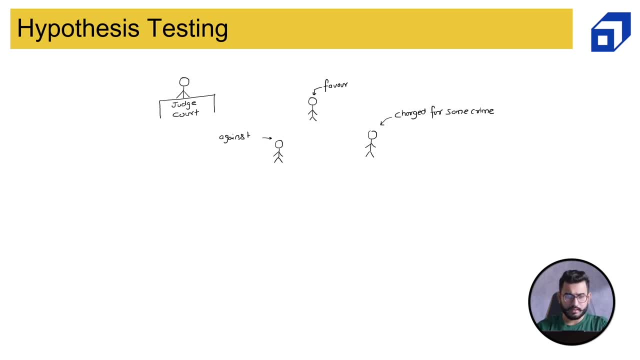 I ask you what will be the thought process this judge will be having in his or her mind regarding this particular person who has been charged for some crime. you guys can easily say that the judge will be having two assumptions or maybe two hypotheses or two thought process. if I, if I tell you like, if we 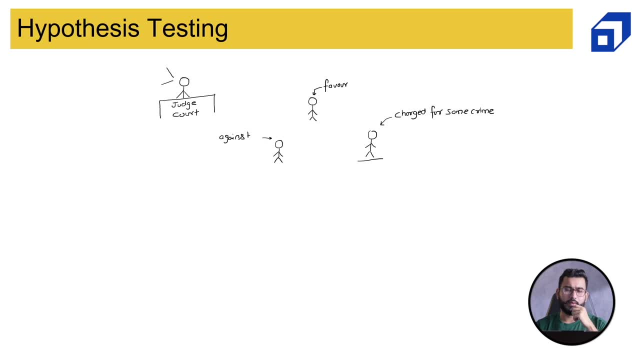 think in general English it would be two thought process: either the person is guilty or the person is innocent, right? so that is what the judge will also be having in their mind. so either the person is guilty or the person is innocent. now judge will decide after listening to both the lawyers of the particular lawyer who is talking in. 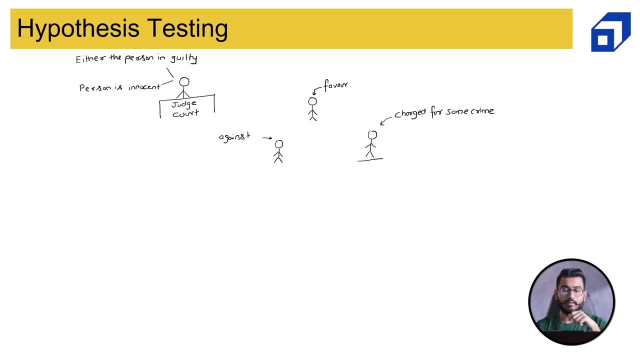 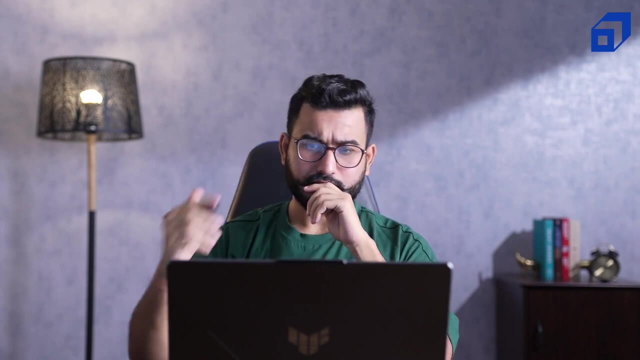 favor of the charged person and then another lawyer who is talking in favor or in the against the charged person. so the judge will listen to both these parties and then they will declare or they will come to a particular conclusion. right now, this is basically you can say. this is basically the. 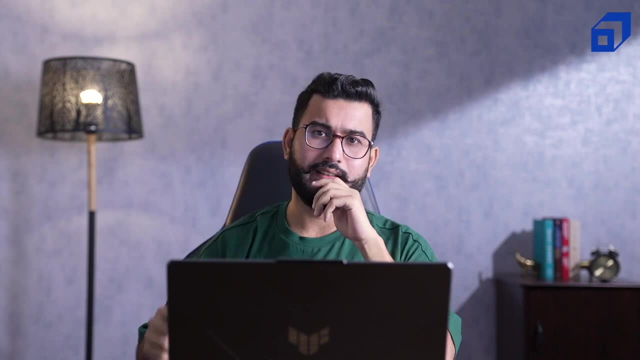 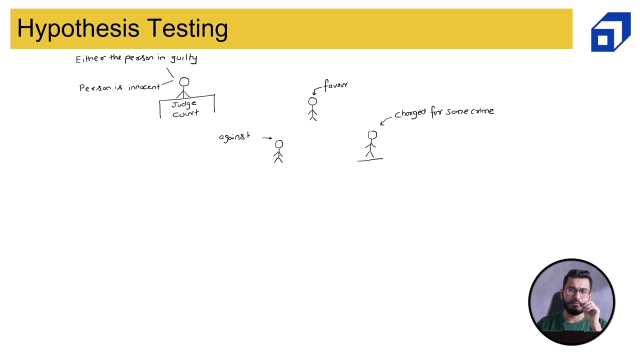 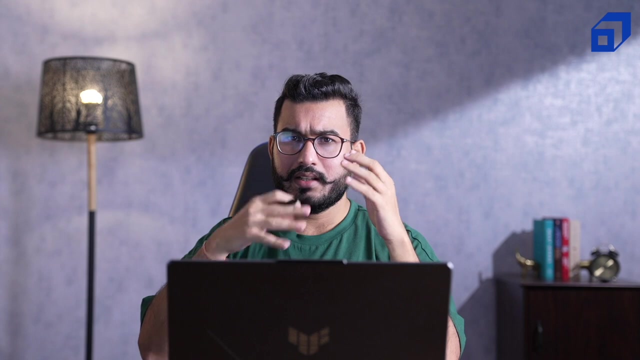 framework of what hypothesis testing is. so in hypothesis testing we have two thought process, two assumptions, and we try to conclude, we try to prove one of them. this is a very raw definition. this is not hundred percent correct, but the reason I am talking in this way is because I wanted to create a base of what exactly is hypothesis. 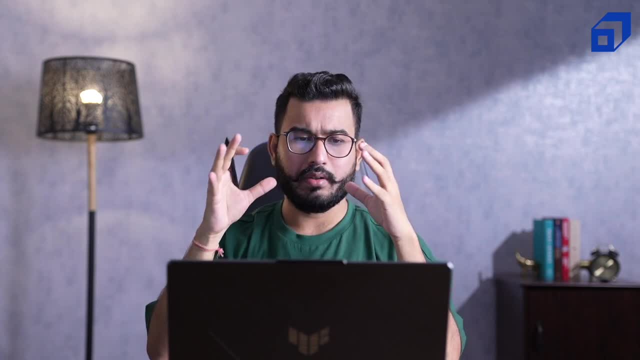 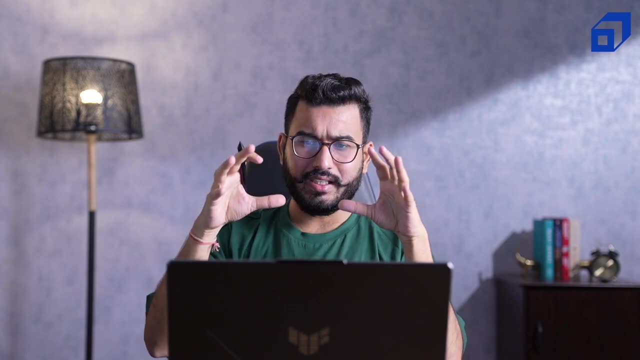 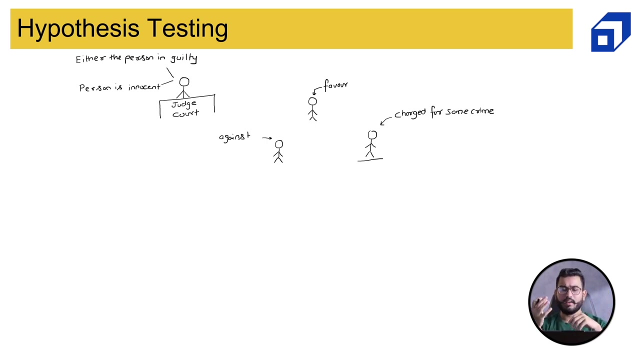 testing. so just keep this example in your mind and whenever somebody is asking you what exactly is hypothesis testing, you can just say that this is a hypothesis testing. you can just generate this picture in your mind: that there is a courtroom, there is a judge who is listening to both the lawyers, one in. 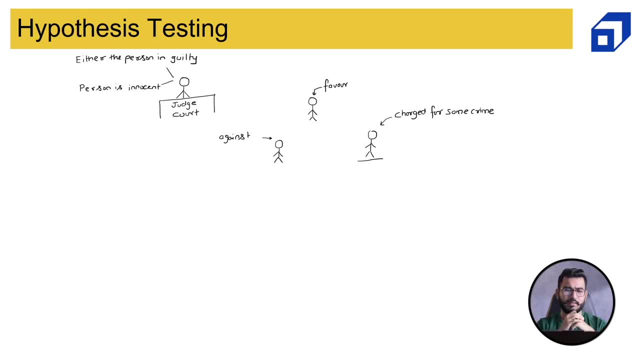 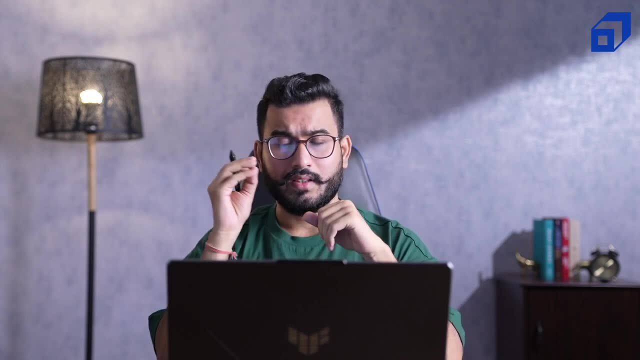 favor and one in against, and there is a convicted person. now either the person is guilty or the person is innocent. these are the two hypothesis that the judge will be having in their mind. after listening to the whole whole conversation between these two lawyers, the judge will come to a conclusion, and that is what. 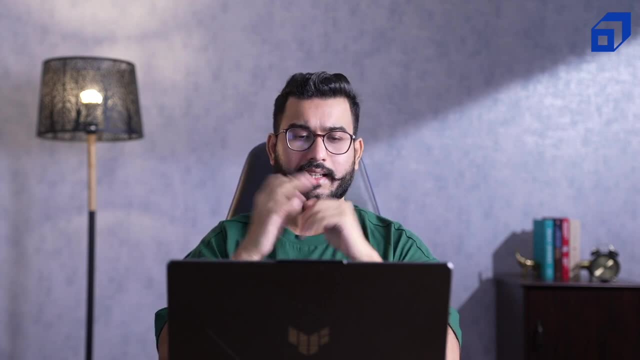 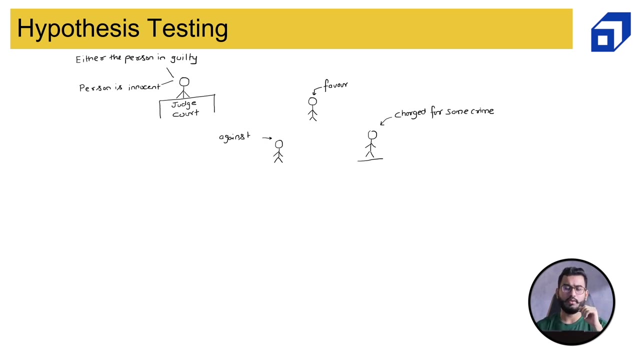 the conclusion which we are trying to achieve right. so the complete hypothesis framework is having two stages. number one is to formulate the hypothesis. so, given a problem statement, we have to formulate the hypothesis. so formulation, formulation of the hypothesis. and number two is the test. So we will perform the test to reject or to fail to reject one of the 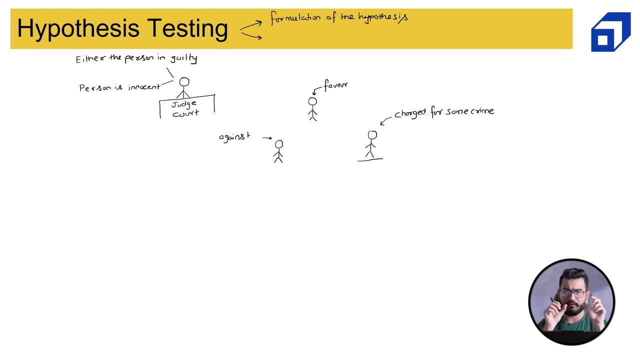 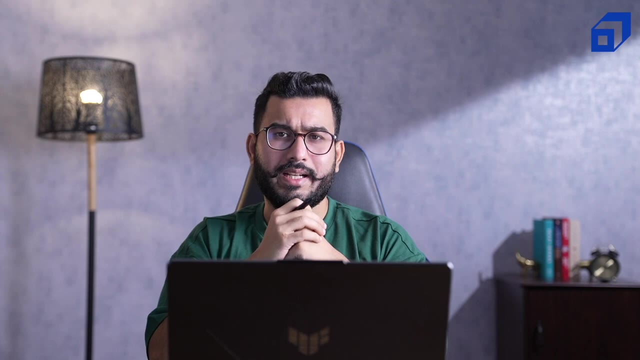 hypothesis. now please don't worry about the term which I have just said- reject or failed to reject- but just remember that we will first formulate the hypothesis given a problem statement. so let's say your manager has given you a problem statement, you will first formulate the hypothesis and then you 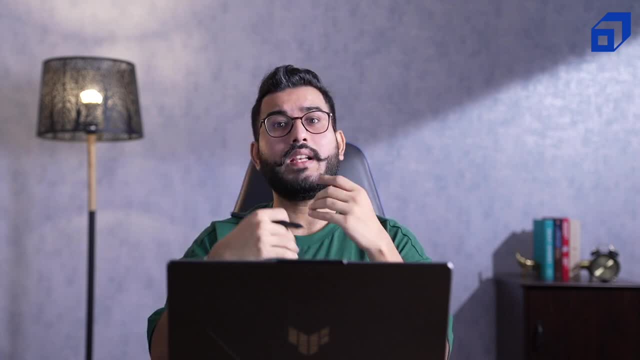 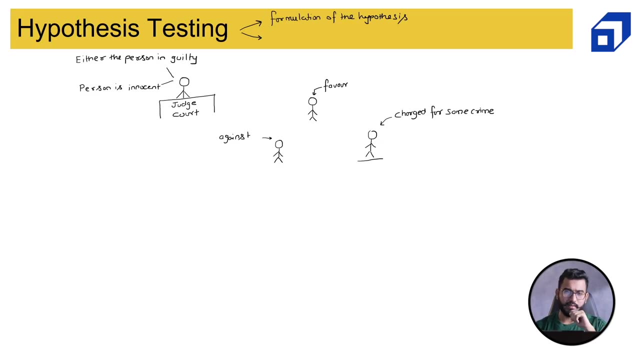 will perform the test. Based on the test result, you will make some conclusions. So this is the simple process of hypothesis testing. So the next step is testing or performing test and then, finally, conclusion. Now let's understand the formulation of hypothesis, As I just told you that this judge, this judge, would be having two thought processes in his 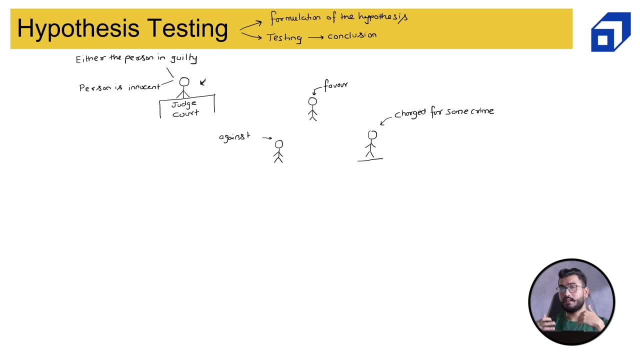 mind or in their mind: either the person is guilty or the person is innocent. Now there is a formal word or there is a formal name given to these two thought processes. One is known as the null hypothesis and another one is known as the alternate hypothesis. 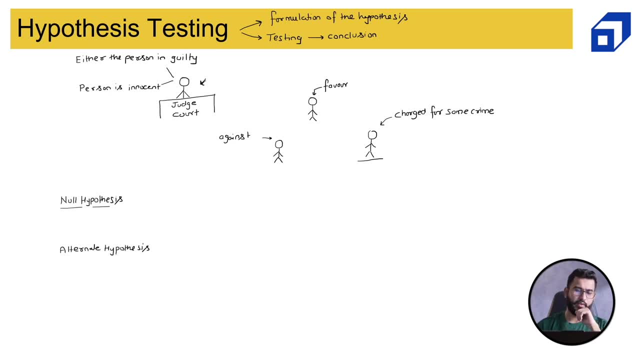 null and alternate hypothesis. now, what is null hypothesis now, if i ask you, before this person was charged, charged for some crime, before this person was taken to the court, initially this person was innocent, right? so null hypothesis talks about the initial state of anything or initial state of the particular, uh, particular item or particular case. that 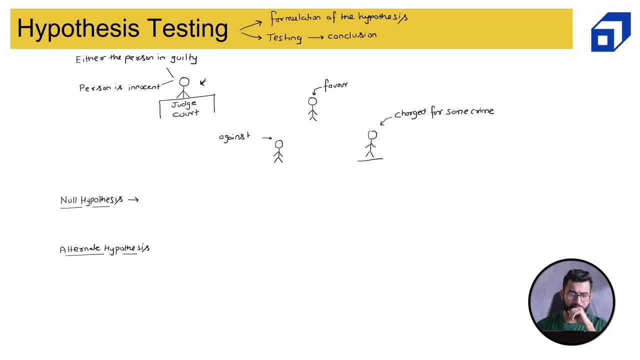 we are trying to test. so null hypothesis is basically the initial state of the case. this we are trying to test, so the initial state of this person is that this person was innocent before this person was taken to the court, before this person was charged for some crime. this person 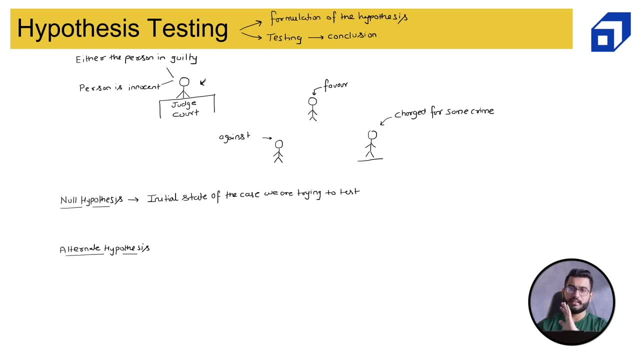 was innocent. before anything happened to him he was innocent. so so my null hypothesis is: this person was innocent. before anything happened to him he was innocent. this person was innocent, um. the person is so h naught, so null hypothesis can also be represented as h naught. 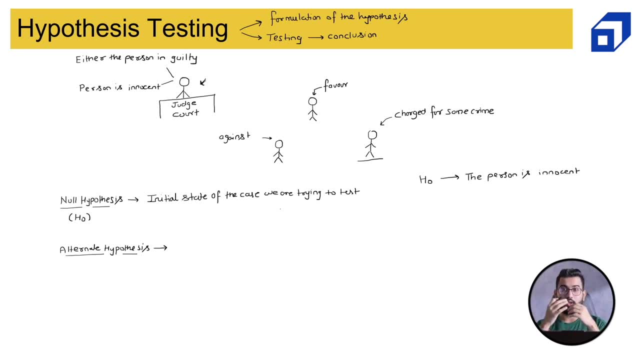 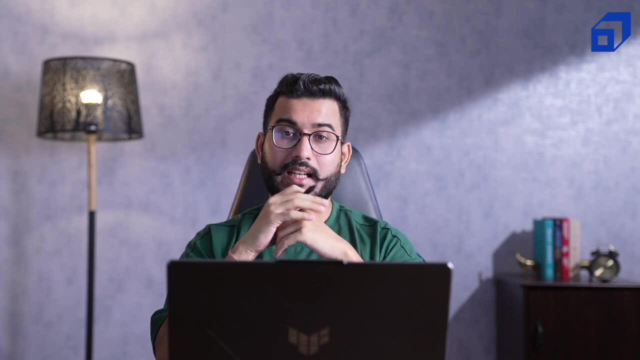 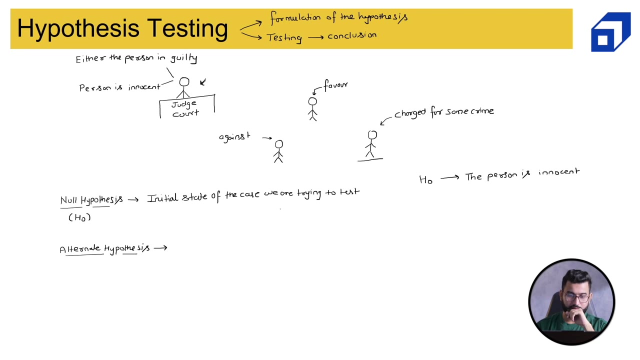 the person is innocent. now the alternate hypothesis is: what new thing spend to this person is this person has been charged for crime. now, So this is the new thing, or new state or the claim of the case. we are trying to test, we are trying to prove. 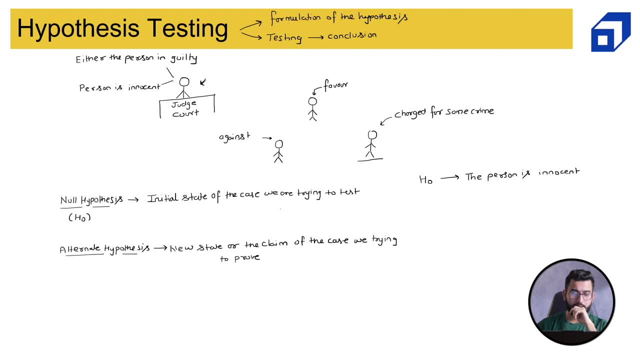 So HA alternate hypothesis can be represented as HA and in this case it will be. the person is. the person is guilty. So this is how we can formulate the hypothesis. Please remember: null hypothesis represents the initial state of the person or initial state of the case. 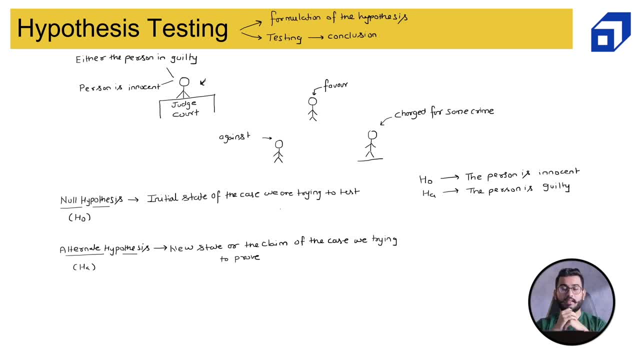 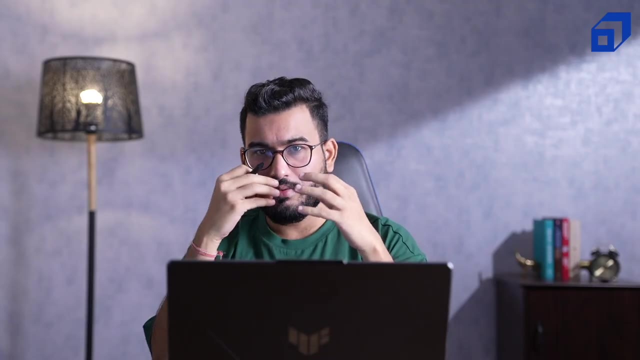 which we are trying to test and alternate. hypothesis is basically the state of the person, Basically the new finding, the new thing or the new happening for the particular case which we are trying to prove or which we are trying to test. Let's take few examples just. 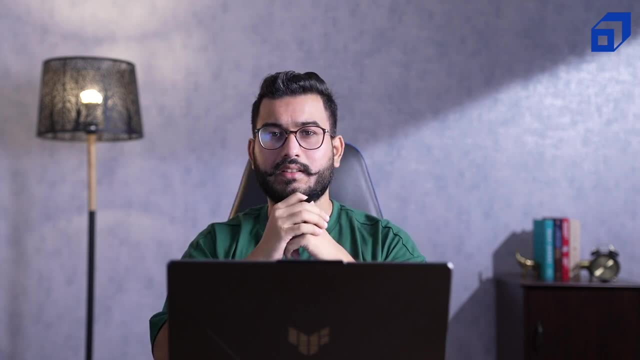 to understand how we can formulate hypothesis given any problem statement. So right now, this was not the problem statement, This was a very plain example. but now we will be looking at some problem statements which will have some sample, mean, population mean, standard deviation, to understand how we can formulate the hypothesis. Now, before we talk about some business examples, 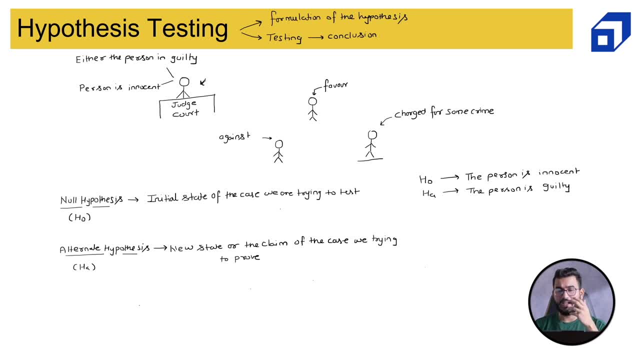 to better understand how to formulate the null and alternate hypothesis. we will understand a very small topic which is really important when we conclude. So whenever we conclude the hypothesis testing during conclusion, we say that we reject null, or either we say that we fail to reject null. 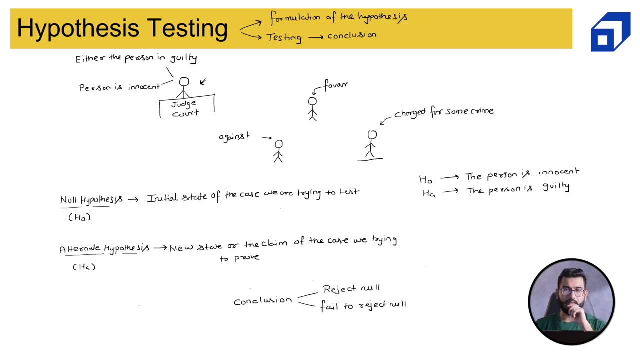 Now we never say that we accept null or we accept alternate. So what we never say, We never say, we never say we accept null or we accept alternate. Now there is a reason for this. So this is the something which I should mark in red color, because this is wrong. 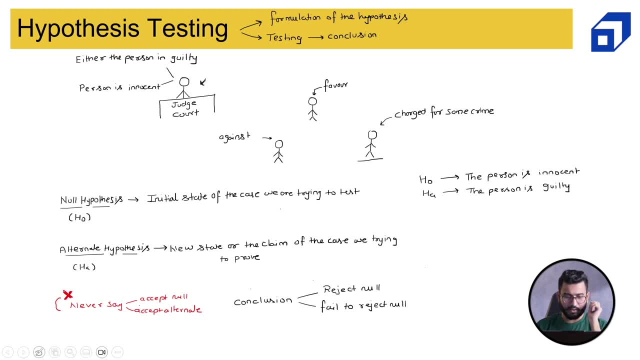 We never say this: Thank you. Now, the very first thing that we should understand is: why are we only rejecting null and fail to reject null? Why it is only null, Why it is not alternate? Well, the reason is because null hypothesis is something that we know, that we certainly know, So we are 100% sure. 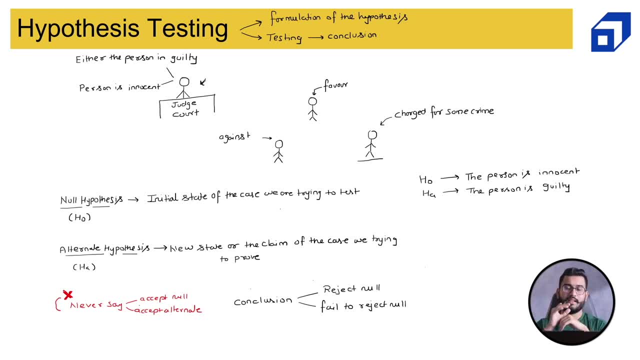 that this person was innocent before committing crime, Right, Right. So the reason why we conclude on the null hypothesis is because null hypothesis is the statement which we are certain about. We know that initially, this is something which actually happened. The person was actually innocent and we are certain about it, We are 100% certain. 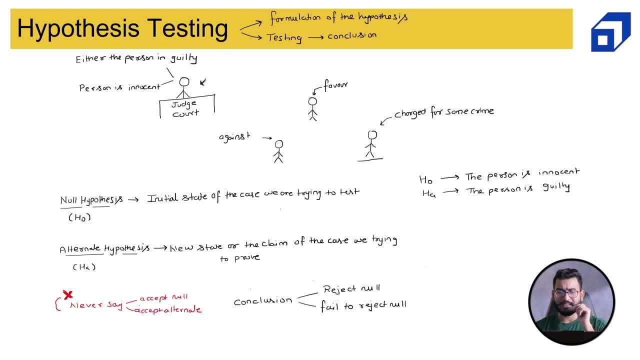 Okay about it. Now why we don't say except null? If I say except null, we are completely ignoring the fact that the person was guilty. Now, it might be because of the lack of evidence. So if I say I except null, I am 100% sure that the person was innocent. It might be because 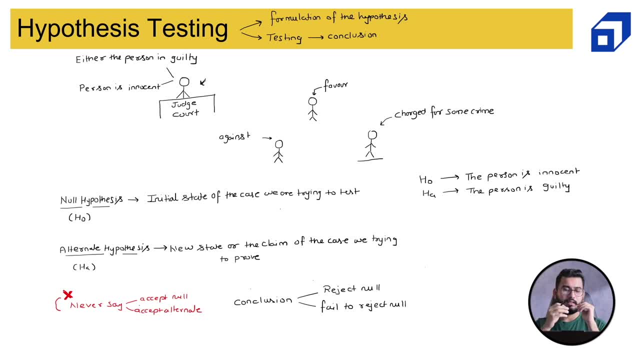 of lack of evidence. So let's say, this person who is talking against the charged person, he was not able to present enough evidence against the court, due to which he was not able to prove that the person is guilty. So when I say that I except null, I am basically: 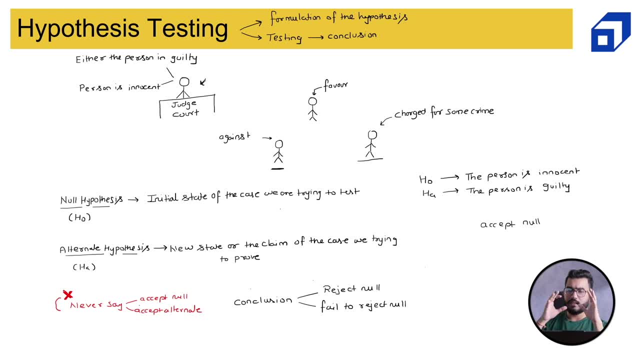 ignoring the fact and I am 100% sure that the person was innocent. So when I say that I except null, I am basically ignoring the fact and I am 100% certain that that this person is innocent, and I am ignoring the fact that this person is guilty, which is: 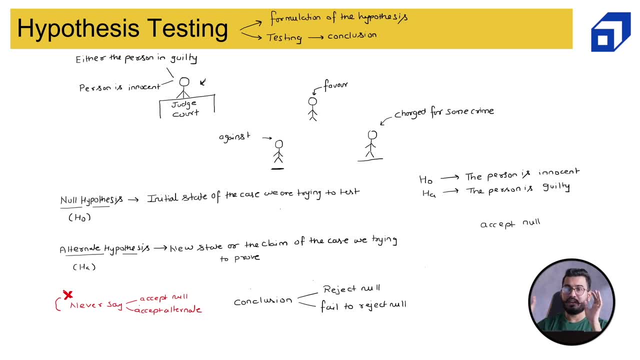 not true. We have to be uncertain, We have to keep some uncertainty. So the uncertainty is the lack of evidence. We, when we say that I reject null, I'm saying that I'm rejecting null, but I'm not saying I'm accepting null. Rejecting null means I'm I'm not a hundred percent sure. 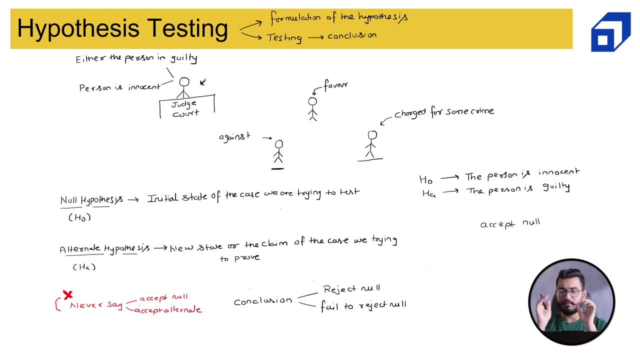 And it might be because of the lack of evidence. Now, when I say, when I say when I, when I say except alternate, the reason why I don't say except alternate, So except alternate, basically mean that I'm a hundred percent sure that the person is guilty. Now again this: there is a 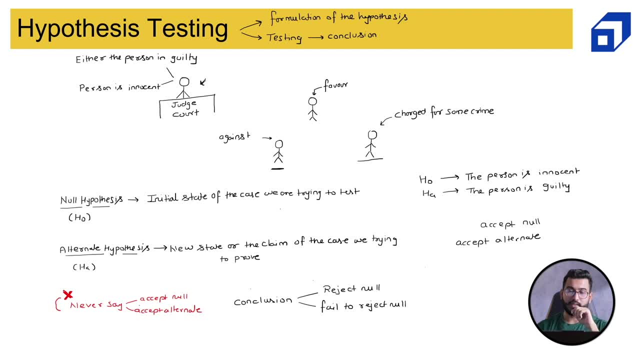 there might be the lack of evidence. The person who is talking in favor of this person was not able to collect evidence: Adams, Okay, Okay, evidence to prove that this person was innocent or this person is innocent. so again, when we say we accept alternate, we are completely ignoring the fact that 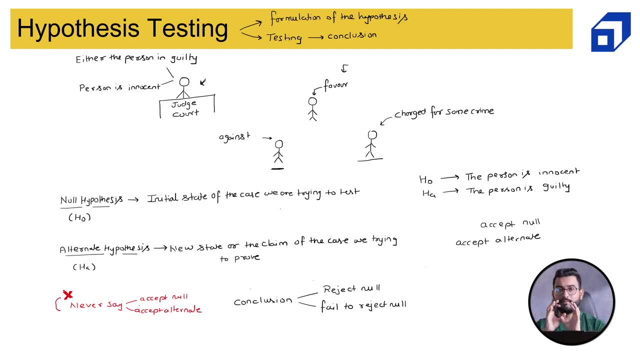 there is some uncertainty that can happen. so, in order to make sure that while we are concluding something, we have the uncertainty in our decision and there are chances or there are possibilities of other thing happening, because of the lack of evidence, we only say that we either reject null or we 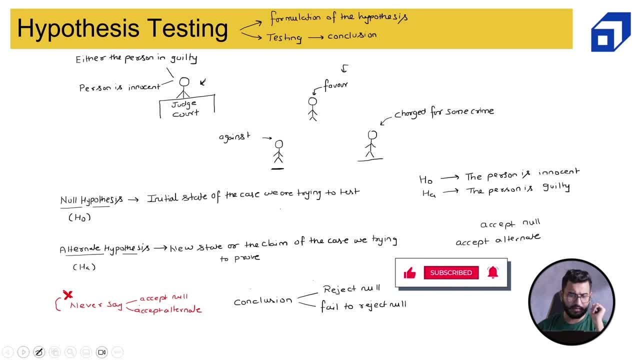 fail to reject null. I hope this makes sense. if it is not making sense, just remember one thing: we we only say reject null or fail to reject null. we only use the null hypothesis because we are hundred percent sure that null was true. Null happened. Null happened in reality. This person was innocent in reality. 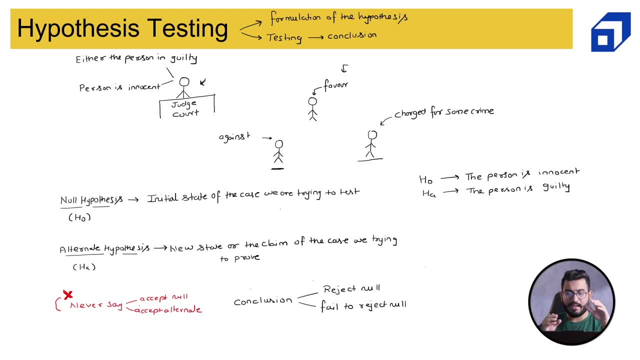 That is the reason we use null. The second reason why we do not say except null or except alternate is because there might be lack of evidence due to which I was not able to prove the statement. So in order to include the uncertainty in my conclusion, we only reject or fail to reject null. 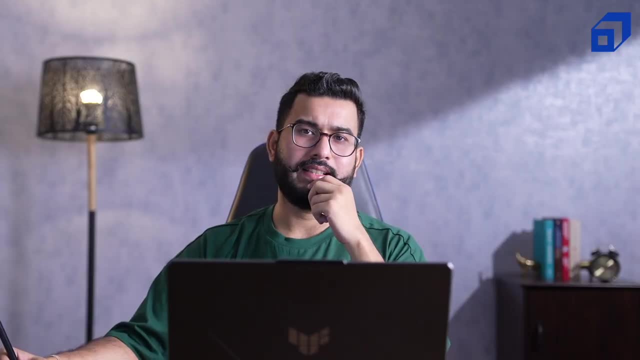 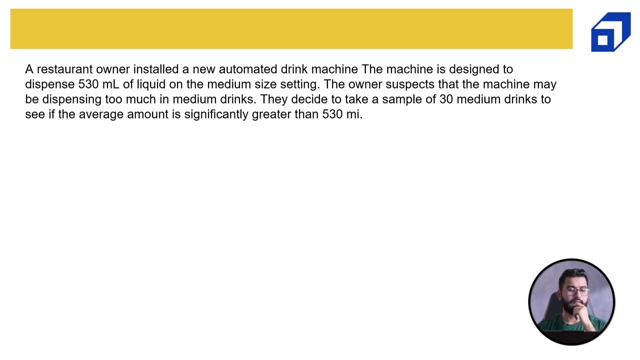 I hope this makes sense Now, given a particular problem statement how we can formulate the null and alternate hypothesis. So in this particular question it states that a restaurant owner installed a new automatic drink machine. The machine is designed to dispense 530 ml of liquid. 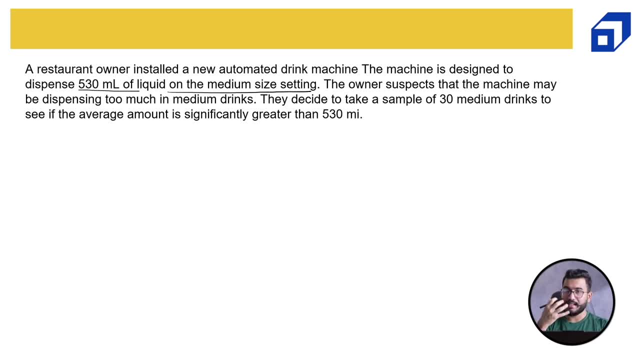 on medium size setting. Now, what is the initial state of this machine? So we know that the machine was designed to dispense 530 ml. This is the initial state of the machine. So let me just highlight this. This is the initial state of the machine. The owner suspects that the machine may. 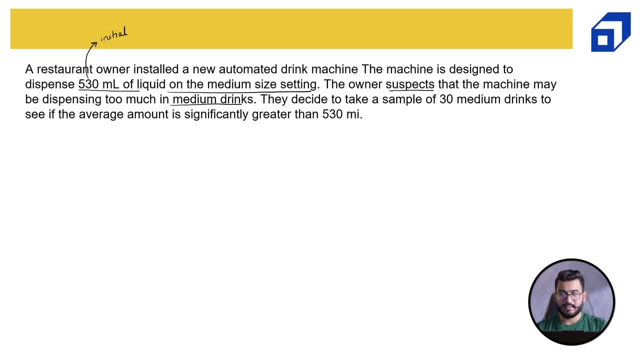 be dispensing too much in medium drink. They decide to take a sample of 30 medium drink to see if the average amount is single. Now what the owner wants to test if the average amount is greater than 530 ml. So this is the new finding. New finding. So my alternate hypothesis is that the average amount 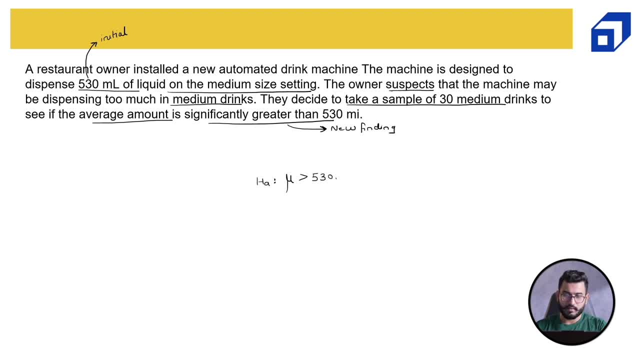 is greater than 530 ml. My null hypothesis will be: the average amount is less than or equal to 530.. Now why I am using less than or equal to. Now please remember: in the question it says the machine is designed to dispense 530 ml of liquid, So I should have written null as. 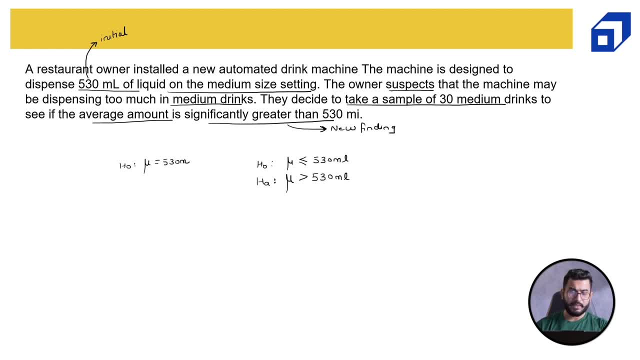 average is equal to 530 ml. But please remember one thing: I hope you guys remember when we were talking about continuous random variable and the distribution of continuous random variable, We know that the point probability is zero, So is equal to 530 ml. Let's say this line: this line is 530 ml. 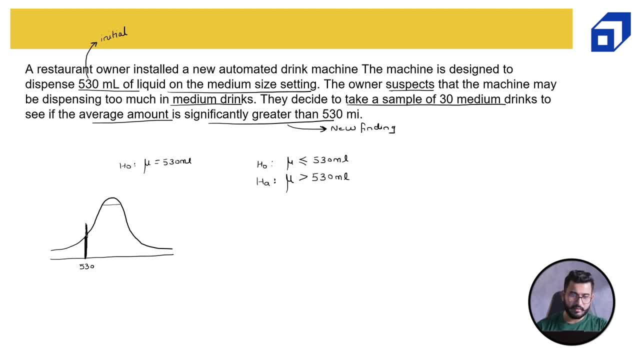 Now greater than 530 ml? is this region Above the line? everything is greater than 530 ml. This is greater than Now. if I use alternate as greater than 530 ml and null as is equal to 530 ml, I will never be considering this region the lower region, And that would not be helping us. 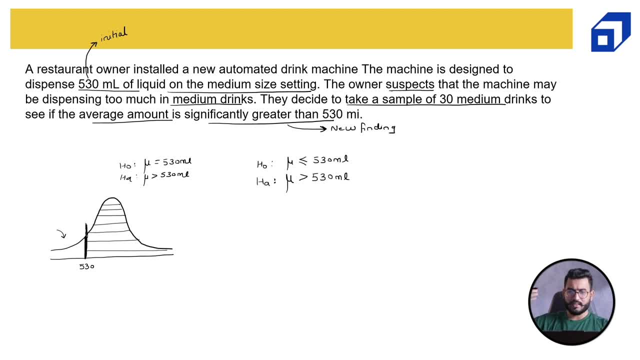 to arrive at a conclusion. So, for example, if I'm getting a value which is lying below 530 ml, then in that case, if I do not consider this area, I would not be able to conclude anything. So that is the reason, in order to make sure that I'm covering up the complete. 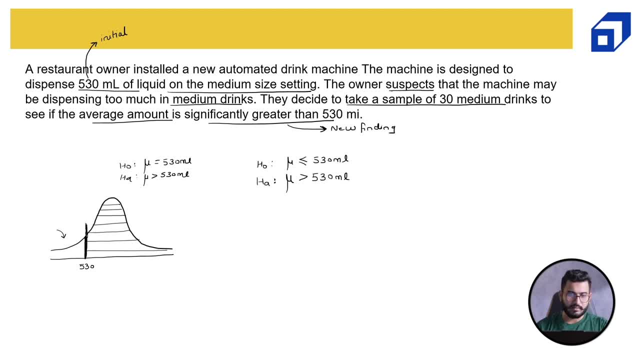 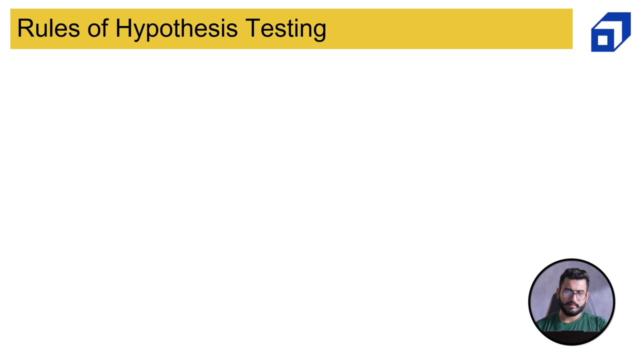 distribution we use less than or equal to, So we get this part also, And then we will be able to cover up the complete area under the curve. There is one rule also, the rule of hypothesis testing- that when we talk about or when we formulate the null hypothesis, 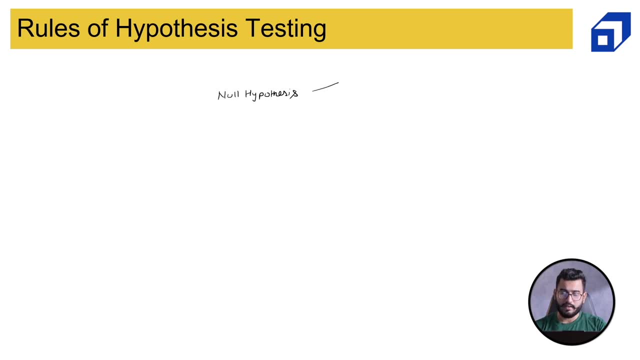 the null hypothesis, always will always have. they will always be having less than equal to sign, greater than equal to sign or equal to sign, While alternate will always have less than greater than or not equal to. This is rule number one. Rule number two is rule number three. 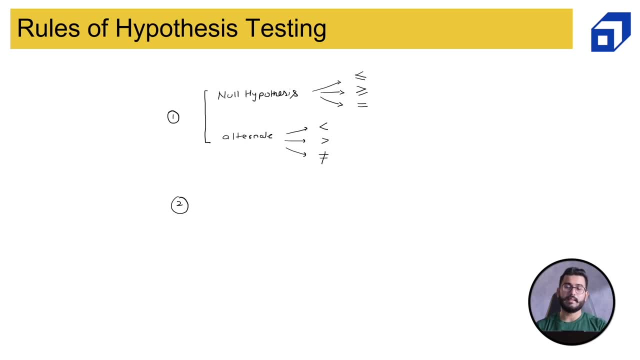 null and alternate are 100% opposite to each other. so null and alternate are 100% opposite to each other, which basically means: if, in my hypothesis formulation, if I get my alternate as less than, this will be greater than or equal to. if this is greater than, this will be. 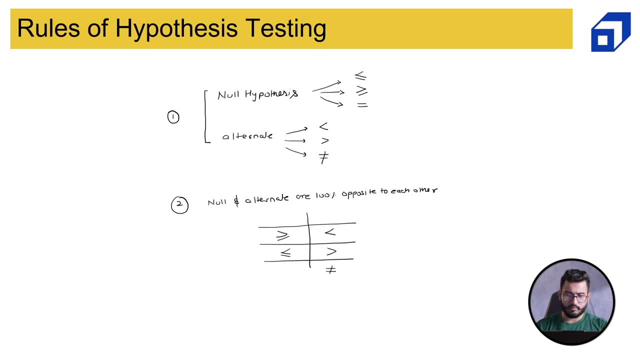 less than or equal to. if this is not equal to, this will be equal to. this is my alternate, this is my null. the third rule is: always start by formulating alternate. always start by formulating alternate. now, these are the three rules which. so, if you remember, 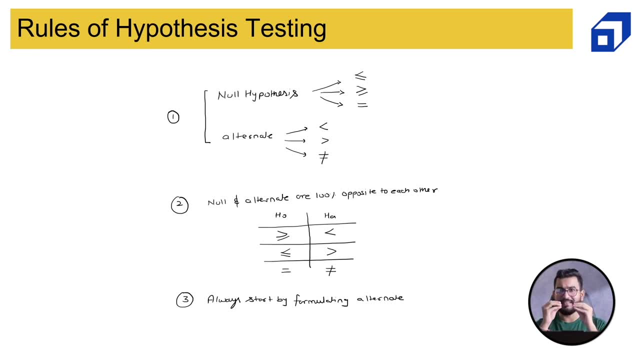 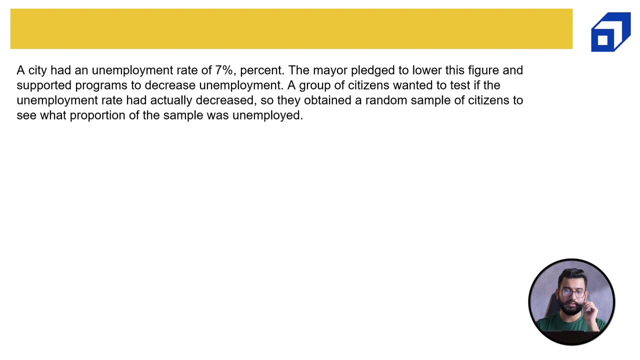 them you can formulate the hypothesis for any given problem. let's try to look into second problem. a city had an unemployment rate of 7%. now, this is my initial state. this is something which is initially given to us, that we all know in the complete city that unemployment 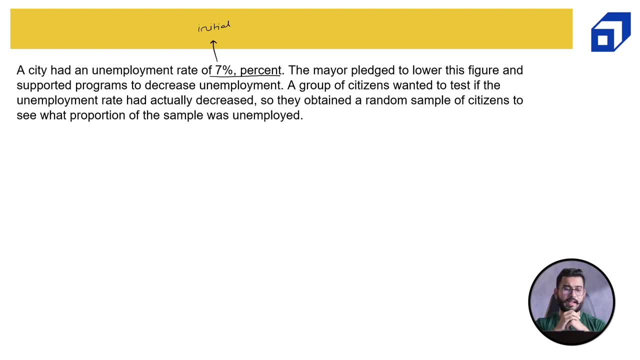 rate is 7%. the mayor pledged to lower this figure and supported program to decrease unemployment. a group of cities and want to test at the unemployment rate has actually decreased. so now what we want to test, or what is my new finding? now, new finding is that the unemployment 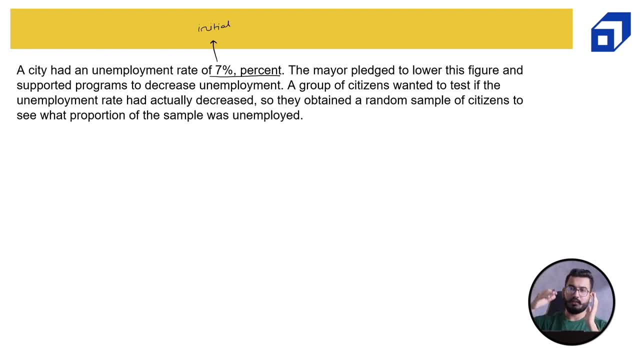 rate has to be decreased, it has to go down, it has to go below 7%. so I will start by writing my alternate hypothesis, which is: average, less than 7%. the opposite of this, average, greater than or equal to to 7%, would be my null hypothesis. Let's take one more example. eHealth insurance claimed that in 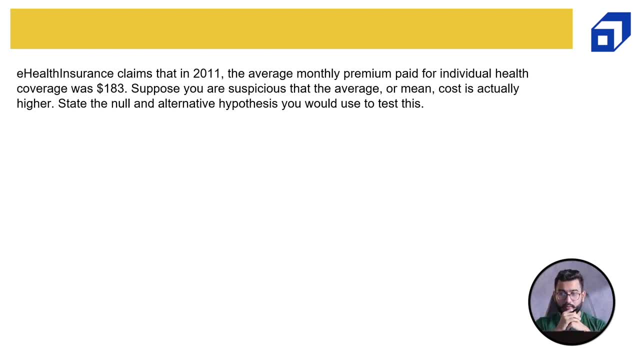 2011, the average monthly premium paid for individual health coverage was $183.. This is the initial statement made by the company. So this is my initial claim, or initial state. initial. Suppose you are suspicious that the average or mean cost is actually higher. Now the new finding. 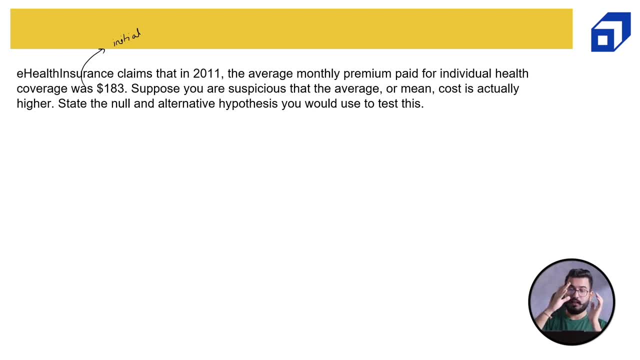 the new thing that you wanted to test is: The average is actually higher than this number. So my alternate: the average is greater than $183. null. The average is less than or equal to $183, simple. Let's take one more example. 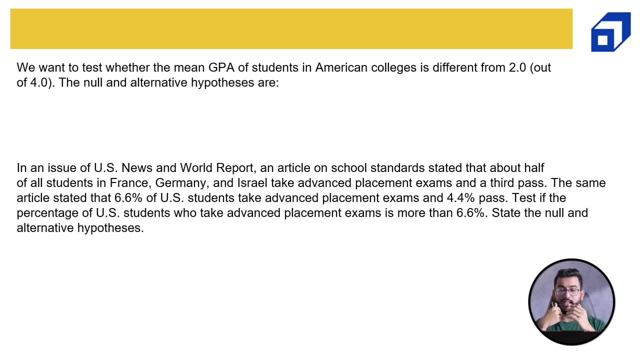 We want to test whether the mean GP of students in American college is different from 2.0. Now this is what we want to test In this question. we are not given with the initial limit. We are going for a minimum old year. We are not going to give to the axes that countries. 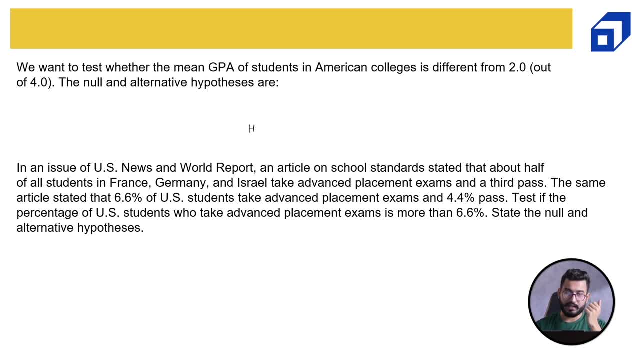 and filho콕 primary предtüz y así como universities y otras zonas de ecxercicio, ECU, alias state. So we know the alternate. that average is not equal to 2.0.. Null will be. the average is equal to 2.0.. In an issue of US News and World Report, an article on school standard. 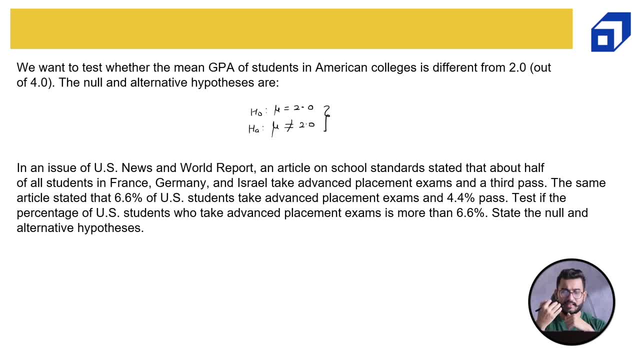 stated that about half of the students in France, Germany and Israel take advanced placement exam and third pass. The same article states that 6.6% of US students take advanced placement exam and 4.4% pass Test. if the percentage of US students who take advanced placement 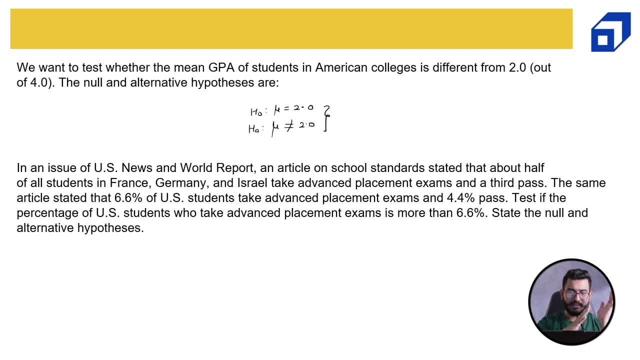 exam is more than 6.6%. So there is a magazine or there is some report which already stated that 6.6% of US students take advanced placement exam. You want to test that if this number is more than 6.6%. 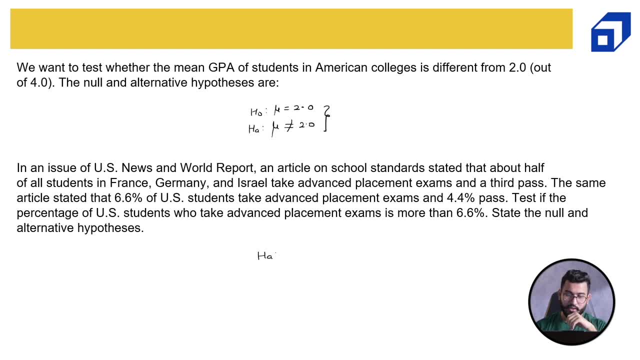 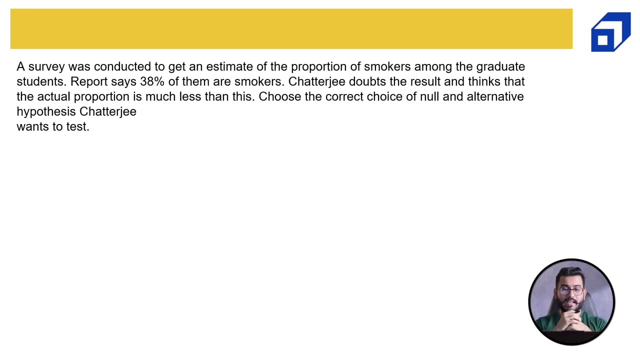 So what you are interested in testing, the alternate will be average is greater than 6.6%, while null is average is less than or equal to 6.6%. Okay, last question: a survey was conducted to get an estimate of proportion of smokers. 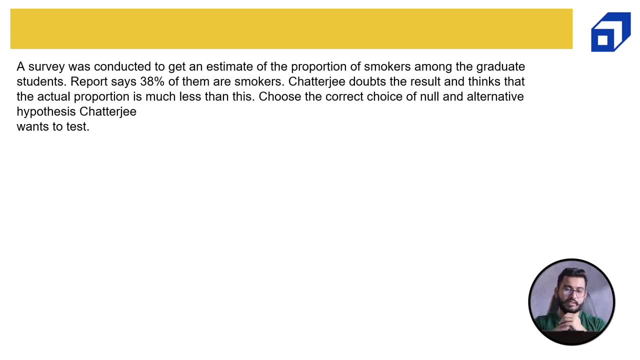 among the graduate student report says 38% of them are smokers. So there is a report which says 38% of the graduate students are smokers. Now, this is the initial state. This is already given in the. in some report this is already proven. 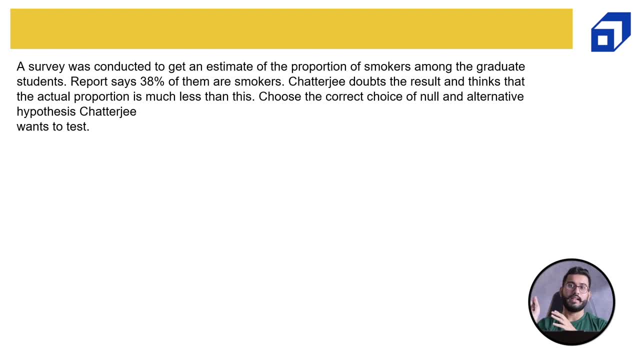 But now Chatterjee doubts the result. Now we have a new finding. this person is suspicious. The person says Chatterjee doubts the result, think that the actual proportion is less than this. So there is a benchmark: 38%. there is a new finding in the Chatterjee. Chatterjee is thinking: 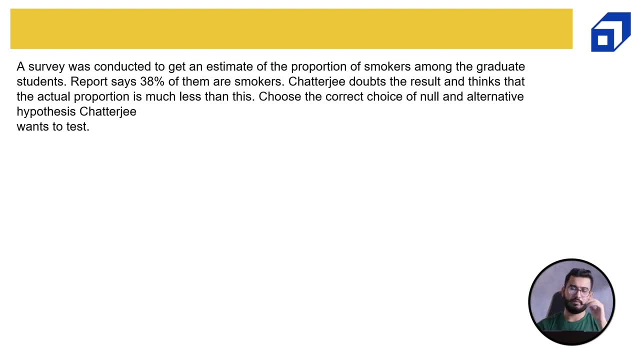 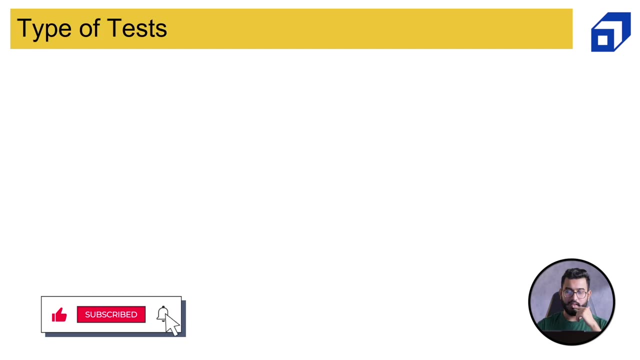 that the actual proportion is less than 38%. So what is alternate? That the average is less than 38%, which is what Chatterjee thinks, while the report says it is greater than or equal to 38%. This is my null and alternate hypothesis. 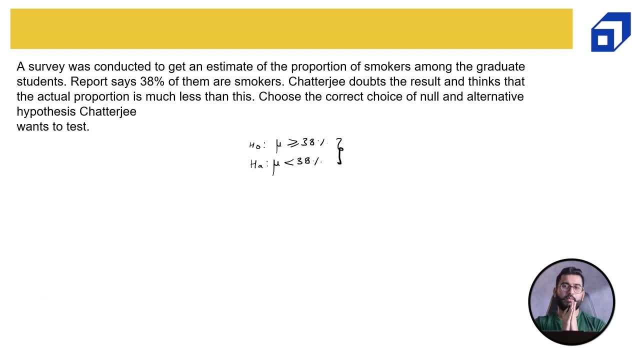 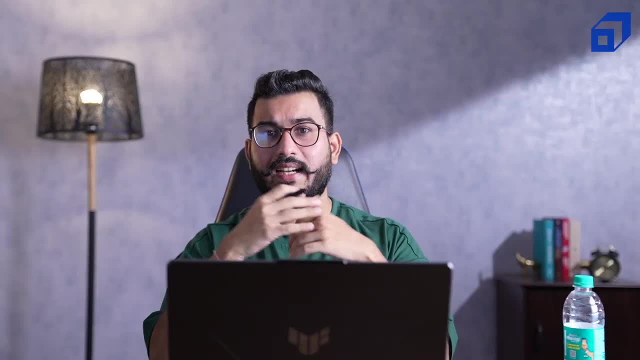 So I hope now you guys are clear with the first stage of hypothesis testing, which is how to formulate the null and alternate hypothesis given a particular business statement. Now let's try to understand what are the various types of tests we have in the hypothesis testing. 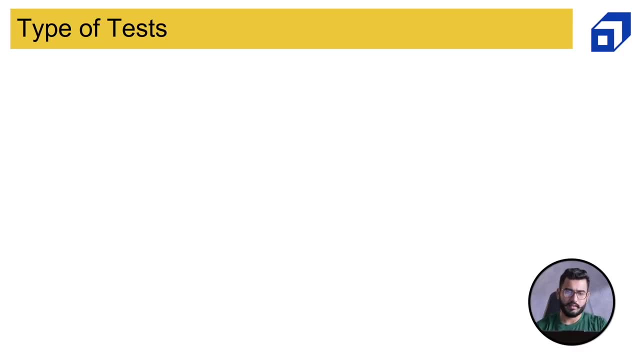 topic. Okay, So there are two kinds of tests. Number one is known as the Z test. The second one is known as the T test. Now, within Z test, we have two methods. One is known as the confidence interval, confidence interval estimation or confidence interval. 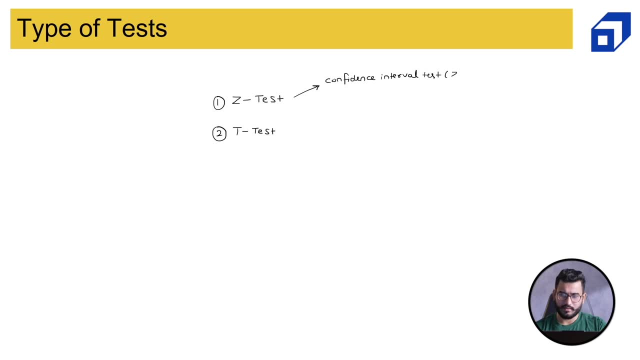 test, also known as the Z test Or the Z value method. Then we have significance test, also known as the P value method. So within Z test we have Z value method and the P value method. Within T test, we have three or three types of tests. 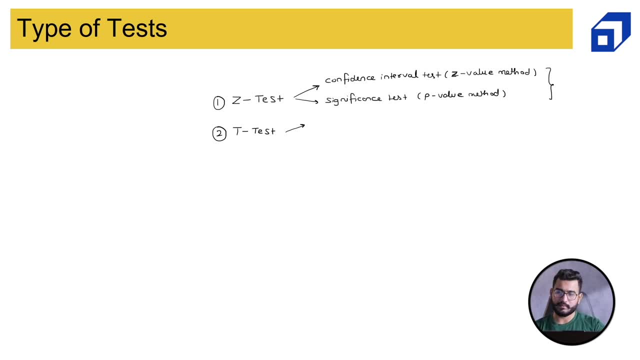 So these are the two methods to perform Z test. But within T test we have three types of tests based on the problem statement. Number one is one sample T test. Second, one is paired sample T test And the third one is independent sample T test. 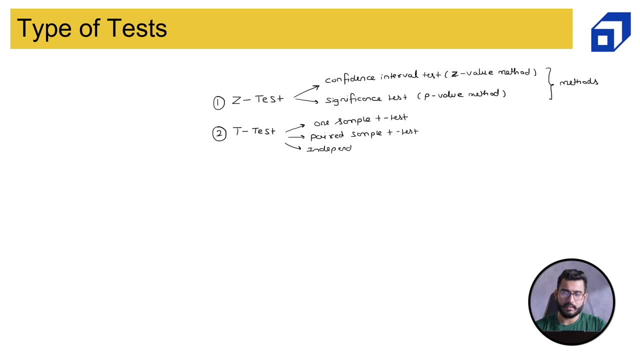 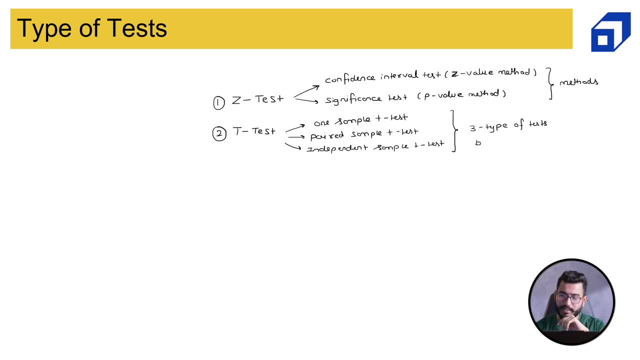 statement. So three types of tests based on the problem statement. Okay Now, when to use Z test. When to use Z test. Okay Now, when to use Z test. When to use T test. So I will first talk about when to use Z test. 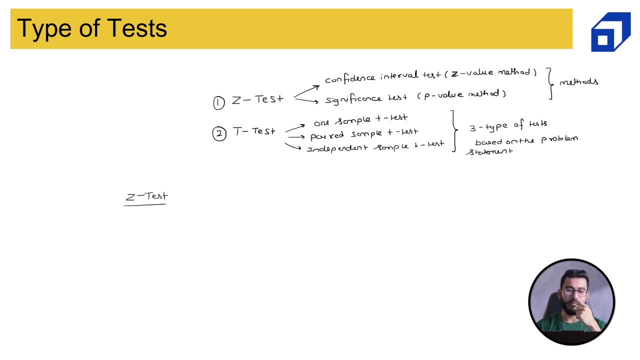 And when we will be starting the T test. I will talk more about when to use T test. So when to use Z test, You have to check for two things. Number one: the number of observations in your sample in the sample should be equal. 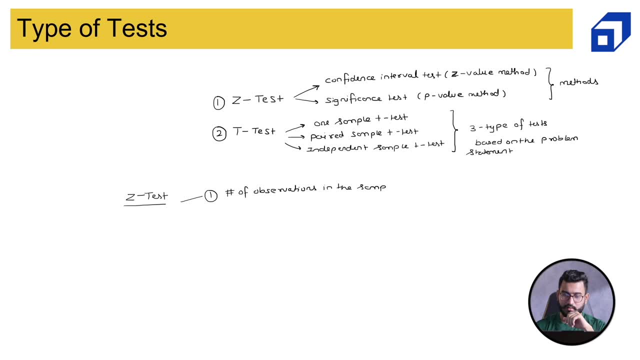 to the number of observations in the sample. Okay, Okay, Okay, Okay, Okay. So if we take the number of observations in the sample, it should be more than 30.. And the second condition is the population. standard deviation is known. 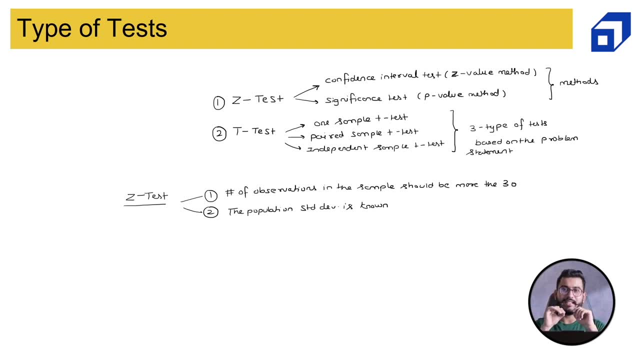 Now, please remember, this is a very important interview question, a very common interview question about what is the difference between Z test and T test. Okay, Z test and T test. I'm just talking about Z test as of now, When we start the T test. 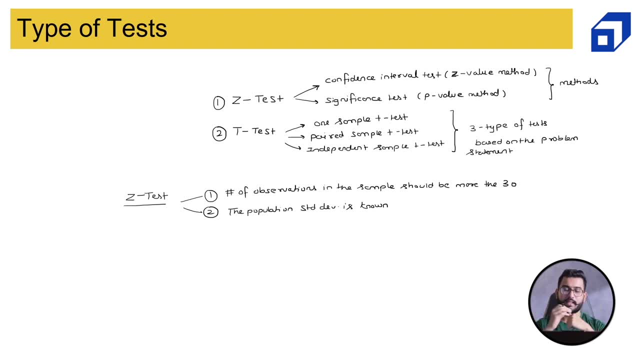 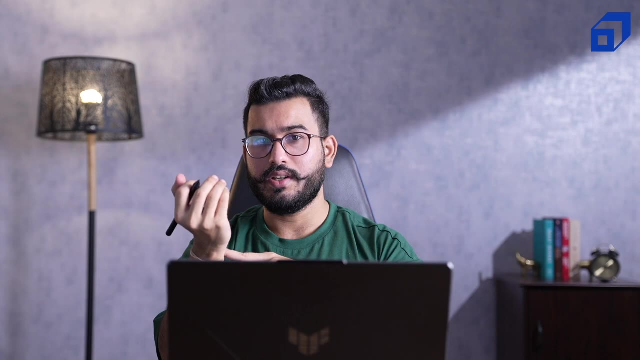 I will show you the rules of when to use a T test, But please remember this is a very important topic. This is a very common interview question: the difference between Z test and T test. So if I do not know the population standard deviation and I know the sample standard deviation, but my 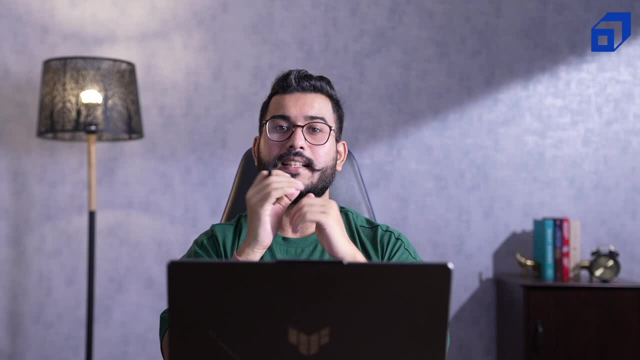 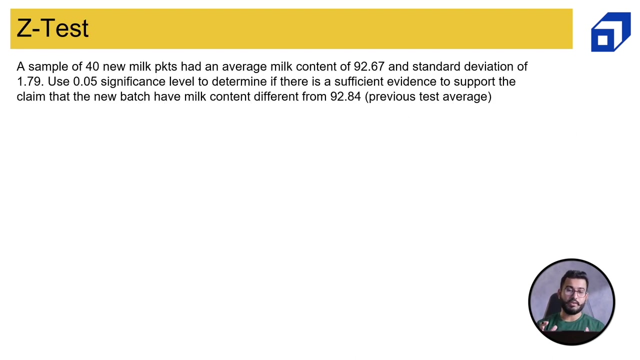 sample size is more than 30, then still Z test is applicable. Now directly jump to a problem statement. Let's formulate the hypothesis, apply the Z test and let's try to conclude In this question. we are given with a sample of 40 new milk packet had an average milk content of 92.67. So 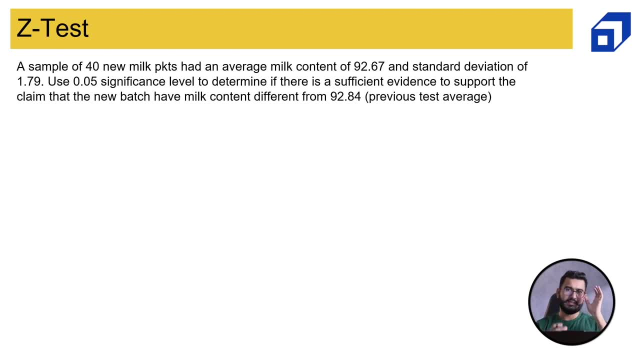 within a milk packet you will find out some quantity of milk and some quantity of water. So it has been given that a sample of 40 new milk packet had an average milk content of 92.67 with a standard deviation of 1.79.. So this standard deviation is the sample standard deviation. Now, 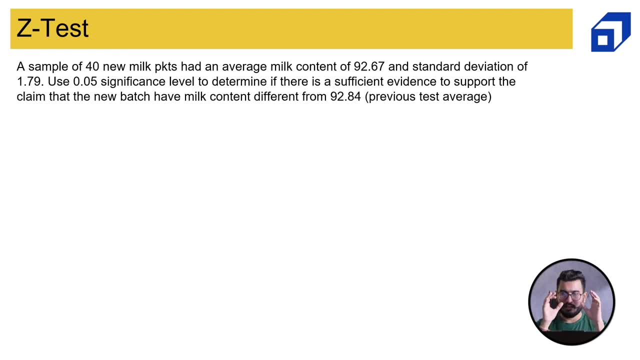 since my sample size is more than 40, Z test is applicable over here. Use 0.05 significance level to determine if there is sufficient evidence to support the claim that the new batch has milk content different from 92.84.. Now, as of now, the complete question may be sounding really. 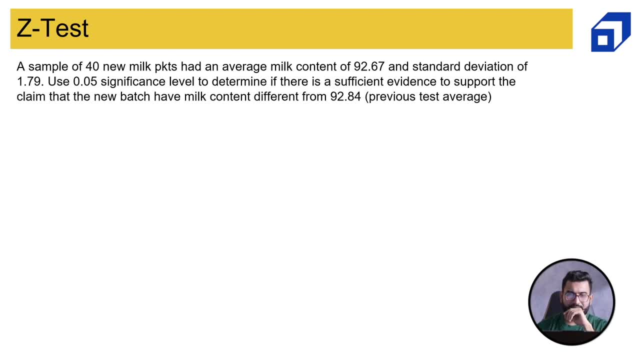 German to you. Don't worry about it. Let's try to decode this particular problem. So assume that you work as a quality test. You work as a, let's say, as a scientist in the quality test department of this milk producing factory or milk packet factory. So you work as a scientist. 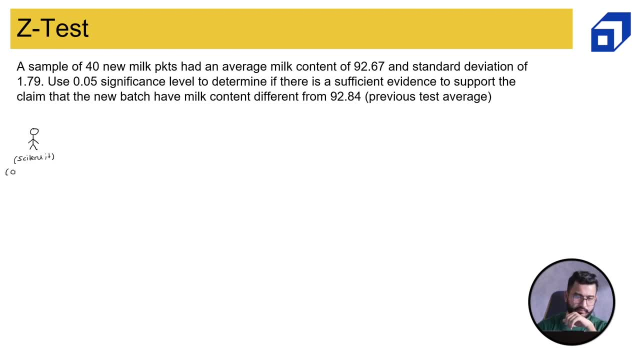 in the quality test department. quality test department and on the daily basis. let's say, this factory, on the daily basis, is producing 1 lakh milk packet, 1 lakh milk packets. so on the daily basis, this factory is producing 1 lakh daily packet. now, as a scientist, it is completely impossible for you to test all the milk packet. 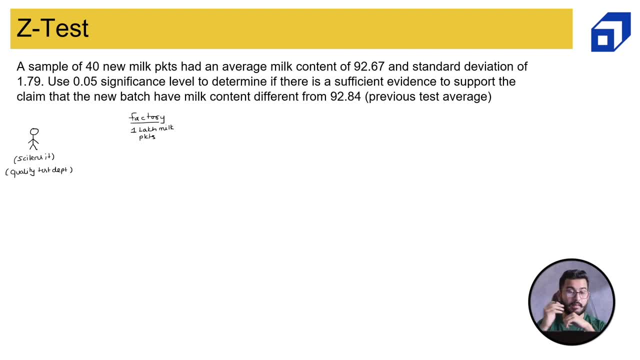 right. so what is the correct procedure? we have already learned about it. we will take a sample out of it. so let's say, on the daily basis you are taking a sample of 40 milk packet. so let's say I have just drawn a table on my screen. let's say: this represent the day in the month, so day of. 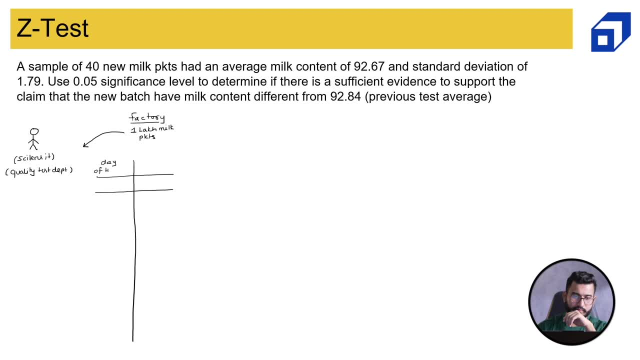 the month on. this represents the average milk quantity. so let's say, on day one, the average milk quantity. so on day one you sampled out 40 milk packets out of the population of 1 lakh milk packet that was produced. on that particular day you sampled out 40 random milk packets. after performing the test on all those 40 packets. 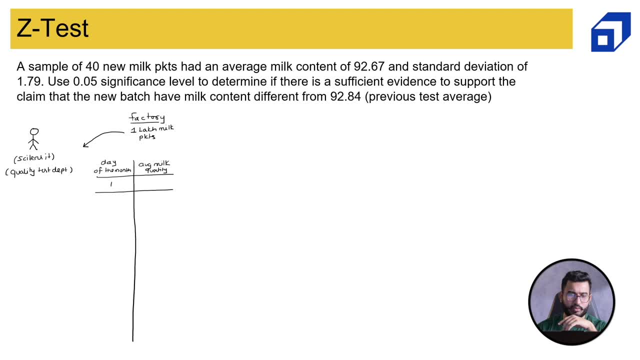 the average milk content came out to be, let's say, 92.5. then on another day, the average came out to be 92.7. on another day, the average came out to be, let's say, 92.8. on another day, the average came out to be, let's say, 92.27. and you have been doing this. 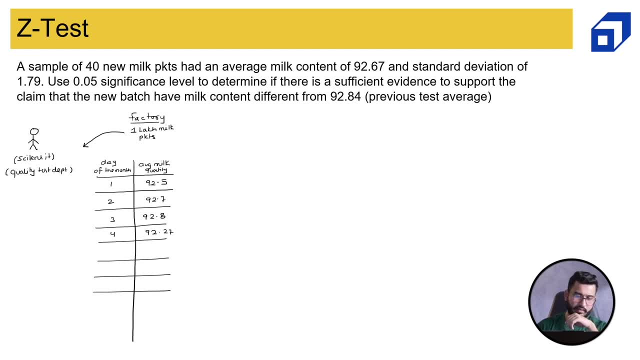 thing, let's say for last one month, so let's say on day 30. so I'll just put dot dot dot in this, in this table. on day 30 the average came out to be ninety two point six six. now, when you looked at the month, 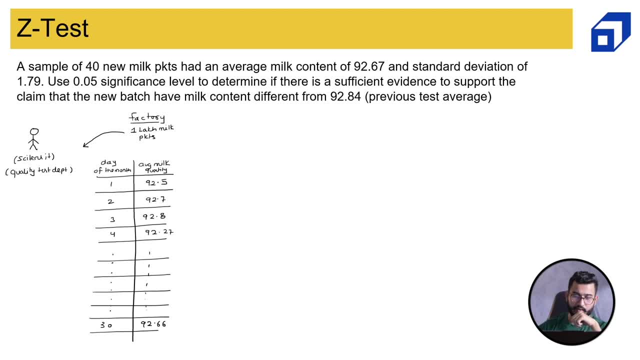 average, the complete month average. the monthly average was ninety two point eight four. now this is what has been given to us. so another day, let's say another month, another day when you were testing 40 new milk packet, 14 you milk packets, your average came out to be ninety. 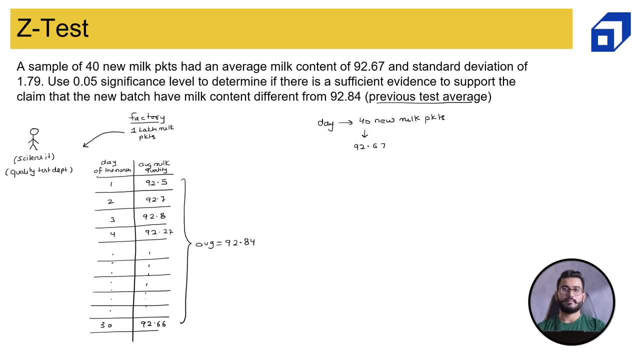 two point six seven. so I hope this, this complete picture, is making sense. you have been doing the test for all the days, from day one to day thirty, from last one month, and the average was ninety two point eight four, and this is, let's say you can say that this is above Ikran. 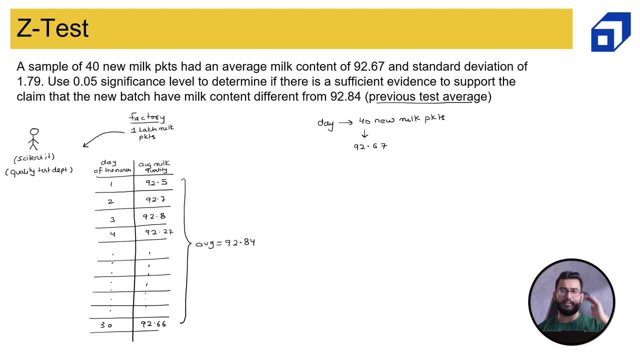 the quality above the quality cutoff. but on one particular day, after testing this 40 new milk packets, the average came out to be 92.67. now you want to perform the test to check if this number, the new mean, the new sample mean, is in the significance range, or is this? 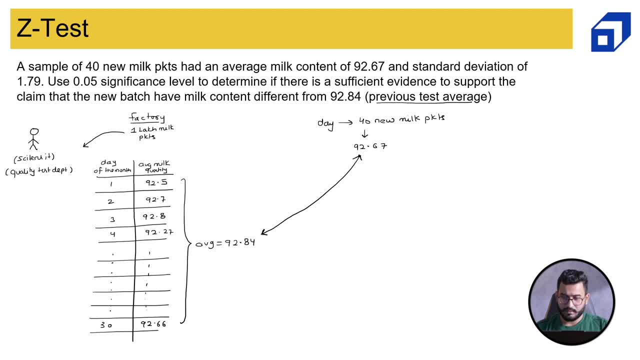 number is ninety two point six, seven, is statistically significant or statistically same as ninety two point eight, four or not? so what we want to test is ninety two point six, seven statistically same as ninety two point eight, four, four or not. This is what we want to test. So if these two numbers are statistically 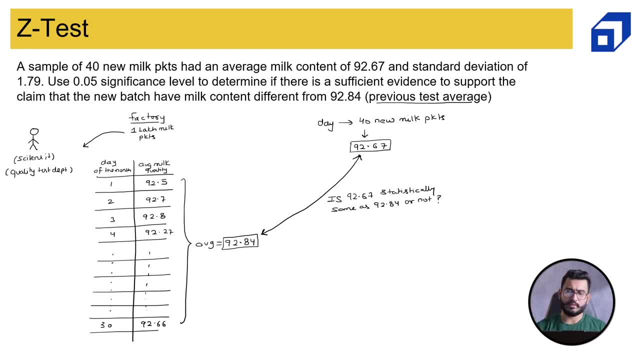 same, then we will approve this, this, this batch, this batch of new 40 milk packets. If they are different, if they are statistically different, we will reject the complete lot because the milk content is less than the acceptance. This is what the complete scenario. 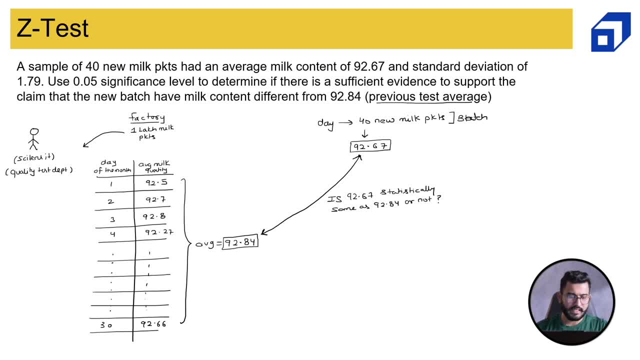 is Now the number one thing that we will do is to formulate the null and alternate hypothesis. So my alternate hypothesis will be that the average is not equal to 92.84.. Why I'm using 92.84 over here? Because that is my previous or previous proven value. This 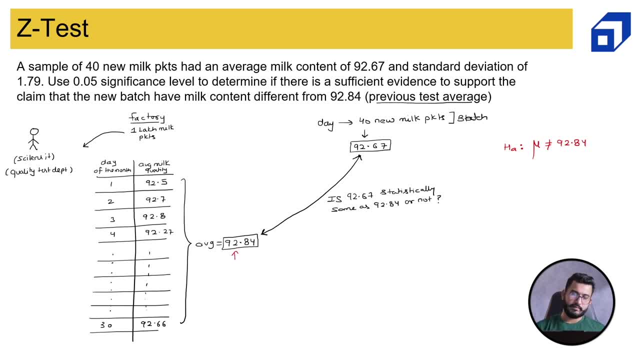 is my initial value, right, Initial. Now alternate, or sorry, null will be. the average is equal to 92.84.. Okay, Now please remember one thing: Whenever we have a not equal to sign, this basically mean I have to perform the test, uh, which will be a two tail test. So let's quickly understand this. 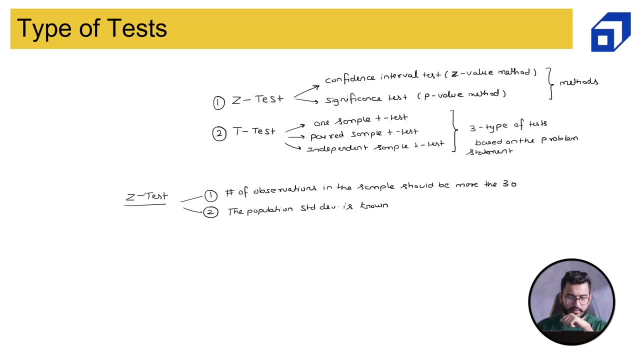 part. If I'm having not equal to sign in my alternate hypothesis, then my rejection region. So what is rejection? What is acceptance? We will talk about it, Don't worry, But my rejection region will be on both the side. So this is my rejection region. This is my rejection region If I'm 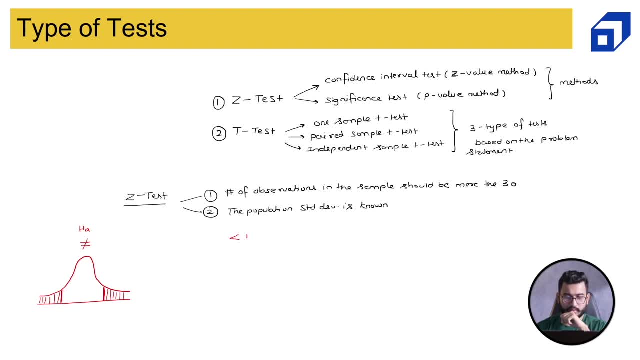 having less than sign in my alternate hypothesis, then my rejection region will be on left side- This side, So just see the arrows. So the arrow is pointing on the left, So my rejection region is on the left. If I'm having greater than sign in my alternate hypothesis, then 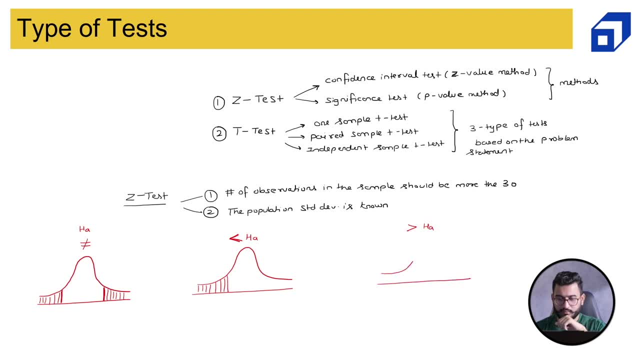 my rejection region will be on the right, which is on the this side. So just see the arrow. arrow is pointing towards the right. So my rejection region region is on the right Now, since I'm having not equal to sign in my alternate my that this particular test. 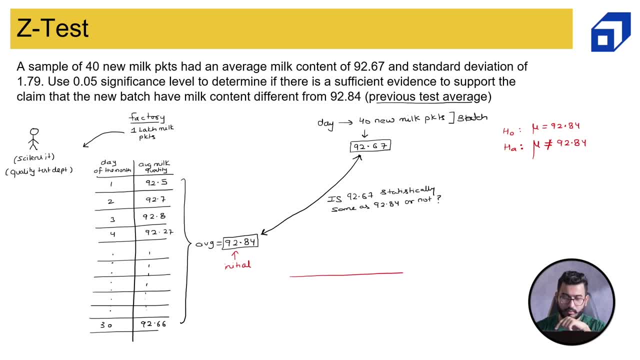 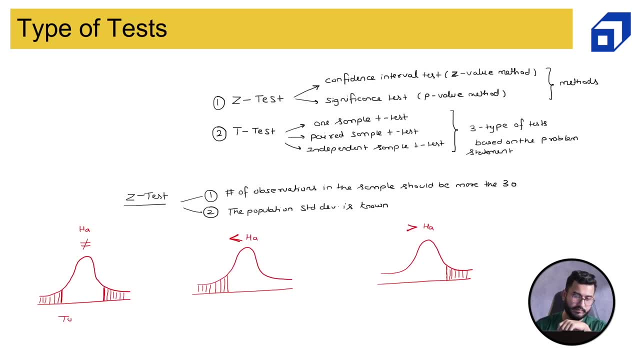 I'm having not equal to sign in my alternate. Now, since I'm having not equal to sign in my alternate, my that this particular test- I'm having not equal to sign in my alternate- this particular test- would be a two tail test, So this is known as a two tail test. 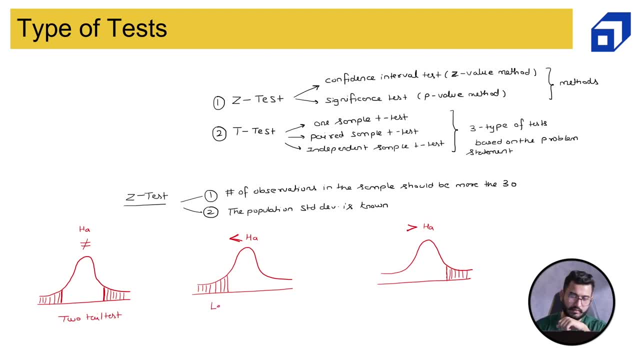 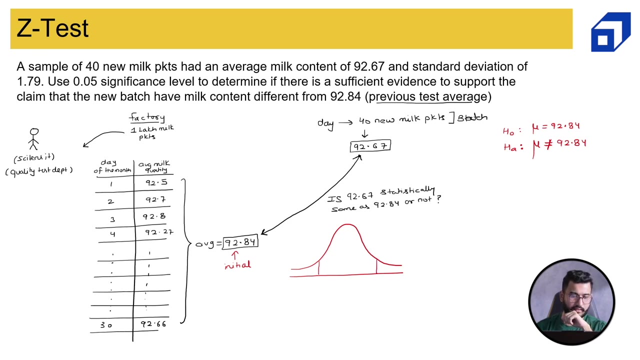 This is known as a left tail. This is known as a right tail test. So this is my two tail test. So my rejection region is on the both end. I'll just highlight it. This is my two tail test. So this is my two tail test. So this is my two tail test. So this is my two. 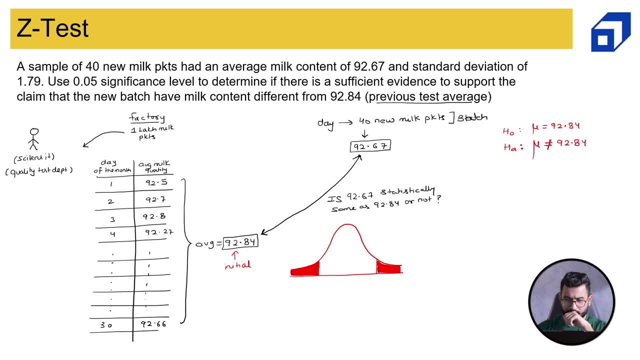 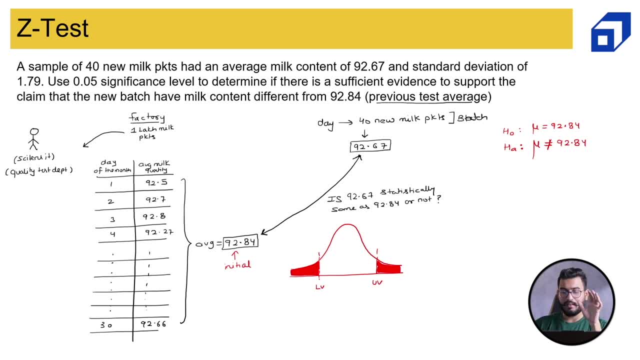 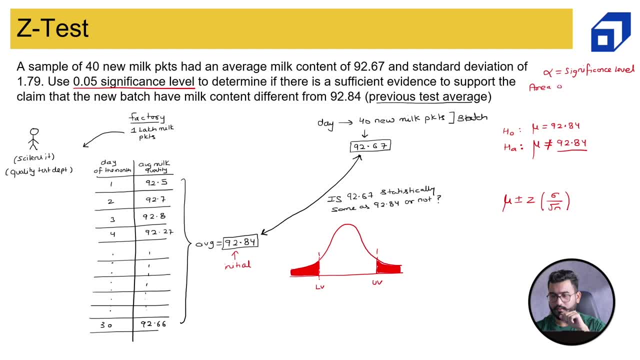 area of rejection, which is 0.05.. So, out of the complete area which is 1, 0.05 is the area of rejection. Now, since I am having area of rejection or rejection region, these are my rejection regions. Rejection region: This is also my rejection region Since my rejection. 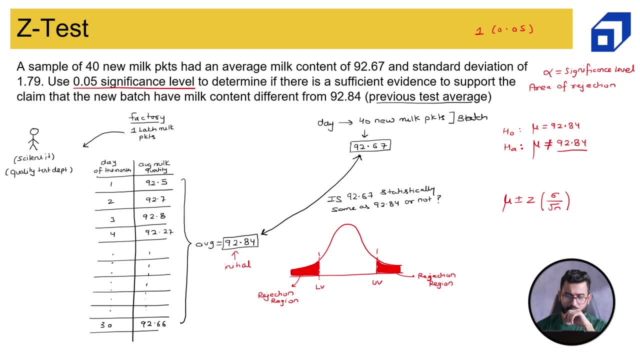 region is on both the end. I have to divide this significance or area of rejection by 2.. So 0.05 divided by 2 will be 0.025.. So from here to here, the area is 0.025.. So I. 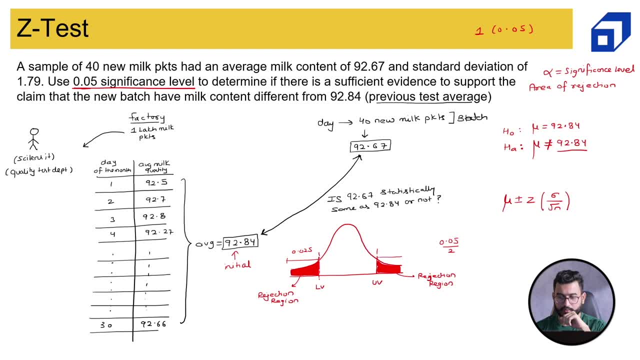 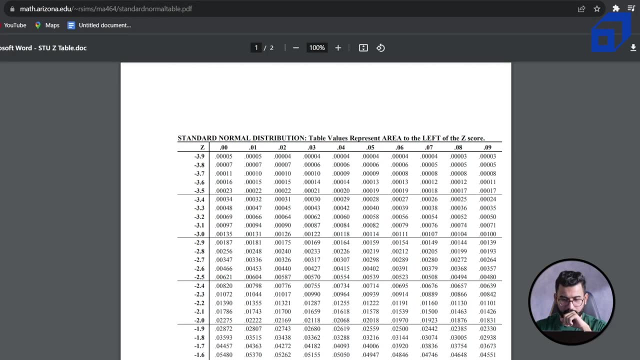 have to divide. from here to here, the area is 0.025.. Now, what is the Z value over here? What is the Z value over here? We already know this, but let's quickly find out the Z value at 0.025.. So 0.025 over here and the value is minus 1.9 and 6.. Similarly, for the 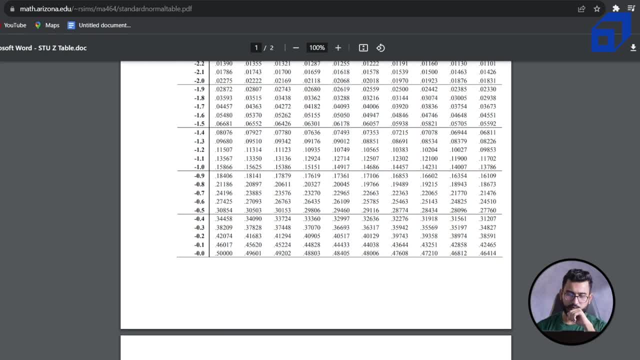 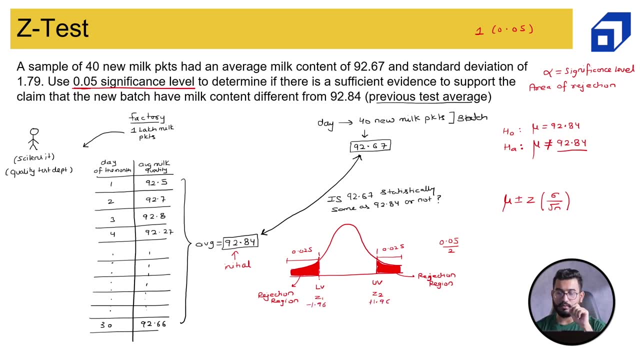 positive side, it will be plus 1.96.. Okay, So this is minus 1.96 plus 1.96.. Now, using this, we will find out the lower value and upper value. So 92.84 plus minus 1.96. sigma, which is standard deviation, is 1.79 divided. 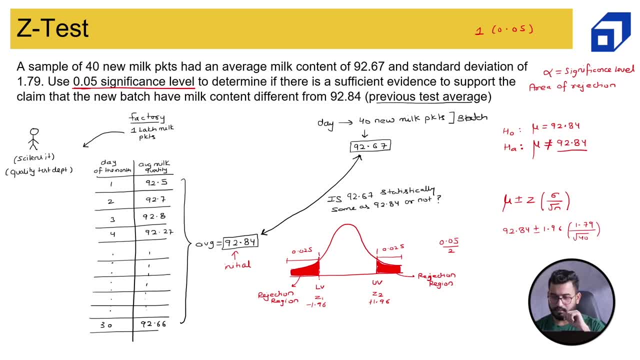 by root of 40. So we will get 92.286, 93.96.. So here we will have 92.286.. Here we will have 93.394.. Now this is the range which has been given to us or which we have derived using the population mean. So now, if my sample 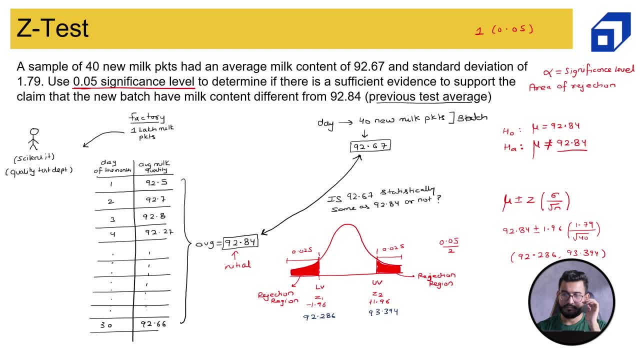 mean: this is my sample mean. Okay, So this is my sample mean. Okay, Okay, So this is my sample mean. If my sample mean lies between, or maybe in, the acceptance range, this is my acceptance range, Acceptance range. So if my sample mean lies in the acceptance range, we say that. 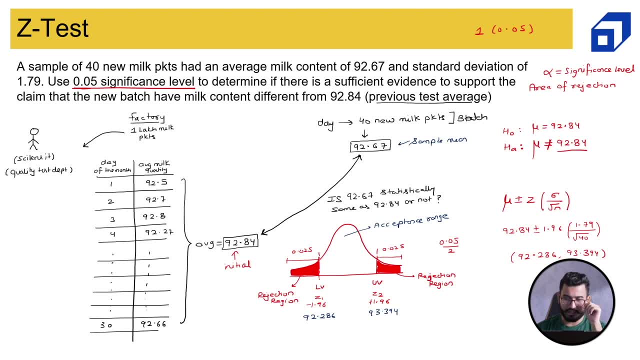 we fail to reject null, So 92.67 will lie somewhere between this over here, since it is lying in the acceptance range. Okay, if sample mean lies in acceptance range, we conclude that we fail to reject null. Otherwise, if it is in the rejection region, if sample mean- so I forgot to write mean falls or? 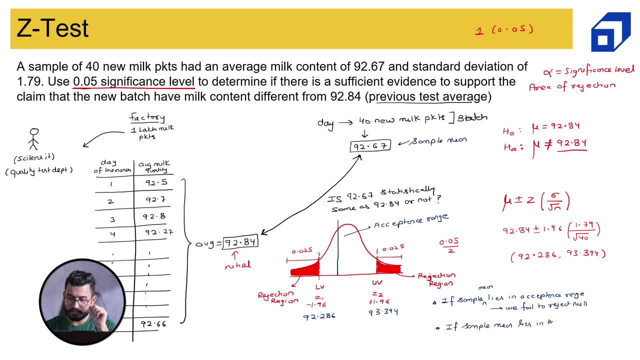 lies in the rejection region. we reject null. We reject null. So, as of now, what conclusion we will derive? The conclusion will be: we fail to reject null. Why? Because the sample mean is within the acceptance region or within the boundary which we have derived from the 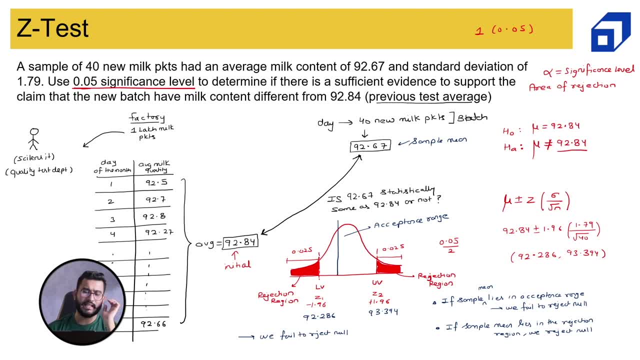 method using the population mean. This is also known as the hypothesized mean. The reason hypothesized mean is because we hypothetically call it as a population mean, but it is not the true population mean. So if you are getting confused, just be very clear. This is a sample. 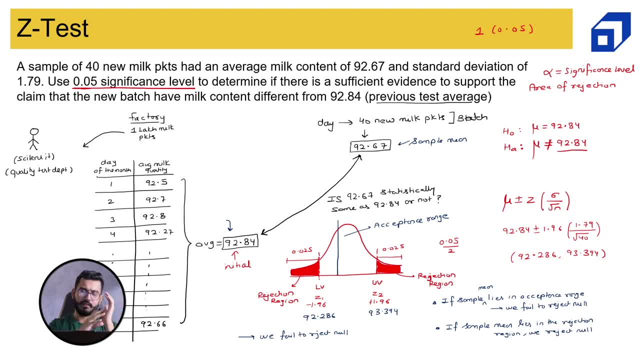 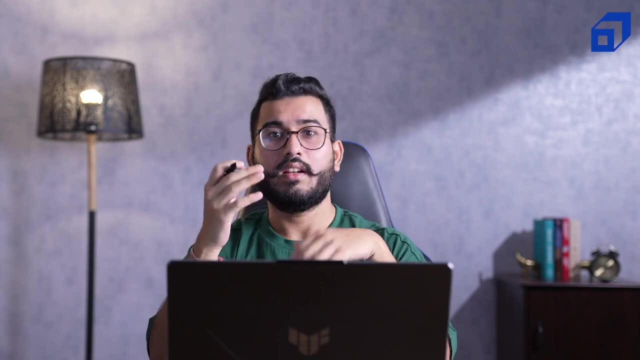 mean 92.67,. 92.84 is my population mean And using the population mean we have derived a range. If my sample mean falls within this range, we fail to reject null. If it is outside the range, we reject null. I hope this question makes sense. If it is not, let's take one more. 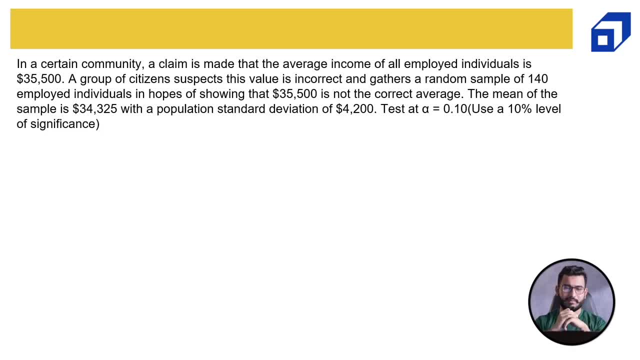 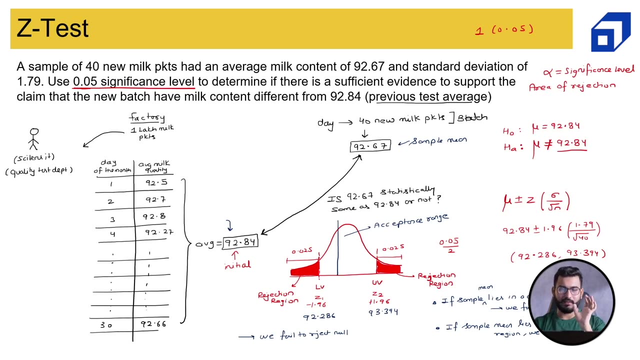 example. Now let's try to solve this particular problem, And I would advise all of you to pause this video and try to solve this problem by yourself, because we have already seen one example. You have to just follow the steps and try to solve this problem and try to pause. 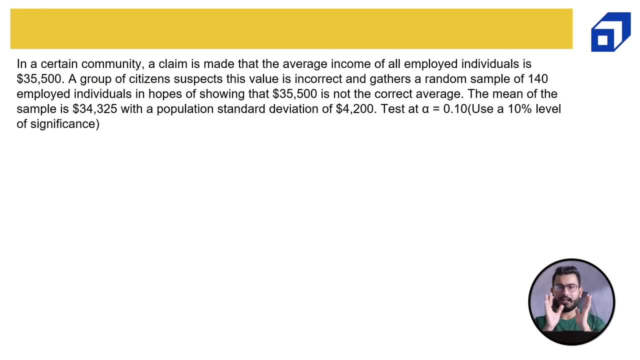 the video and just try to solve it by yourself. I hope you guys would have solved it by yourself. If not, let's try to solve it. The question says: in a certain community a claim is made that the average income of an employed individual 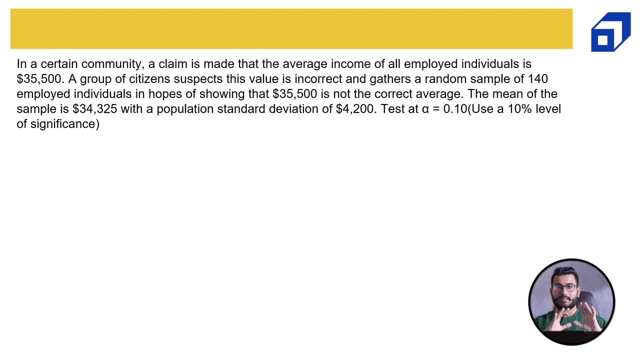 is $3,500.. Now, again, there is some initial statement which has already been proven, that the average income is $3,500.. So this is my initial statement, Initial statement. So I am going to say that the average income of an employed individual is $3,500.. Now let's. 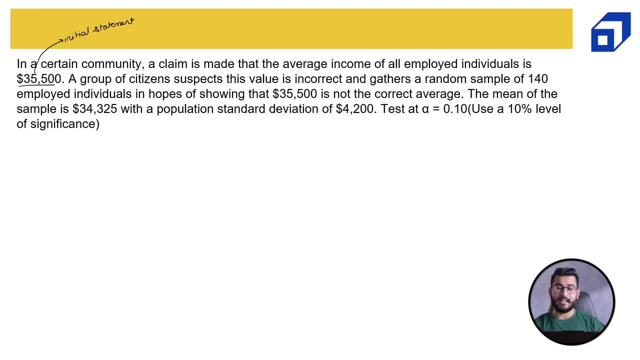 try to solve this problem. A group of citizens suspect that a value is incorrect and gather a random sample of 140 employed individual in a hope of showing $3,500 is not the correct average. The mean came out to be $34,325.. So what the group of citizens did? they collected. 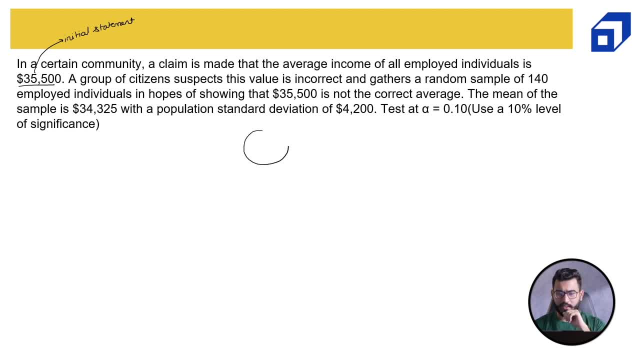 a sample of 140 people and they obtained the sample mean to be $34,325.. Now let's try to solve this problem With the population standard deviation, the population standard deviation, So this is not sample standard deviation. So here we have been given with the population standard. 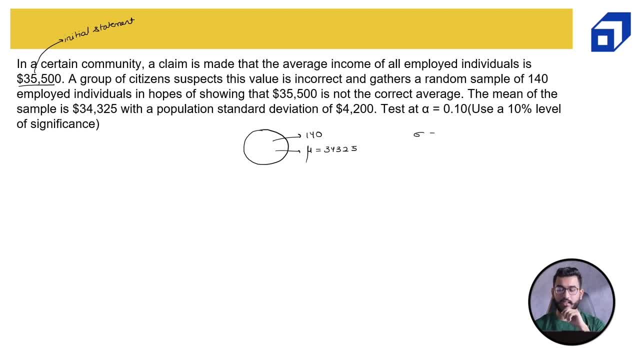 deviation of $4,200.. The alpha, alpha. what is alpha? The area of rejection, area of rejection is given as 0.10, which is 10%. Now let's start with the formulation of the hypothesis. My alternate hypothesis is that the average 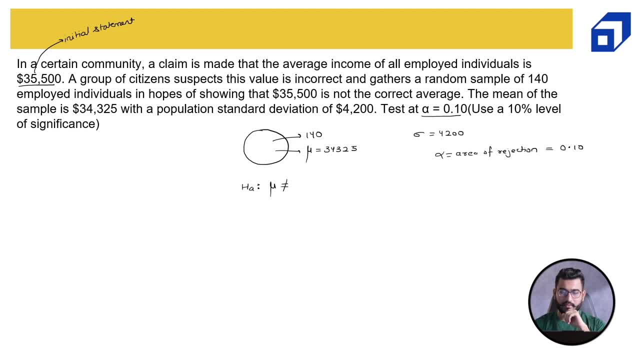 is not equal to $3,500. Because $3,500 is the initial value or initial state. So group of citizens wants to prove that $3,500 is not the correct average. So that's my alternate. Null will be opposite of this. Mean is equal to $3,500. 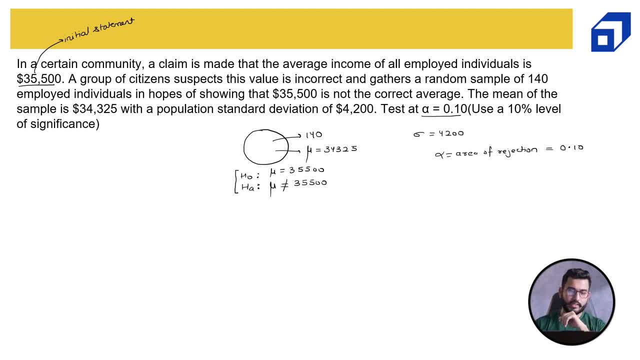 Now what is my second stage? I will find out the lower critical value and the upper critical value. So here is my normal distribution. Since I'm having not equal to sign in my alternate hypothesis it is the two tailed test. My area of rejection is on both the end, So this is also area of 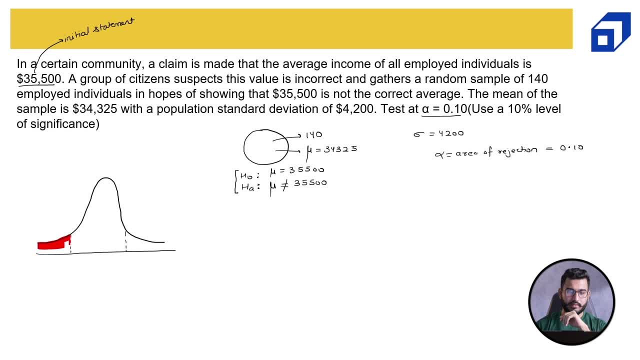 rejection, and this is also my area of rejection. Now let me calculate the third increase in the total 채 auf YouTube data. So we're doing less than 1%. your value now. Now we have to find out the lower critical value and the upper critical value. 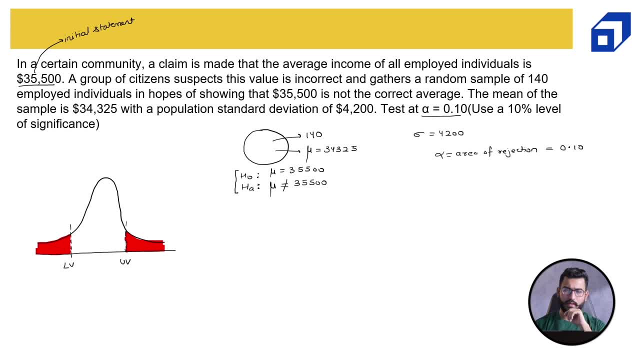 Before that, we are given with the alpha of 0.10.. Since I'm having rejection region on both the ends, my alpha will be divided by 2.. So 0.1 divided by 2, so this will be 0.05. from here all the way up to here. 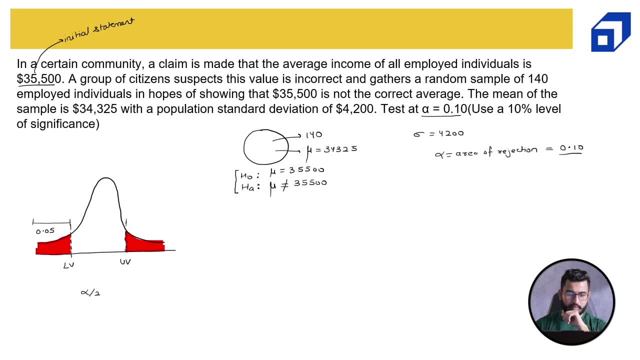 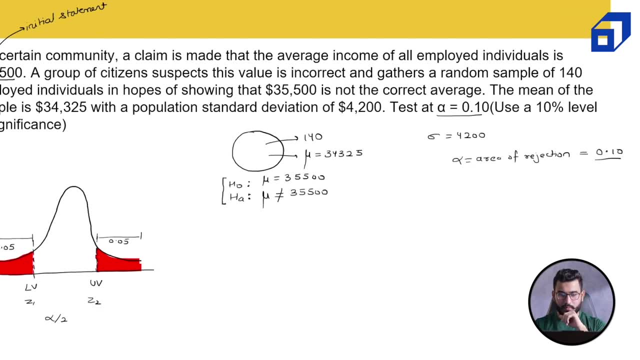 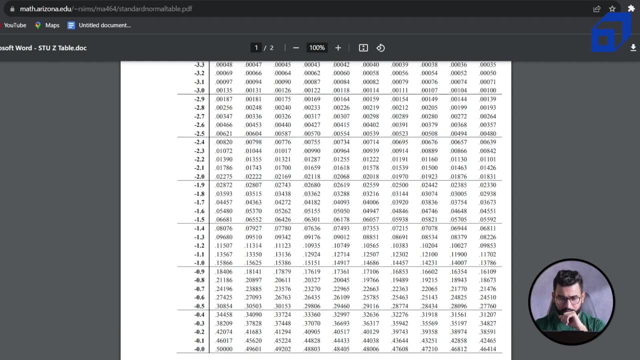 And this will also be 0.05.. So what is the Z value over here? Again, we will use the Z table, So we have to look at 0.05.. So 0.055 over here. Maybe we can take this one, or maybe this one. 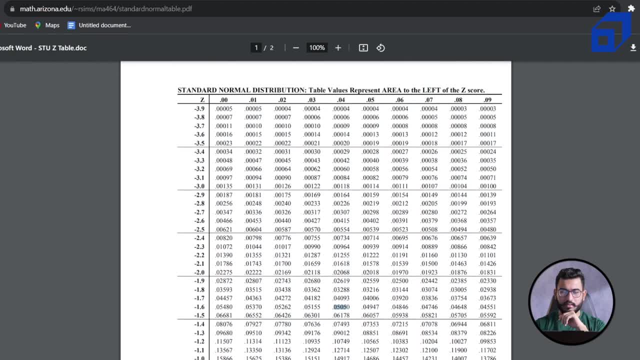 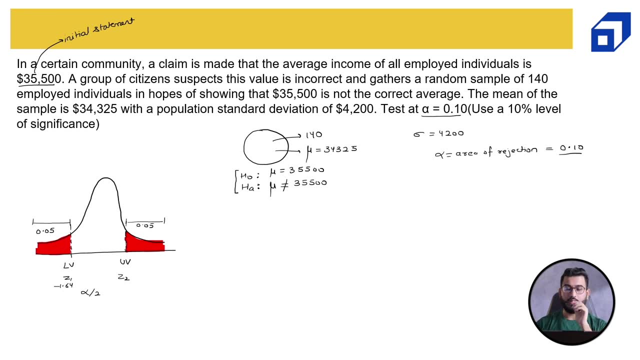 So minus 1.64 or 6.5, you can take any one, So I'll go with minus 1.64.. So this is minus 1.64.. This is minus 1.64.. This is plus 1.64.. 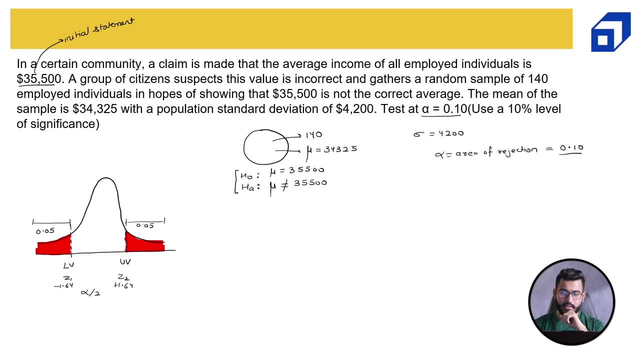 Now I have the Z value. I have all the values. Let's calculate the range Mean plus minus Z times of sigma divided by root of n. My mean is 35,500 plus minus 1.64.. Standard deviation is 4,200 divided by root of 140. 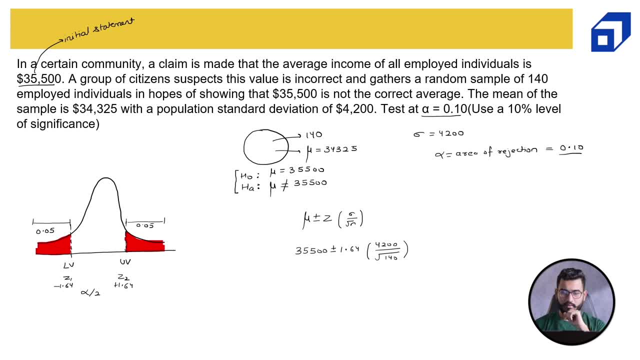 So the range would be 34917.76,36082.24.. So this value- lower value is 34917 and the upper value is 36082.. Now, where my sample mean is lying at 34325.. So my 34325 will lie at 34325.. 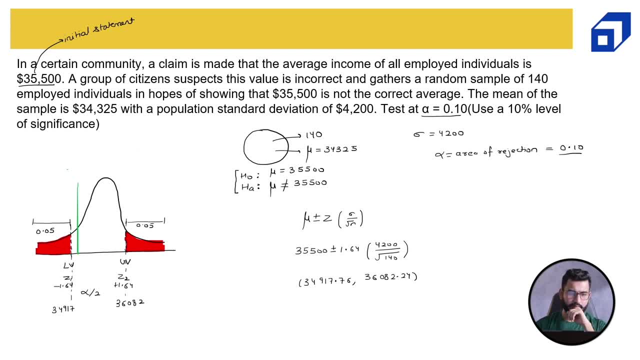 So my 34325 will lie somewhere over here, right, 34325 in the acceptance region. Since it is falling in the acceptance region, we conclude that we fail to reject null And that basically means the claim that was made was correct, which basically means this: 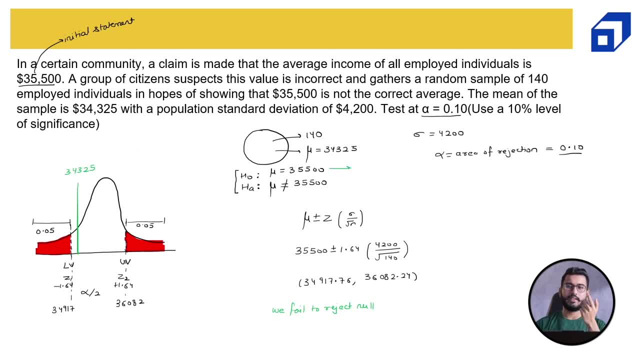 alternate. Oh sorry, Null is actually true. Now I'm just saying we fail to reject null, But. But maybe because the sample size was less or because the sample collection process was biased, due to which the citizens were not able to prove that 35,500 is a wrong average. 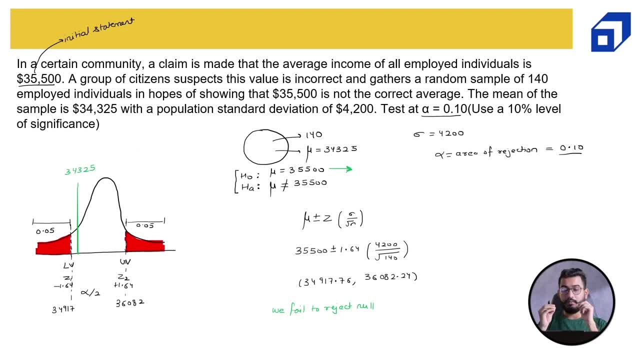 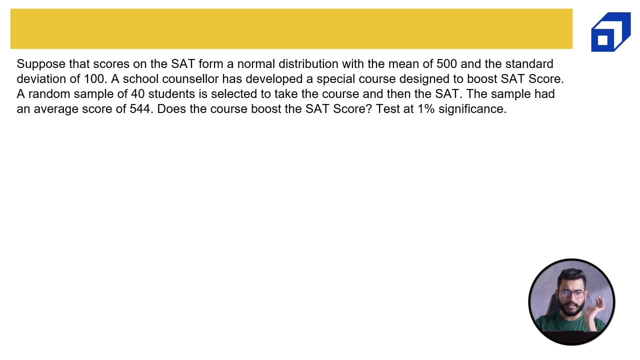 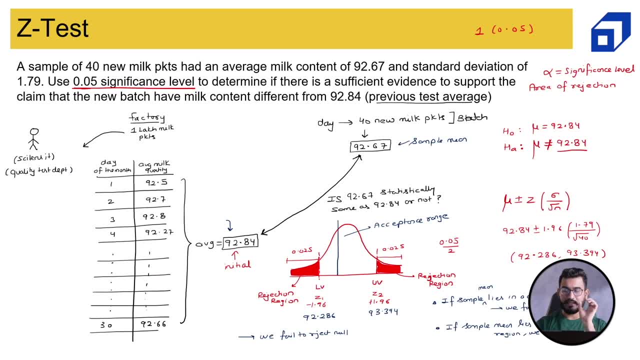 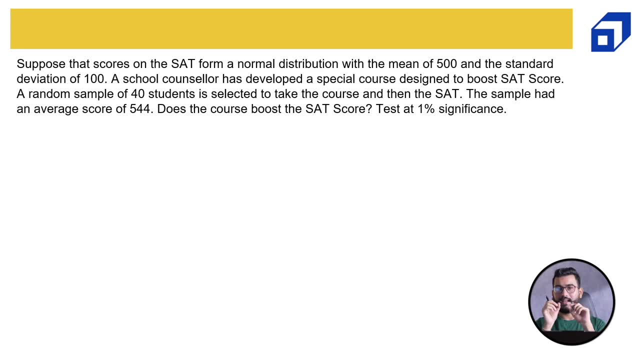 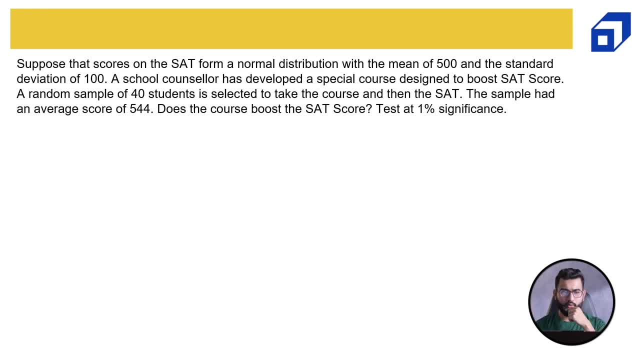 So that question says: suppose the scores on that SAT? So SAT format is one of the examination Formed, a normal distribution with a mean 500 and a standard deviation 100.. The school counselor has developed a spatial course designed to boost SAT score. a random. 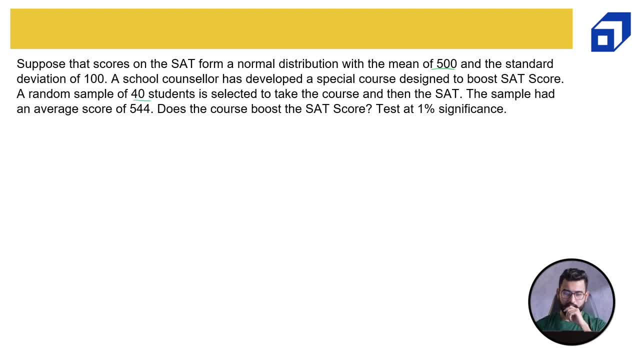 sample students is selected. So we have a sample of 40 students and the sample average came out to be 544 after they have gone through the course and they have attempted the SAT examination. The question already states that the SAT score is having a normal distribution with mean 500 and a standard deviation. 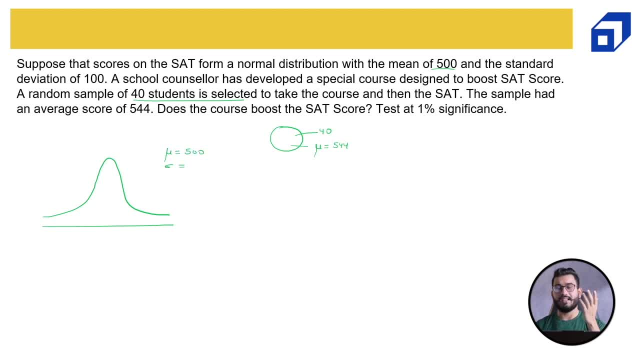 of 100. So this is my population parameter. you may assume this is. these are the population parameters. Now, does the course boost their score? So my alternate hypothesis is: does the average is greater than 500? because if the course boosts the score, it should be greater than the population average, which is 500. 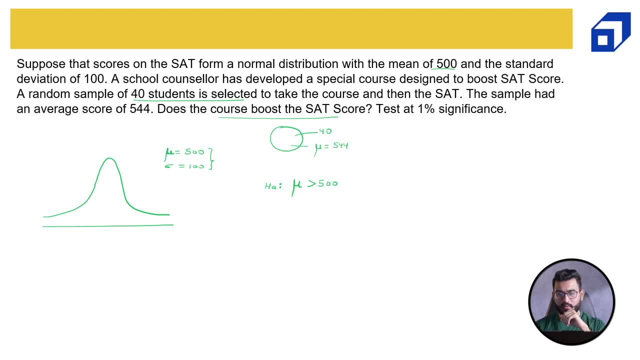 right Null is it is less than or equal to 500. right Now, greater than 500 basically mean it is the arrow is pointing on the right side, so it is a right tail test. so my rejection region will be on the right end. This is my. 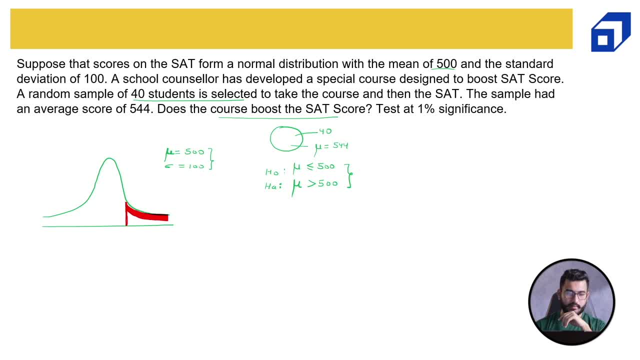 rejection region. Now what we have to do again, we have to find out the Z value over here. so let us find out the Z value over here. Now, to find out the Z value, the area of rejection alpha is given as 1 percent, which is 0.01. so this area from this, 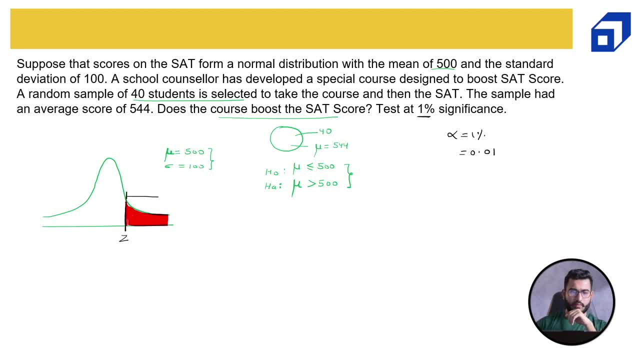 point all the way up to the end is 0.01.. So what is the area from this point all the way up to this point? It will be So. now we will use the Z table to find out the Z value at the AUC of 0.99.. 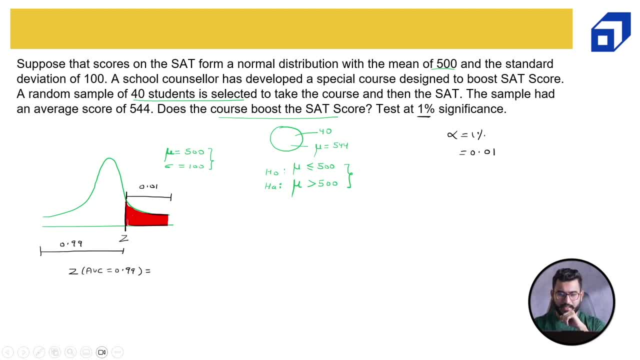 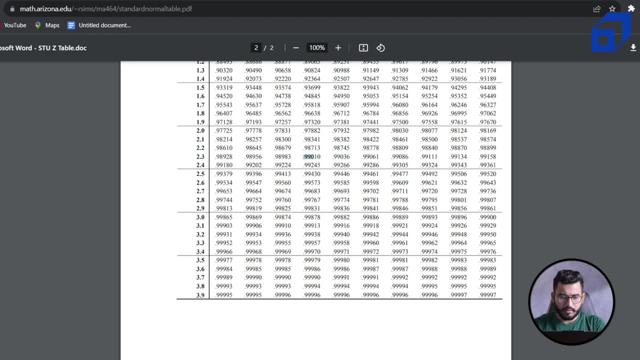 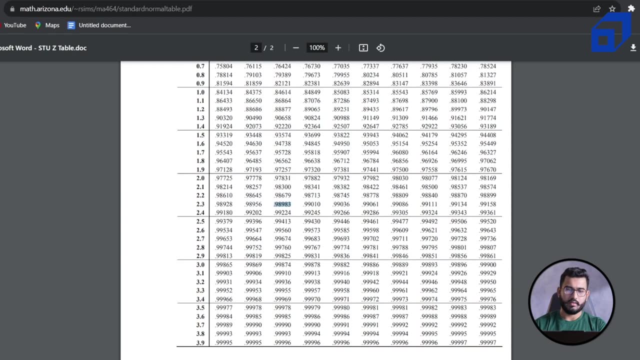 So let's use the Z table. So 0.99,. what is the Z value? So either we can go with this value or this value. So this is 2.32 or 2.33, so I'll go with 2.32.. 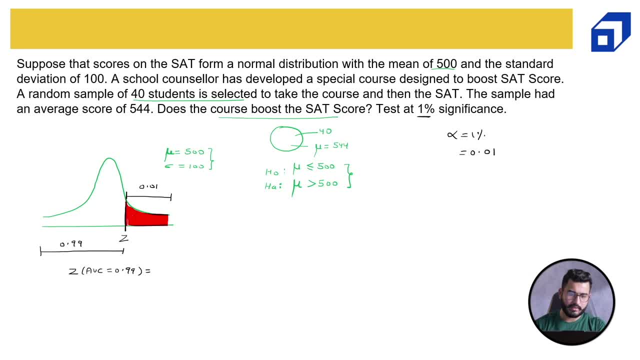 So Z value is 2.32 and this is plus. Now let's apply the formula mean plus Z times of sigma, divided by root of n. Remember the lower value will now be minus infinity. We have to just find the upper value. So mean is 500 plus 2.32.. 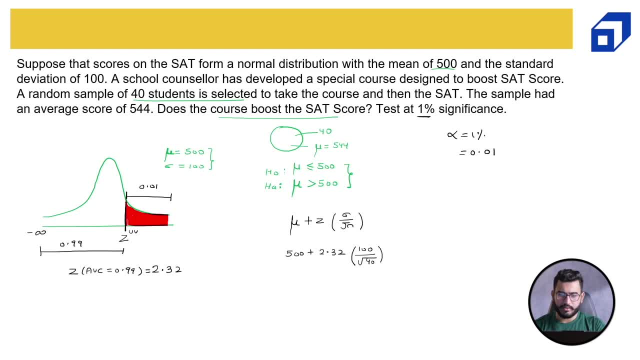 Sigma is, which is the standard deviation, is 100.. So this will come out to be 36.6.. So the total is 0.33.. The sample is 536.6.. So this value over here is 536.6.. 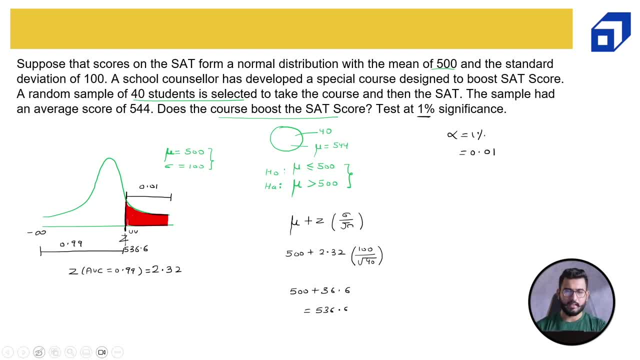 Now where my sample mean is lying at. My sample mean was 544.. 544 will lie on this side, right On the rejection side, this side, So this will be 544.. So, since my, since my sample mean is 544.. 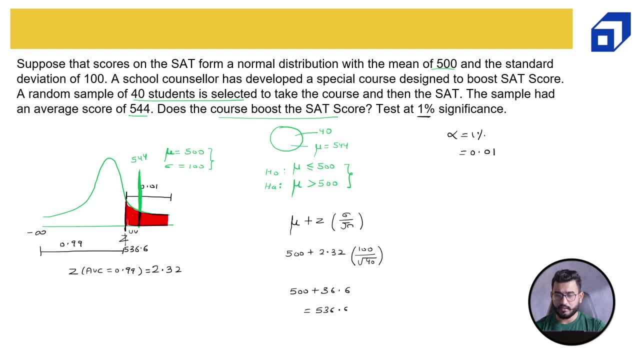 So since my sample mean is lying at the rejection region, we conclude that we reject null. So if I reject null, that basically means the course does increase the SAT score. The course does increase the SAT score. Now, please remember, this statement is based on this particular sample. 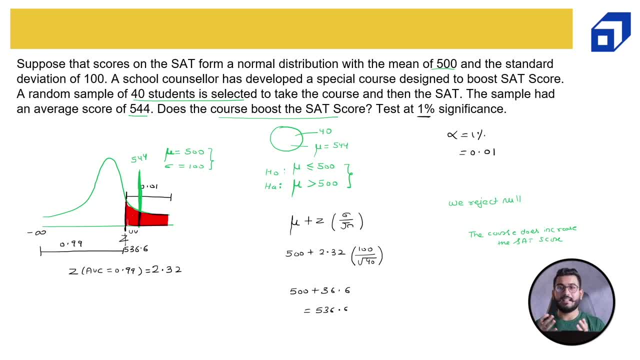 I'm not saying it will always increase. It will always increase the SAT score. Based on this sample, the conclusion is that course does increase the SAT score, But it might be because of some uncertainty. It might be because when we were selecting the students, we have only selected the intelligent. 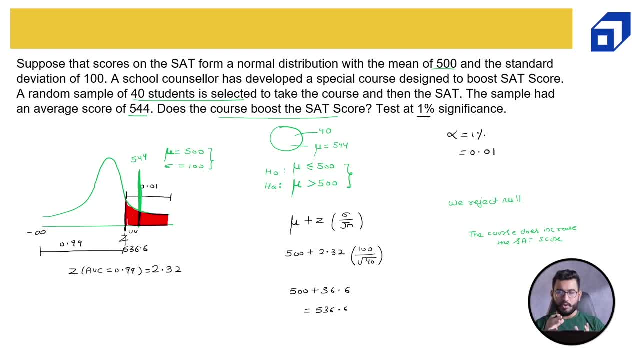 students with higher IQ And that is the reason we obtained the average, which is greater than the population average. Okay, So it might be because of the uncertainty also. So that is the reason we say we reject null. We are not saying we accept alternate. 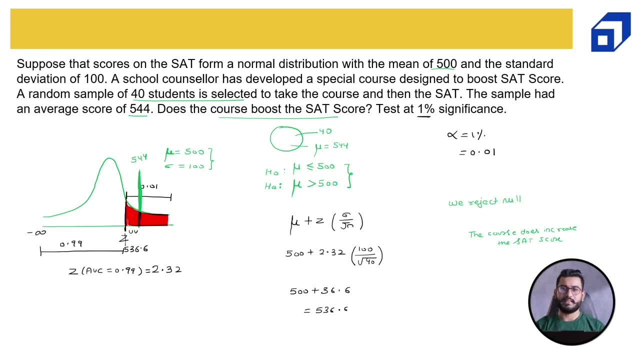 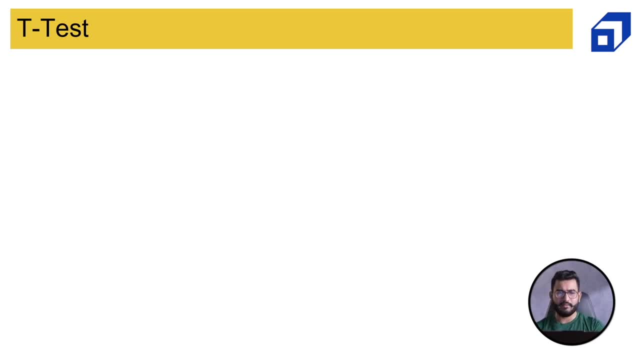 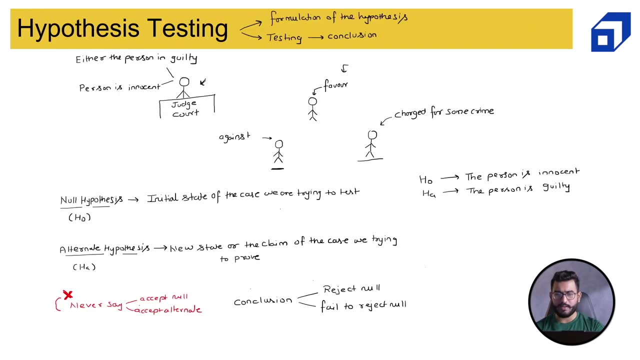 We will not say that. I hope now the thing is making more sense. So now let's talk about t-test. We have already seen z-test in very much detail. We have solved three problems. Now let's talk about t-test. And before we jump into solving few problems, 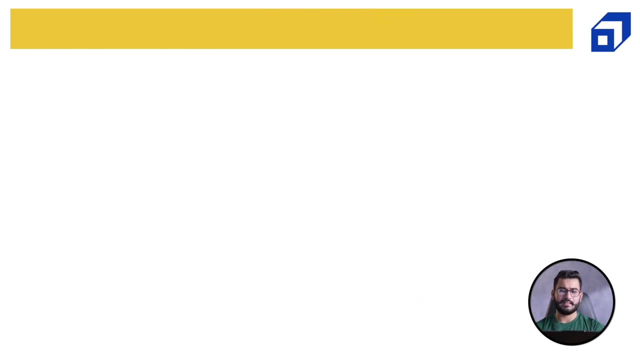 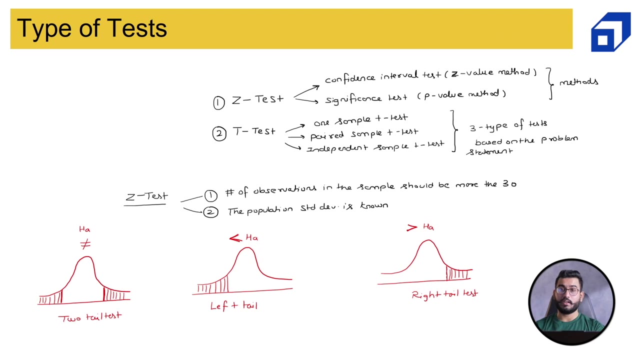 Let's talk about t-test. Okay, So we have solved three problems using t-test. Let's first of all understand when to use a t-test. So we have already talked about z-test. Now let's write down the conditions for t-test. 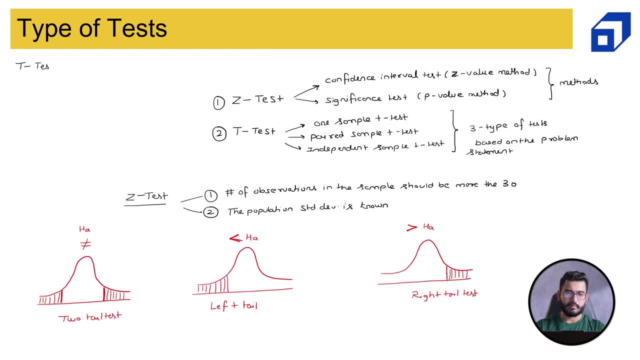 So I will write it over here: t-test. So we use t-test condition number one when the number of observations in the sample is less than 30. So the number of observations is less than 30.. This is my first check. The second check is population standard deviation is unknown. 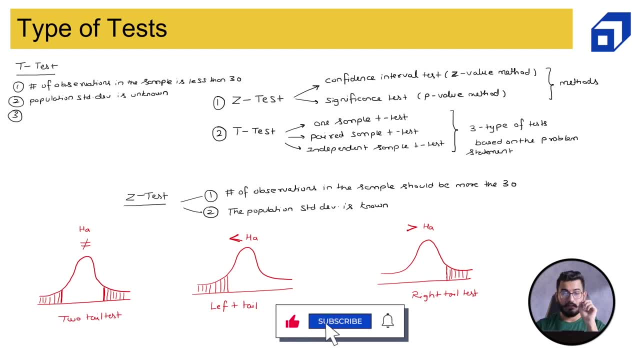 The third check is: the sample has been taken out from a population which is known to be normally distributed. The sample has been taken out from a population which is known to be normally distributed. Now, What is the difference? The difference meaning of the sample has been taken out from a population which is known to be normally distributed. 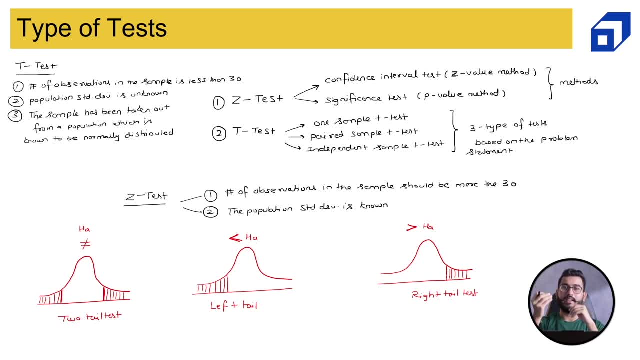 So let's say I take example of income. I know that in India the income is normally distributed. Now, if I take a sample of five people now, this sample will satisfy the t-test parameters because I know that it has been taken out from the population which is normally distributed. 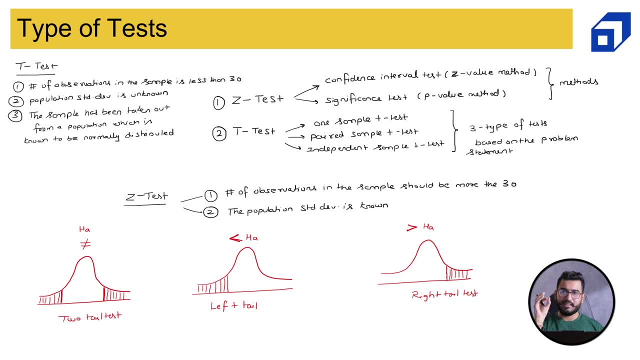 The number of observations in the sample are less than 30 and the population standard deviation is unknown. So I don't know what is the standard deviation of the income in my Indian population, because the population is really large, right? So before we apply t-test we have to check these. 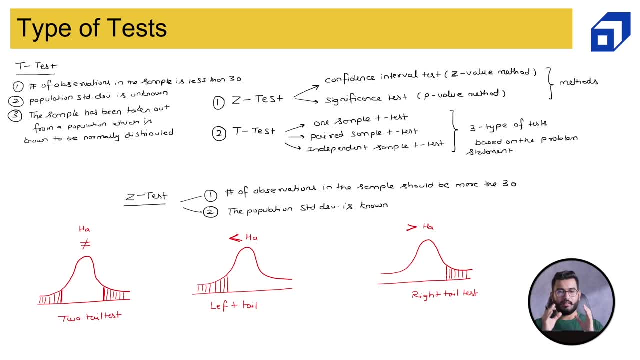 conditions, we have to check these parameters. Now let's solve a problem to understand this, As I have already told you that t-test can be performed, or there are three types of t-test based on the problem statement. So let's try to understand them very briefly: about what kind of problem statement satisfy which kind of t-test. 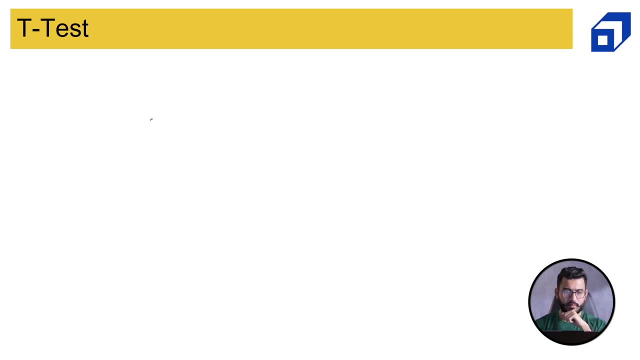 Now there can be three type of t-test: One sample t-test, paired sample t-test, boroboutplus, eight samplesf, mehrere t-test- visae k, Lydia A, Moscav computing and finally the independent sample t-test. 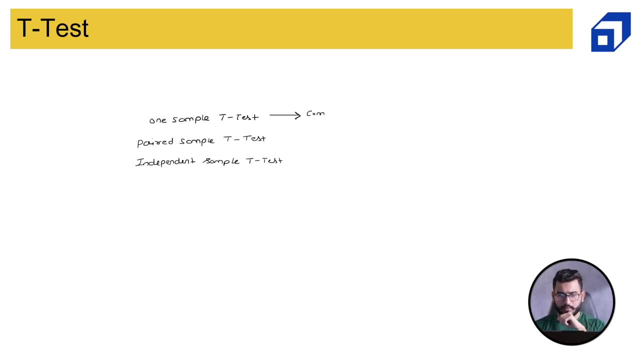 So, regarding one sample t-test, we try to compare the mean of single group with known mean for other group. Now, if it is not making sense, don't worry, we will. when we will be solving a problem, then I'll better explain you this Paired sample t-test. here we compare the mean of 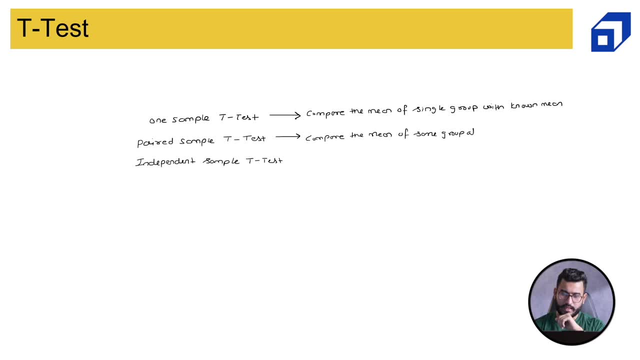 the same group at 2 times, or 2 times 2 different time, so at 2 different time. In independent sample t-test We compare the mean of Paired Sample t-test, two different groups. Now, if it is not making sense, don't worry, we will take example of. 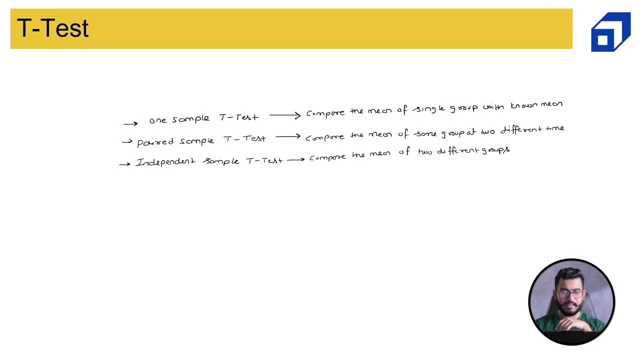 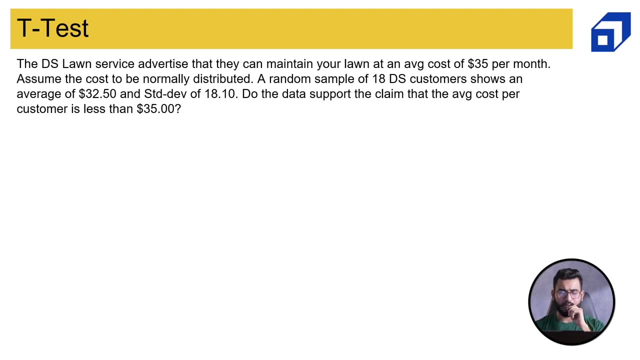 each one of them and then it will make more sense. Let's start with one sample t-test. So a DS lawn service advertised that they can maintain your lawn at an average cost of $35 per month. Now this is what their proven value is, the initial value that they have. 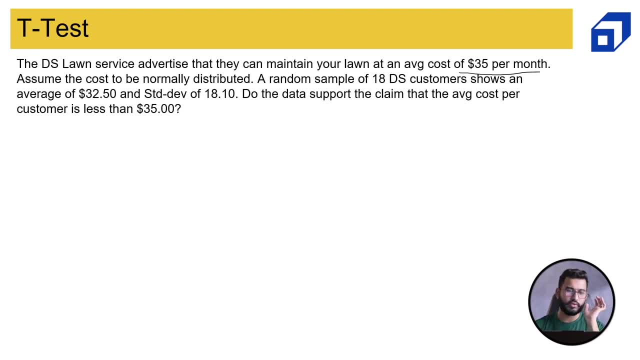 given. Assume the cost to be normally distributed. Now this is a very important sentence. The population is normally distributed. that has been given to us. A random sample of 18 DS customers shows the average of 32.50.. So we have 32.50.. 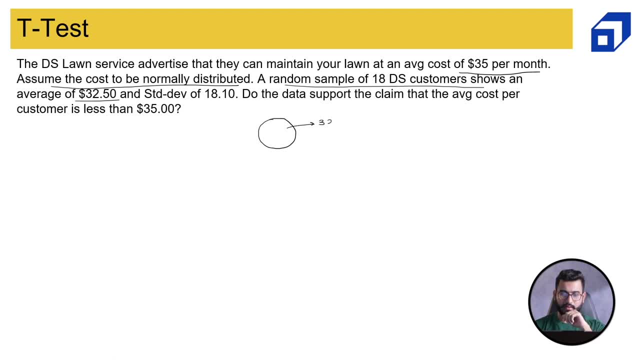 We have taken a sample. The sample is having the mean of 32.50 and the sample is standard deviation to be 18.10.. Now we know that this sample has been taken from a population in which the cost was normally distributed. Cost was normally distributed. So, first of all, 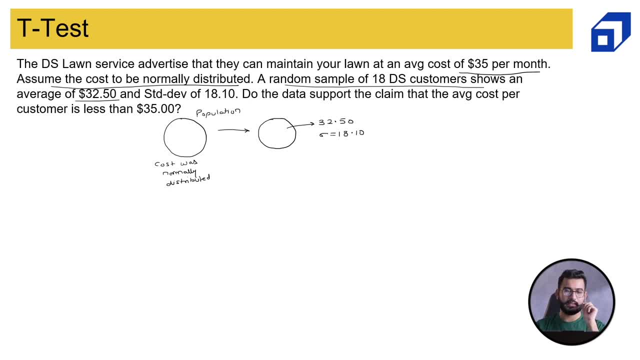 let's check whether this question or this particular problem satisfies the condition of t-test or not. The very first condition is: the number of observations in the sample should be less than 30. Here my n is 18.. So yes, first condition is satisfied. Second, 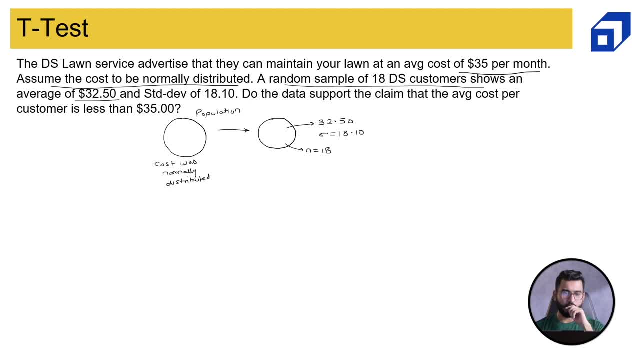 condition is the population standard deviation is unknown. Yes, we do not know the population standard deviation, but we know the sample standard deviation. And the third one is the sample has been taken out from the population which is normally distributed. So this particular sample has been taken out from a population where the cost was normally distributed. 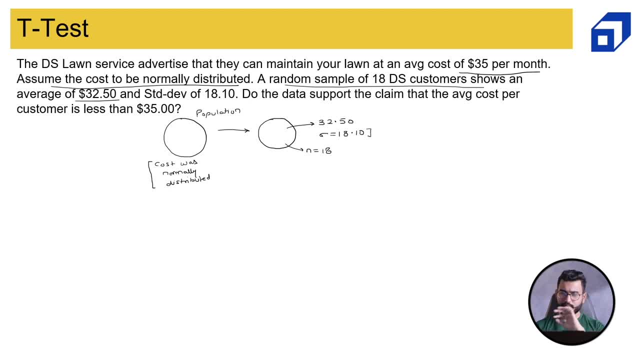 So all the three conditions are satisfied. Let's try to see the procedure Now. number one: we have to formulate the hypothesis. So my alternate hypothesis would be that the average average cost is less than 35.. So this is what we want to test. So average cost is less than 35. This is what we want to test. So 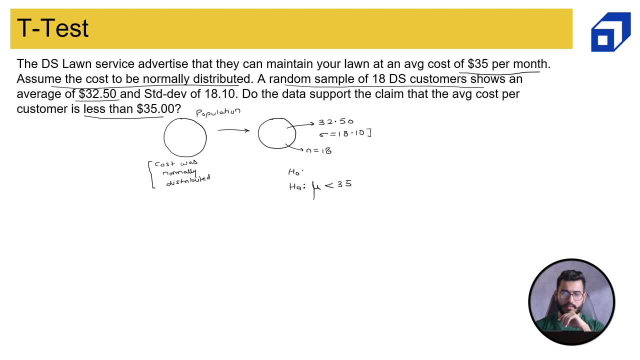 average is less than 35, null will be: average is greater than or equal to 35.. So this is my null and alternate hypothesis. Again, since I am having less than sign, in my alternate it is a lower tail test. So lower tail test. Now we will find out the t critical. Now t. 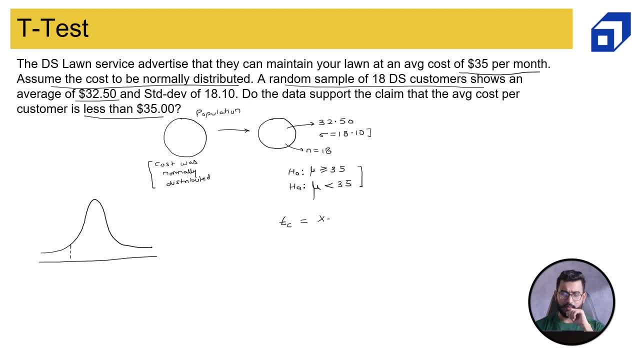 critical formula is similar to z value, x minus mu, divided by sigma, divided by root of n. I hope you guys remember the z value formula. when we were talking about the z scaling, The z value formula was x minus mean divided by sigma. Now here I am using sigma divided. 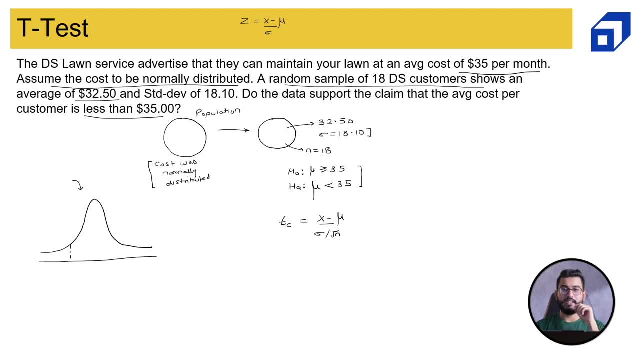 by root of n is because this distribution is a sampling distribution and the standard deviation of the sampling distribution is given as sigma divided by root of n, according to the central limit theorem. right Now, what is x? X is my sample mean, which is 32.50.. Mu is my population mean, which is 35 divided by sigma 18.10 divided. 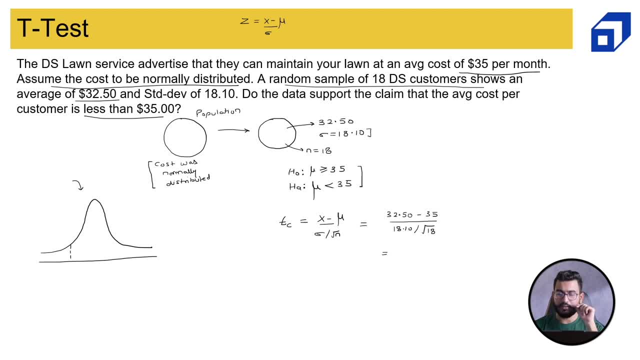 by root of 18.. What is the value? You guys can quickly calculate it. I have already calculated it. So this will be minus 1.30.. Sorry, there is a one, one correction. This is not t critical. This will be t estimated. t estimated. 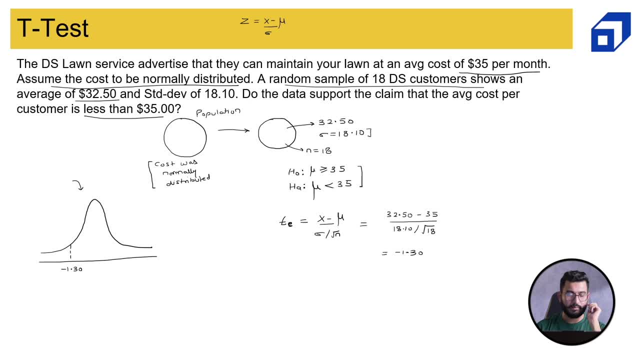 So t estimated is 1 minus 1.30.. Now we will find out the t critical, which is calculated using the t table, and t table requires your alpha, which is given as so okay, I haven't written alpha, So let's assume alpha to be 0.05.. So alpha is 0.05 and degree of freedom. Now, degree of freedom is given as 0.05 and 0.05, and the term that I am going to use when I am calculating alpha is: Let's say that I am going to read alpha and I am going to write alpha as alpha, and I am going to write alpha as alpha, So alpha is 0.05.. So alpha: 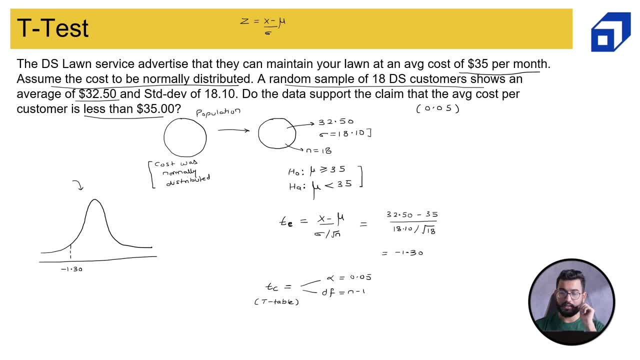 is 0.05.. So alpha is 0.05.. So alpha is equal to 0.05.. That is the whole example. So alpha is given as n-1.. But what is degree of freedom? What is degree of freedom? So let's understand. 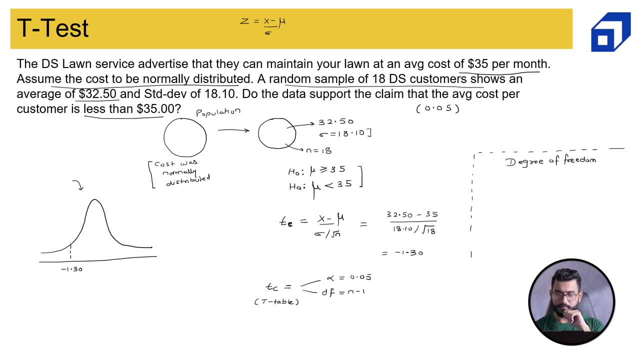 degree of freedom. Now, let's say there are 3 people: 1,, 2 and 3.. These are the 3 people. and let's say these are A, B and C, And this is Sumit. Now what I am asking A, B, C to do. 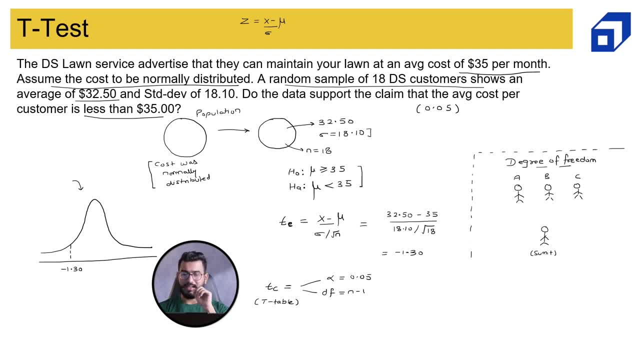 I am asking A, B, C to choose one number in such a way that the total is 10.. Now, let's say so. let's write down A, B, C, Sumit And the total. Now we already know that the total in all the cases would be equal to 10.. 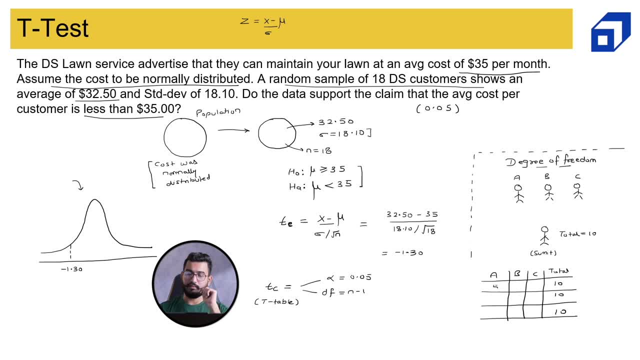 So let's say A has chosen 5, B has chosen 3.. Then C is bound to choose 2.. Let's say A has chosen 5, B has chosen 5.. Then C is bound to choose 0.. Let's say A has chosen. 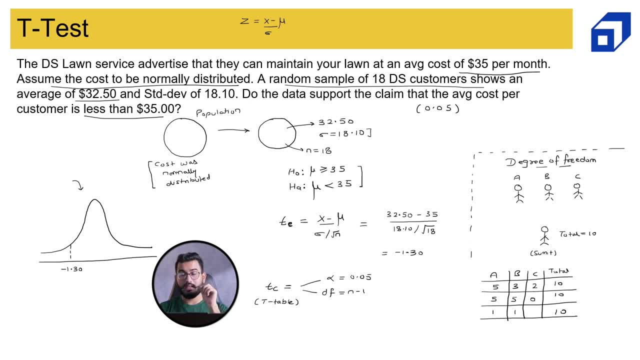 2, B has chosen 4.. Then B has chosen 6. But A has chosen 1.. So let's say C has chosen 1, B has chosen 1. Then C is bound to choose 8.. Now you hear, you guys can see that the 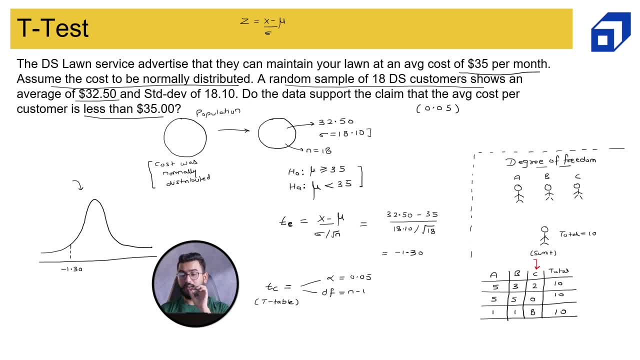 third component, or the third data point in my summation, is not free to choose a value when we already know the total: Sumitica & Singh, Sumitica & persuade, Sumitica & persuade, Sumitica & persuade. C is always bound to choose a value that is left out. So degree of freedom talks about how many. 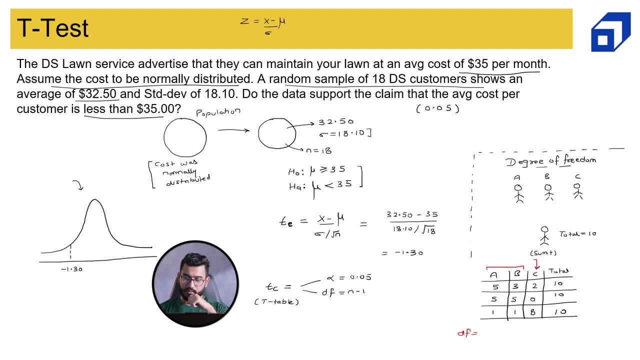 observations in your data, are free to choose a value: The number of observations in the data, in the data that are free to choose a value. Now, here, since we know the sample average, since we already know the sample average, the degree of freedom will always be n-1. 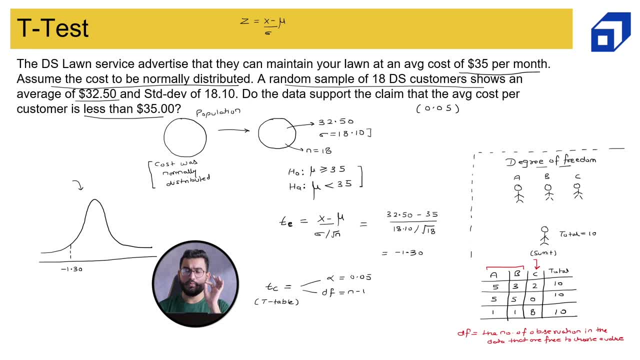 because there will be always one value which will be bound, or to choose a value that can make the average to come out to be what we are given with. So here, degree of freedom will be n minus 1,. n is 18, so 18 minus 1 is 17.. Now we will use the 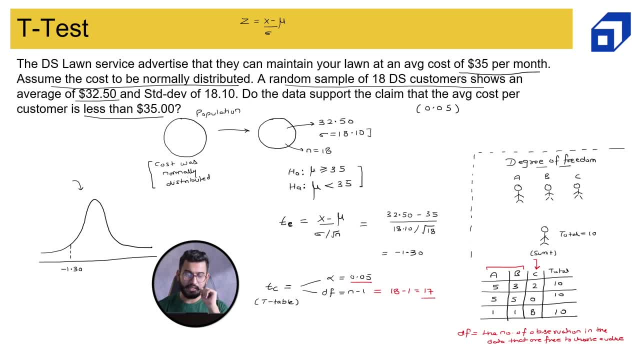 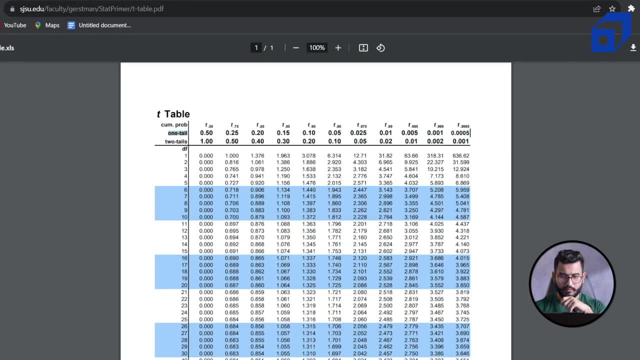 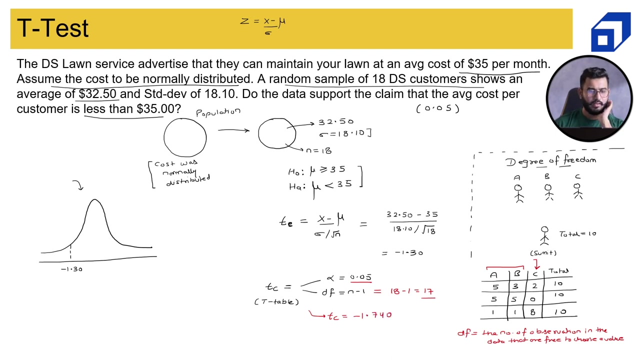 t table with these two parameters to find out the t critical value. So let's use the t table. So this is a one tail test with the significance of 0.05 and the degree of freedom to be 17.. So here, so correct value is minus 1.740.. So t critical is minus 1.740.. Now I 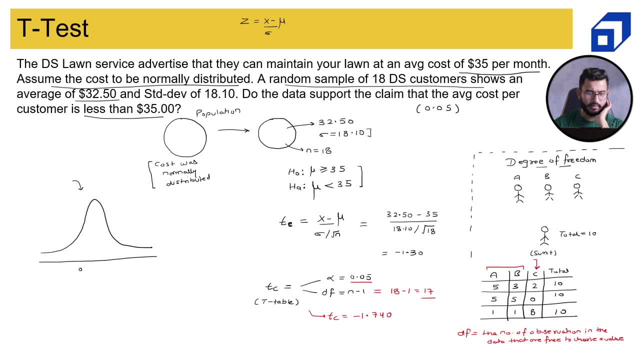 will quickly delete this because I do not have to write this first. First of all, we will write the t critical minus 1.740.. Now, where this minus 1.30 will lie? Well, it will lie. t estimate, t estimate will lie, let's say so. minus 1.3, minus 1.3 will lie over. 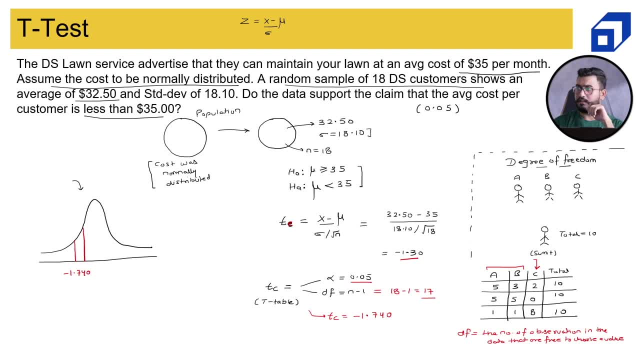 here, right? So this is my, this is my rejection region, This is my rejection region, which is below the t critical value And my t estimated is beyond the t critical value. So this is the boundary of t critical and this is my t estimate. Now, since t estimate is on the 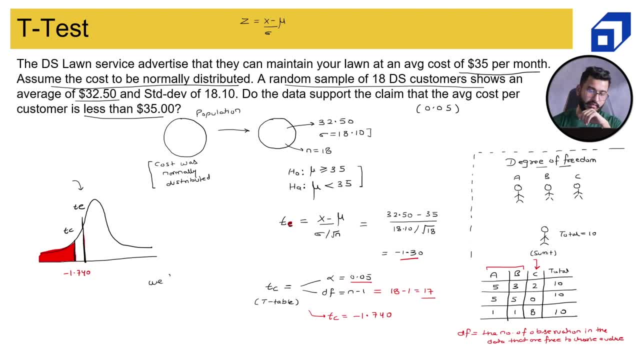 accepting side, we say that we fail to reject null, which basically means that this statement- it is greater than or equal to 0.. 35, that basically means those people, or those people who were doubting, who were having the doubt regarding this DS loan service, they were actually correct that, based on this. 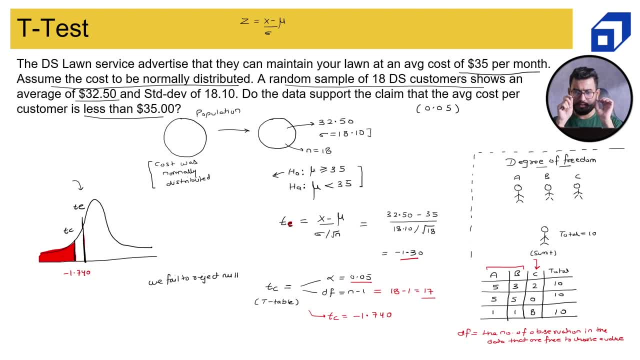 sample, we can conclude that the average cost that this DS loan service charges for maintaining a loan is not 35 or less than 35, it is more than 35.. I hope this is making sense. This was one sample t-test, One sample t-test. 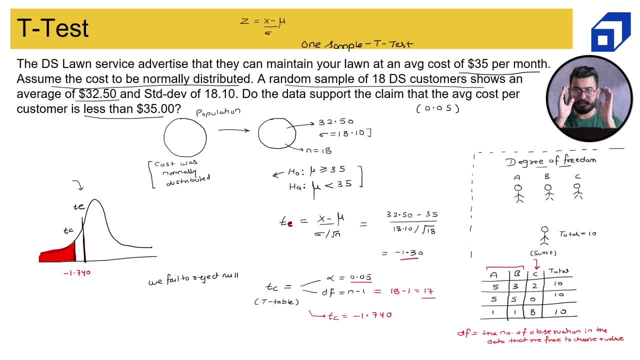 Now the reason it was one sample t-test is because we have one group, we have a known mean, which is 35. And we are comparing the prices sample mean with the known mean. So this is one sample t-test. Now in the paired, 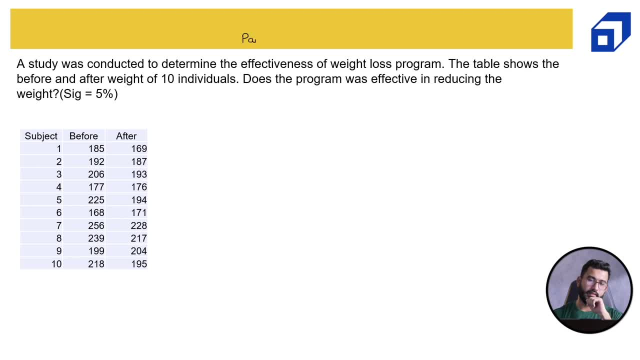 sample t-test. this is the example of paired sample t-test. Here we compare the average of one group at two different time. So here you can see that we have before result and after result. Let's try to solve this problem to better understand this. So here in this question we are given with the problem. 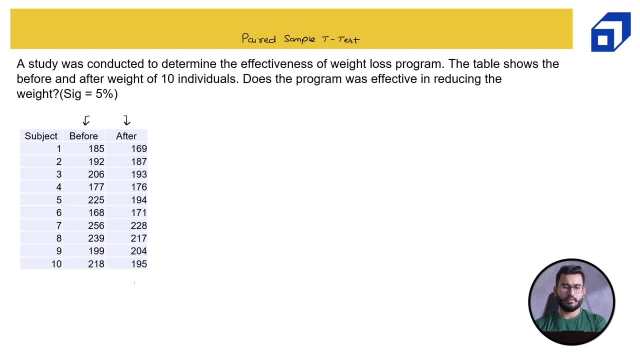 statement states that a study was conducted to determine the effectiveness of a weight loss program. The table shows before and after weight of 10 individuals Does the program was affecting in reducing the weight? We have to test at a significance of 5%. Now if we logically think about this question. 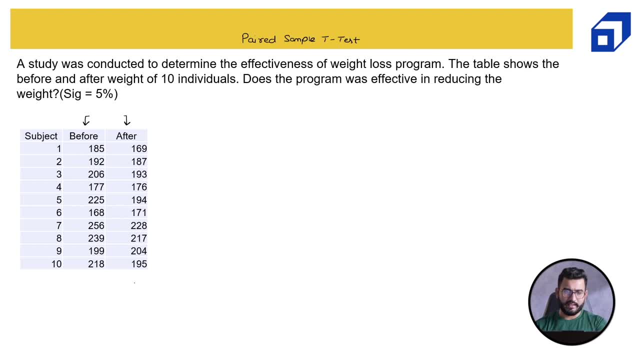 the program will be called effective when the difference- What is the difference After minus before, When the difference is negative? So let's calculate the difference. I have already calculated it, So I'll just fill the table. So 169 minus 185 minus 16 minus 5 minus 13 minus 1. 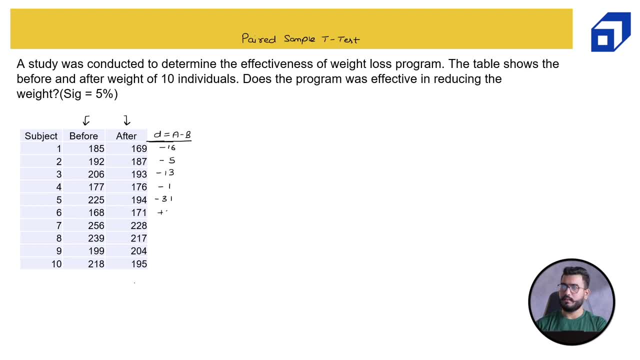 minus 31 plus 3, minus 28.. Minus 22 plus five and minus 23.. Now these are the differences. If this differences negative, that basically means The person obtained or the person achieved the weight loss. If it is positive, that means: 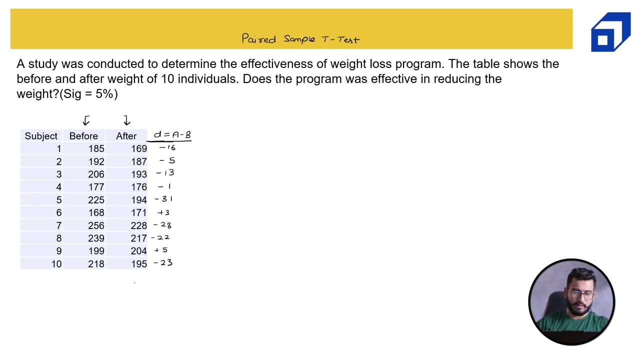 the person achieved gain. So if I look at this observation of individual number 6, the person was having a weight of 168, it increased to 171. So the person gained 3 units of weight, while this person, whose weight was 218. now it came to 195.. So this individual achieved a loss in. 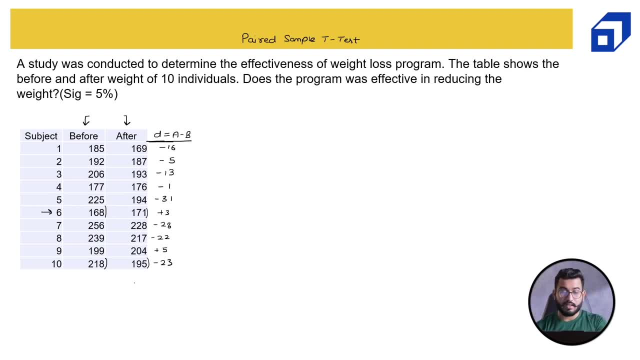 the weight of 23 units. Now I will call this program effective if the average difference is below zero. right Below zero means negative. So my alternate, my null alternate hypothesis will be: the average is less than zero, because initially I will consider that the program 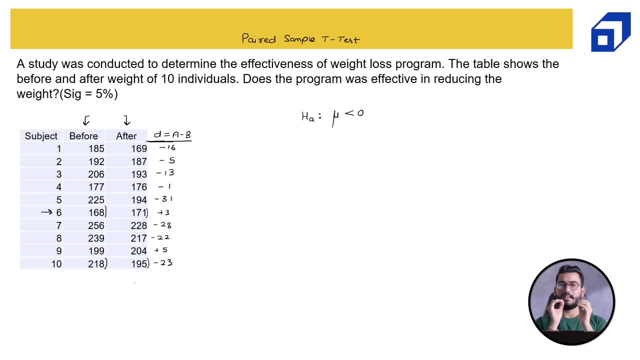 is not effective. Initially I will consider that the program is not effective. So initial statement will be: the average is either greater than or equal to zero. So assume that this is a number line of differences d, where if my average average difference is zero or above, this is zero or positive, then my program 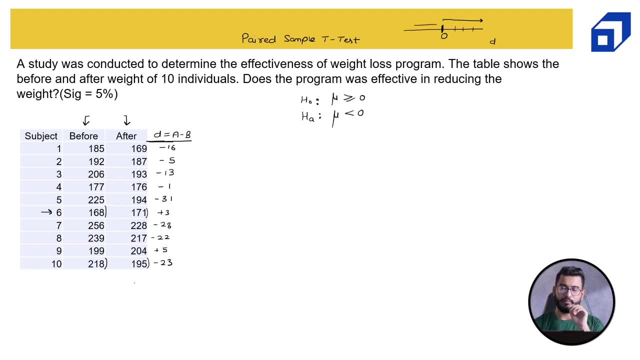 is not effective. If it is negative, then my program is effective. So these are my null and alternate hypothesis. Now what we have to do. this is my sample, So I need the sample mean. So mu x, My average of differences. So I'll just write mu d, The. 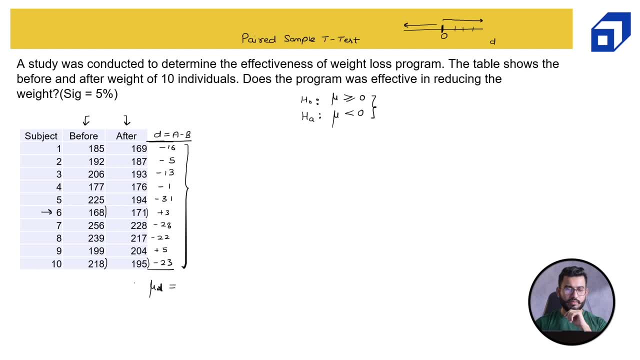 average of differences. I have already calculated it. You guys can use Excel for this quick calculation. So the average difference is minus 13.1 and the standard deviation of the sample is 13.02.. This is my sample statistic. Now I will calculate the t estimate. T estimate is x-mean divided by sigma, divided by root. 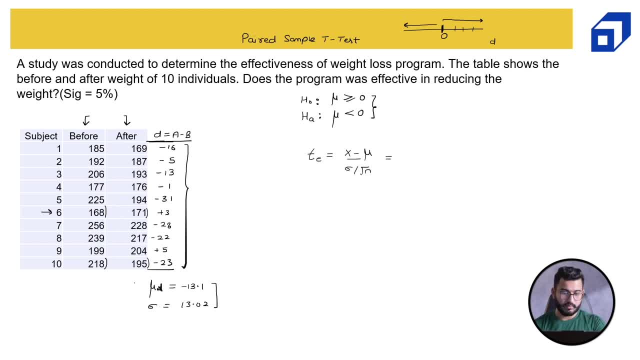 of n. My X is greasy minus 13.1.. My mu is 13.1.. Population mean is zero. Population mean is zero, which we have, as we know, at least 10,000,. we can say that I know what that is. 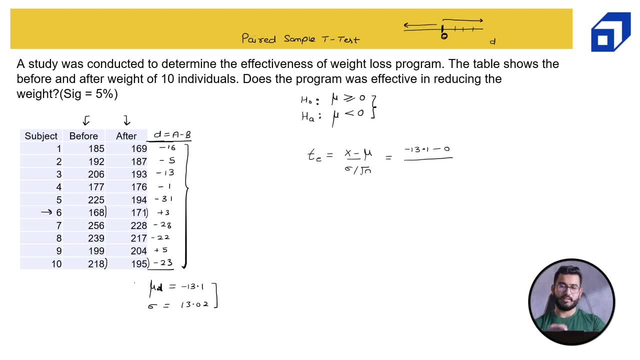 we have assumed that there is no change, there is no gain, there is no loss. zero Sigma is 13.02. divided by root of n, n is 10.. Now this will come out to be minus 3.18.. 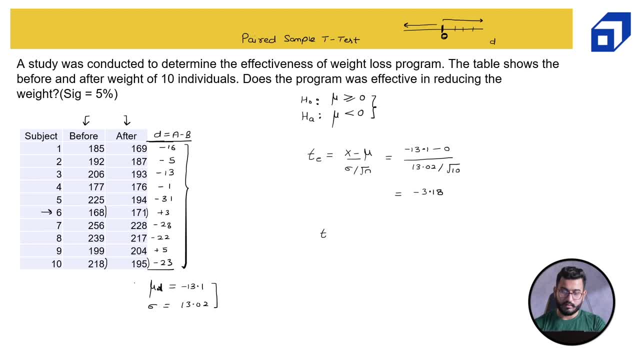 Now using the alpha, which is 5%, so 0.05, and degree of freedom, which is n minus 1,, which is 10 minus 1,, which is 9,, I will find out the t critical using the t table. So let's quickly do. 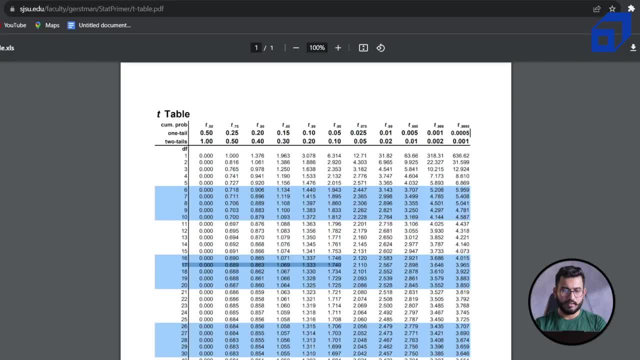 this. So degree of freedom. So this is a one tail test. significance: level: 0.05, degree of freedom to be n: 9.. So here we have the value 1.833, 1.833.. Now, since it is a lower tail test, because 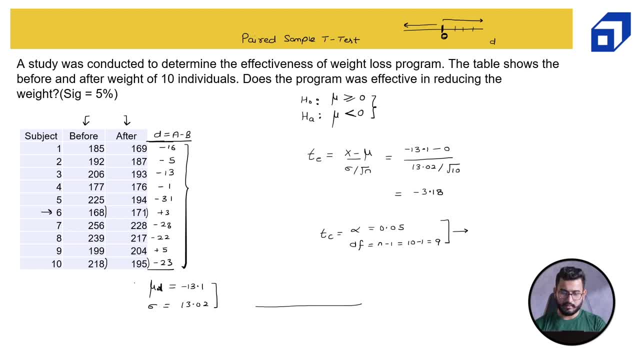 I am having lower sign or less than sign. so the value t critical will be. let's say this: t critical is minus 1.833.. Now, where this minus 3.18 will lie? Minus 3.18 will lie over here t estimate. Now, since it is lying on the rejection region, we conclude. 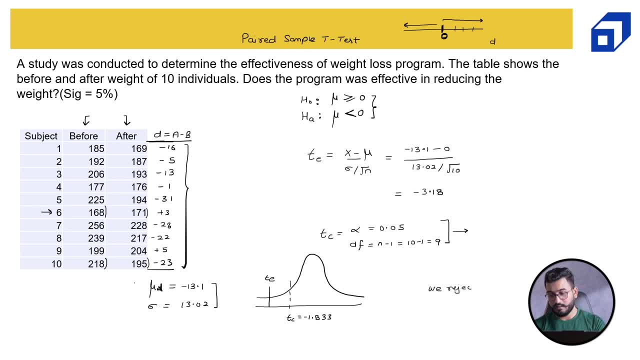 that we reject null, which basically means. which basically means: yes, based on this sample, the program was actually found effective. So, yes, based on this sample t estimate, The program was found to be effective. Now, here you can see that the reason we call this 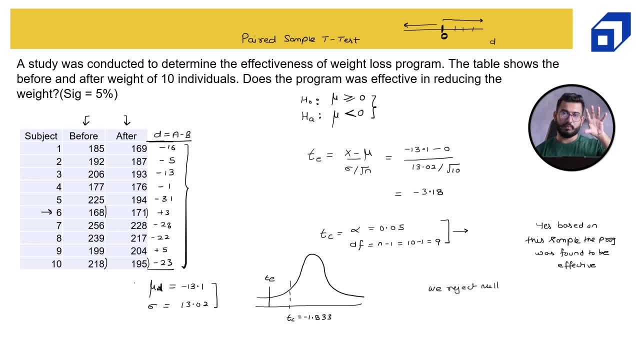 as a paired sample t test is because we were having the same group but at two different times, before and after, Same set of people before and after. So paired sample t test We are. we are comparing their average or the average difference. 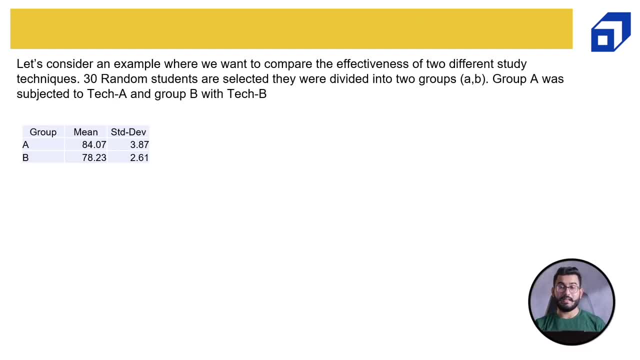 Now we have independent sample t test, which basically means now we have two different group, group A, group B, and we have to compare them. So let's see this example. So this is the example of independent sample t test And in this particular test we are having two different. 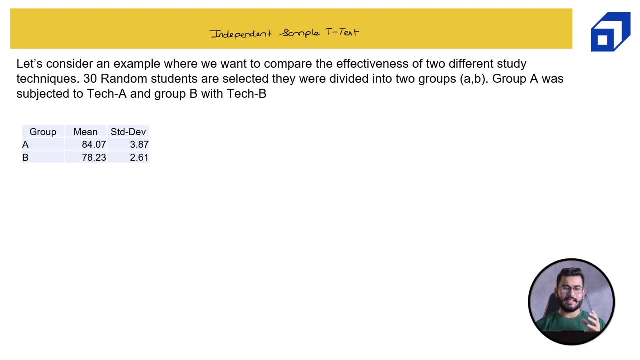 group. Now, if you read the question, it says: let's consider an example where we want to compare the effectiveness of two different studies. So we will be comparing two research techniques. uh, 30 random students are selected. They were divided into two groups. 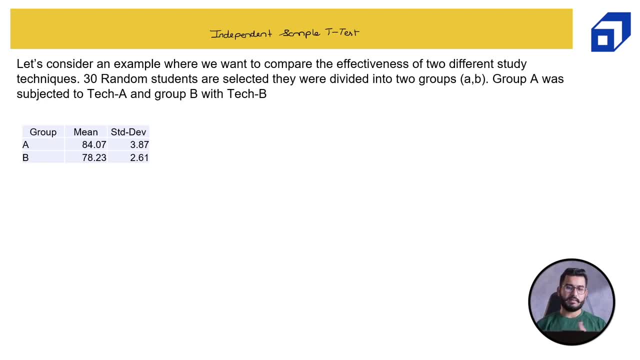 Group a was subjected to technique A. Group b was subjected to technique B. Now, please remember, uh, I'm having total number of students to be 30. Where, uh, we have divided them into two equal groups. So that basically means group A consists: 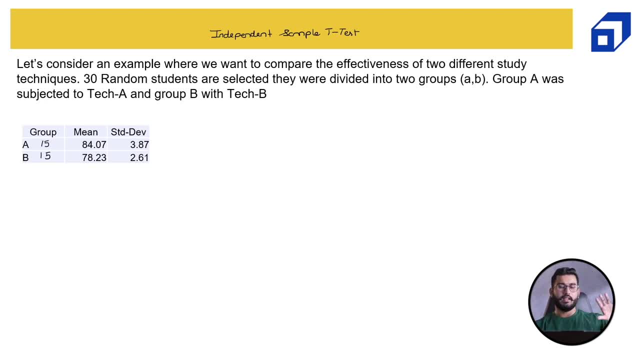 of 15 students. Group B consists of 15 students. Group A consists of 15 different students- different students. group B consists of different students. so these two, these two groups, are not having any association between them. they are two different groups. now I want to compare whether technique A and technique B. 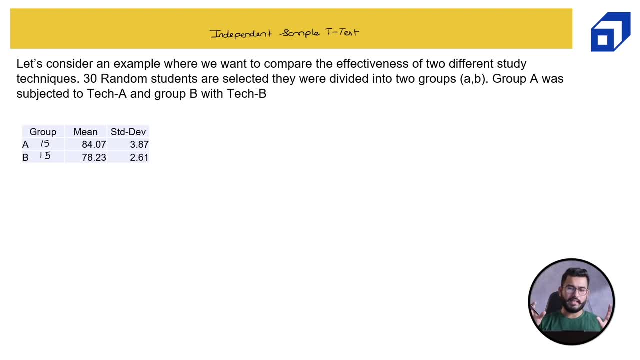 whether they are same or different. that's what my tested: whether they are same or whether they are different. so my alternate hypothesis will be: average of A is not equal to average of B. my null hypothesis will be: average of A is equal to average of B. so my null hypothesis is that I am initially assuming that these 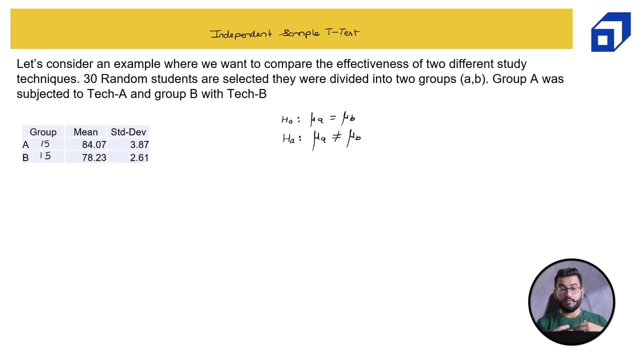 two techniques are same, where what I want to prove that these two techniques are different. so that's my null and alternate, alternate hypothesis. now we will follow the same procedure, but there will be a minute difference in the t equation estimate. The formula for t estimate is: x1- average minus x2. average minus mu1 minus mu2. 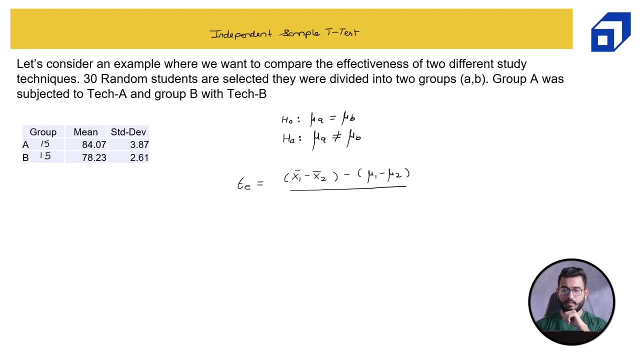 divided by square root of sigma1 square divided by n1, plus sigma2 square divided by n2.. So here in my table I'm already given with mu1 and mu2.. So let's fill the table, fill this formula: mu1 is 84.07 minus 78.23 minus mu1 and mu2.. So we are assuming that mu1 is equal to mu2.. 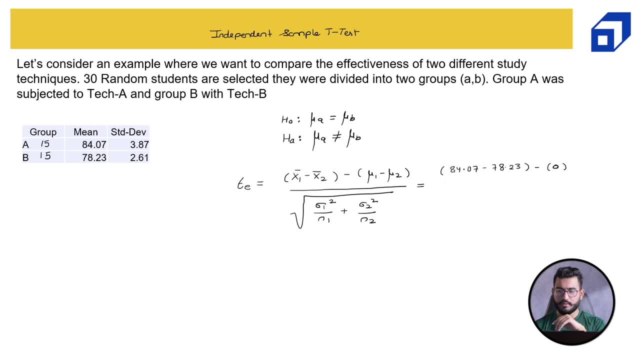 So this will come out to be 0.. Since we are assuming, my null hypothesis is that these two average, the population average, are same, So mu1 minus mu2 will always be 0.. Then square root of sigma1 square, So 3.87. 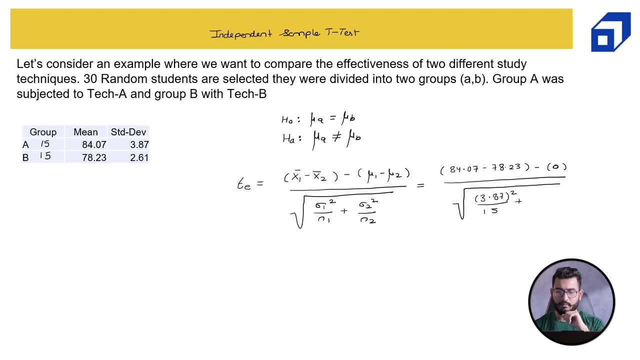 to the whole square divided by n1,, which is 15 plus 2.61 to the whole square divided by 15.. If I solve this, we will get 3.02.. This is my t estimate. Now, this is a two tailed test, right. 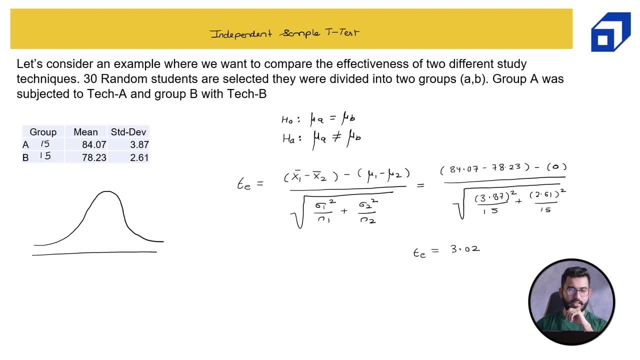 This is a two tailed test because I'm having 0 equal to sign my alternate hypothesis. Two tailed test We have not given with alpha. Let's assume alpha to be 0.05.. So this portion will be 0.025.. This portion will be 0.025 and both are my rejection region. 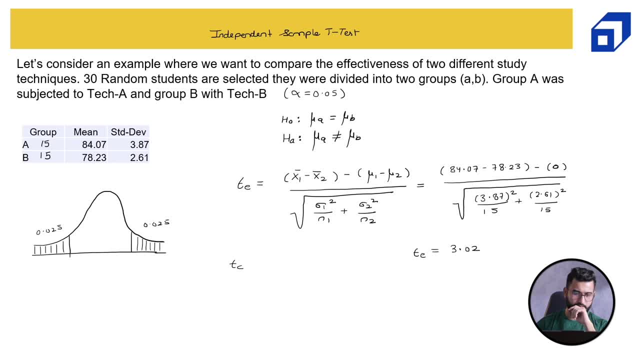 Now I want to find out T critical, which is this point? T critical? Again, we have to use alpha, which is 0.025, and we need degree of freedom. Now, in the case of independent sample T test, the degree of freedom is given as N minus, so degree of freedom is given. 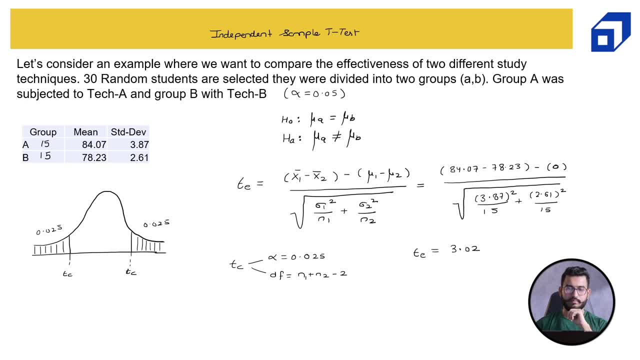 as N1 plus N2 minus 2.. So my N1 is 15 plus 15 minus 2, which is 27.. So I will be using alpha 0.05,- sorry, alpha 0.025, T critical as 27 to obtain the T critical value using 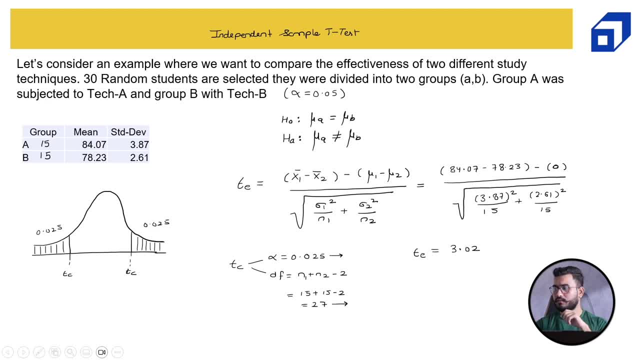 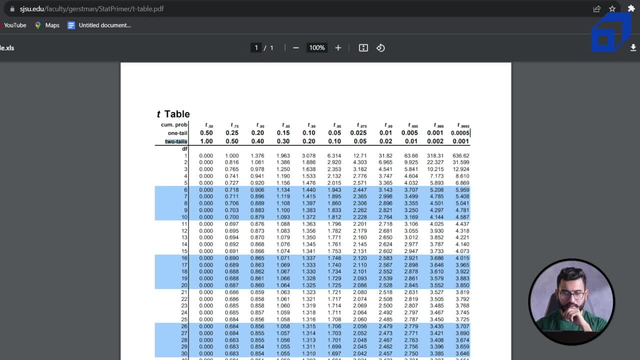 the T table. Let's do that. So I am now in the two-tailed test And we have to look at 0.025.. So two-tailed test alpha is given as 0.05, right Alpha. 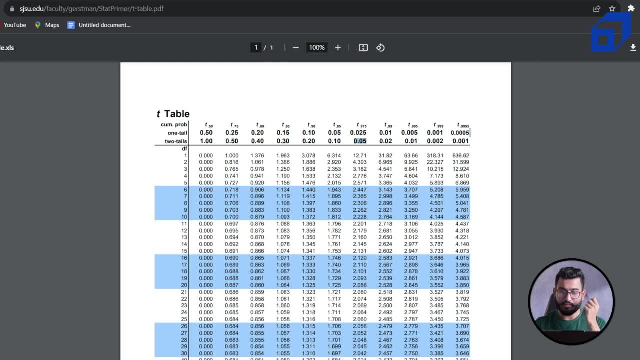 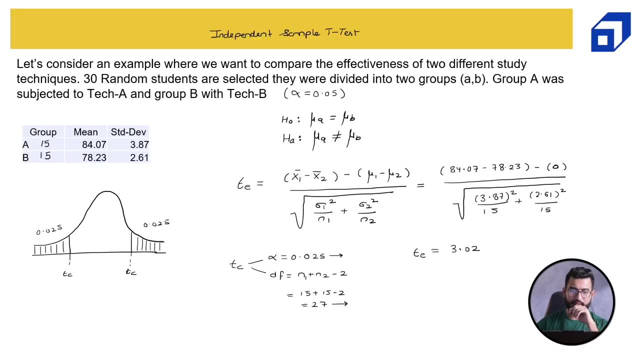 is given as 0.05.. We can use so what is my, what I have done, Since I have divided it by 2 in my T table. it gives from the left. it gives the T critical value from the left. 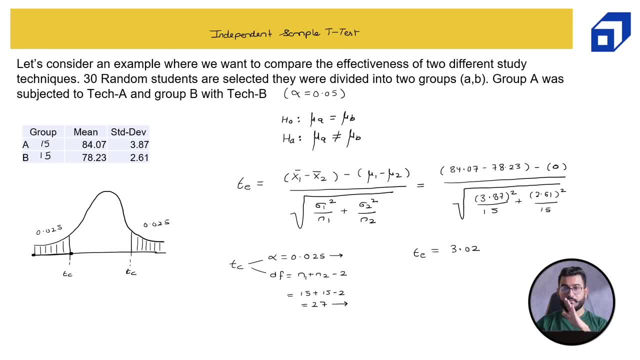 So if I go with 0.025 from the left, I will get this value, And if I go from this value to this, if I have to find out this value, it will be 0.05, see 0.95.. So let's use. 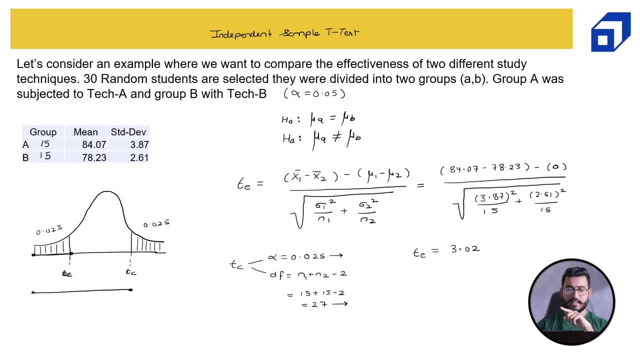 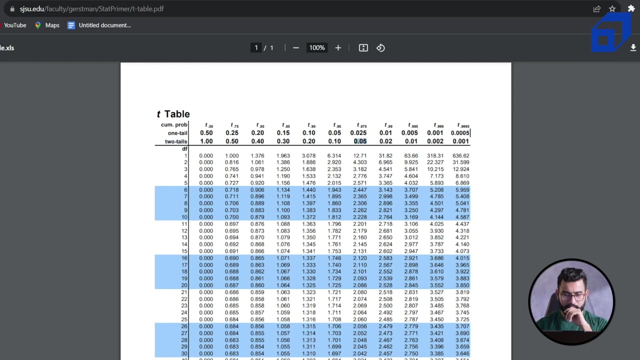 one-tailed test or, if you want to use, you can use two-tailed test at the alpha of 0.05.. We can use any one of them For avoiding any confusion. tail test at alpha of 0.05.. So let's look into that. So two tail test: alpha is 0.05 and we 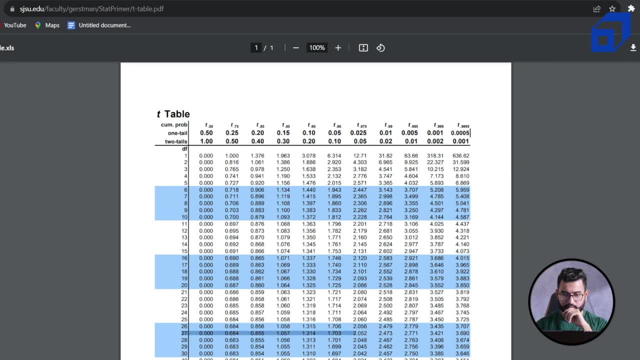 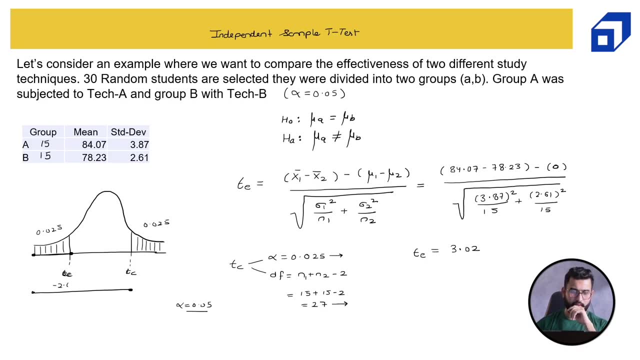 are given degree of freedom as 27.. This is 2.052.. So my decretal is minus 2.052 and this will be plus 2.052, right, Because always they are complementary to each other. 3.02, where this: 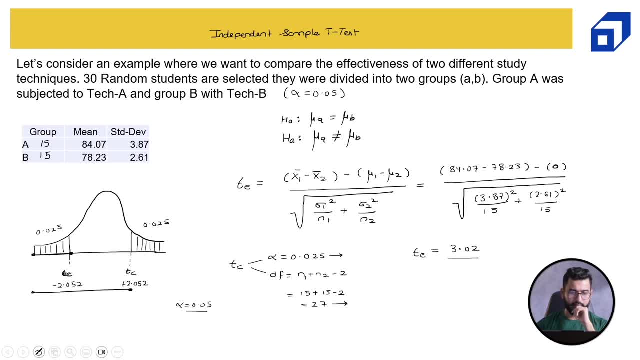 will lie. 3.02 will lie somewhere over here on this rejection region. This is T estimate, Since it is lying on the rejection region. we say that we reject null, And when we reject null basically mean they are not same. 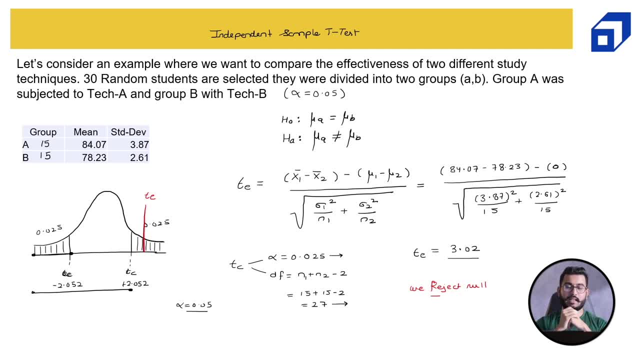 They are different. So, based on this particular sample, we can give that these two techniques are different from each other. So, based on this sample, we can give that these two techniques are from each other. This is what independent sample t-test is. Now we have completed our. 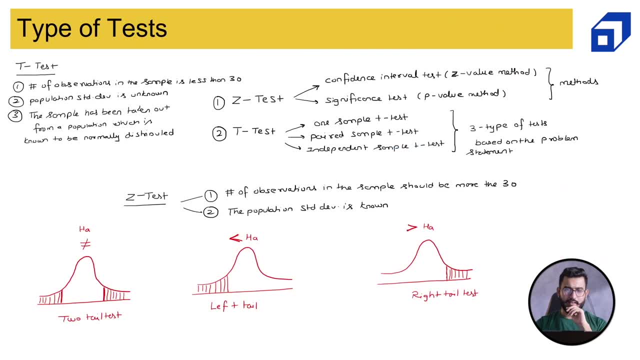 discussion on hypothesis testing. So we have talked about how we can perform. So we started our discussion with how to formulate the hypothesis. Then we talked about the two kind of tests: z-test and t-test. Within z-test we looked at two methods: z-value method, p-value method. 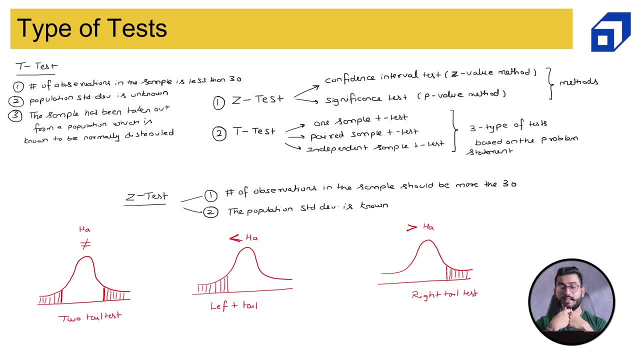 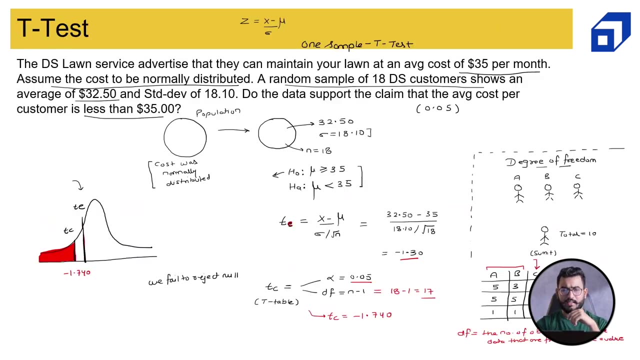 Within t-test, we looked at the various types of tests, which are based on various types of problem statements- One sample t-test, paired sample t-test, independent sample t-test- and we solved a variety of problems, also to make our understanding more concrete. Now we are going. 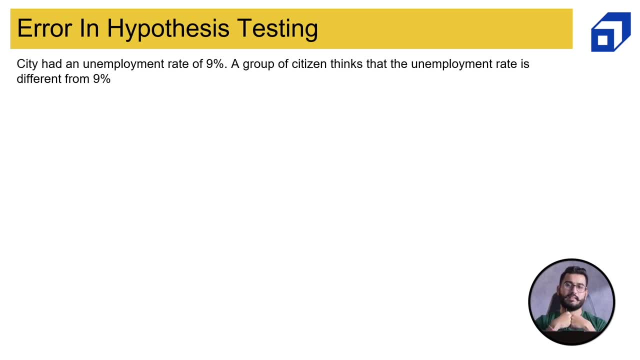 to talk about a topic which is known as error in hypothesis testing. As I talked initially that there might be some uncertainty that my test goes wrong, Since this is a test which we are performing on the sample, we can never be 100% sure that what. 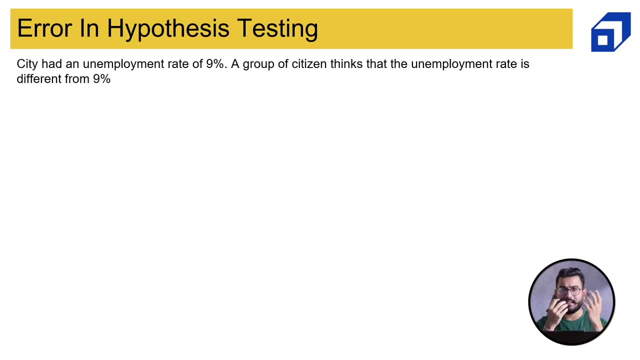 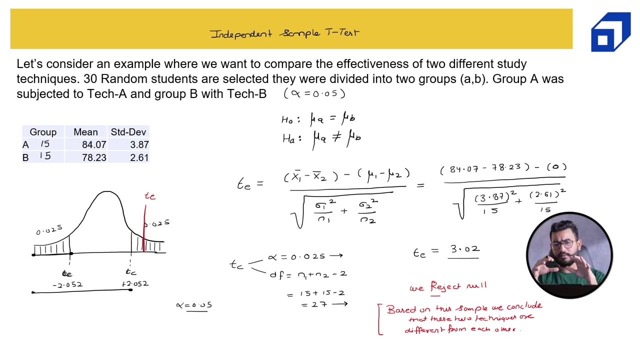 result my test is providing us, or the conclusion that we made from the test, is always going to be 100% true. Let's say, my test concluded that we reject null. or let's take one example: In this particular example, we have rejected null right. What if this was actually not true? So, based on 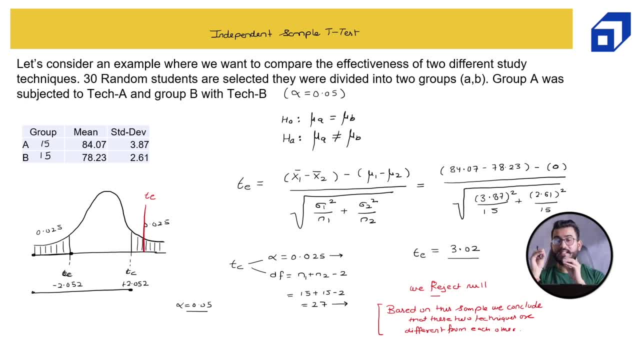 these two samples, we can say that we have rejected null. So, based on these two samples, we can say that we have rejected null. So, based on these two samples, we concluded that we reject null. But what if, in reality, overall? so, as of now, we have taken a sample of 15, 15 students And just because of 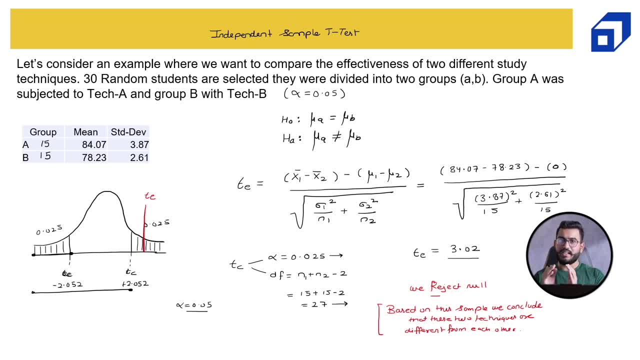 the sample of 15, 15 students, we concluded that we reject null. But what if? in reality, if I take a much bigger sample, in reality, this, this is not true. This is not true. Both techniques happen to be same, Then that is known as the error in hypothesis testing. So how we can. 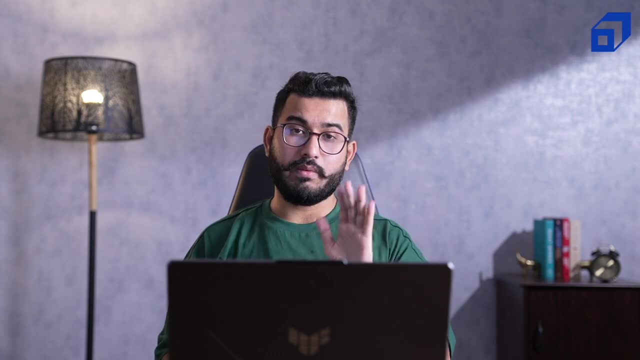 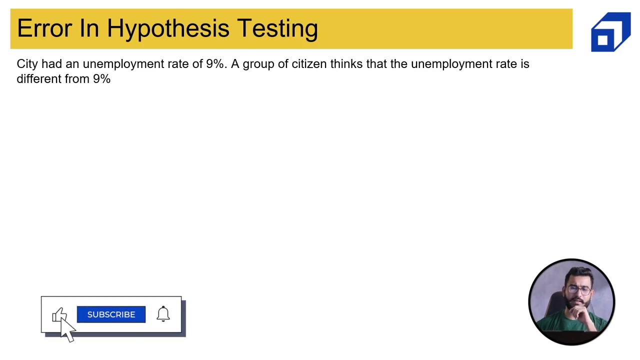 avoid this error. Before we can avoid this error, we have to be very much clear with what kind of error hypothesis testing can lead us, or what kind of errors we can encounter while performing hypothesis testing. Let's try to understand that now Before we talk about this particular problem. 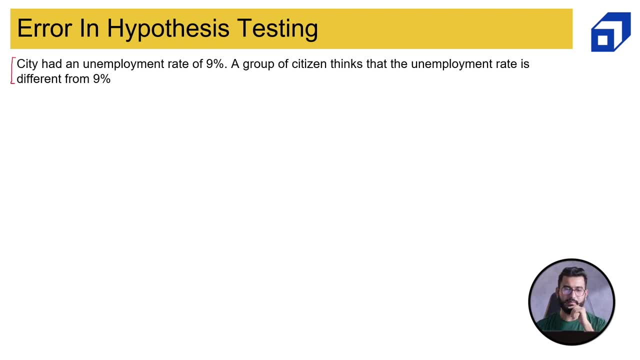 so I have written one condition. or I have written one condition, So I have written one condition. or I have written one problem statement. Let's try to summarize what are the various error we can encounter while performing hypothesis testing. So we can summarize the type of error in a two. 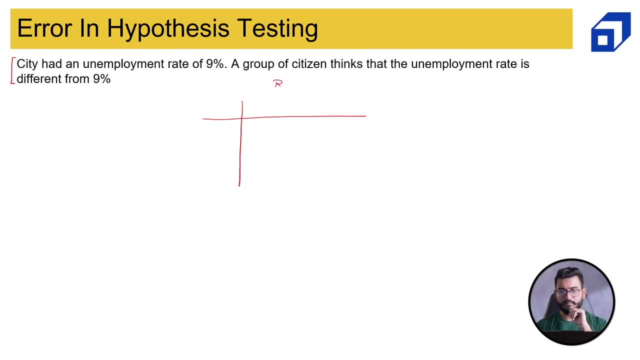 cross two matrix. This is the reality And this one is the test result, Or hypothesis test result. Hypothesis test result: Now, there can be four type of scenarios. So in reality, the null hypothesis was true. So H naught was true And H naught was false. Here we rejected. 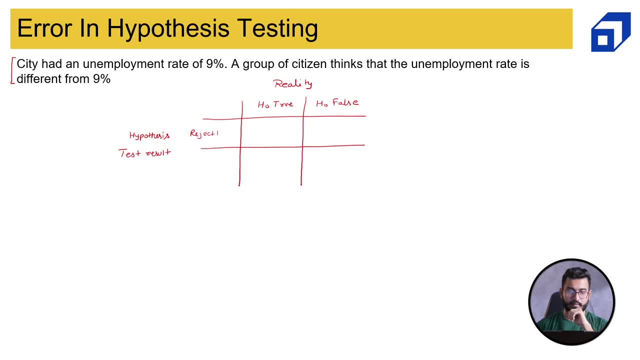 H naught And we failed to reject H naught. Now, when H naught was false and we rejected H naught, this is a good thing, right? So this is my correct conclusion. So I'll write correct over here. This is correct. 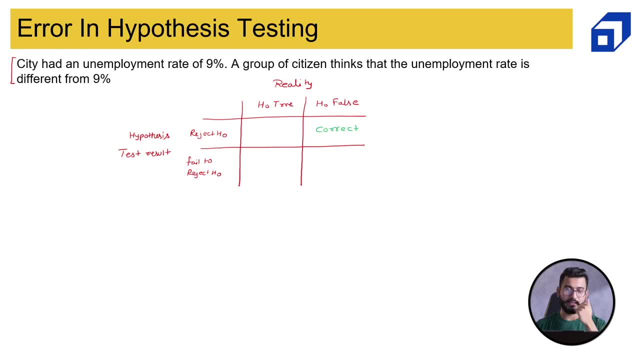 When my H naught was true and we failed to reject H naught. this is also correct. Now, where is the error? Error is, in these two cases, When my H naught was true in reality. So in reality, let's say in reality. I know that the program is not effective, So in reality, program. 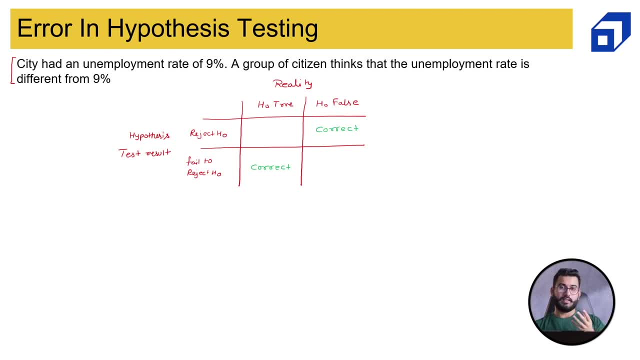 is not effective. But based on the, based on the sample, we concluded that program is effective. So this is a wrong estimation or wrong result. So this is a wrong estimation or wrong result. So this is known as the type I error, Type I error, and this is represented by alpha. So alpha, which is 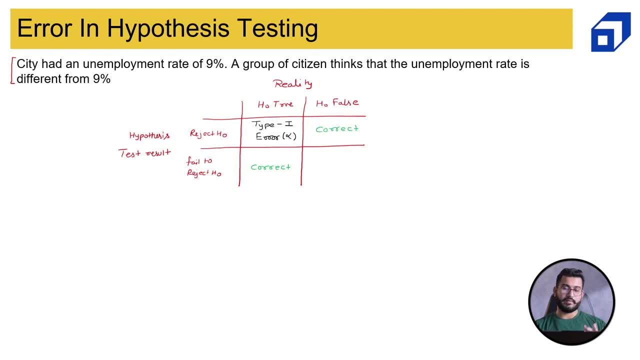 area of rejection in all the questions that we have solved is basically the probability of Type I error. What is the probability that I will commit? the Type I error is is basically given by alpha, And this is known as the type I error, And which one S is basically written as concealer. 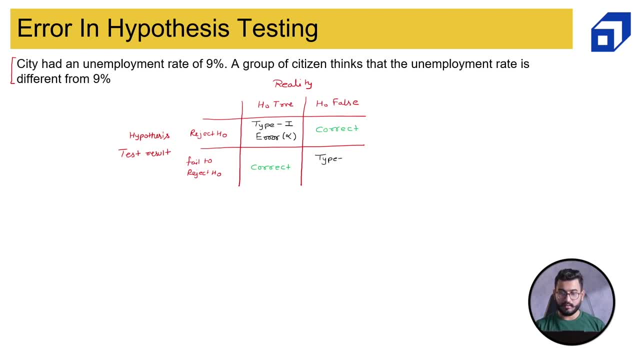 S is the response surface, S is модIf barrier, S can be the direction and is technically a response surface. And what is the EXAMPLE area of servant failure? alpha is considered when we트를 type 2 error When when your H naught was false. so in reality my null hypothesis was wrong. So 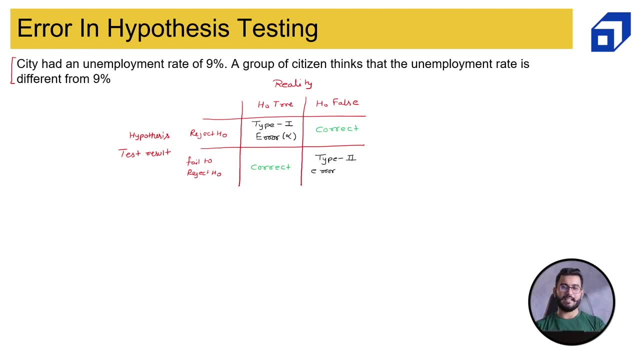 in reality, let's say: in reality, let's say: the program is not effective. So in reality, let's say: program is effective and we failed to reject H naught, So we concluded that program is not effective. That's a type 2 error. If this is confusing you a lot, don't worry. Now let's. 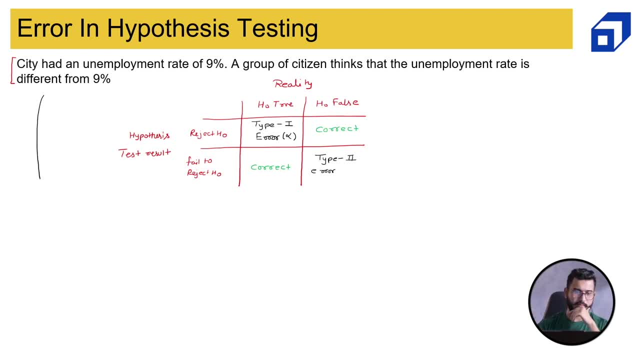 look into examples. Let's look into this example. City had an unemployment rate of 9%. So what is my null hypothesis? My null hypothesis is that the city had an unemployment rate of 9%. Group of citizens thinks that the unemployment rate is different from 9%. 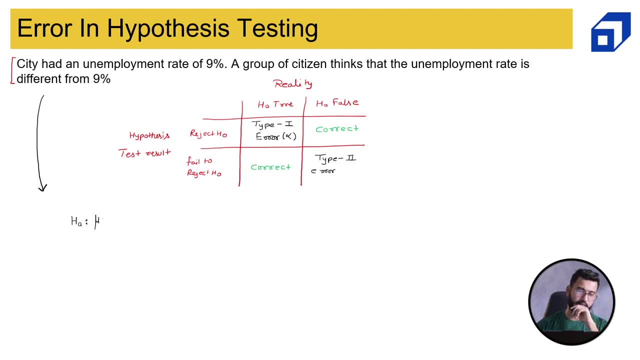 So alternate is average is not equal to 9%. Null is average is equal to 9%. This is my null and alternate hypothesis. Now if I commit type 1 error, then what will be the case? So type 1 error means H naught is true in reality, but we reject H naught. So what is the meaning of this? 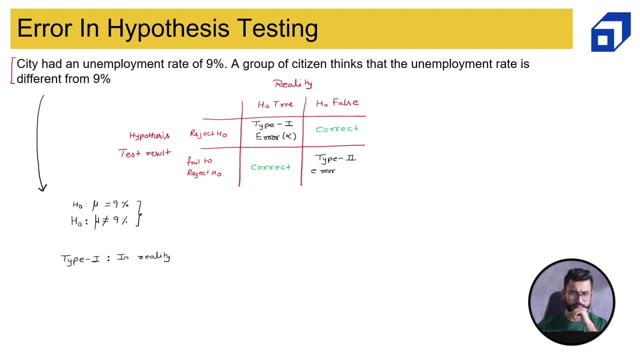 So in reality, unemployment rate was 9%, But we concluded that it's not 9%. We rejected H naught right. So in reality unemployment rate was 9%, But we concluded that it's not 9%. We rejected H naught right. 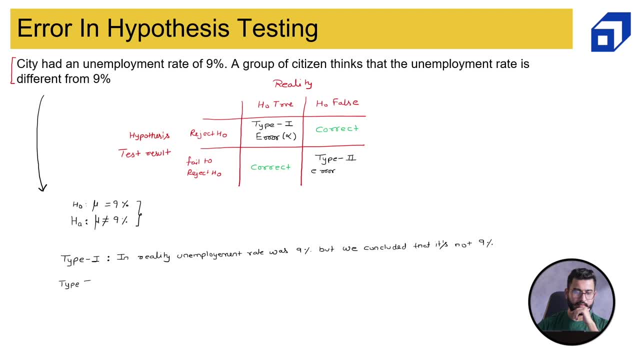 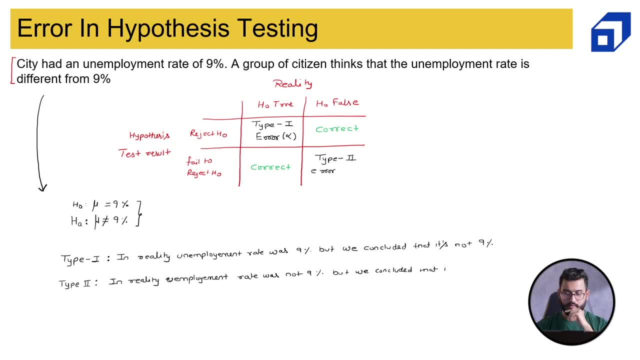 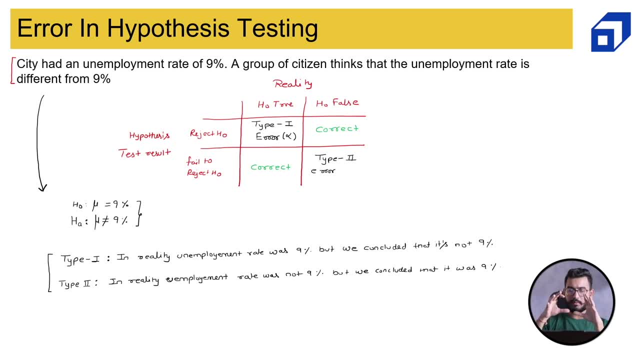 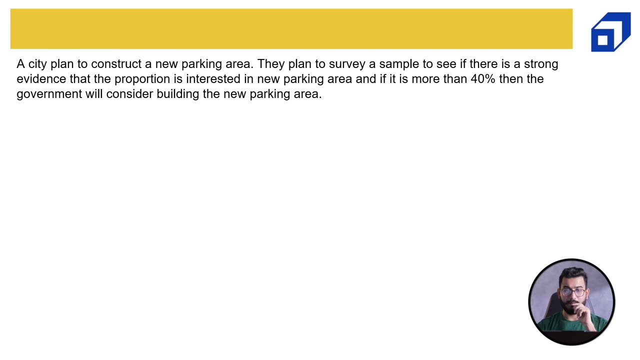 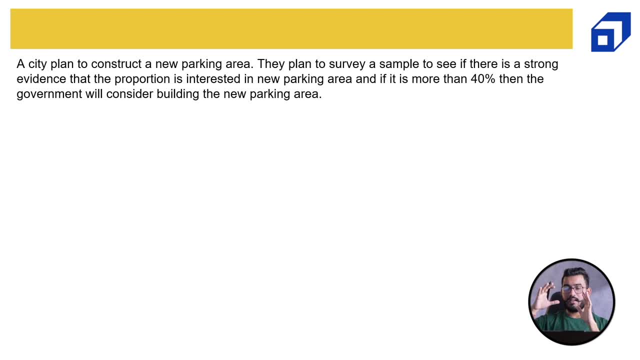 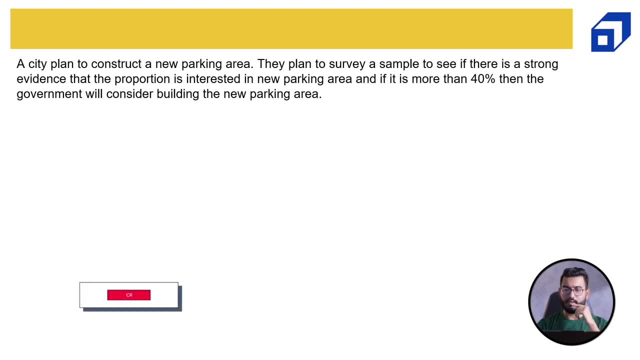 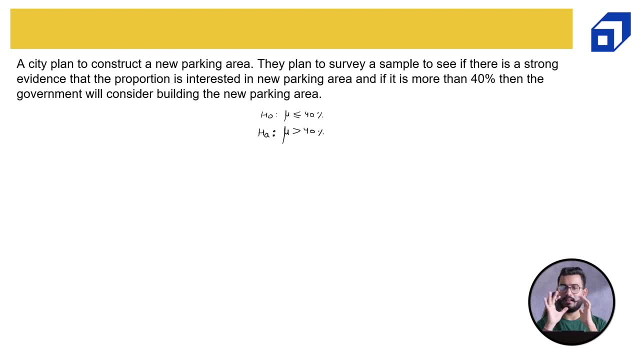 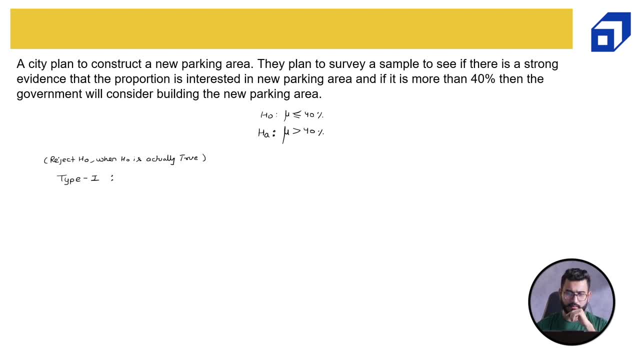 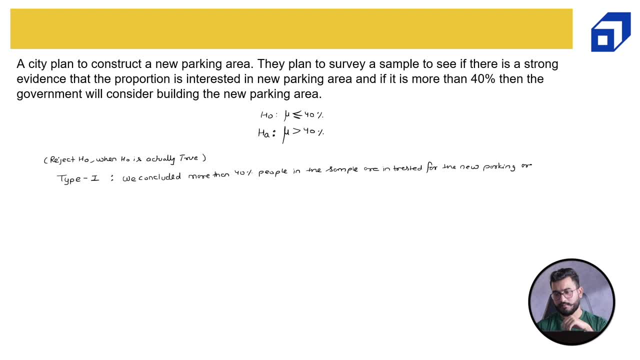 new parking area while in reality, in reality, less than 40% people were interested. so this is my type 1 error. what is type 2 error? type 2 error is basically we fail to reject H naught. fail to reject H naught when H naught was actually false. so what is our conclusion for this? we fail. 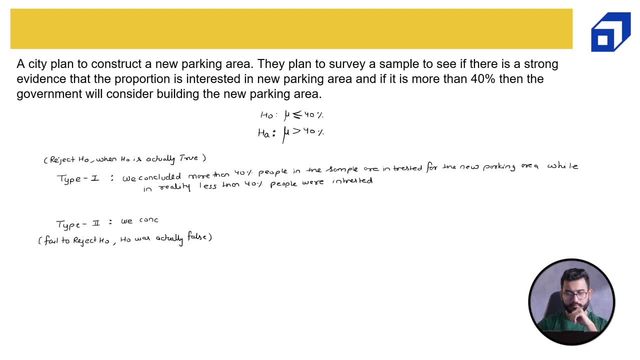 to reject H naught. so we concluded: we concluded that less than 40% people were interested in 40% people are interested for the new parking area, for the new parking area, while in reality, in reality, H naught was actually false. so, in reality, more than 40% people were interested. now, if I ask you, if, let's say, you are a government body and you 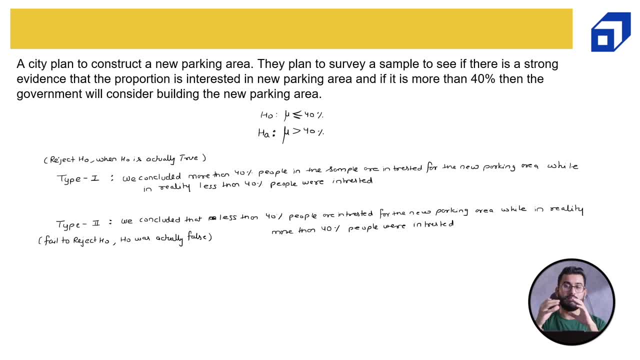 are performing this test. which particular error is more problematic for you as a government body? as a government body- type 2 error- you can see that it is problematic for us because we have concluded that less than 40% people are interested in H naught, while in reality H naught was actually. 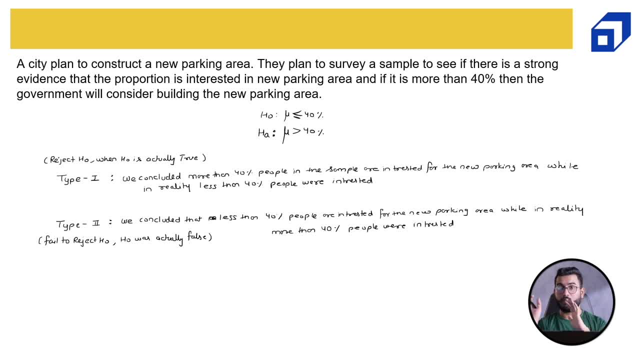 the new parking area, which basically mean we will not build the new parking area. So the consequence of the type 1 error would be: government will choose not to build the new parking area when it was actually required parking area when it was actually required. So what is the end problem for this major consequence that will happen to the government? 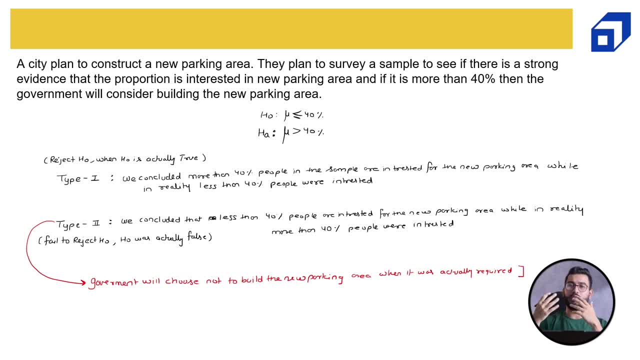 Well, people will not be happy with the government, right. So people will not be happy with the government right. What is the consequence of type 1 error? Now? the consequence of type 1 error is that the government will build a new parking area when it is not required, So government will end up. 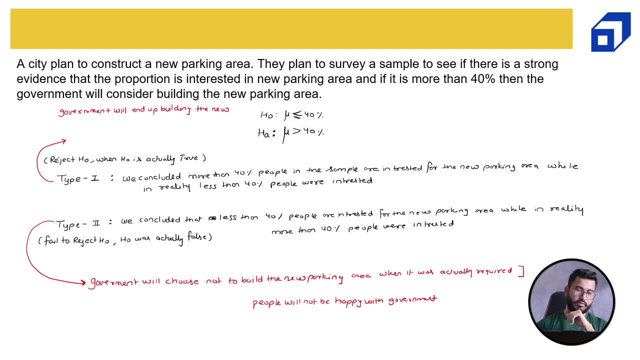 building the new parking area when it is not required, And what is the consequence that government will will be facing? Government will be investing some unnecessary amount from their budget in building up this new parking area, which will impact their budget, So impact their impact. 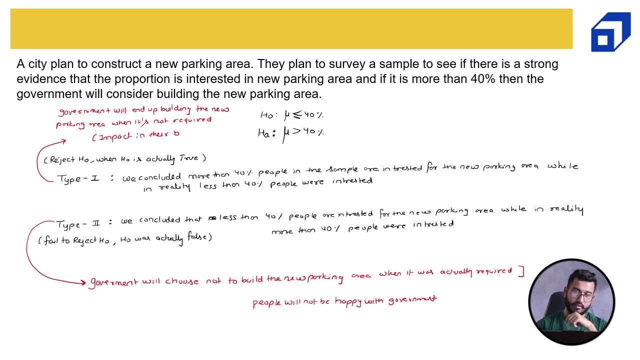 also impacts their overall impact on the city. Now, as a government body, you need to decide which particular error you want to reduce Because, see, since we are doing hypothesis testing, since we are doing estimations, we can not be free from error. 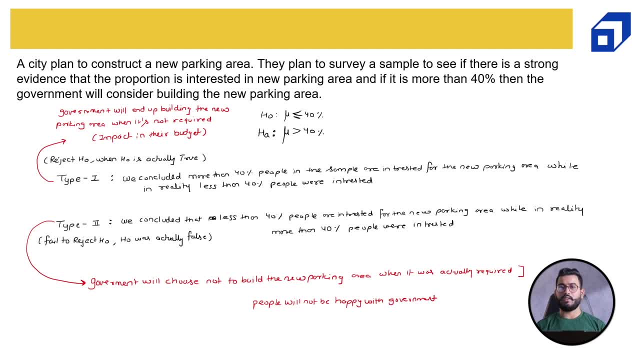 There will be some kind of error, but you have to decide which error you are ready to bear or which error is less problematic based on your particular design. problematic for you. So if you are a government body, you have to decide whether you are ready. 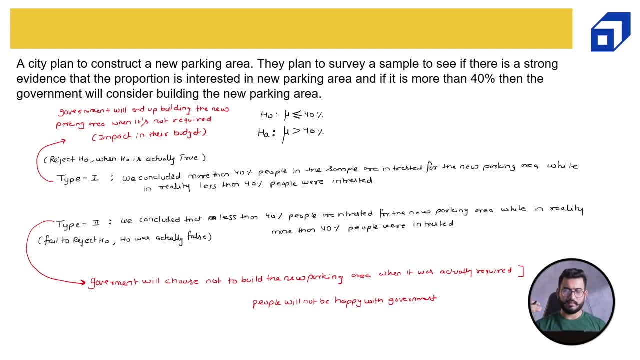 to face the impact in your budget or whether you are ready to face that people will not be happy with you. Well, if I would be a government, I would not be taking up the type 2 error on me, because I want my people to be happy, So I would do something with the budget I. 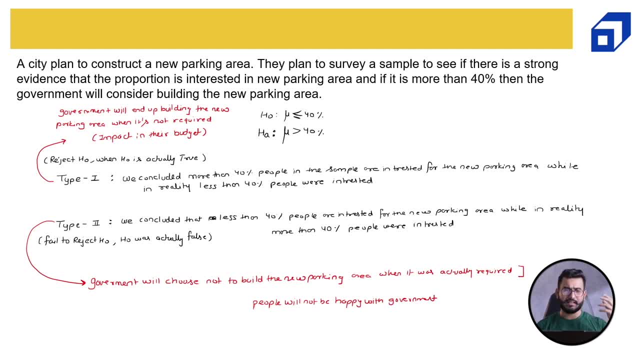 would try to maybe cancel some ongoing projects or maybe cancel some new projects, But I don't want my people to be unhappy with the government. Right, Let's take one more example to understand how we can adjust the alpha, because we know the alpha value. Right, We can do the alpha. 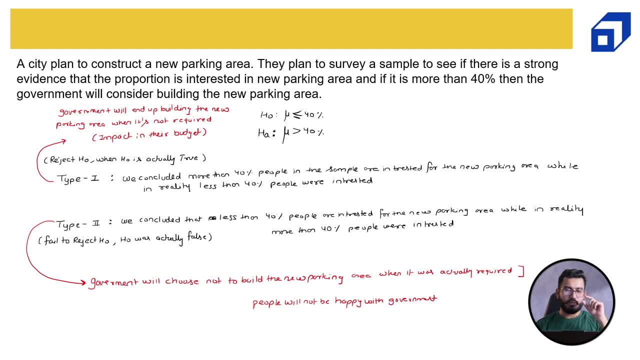 value. We can increase or decrease the alpha value to increase the chances of type 1 error and reduce the chances of type 2 error. So you can- you can assume that if I'm having a number line then if I want type 1 error to be high. 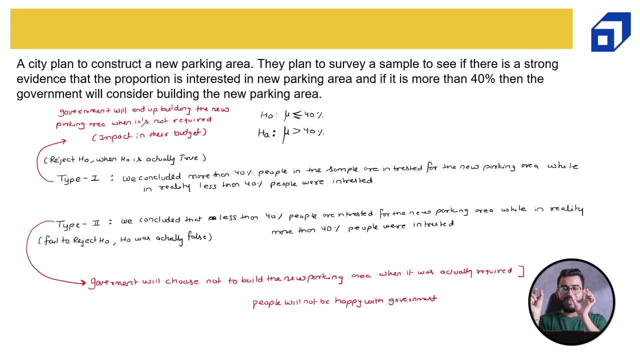 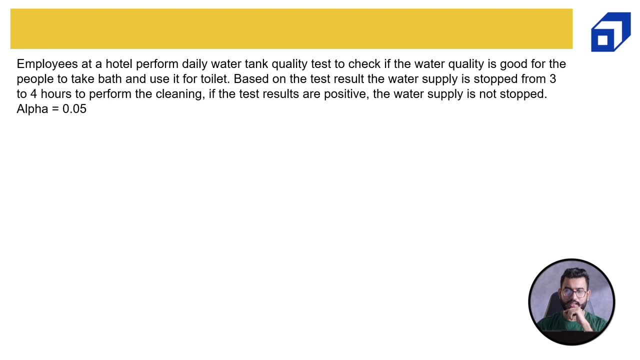 I can increase the value of alpha and it will eventually reduce the type 2 error, the chances of type 2 error. It is like a number line, You can shift it. Let's see one last example. So employee at a hotel performed daily water tank quality test. Okay, To check if the water. 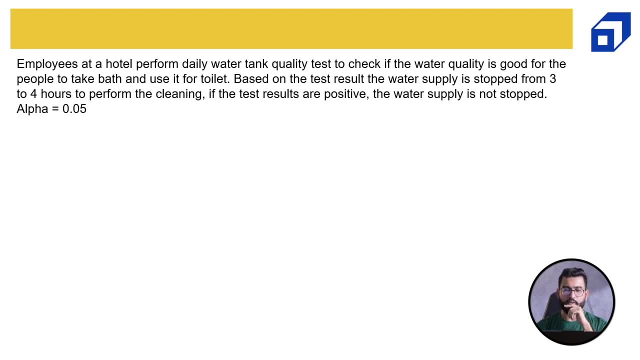 quality is good for the people to take bath and use it for toilet. Based on the test result, it stopped for three or four hours for the to perform the cleaning process or for the cleaning process. If the test results are positive, the water supply is not stopped. 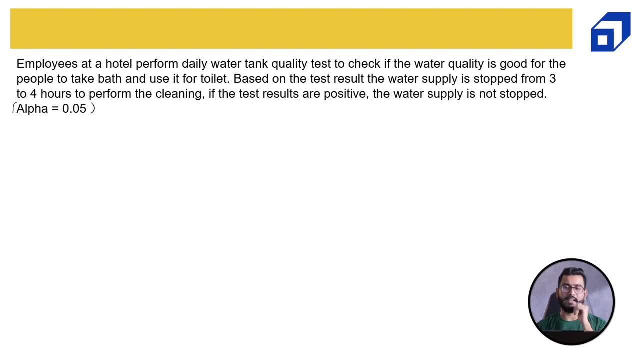 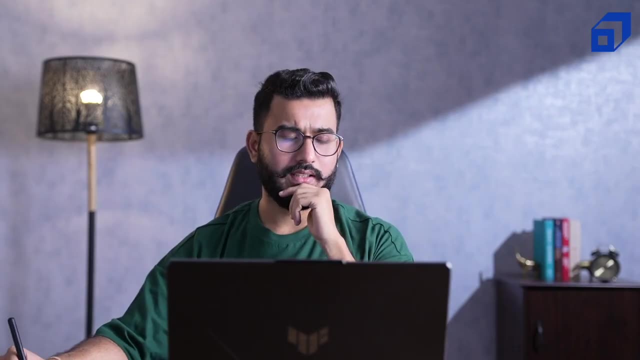 Test at alpha of 0.05.. And this question: we are provided with the alpha of 0.05.. What is the alternate hypothesis? Let's you guys can pause the video, think about it and then you can maybe comment on the chat section. So now let's try to understand this question. 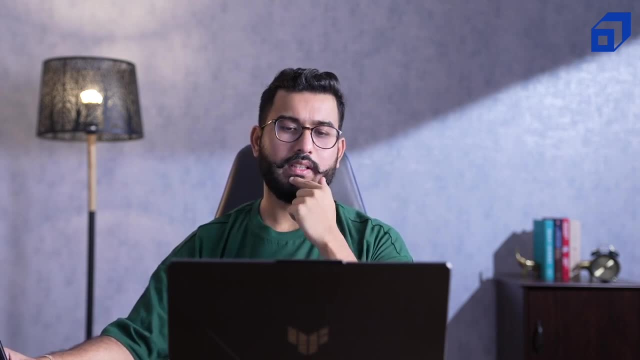 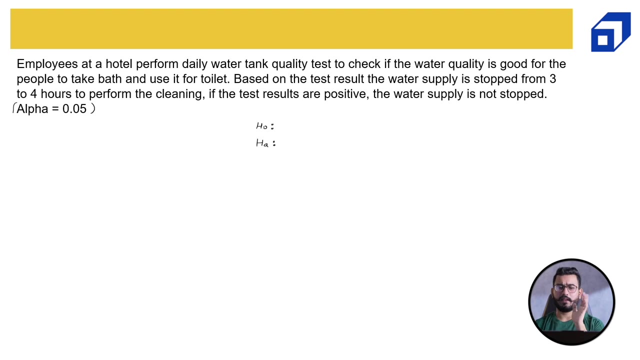 and I hope you guys would have already guessed or what is going to be the alternate and the null, null hypothesis. My null hypothesis would be that the water quality is fine, So water quality is fine, It's good, Fine or good. My null would be sorry. my alternate would: 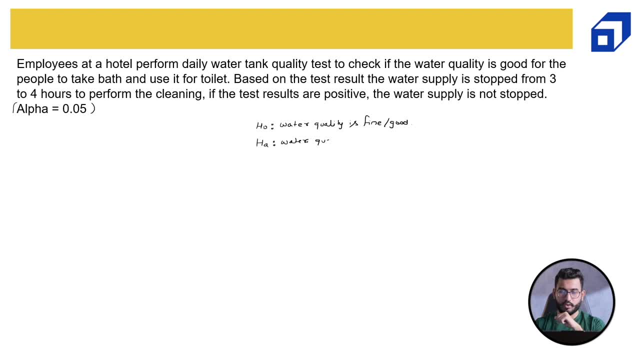 be. water quality is not good Right Now. what is the type 1 error? The type 1 error is basically that we reject H naught when it was. so let's write it down: We reject H naught when H naught was actually. 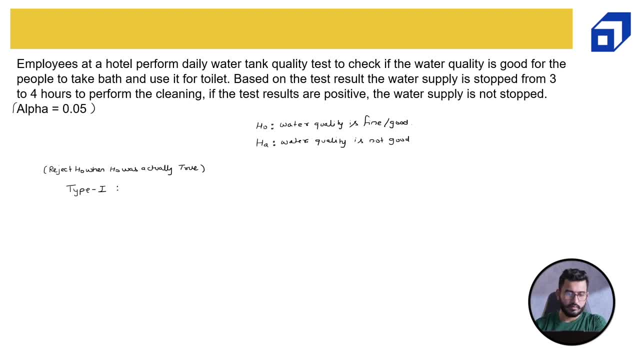 true in reality, Right? So what is the meaning of this? We reject H naught. so we rejected that water quality is fine when H naught was actually true. So what will happen? So we will close the close the water supply. We'll close the water supply when it was not required. 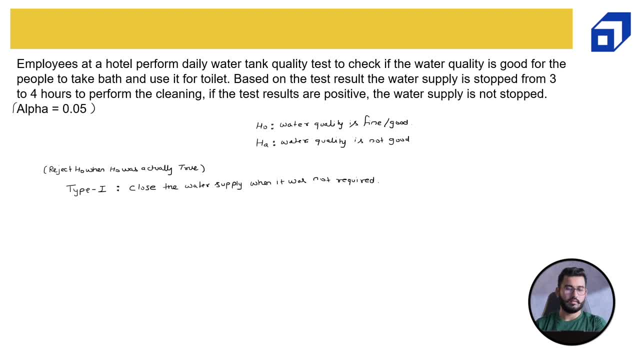 Okay, Yes, right. What is type II error? Type II error is we fail to reject H0 when H0 was actually false. So what will be the consequence for this? So we fail to reject H0.. So which basically means we concluded that the water quality is good when H0 was actually false. So that 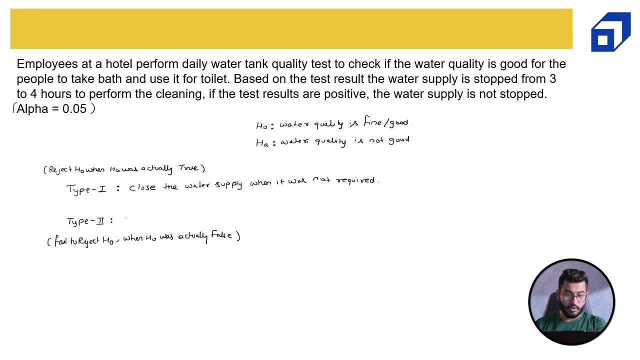 basically means we will not close the pool, or we will not close the water supply, or maybe we let's not write. we let's write: the water supply was not stopped. Water supply was not stopped when the water quality was bad. Water quality was bad or not good. Now, 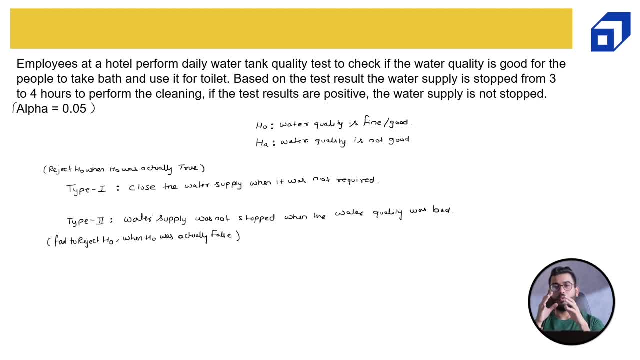 which one is more problematic? So, if you are a hotel owner, then which one is more problematic for you? So, if I go with the type I error, we have to close the water supply when it was not required, which basically means we will clean, or your. 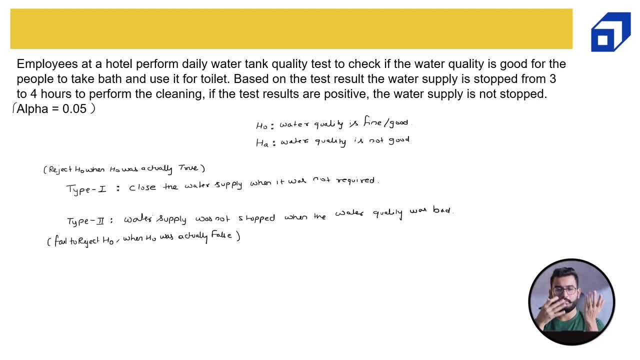 your employee or the, maybe your the- the people who clean the tank. they will perform the cleaning process, but there will be a stoppage of water supply for three to four hour. maybe this is not a big problem because maybe you can decide the window of afternoon and then the water cup to supply can be stopped for. 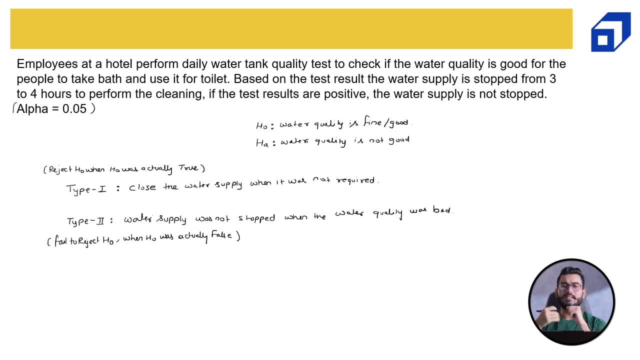 three to four hour and it will not impact the the service right. so when you have to stop the water supply, you have to also think that it may impact the service, but it will eventually not going to harm you in a very large scale because you can choose the window in the afternoon when most of the people are. 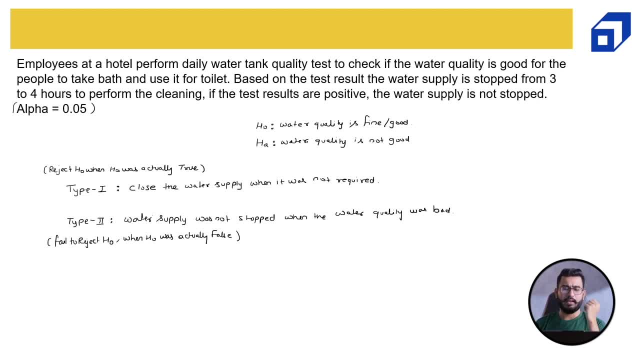 either out of the hotel or out of the hotel, or maybe involved in some other activities. they would not be using the the bathroom, right? what is the consequence of type 2 error? water supply was not stopped when the water quality was bad. now this is a more problematic. 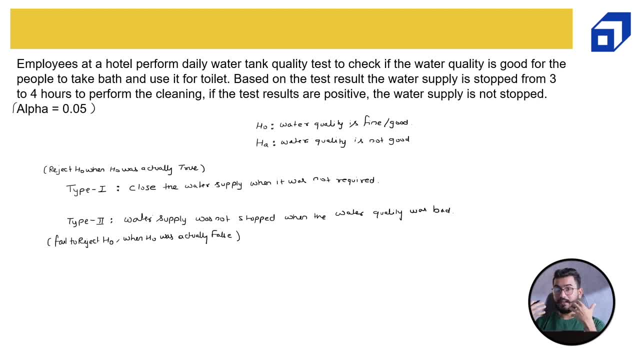 condition. let's say somebody is having a sensitive skin and that person is staying in your hotel. and if you do not clean the water- and let's say that person has taken bath in the contaminated water- the person can attract some kind of disease which can eventually land your. 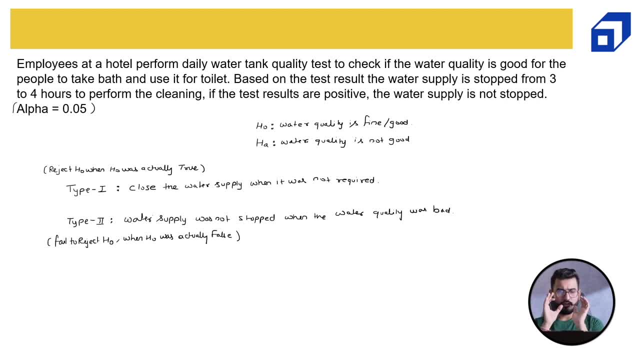 hotel into a big problem, right? so type 2 error is definitely very problematic for you. now. we have already learned that alpha is the probability of type 1 error. so alpha is the probability of committing type 1 error for an error. and if you increase the probability of committing, 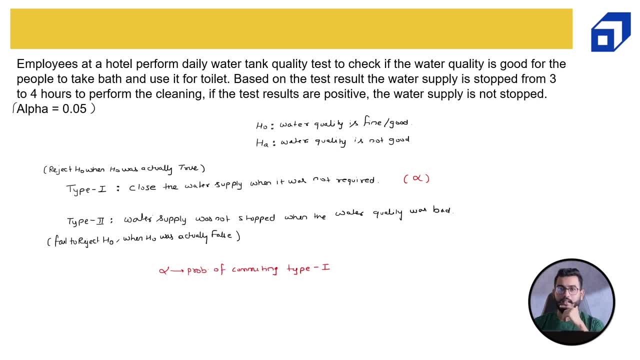 type 1 error for other error, there are more chances that I will commit type 1 error. so let's say that type 1 error, but it will reduce the chances of type 2 error. so right now my alpha value is 0.05. if I increase this to 0.10, then what?